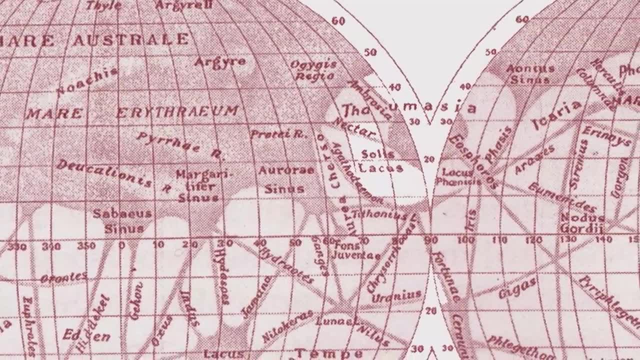 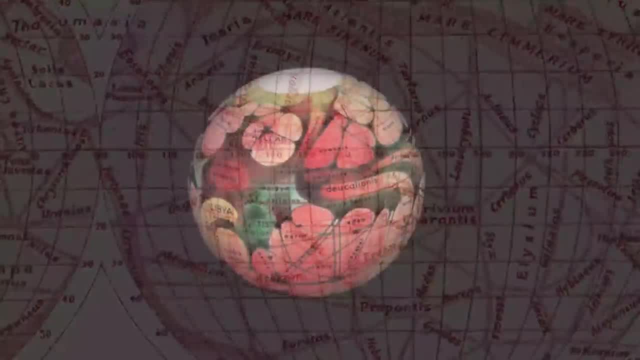 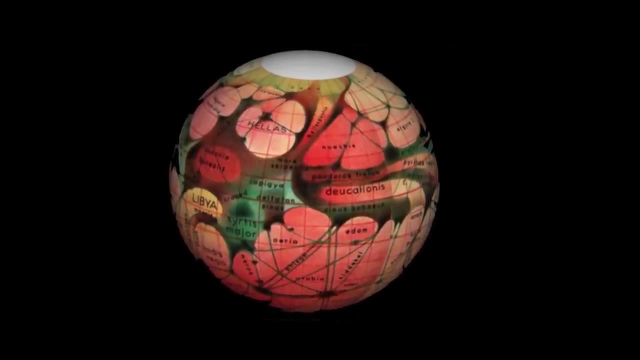 Giovanni Schiaparelli made what he thought was the most accurate map of Mars yet drawn On it, he showed canals. In the early 20th century American astronomer Percival Lowell was convinced the canals were signs of a civilization existing on the Red. 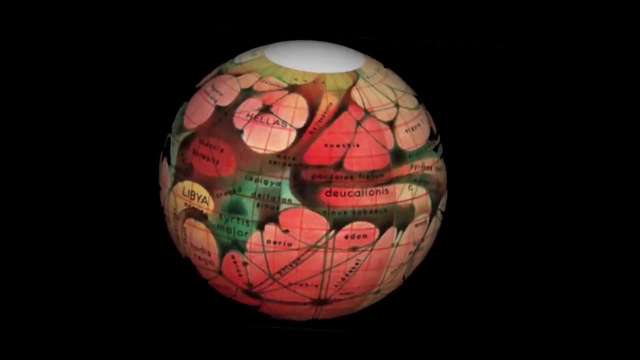 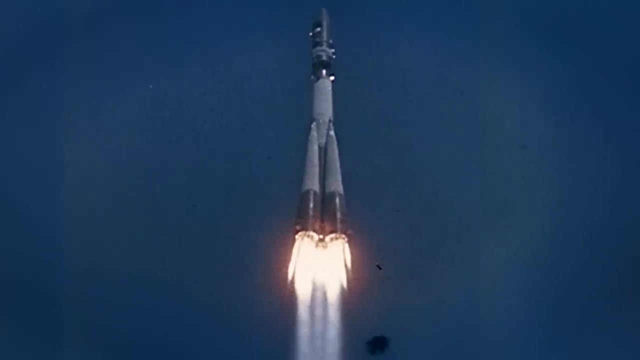 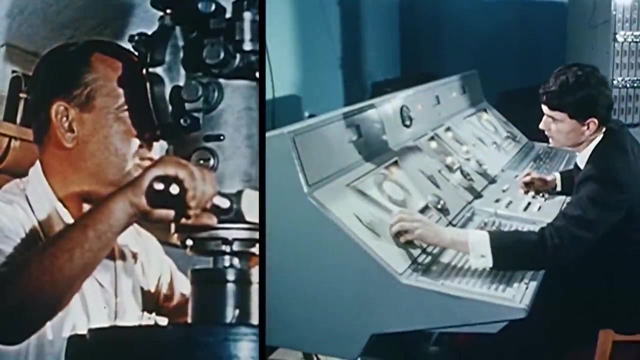 Planet. So began the search for life on Mars. In 1962, the Soviet Union sent the first probe, the Mars M1, on a flyby mission. It was an audacious project And it failed, the first of many failures by both the Soviet Union. 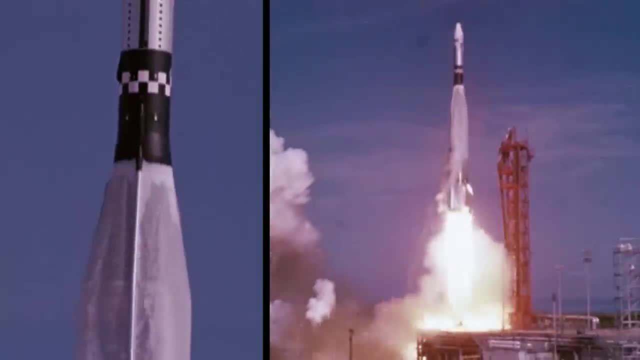 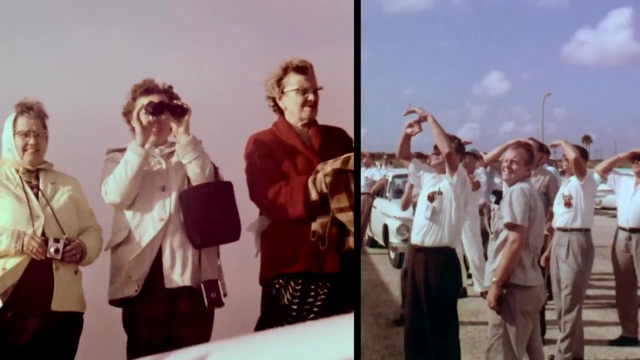 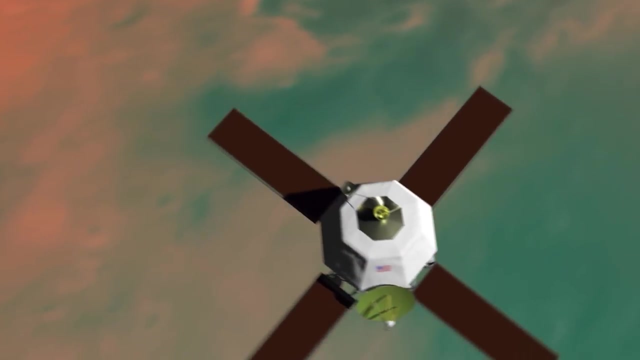 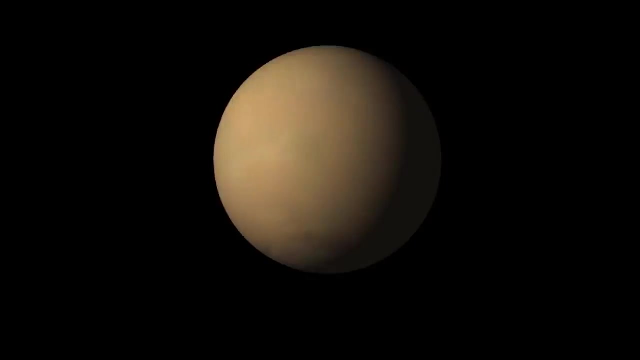 and the United States Cold War rivalry provided the motivation for these early missions. In 1971, NASA sent Mariner 9 to Mars. It was the first probe to orbit another planet, But scientists discovered that Mars was enveloped in a planetary dust storm. On-orbit photography revealed little more than a red cloud. 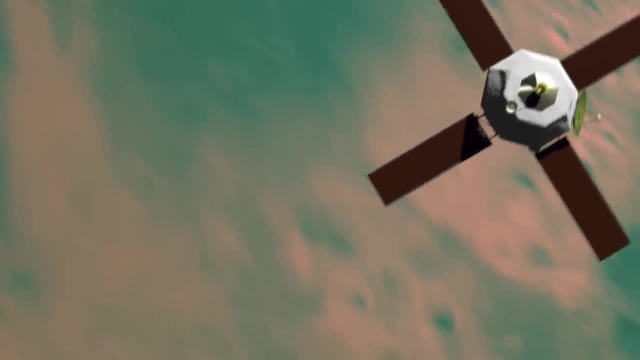 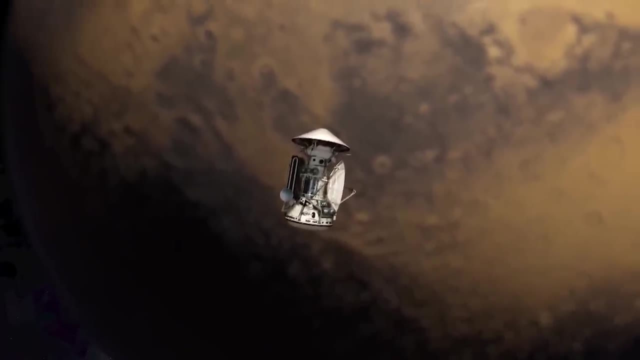 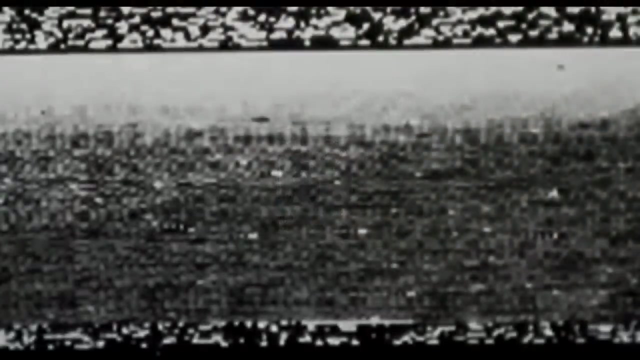 Soon, Mariner 9 was joined by two Soviet orbiters, both equipped with landers. The Mars 2 lander crashed, but the Mars 3 lander made it to the surface. It returned one garbled image and then stopped functioning. 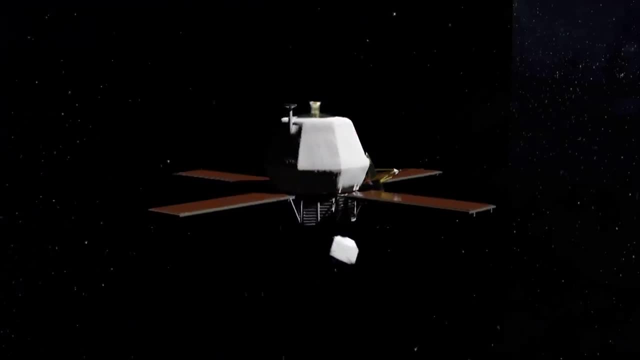 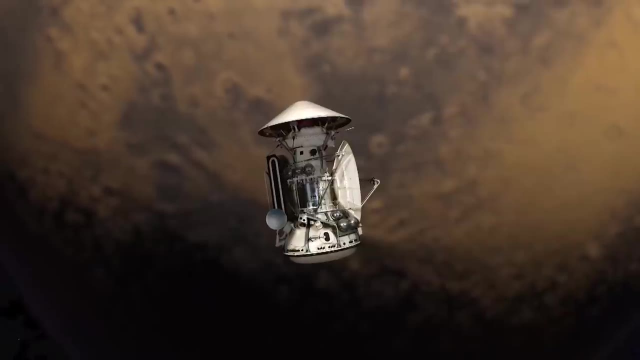 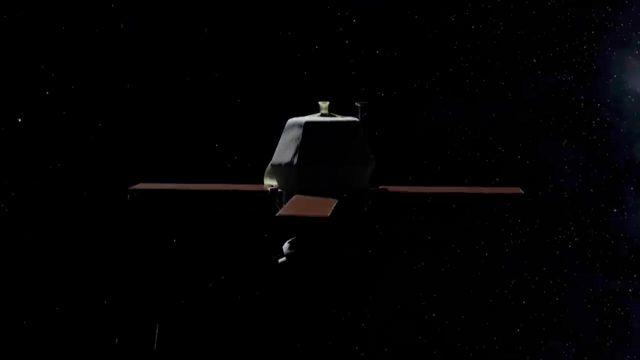 Mars now had three orbiting spacecraft, all looking at a dusty, featureless planet. The two Soviet probes were identical, but the American probe had one key design difference: While the Soviet orbiters began photographing the planet following predetermined schedules, NASA were able to command Mariner 9 to wait, In hopes that it would make it to Mars. they 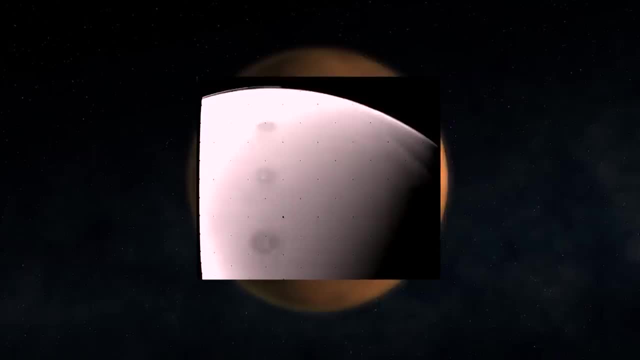 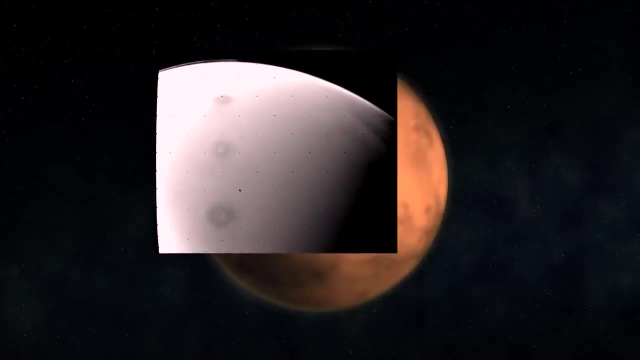 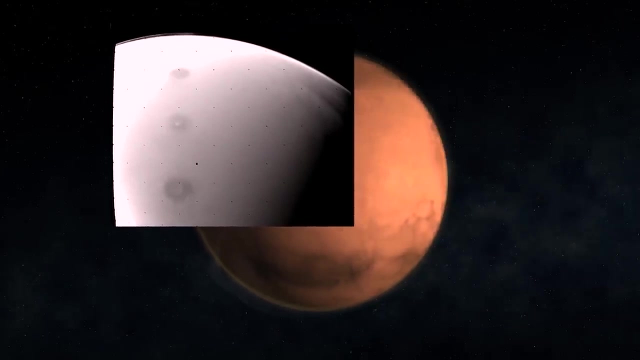 hoped that the dust would eventually settle. It took months for the atmosphere to clear, but when it did, Mariner 9 saw three craters protruding above the dust. They were the tops of giant volcanoes on what was called the Tharsis Plateau. 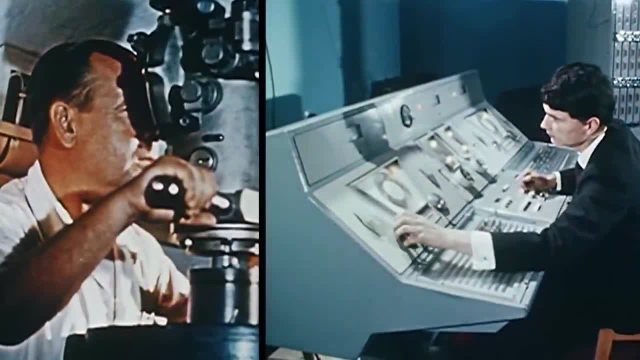 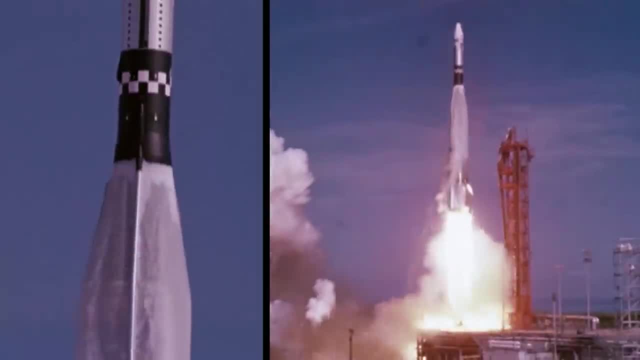 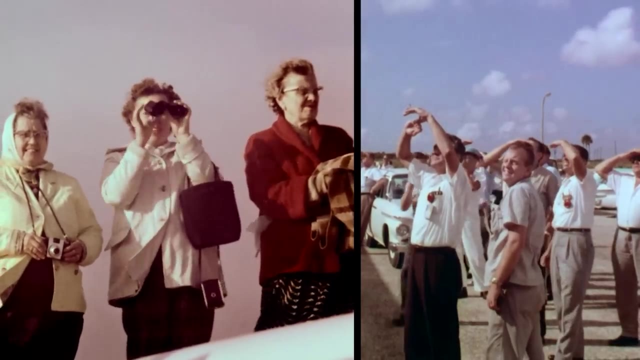 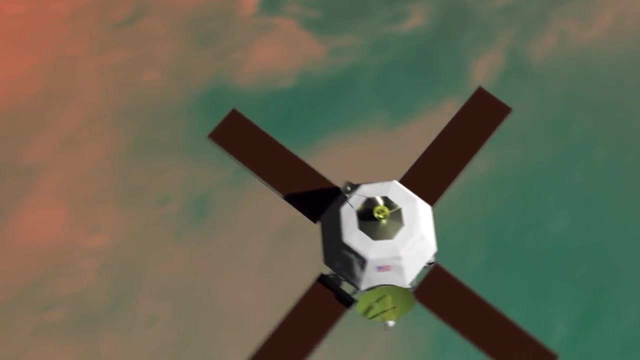 audacious project And it failed, the first of many failures by both the Soviet Union and the United States. Cold War rivalry provided the motivation for these early missions. In 1971, NASA sent Mariner 9 to Mars. It was the first probe to orbit another planet, But scientists discovered that Mars was enveloped. 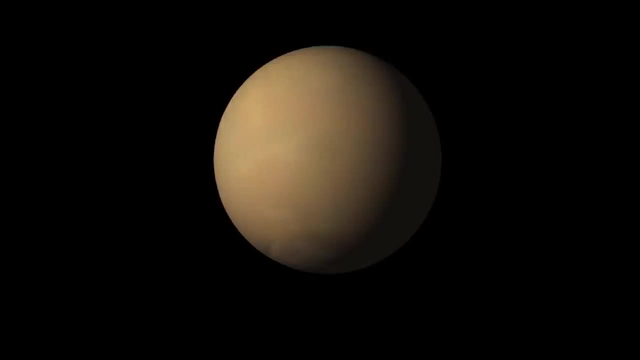 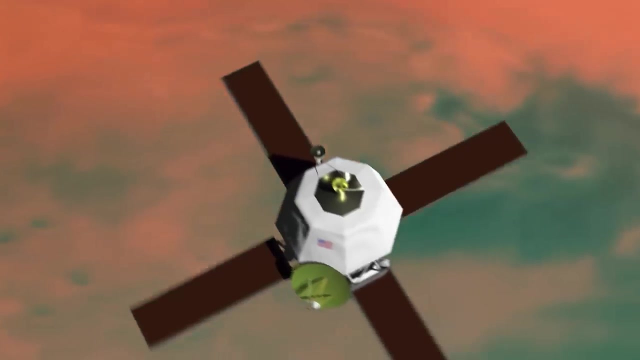 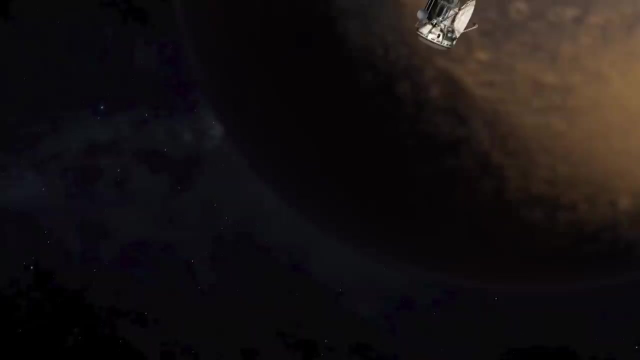 in a planetary dust storm. On-orbit photography revealed little more than a red cloud. Soon Mariner 9 was joined by two Soviet orbiters, both equipped with landers. The Mars 2 lander crashed, but the Mars 3 lander made it to the surface. 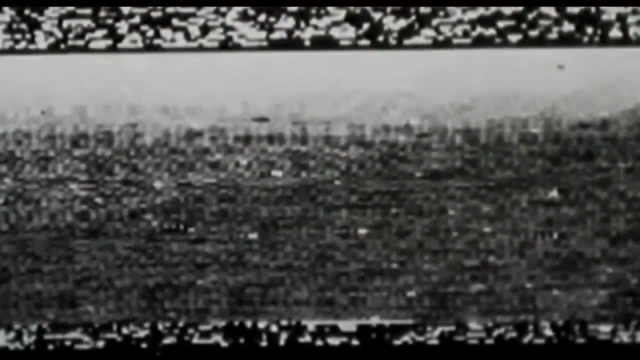 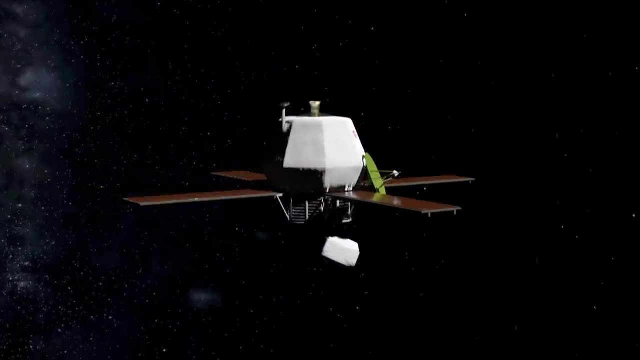 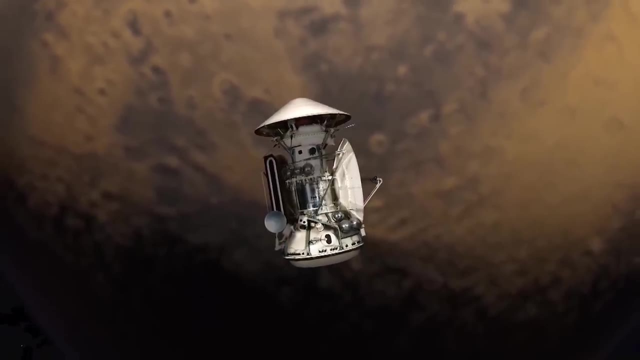 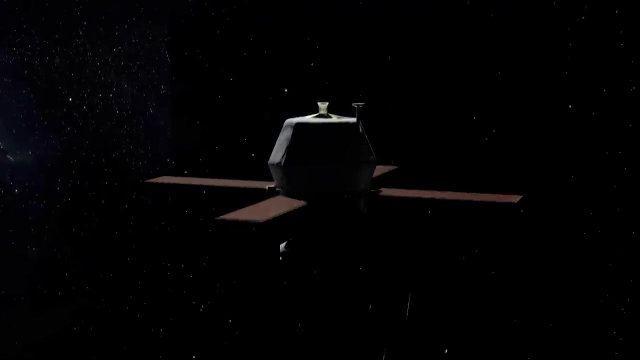 It returned one garbled image and then stopped functioning. Mars now had three orbiting spacecraft, all looking at a dusty, featureless planet. The two Soviet probes were identical, but the American probe had one key design difference, While the Soviet orbiters began photographing the planet following predetermined schedules. 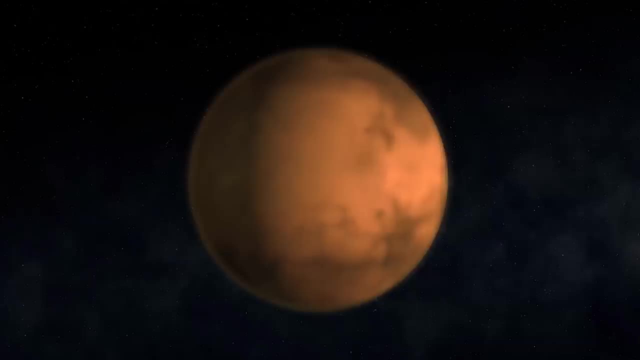 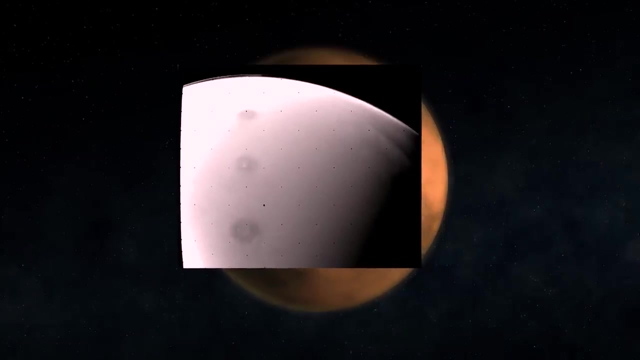 NASA were able to command Mariner 9 to wait, In hopes that it would make it to Mars. they hoped that the dust would eventually settle. It took months for the atmosphere to clear, but when it did, Mariner 9 saw three craters. 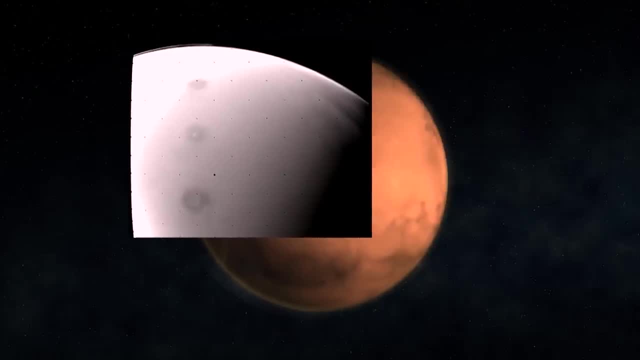 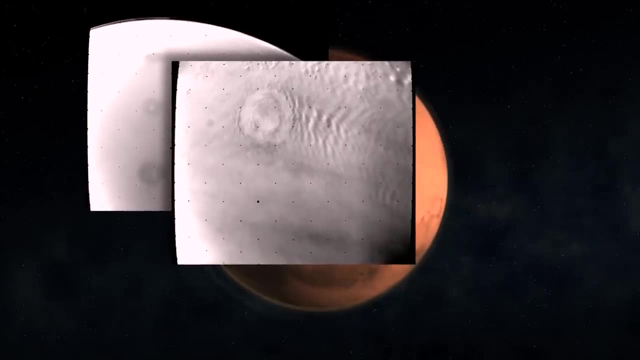 protruding above the dust. They were the tops of giant volcanoes on what was called the Tharsis Plateau. Soon, more complex geological features began to emerge. In places the surface was cratered, suggesting the tectonic forces that constantly renewed the surface. The surface was crated. 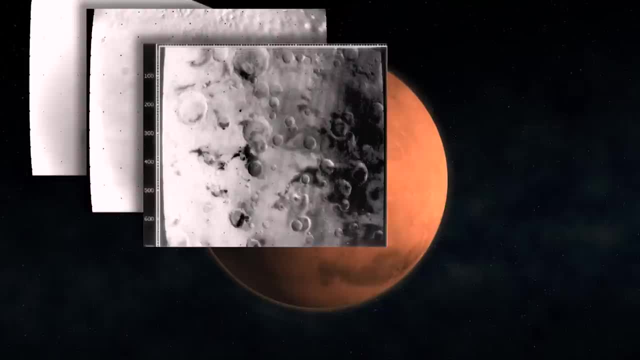 suggesting the tectonic forces that constantly renewed the surface. The surface was cratered, suggesting the tectonic forces that constantly renewed the surface. the Earth's surface were absent on Mars, Volcanic activity that built the solar system's largest volcanoes. 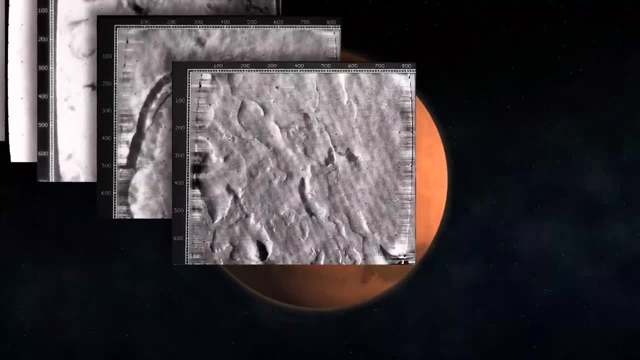 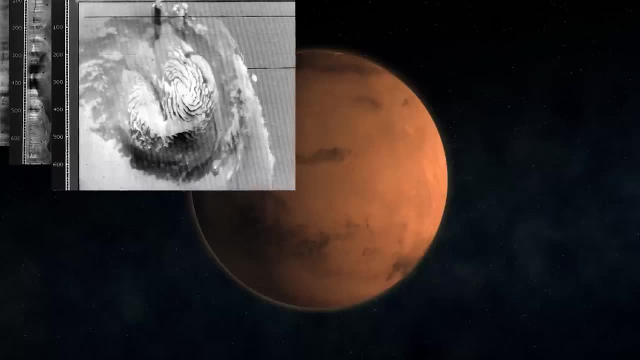 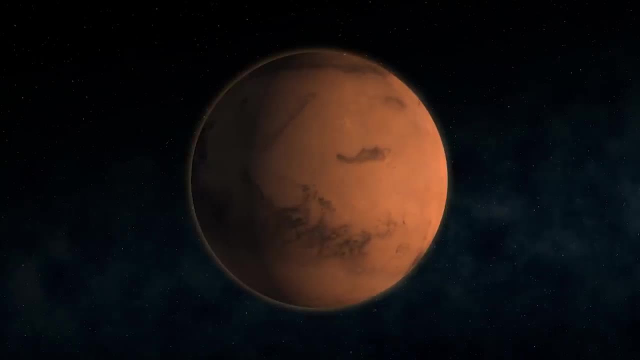 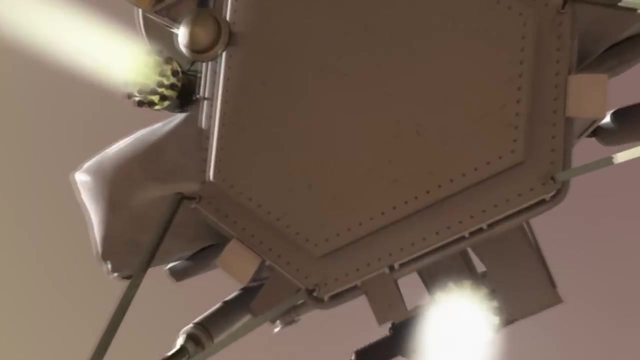 had stopped billions of years ago. This enabled NASA scientists to compile an accurate global map of Mars and to decide upon landing sites for the Viking probes that followed in 1976. Viking 1 and 2 were identical orbiters with landers that both made successful landings on the surface. 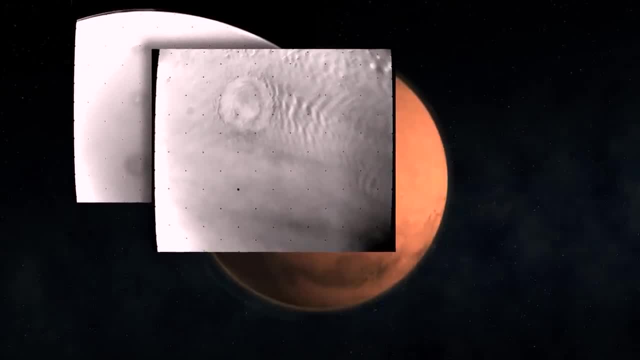 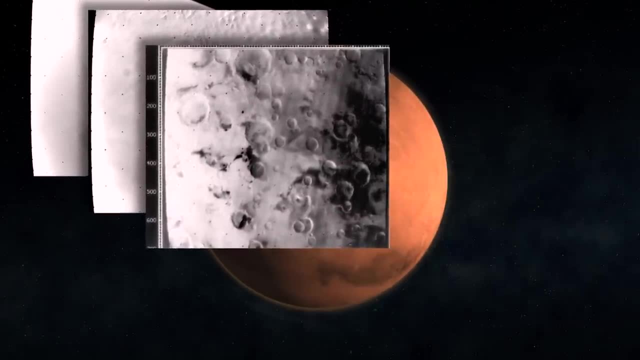 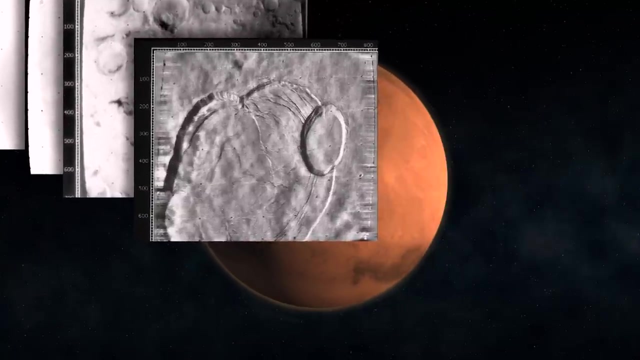 Soon, more complex geological features began to emerge. In places, the surface was cratered, suggesting the tectonic forces that constantly renew the Earth's surface were absent. on Mars, Volcanic activity that built the solar system's largest volcanoes had stopped billions of years ago. 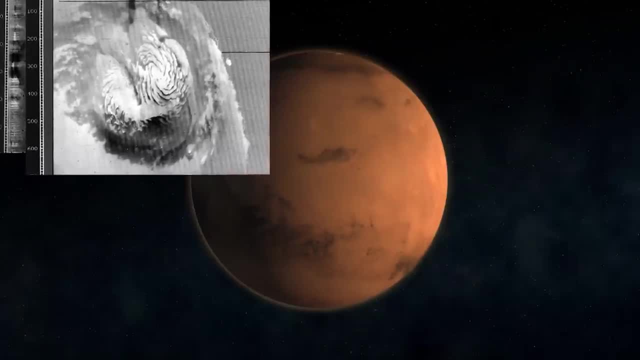 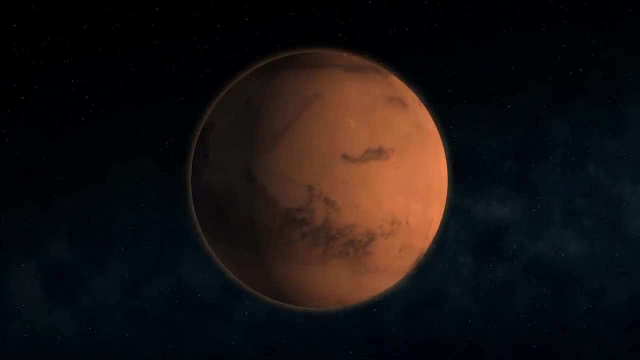 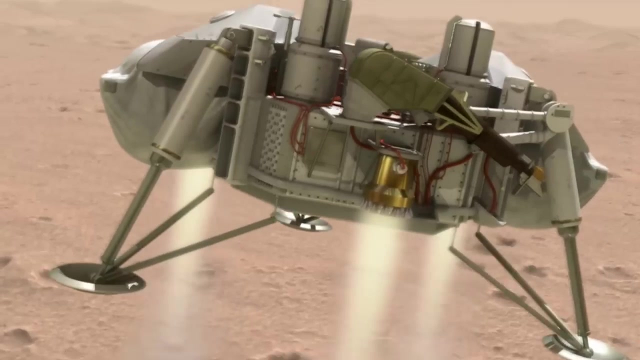 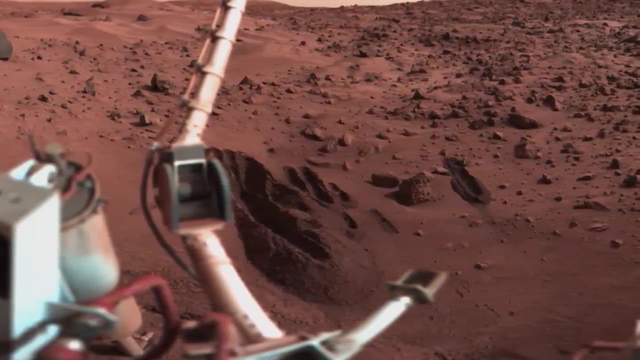 This enabled NASA scientists to compile an accurate global map of Mars and to decide upon landing sites for the Viking probes that followed in 1976.. Viking 1 and 2 were identical orbiters with landers that both made successful landings on the surface. Both returned pictures of the Martian landscape. The primary objective. 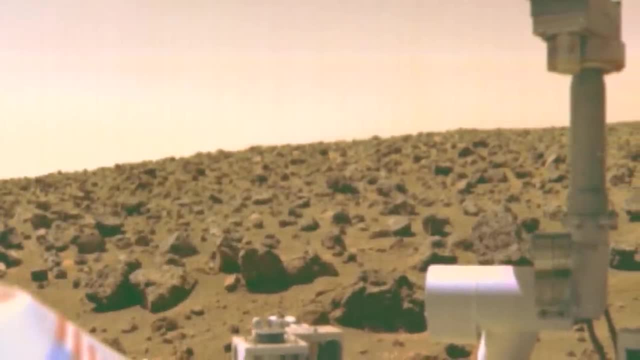 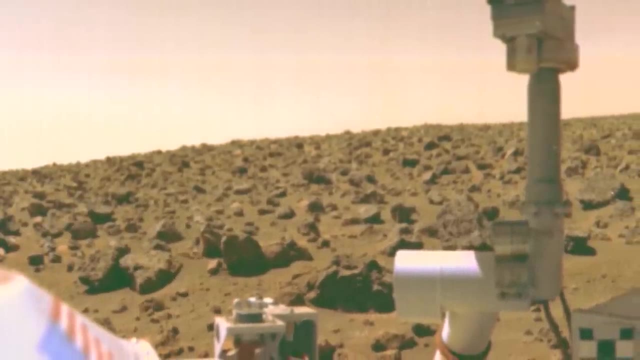 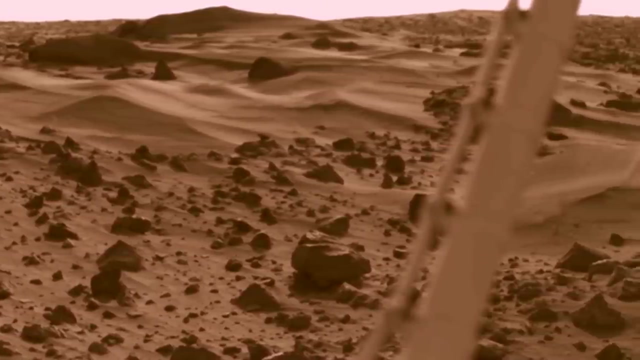 of the Viking program was to find signatures of life, but researchers now feel the three experiments tasked with carrying out the analysis had limitations, As researchers on Earth began. When the Earth began looking for traces of life in extreme environments, they began to rethink where life on Mars might survive. 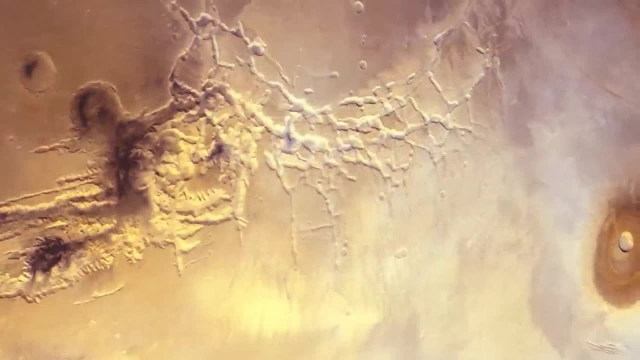 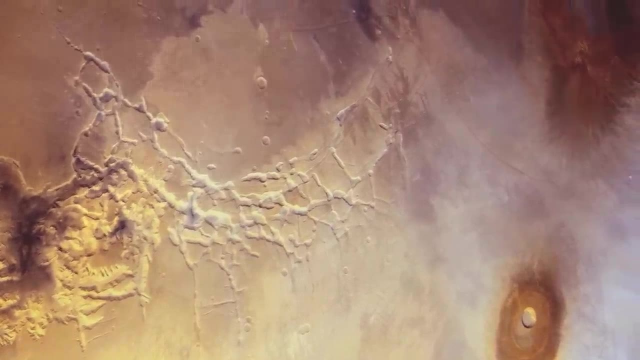 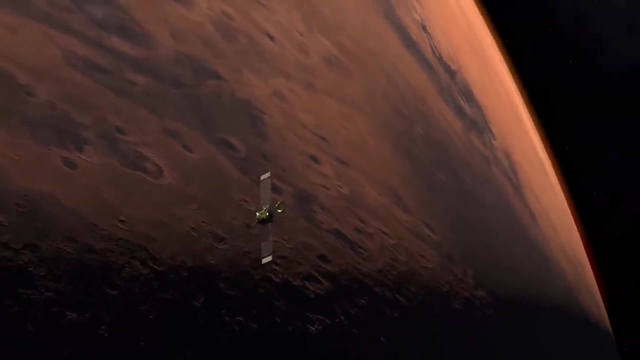 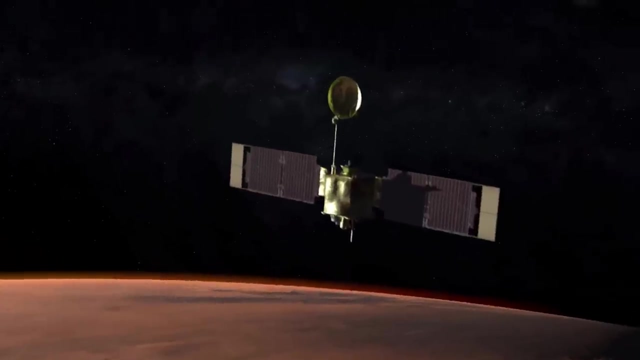 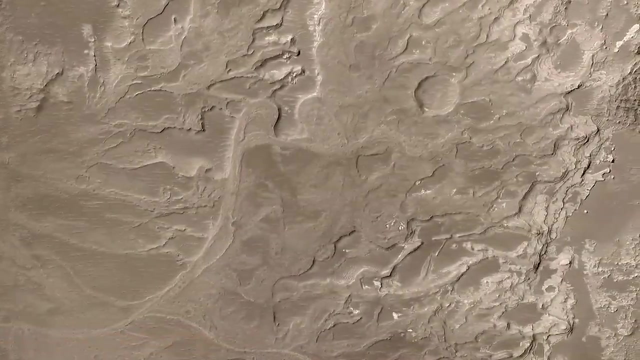 Yet the consensus at the time was that Mars was sterile and the idea of life on Mars died. After a 20-year hiatus in Mars research, the Global Surveyor went into orbit in 1996.. The pictures it relayed back were clearer than anything yet seen from the Red Planet. 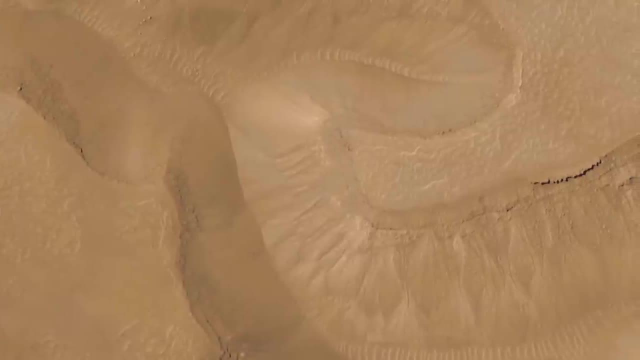 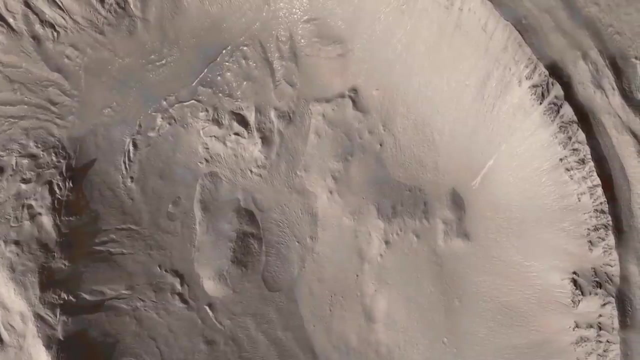 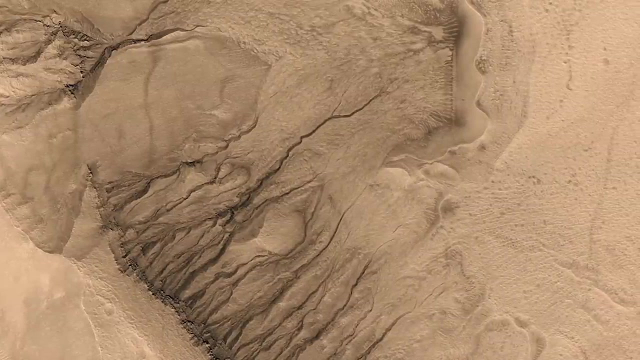 Although most Mars orbiters had been tasked with mapping the planet's surface, this was different. The high-resolution images that the Mars Global Surveyor sent back revealed rivers and even River Delta, but the occasional impact crater suggested that nothing has flowed in these systems for billions of years. In July 1997, another probe arrived. The Mars Pathfinder was one of a new breed of missions being pushed by NASA's new administrator under the guiding philosophy of faster, better, cheaper. The idea was to cut development times, cut budgets and, although the risk of failure would rise, 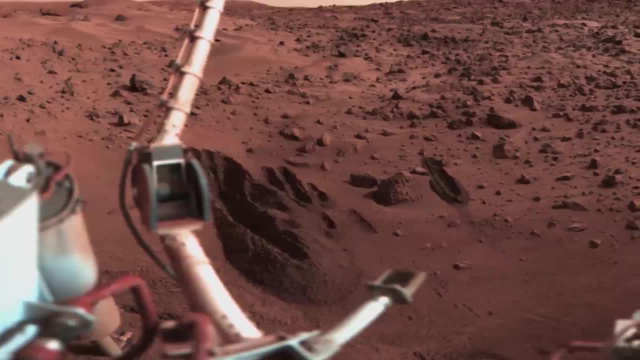 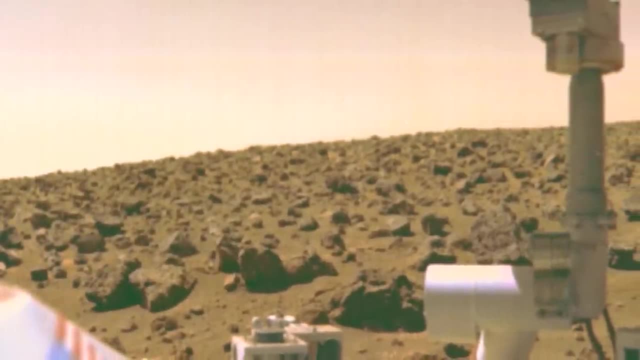 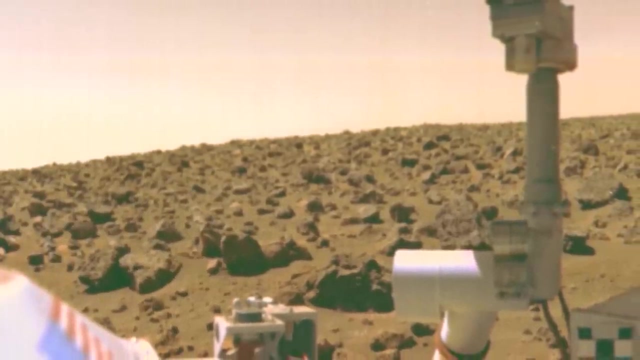 Both returned pictures of the Martian landscape. The primary objective of the Viking programme was to find signatures of life, But researchers now feel the three experiments tasked with carrying out the analysis had limitations, As researchers on Earth began looking for traces of life in Earth. 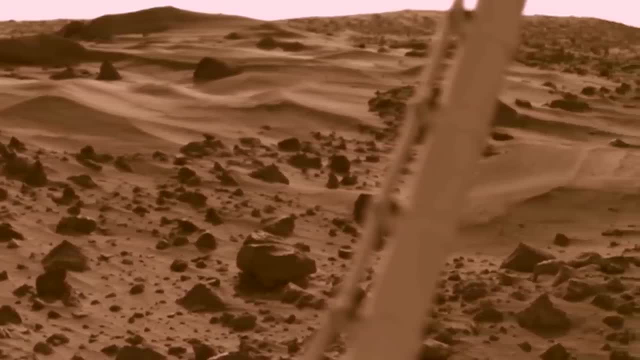 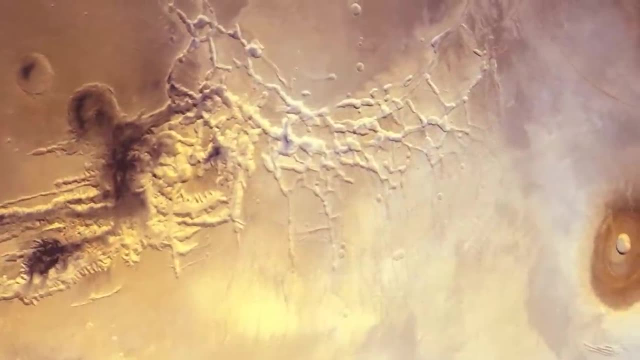 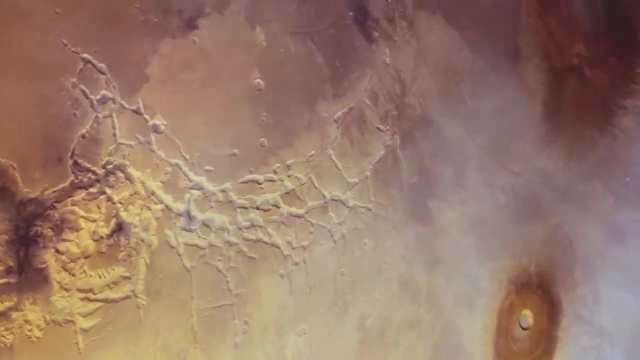 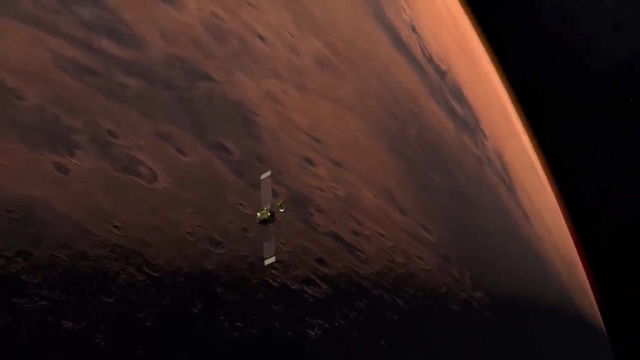 and in extreme environments, they began to rethink where life on Mars might survive. Yet the consensus at the time was that Mars was sterile and the idea of life on Mars died. After a 20-year hiatus in Mars research, Mars Global Surveyor went into orbit in 1996.. 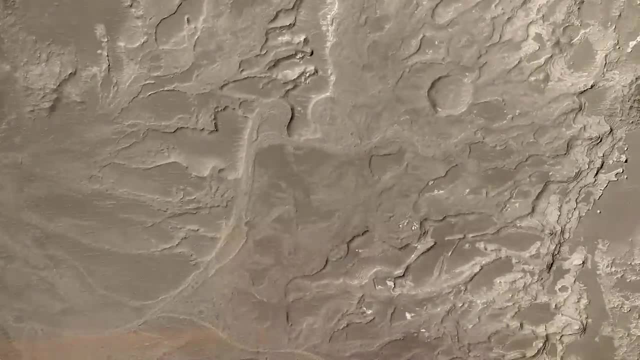 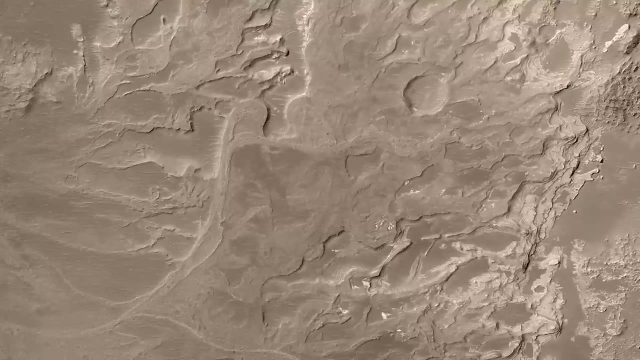 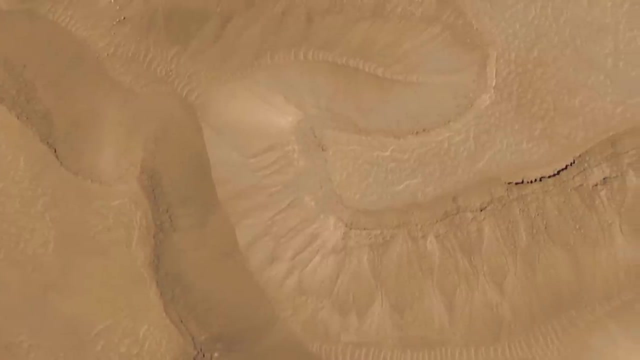 The pictures it relayed back were clearer than anything yet seen from the red planet. Although most Mars orbiters had been tasked with mapping the planet's surface, this was different. The high-resolution images that the Mars Global Surveyor sent back revealed rivers and even river deltas. 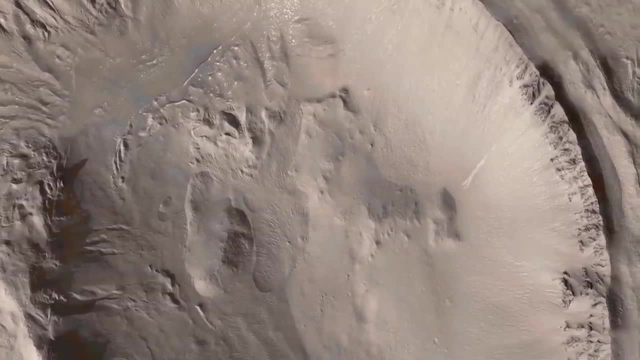 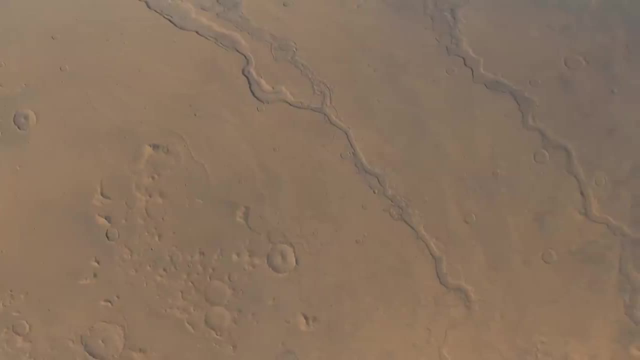 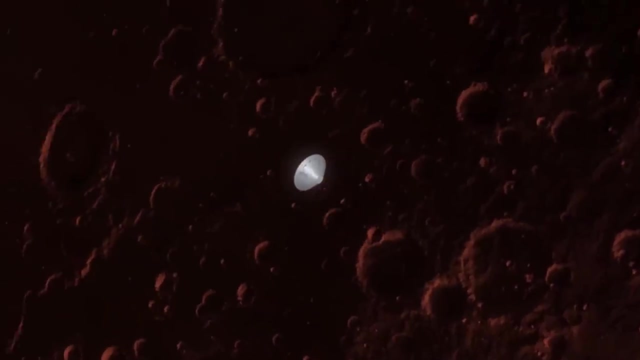 but the occasional impact crater suggested that nothing has flowed in these systems since the beginning of the 20th century. NASA has suggested that nothing has flowed in these systems for billions of years. In July 1997, another probe arrived. The Mars Pathfinder was one of a new breed of missions. 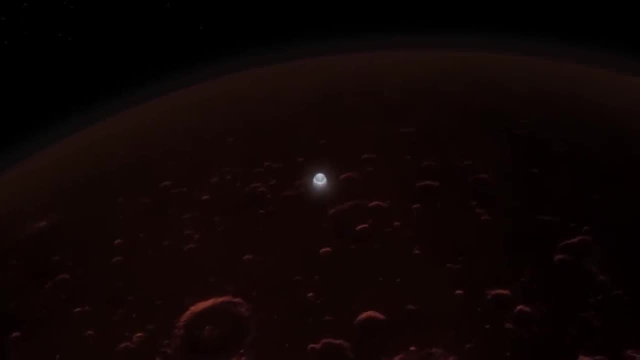 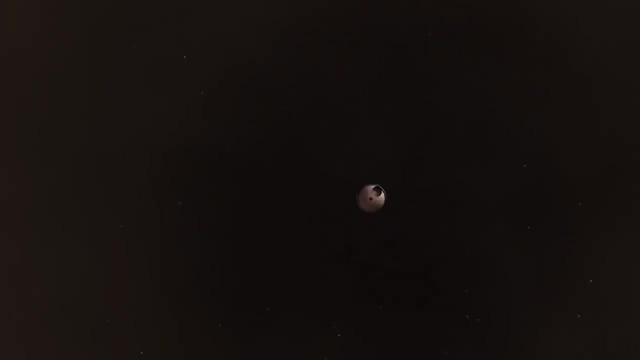 being pushed by NASA's new administrator under the guiding philosophy of faster, better, cheaper. The idea was to cut development times, cut budgets and although the risk of failure would rise, the reduced price tag could mean more missions. Pathfinder would land a small rover on the surface. 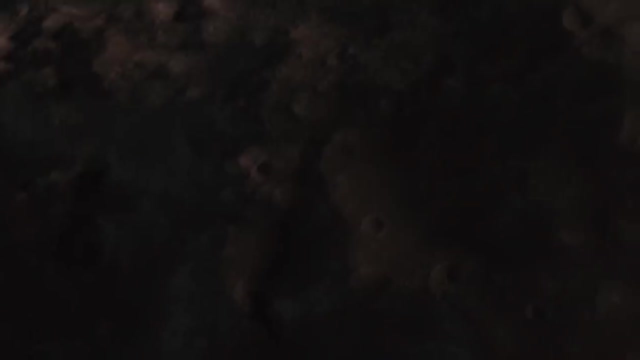 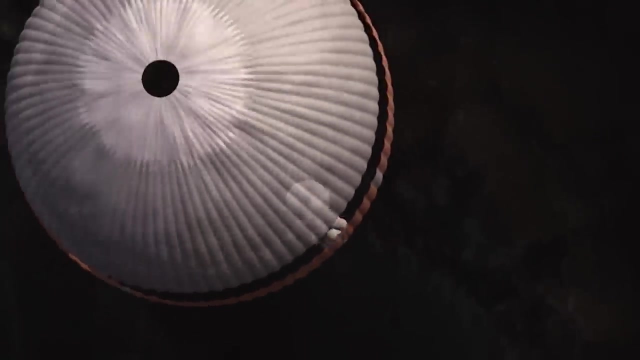 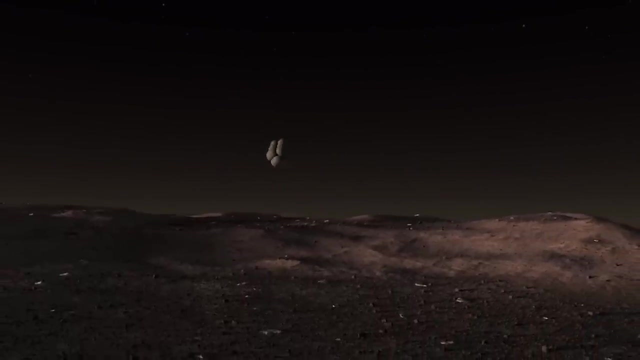 To do this, it used radically new airbag technology. The technique drew more from automotive safety systems than from previous space missions. The landing site in Mars' northern hemisphere known as Aris Vallis is one of the planet's rockiest areas. 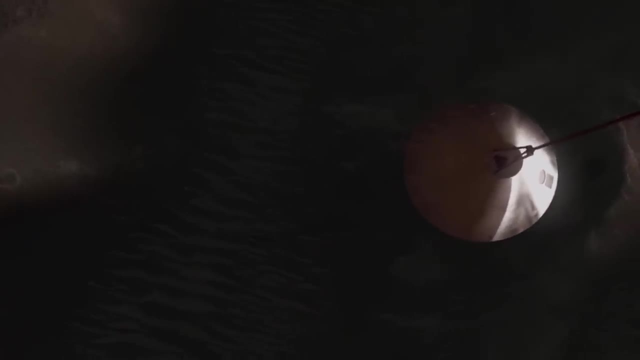 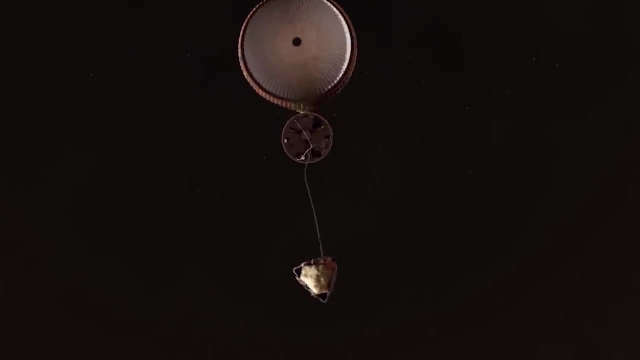 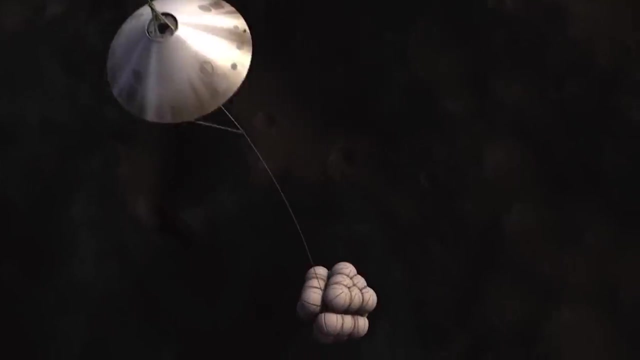 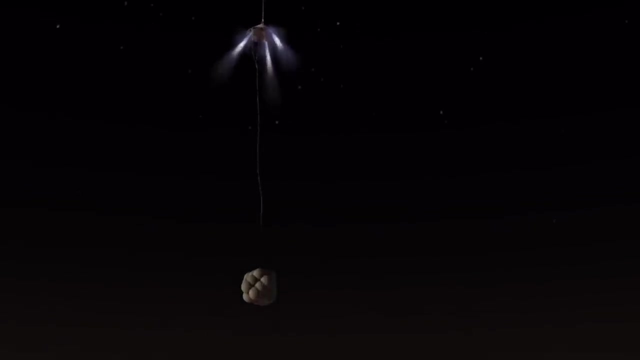 the reduced price tag could mean more missions. Pathfinder would land a small rover on the surface. To do this, it used radically new airbag technology. The technique drew more from automotive safety systems than from previous space missions. The landing site in Mars' northern hemisphere known as Aris Vallis. 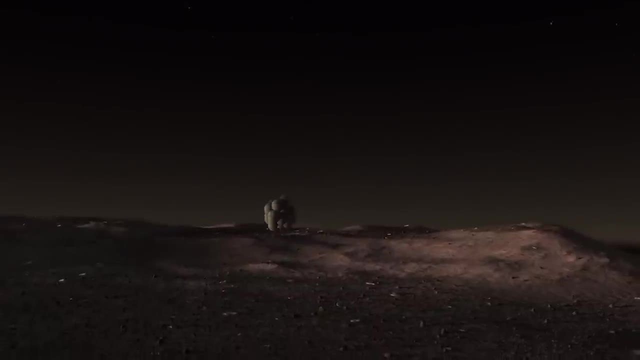 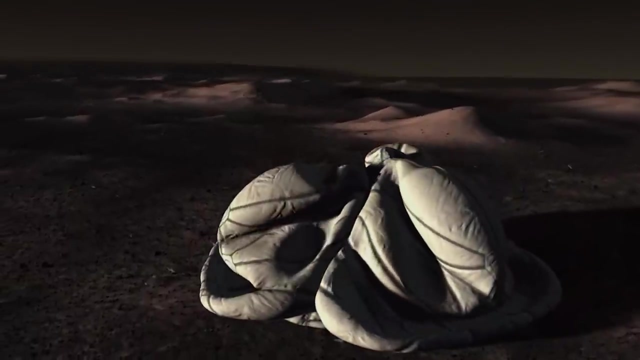 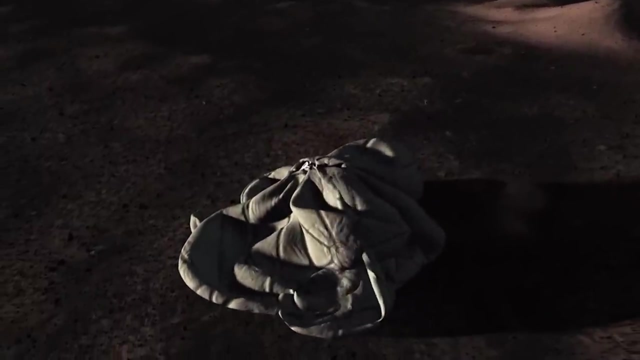 is one of the planet's rockiest areas, yet it was thought to be a safe area to land. The broad array of different rock types are believed to have been deposited during an ancient flood. The new landing technique worked perfectly and served as a proof of concept that would be used on future missions. 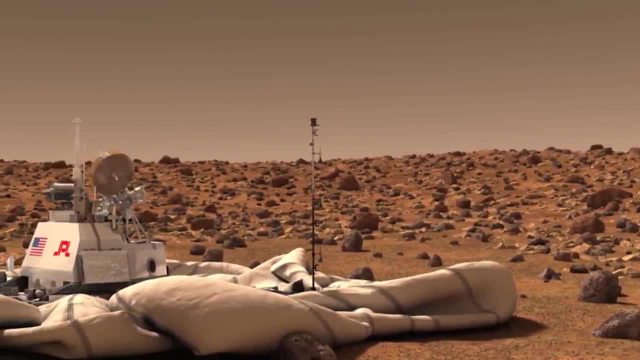 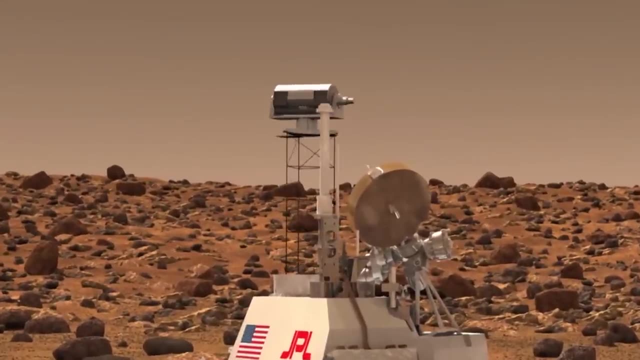 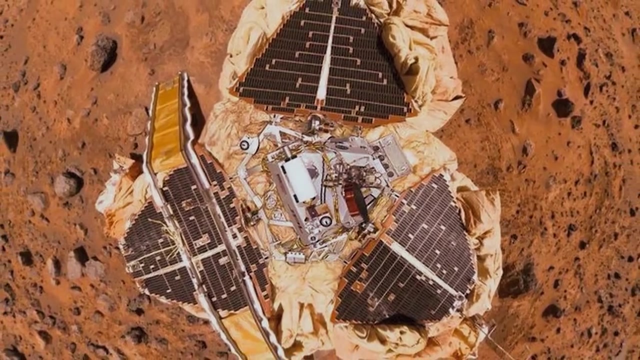 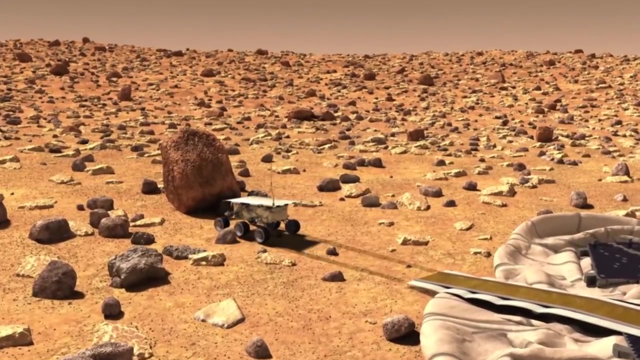 Pathfinder consisted of a base station equipped with three solar panels that unfolded like petals. There were sensors to measure atmospheric pressure, air temperature and wind speed, as well as a transmitter to communicate with Earth. In addition, Pathfinder acted as a base station for the Sojourner rover that explored the surrounding area. 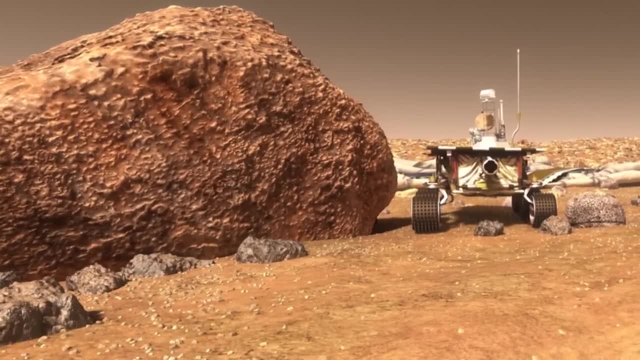 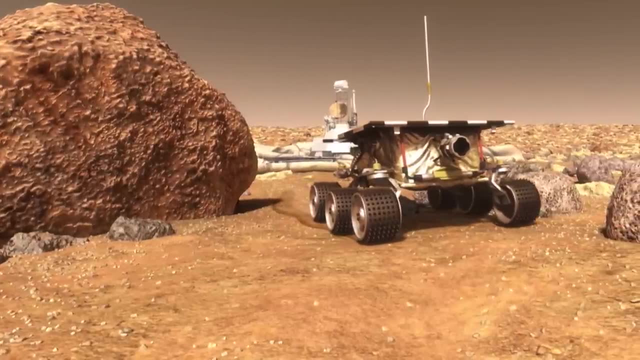 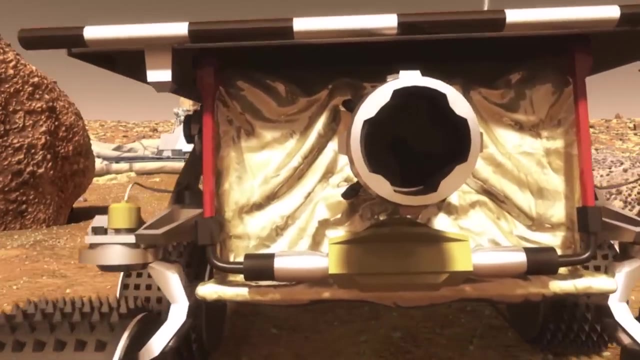 Sojourner was fitted with cameras and an alpha-particle X-ray spectrometer. It was the first mission to have its own website. The rover returned thousands of images and important detail about the atmosphere and geology, and its popularity guaranteed more Mars missions. 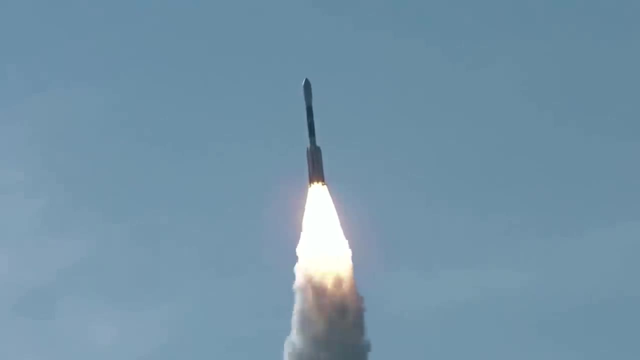 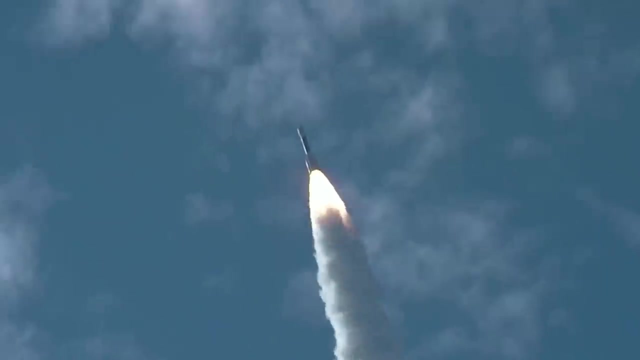 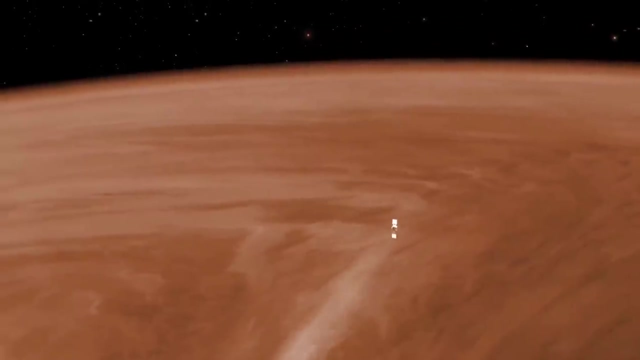 On the morning of April 7, 2001,, another Mars orbiter was launched. Mars Odyssey was equipped with three primary instruments and it had the ability to act as a relay satellite between future surface missions to the Red Planet and Earth. On its arrival at Mars, it used a new technique to go into orbit. 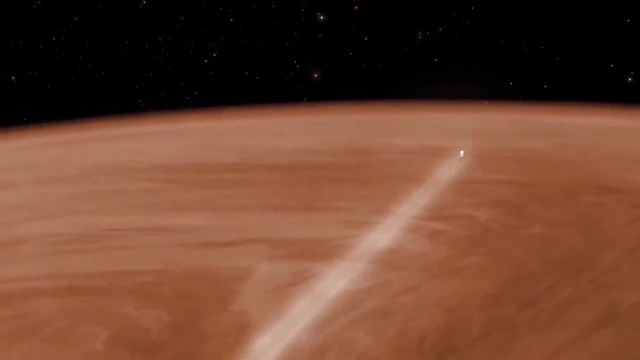 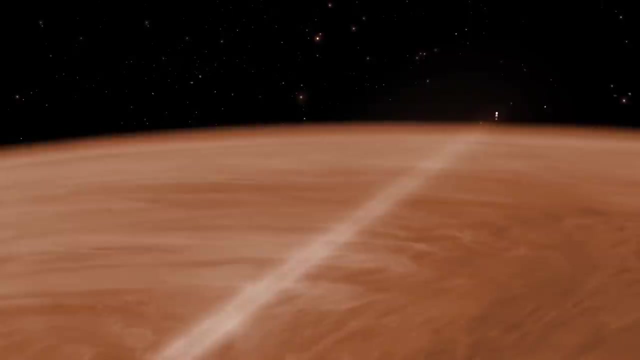 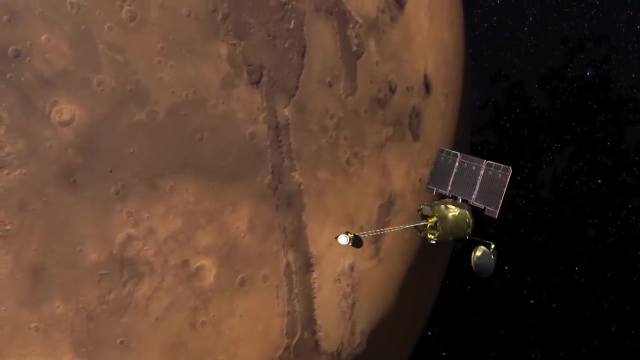 After firing a relatively brief pulse of its engine, Mars Odyssey went into a highly elliptical orbit that, at its closest approach, had it skimming the planet's thin upper atmosphere. Called aerobraking, this technique allowed the craft to circularize its orbit over a period of three months. 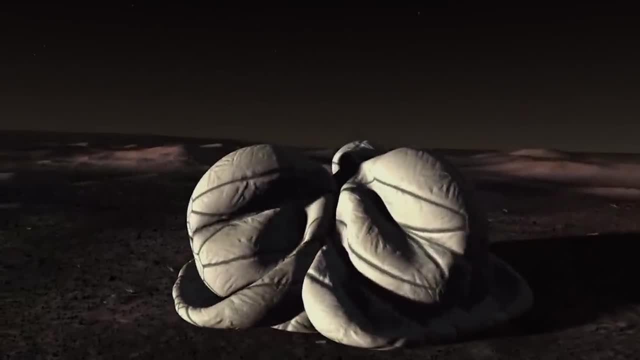 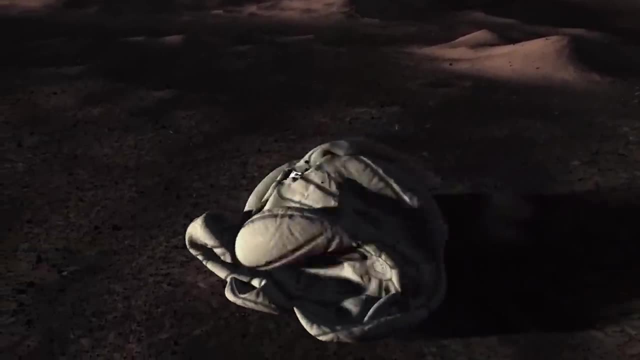 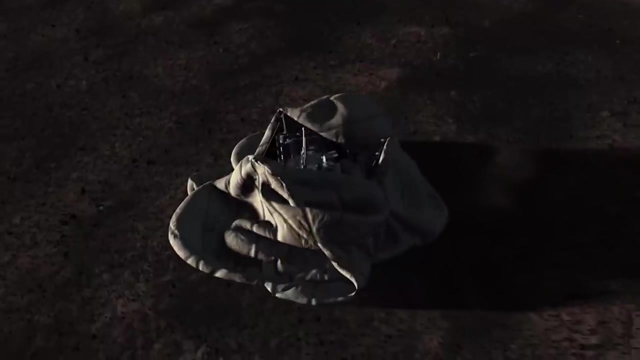 yet it was thought to be a safe area to land. The broad array of different rock types are believed to have been deposited during an ancient flood. The new landing technique worked perfectly and served as a proof of concept that would be used on future missions. 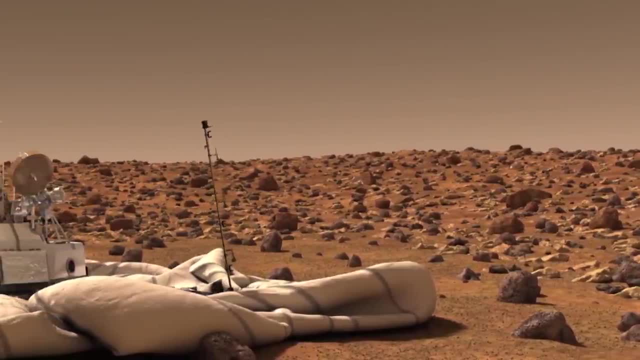 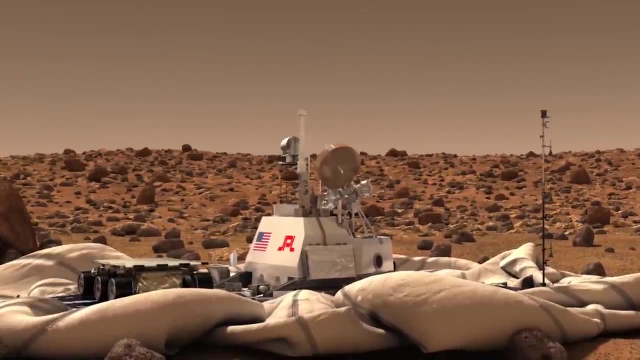 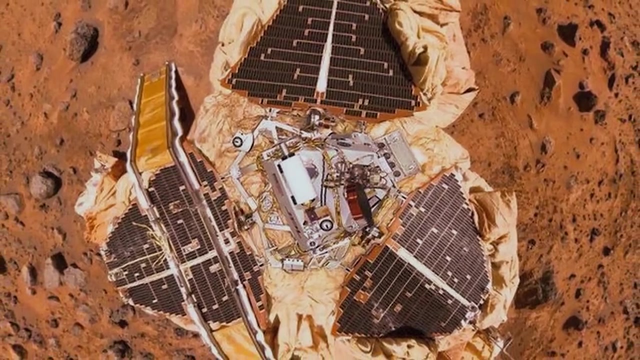 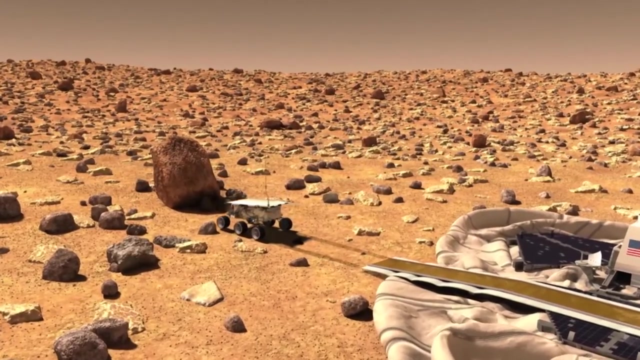 Pathfinder consisted of a base station equipped with three solar panels that unfolded like petals. There were sensors to measure atmospheric pressure, air temperature and wind speed, as well as a transmitter to communicate with Earth. In addition, Pathfinder acted as a base station for the Sojourner rover that explored the surrounding area. 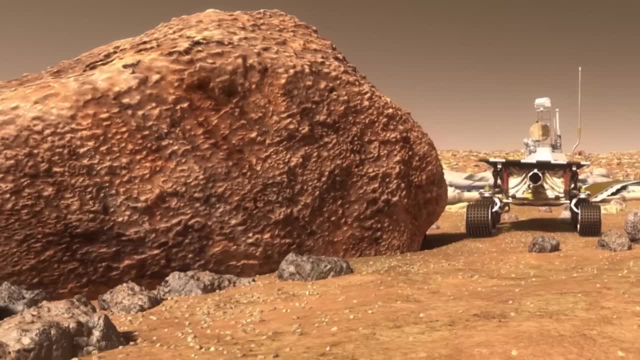 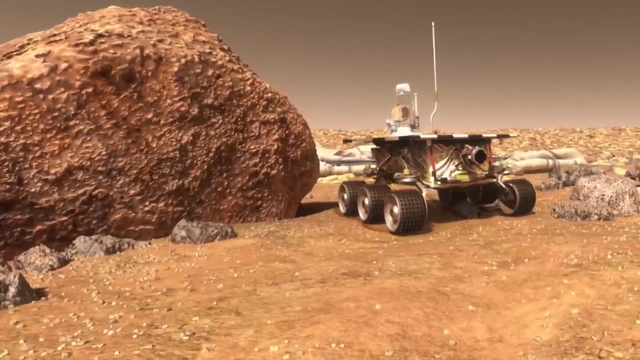 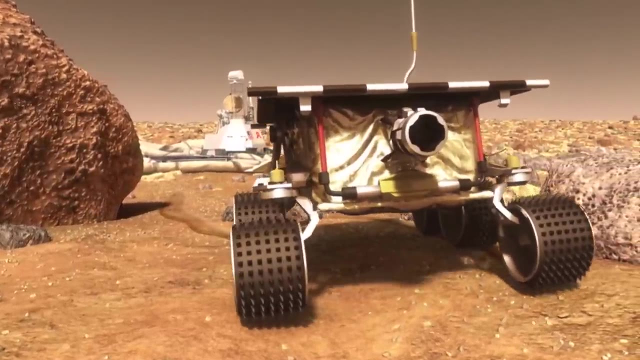 Sojourner was found to be the first rover to land on Mars. Sojourner was fitted with cameras and an alpha-particle X-ray spectrometer. It was the first mission to have its own website. The rover returned thousands of images and important detail about the atmosphere and geology. 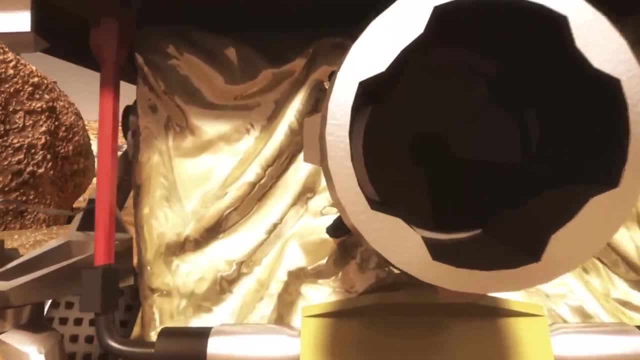 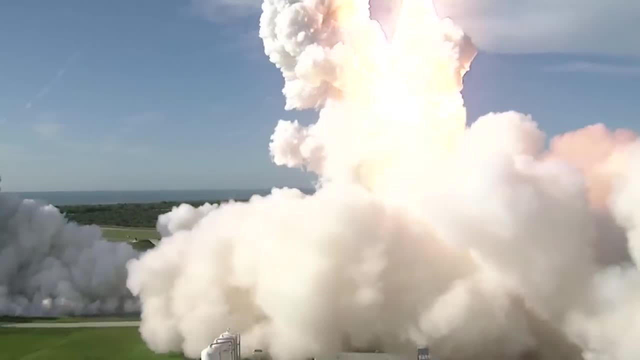 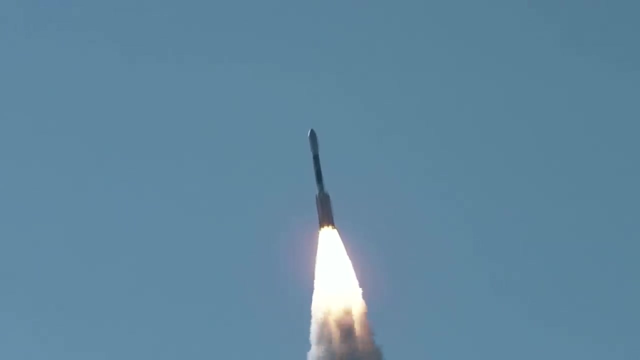 and its popularity guaranteed more Mars missions. On the morning of April 7, 2001,, another Mars orbiter was launched. Mars Odyssey was equipped with three primary instruments and it had the ability to act as a relay satellite between future surface missions to the Red Planet and Earth. 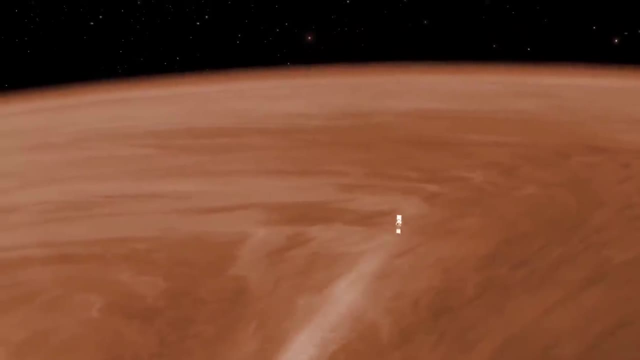 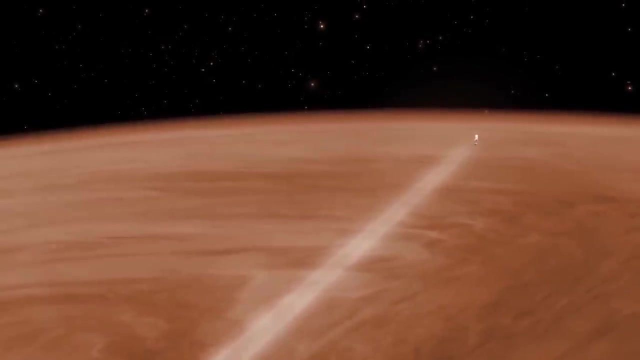 On its arrival at Mars, it used a new technique to go into orbit. After firing a relatively brief pulse of its engine, Mars Odyssey went into a highly elliptical orbit that, at its closest approach, had it skimming the planet's thin upper atmosphere. 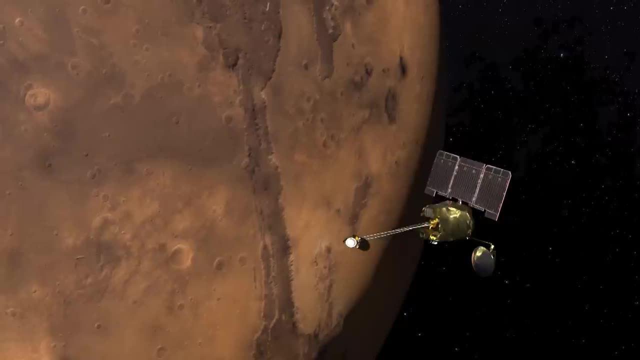 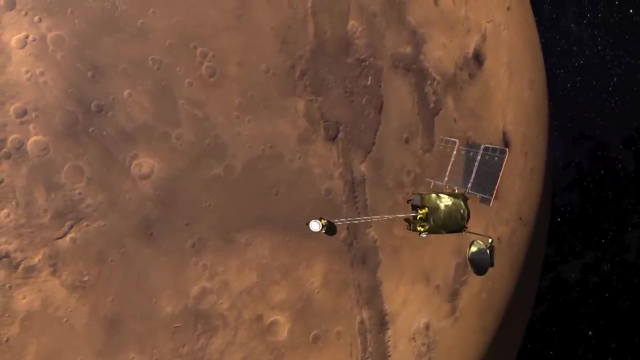 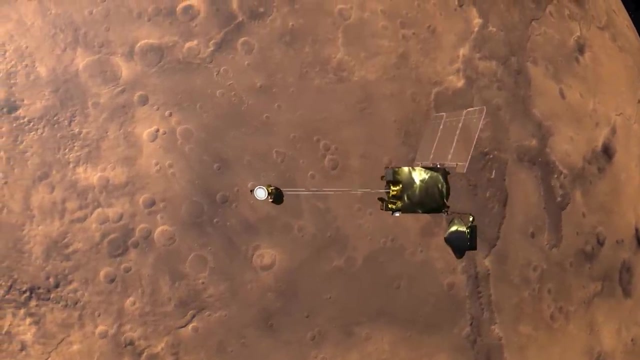 Called aerobraking. this technique allowed the craft to circularize its orbit over a period of three months and it saved around 200 kilograms of fuel. The probe is still in operation today, breaking all records as the longest-serving Mars mission. 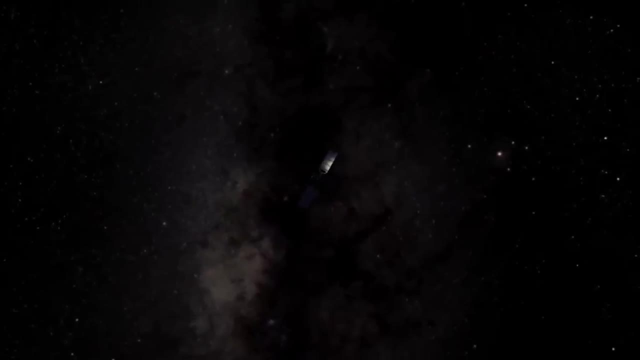 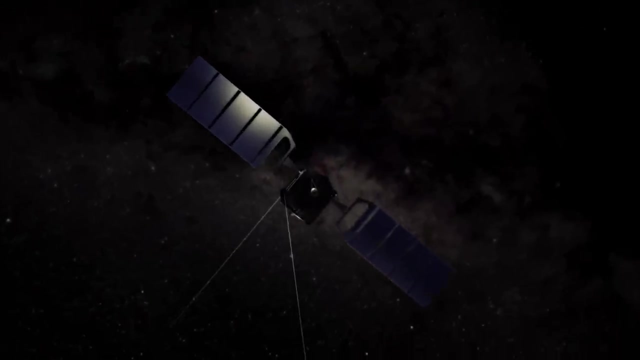 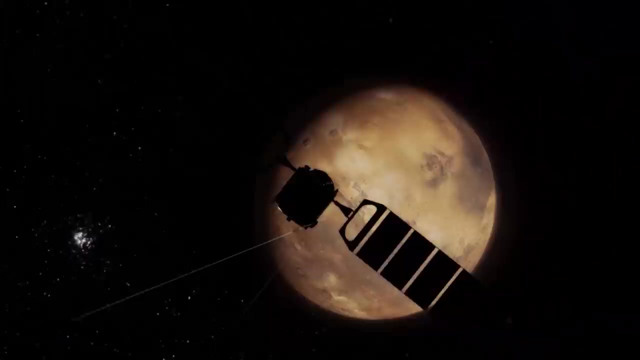 In December 2003,, a new player arrived at Mars. The European Space Agency, using a Russian launcher, had sent Mars Express, its first planetary explorer. It was equipped with a lander known as Beagle, Though all contact was lost with the lander. 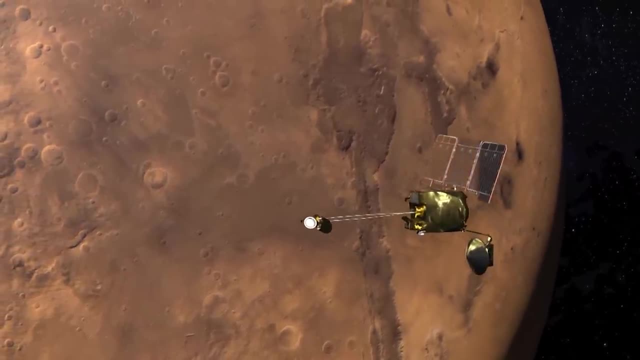 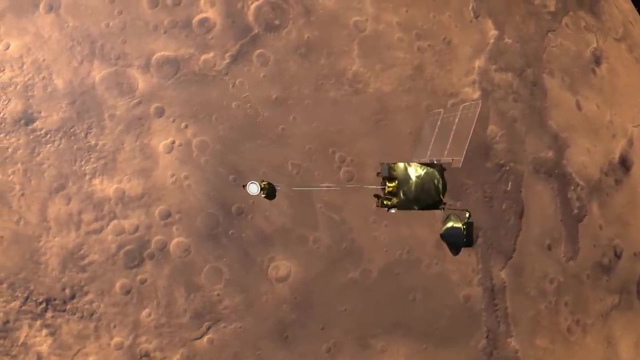 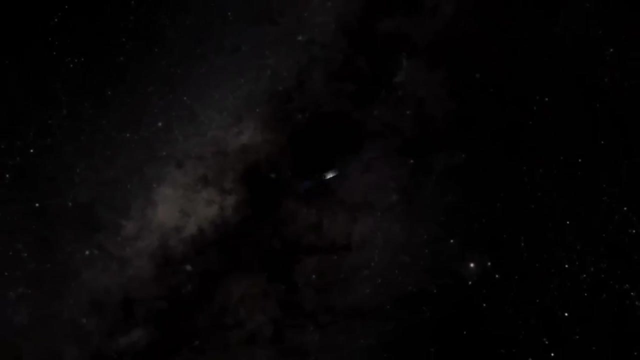 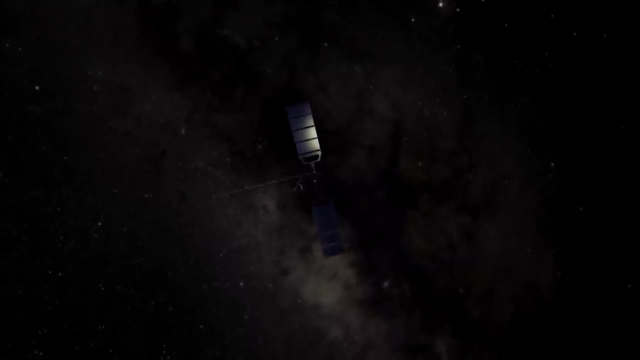 and it saved around 200 kilograms of fuel. The probe is still in operation today, breaking all records as the longest-serving Mars mission. In December 2003, a new player arrived at Mars: The European Space Agency, using a Russian launcher. 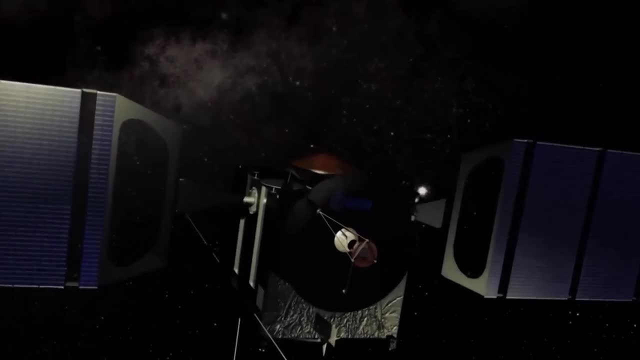 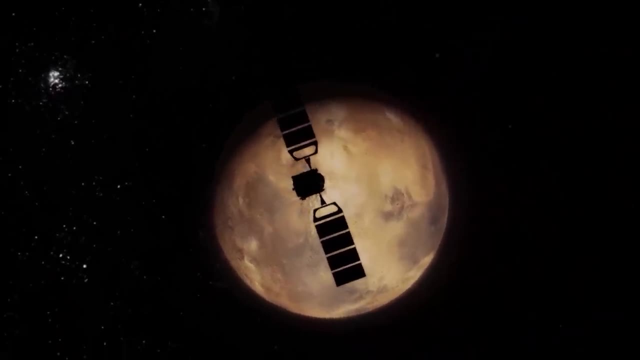 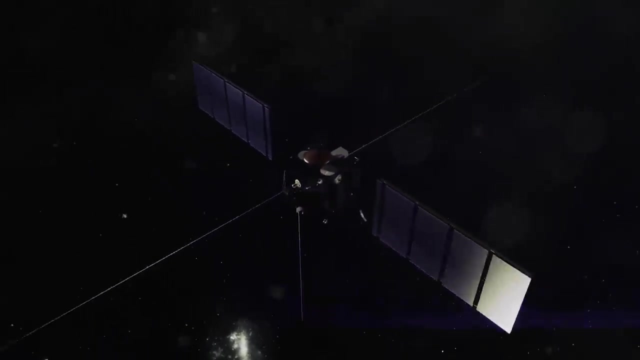 had sent Mars Express, its first planetary explorer. It was equipped with a lander known as Beagle. Though all contact was lost with the lander, Mars Express continues to return valuable data. The mission has been granted several extensions, the latest till 2020.. 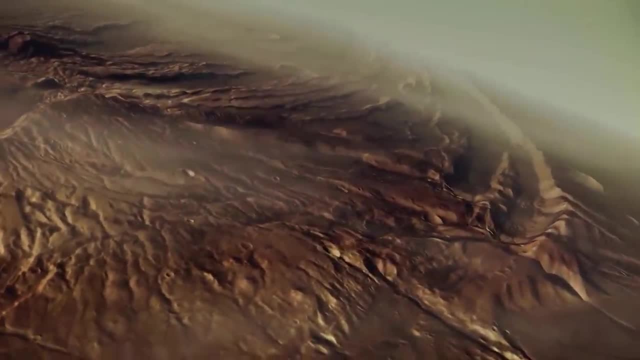 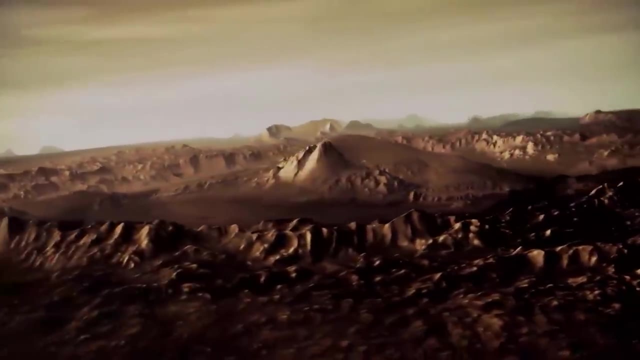 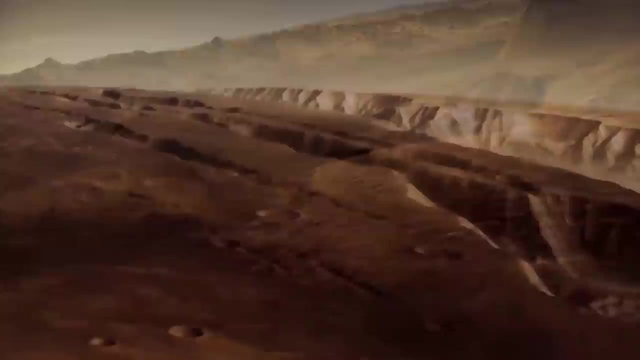 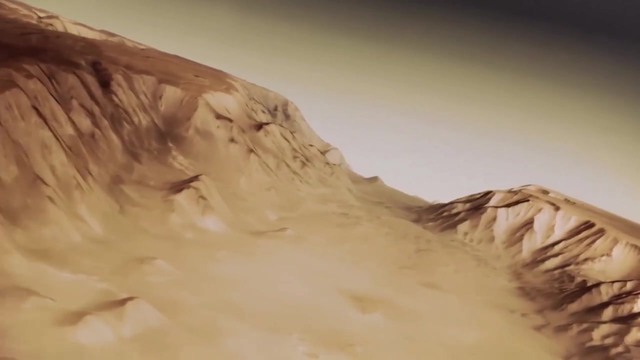 Equipped with a high-resolution stereo camera, the probe returned unique 3D views of the planet's surface. The orbiter determined that the polar ice caps contain a blend of frozen CO2 and water ice In the atmosphere. Mars Express detected first methane. 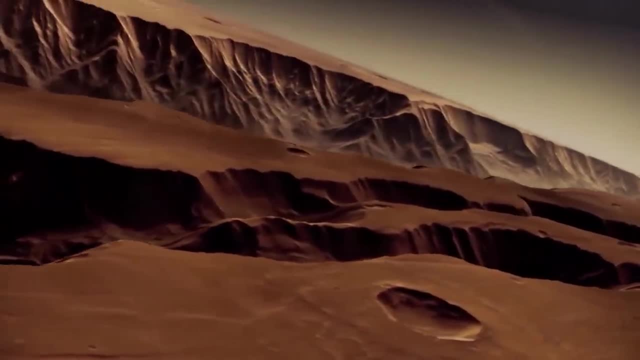 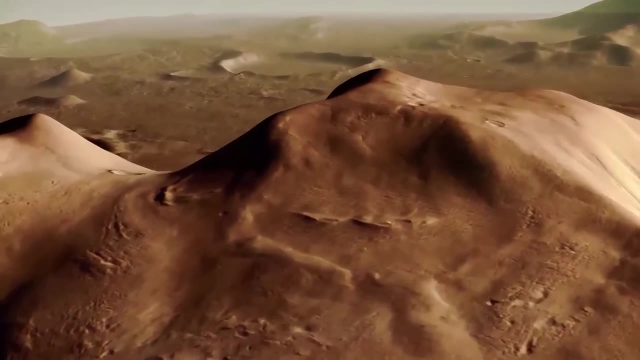 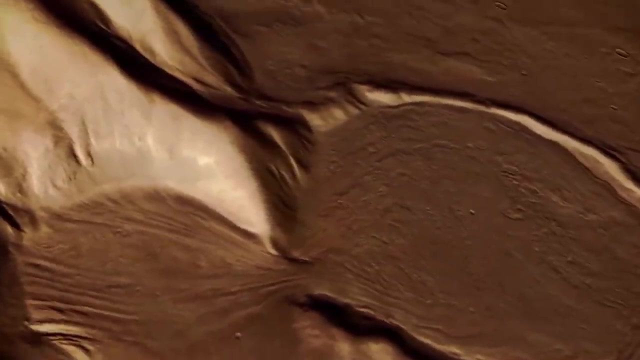 and then ammonia. Both gases deteriorate rapidly in sunlight, so there must be sources on Mars continually producing them. Methane and ammonia can rarely be made inorganically, but they're generally associated with life. One month after Mars Express went into orbit. 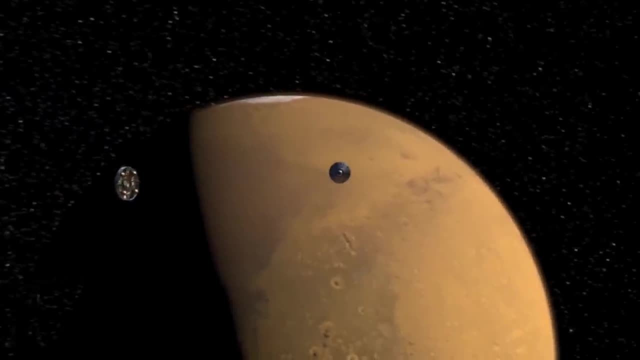 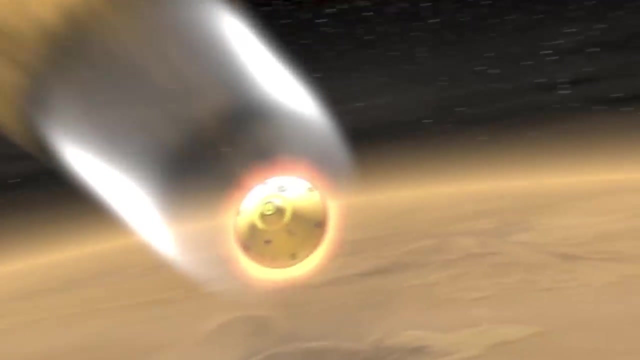 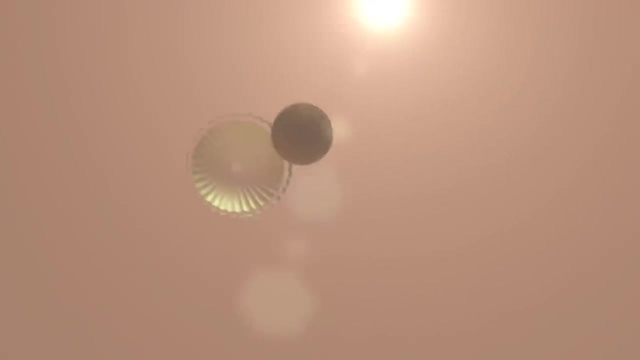 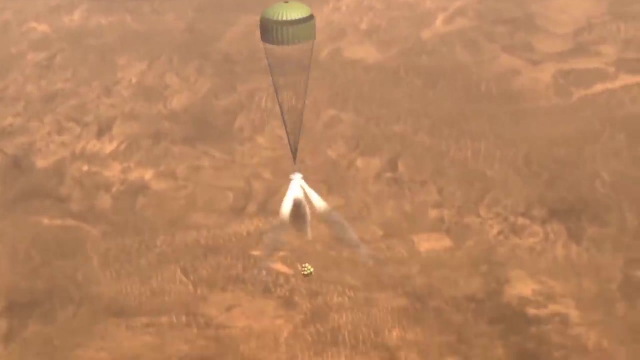 a NASA lander arrived at Mars, followed three weeks later by a second identical craft. They were the Mars Exploration Rovers called Spirit and Opportunity. Spirit the first to land was targeted at the Gusev crater. Opportunity would land at the Meridiani Planum. 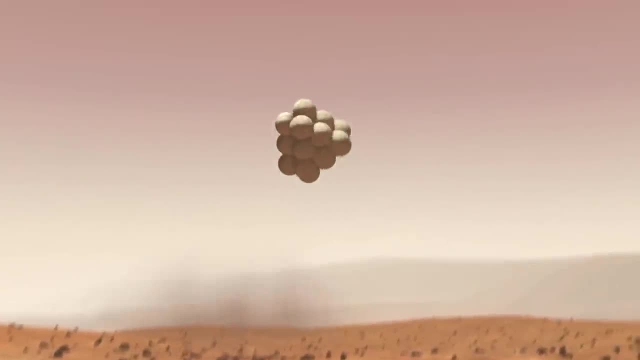 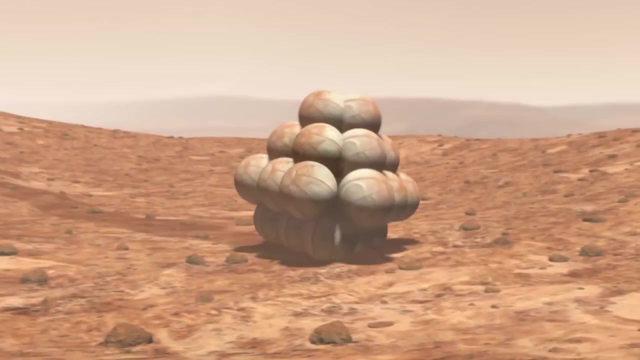 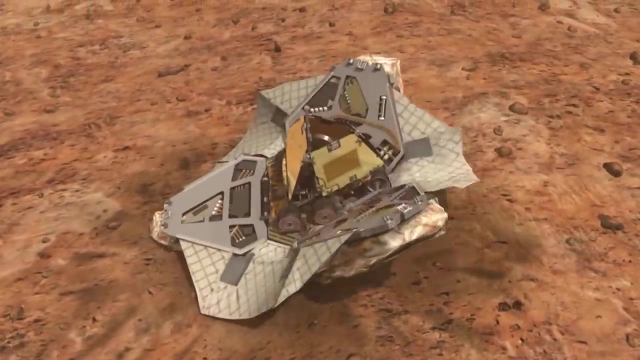 on the opposite side of Mars. It was the first time that the lander landed on Mars. Although they were much heavier than their Pathfinder predecessor, they used the same bounce landing technique. Both landings were successful and on target After the craft had righted itself. 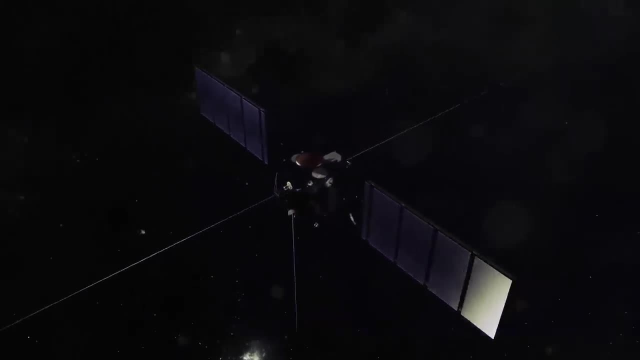 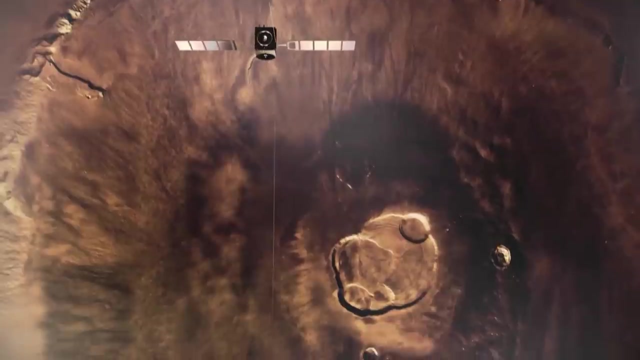 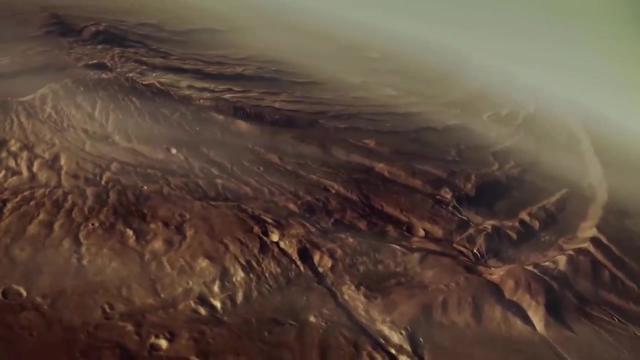 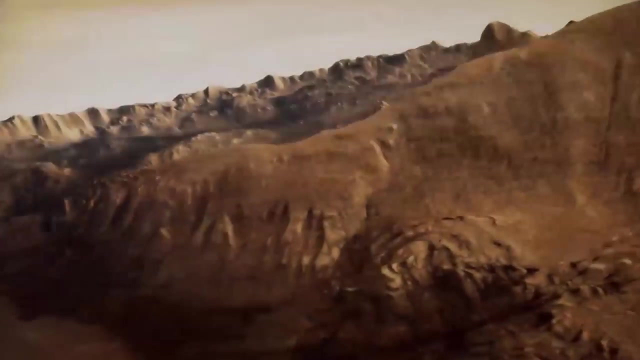 Mars Express continues to return valuable data. The mission has been granted several extensions, the latest till 2020.. Equipped with a high-resolution stereo camera, the probe returned unique 3D views of the planet's surface. The orbiter determined that the polar ice caps. 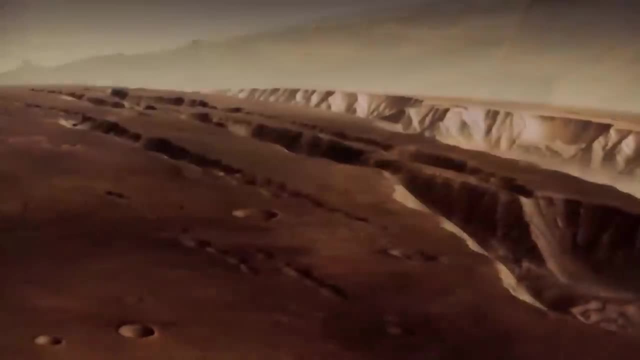 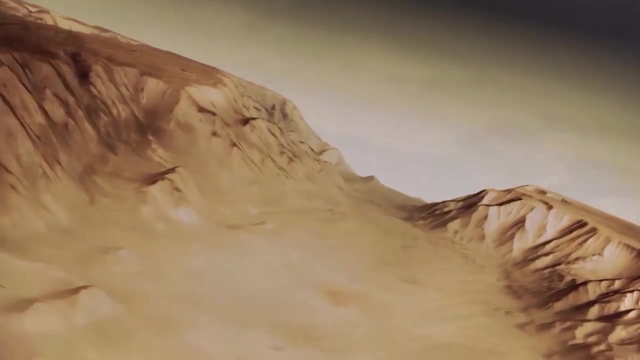 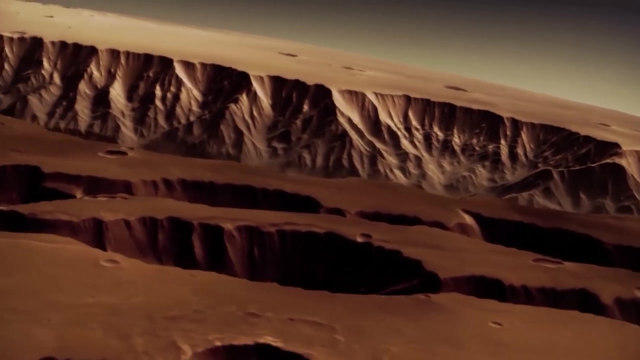 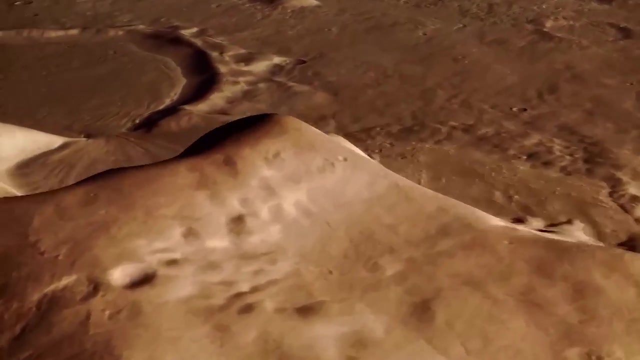 contain a blend of frozen CO2 and water ice In the atmosphere. Mars Express detected first methane and then ammonia. Both gases deteriorate rapidly in sunlight, so there must be sources on Mars continually producing them. Methane and ammonia can rarely be made inorganically. 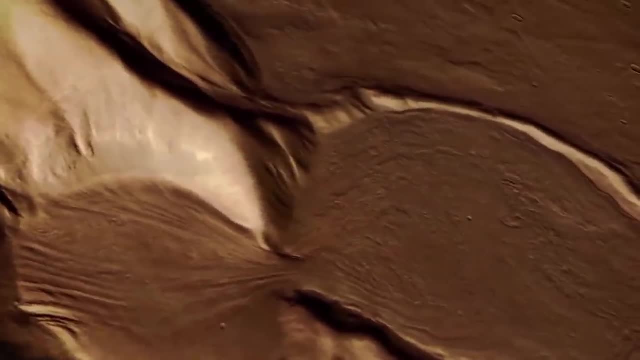 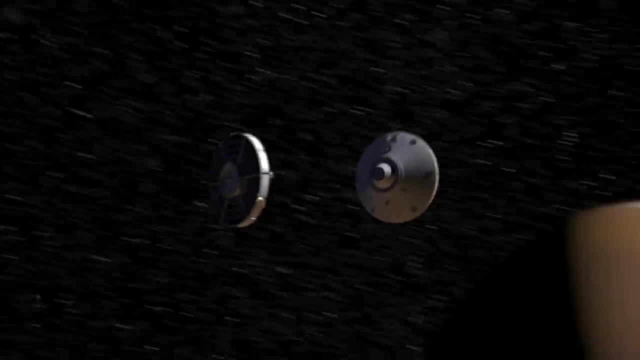 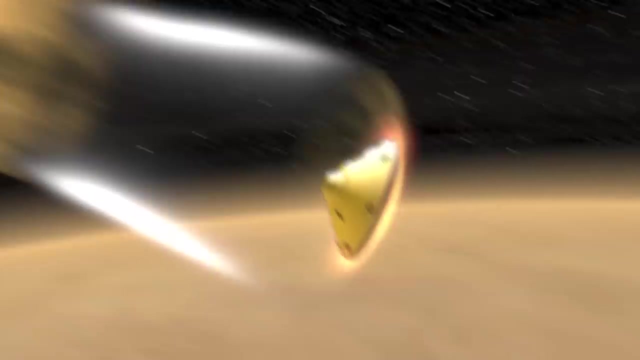 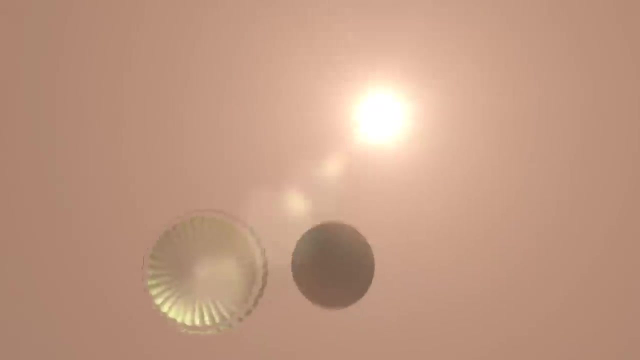 but they're generally associated with life. One month after Mars Express went into orbit, a NASA lander arrived at Mars, followed three weeks later by a second identical craft. They were the Mars exploration rovers called Spirit and Opportunity Spirit, the first to land. 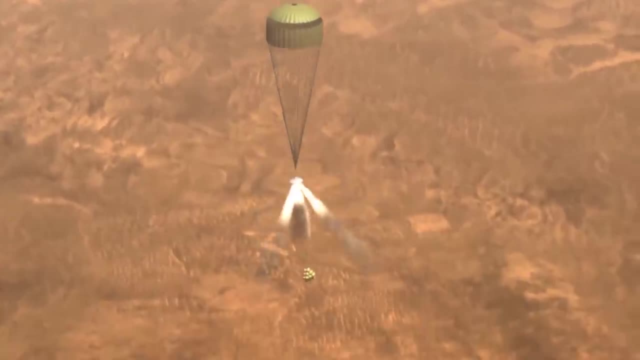 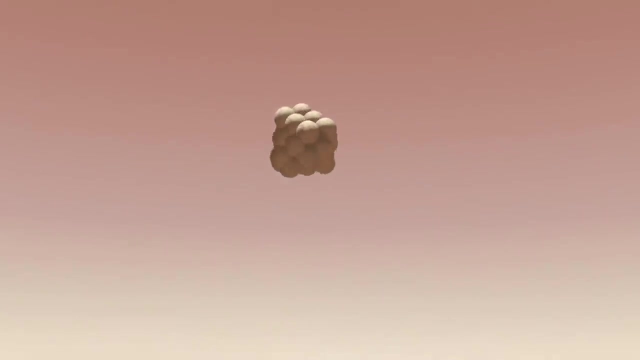 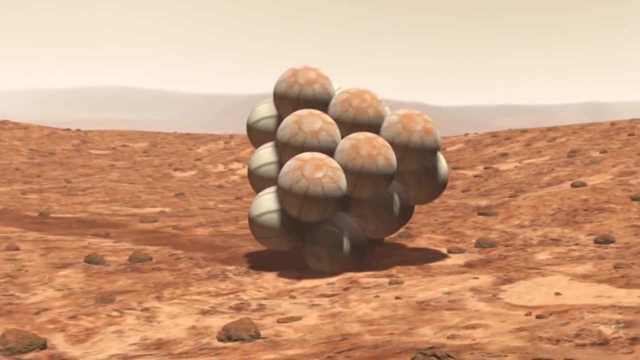 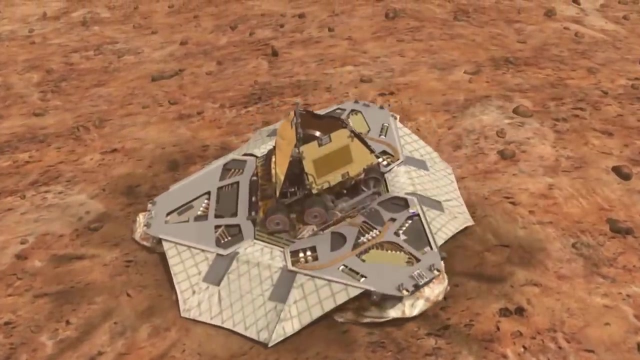 was targeted at the Gusev crater Opportunity would land at the Meridiani Planum, on the opposite side of Mars. Though they were much heavier than their pathfinder predecessor, they used the same bounce landing technique. Both landings were successful and on target. 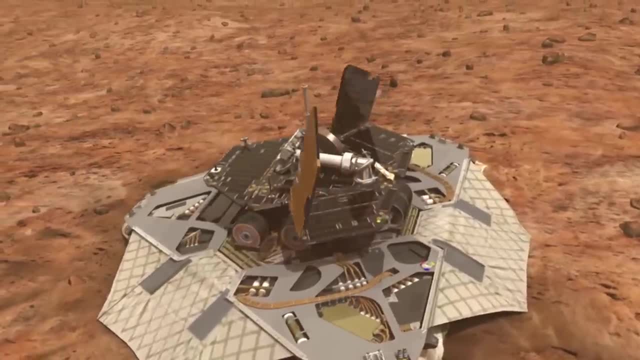 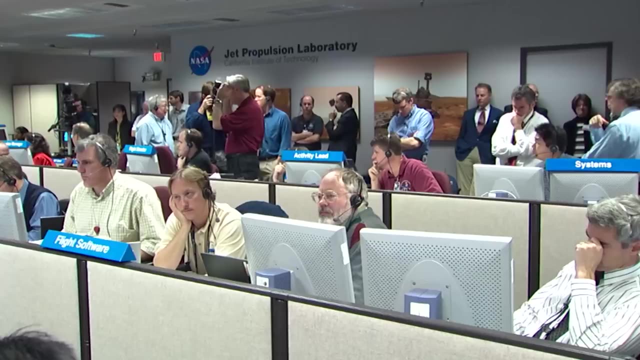 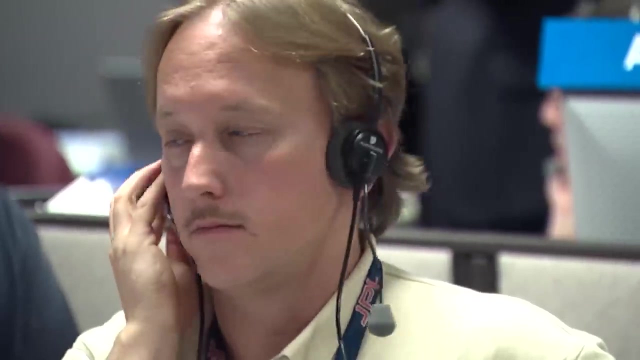 After the craft had righted itself, it detached from the lander and began autonomously unfolding its solar panels and camera mast. While this was happening, the team back at the Jet Propulsion Laboratory waited. Signals confirming the craft's safe arrival took 15 minutes to travel back to Earth. 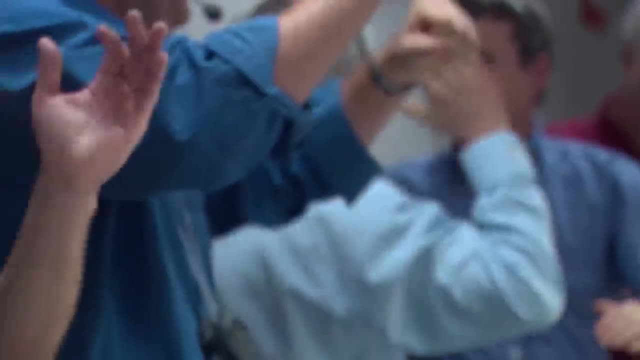 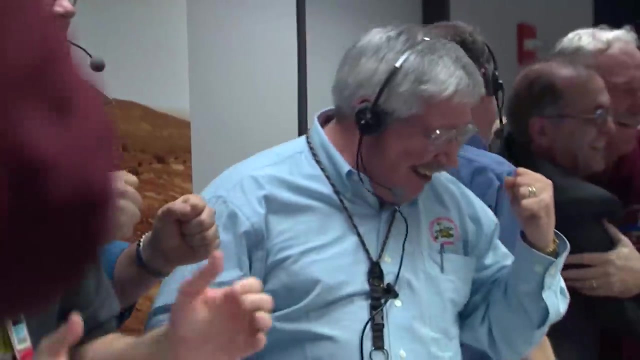 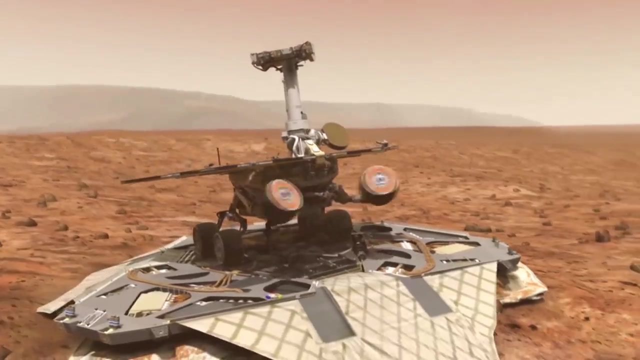 The NASA crew were impressed by the success of their mission. It was a great experience to see the stars in the space of space. Many of these people had invested years of their lives in this project and the real mission had only just commenced. Both rovers were designed to operate for 90 Mars days. 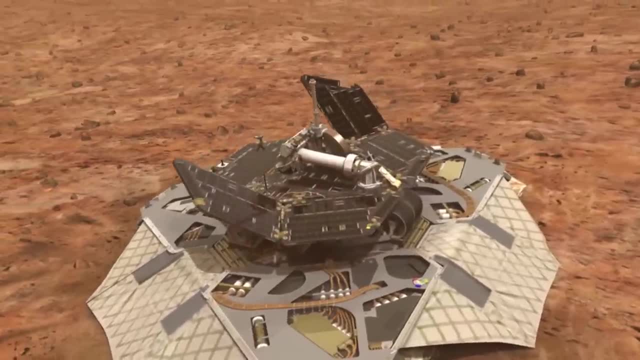 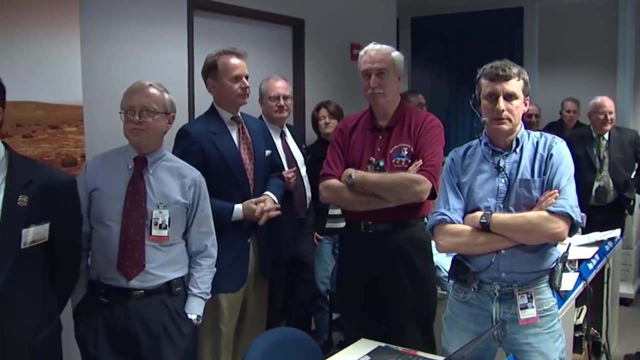 it detached from the lander and began autonomously unfolding its solar panels and camera mast. While this was happening, the team back at the Jet Propulsion Laboratory waited. Signals confirming the craft's safe arrival took 15 minutes to travel back to Earth. 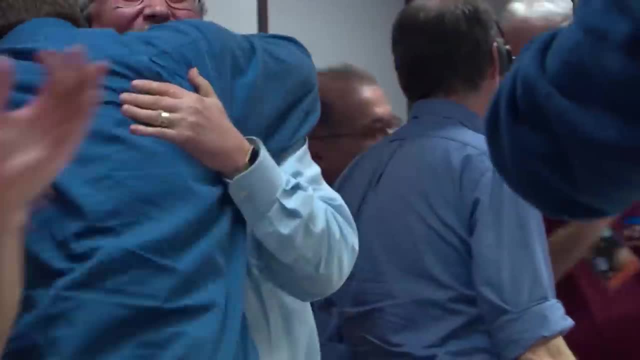 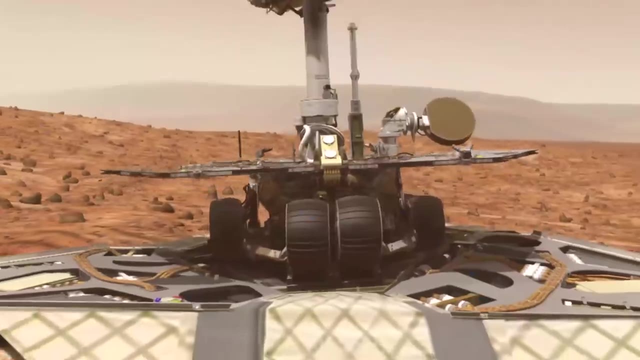 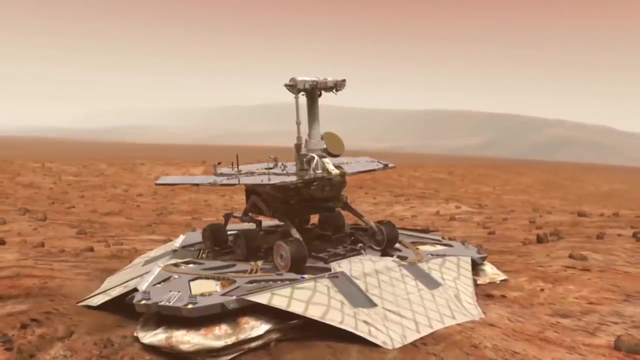 Many of these people had invested years of their lives in this project and the real mission had only just commenced. Both rovers were designed to be able to fly and both rovers were designed to operate for 90 Mars days. A solar day on Mars is about 40 minutes longer than an Earth day. 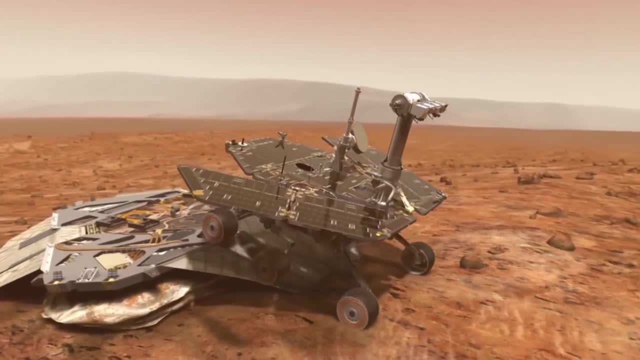 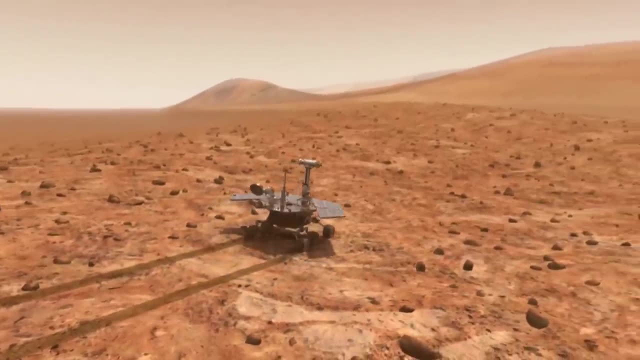 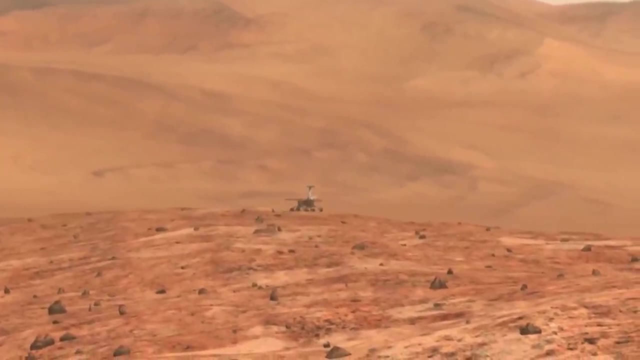 And to avoid confusion, the science team operating the rovers refer to a Martian day as a Sol Mission. designers knowing about the dust storms on Mars felt that the solar panels on the two rovers would eventually be blocked with dirt and stop functioning. 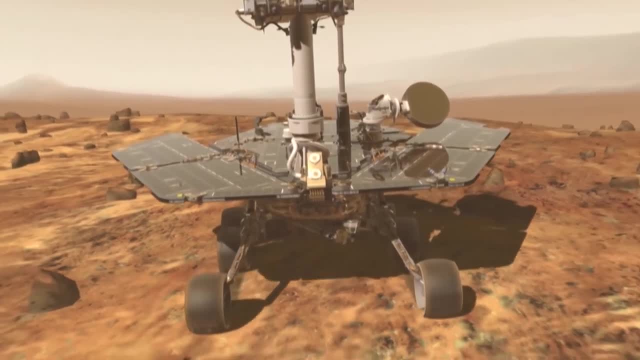 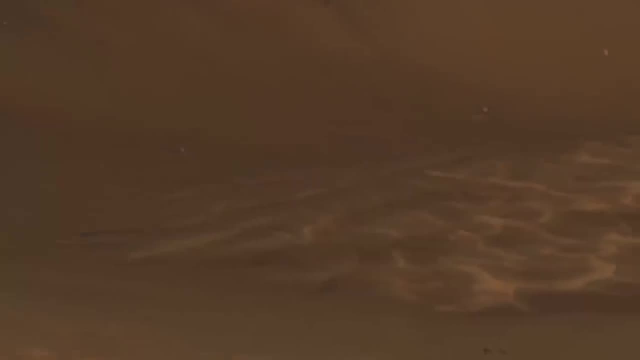 But it became clear that the winds on Mars were clearing the panels. Soon NASA announced that Opportunity had found evidence confirming liquid water had once flowed on Mars. There were pictures from the Meridiani Planum of stratified patterns in the rock, suggesting sedimentation. 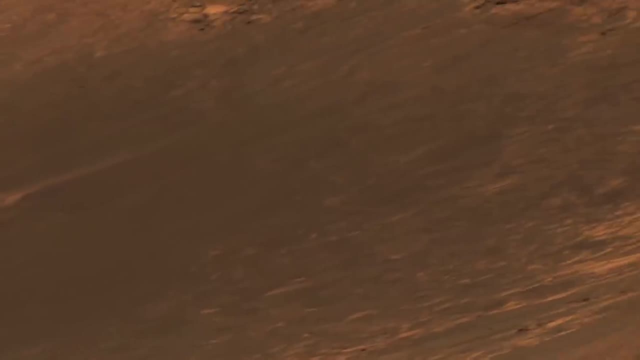 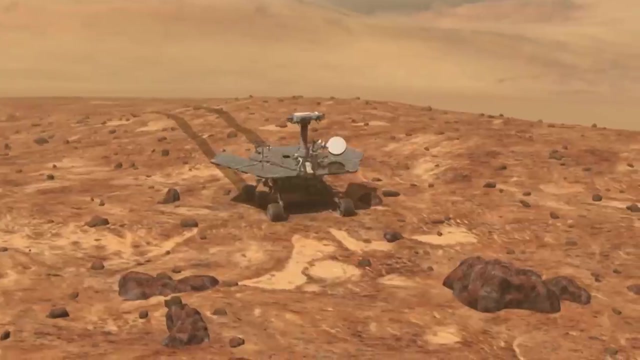 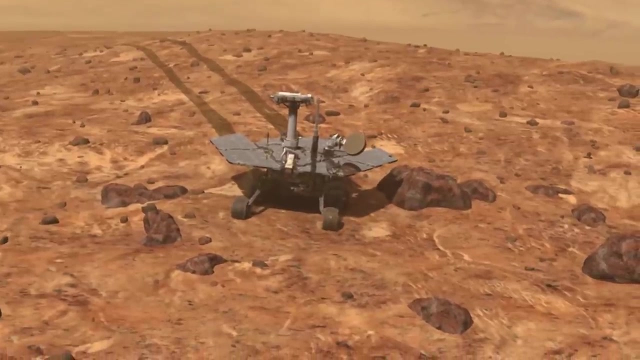 The distribution of chlorine and bromine at the site were clues to the area's past as the shore of a salty sea. In April 2004,, NASA announced it would extend the rovers' missions from three to eight months. It would be the first of many such mission extensions. 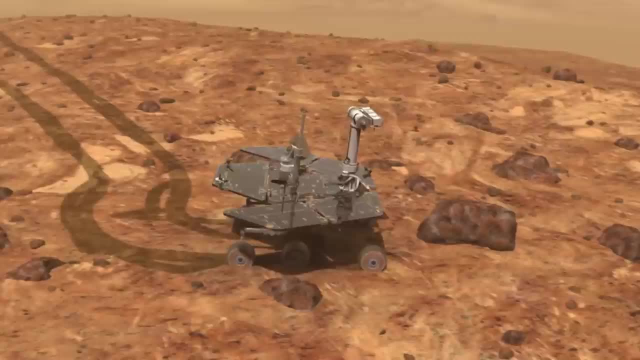 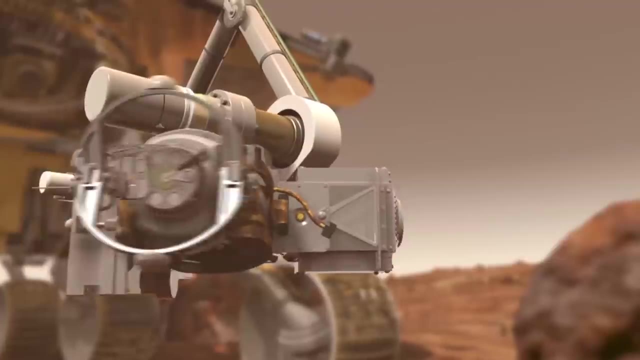 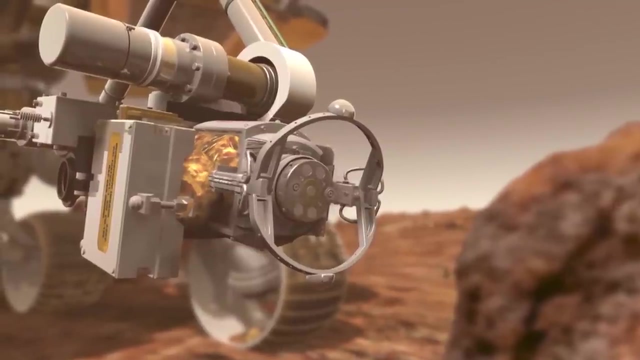 The rovers were equipped with an abrasion tool to grind away a portion of a rock's surface for a more detailed, uncontaminated analysis of geological samples. This was first done by Spirit at a rock named Adirondack at Gusev Crater. 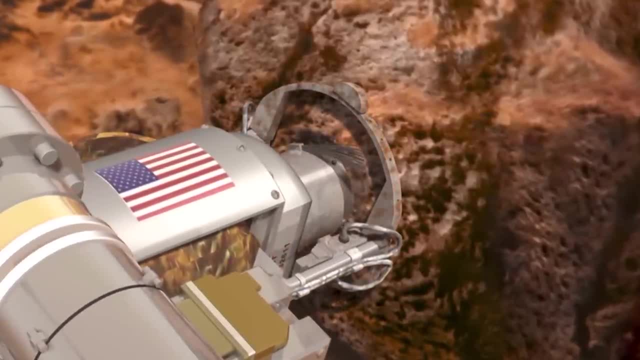 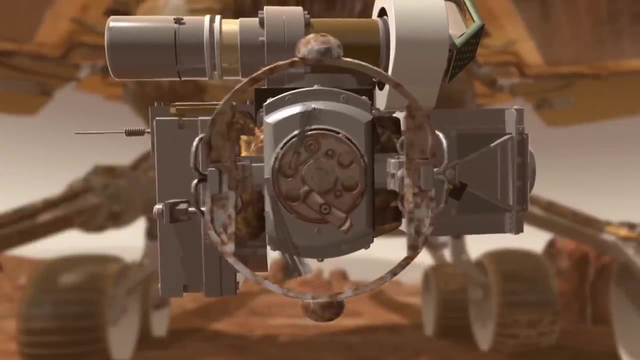 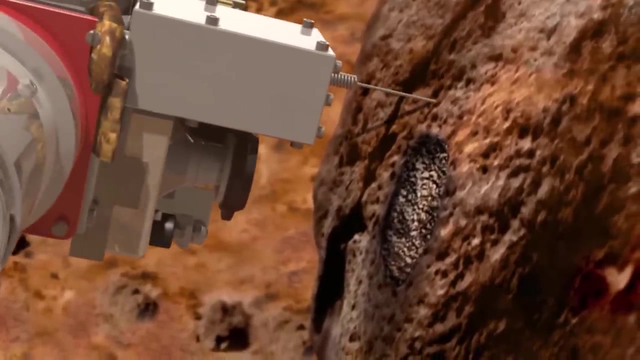 It was a first in planetary geology. Researchers agonized before using the tool because of the drain it makes on the rover's energy budget. The rock was made of olivine pyroxene and magnetite, making it very similar to volcanic basalt. 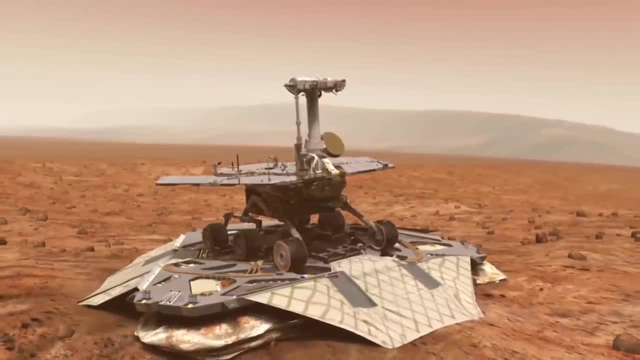 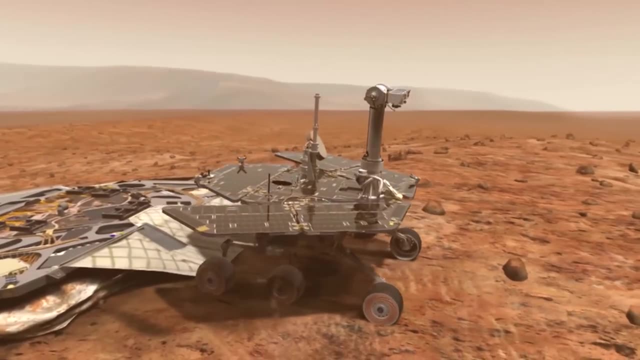 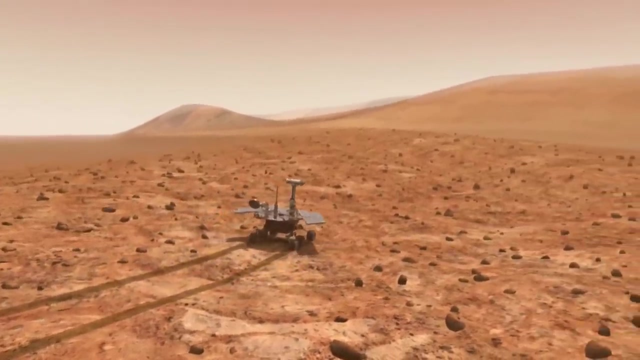 A solar day on Mars is about 40 minutes longer than an Earth day And, to avoid confusion, the science team operating the rovers refer to a Martian day as a Sol Mission. designers knowing about the dust storms on Mars felt that the solar panels 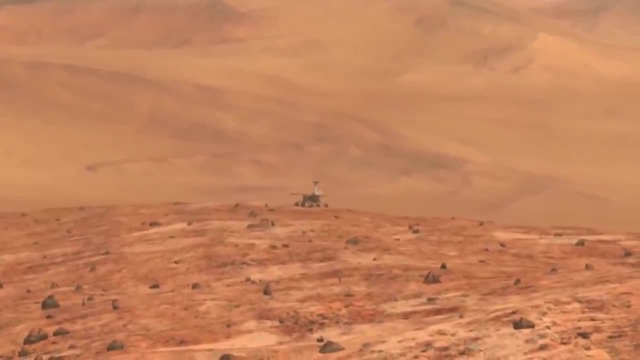 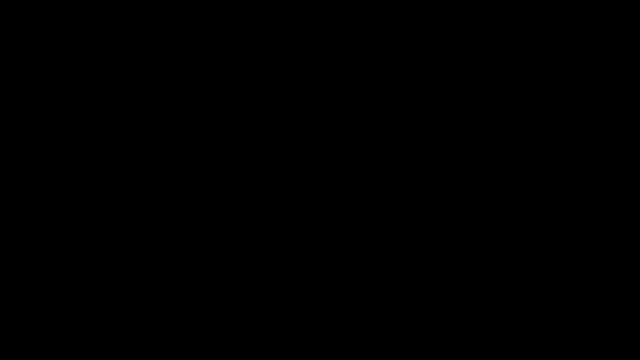 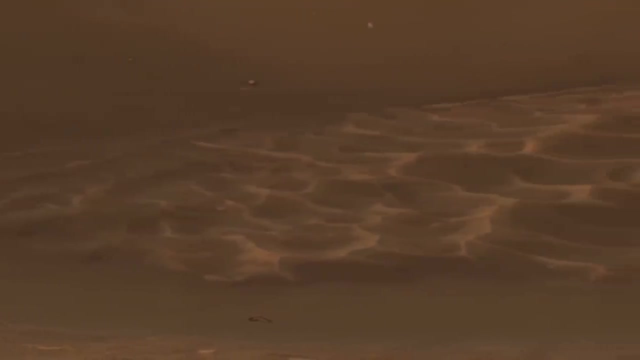 on the two rovers would eventually be blocked with dirt and stop functioning. but it became clear that the winds on Mars were clearing the panels Soon. NASA announced that Opportunity had found evidence confirming liquid water had once flowed on Mars. There were pictures from the Meridiani Planum of stratified patterns in the rocks, suggesting 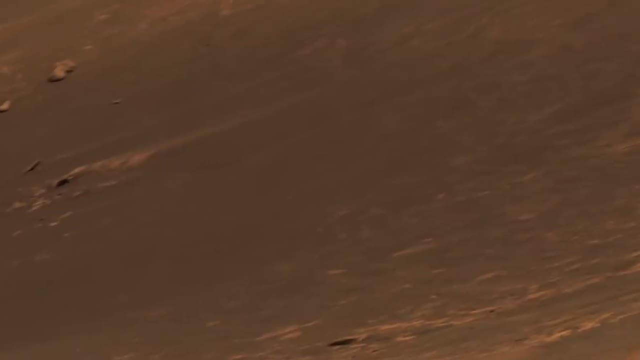 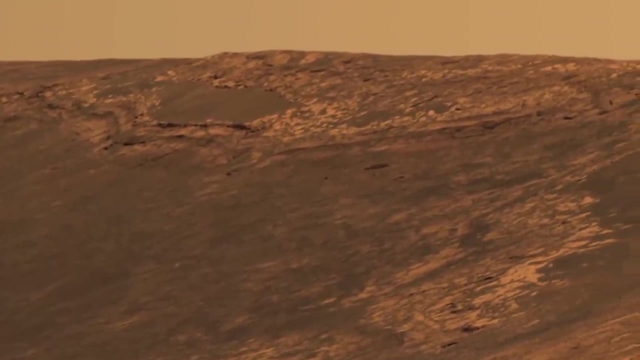 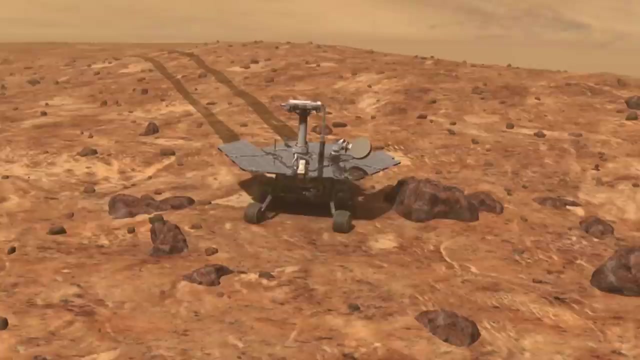 sedimentation, The distribution of chlorine and bromine at the site were clues to the area's past as the shore of a salty sea. In April 2004,, NASA announced it would extend the rover's missions from three to eight months. It would be the first of many. 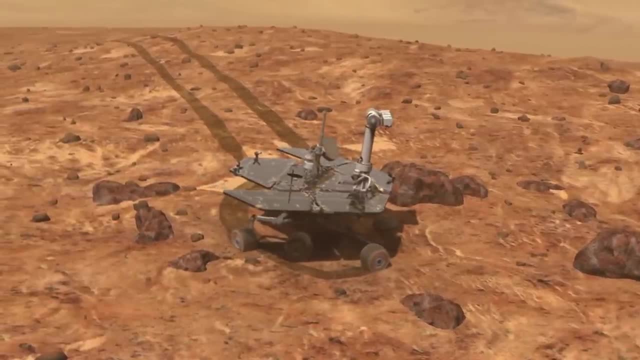 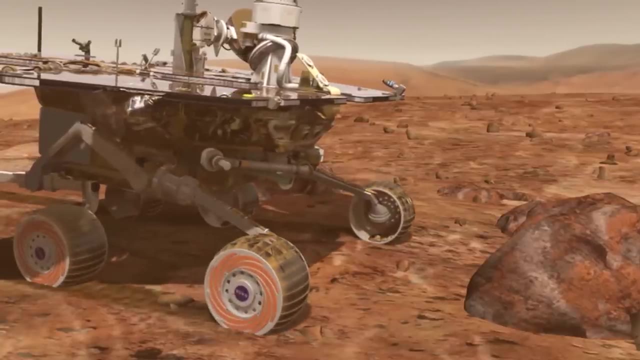 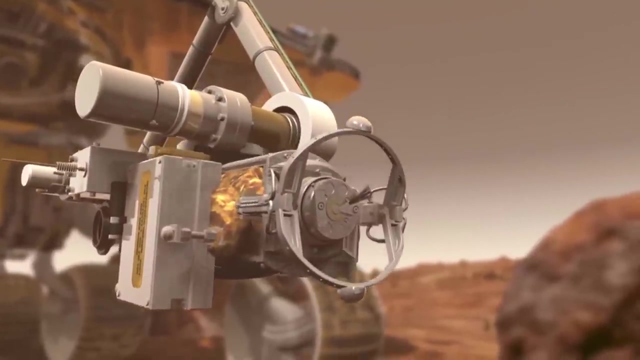 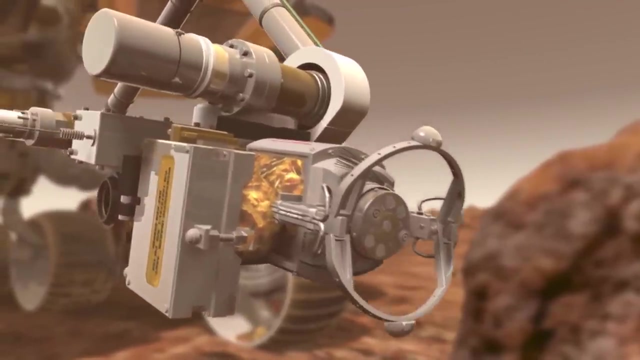 such mission extensions. The rovers were equipped with an abrasion tool to grind away a portion of a rock's surface for a more detailed, uncontaminated analysis of geological samples. This was first done by Spirit at a rock named Adirondack at Gusev Crater. 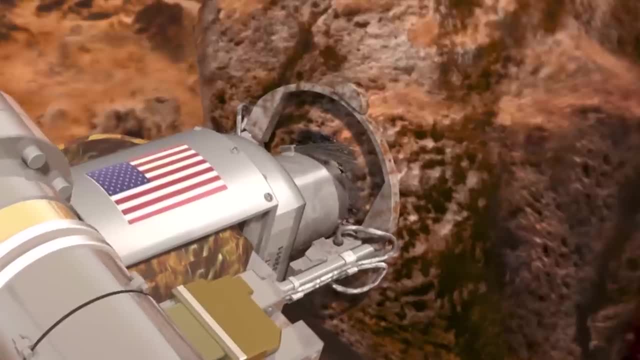 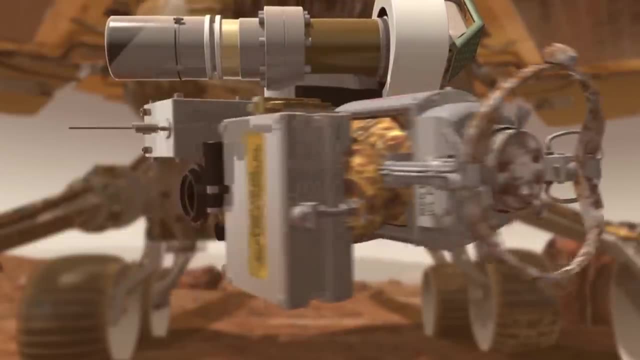 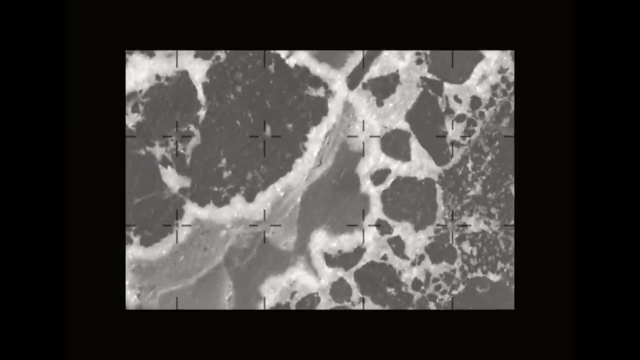 It was a first in planning. It was the first time in the world that the rover was used in planetary geology. Researchers agonized before using the tool because of the drain it makes on the rover's energy budget. The rock was made of olivine pyroxene and magnetite, making it very similar to volcanic. 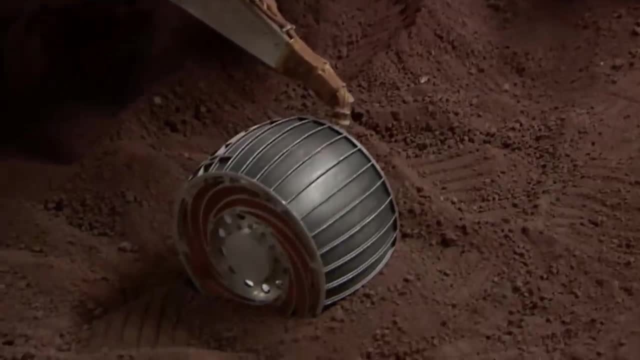 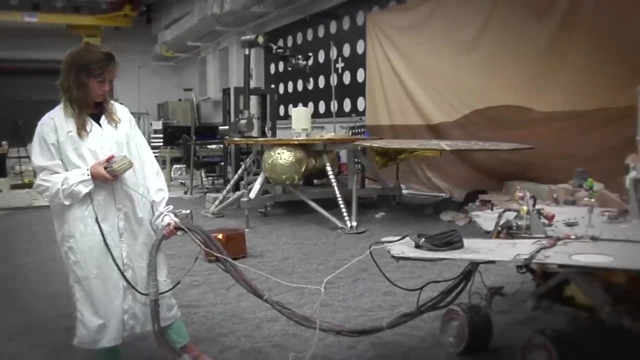 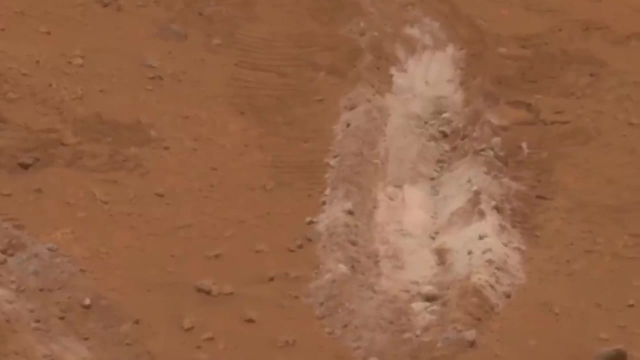 basalt on Earth. When Spirit's right front wheel stopped working, engineers used a duplicate rover to devise a reversing technique that enabled the rover to drag its frozen wheel. This was the first time the rover was used in a geological study. This left a furrow behind in the soil, which presented a new area of research for the science. 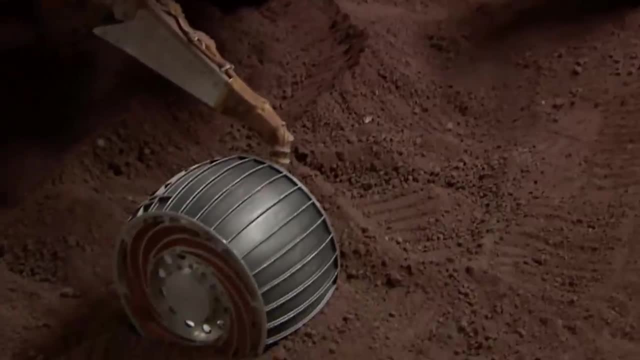 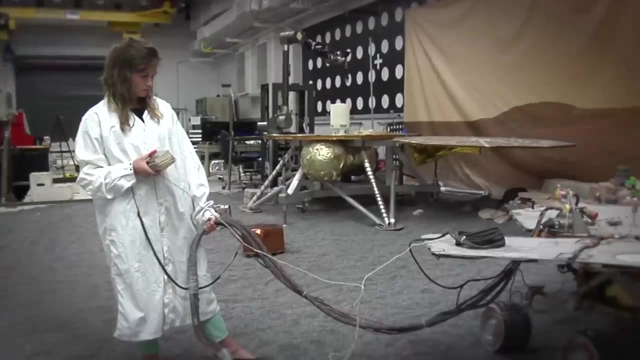 When Spirit's right front wheel stopped working, engineers used a duplicate rover to devise a reversing technique that enabled the rover to drag its frozen wheel. This left a furrow behind in the soil, which presented a new area of research for the science team. 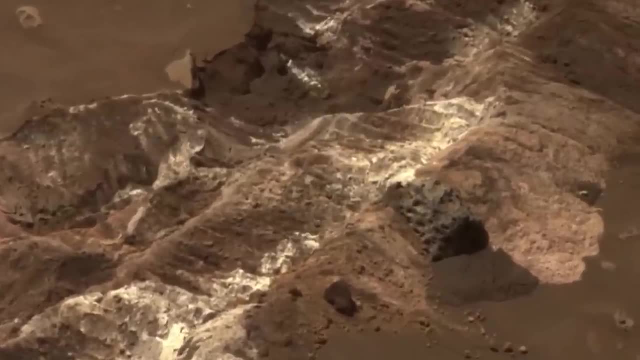 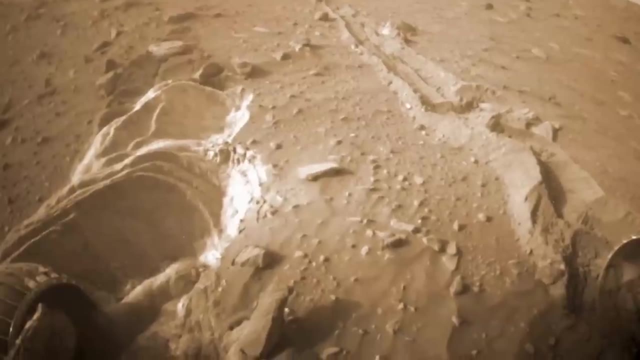 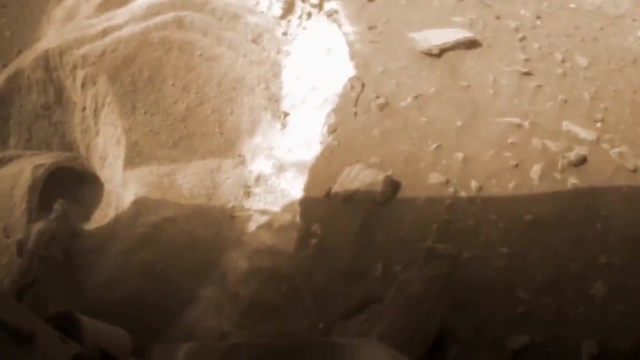 White or yellow deposits seen within the furrow were various types of salts that only form in the presence of hot water. The deposits were then transferred to the surface of hot water On Earth. hot water provides an environment in which microbes can thrive. Spirit limped on for another three years. 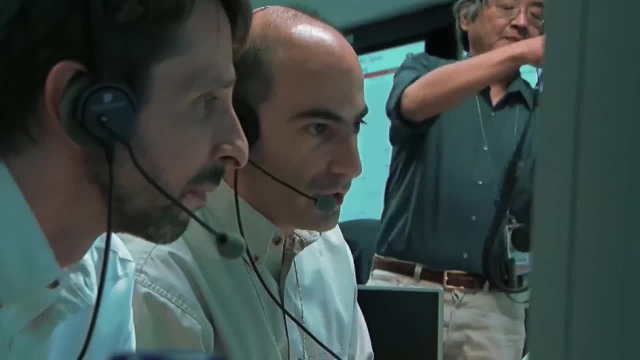 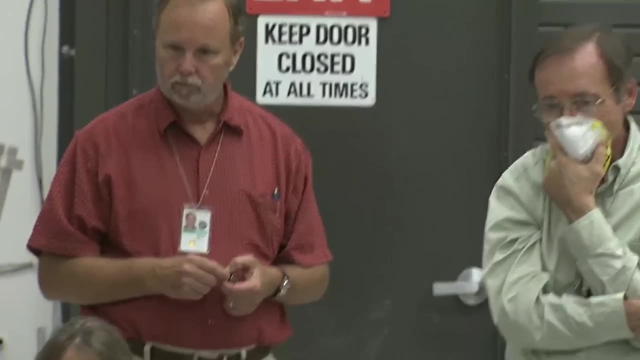 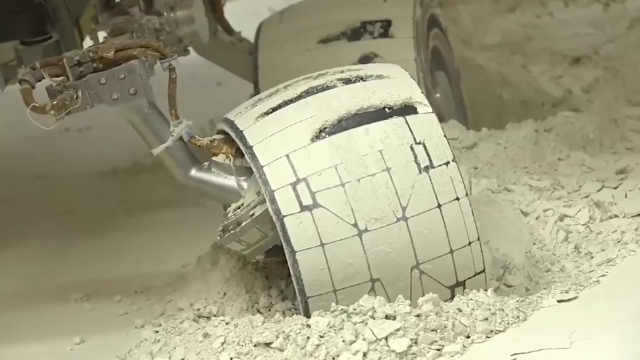 before it became stuck in loose sand Again, the engineers began working with a replica, which they placed in an identical situation. When nothing was able to free the rover, it was declared a stationary research platform. Further attempts were made to position the rover so its solar panels could operate more effectively. 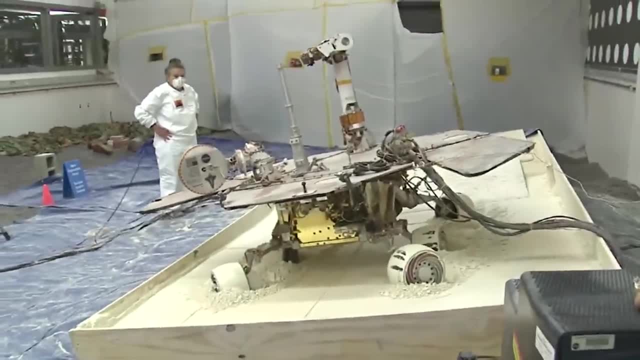 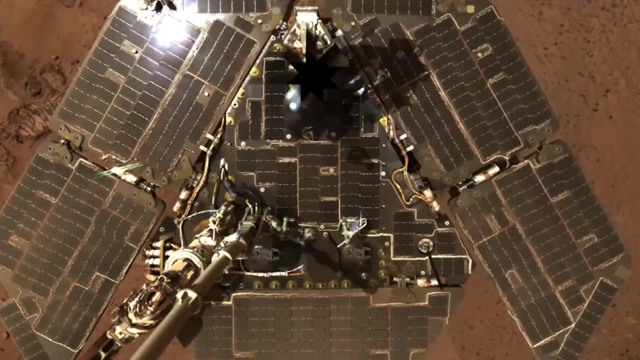 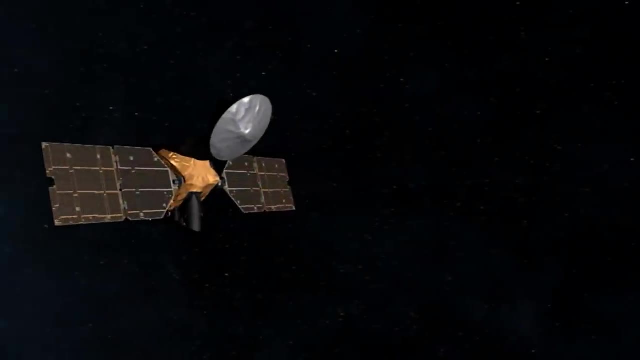 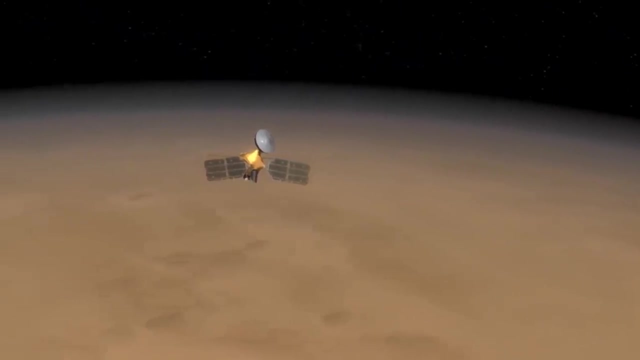 but even this was not possible. The last communication from Spirit was in March 2010.. Opportunity lasted until June 2018, when dust clogged its solar panels. In March 2006,, NASA's Mars Reconnaissance Orbiter arrived at Mars and began the now routine business. 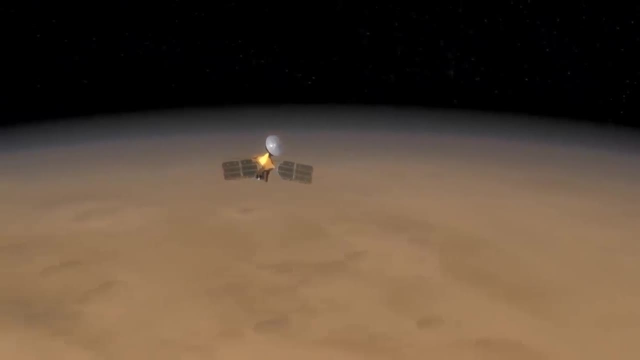 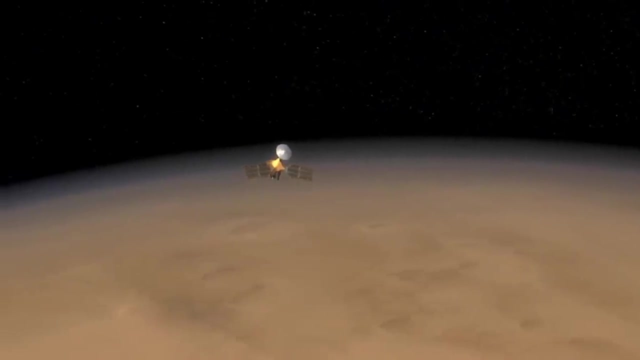 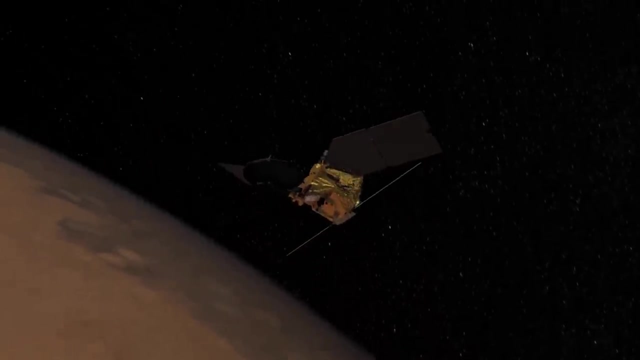 of aerobraking. Though this procedure took roughly six months, the saving in fuel will see the craft functioning at Mars into the 2030s. One of the primary functions of the new orbiter is as a communications relay station. Its three-meter antenna transmitting 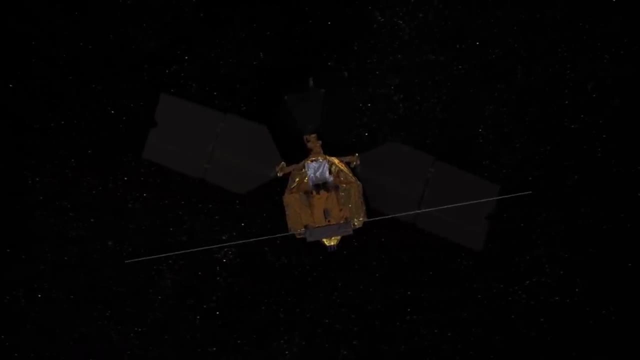 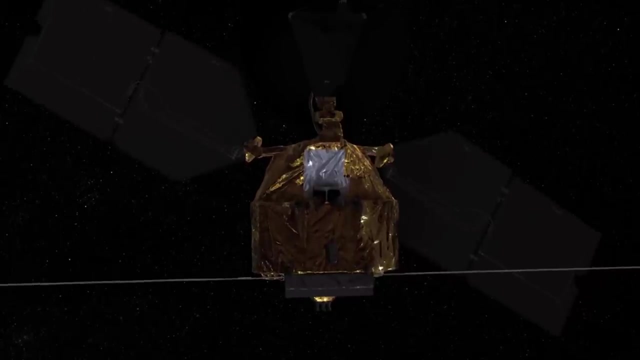 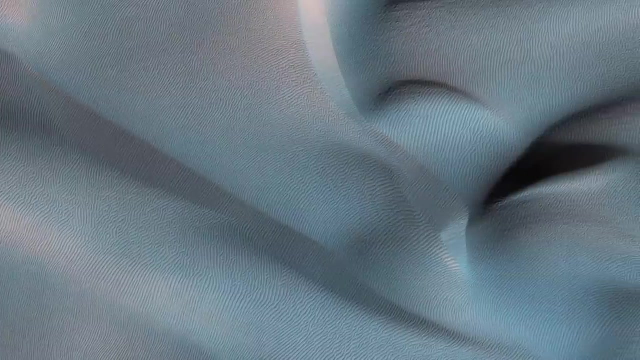 in the ultra-high frequency band enables very high data rates. By November 2013, it had tripled the amount of data sent to Earth by all the other NASA missions combined. Its high-resolution camera began revealing the surface of Mars in the finest detail. 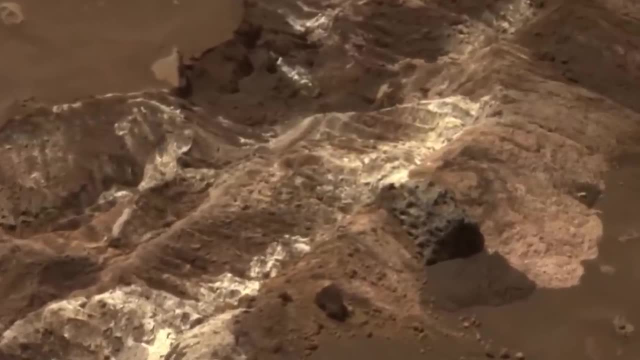 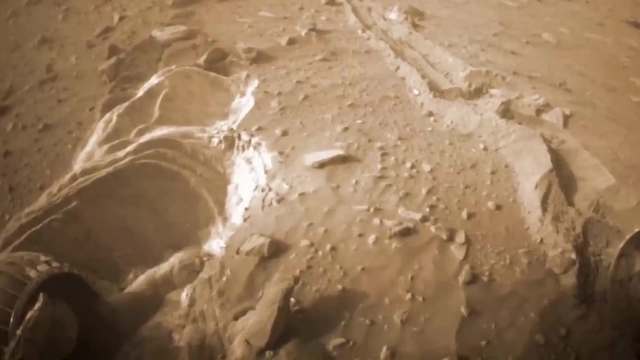 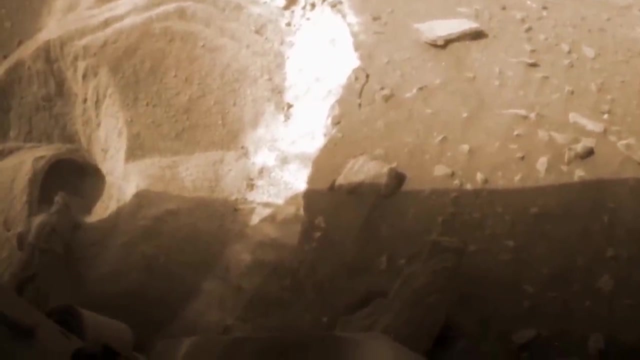 team. White or yellow deposits seen within the furrow were various types of salts that only form in the presence of hot water On Earth. hot water provides an environment in which microbes can thrive. Spirit limped on for another three years before it became stuck in loose sand. 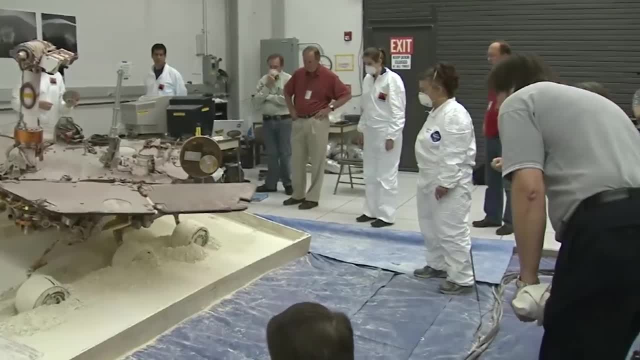 This was the first time the rover was used in a geological study. It was the first time the rover was used in a geological study. It was the first time the rover was used in a geological study. This was the first time the rover was used in a geological study. 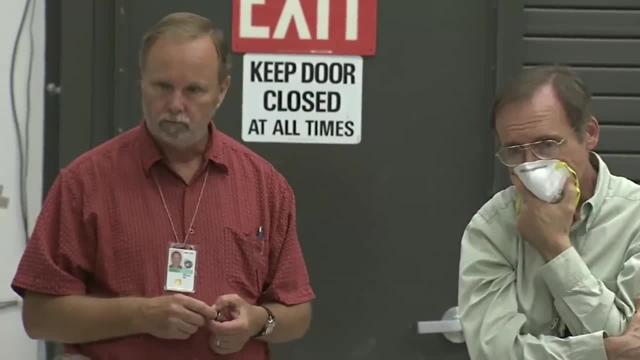 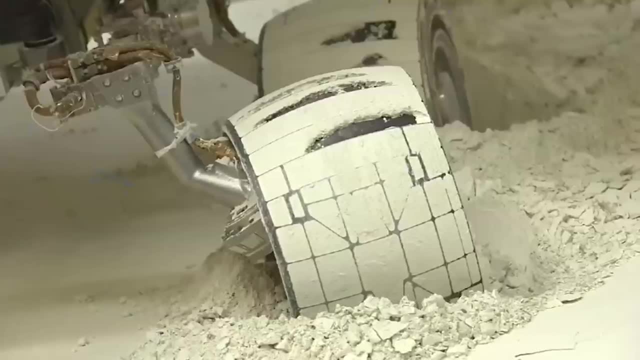 This was the first time the rover was used in a geological study. Again, the engineers began working with a replica, which they placed in an identical situation. When nothing was able to free the rover, it was declared a stationary research platform. Further attempts were made to position the rover so its solar panels could operate more. 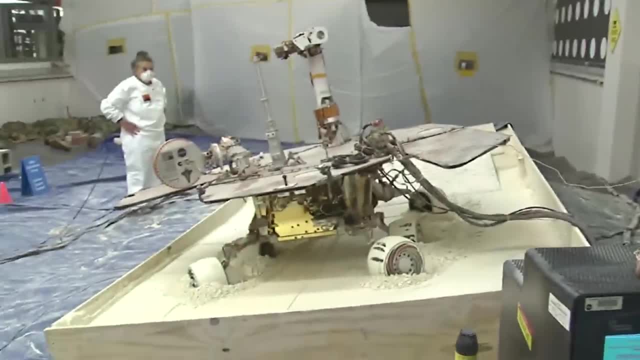 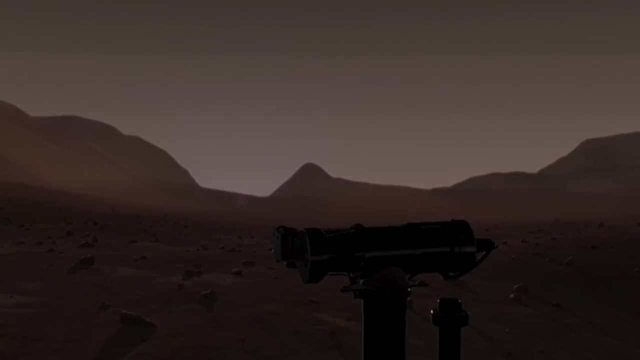 effectively. but even this was not possible. The last communication from Spirit was in March 2010.. Opportunity lasted until June 2018, when dust and air had entered the rover. The rover was now working just as well, but with an email. 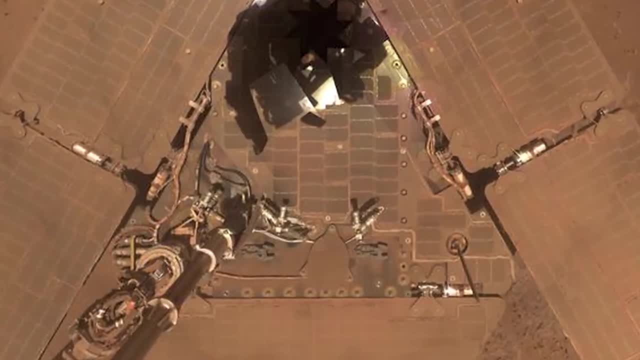 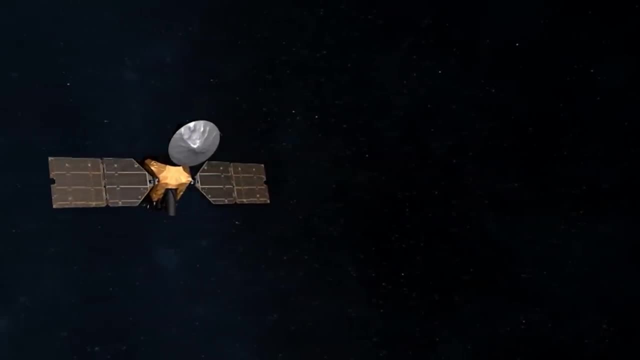 The probe were still out in search. Here's the list of UFOs. in September, This 왔 Dastur's report clogged its solar panels. In March 2006, NASA's Mars Reconnaissance Orbiter arrived at Mars and began the now. 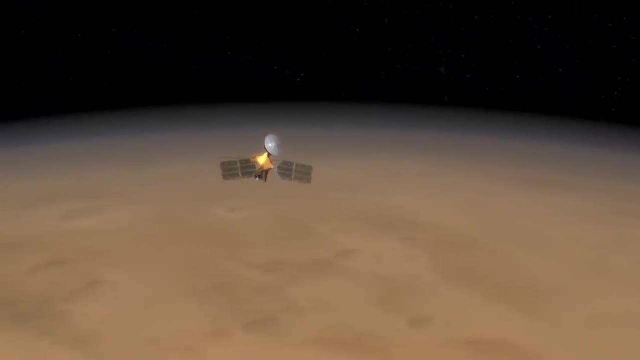 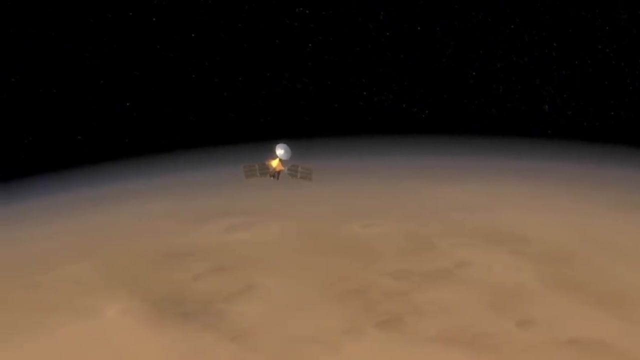 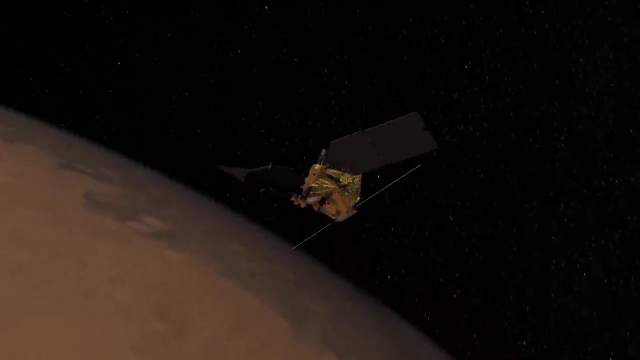 routine business of aerobraking. Though this procedure took roughly six months, the saving in fuel will see the craft functioning at Mars into the 2030s. One of the primary functions of the new orbiter is as a communications relay station. 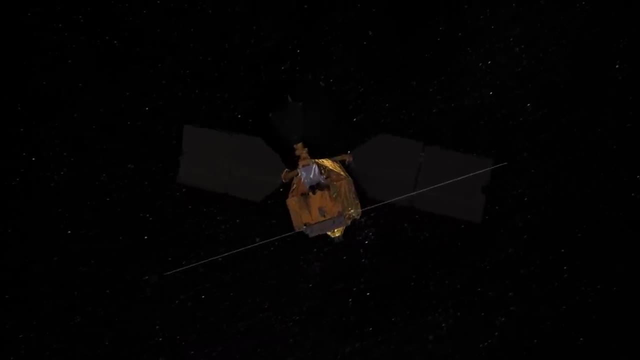 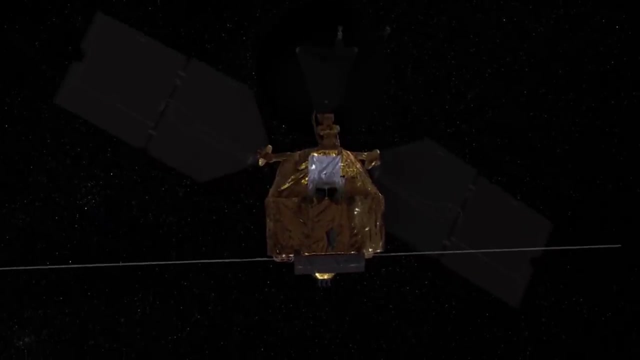 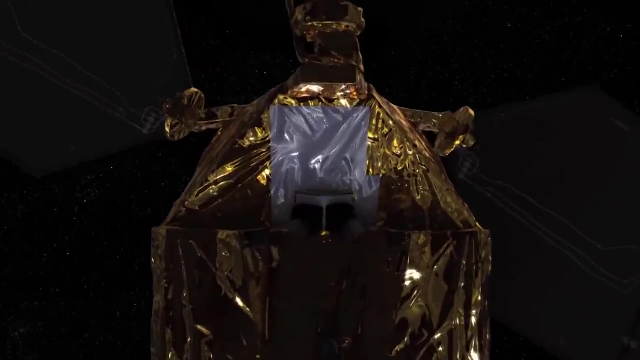 Its three-meter antenna, transmitting in the ultra-high frequency band, enables very high data rates. By November 2013, it had tripled the amount of data sent to Earth by all the other NASA missions combined. Its high-resolution camera began revealing the surface of Mars in the finest detail. 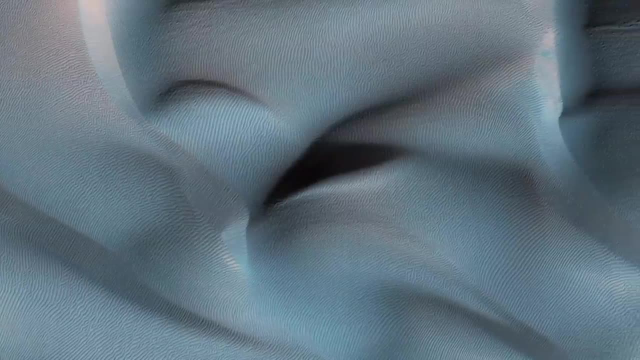 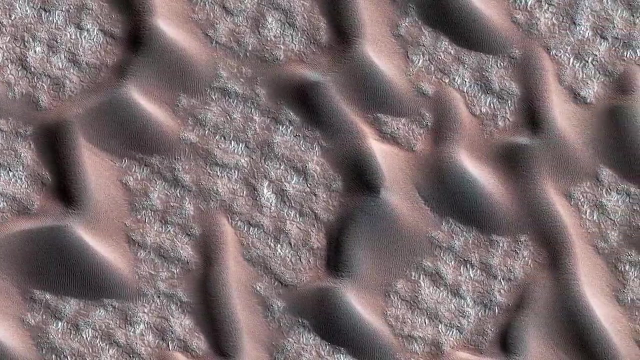 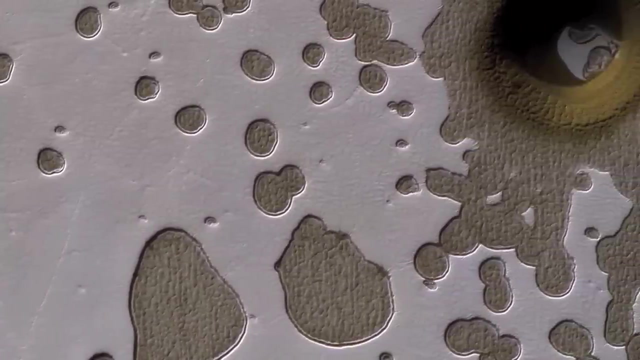 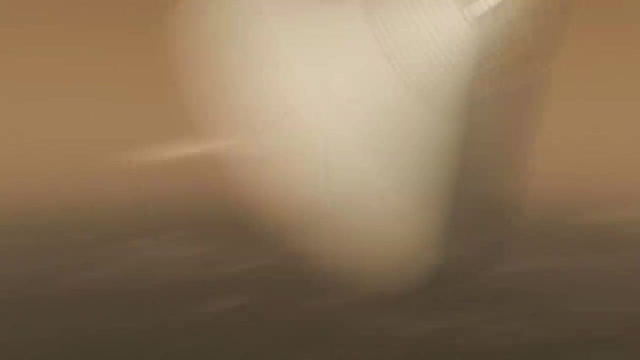 These are active falling dunes in East Coprates, Chasma, The polar region free of the seasonal dry ice, again surrounded by dunes. In the southern hemisphere pits in the residual cap of carbon dioxide, The poles of Mars were now attracting keen interest. 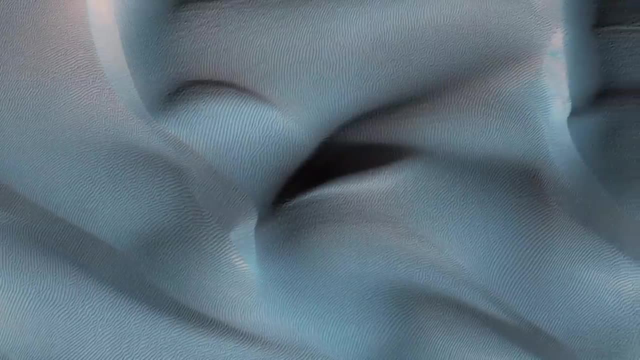 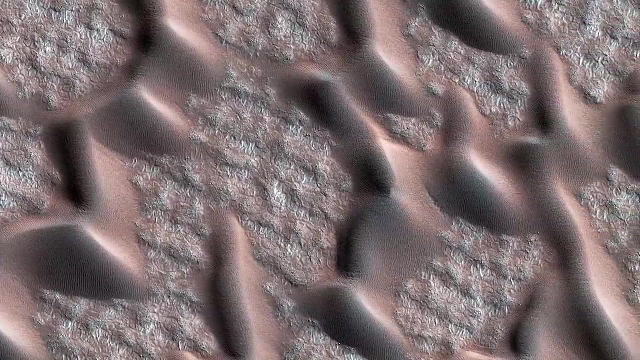 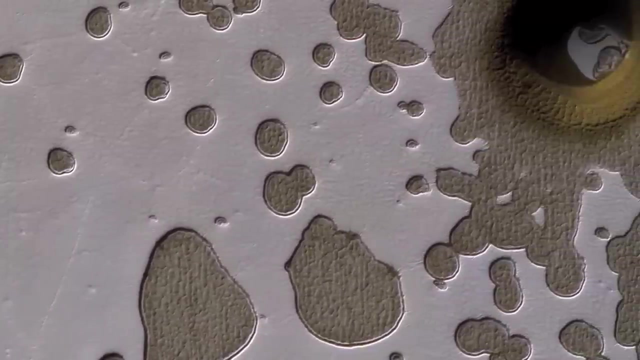 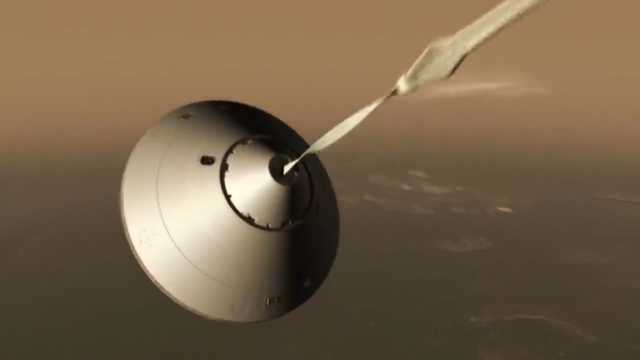 These are active falling dunes in East Coprates, Chasma, the polar region free of the seasonal dry ice, again surrounded by dunes. In the southern hemisphere pits in the residual cap of carbon dioxide, The poles of Mars were now attracting keen interest. 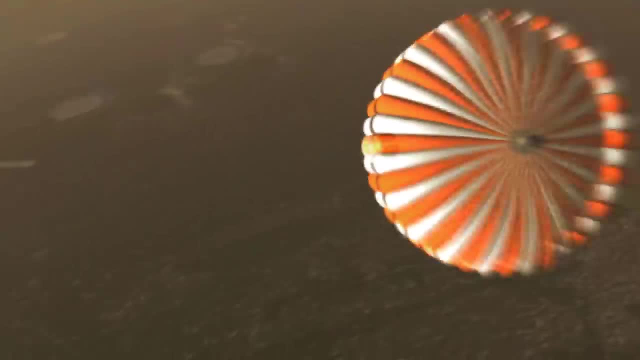 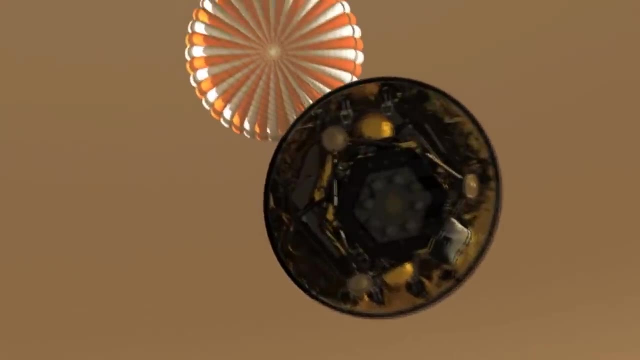 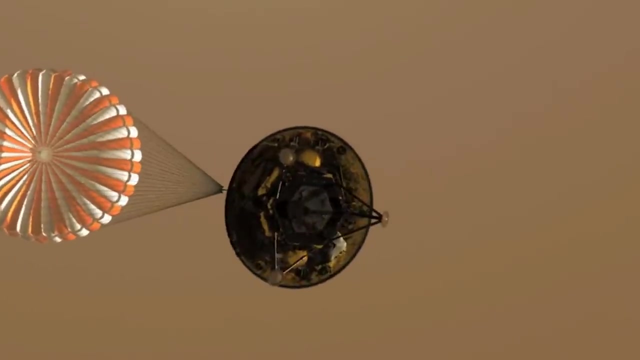 Follow the Water had become NASA's catch cry. The Phoenix lander was targeted at the northern polar region To follow up on information from Mars Odyssey suggesting frozen water lay beneath the surface near the poles, Because imaging had revealed the region to be unvarying. 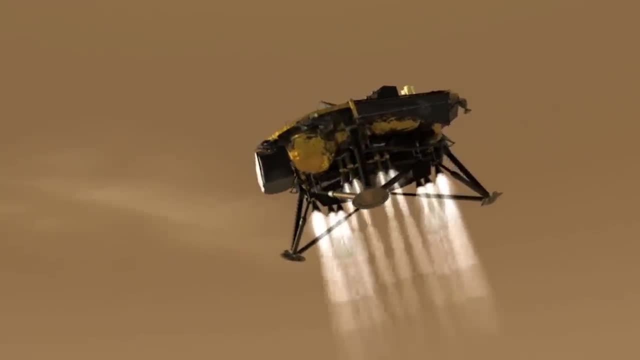 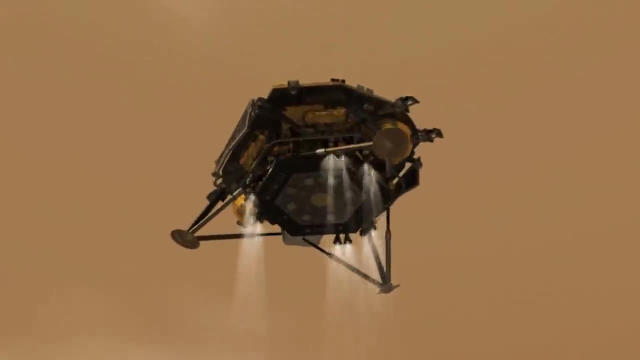 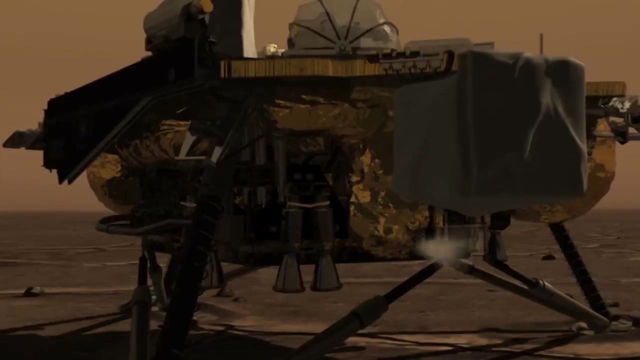 a rover was deemed unnecessary. The lander had been designed to use a parachute to decelerate with rocket thrusters to deliver the craft to the surface, unlike NASA's previous three rovers which had bounced. This decision proved controversial, as one strand of research suggested the rocket fuel 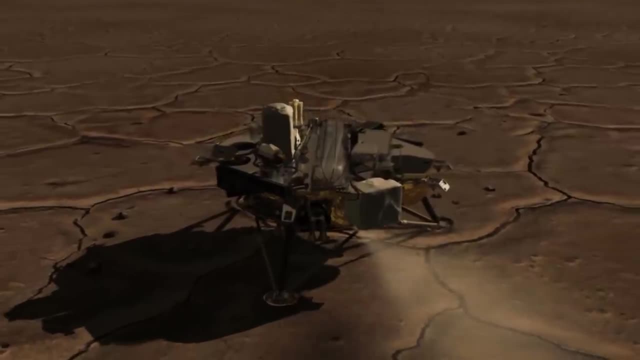 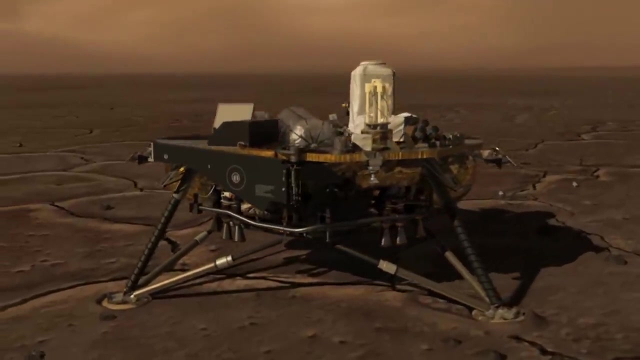 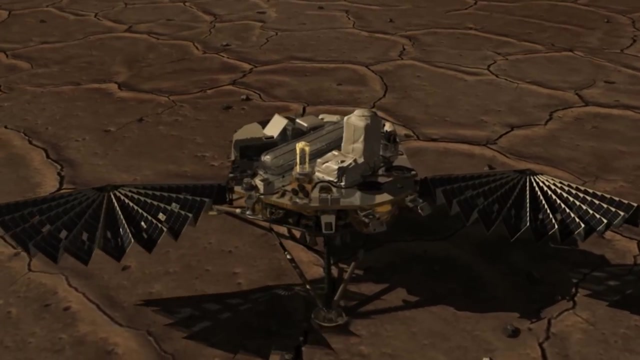 would contaminate the very area that the lander was tasked with analysing. The craft waited 15 minutes to allow any dust to settle before it deployed its solar panels. Phoenix had landed during the early spring in Mars' northern hemisphere, so the solar panels would receive plenty of light. 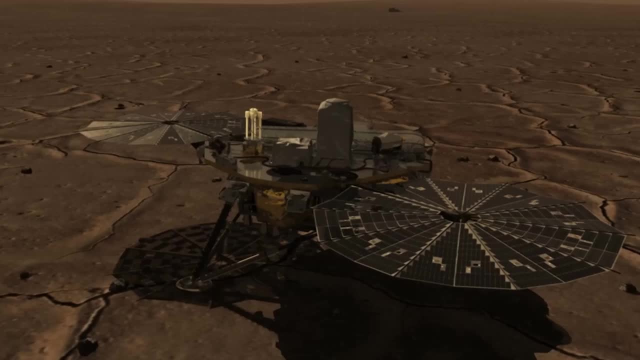 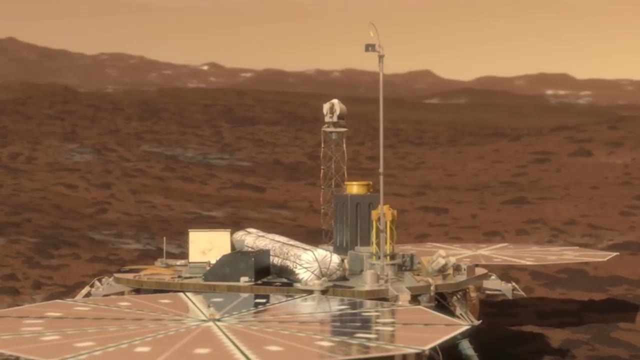 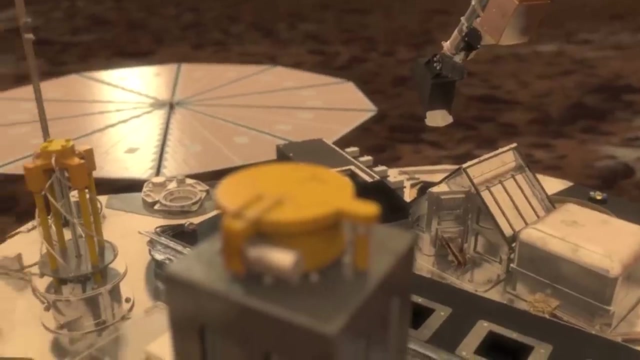 for the planned 90-day mission. As well as its camera, mast Phoenix was equipped with a meteorological station that recorded the daily weather. It featured a wind indicator and pressure and temperature sensors. In addition, a vertically-pointed LiDAR was able to observe cirrus clouds forming in the region. 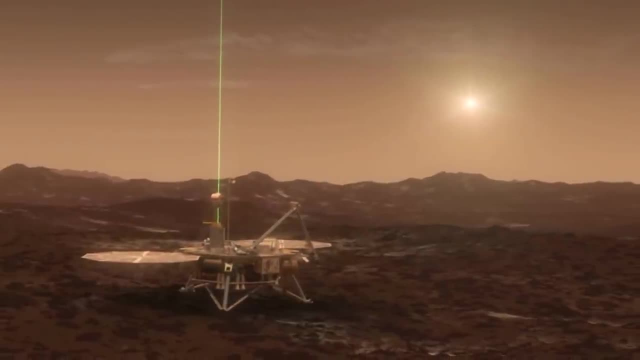 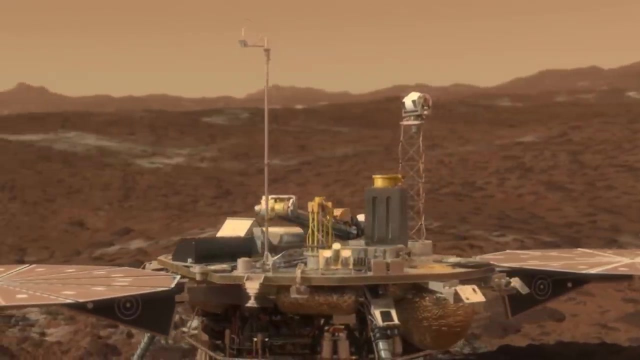 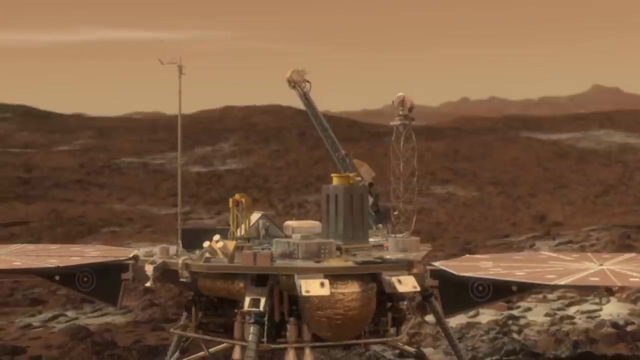 and snow falling in the polar atmosphere. These phenomena had not been observed before. The lander also had a robotic arm that could dig half a metre into the soil and deliver samples to the analyser, a combination of eight high-temperature ovens and a mass spectrometer. 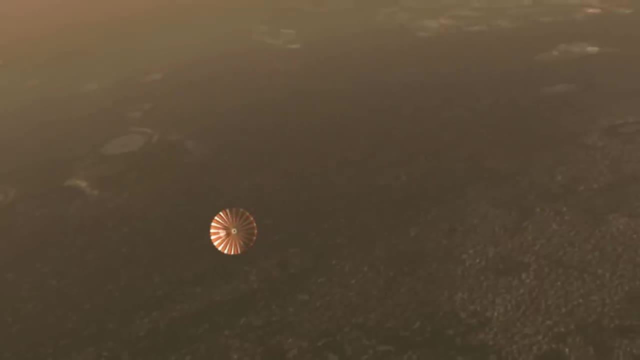 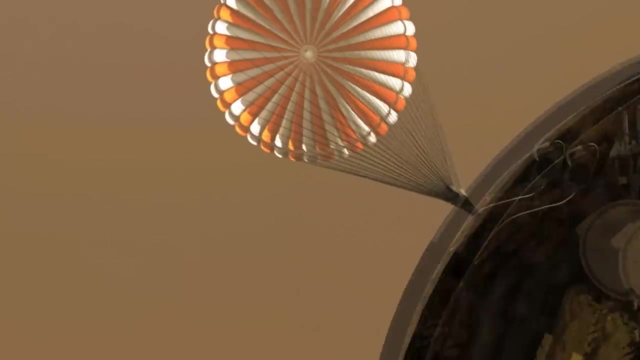 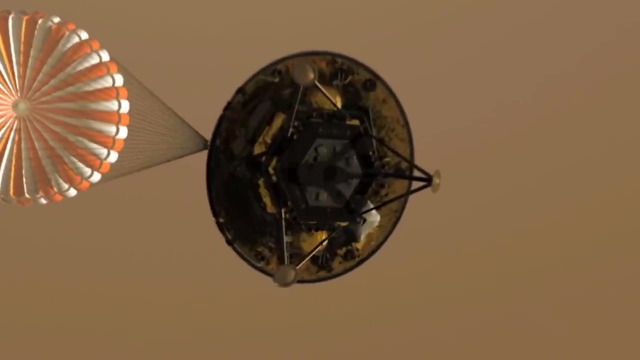 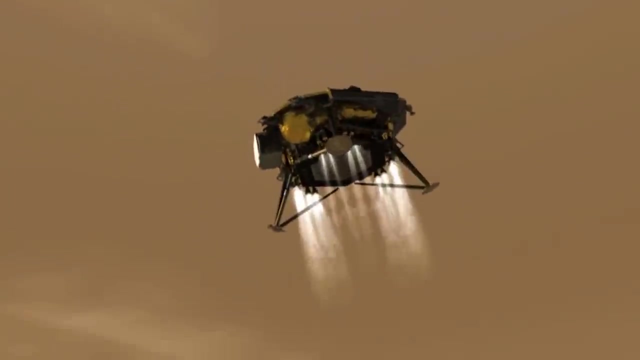 Follow the water had become NASA's catch cry. The Phoenix lander was targeted at the northern polar region To follow up on information from Mars Odyssey suggesting frozen water lay beneath the surface near the poles. Because imaging had revealed the region to be unvarying, a rover was deemed unnecessary. 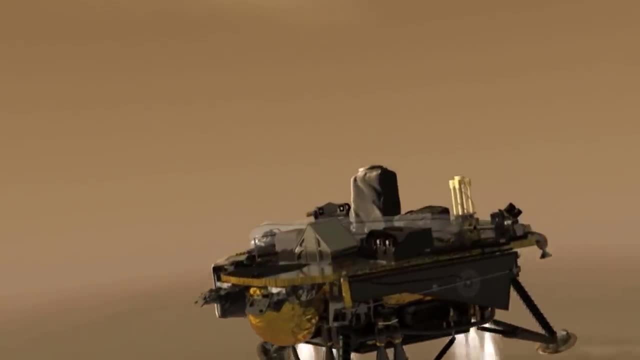 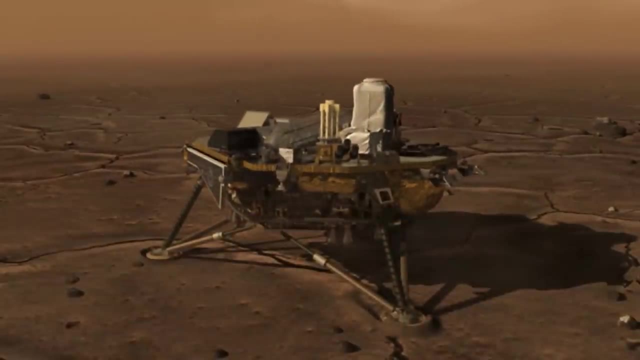 The lander had been designed to use a parachute to decelerate. The landing had been designed to use a parachute to decelerate With rocket thrusters to deliver the craft to the surface, unlike NASA's previous three rovers, which had bounced. 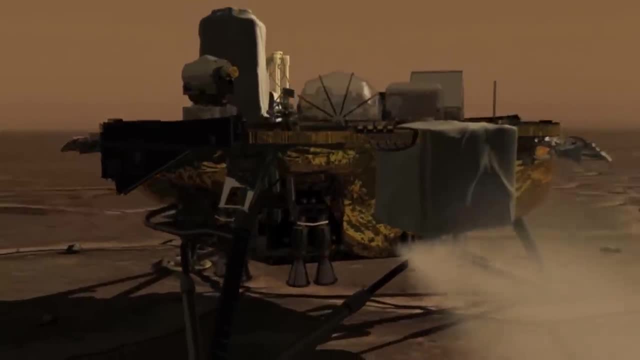 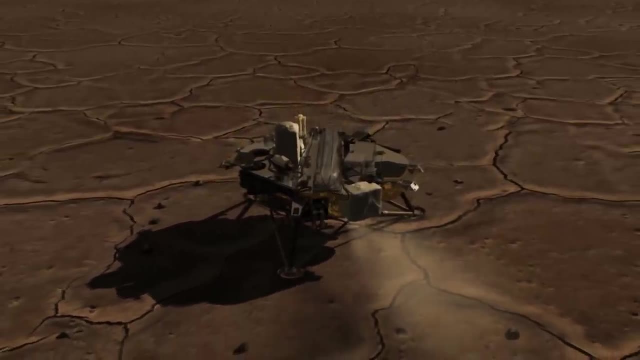 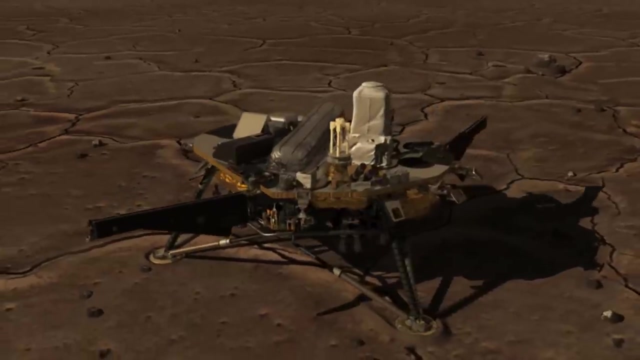 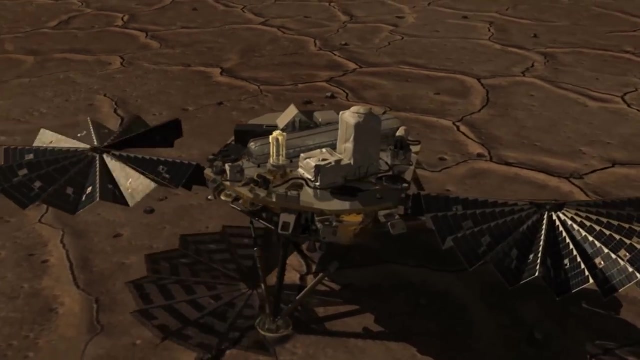 This decision proved controversial as one strand of research suggested the rocket fuel would contaminate the very area that the lander was tasked with analyzing. The craft waited 15 minutes to allow any dust to settle before it deployed its solar panels. Phoenix had landed during the early spring in Mars' northern hemisphere. 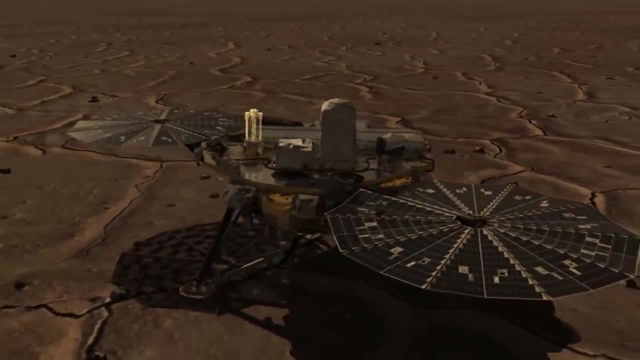 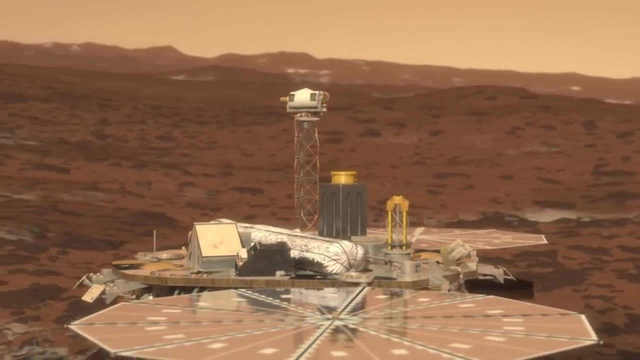 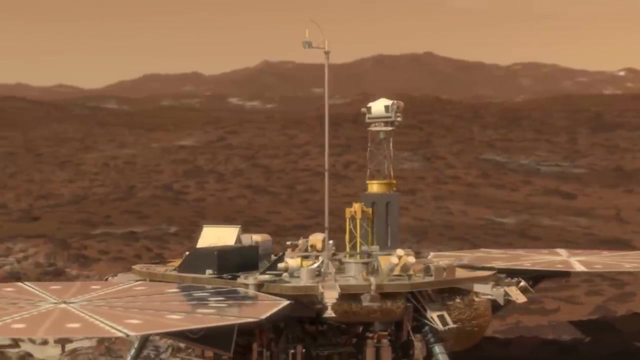 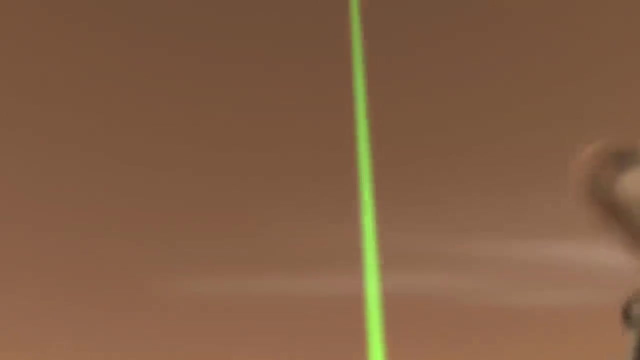 so the solar panels would receive plenty of light for the planned 90-day mission. As well as its camera, mast Phoenix was equipped with a meteorological station that recorded the daily weather. It featured a wind indicator and pressure and temperature sensors. In addition, a vertically pointed lidar was able to observe cirrus clouds forming in the region. 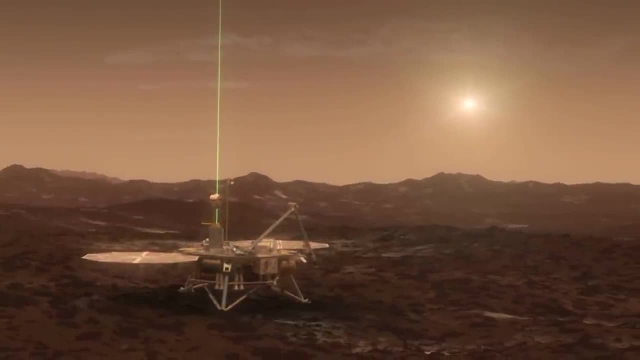 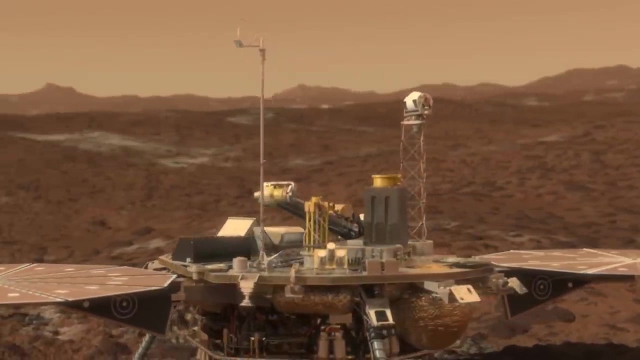 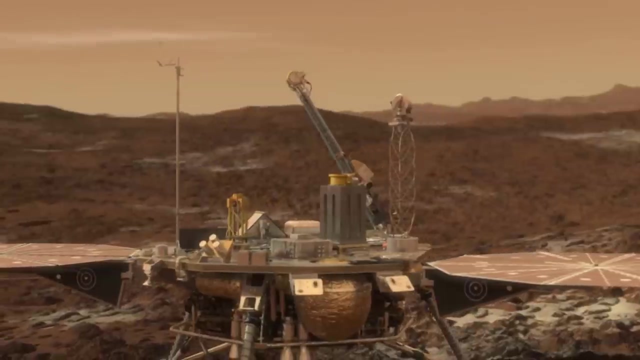 and snow falling in the polar atmosphere. These phenomena had not been observed before. The lander also had a robotic arm that could dig half a metre into the soil and deliver samples to the analyser, a combination of eight high-temperature ovens and a mass spectrometer. 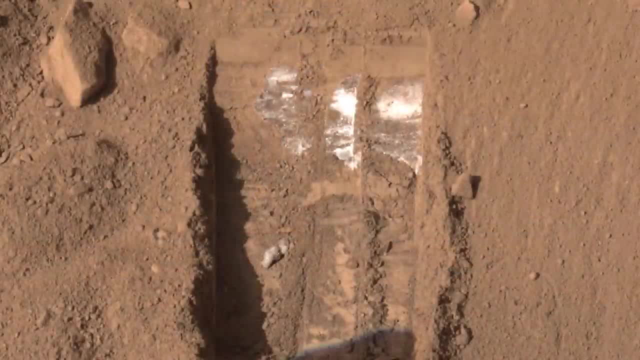 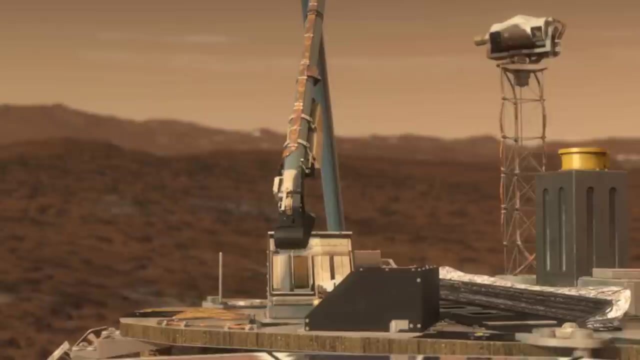 In one excavation, the cameras recorded a white substance which gradually disappeared. Given the temperatures and the time it lasted, it could only have been water ice that sublimated after it was exposed. The soil was slightly alkaline and the presence of perchlorate, which kills bacteria. 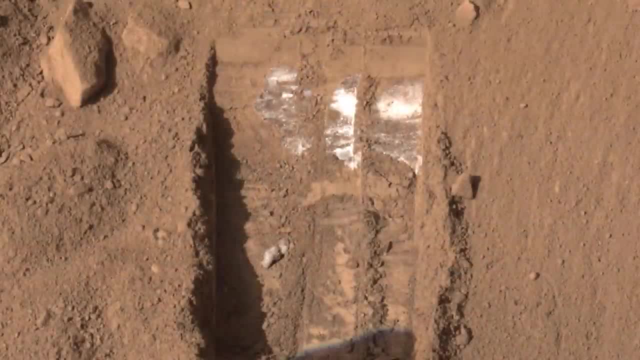 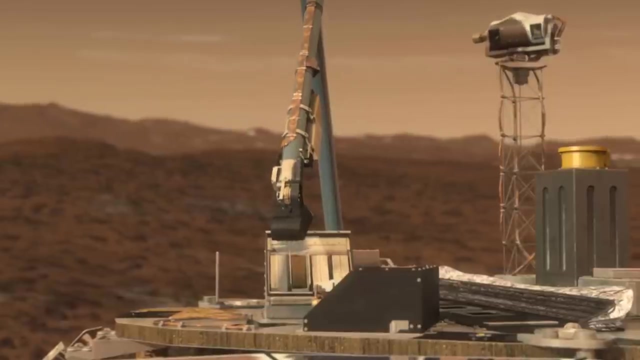 In one excavation, the cameras recorded a white substance which gradually disappeared. Given the temperatures and the time it lasted, it could only have been water ice that sublimated after it was exposed. The soil was slightly alkaline and the presence of perchlorate. 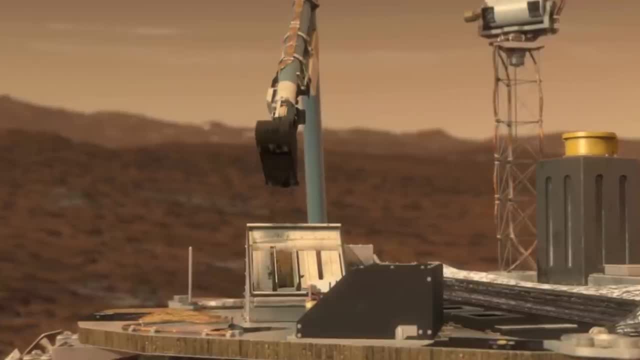 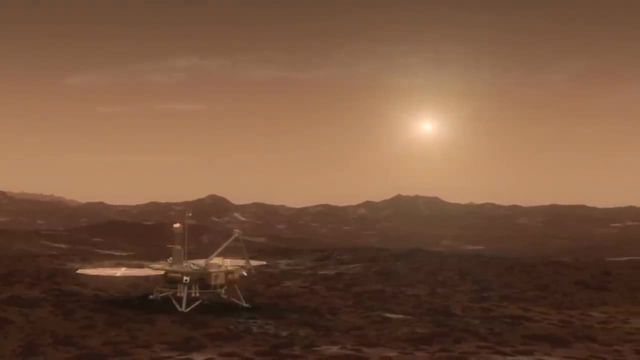 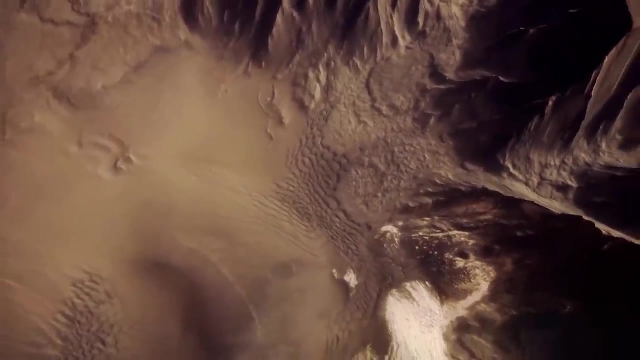 which kills bacteria, was not good news for those hoping for Martian life. Phoenix operated for two months longer than planned before the gathering winter completely shaded its solar panels. While the planet still had subterranean deposits of ice, there was precious little left at the surface. 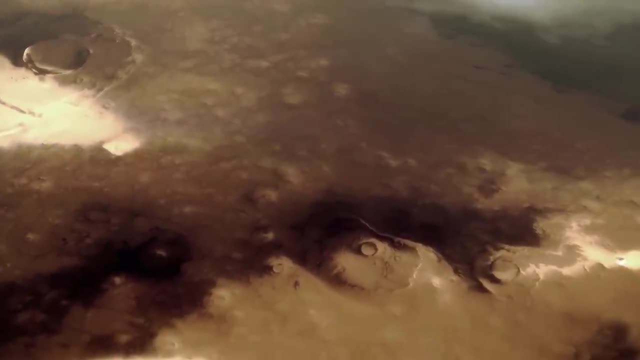 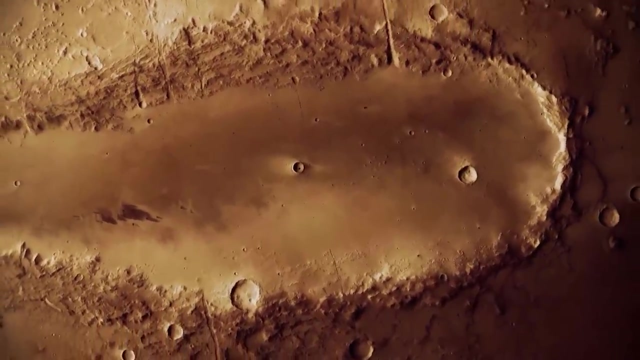 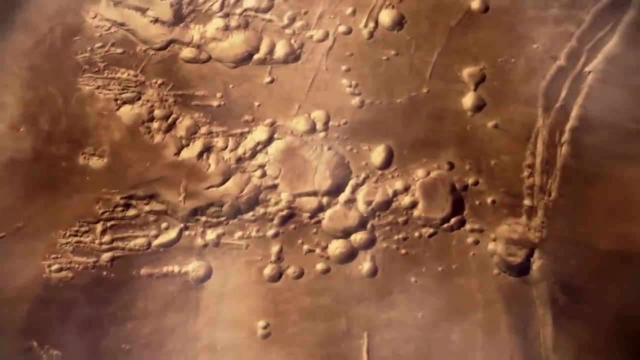 yet it was now understood that many of the red planet's features had been carved by running water. Samples analysed from across the planet affirmed that water and nothing else had made these changes to the Martian landscape. Mars had once been more like Earth. 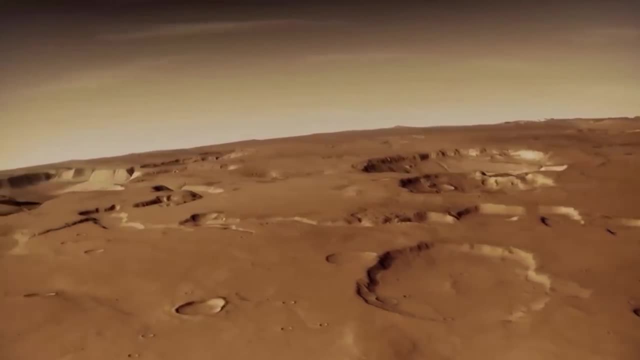 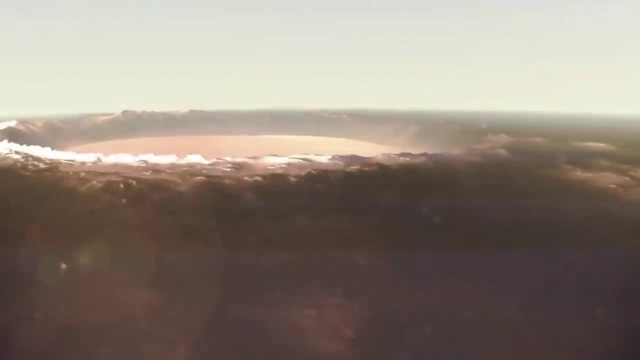 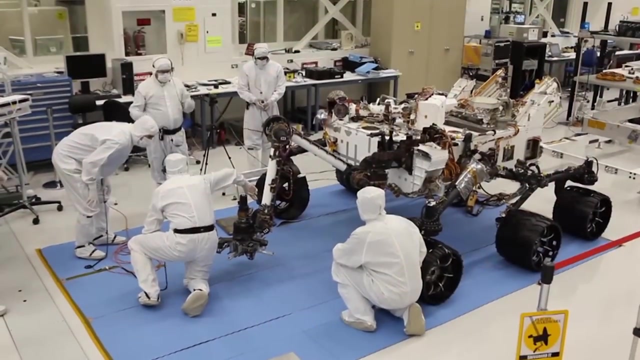 yet it had lost its surface water and most of its atmosphere, and the question of life persisted. Could it have emerged in a world where it could have been in a warmer, wetter past, And could it still be present below the surface? The next Mars mission would be NASA's most ambitious yet. 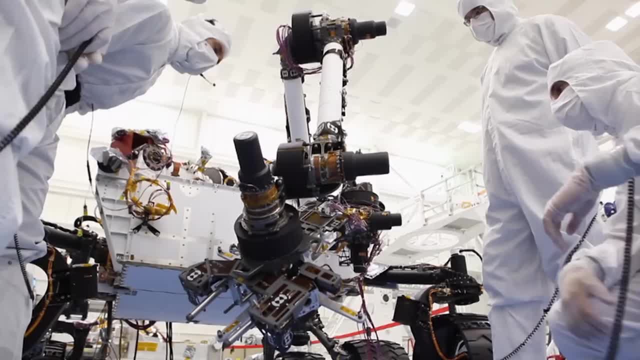 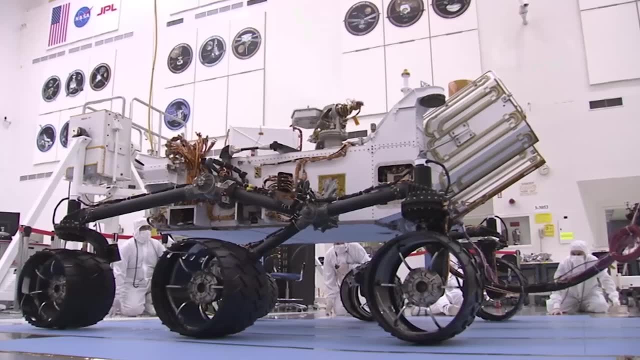 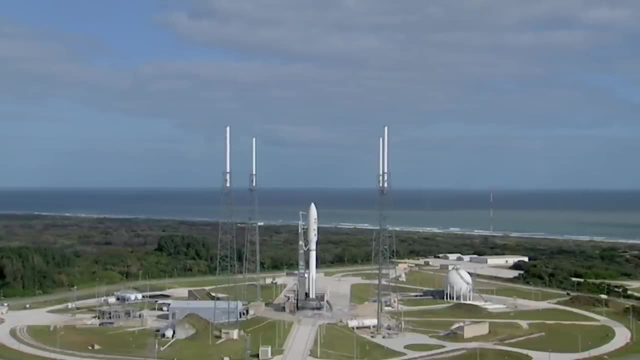 Known as Curiosity. the car-sized rover would be powered by a nuclear battery, making it immune to the dust problems experienced by Spirit and Opportunity. Curiosity was launched on an Atlas V from Cape Canaveral in November 2011.. In mid-2012, it entered the Martian atmosphere. 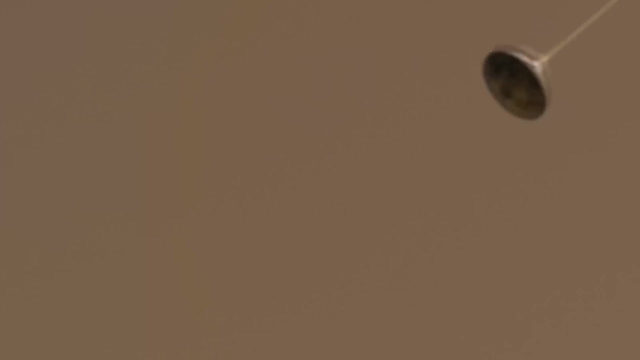 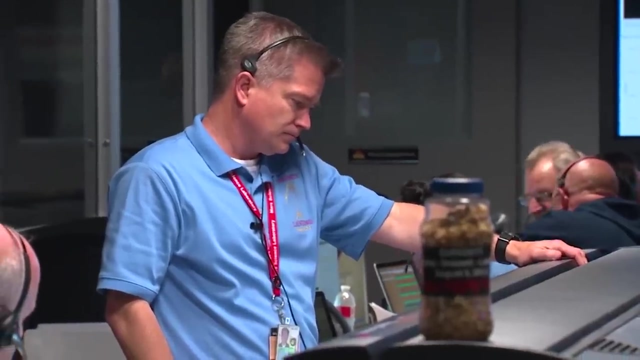 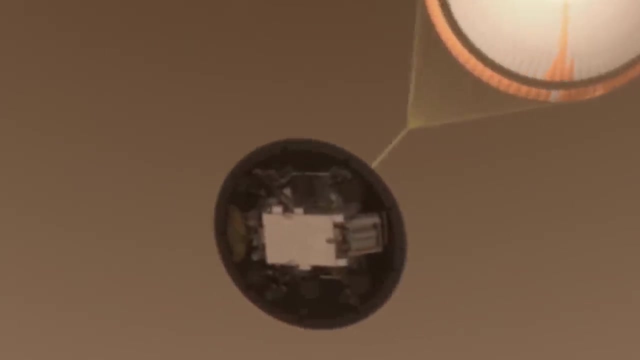 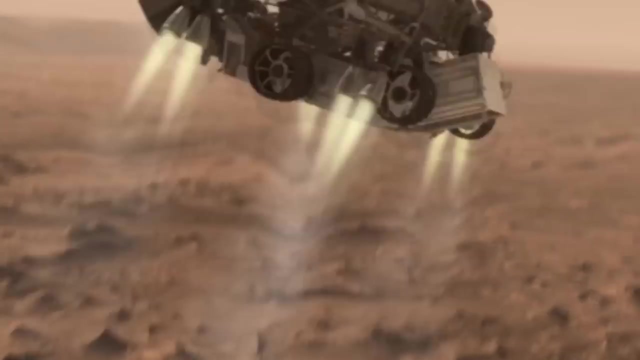 heading for Gale Crater. The Jet Propulsion Laboratory monitored the entry closely but had no control over events In Mars's thin atmosphere. the parachute could only slow the heavy craft to around 320 kilometres per hour, Nearing the surface the rover descent stage. 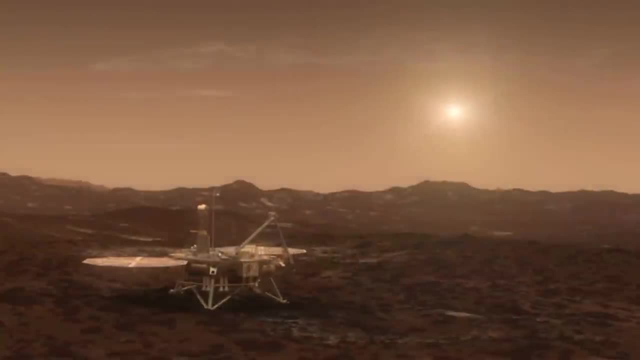 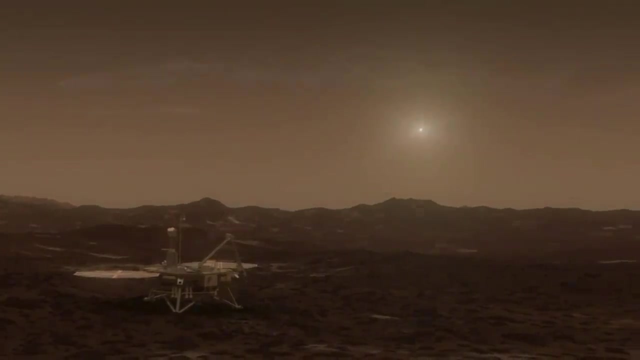 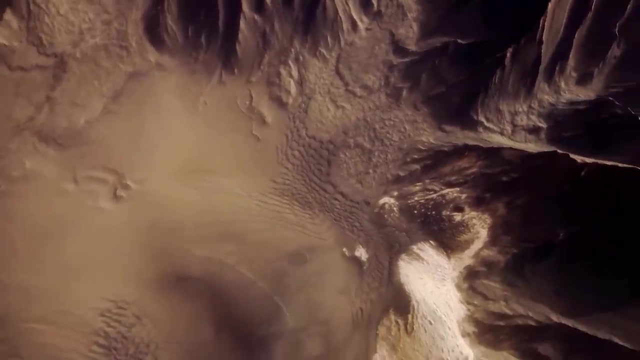 was not good news for those hoping for Martian life. Phoenix operated for two months longer than planned before the gathering winter completely shaded its solar panels. It was only a matter of time before the ice was completely gone, While the planet still had subterranean deposits of ice. 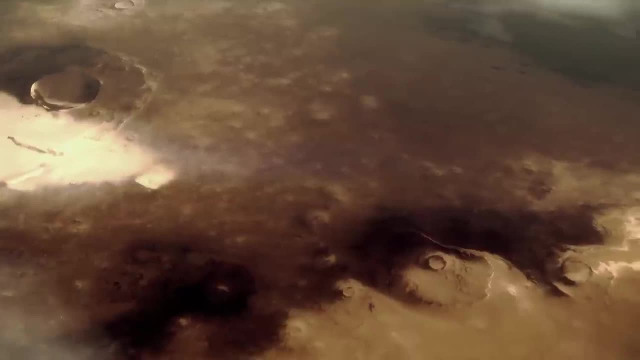 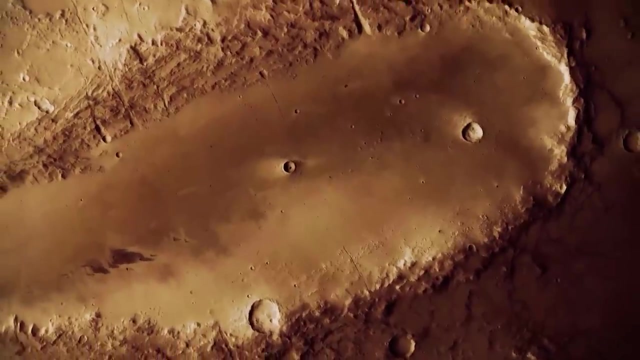 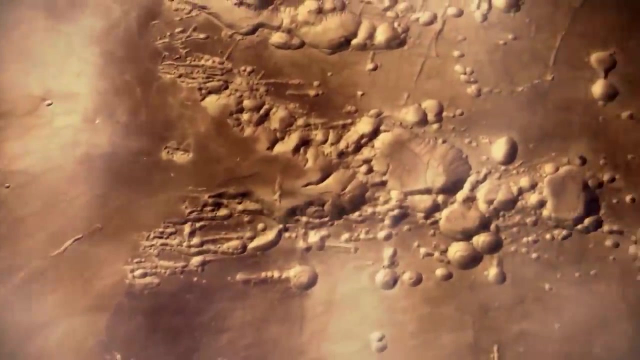 there was precious little left at the surface. Yet it was now understood that many of the red planet's features had been carved by running water. Samples analysed from across the planet affirmed that water and nothing else had made these changes to the Martian landscape. Mars had once been more like Earth. 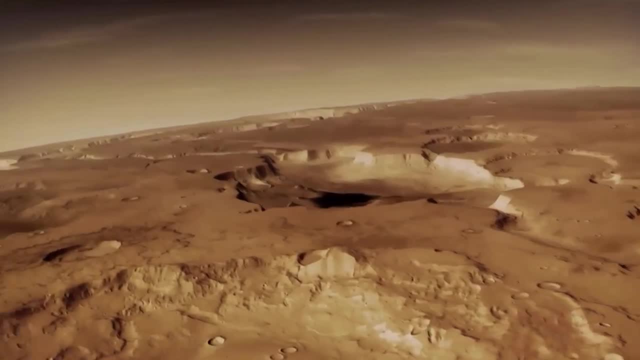 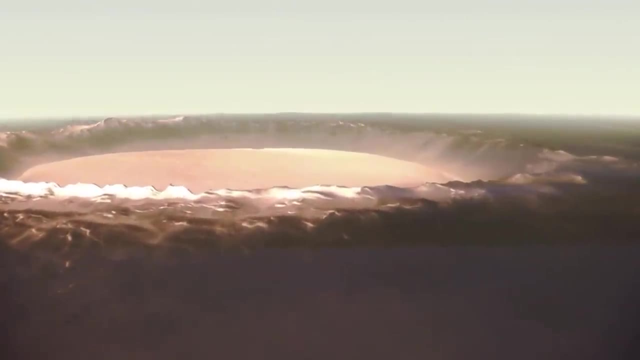 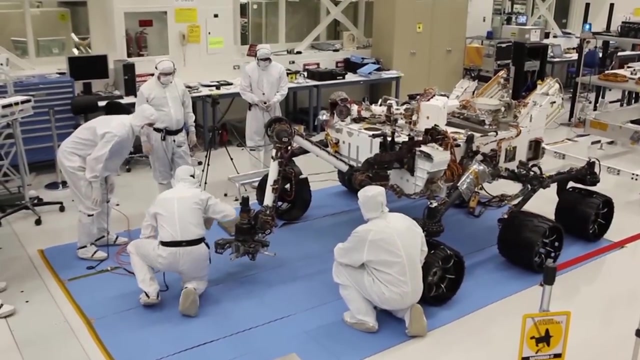 yet it had lost its surface water and most of its atmosphere, And the question of life persisted. Could it have emerged in a warmer wetter past, And could it still be present below the surface? The next Mars mission would be NASA's most ambitious yet. 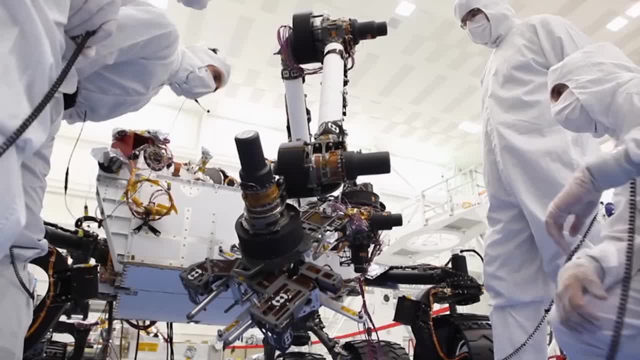 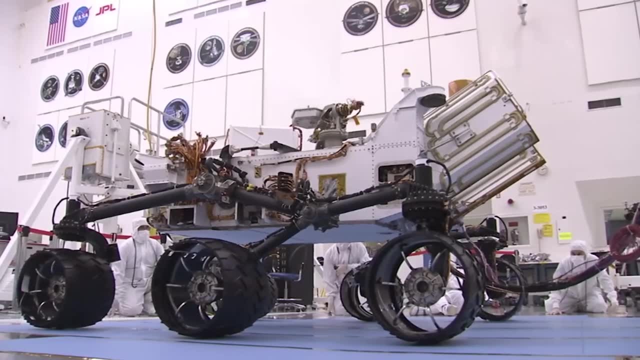 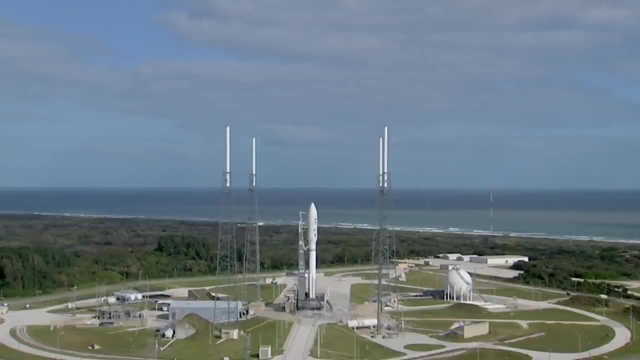 Known as Curiosity. the car-sized rover would be powered by a nuclear battery, making it immune to the dust problems experienced. It was influenced by spirit and opportunity. Curiosity was launched on an Atlas V from Cape Canaveral in November 2011.. 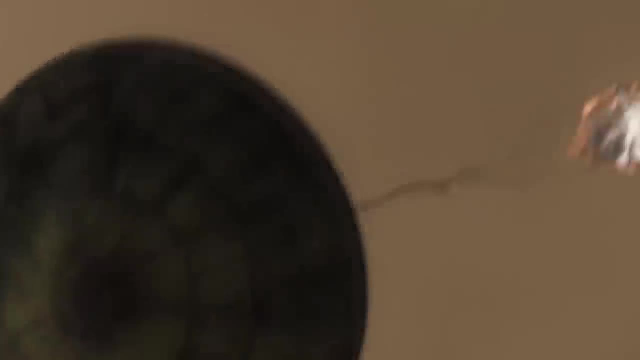 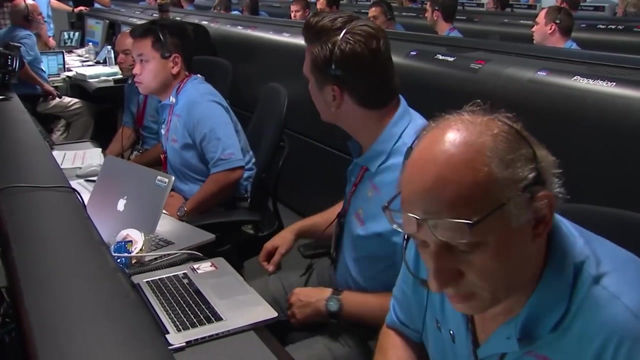 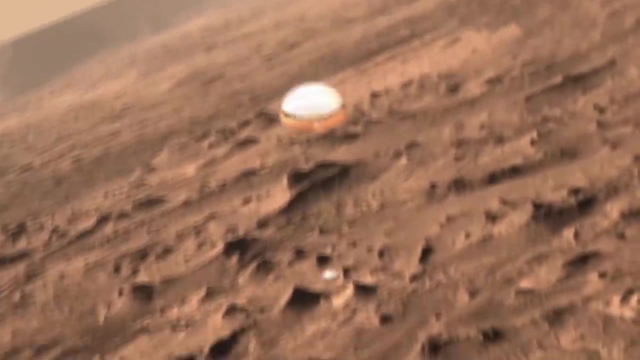 In mid-2012, it entered the Martian atmosphere heading for Gale Crater. The Jet Propulsion Laboratory monitored the entry closely but had no control over events In Mars's thin atmosphere. the parachute could only slow the heavy craft to around 320 km per hour. 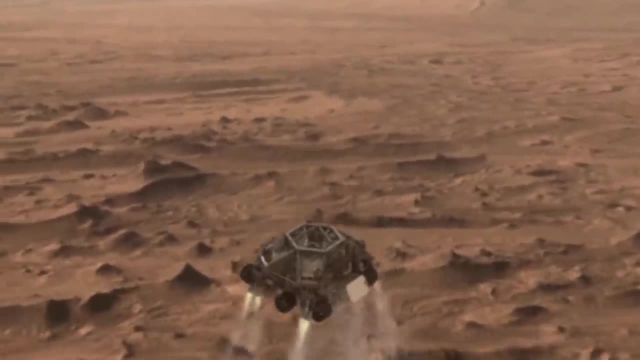 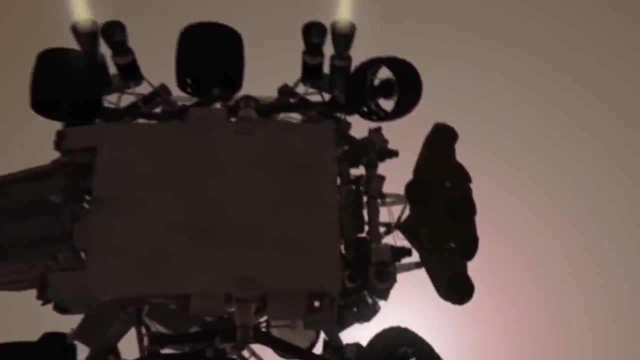 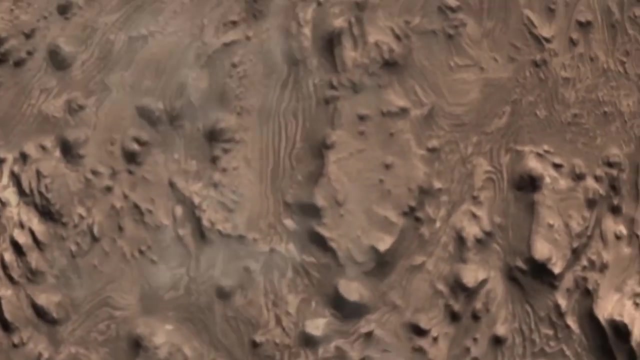 Nearing the surface, the rover descent stage dropped out of the aeroshell and rockets kicked in. At this stage, radar was guiding the lander to the surface and a small camera was recording images of the terrain below the rover. Next, Curiosity was lowered on a tether beneath the descent stage. 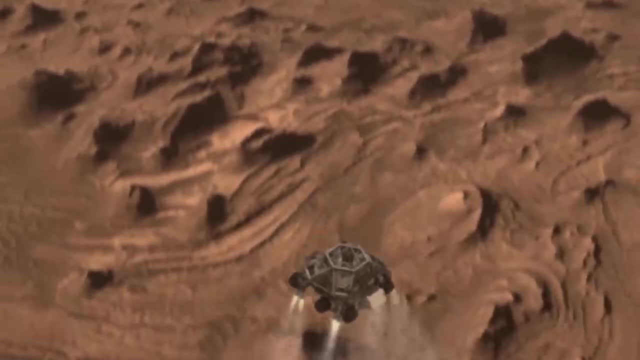 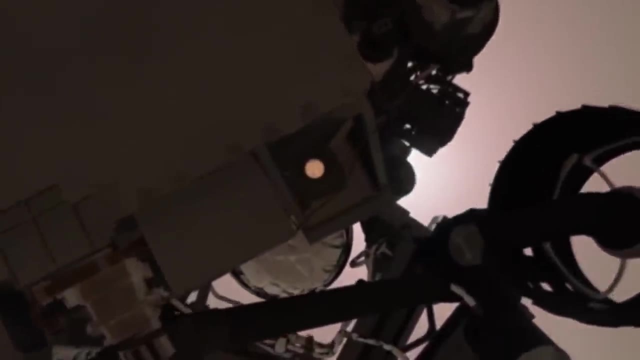 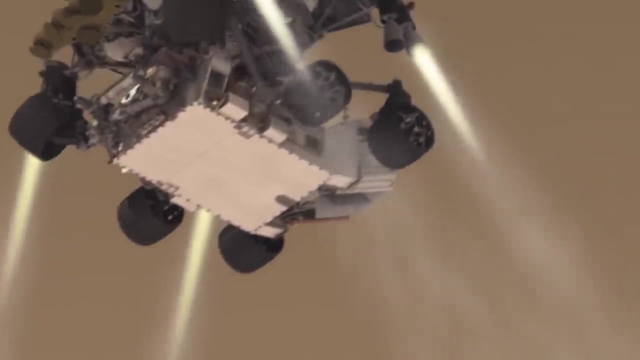 dropped out of the aeroshell and rockets kicked in. At this stage, radar was guiding the lander to the surface and a small camera was recording images of the terrain below the rover. Next, Curiosity was lowered on a tether beneath the descent stage. 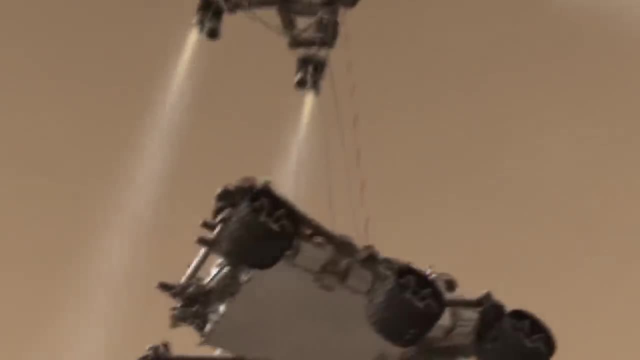 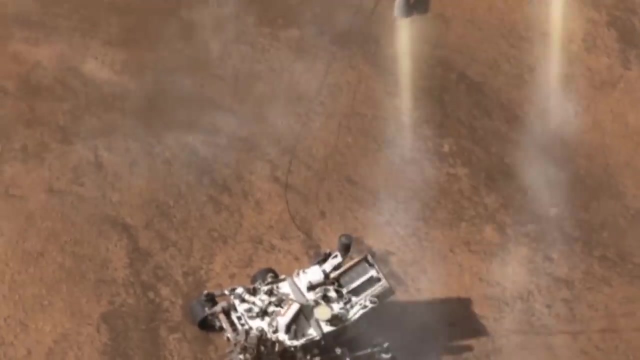 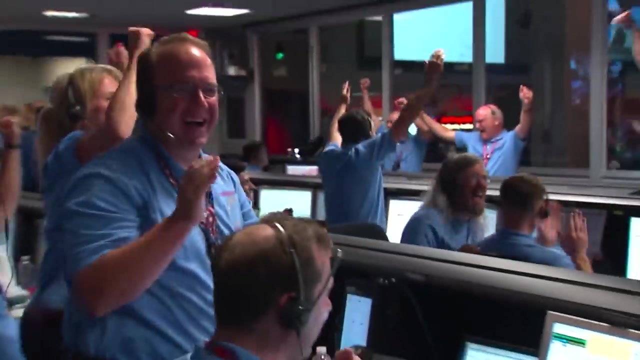 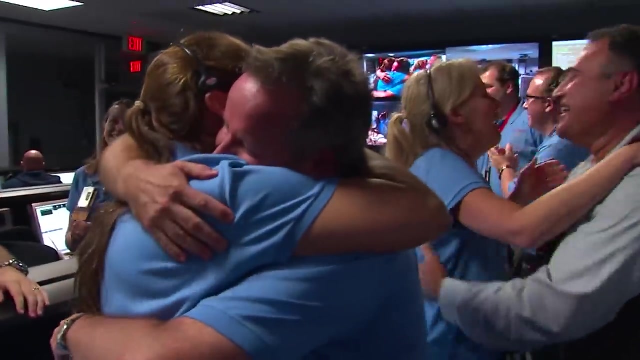 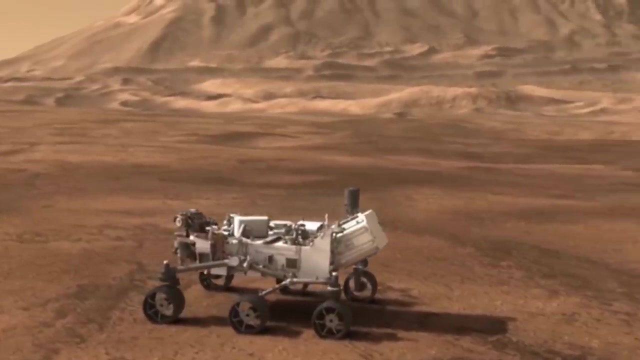 This Skycrane technique was used to avoid too much swirling dust exposing the rover to unnecessary danger. Everything had worked exactly as it was supposed to, and the American engineers were relieved. The landing had been the most precise ever Before Curiosity could start work. 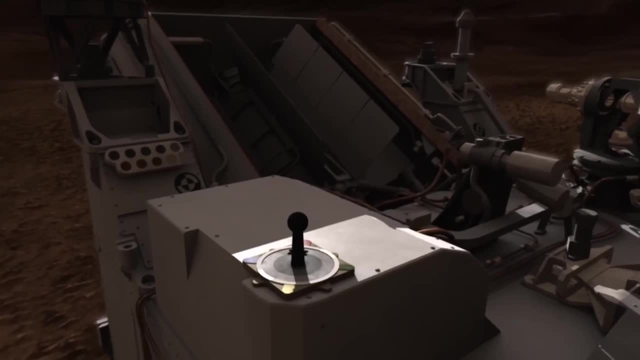 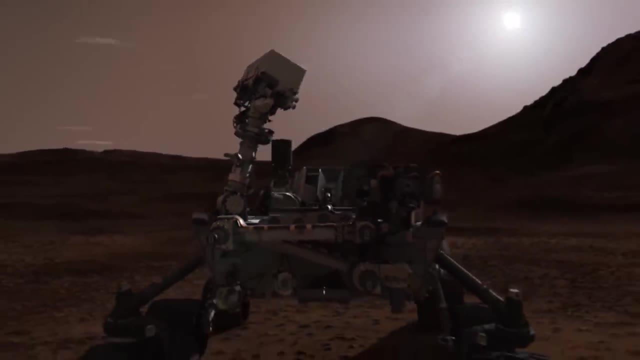 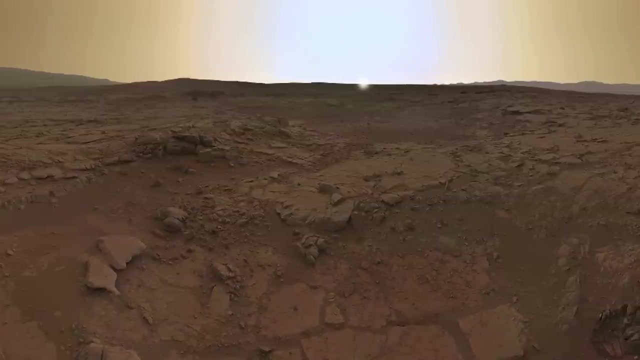 its computer went through a checklist to make certain that all systems were operating correctly. It was a day before the rover deployed its camera mast and communications antennas. It's thought that Gale Crater is 3.5 billion years old and that its sediments have been laid down. 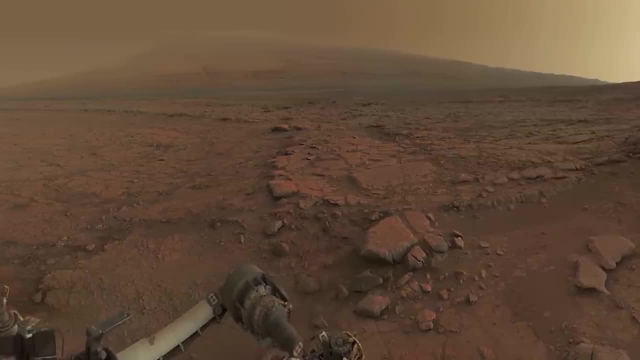 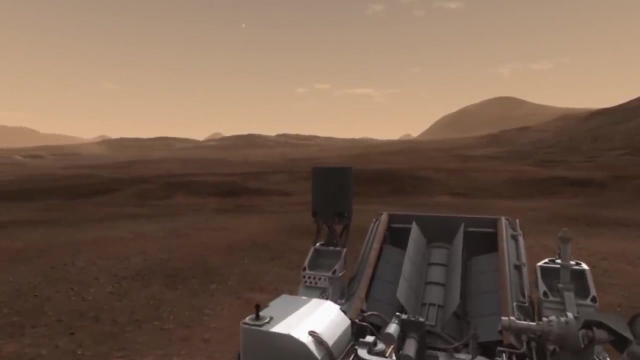 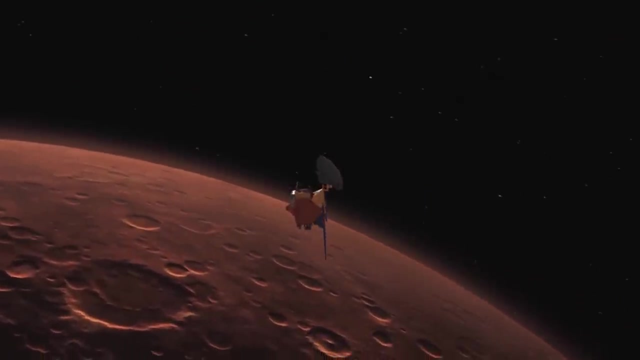 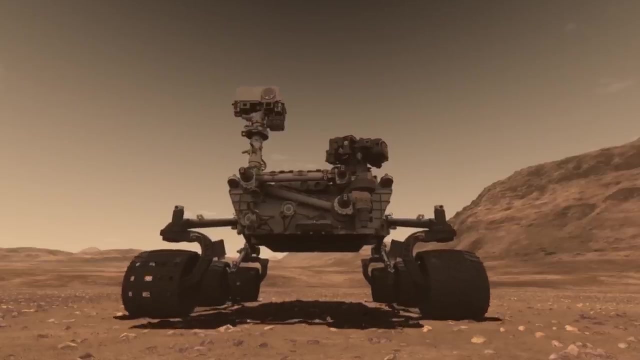 first by water and then by wind. NASA now has a sophisticated mobile science laboratory on Mars, connected to Earth by the most advanced communications link, courtesy of the Mars Reconnaissance Orbiter. The rover's primary objective is to discover if conditions suitable for life ever existed. 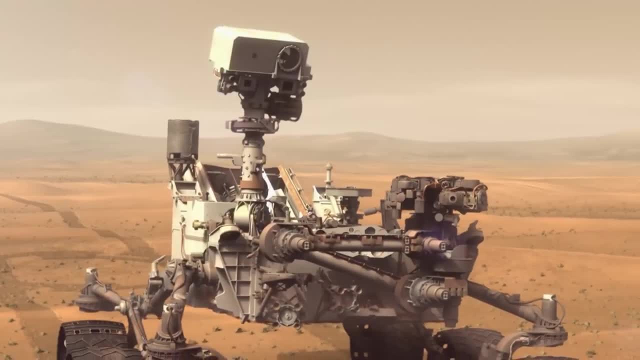 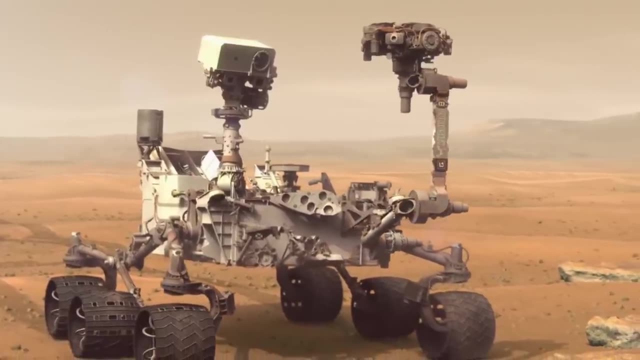 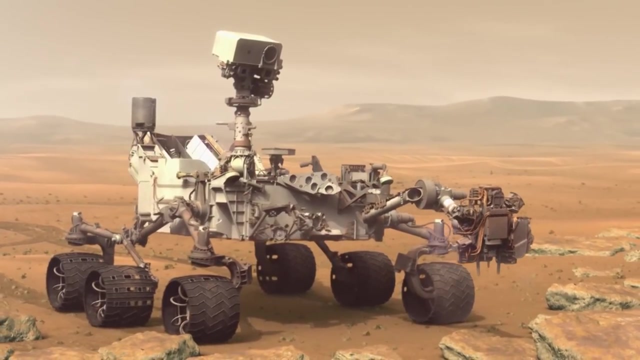 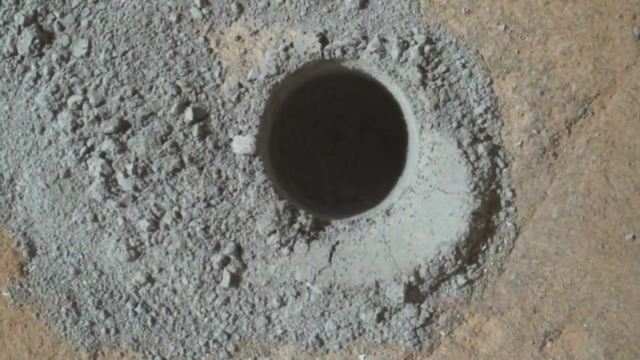 or still exist on Mars. It's also gathering detailed information about the current conditions on the Red Planet, particularly the radiation levels that will have an impact on proposed manned missions. Curiosity has analyzed the dust from a number of holes it drilled, revealing sulfur, nitrogen, hydrogen oxygen. 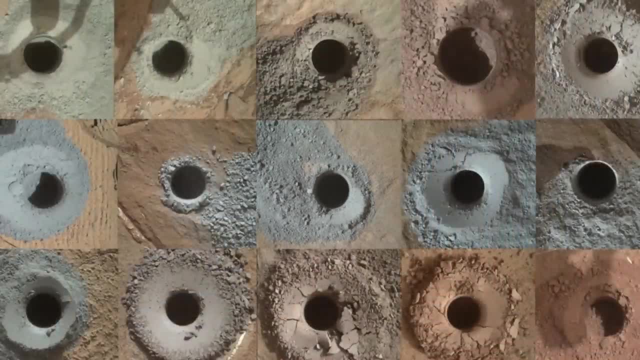 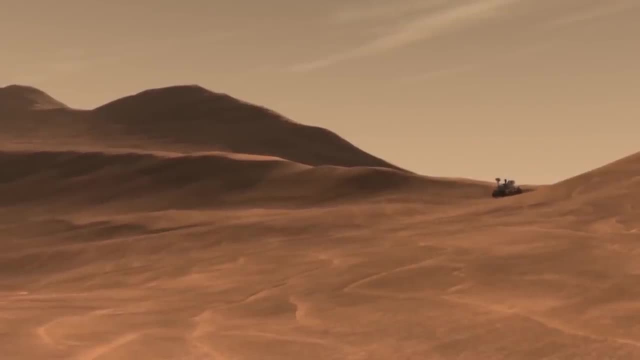 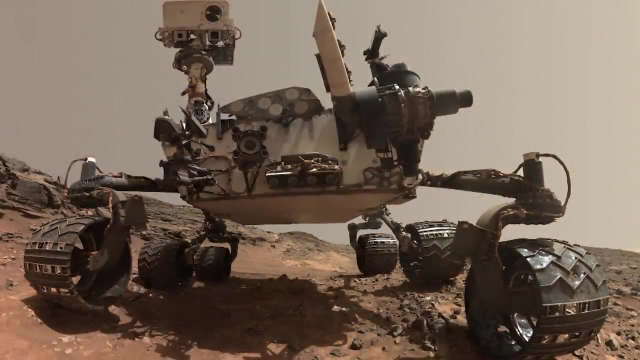 phosphorus and carbon, all elements essential to life. In its six years on the surface of Mars, Curiosity has traveled around 20 kilometers, but the driving is taking its toll. It routinely sends back a series of self-portraits, mainly for diagnostic reasons. 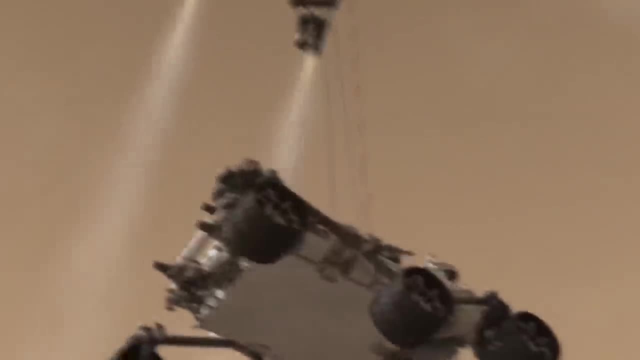 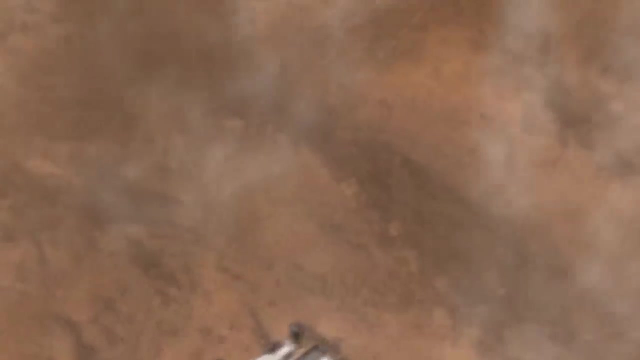 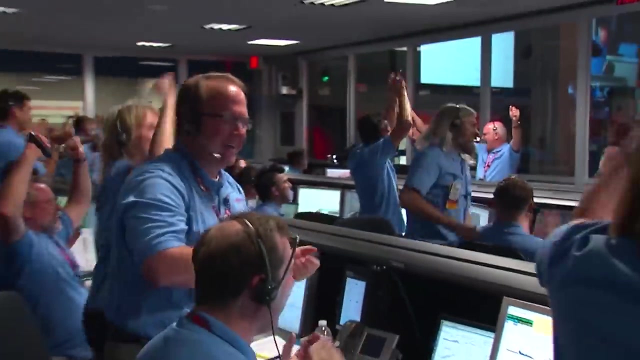 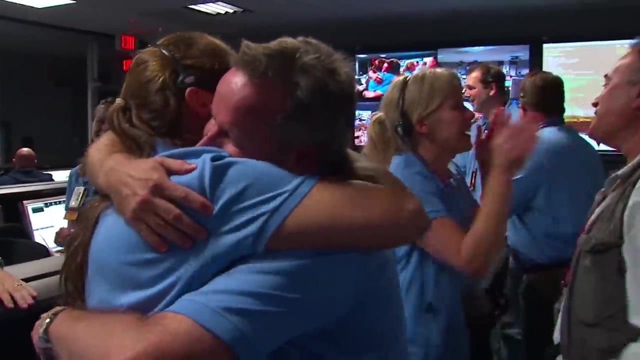 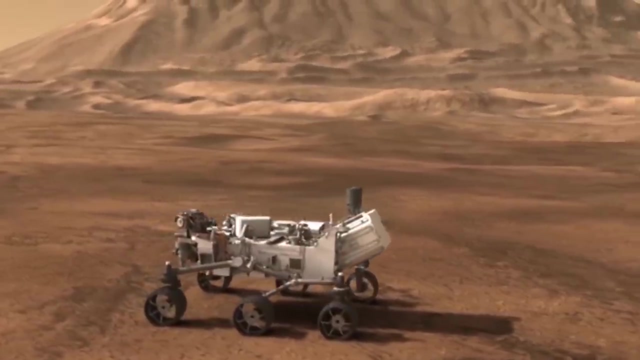 This Skycrane technique was used to avoid too much swirling dust exposing the rover to unnecessary danger. Everything had worked exactly as it was supposed to, and the American engineers were relieved. The landing had been the most precise ever Before Curiosity could start work. 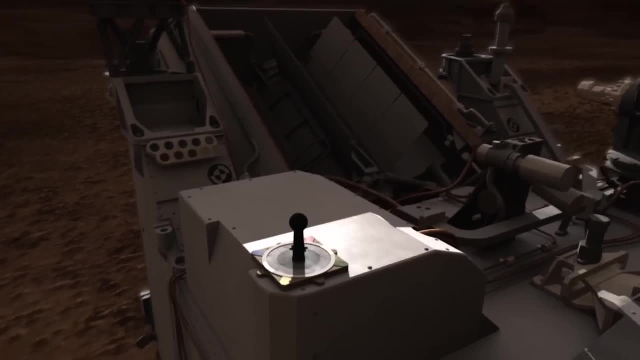 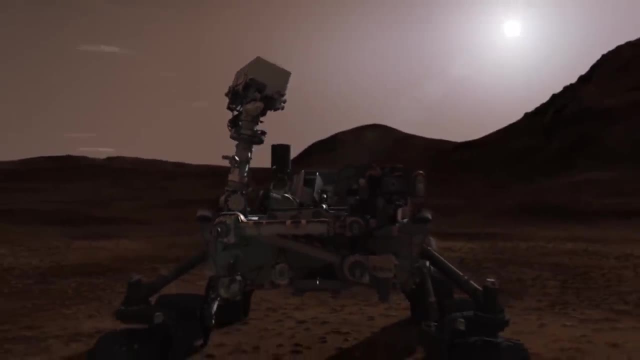 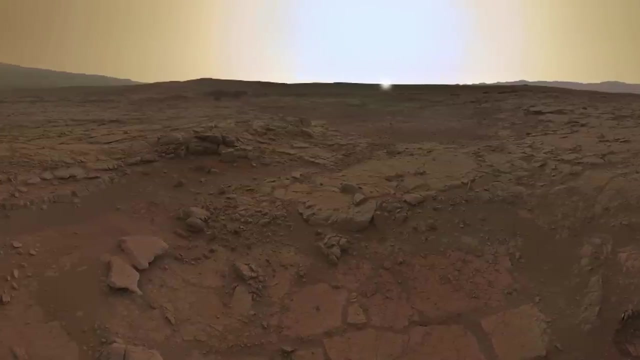 its computer went through a checklist to make certain that all systems were operating correctly. It was a day before the rover deployed its camera mast and communications antennas. It's thought that Gale Crater is 3.5 billion years old and that its sediments have been laid down first by water and then by wind. 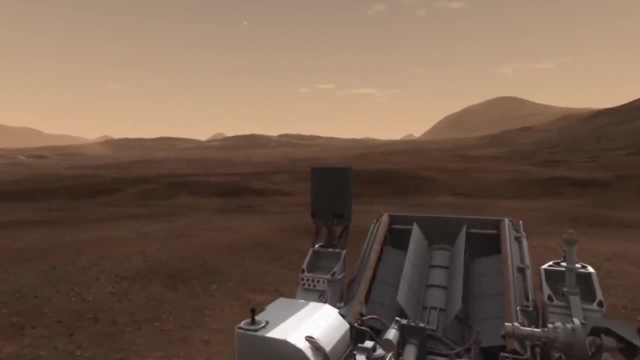 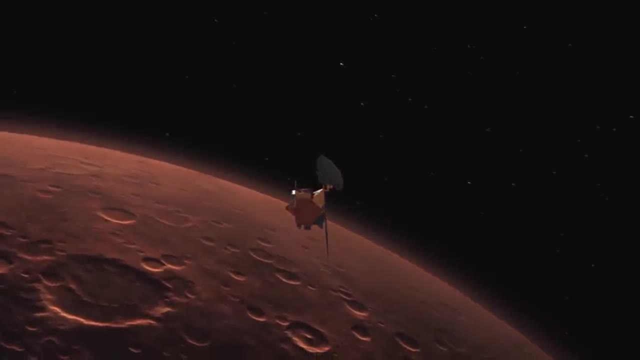 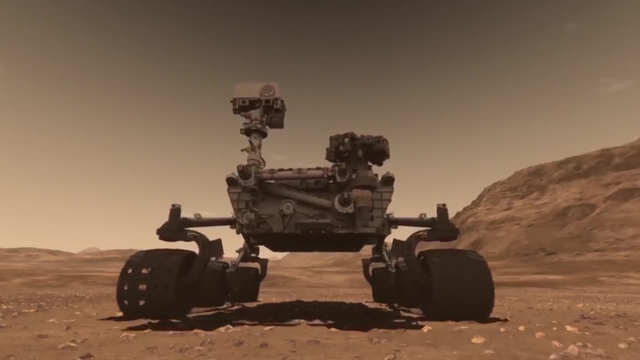 NASA now has a sophisticated mobile science laboratory on Mars, connected to Earth by the most advanced communications link, courtesy of the Mars Reconnaissance Orbiter. The rover's primary objective is to discover if conditions suitable for life ever existed or still exist on Mars. 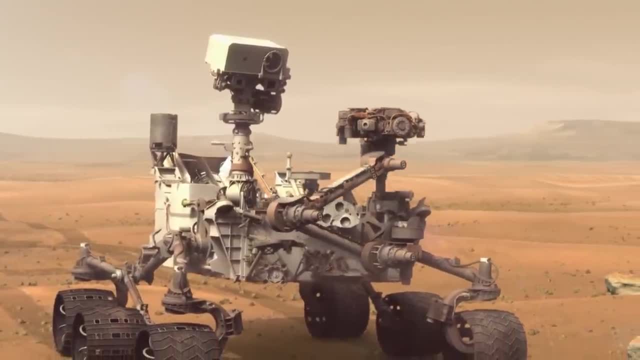 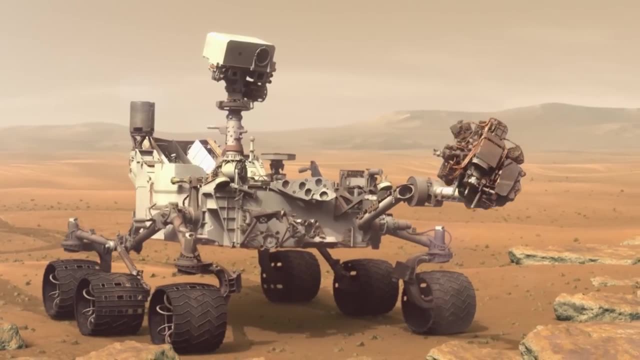 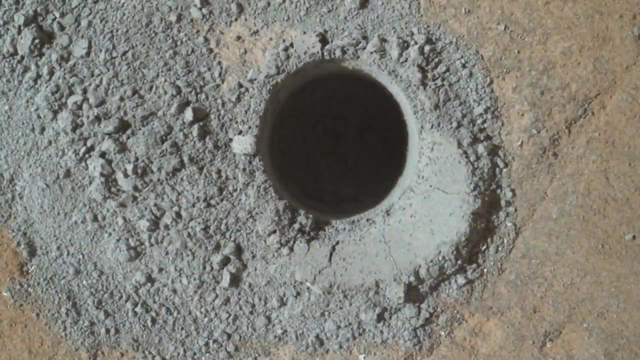 It's also gathering detailed information about the current conditions on the Red Planet, particularly the radiation levels that will have an impact on proposed manned missions. Curiosity has analyzed the dust from a number of holes it drilled, revealing sulfur, nitrogen, hydrogen oxygen, phosphorus and carbon. 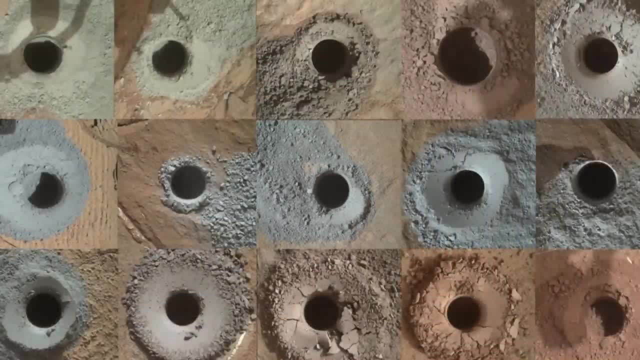 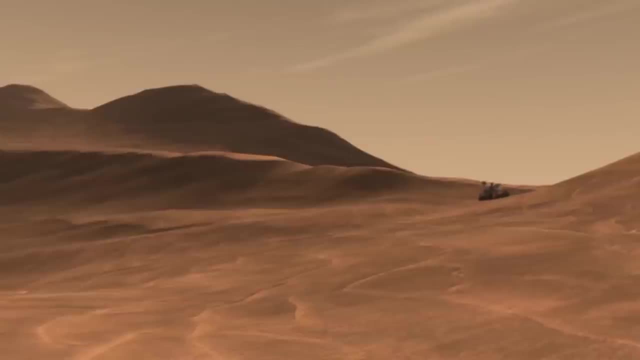 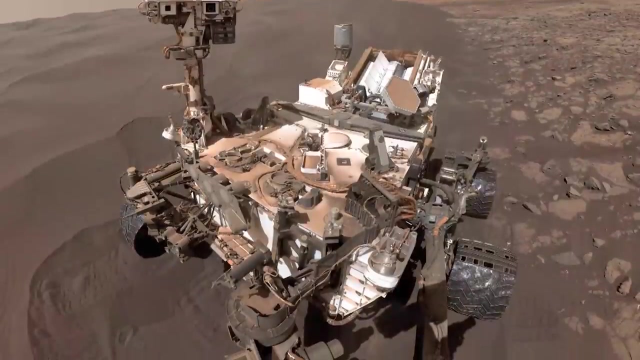 all elements essential to life. In its six years on the surface of Mars, Curiosity has traveled around 20 kilometers, but the driving is taking its toll. It routinely sends back a series of self-portraits, mainly for diagnostic reasons. Its wheels have taken severe damage. 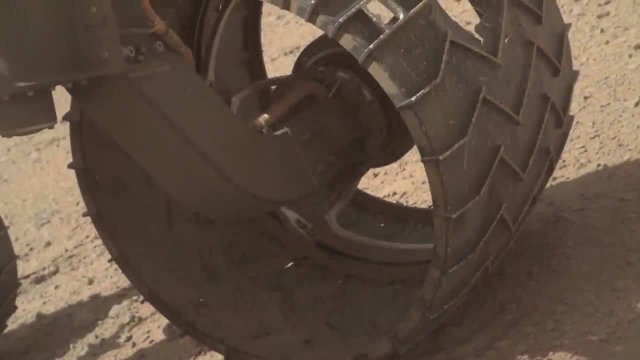 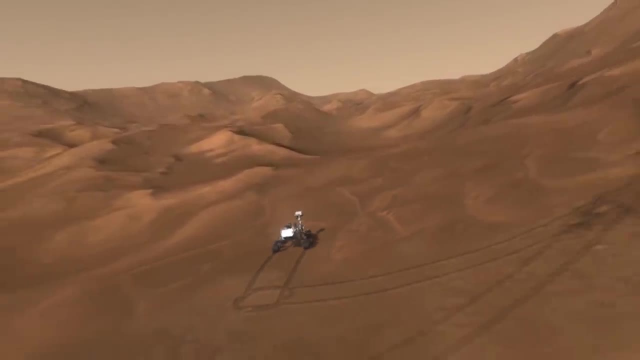 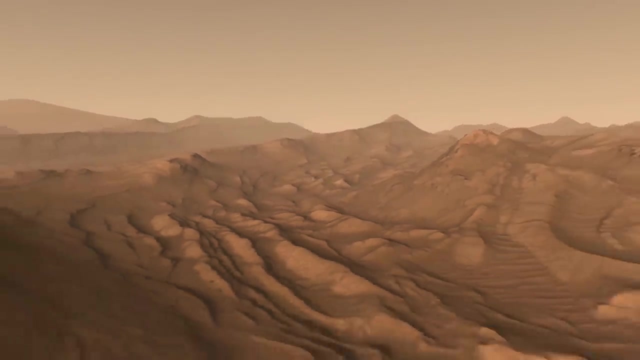 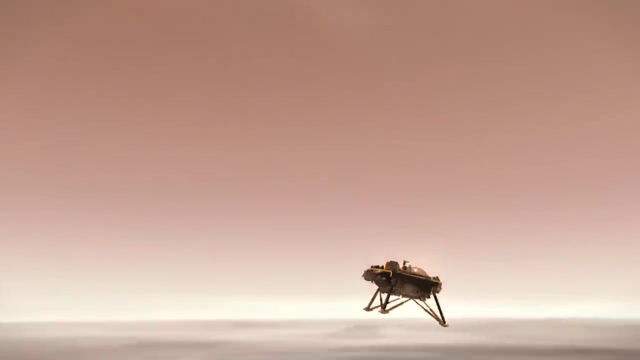 which will undoubtedly lead to design changes for future rovers. Its computers are also giving problems, but a new suite of missions is slated to arrive at Mars in 2020 that will continue profiling the planet. There is one aspect of the Martian environment that has never been investigated. 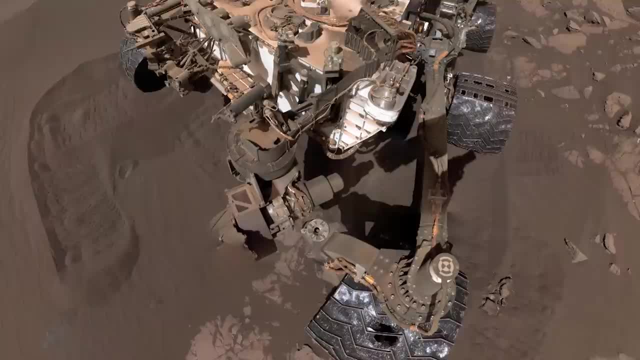 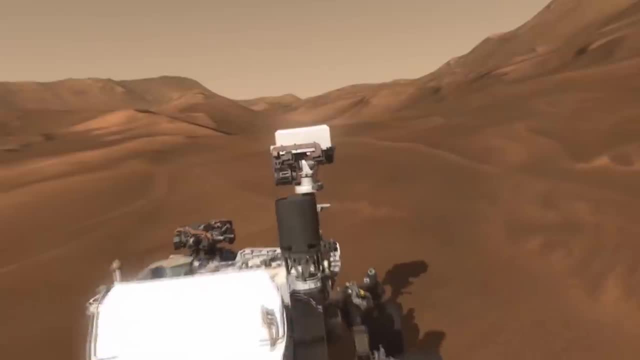 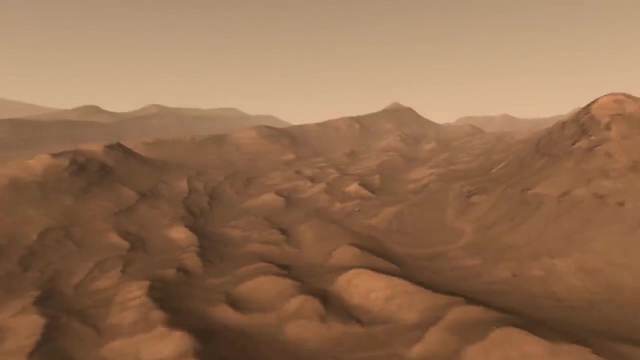 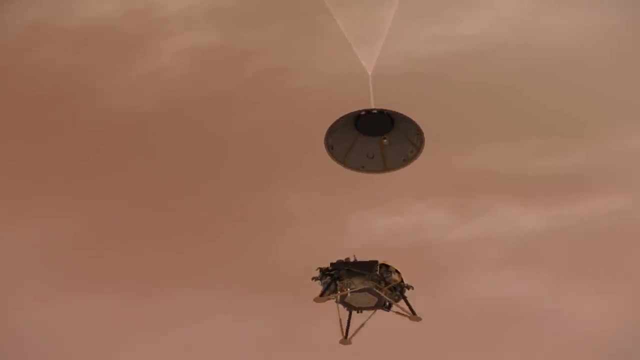 Its wheels have taken severe damage, which will undoubtedly lead to design changes for future rovers. Its computers are also giving problems, but a new suite of missions is slated to arrive at Mars in 2020, that will continue profiling the planet. There is one aspect of the Martian environment. 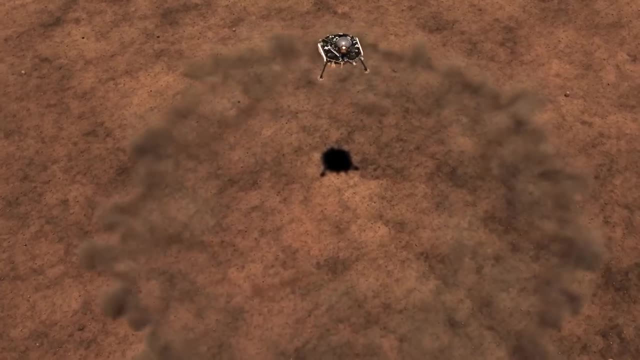 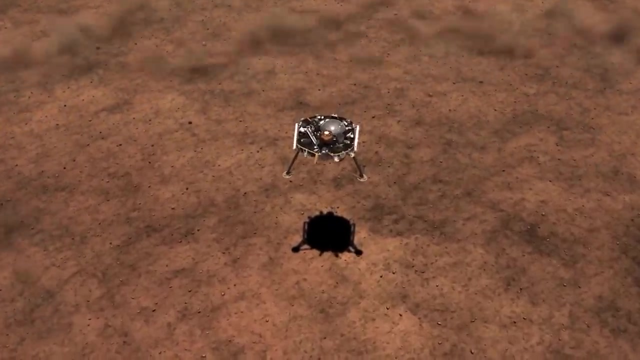 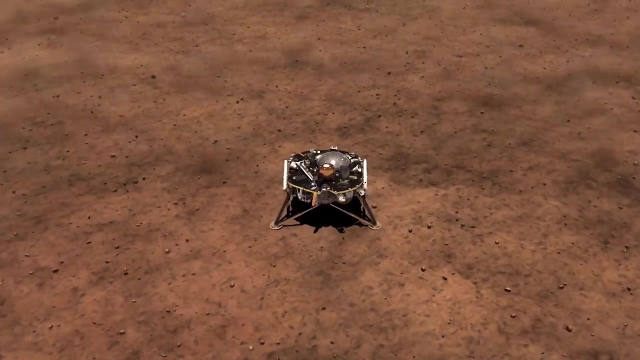 that has never been investigated, but that's about to be addressed. The Mars InSight probe has been targeted at the flat Elysium Planitia, close to the equator, to spend two years investigating the planet's interior. It made a flawless landing in November 2018.. 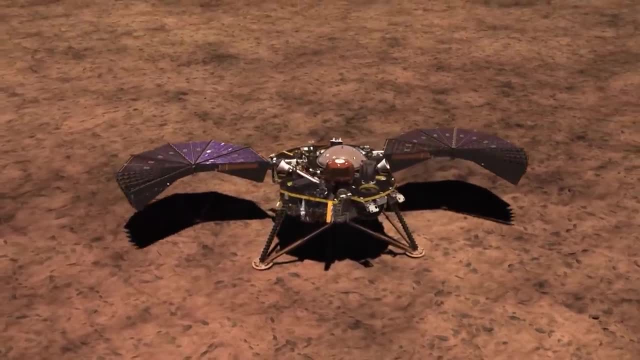 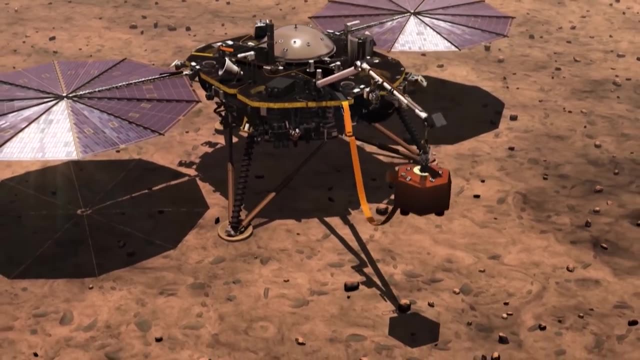 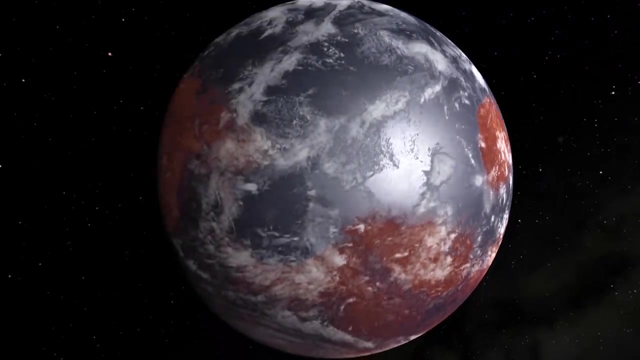 After unfurling its solar array, it spent weeks selecting a suitable site to deploy a seismometer onto the surface to monitor Mars quakes. It's clear that Mars had a warm, wet past, but it's cold and very dry now. 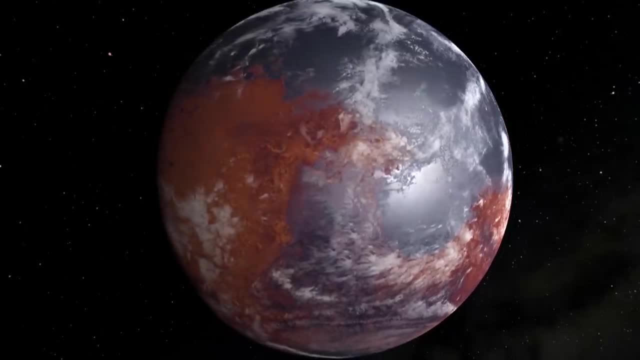 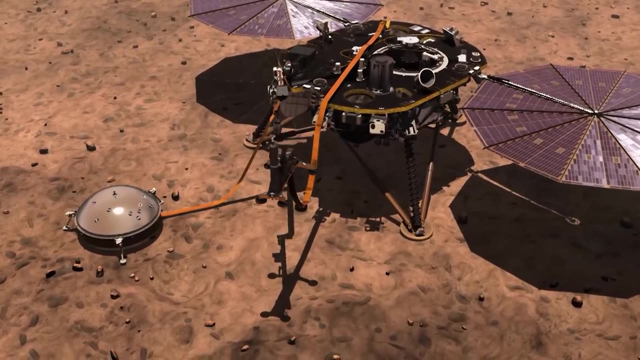 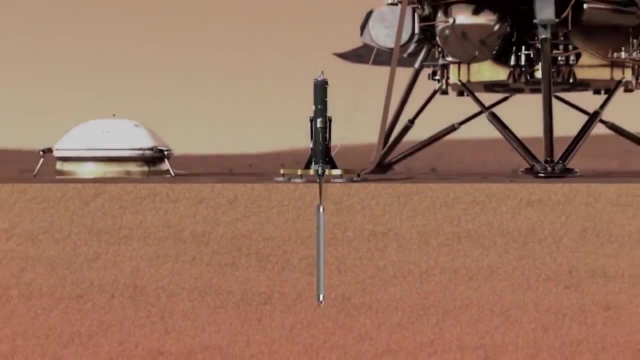 Learning about the planet's geological activity will help us know why Mars has changed. The InSight probe also hammered a thermal sensor into the surface to gather data on heat flow from the planet's core. By understanding processes within Mars, we can learn how the geological histories of Mars and Earth 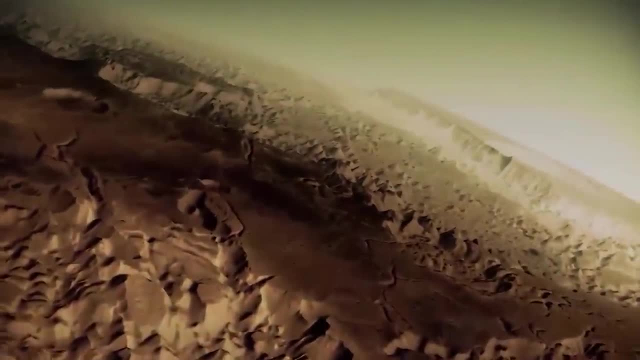 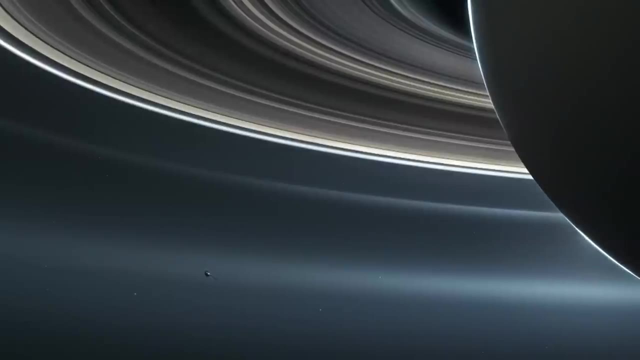 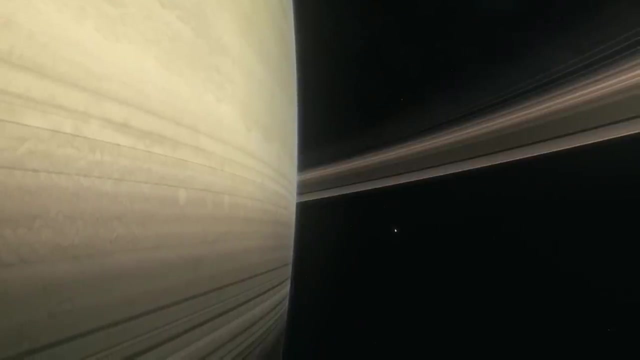 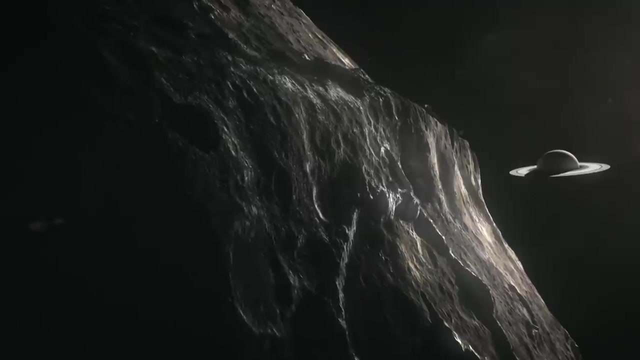 began to diverge. The ringed planet Saturn, More than 100 times the mass of Earth. its metallic core lies beneath 80,000 kilometres of liquid hydrogen and helium. It's called a gas giant. Saturn is orbited by at least 62 moons. each unique, some with complex and dynamic environments. Our only detailed examination of the Saturnian system ended in 2017, when the Cassini probe was intentionally crashed into the planet's dense atmosphere to guard against accidental and dangerous earthquakes, And the Mars probe has been a key source. 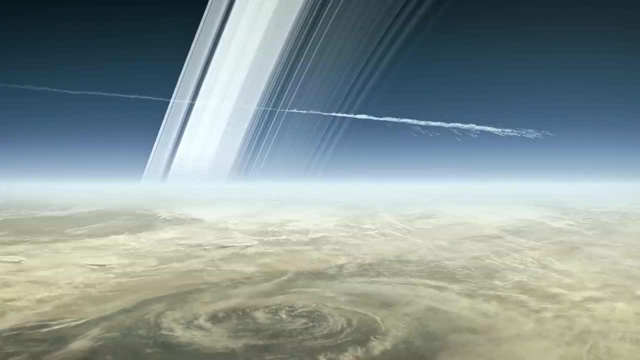 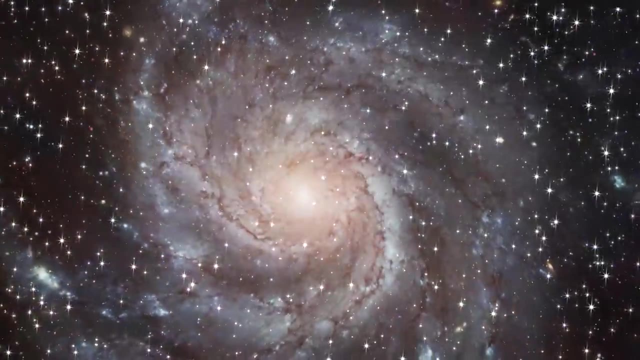 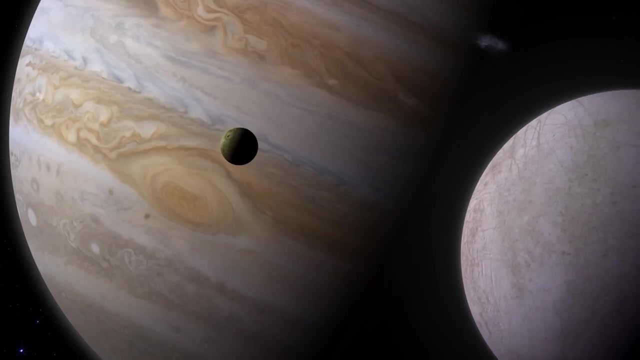 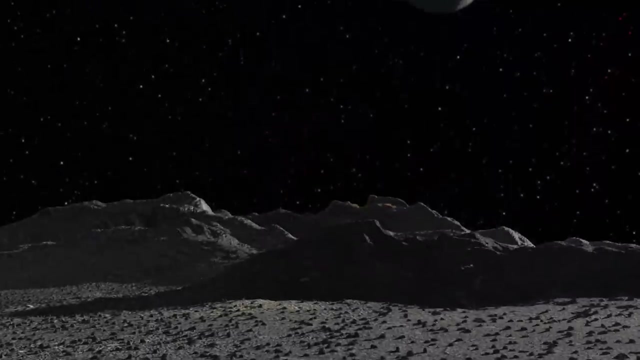 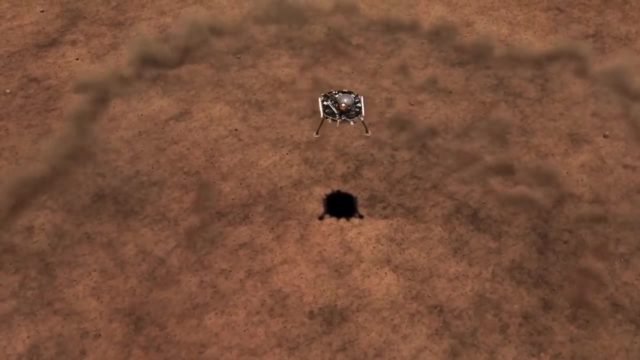 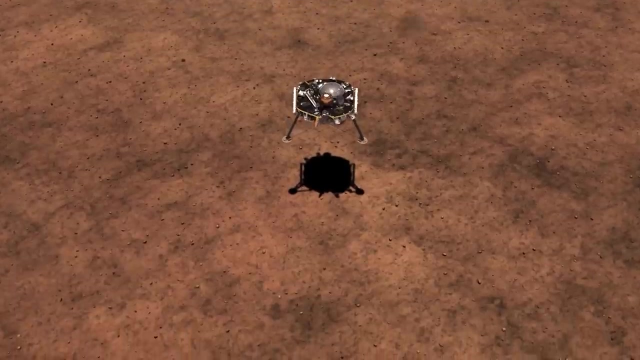 but that's about to be addressed. The Mars InSight probe has been targeted at the flat Elysium Planitia, close to the equator, to spend two years investigating the planet's interior. It made a flawless landing in November 2018.. 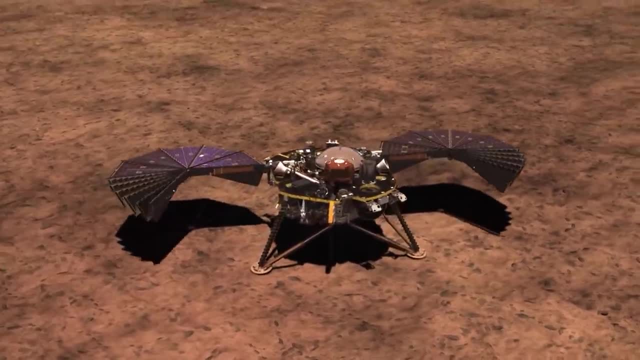 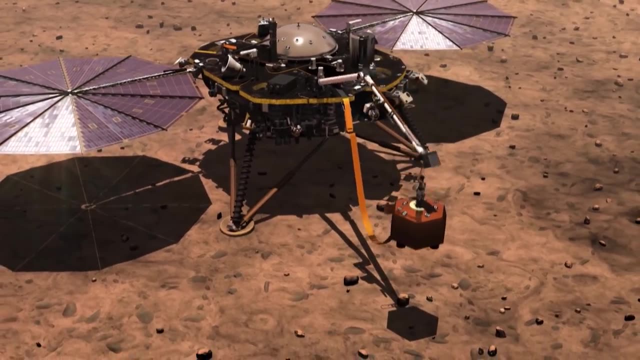 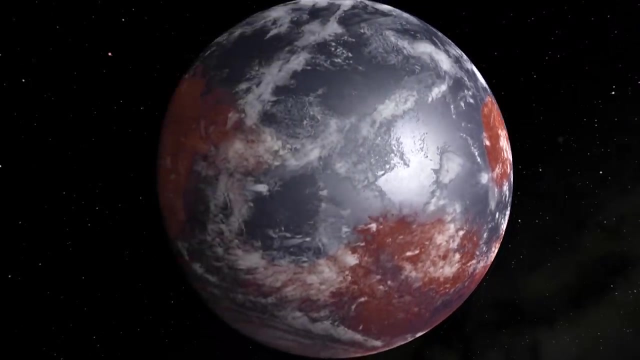 After unfurling its solar array, it spent weeks selecting a suitable spot to deploy a seismometer onto the surface to monitor Mars quakes. It's clear that Mars had a warm, wet past, but it's cold and very dry now. 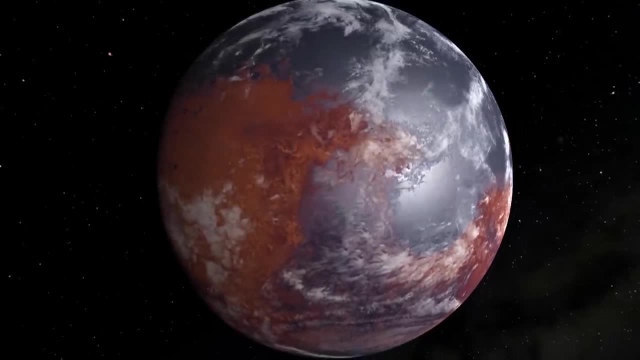 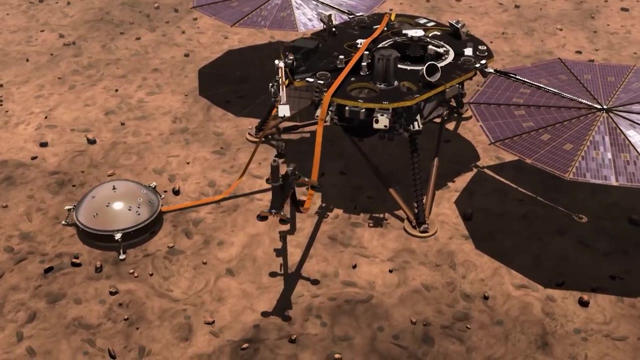 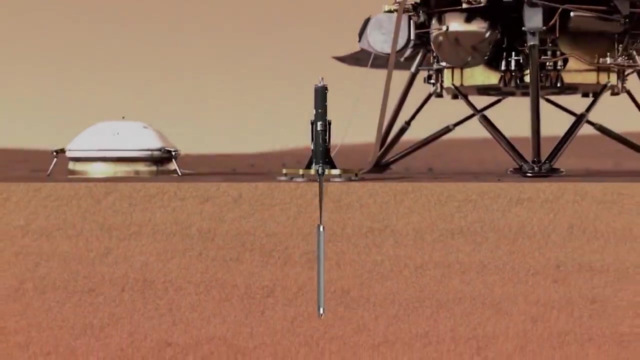 Learning about the planet's geological activity will help us know why Mars has changed. The InSight probe also hammered a thermal sensor into the surface to gather data on heat flow from the planet's core. By understanding processes within Mars, we can learn how the geological histories of Mars and Earth 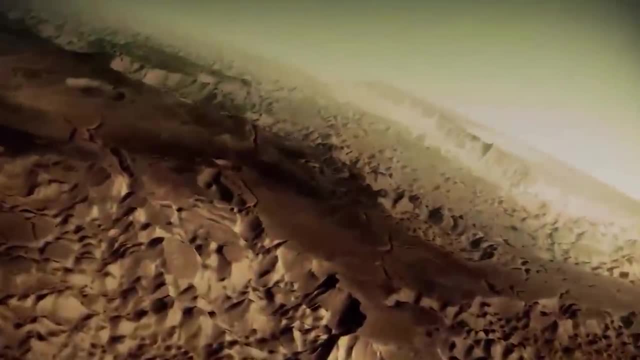 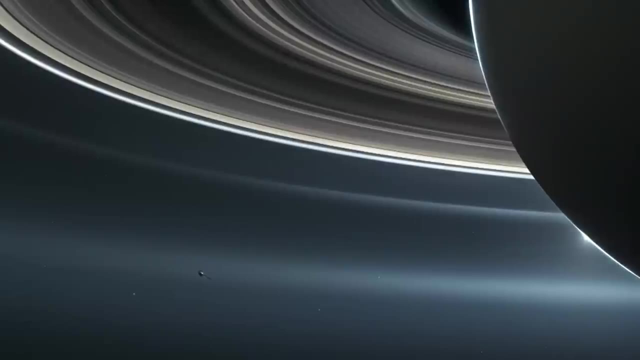 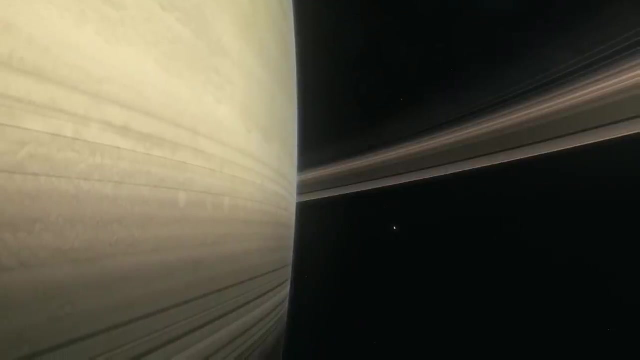 began to diverge. The ringed planet Saturn, More than 100 times the mass of Earth. its metallic core lies beneath 80,000 kilometres of liquid hydrogen and helium. Its core is the Earth's core. It's called a gas giant. 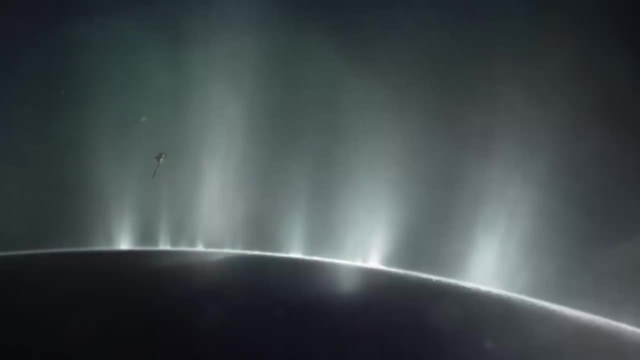 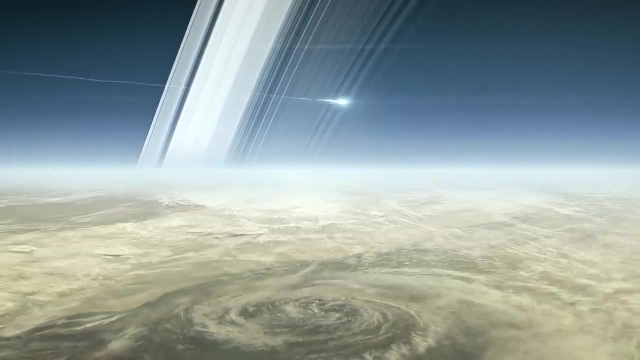 Saturn is orbited by at least 62 moons, each unique, some with complex and dynamic environments. Our only detailed examination of the Saturnian system ended in 2017, when the Cassini probe was intentionally crashed into the planet's dense atmosphere to guard against accidental contamination. 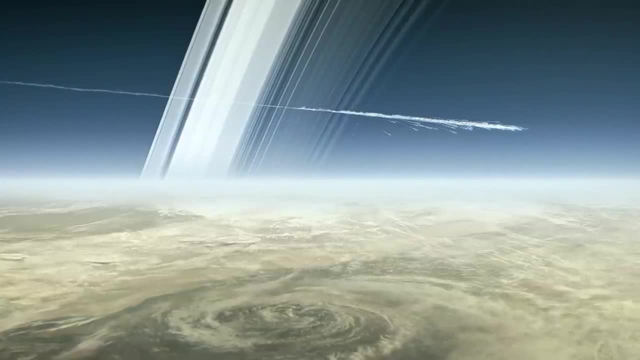 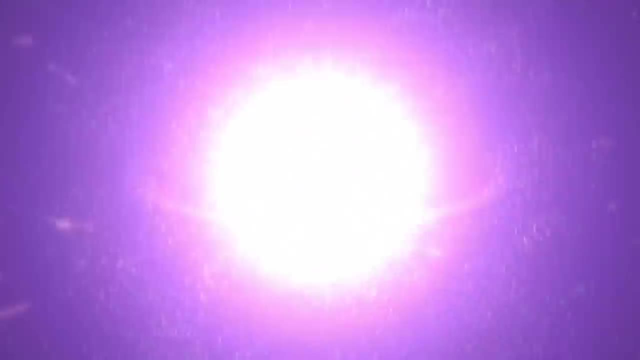 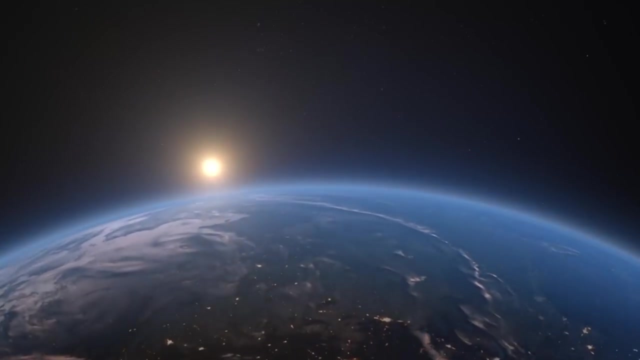 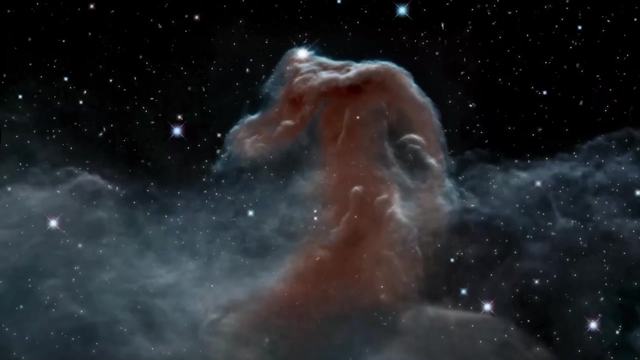 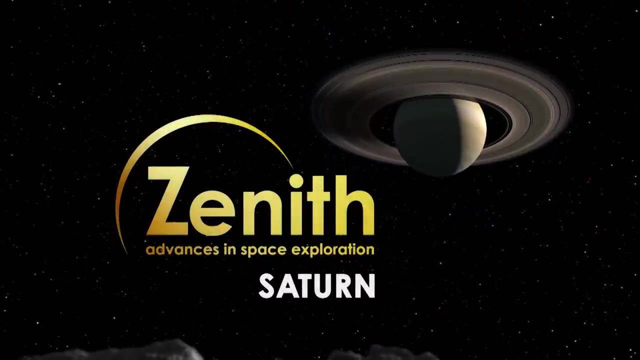 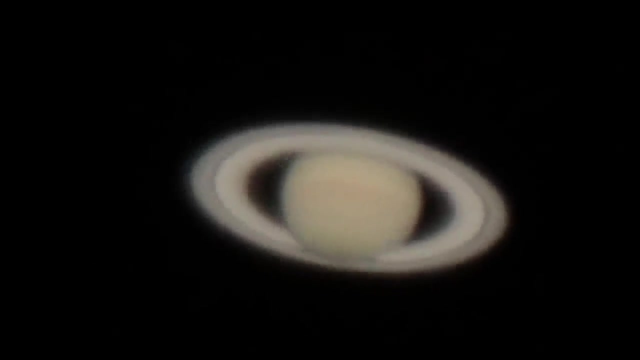 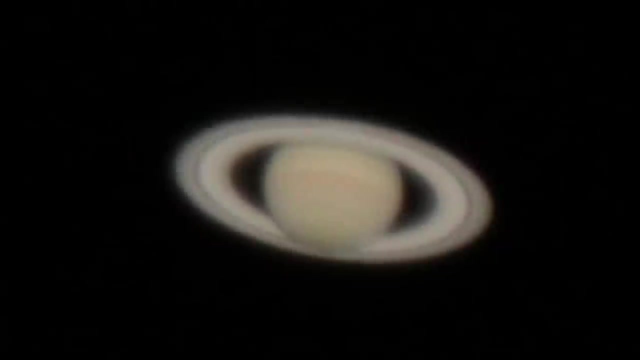 of the moons NASA Jet Propulsion Laboratory, California Institute of Technology. Viewed from Earth, Saturn's rings are visible, but not in any detail. They were thought to be solid until mathematical analysis suggested they were orbiting particles. But how did they get there? 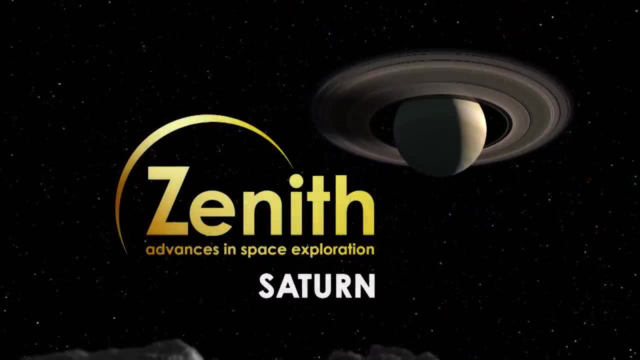 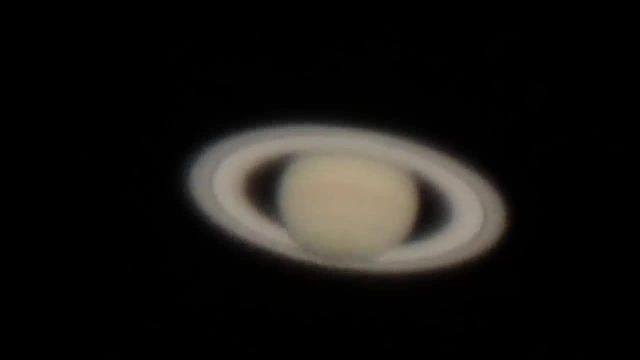 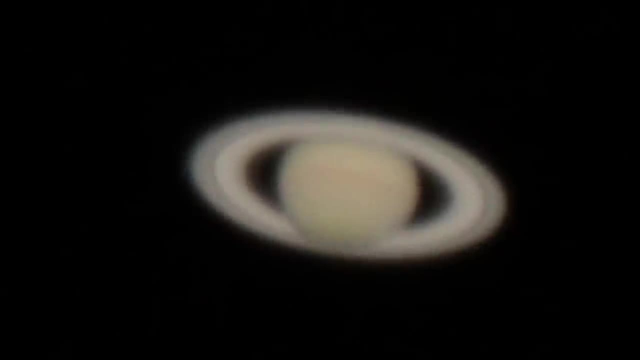 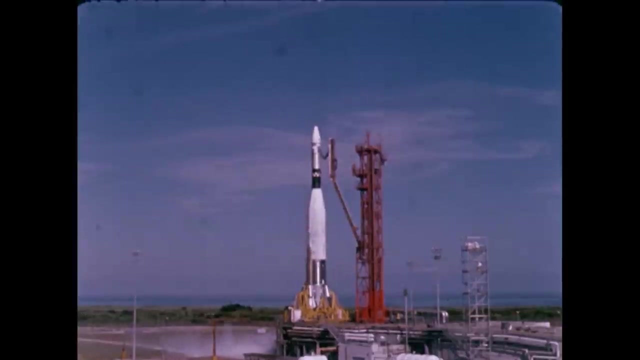 Viewed from Earth, Saturn's rings are visible, but not in any detail. They were thought to be solid until mathematical analysis suggested they were orbiting particles. But how did they get there And why was Saturn alone in having rings? In the early days of space research, Saturn was just too far away. 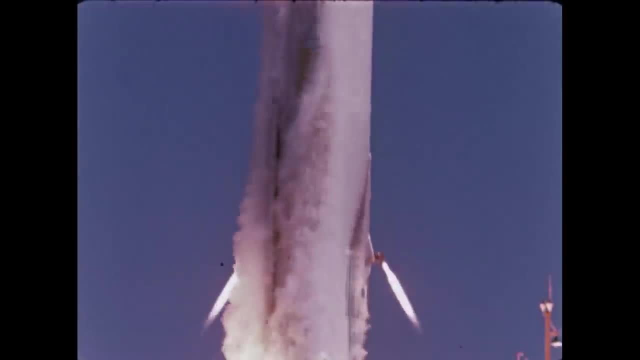 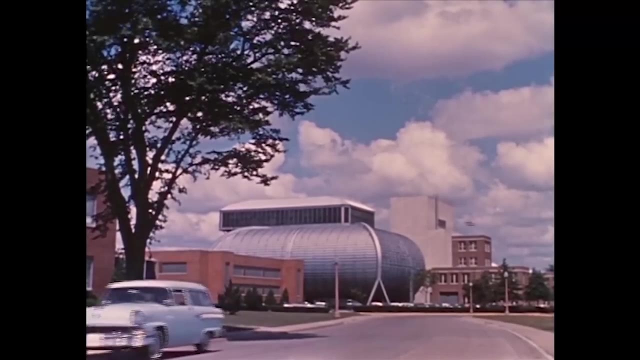 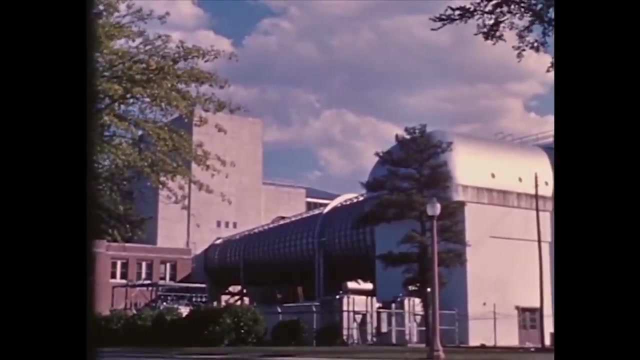 By the way, conventional rockets could only just reach Mars. In 1964, NASA realized that a space probe launched in 1977 could take advantage of a rare alignment of the outer planets to fly past all the gas giants Using gravitational assistance from the planets. 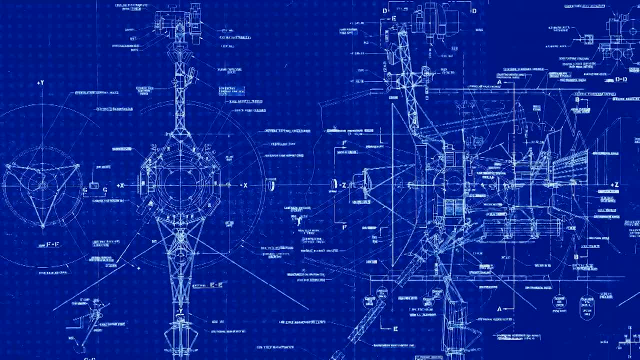 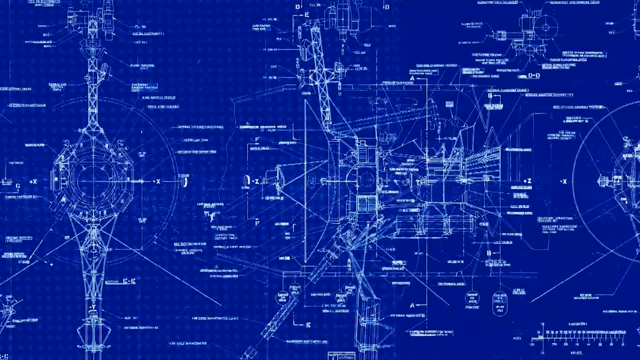 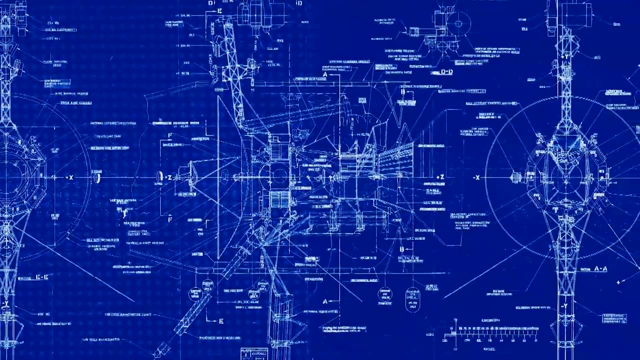 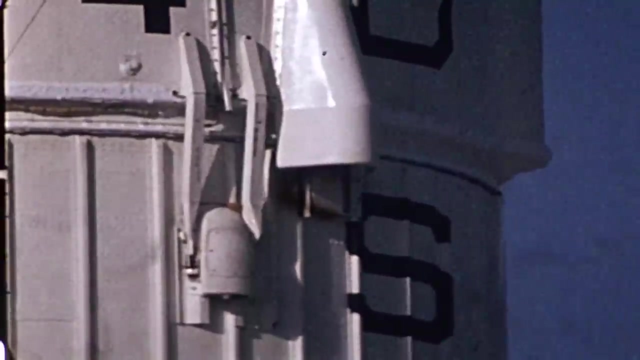 it would just be possible with the technology of the day. An ambitious new mission began to take shape. It was dubbed The Grand Tour. Two probes that were far in advance of anything yet attempted would be part of the Mariner series, Because no spacecraft had been sent beyond Mars. 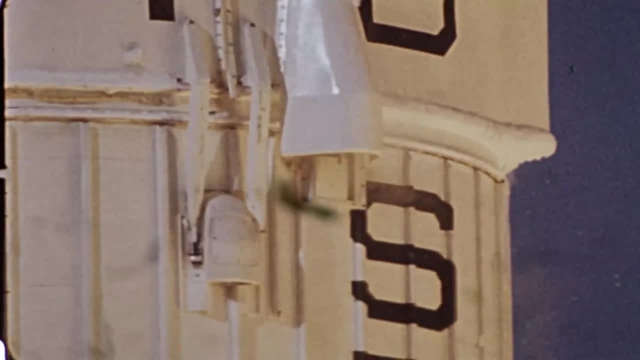 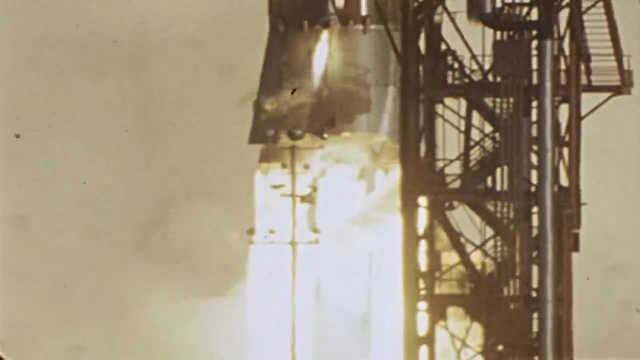 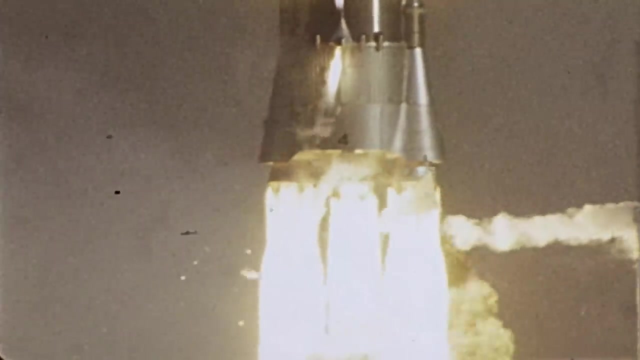 mission planners felt it would be wise to send two rudimentary advanced probes to Jupiter and Saturn to test the deep space environment. Researchers didn't know if it was even possible to cross the asteroid belt between Mars and Jupiter. In 1972, Pioneer 10 was launched towards Jupiter. 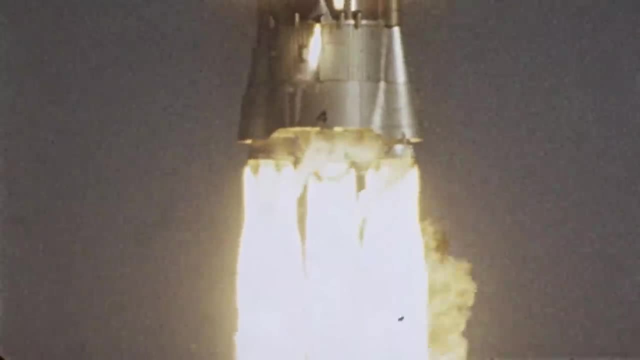 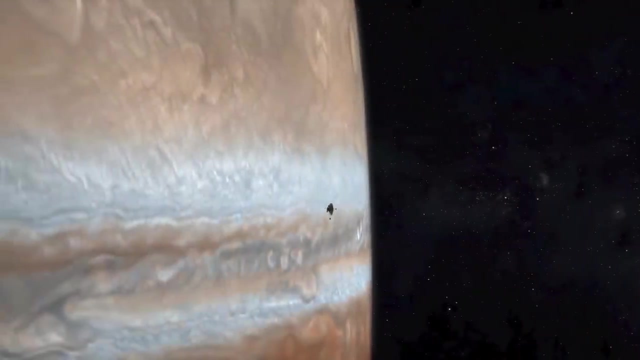 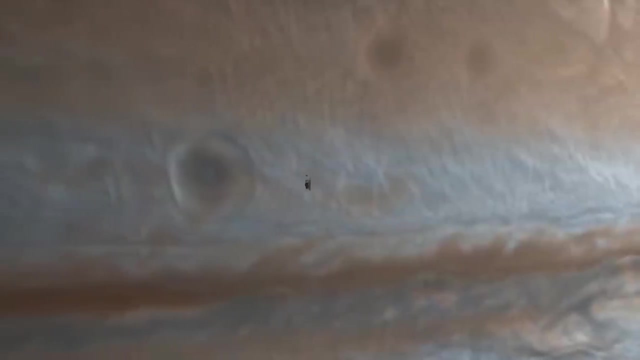 and the following year a twin Pioneer 11, was sent to Saturn. Both craft passed by Jupiter and discovered that the electron radiation there was 10,000 times as strong as at Earth. This was a surprise to engineers at NASA, who had to modify the more sophisticated craft. 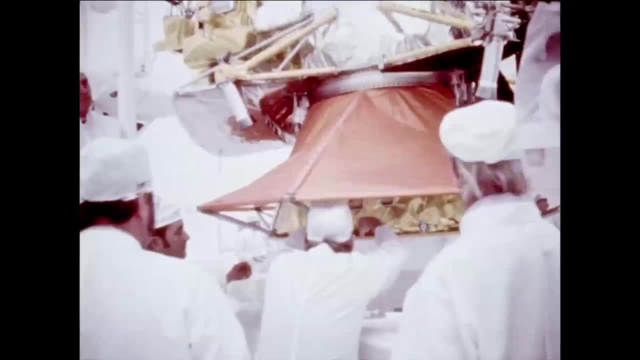 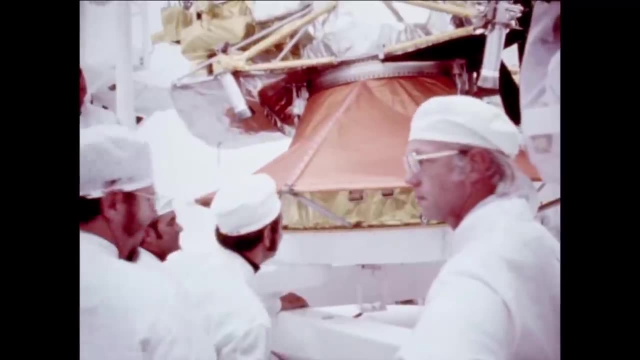 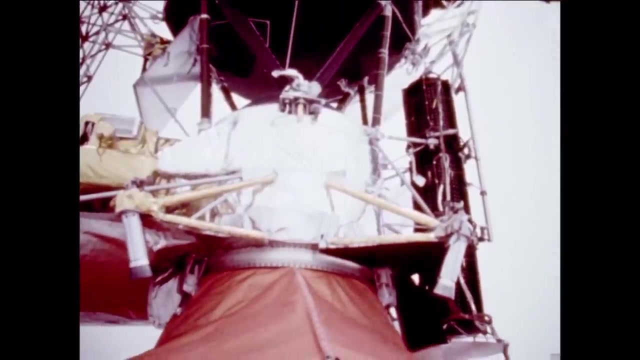 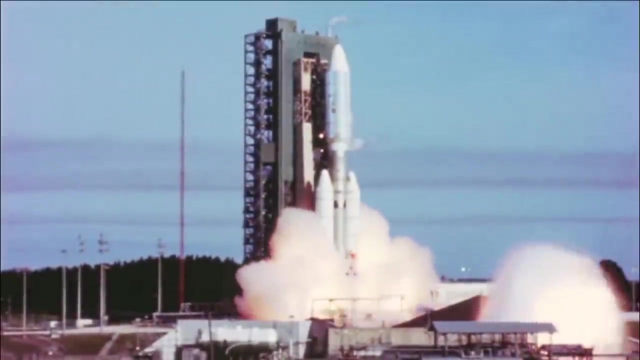 they were preparing for the Grand Tour. The probes being built at NASA's Jet Propulsion Laboratory were part of a program known as Mariner Jupiter-Saturn, but this was soon changed to the Voyager program. They were launched 16 days apart, in late 1977,. 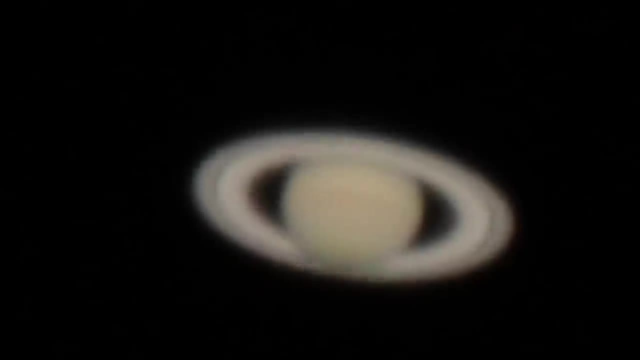 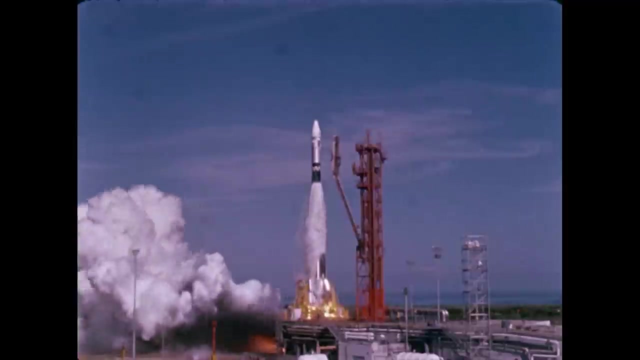 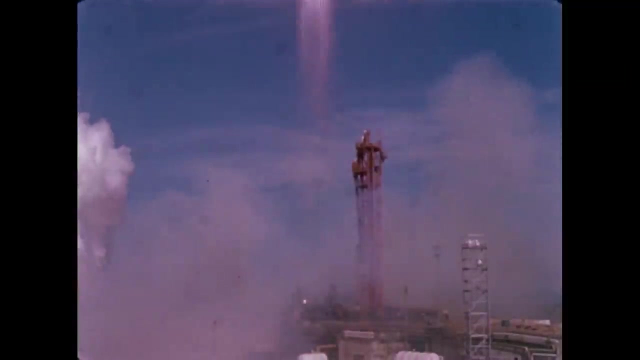 And why was Saturn alone in having rings? In the early days of space research, Saturn was just too far away. Conventional rockets could only just reach Mars. They could only reach Earth. In 1964, NASA realised that a space probe launched in 1977. 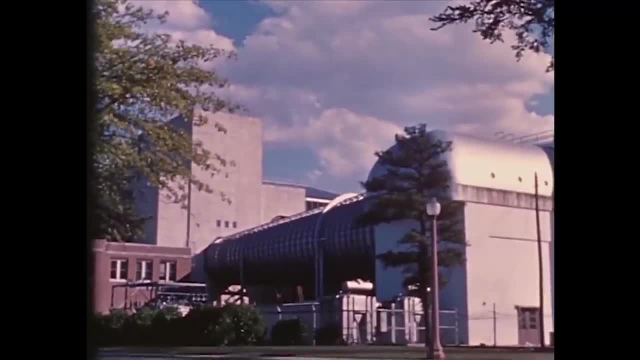 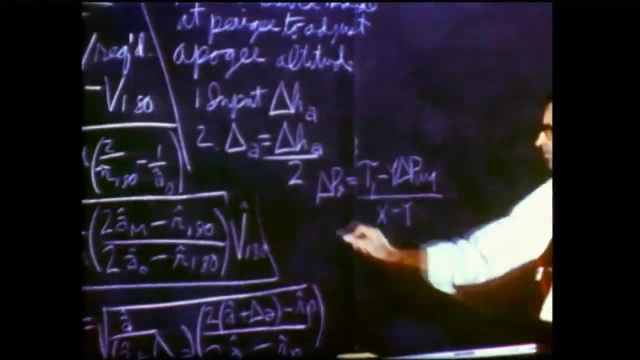 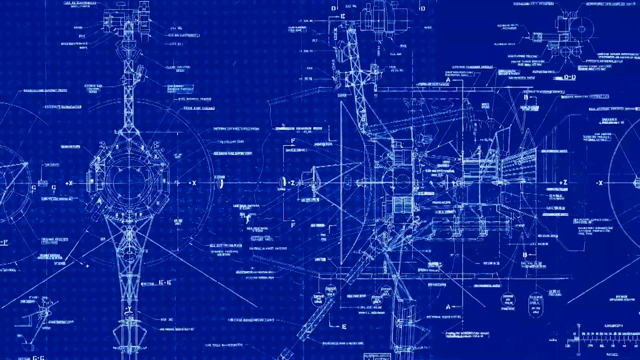 could take advantage of a rare alignment of the outer planets to fly past all the gas giants Using gravitational assistance from the planets. it would just be possible. with the technology of the day. An ambitious new mission began to take shape. It was dubbed the Grand Tour. 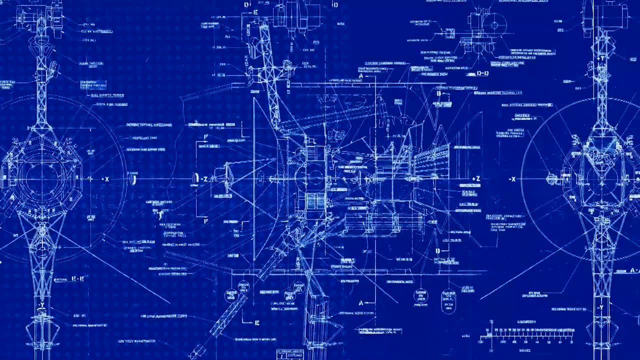 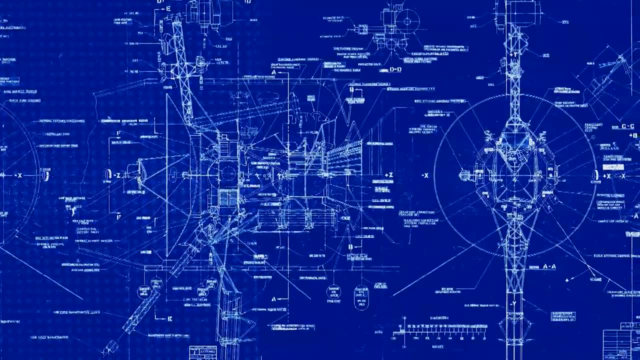 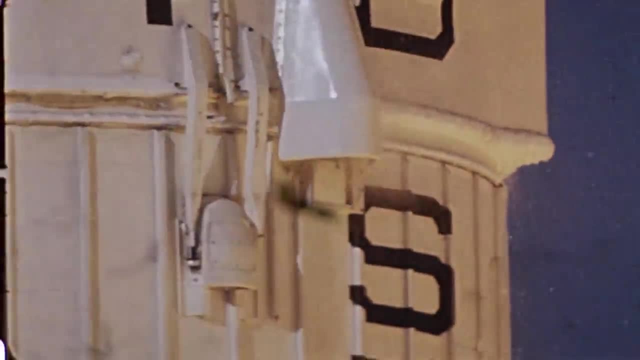 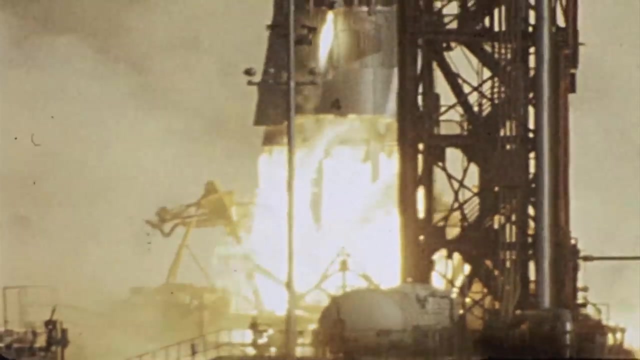 Two probes that were far in advance of anything yet attempted would be part of the Mariner series. Because no spacecraft had been sent beyond Mars, mission planners felt it would be wise to send two rudimentary advanced probes to Jupiter and Saturn to test the deep space environment. 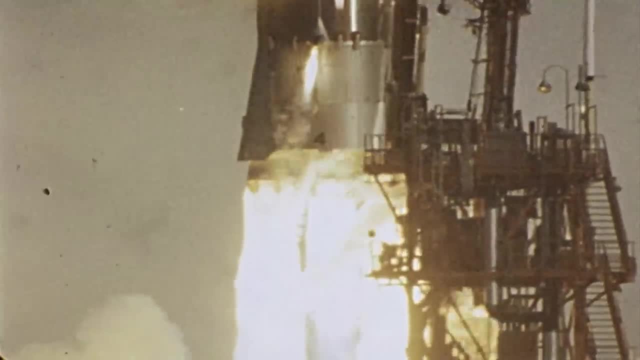 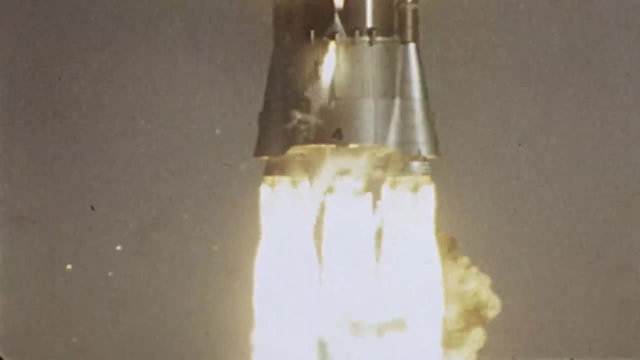 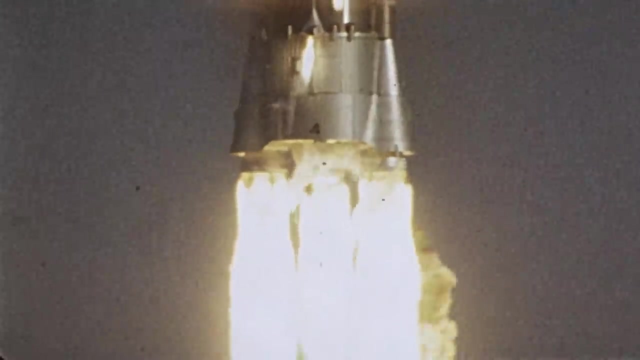 Researchers didn't know if it was even possible to cross the asteroid belt between Mars and Jupiter. In 1972, Pioneer 10 was launched towards Jupiter, and the following year a twin Pioneer 11, was sent to Saturn. Both craft passed by Jupiter. 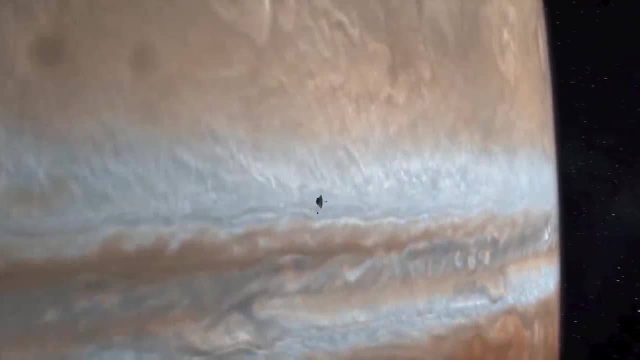 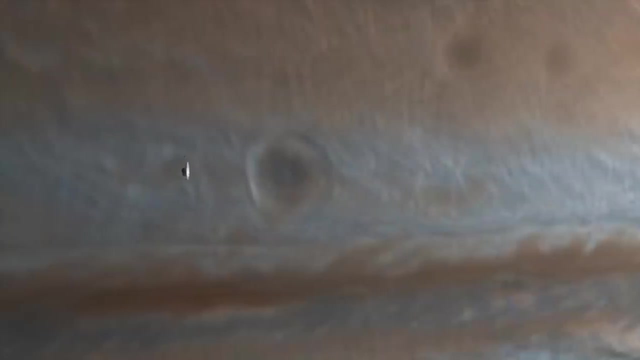 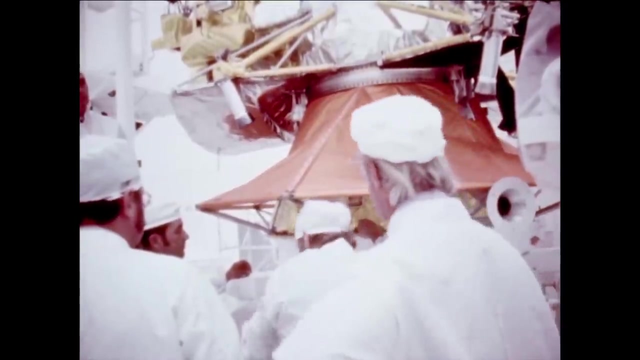 and discovered that the electron radiation there was 10,000 times as strong as at Earth. This was a surprise to engineers at NASA, who had to modify the more sophisticated craft they were preparing for the Grand Tour: The probes being built at NASA's Jet Propulsion Laboratory. 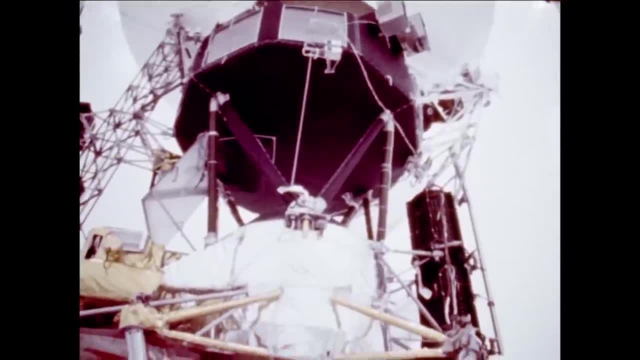 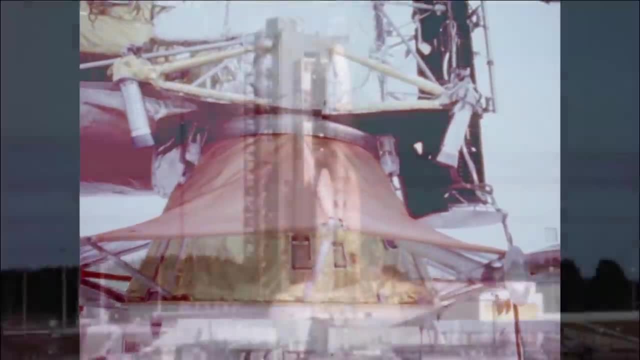 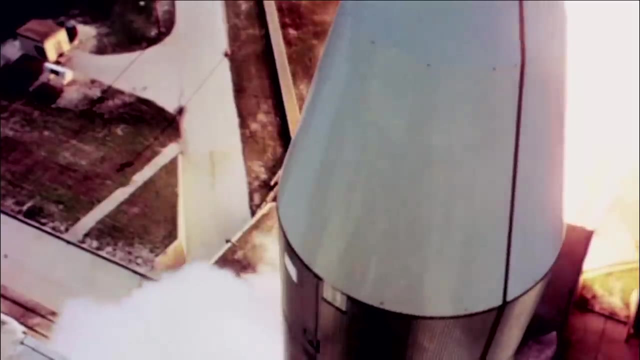 were part of a program known as Mariner Jupiter-Saturn, but this was soon changed to the Voyager program. They were launched 16 days apart, in late 1977, while Pioneer 10 was heading toward Interstellar And Pioneer 11 was still two years away from Saturn. 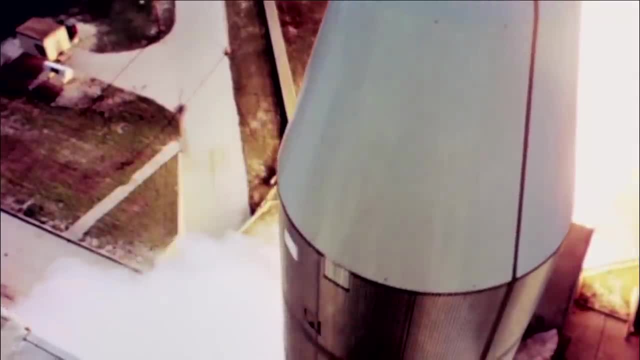 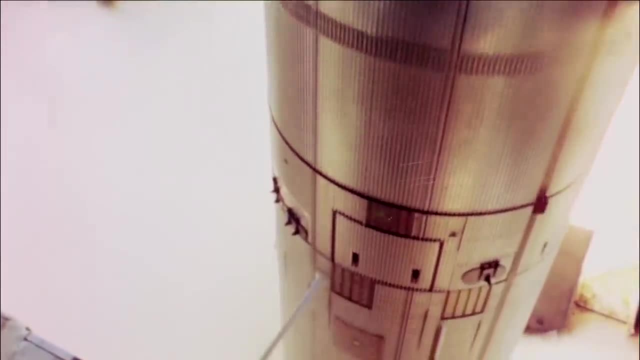 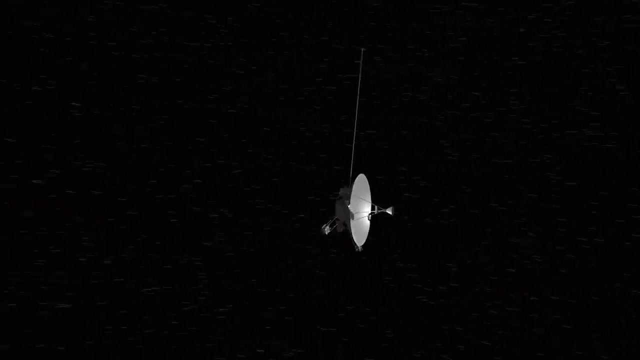 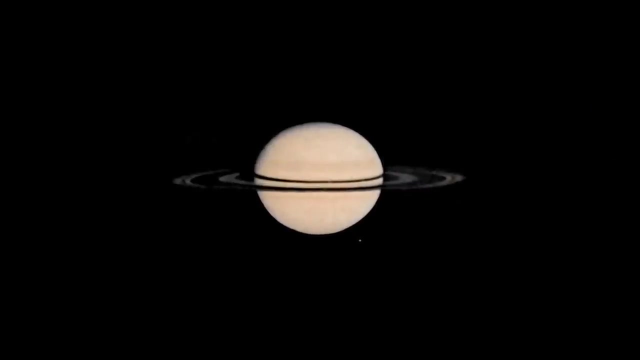 while Pioneer 10 was heading toward interstellar space and Pioneer 11 was still two years away from Saturn, In 1979,, as Pioneer 11 approached the ringed planet, it began sending back pictures far clearer than anything seen before. A new ring, the F ring, was observed for the first time. 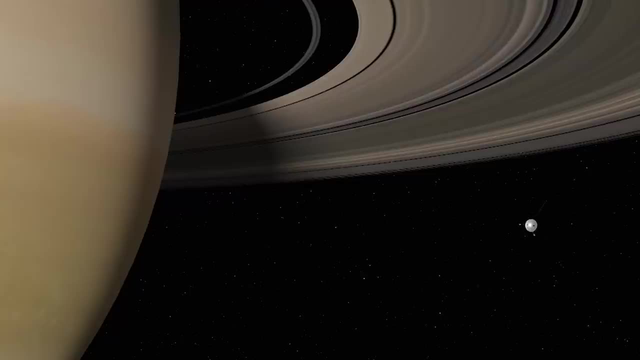 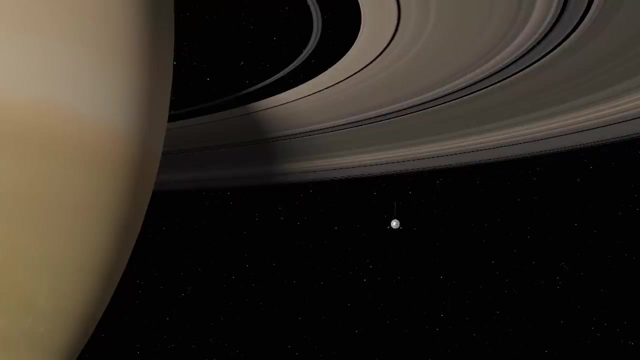 The craft flew by Saturn passing beneath the rings. Mission planners were uncertain how broadly the ring particles spread. If there was a threat to the spacecraft, they were prepared to sacrifice Pioneer 11 to get a clear idea of the environment. they would encounter with the following Voyager craft. The probe passed the ring safely and continued beyond Saturn into interstellar space. NASA received its last communication from the probe on the 24th of November 1995.. The following Voyager 1 and 2 probes were very robust, designed to survive for a very long journey. 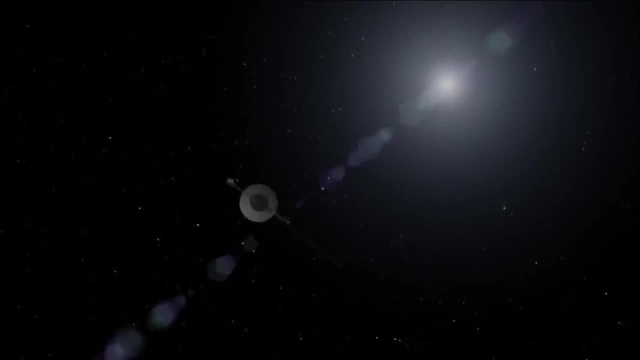 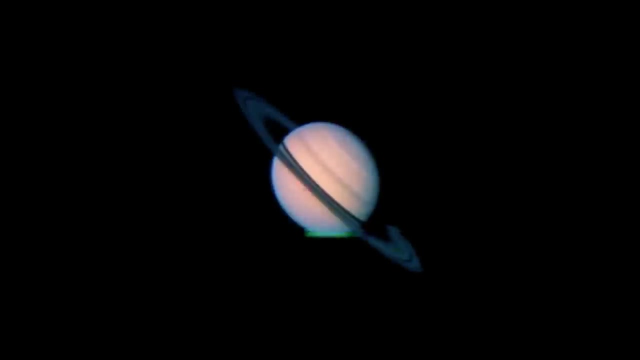 and with far greater technical difficulties. The probes were designed to be able to fly from the moon to the moon and with far greater technical capacity than the Pioneer's. In late 1980, Voyager 1 approached Saturn, Although its high-resolution polarimeter had failed. 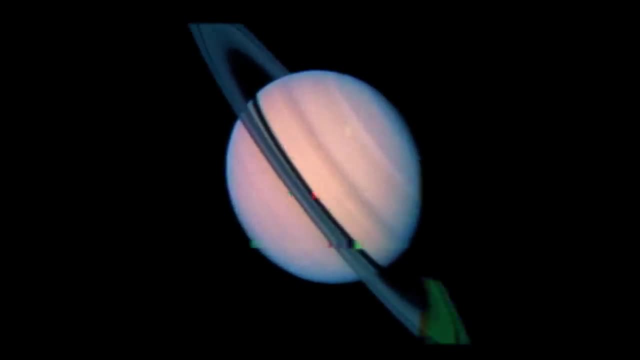 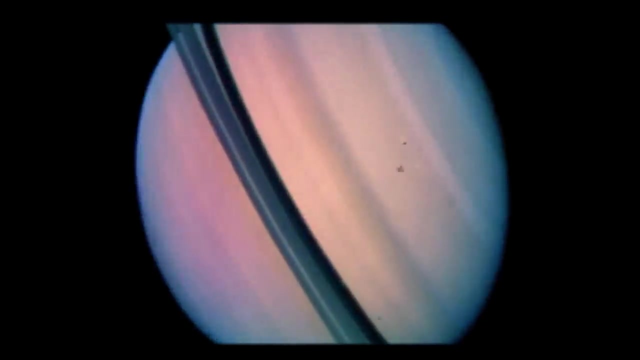 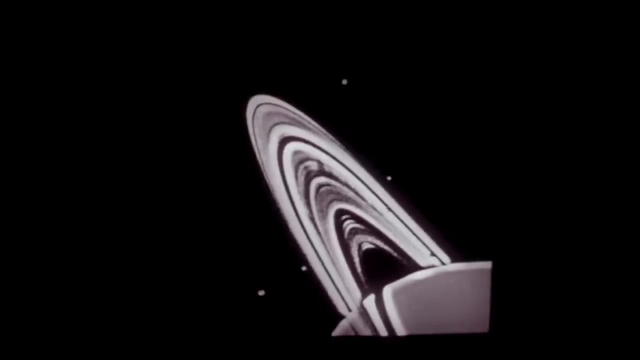 it was still able to see a new ring called the G ring, orbiting 100,000 kilometers above Saturn's cloud tops. For the first time, the probe was able to fly from the moon to the moon. For the first time, researchers could see how the rings moved. 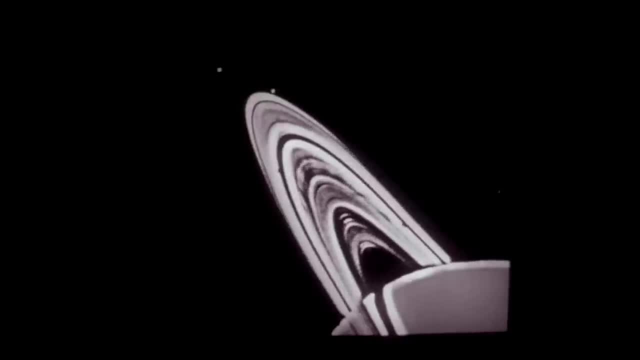 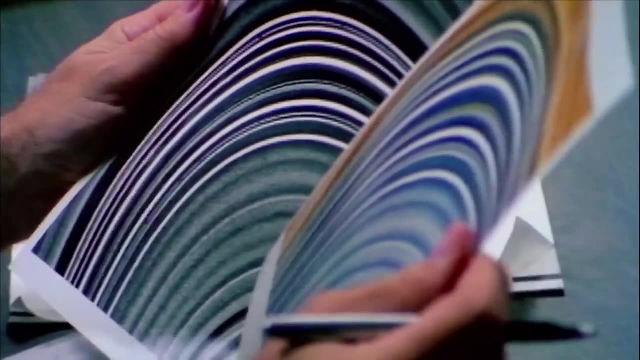 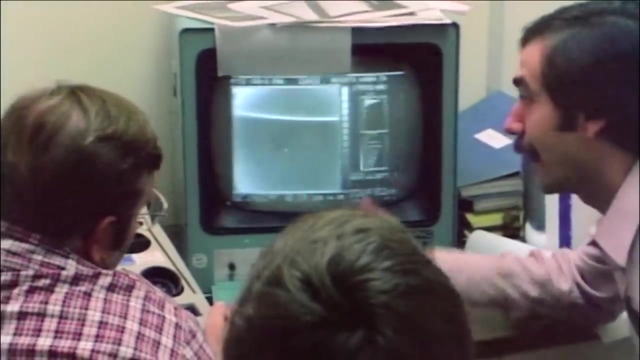 Uneven features within the rings were called spokes. They're transient and are thought to be particles lifted by an electrostatic charge. After such a long preparation, information was now coming into JPL at such a rapid rate that the planetary scientists were overwhelmed. 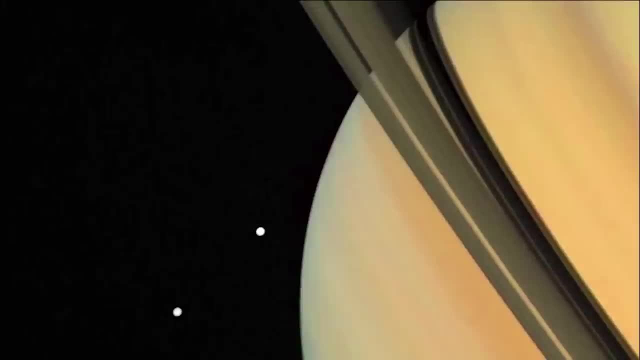 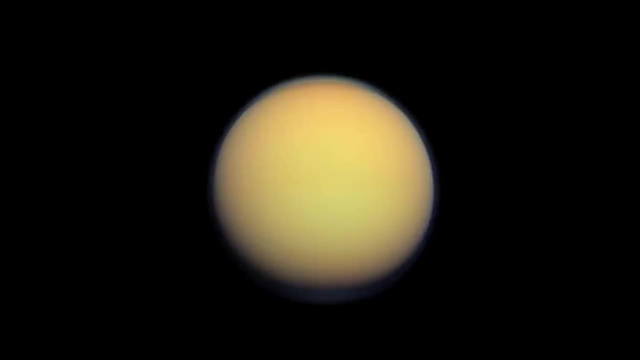 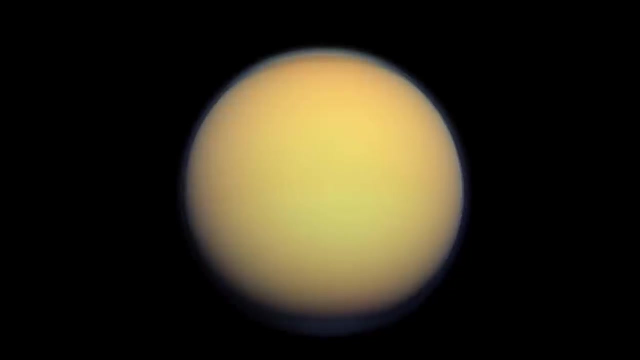 Saturn's moons were of great interest. Voyager 1's path had been chosen because it would take it close to Titan, the solar system's second-largest moon and the only one to hold an atmosphere. But the images were disappointing because the thick atmosphere of methane and nitrogen 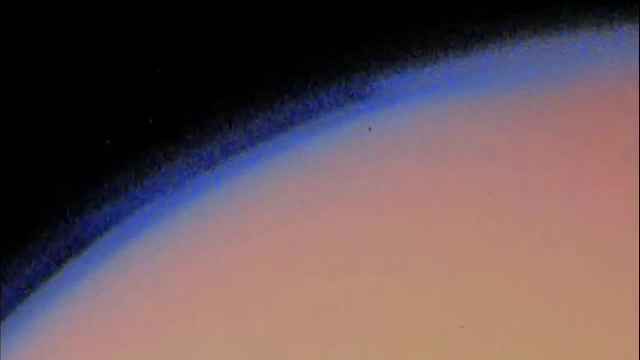 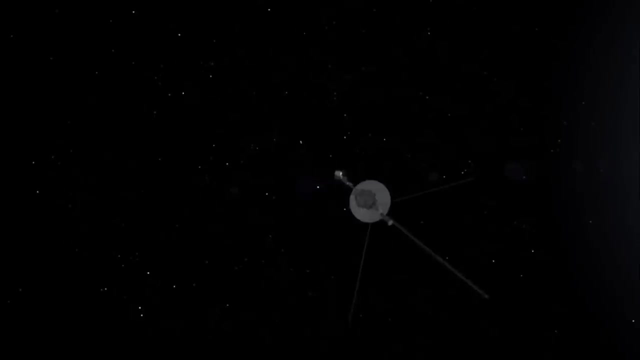 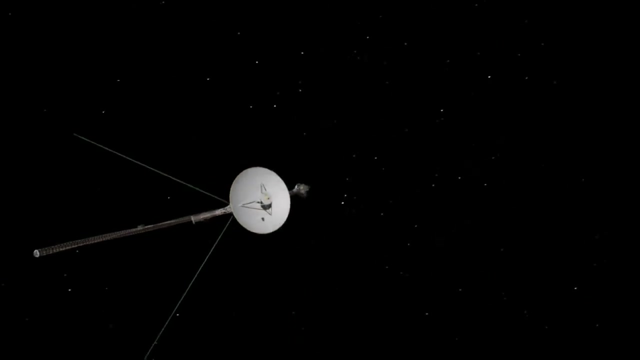 was impenetrable. Voyager 1 now looped up above the solar system on a transatlantic orbit. Voyager 2, up above the solar system on a trajectory that would take it to interstellar space As it looked back at Saturn. 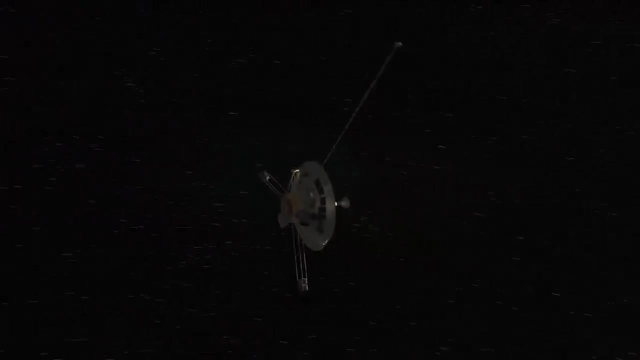 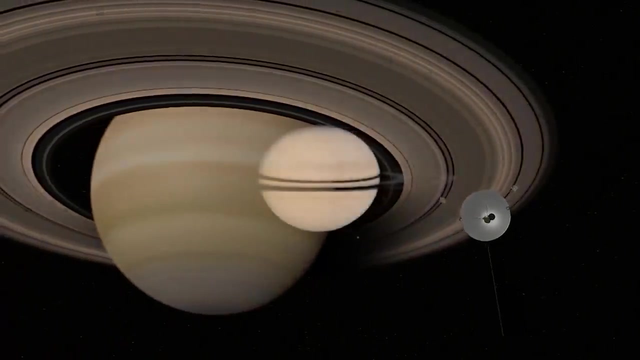 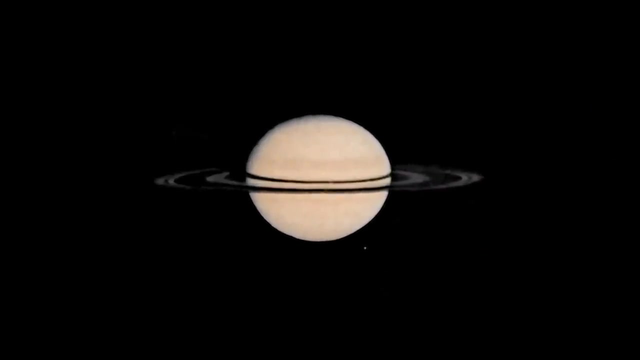 In 1979,, as Pioneer 11 approached the ringed planet, it began sending back pictures far clearer than anything seen before. A new ring, the F ring, was observed for the first time. The ring was the first to be observed on the Earth's surface. 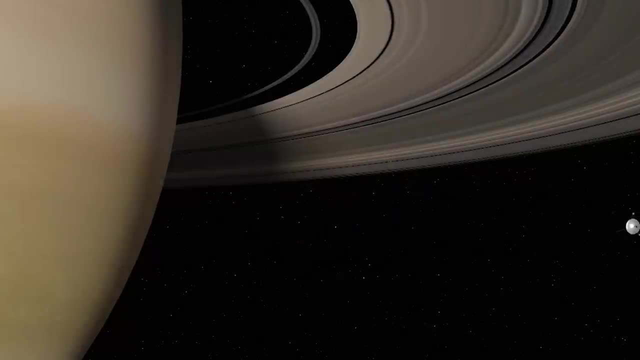 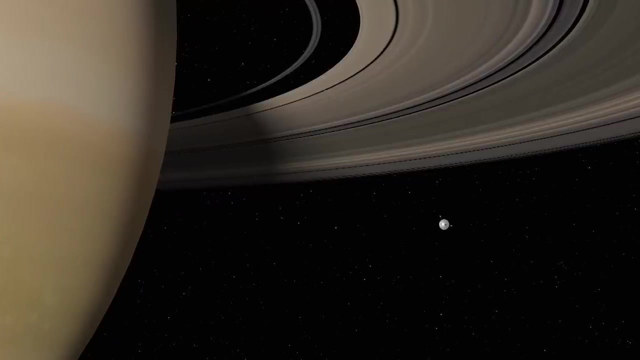 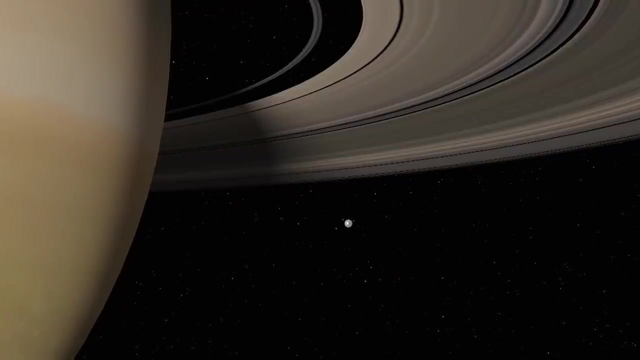 It was also the first to be observed on Mars. The craft flew by Saturn passing beneath the rings. Mission planners were uncertain how broadly the ring particles spread. If there was a threat to the spacecraft, they were prepared to sacrifice Pioneer 11 to get a clear idea of the environment. 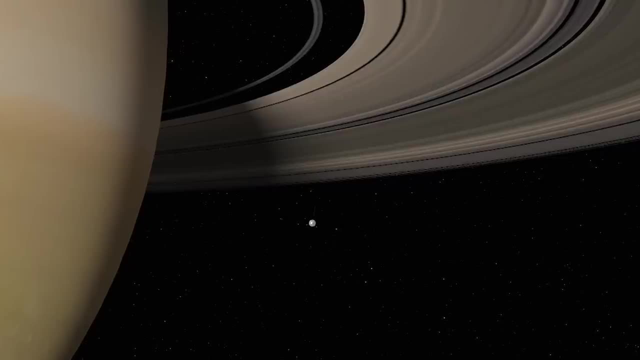 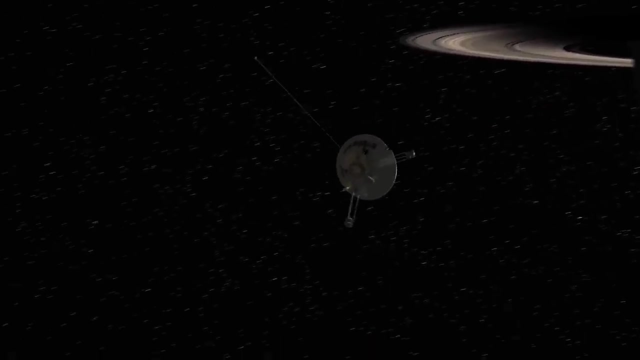 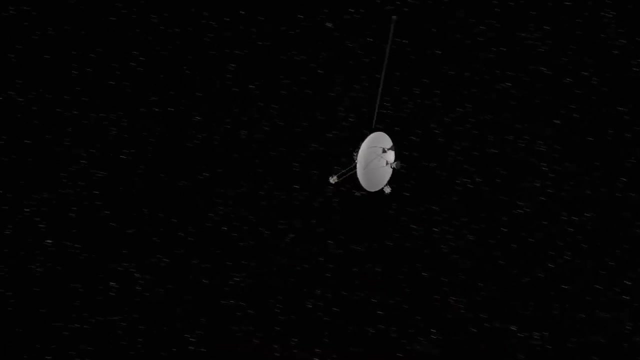 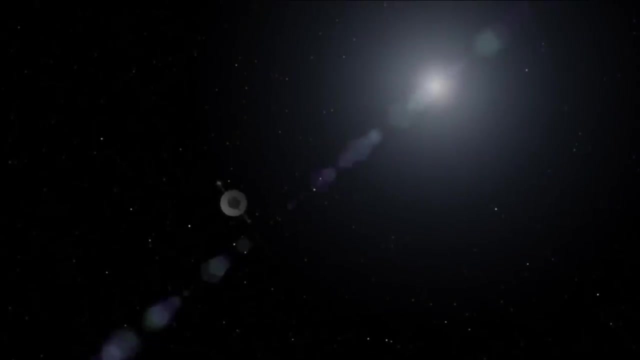 they would encounter with the following Voyager craft. The probe passed the rings safely and continued beyond Saturn into interstellar space. NASA received its last communication from the probe on the 24th of November 1995.. The following Voyager 1 and 2 probes were very robust. 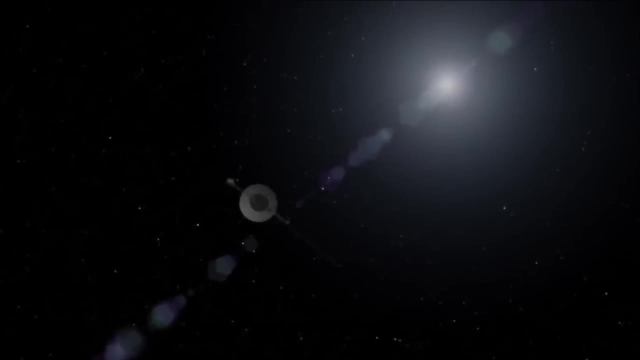 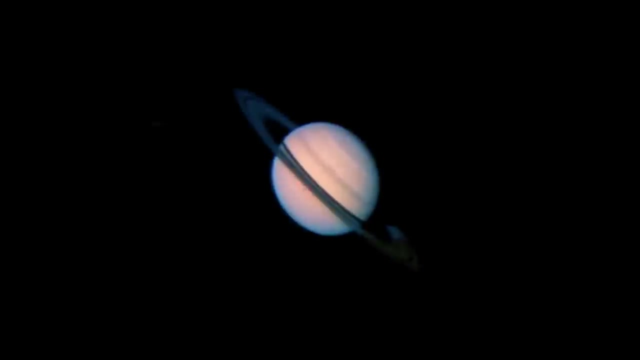 designed to survive for a very long journey and with far greater technical capacity than the Pioneer's. In late 1980, Voyager 1 was launched into space. It was the first time Voyager 1 approached Saturn, Although its high-resolution polarimeter had failed. 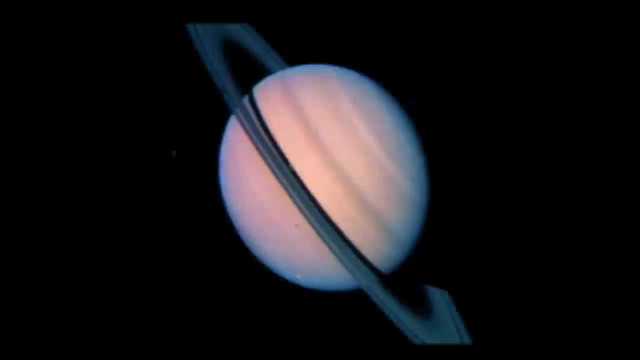 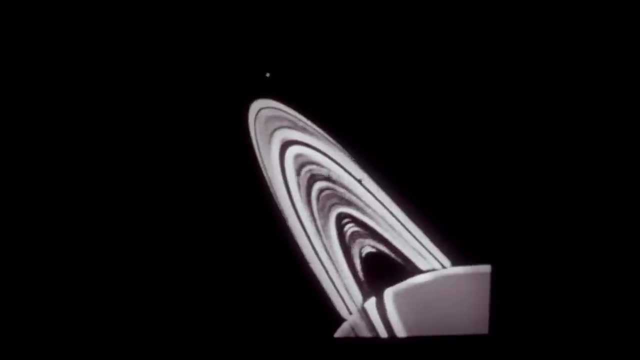 it was still able to see a new ring called the G ring, orbiting 100,000 kilometres above Saturn's cloud tops. For the first time, researchers could see how the rings moved. Uneven features within the rings were called spokes. 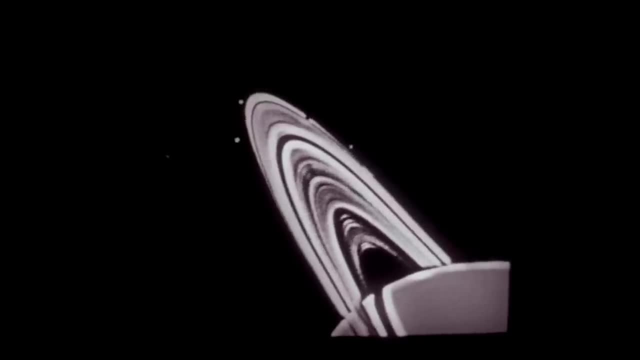 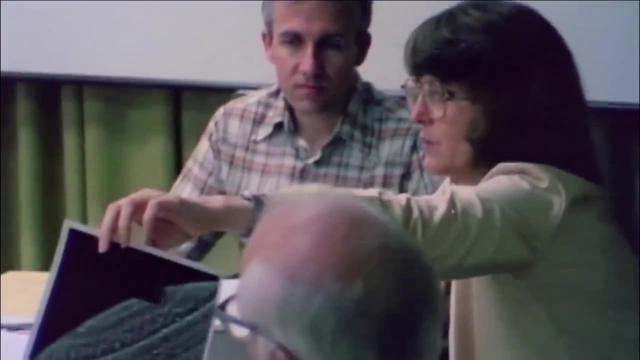 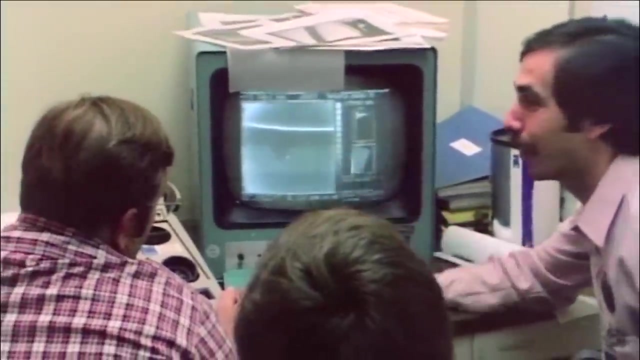 They are transient and are thought to be particles lifted by an electrostatic charge. After such a long preparation, information was now coming into JPL at such a rapid rate that the planetary scientists were overwhelmed. Saturn's moons were of great interest. Voyager 1's path had been chosen. 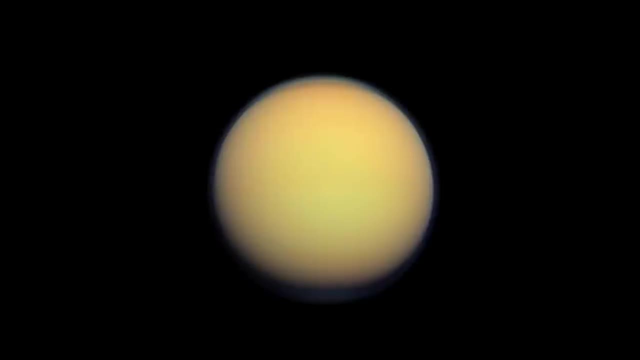 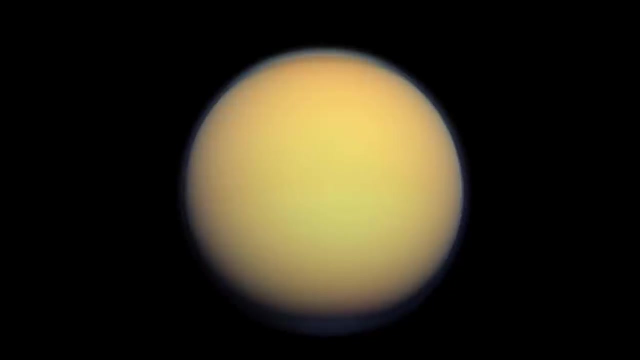 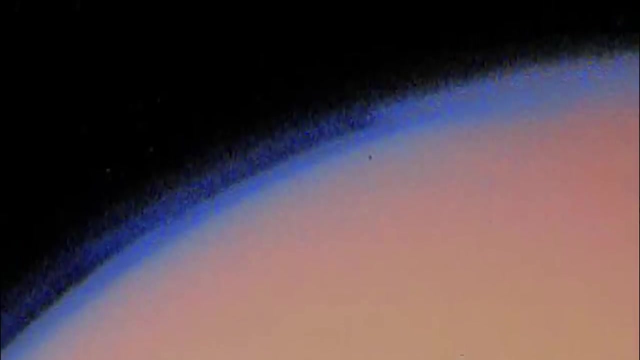 because it would take it close to Titan, the solar system's second largest moon and the only one to hold an atmosphere. But the images were disappointing because the thick atmosphere of methane and nitrogen was impenetrable. Voyager 1 now looped up above the solar system. 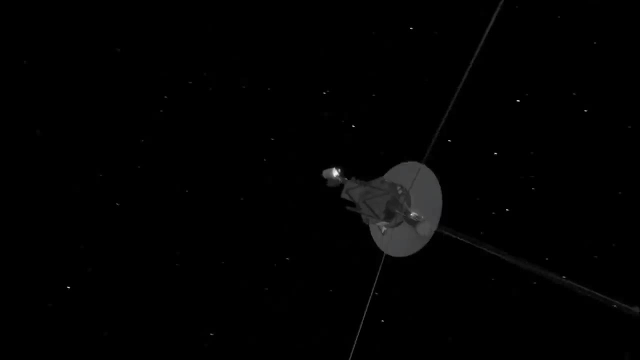 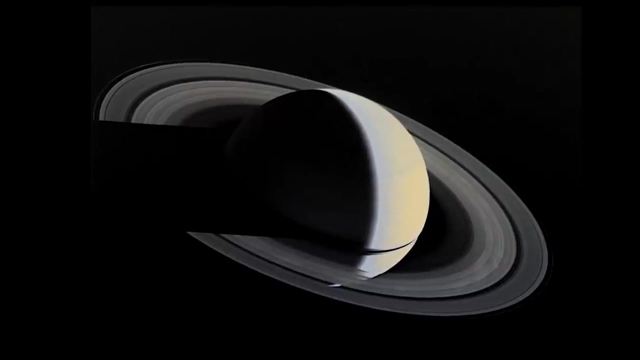 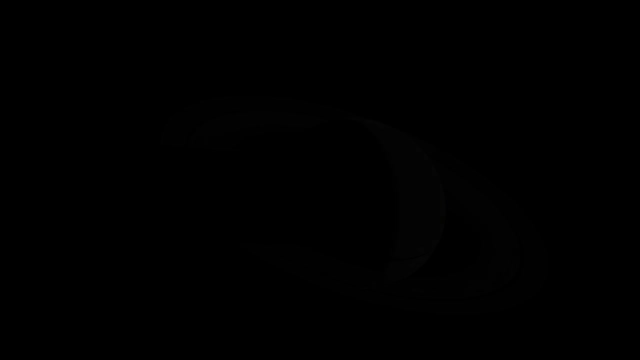 on a trajectory that would take it to interstellar space. As it looked back at Saturn, it captured one last image from a unique angle. It was almost ten months before Voyager 2 neared Saturn. Its different path meant that it could continue on to Uranus. 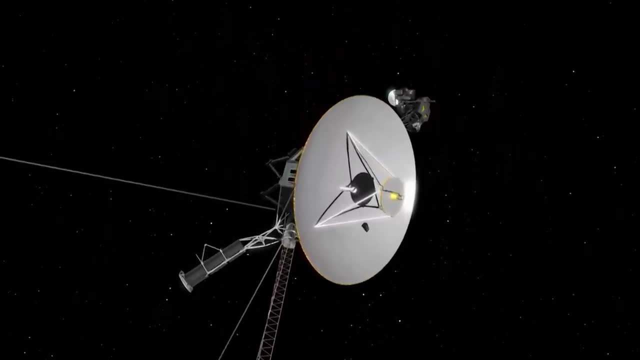 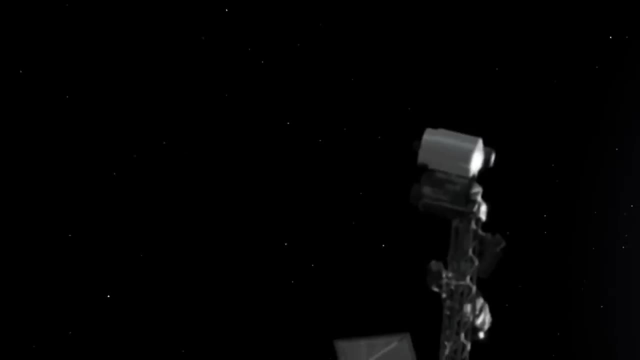 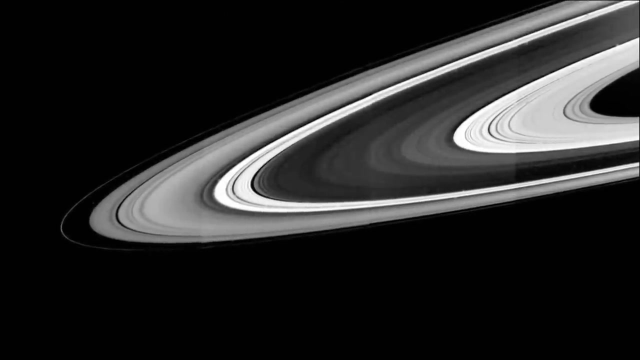 and then to Neptune. Its high-definition camera was still working and planetary researchers were expecting detailed pictures of the rings. They were not disappointed. The varying densities and spacing within the rings was more complex than anyone had expected, But they were not disappointed. The rings are named for letters of the alphabet. 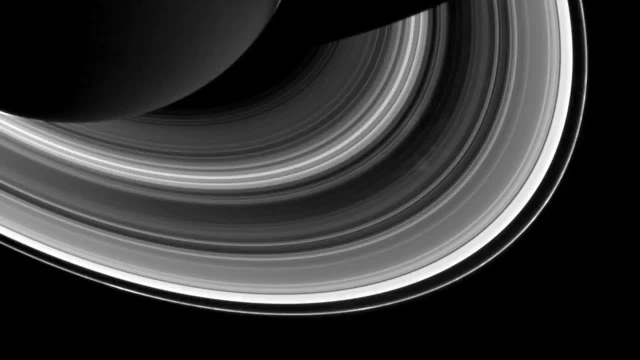 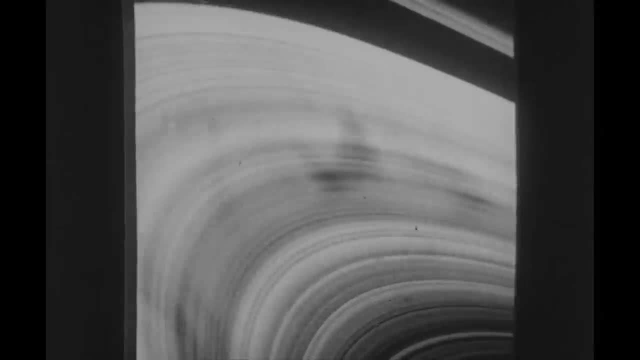 in the order that they were discovered. It became apparent that the rings had changed in the time since Voyager 1 had seen them. Though they stretch from 7,000 to 80,000 kilometers above Saturn's equator, their thickness is, on average, just 30 meters. 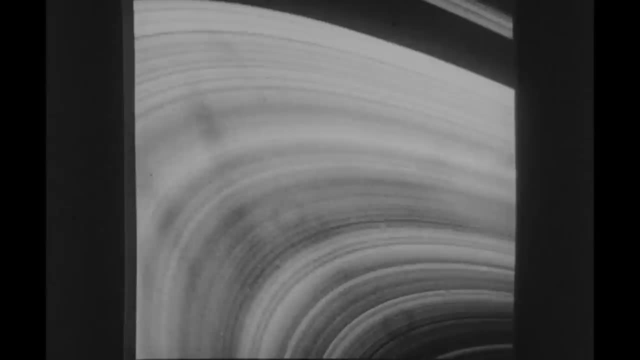 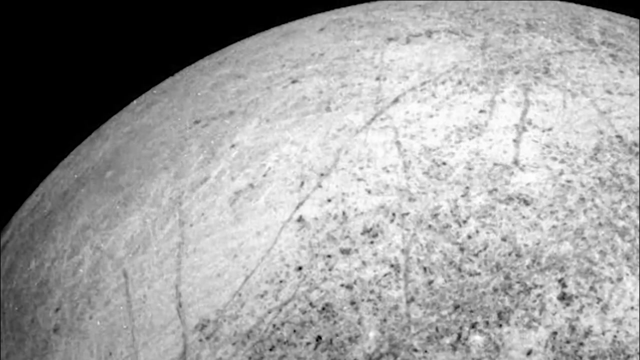 The spacecraft also returned pictures of the moon Enceladus. The moon Enceladus is the second largest moon in the world. It's cracked, uncrated surface was made of ice, below which is an ocean. Ultimately, Voyager 2 left Saturn. 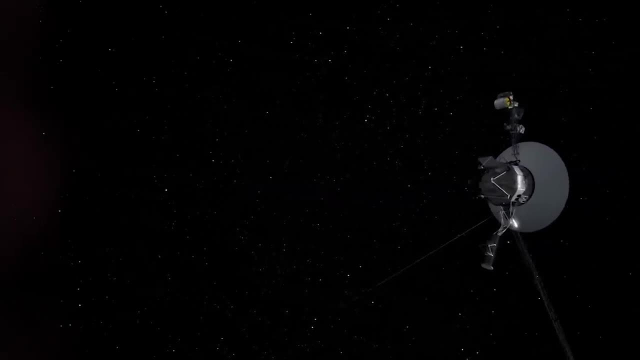 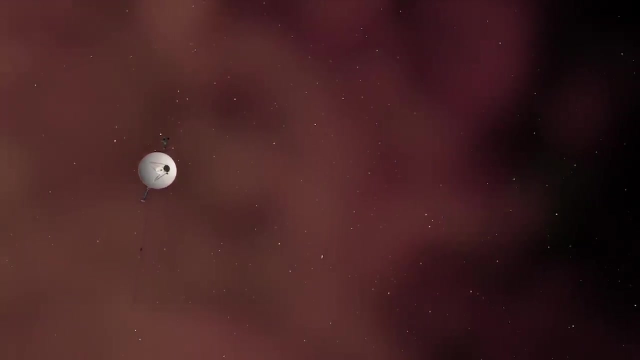 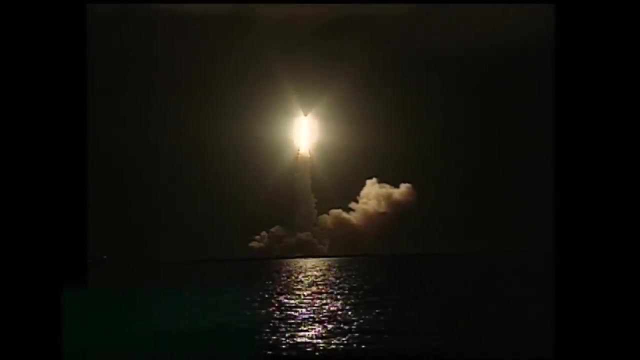 Unable to go into orbit, it sped on toward Uranus. It would be 23 years before another probe visited. And liftoff of the Cassini spacecraft on a 30-mile trek to Saturn. And liftoff of the Cassini spacecraft on a 30-mile trek to Saturn. 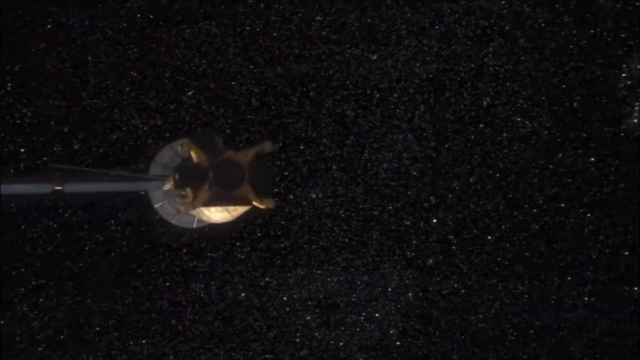 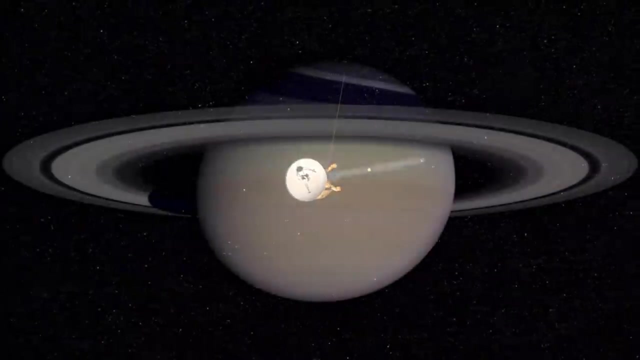 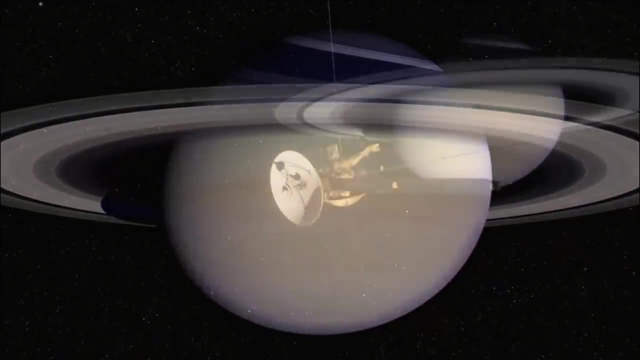 Launched in 1997, Cassini was a collaboration between NASA, the European Space Agency and the Italian Space Agency. It would take more than six years to reach Saturn. Cassini was the biggest, most complex interplanetary spacecraft yet devised. 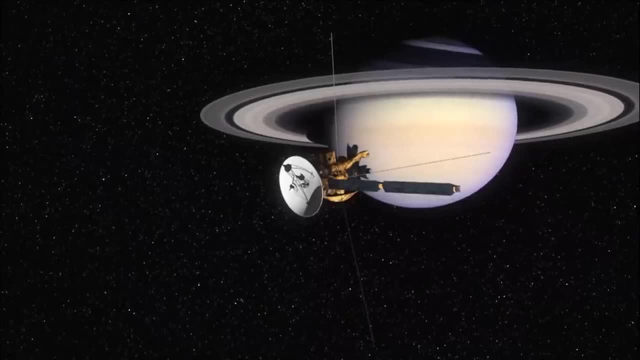 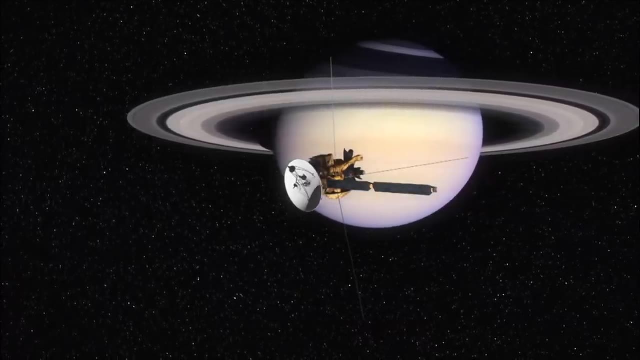 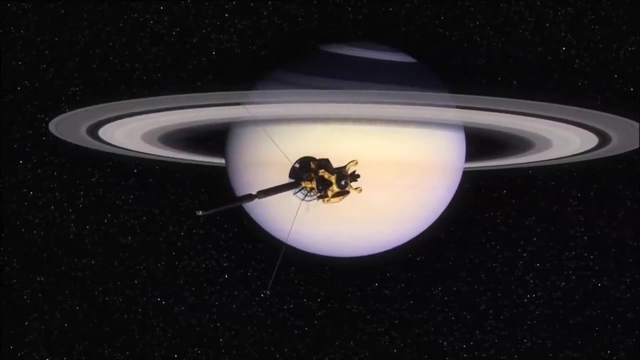 Its 12 different instruments each had a dedicated team of research specialists on Earth to interpret the data it sent back. Its high-gain antenna was used for high-speed data relay back to Earth. Its high-gain antenna was used for high-speed data relay back to Earth. 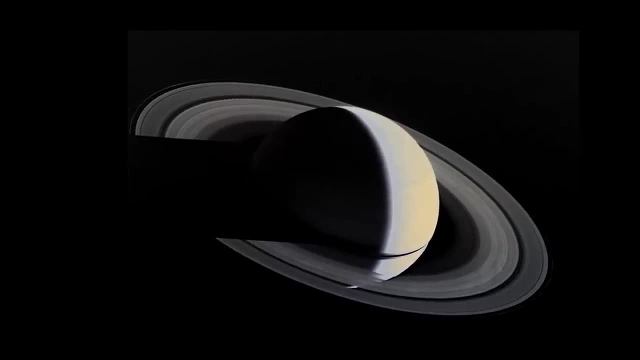 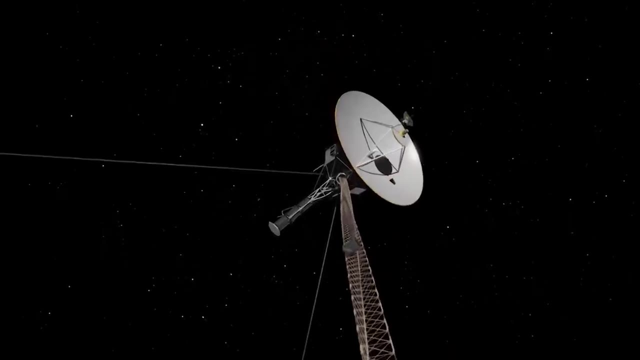 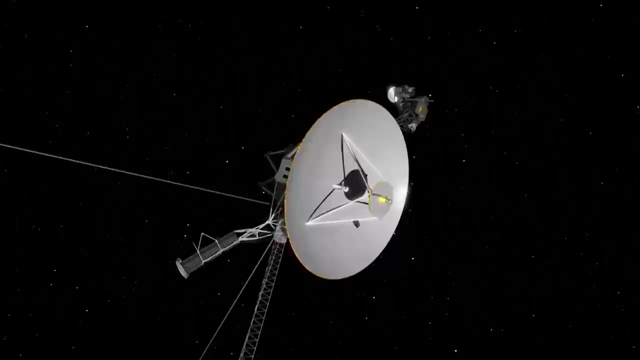 it captured one last image from a unique angle. It was almost ten months before Voyager 2 neared Saturn. Its different path meant that it could continue on to Uranus and then to Neptune. Its high-definition camera was still working and planetary researchers were expecting. 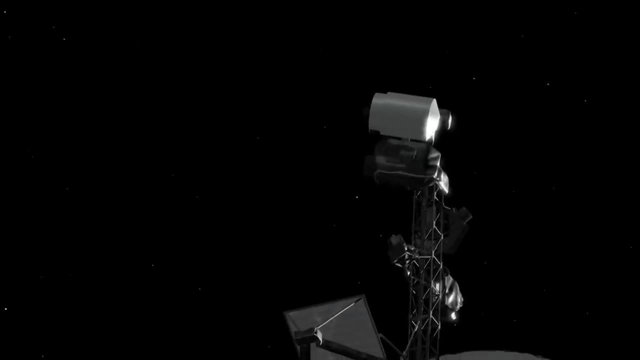 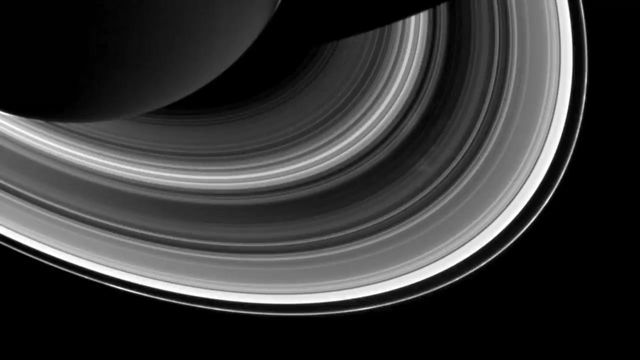 detailed pictures of the rings. They were not disappointed. The varying densities and spacing within the rings was more complex than anyone had expected. The rings are named for letters of the alphabet in the order that they were discovered. It became apparent that the rings had changed. 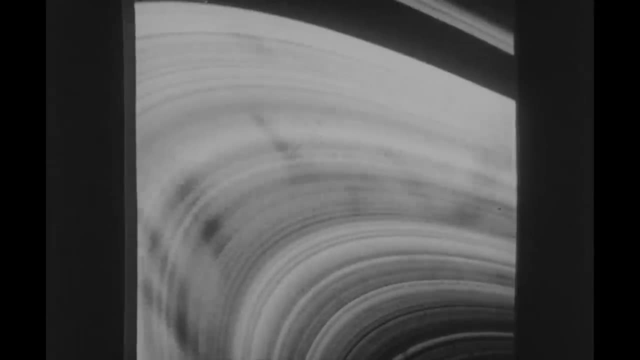 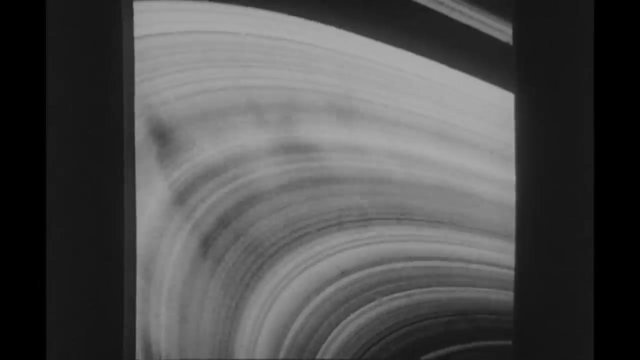 in the time since Voyager 1 had seen them. Though they stretch from 7,000 to 80,000 kilometers above Saturn's equator, their thickness is, on average, just 30 meters. The spacecraft also returned pictures of the moon Enceladus. 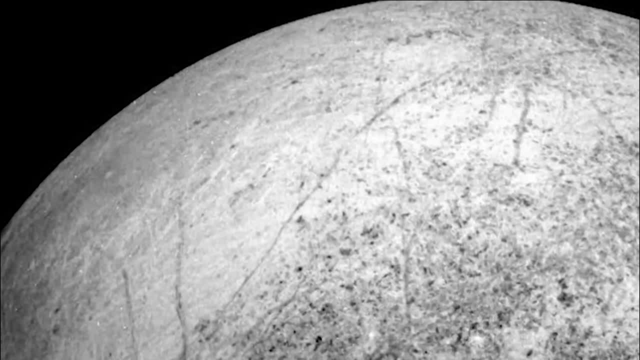 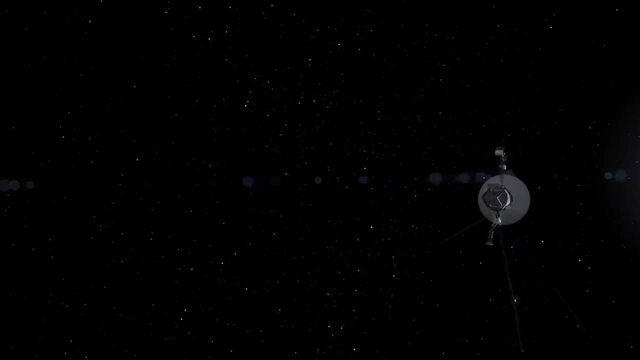 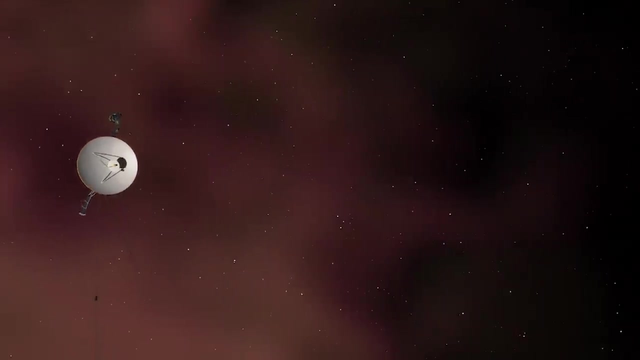 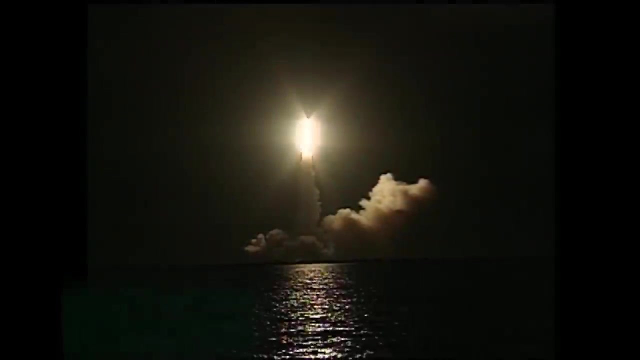 Its cracked, uncrated surface was made of ice, below, which is an ocean. Ultimately, Voyager 2 left Saturn Unable to go into orbit. it sped on toward Uranus- It would be 23 years before another probe visited- And liftoff of the Cassini spacecraft. 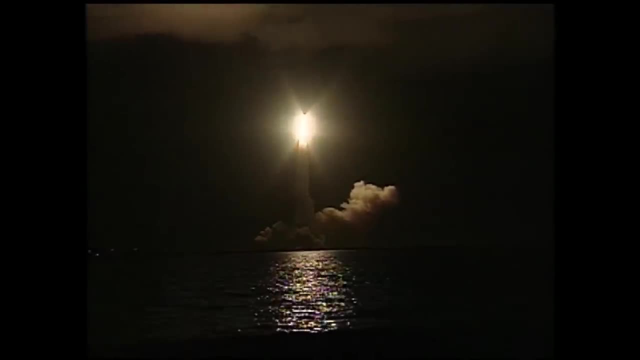 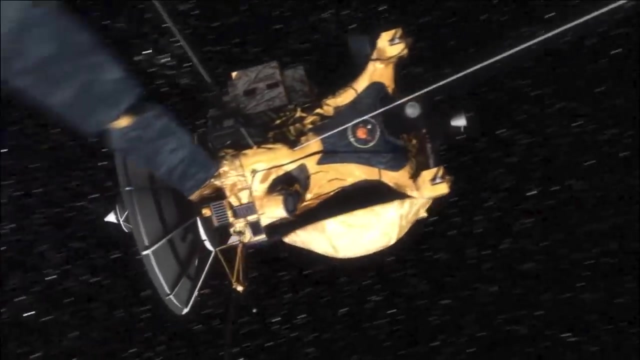 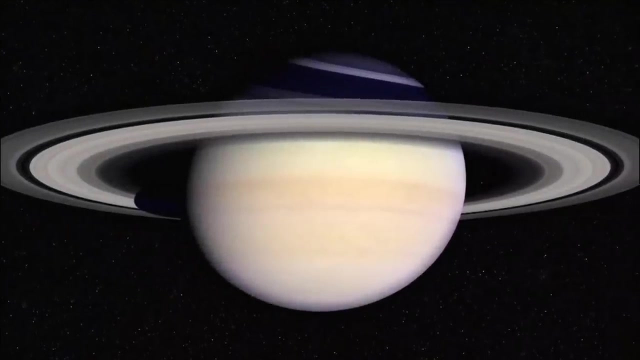 on a 30-mile trek to Saturn. Launched in 1997, Cassini was a collaboration between NASA, the European Space Agency and the Italian Space Agency. It would take more than six years to reach Saturn. Cassini was the biggest, most complex. 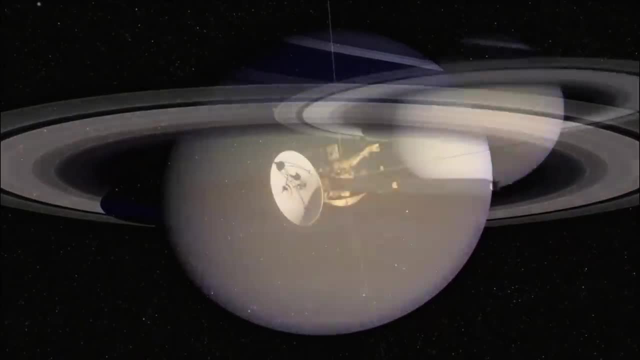 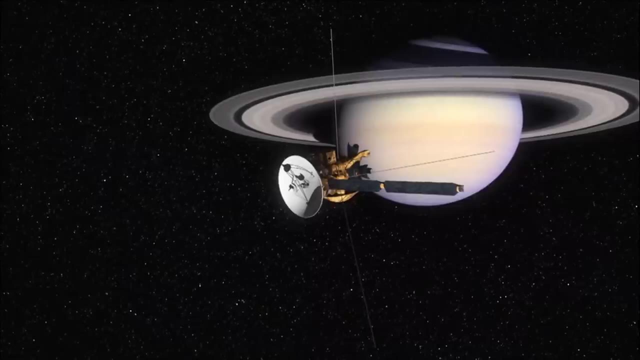 interplanetary spacecraft yet devised Its 12 different instruments each had a dedicated team of research specialists on Earth to interpret the data it sent back. Its high-gain antenna was used for high-speed data relay back to Earth. It was also used to send data back to Earth. 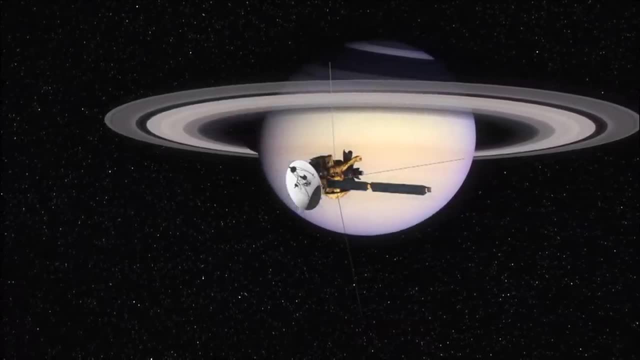 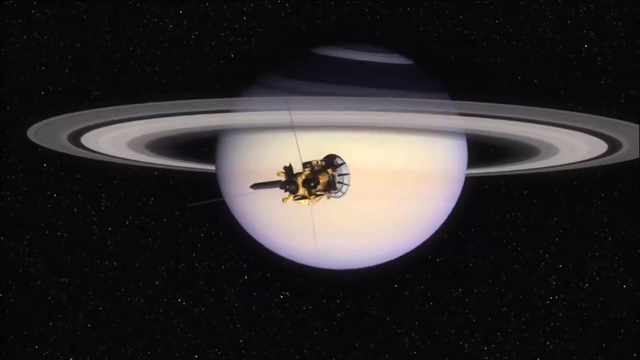 from the Earth's atmosphere. Cassini was the largest, most complex interplanetary spacecraft yet devised. Its high-gain antenna was used for high-speed data relay back to Earth, But in what's called a RAM maneuver it was sometimes used as a shield. 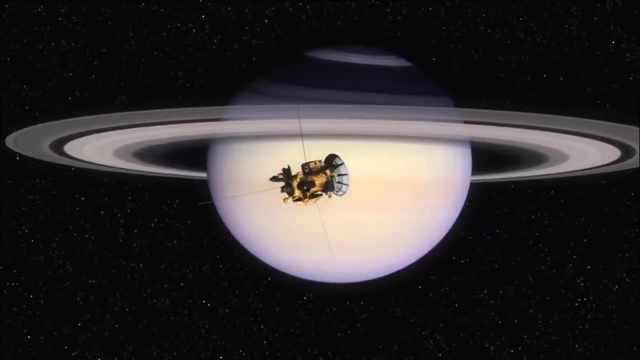 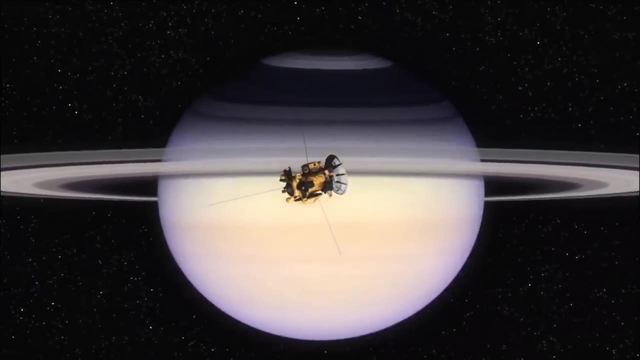 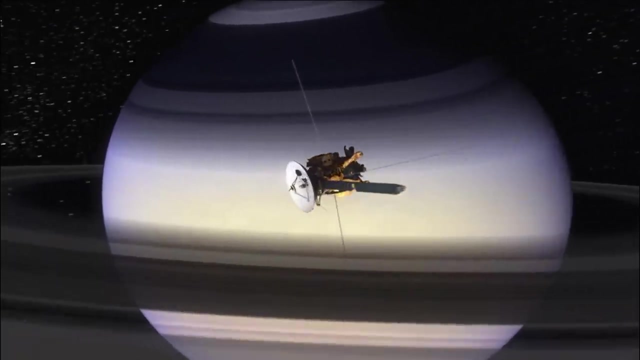 But in what's called a RAM maneuver, it was sometimes used as a shield to protect the spacecraft from debris impact, especially when crossing the plane of Saturn's rings. especially when crossing the plane of Saturn's rings. On the 1st of July 2004,, it fired its engine to go into orbit around Saturn. 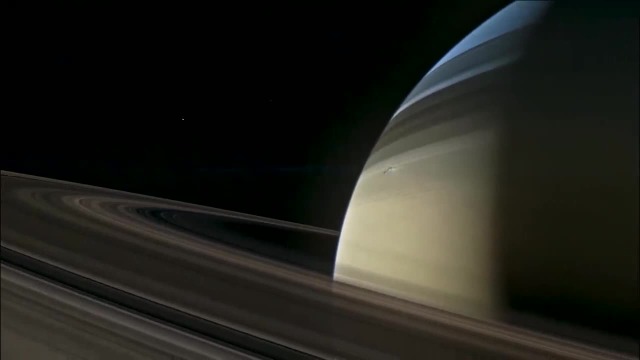 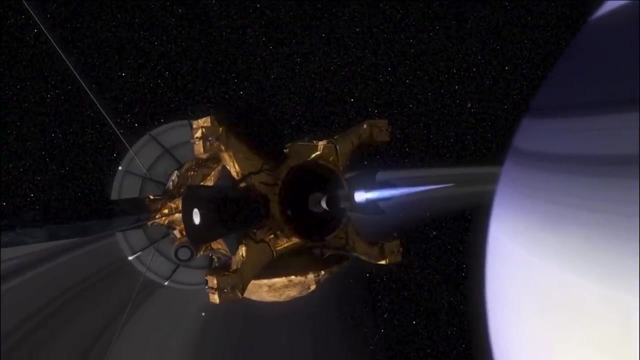 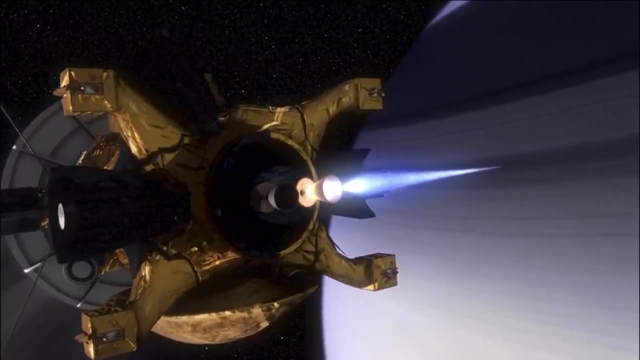 On the 1st of July 2004,. it fired its engine to go into orbit around Saturn. It was designed not to fail. Beside its main engine was a backup in case the primary engine did fail. It had sixteen monopropellant thrusters: eight prime and eight more also as backups. 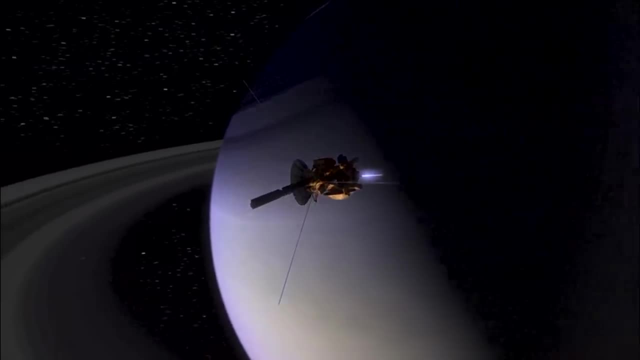 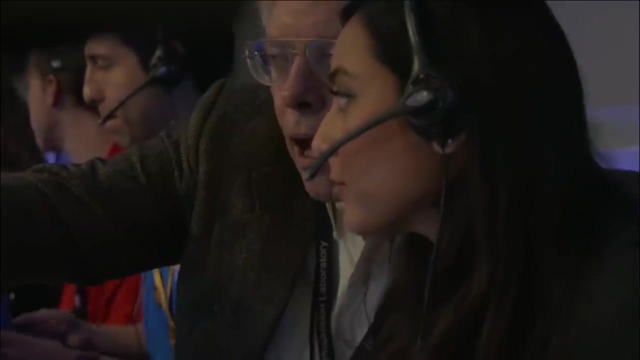 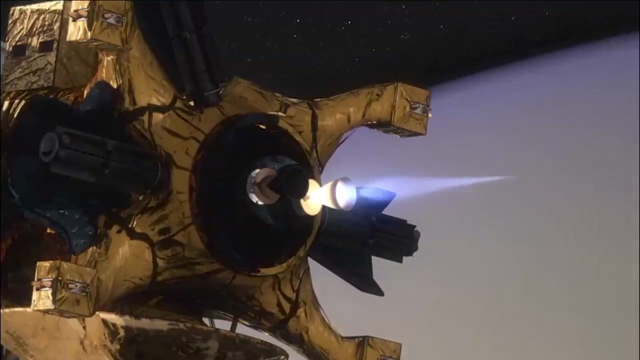 It had sixteen monopropellant thrusters, eight prime and eight more also as backups In mission control of the Jet Propulsion Laboratory. the engineers could not know what was going on. The time delay and Cassini's disappearance behind Saturn meant that much of the telemetry was recorded for later replay back to Earth. 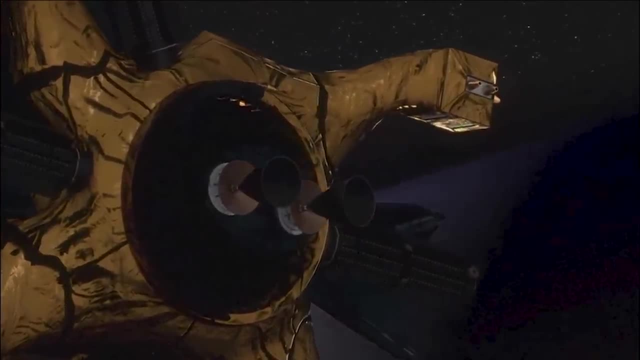 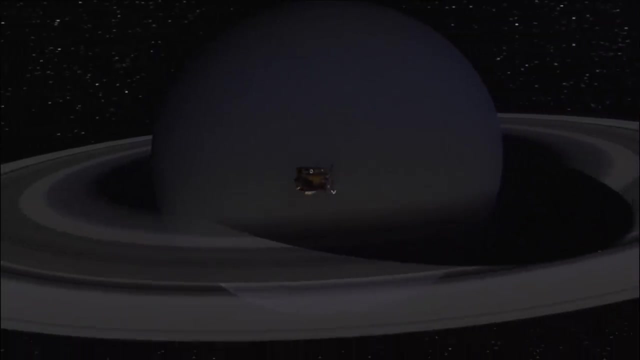 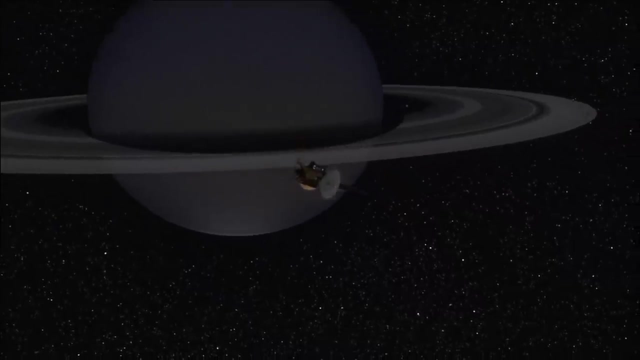 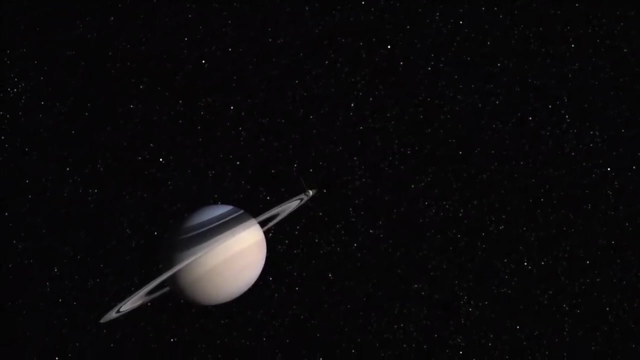 The engine burn lasted for 106 minutes. Cassini was the first probe to employ a solid-state recorder, unlike the earlier Voyager craft that registered data on a mechanical tape recorder, Cassini's first orbit followed a highly elliptical path that would take it out past the moon Titan. 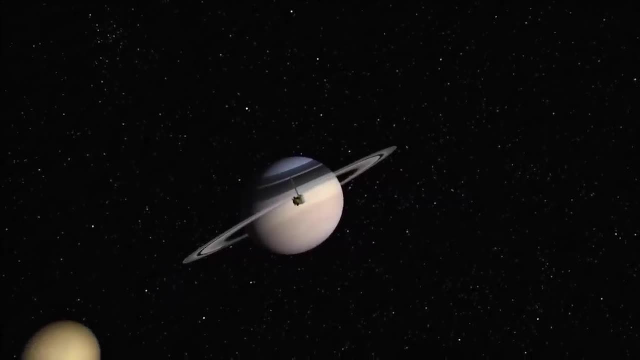 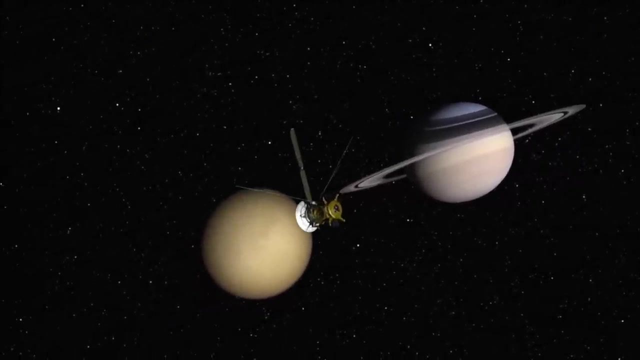 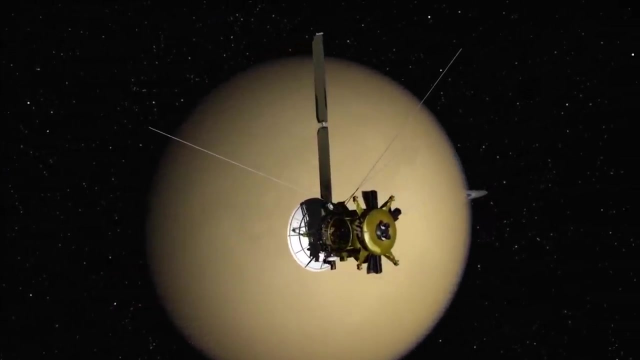 This was important for two reasons. Its gravity would be necessary in modifying Cassini's course, so Saturn and its other moons could be observed from different perspectives. Secondly, Titan, with its dense atmosphere, was targeted as an area of major interest for the Cassini team. 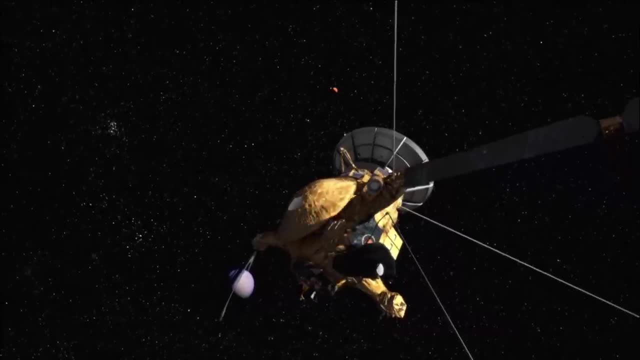 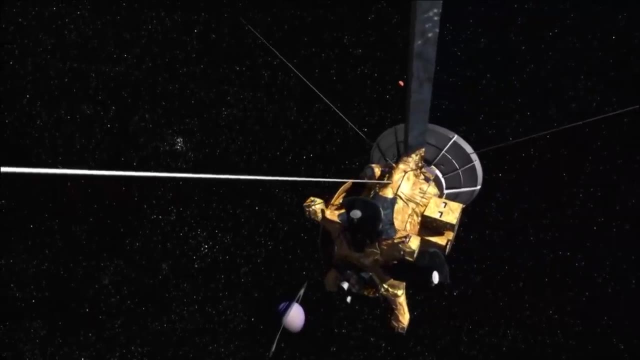 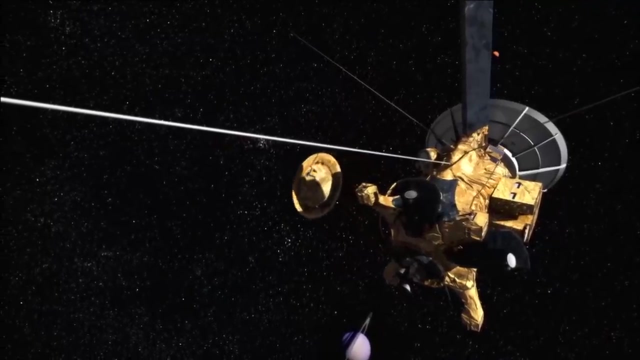 The European Space Agency had built a small craft called Huygens attached to the side of Cassini. On its second approach to Titan, the Huygens probe was released. It was equipped with a heat shield, a parachute and enough battery power to last for several weeks. 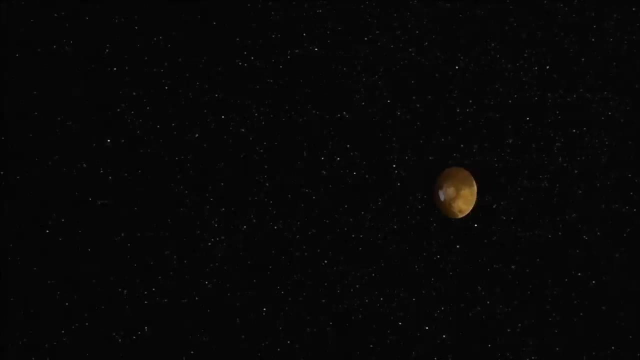 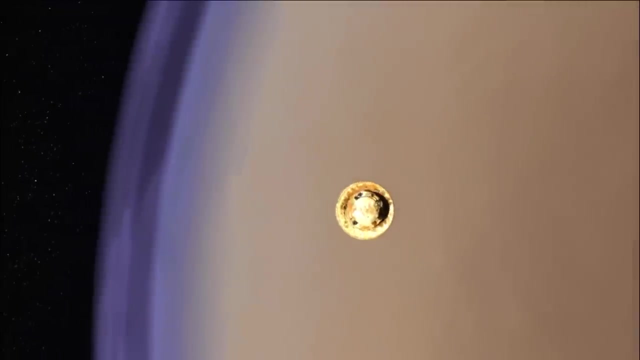 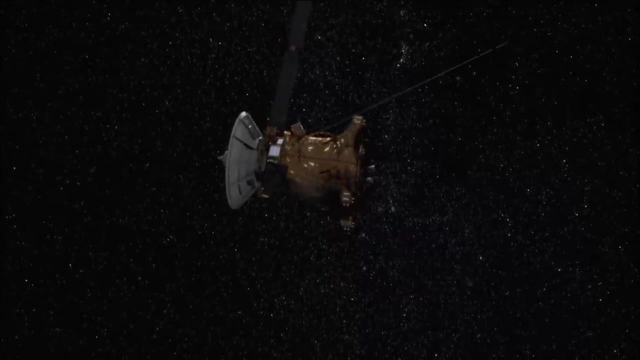 Over a 20-day period, Huygens drifted for 4 million kilometers. It would transmit data back to the orbiting Cassini, which would later relay it to Earth. Three days after separation, Cassini made a course correction that would prevent it colliding with Titan. 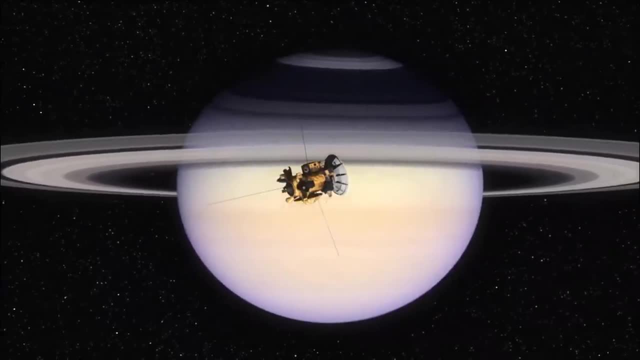 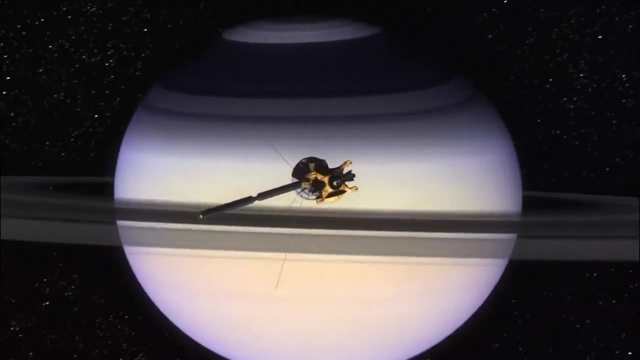 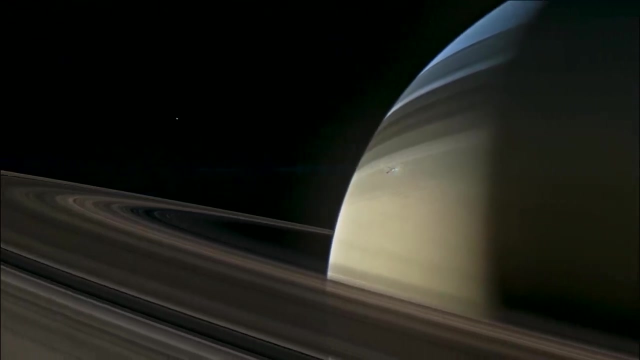 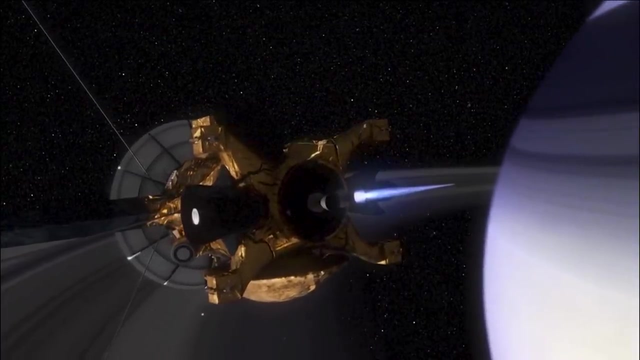 to protect the spacecraft from debris impact, especially when crossing the plane of Saturn's rings. On the 1st of July 2004,, it fired its engine to go into orbit around Saturn. It was designed not to fail. Beside its main engine was a backup. 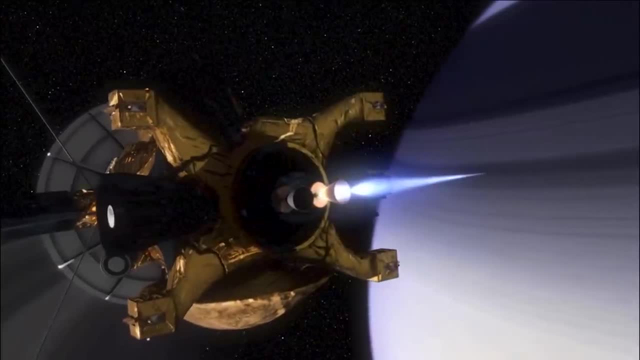 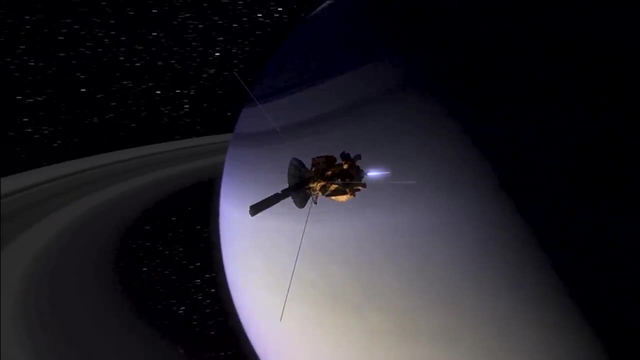 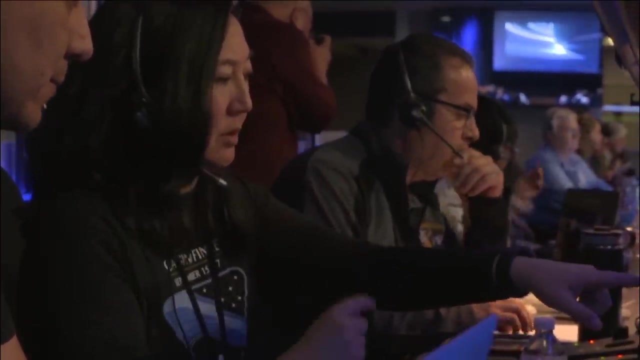 in case the primary engine did fail. It had 16 monopropellant thrusters, eight prime and eight more also as backups In mission control of the Jet Propulsion Laboratory. the engineers could not know what was going on, The time delay and Cassini's disappearance behind Saturn. 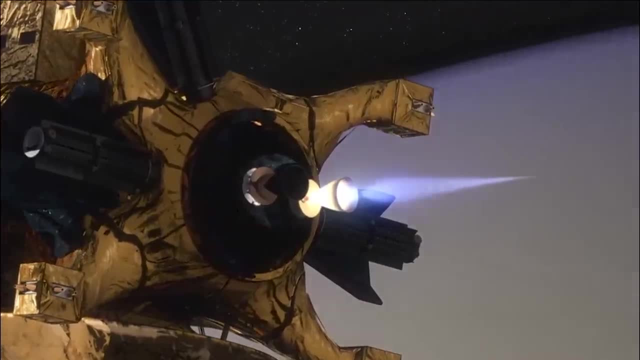 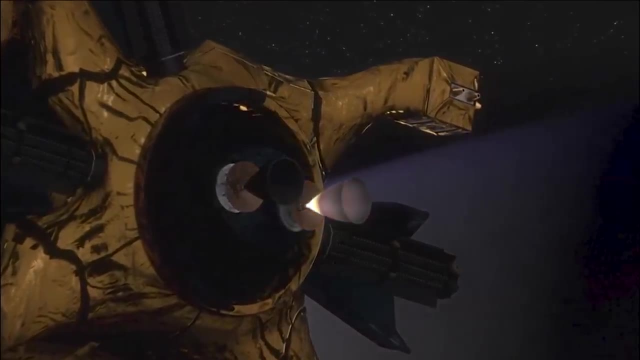 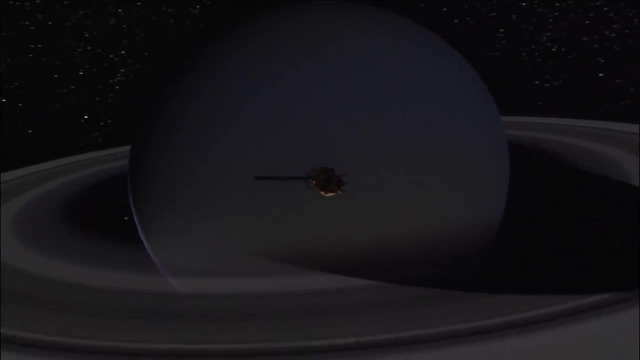 meant that much of the telemetry was recorded for later replay back to Earth. The engine burn lasted for 106 minutes. Cassini was the first probe to employ a solid-state recorder, unlike the earlier Voyager craft that registered data on a mechanical tape recorder. 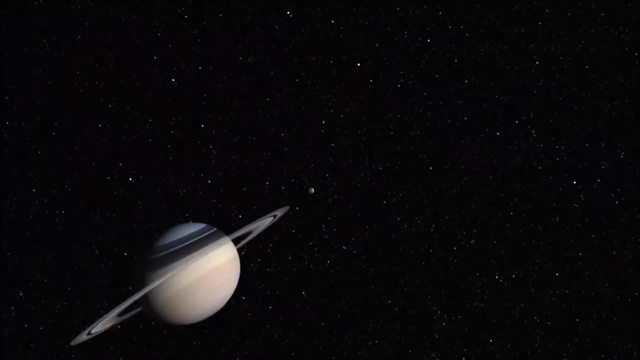 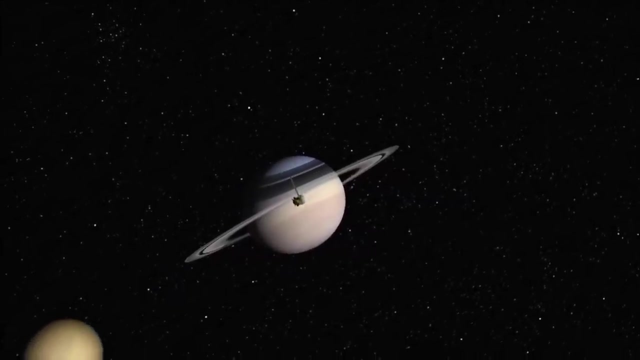 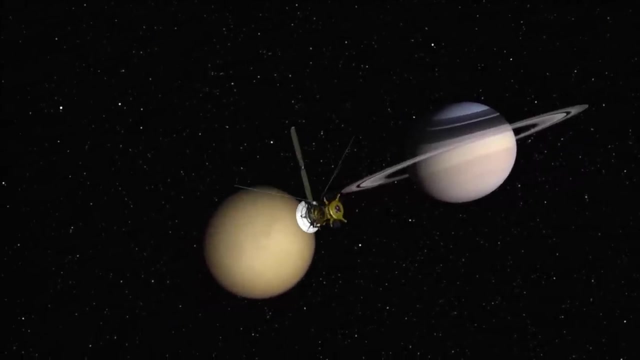 Cassini's first orbit followed a highly elliptical path that would take it out past the moon Titan. This was important for Cassini for two reasons. Its gravity would be necessary in modifying Cassini's course, so Saturn and its other moons could be observed from different perspectives. 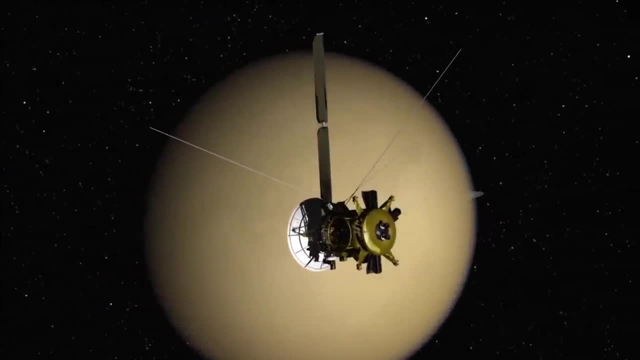 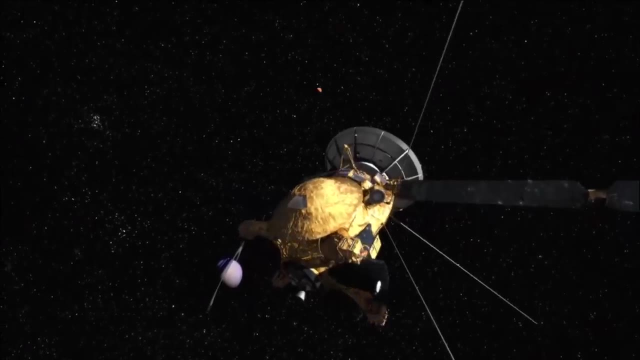 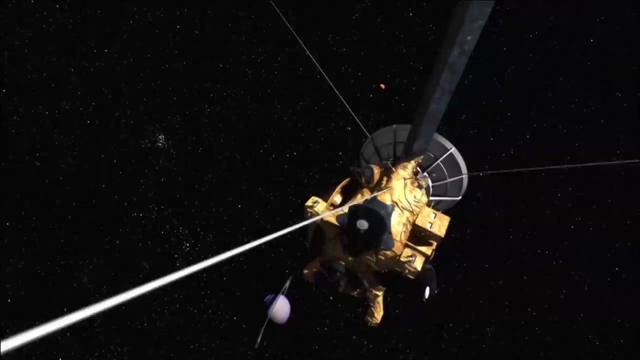 Secondly, Titan, with its dense atmosphere, was targeted as an area of major interest for the Cassini team. The European Space Agency had built a small craft called Huygens attached to the side of Cassini On its second approach to Titan. 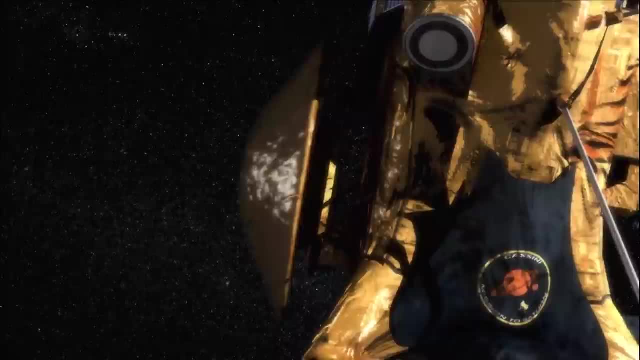 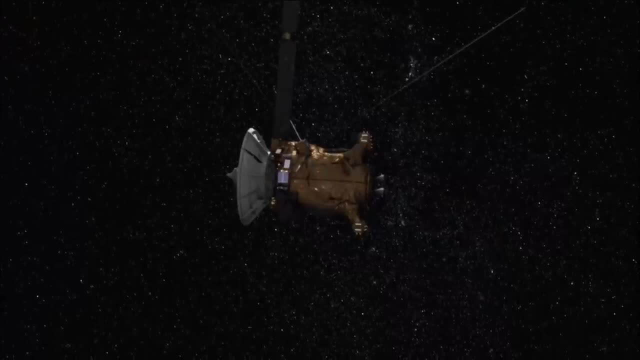 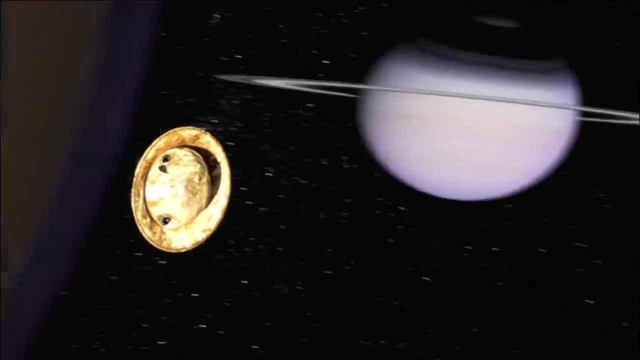 the Huygens probe was released. It was equipped with a heat shield, a parachute and enough battery power to last for several weeks. Over a 20-day period, Huygens drifted for 4 million kilometers. It would transmit data back to the orbiting Cassini. 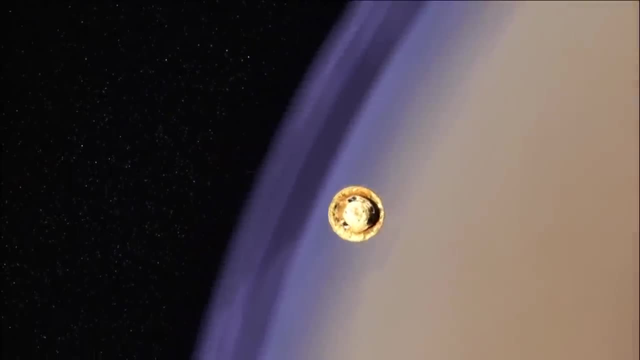 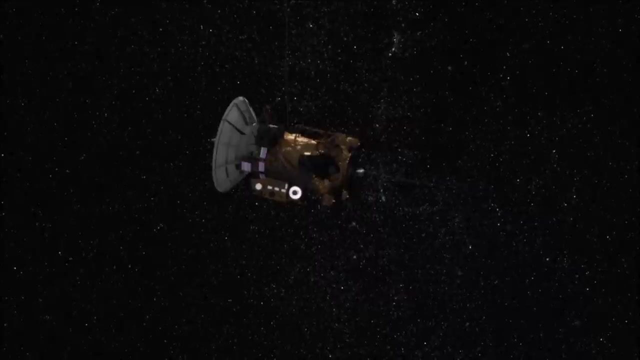 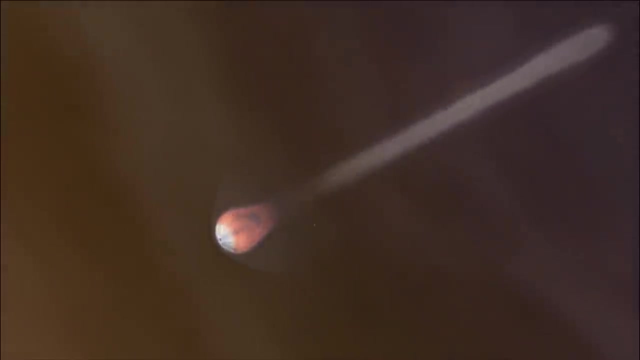 which would later relay it to Earth. Three days after separation, Cassini made a course correction that would prevent it colliding with Titan. As Huygens reached Titan's atmosphere, Cassini was coming around for its third close approach of the moon. 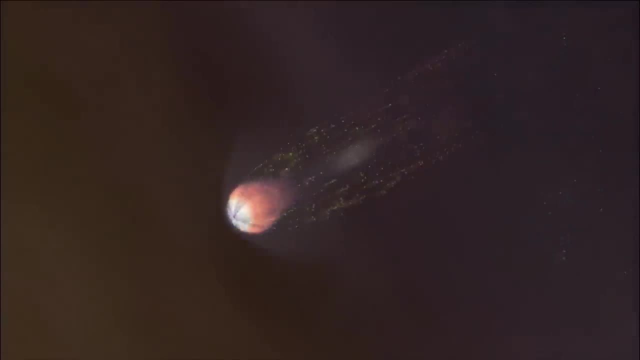 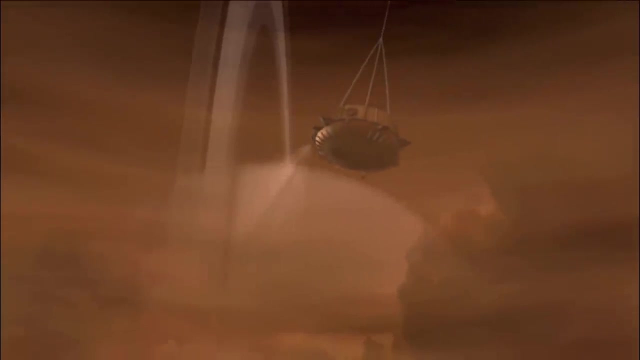 As Huygens reached Titan's atmosphere, Cassini was coming around for its third close approach to Earth. The Huygens were on the edge of the Moon, ready to receive signals from the lander While it drifted to the surface of Titan. 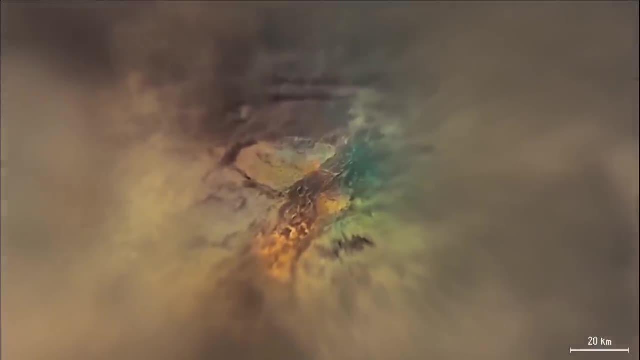 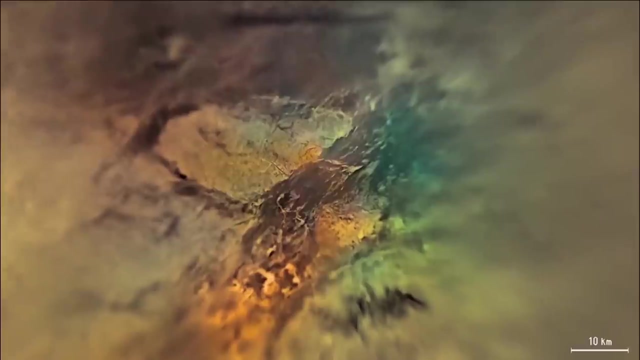 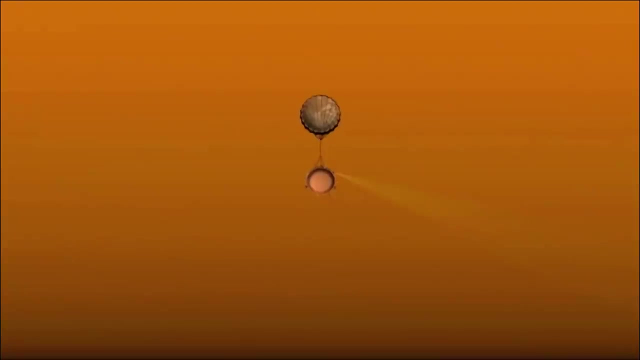 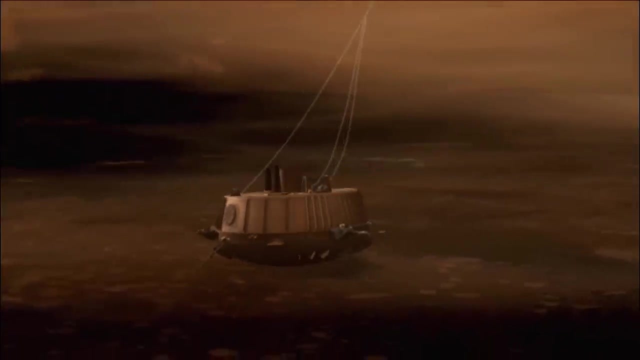 Huygens sampled the atmosphere and recorded images of the landscape. Pictures from beneath the clouds revealed low hills and channels cut by flowing liquid. There were few impact craters, but the rocks that existed were heavily eroded. It was the first landing on a body in the outer solar system. 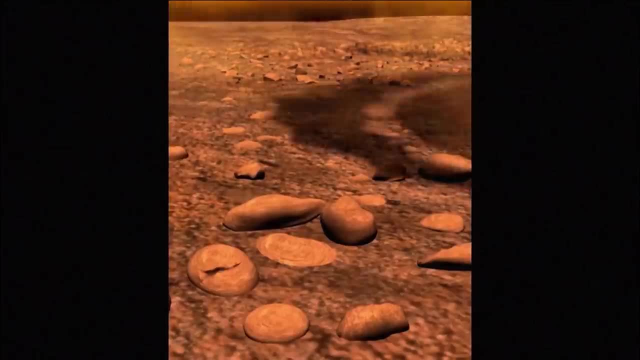 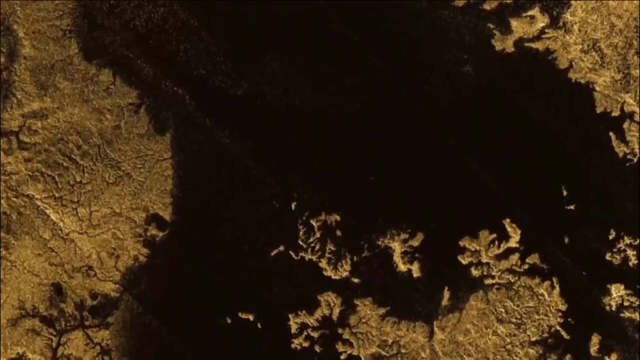 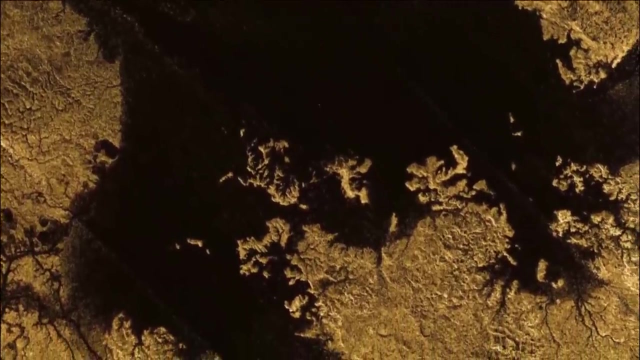 Images from the surface showed weathered rocks made of water ice. What surprised everybody was that Titan is a geologically active world, and liquid ethane and methane, rather than water, have carved the features As Cassini continued looping out around Titan. it used radar to map the Moon's surface, confirming the widespread distribution of hydrocarbon lakes. The probe discovered that rain fell on Titan, but it was a mixture of liquid, ethane and methane. The Moon has weather and other erosive forces similar to Earth. 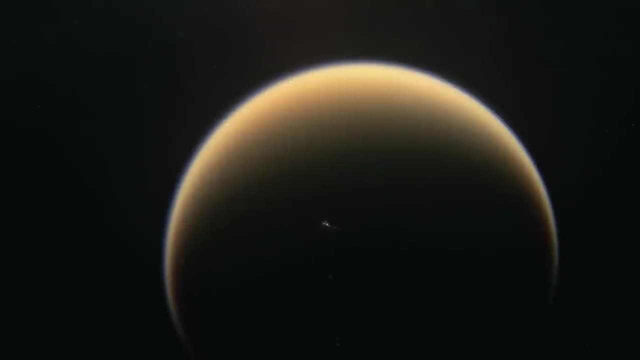 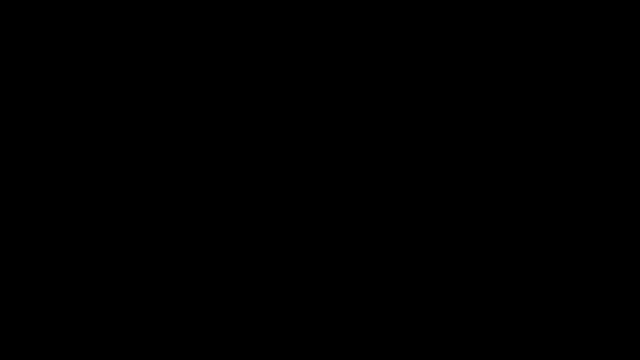 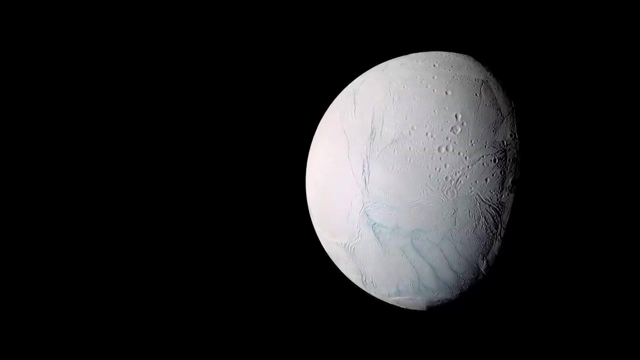 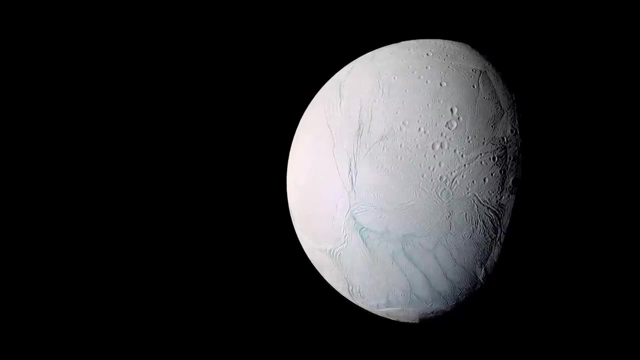 but the chemistry is radically different. The small Moon Enceladus drew attention to itself as the whitest, most reflective body in the solar system. Its surface shows cratering in the north, but the south has giant cracks known as tiger stripes. 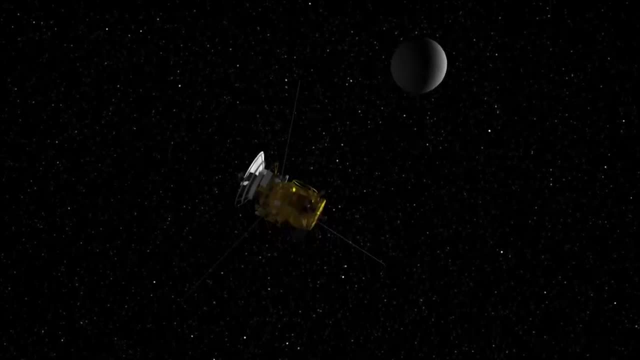 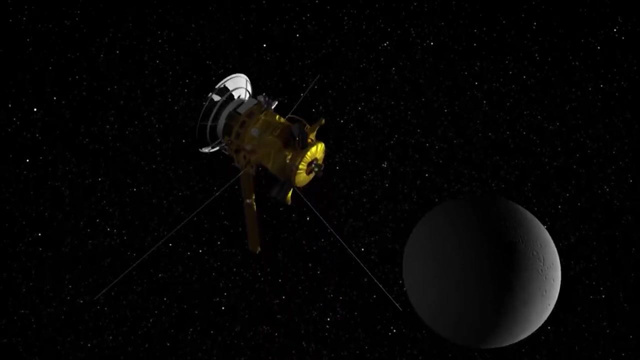 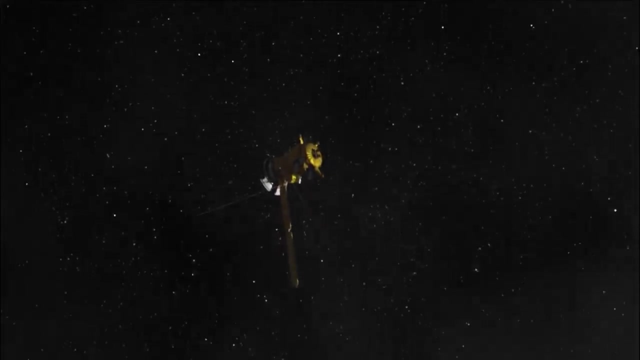 On Cassini's first loop past Enceladus, the magnetometer team noticed an odd deflection of Saturn's magnetic field, as though the small Moon had an atmosphere. During its second pass, the team noticed the same phenomenon. They asked for the next traverse of Enceladus to pass much closer. 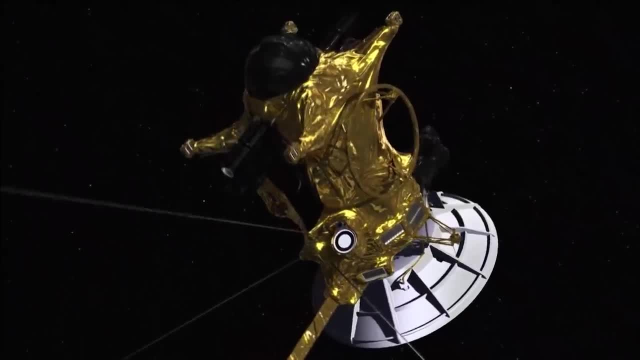 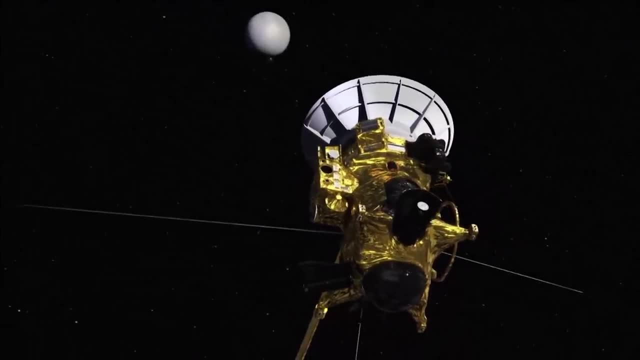 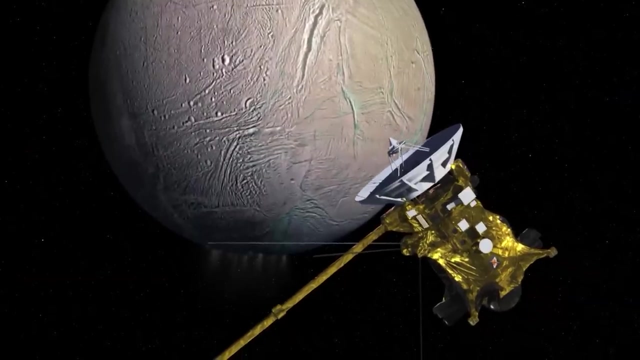 so Cassini's course was modified to fly just 175 kilometers above the icy Moon. The probe passed through a plume of water vapor emanating from the tiger stripes. It contained common salt. In all, Cassini made 24 swoops past Enceladus. 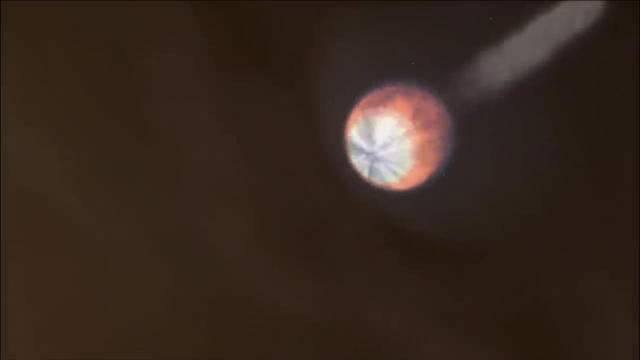 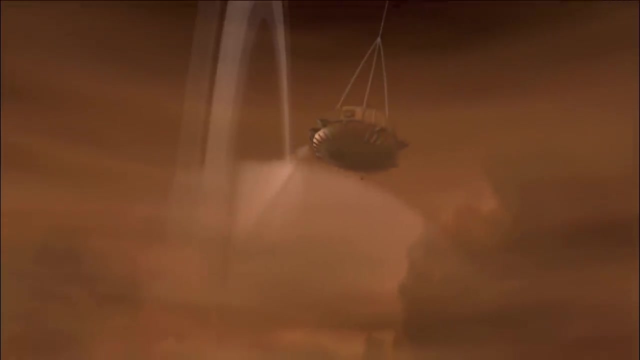 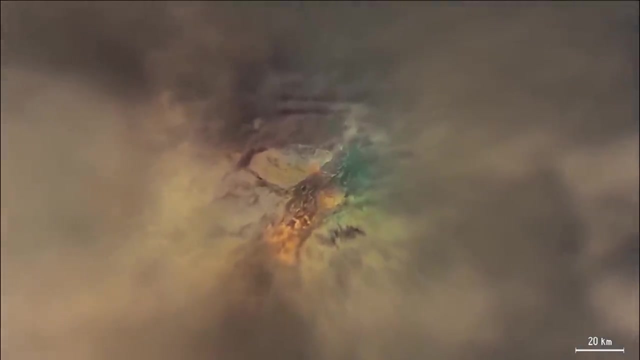 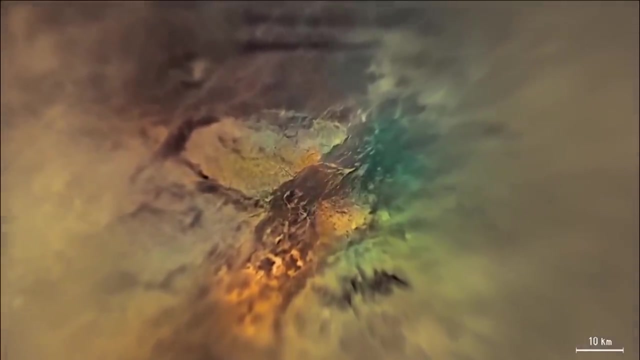 ready to receive signals from the lander. While it drifted to the surface of Titan, Huygens sampled the atmosphere and recorded images of the landscape. Pictures from beneath the clouds revealed low hills and channels cut by flowing liquid. There were few impact craters. 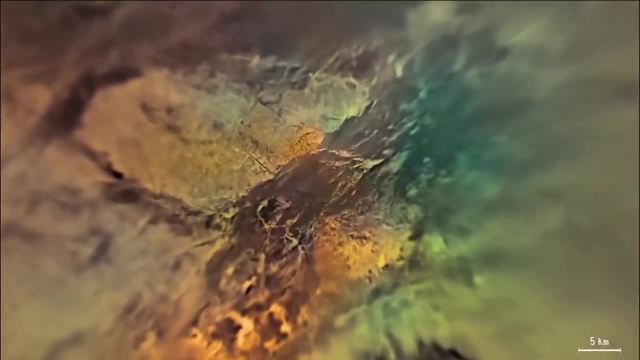 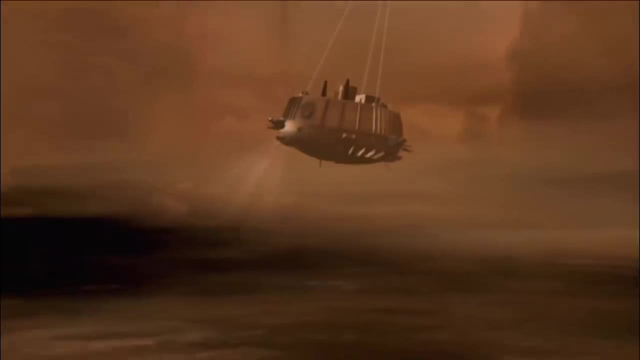 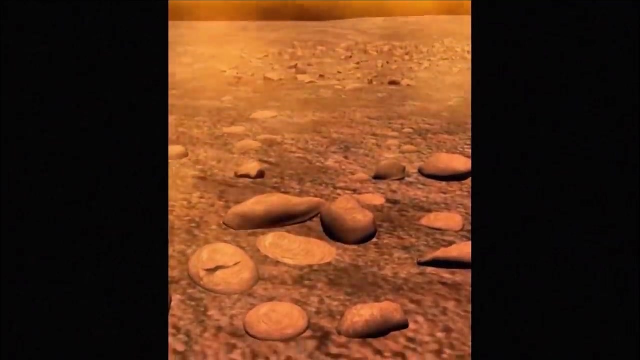 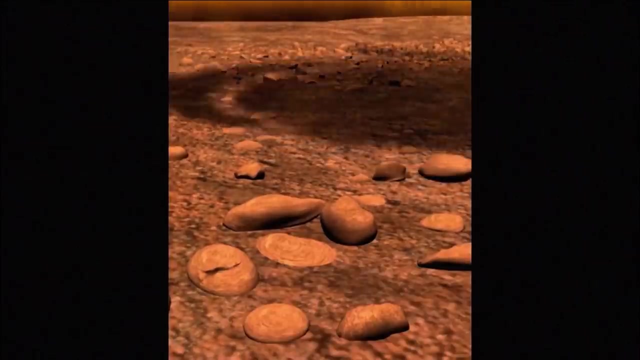 and those that existed were heavily eroded. It was the first landing on a body in the outer solar system. Images from the surface showed weathered rocks made of water ice. What surprised everybody was that Titan is a geologically active world where liquid ethane and methane rather than water. 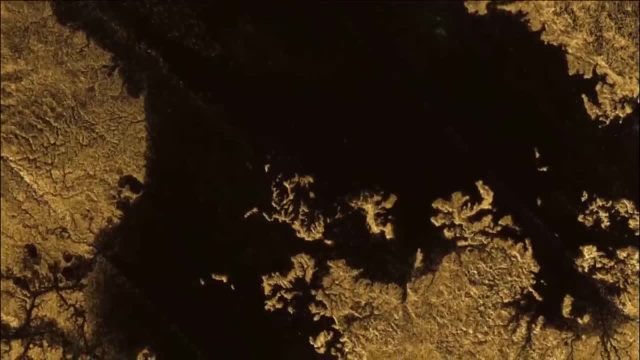 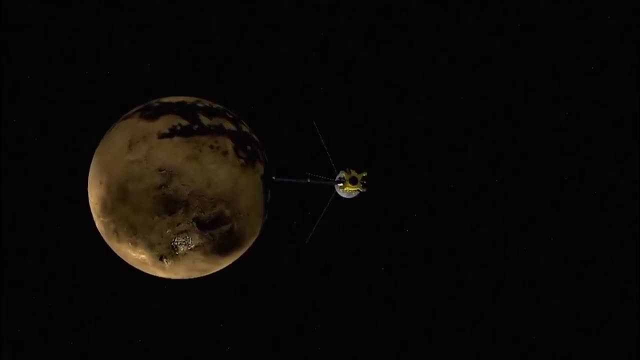 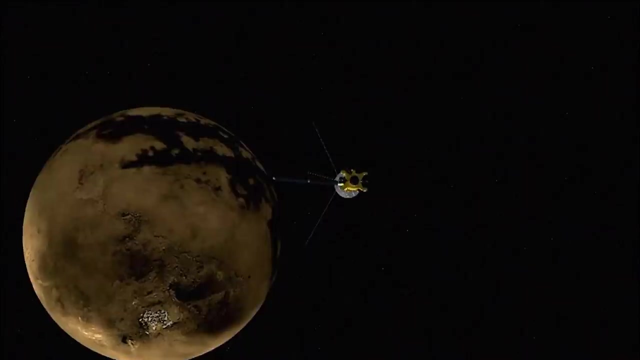 have carved the features As Cassini continued looping out around Titan. it used radar to map the moon's surface, confirming the widespread distribution of hydrocarbon lakes. The probe discovered that rain fell on Titan, but it was a mixture of liquid, ethane and methane. 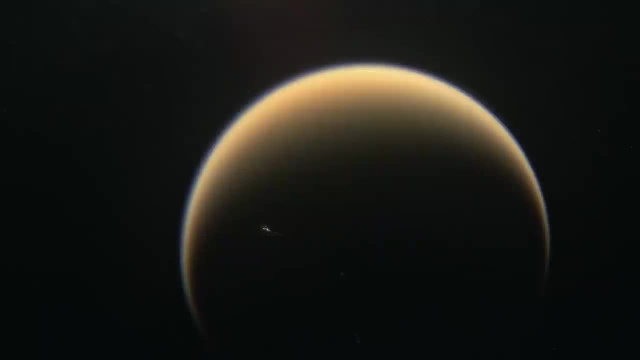 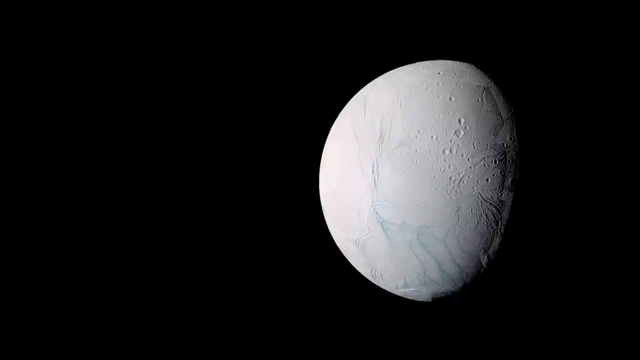 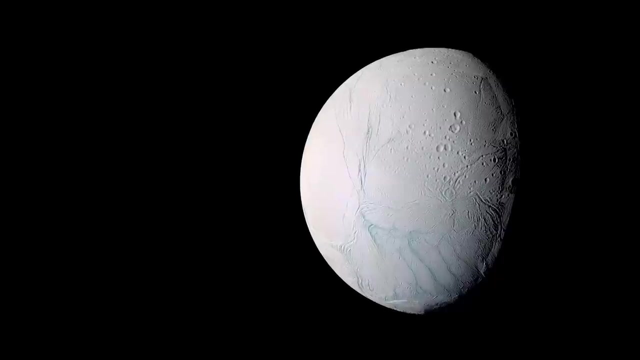 The moon has weather and other erosive forces similar to Earth, but the chemistry is radically different. The small moon Enceladus drew attention to itself as the whitest, most reflective body in the solar system. Its surface shows cratering in the north. 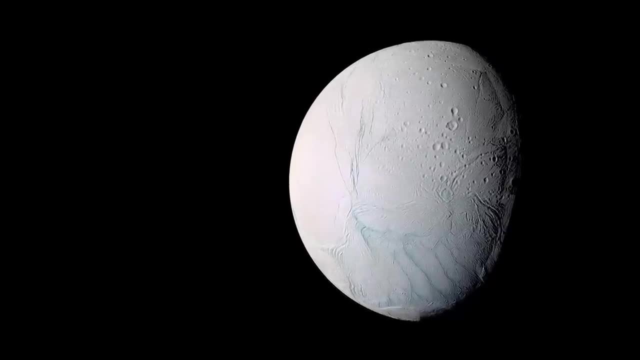 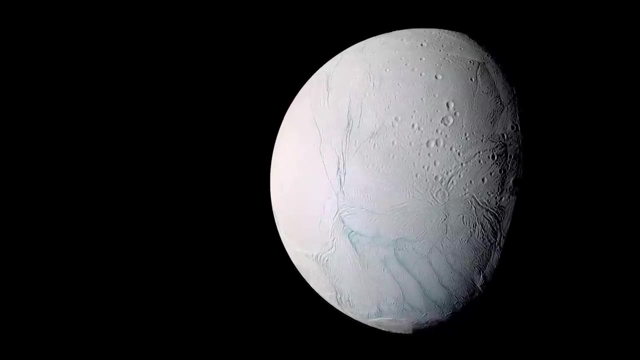 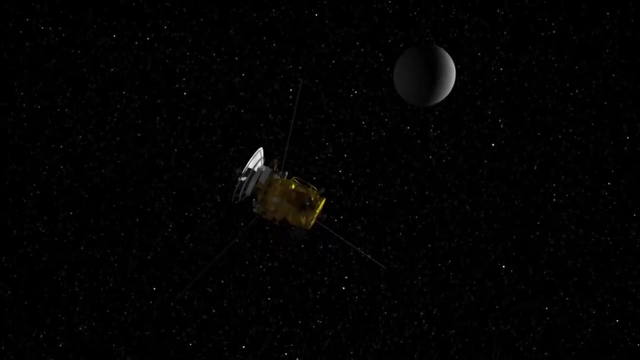 but the south has giant cracks known as tiger stripes. On Cassini's first loop past Enceladus, the magnetometer team noticed an odd deflection of Saturn's magnetic field, as though the small moon had an atmosphere. During its second pass, 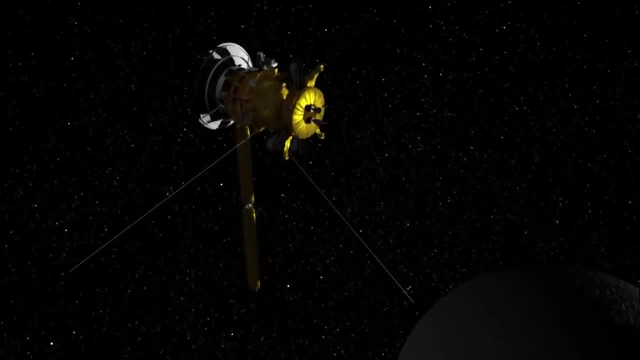 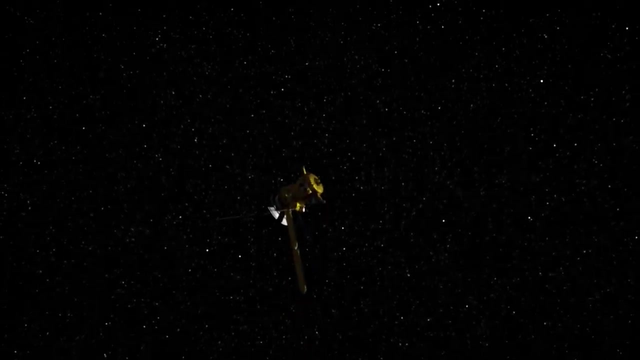 the team noticed an odd deflection of Saturn's magnetic field, as though the moon had an atmosphere. During its second pass, the team noticed the same phenomenon. They asked for the next traverse of Enceladus to pass much closer, so Cassini's course was modified. 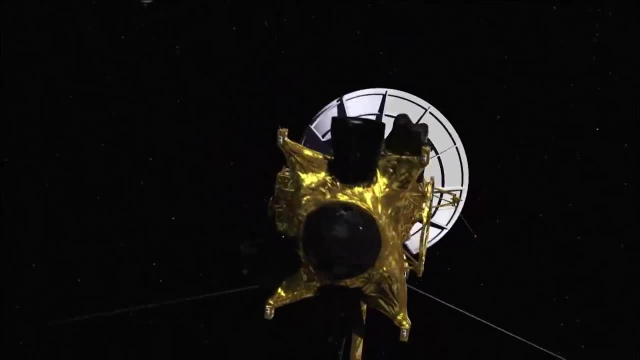 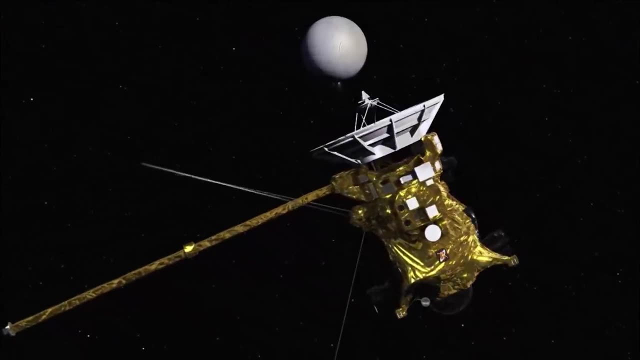 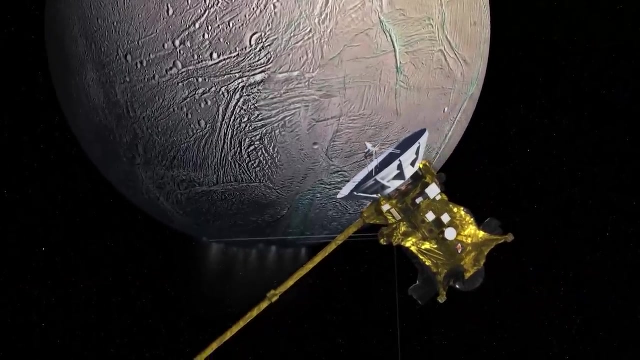 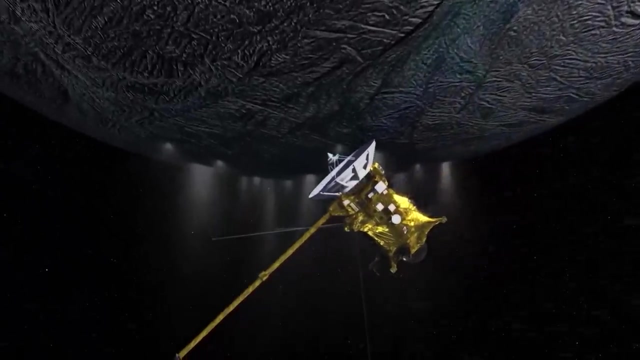 to fly just 175 kilometres above the icy moon. The probe passed through a plume of water vapour emanating from the tiger stripes. It contained common salt. In all, Cassini made 24 swoops past Enceladus, with the closest approach, flying just 25 kilometres above the surface. 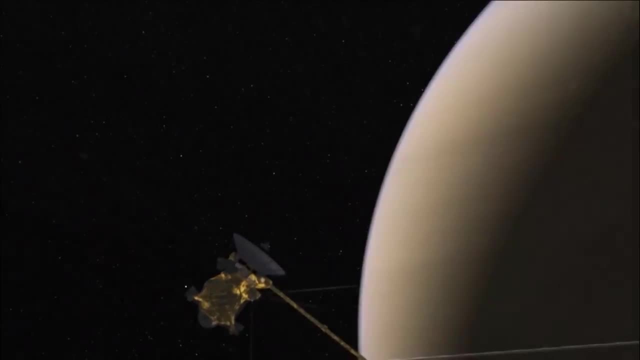 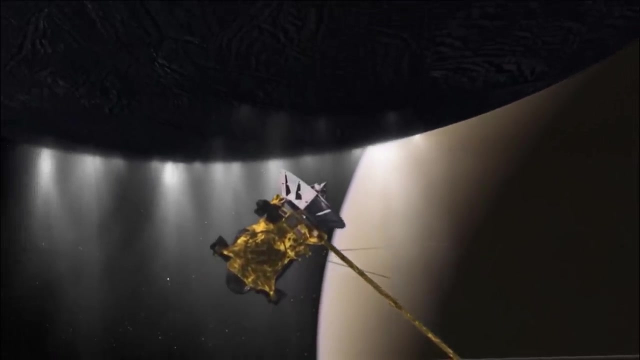 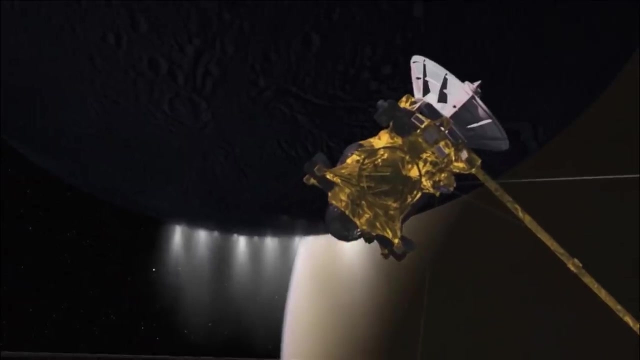 Each one of the probe's instruments gathered different evidence about the jets of water expelled through the cracks in the moon's south. On Mars, rovers have been combing the surface looking for traces of life, but Enceladus was flaunting remarkable signs. 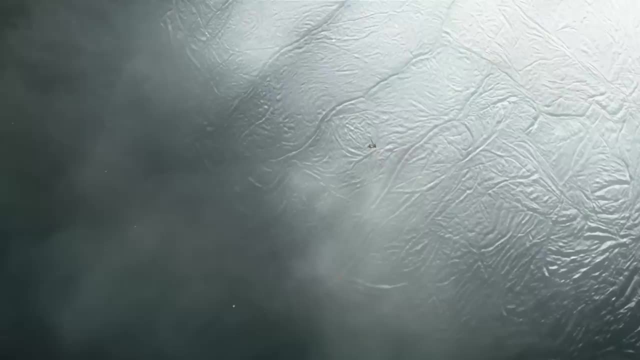 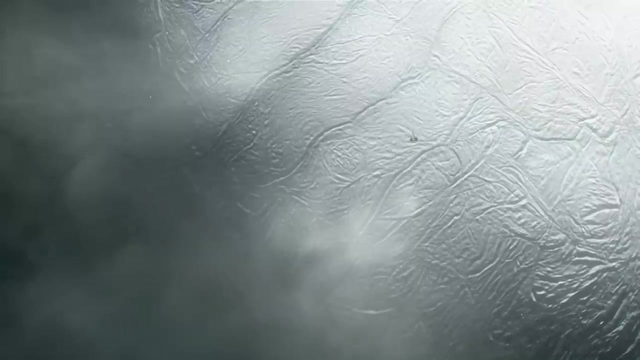 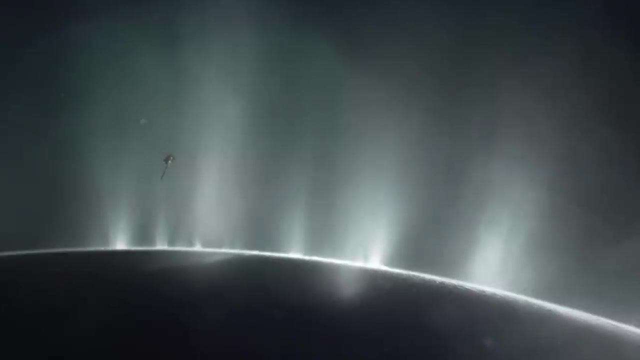 It was only a matter of time before Cassini was able to find out what was actually happening. Gravitational analysis revealed a liquid ocean beneath the ice, and infrared detectors saw heat emanating from the cracks As well as salt. the science team discovered traces of silica. 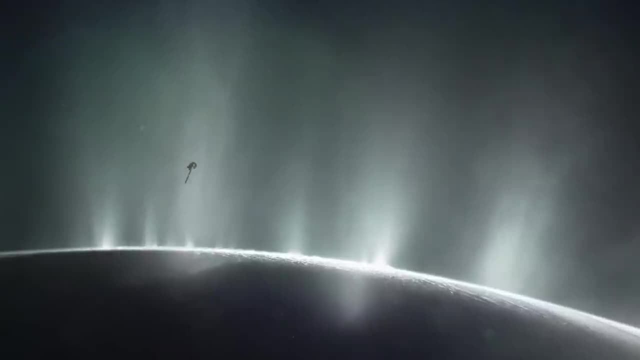 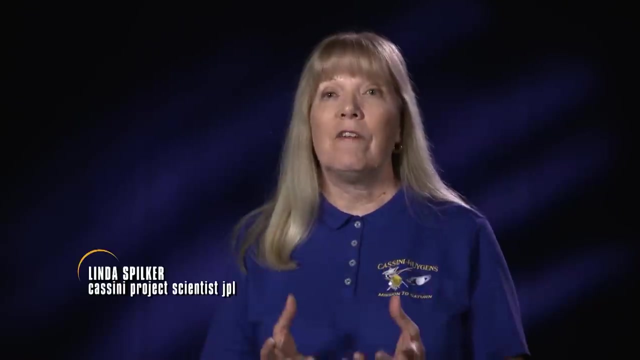 that can only dissolve in hot water. Hydrogen and organic compounds were also detected. We know from Cassini that Enceladus has a global ocean, so you have water. We also know that there are organics coming out because they've been directly measured. 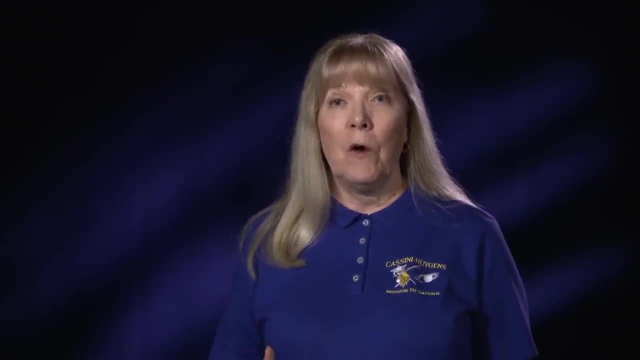 both in the gas and in the particles. We also know there's a source of energy. The South Pole was hotter than the rest of Enceladus, And then we found evidence that deep inside there are hydrothermal vents on the seafloor of Enceladus. 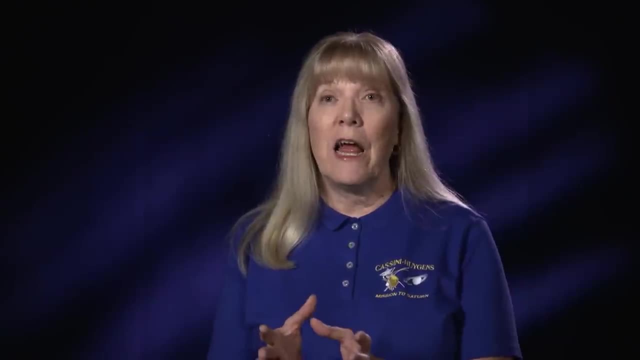 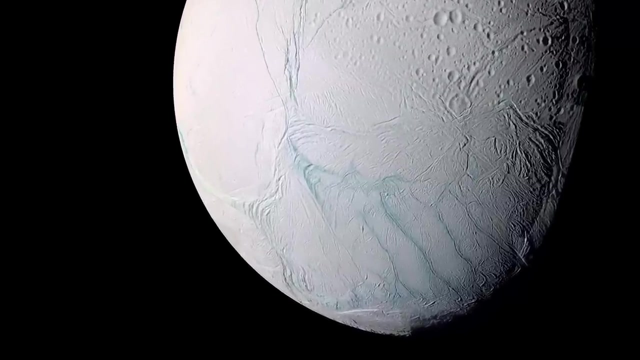 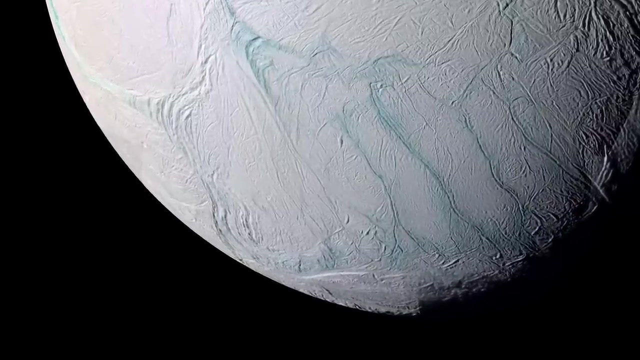 So these hydrothermal vents would supply the heat and the nutrients that could possibly support life. With a diameter of 500 kilometres, Enceladus is just too small to sustain a hot core via radioactive decay. Gravitational squeezing by Saturn explains some of the heating. 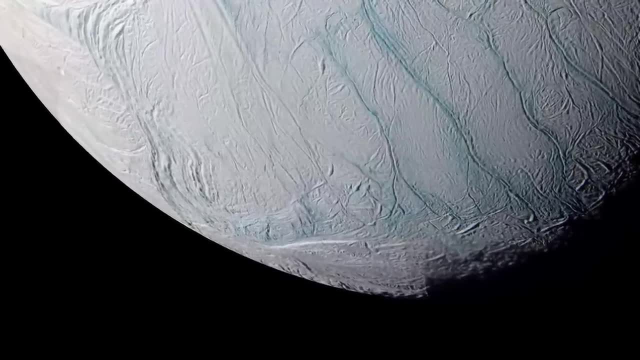 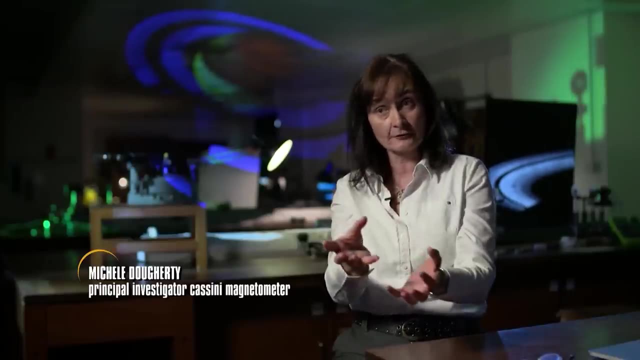 but the source of the high temperatures detected remains a mystery. But not only is there liquid water underneath the surface, but there's organic material, there's a heat source. You know when people get excited about the potential for life elsewhere in the surface. 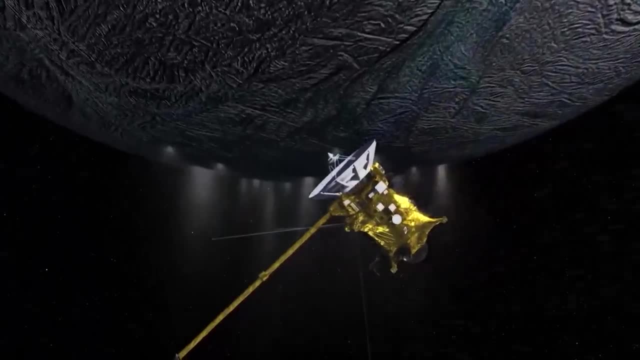 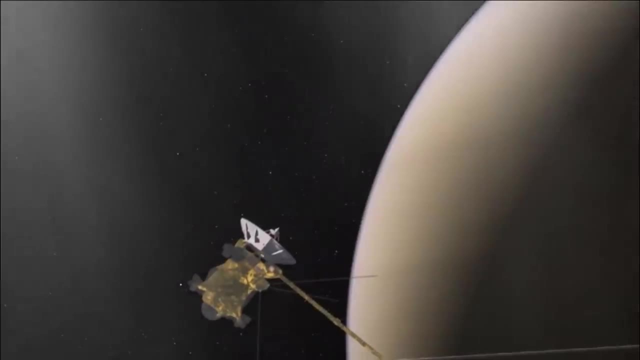 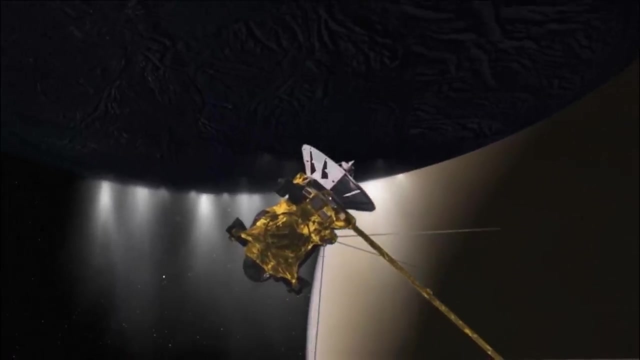 with the closest approach, flying just 25 kilometers above the surface. Each one of the probe's instruments gathered different evidence about the jets of water expelled through the cracks in the Moon's south. On Mars, rovers have been combing the surface looking for traces of life. 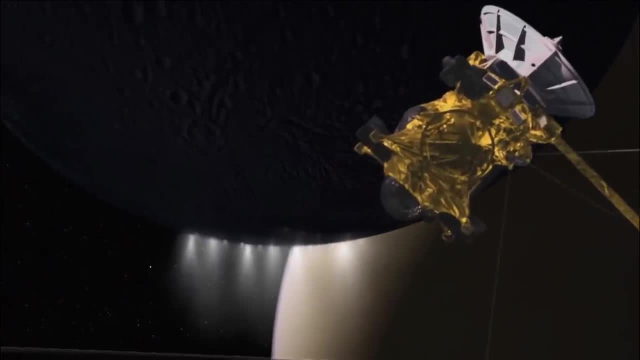 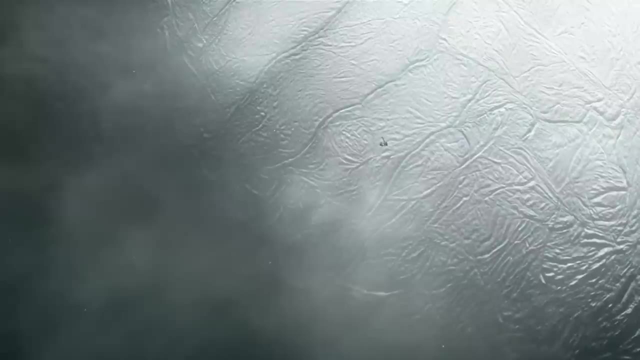 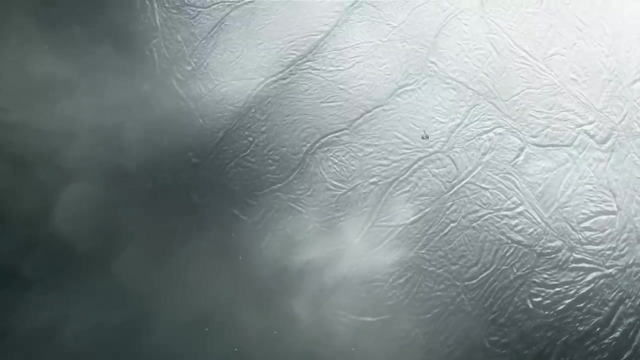 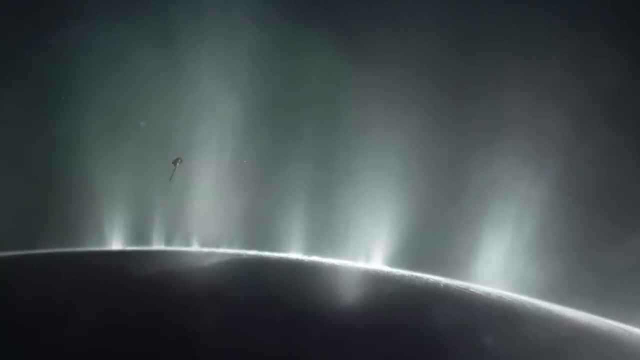 but Enceladus was flaunting remarkable signs. Gravitational analysis revealed a liquid ocean beneath the ice, and infrared detectors saw heat emanating from the cracks, As well as salt. the science team discovered traces of silica that can only dissolve in hot water. 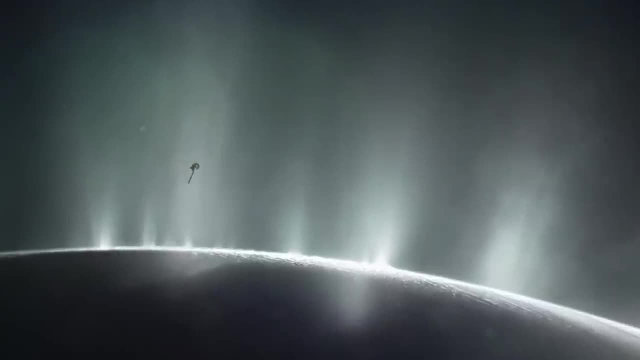 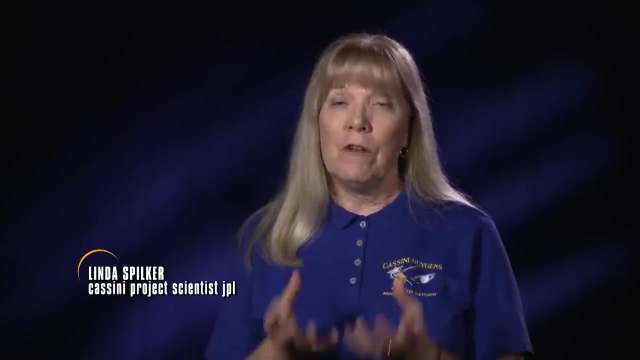 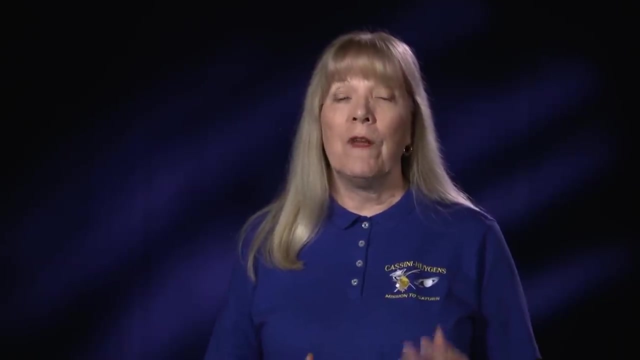 Hydrogen and organic compounds were also detected. We know from Cassini that Enceladus has a global ocean, so you have water. We also know that there are organics coming out, because they've been directly measured both in the gas and in the particles. 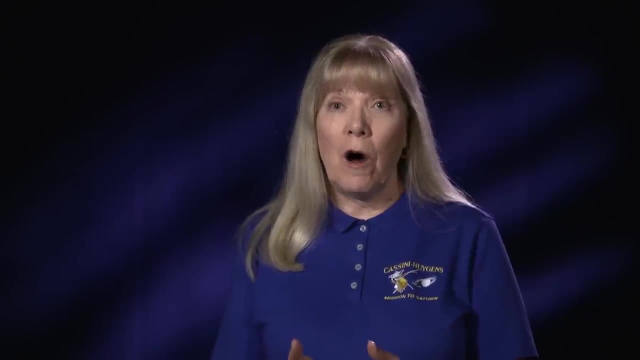 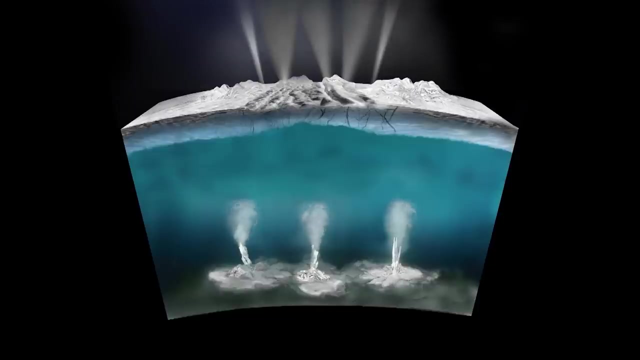 We also know there's a source of energy. The South Pole was hotter than the rest of Enceladus, And then we found evidence that deep inside there are hydrothermal vents on the seafloor of Enceladus. So these hydrothermal vents would supply the heat and the nutrients. 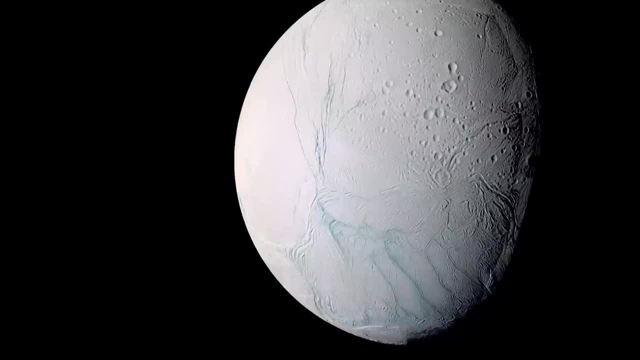 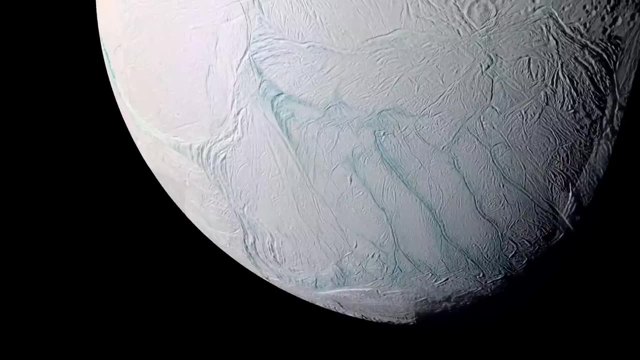 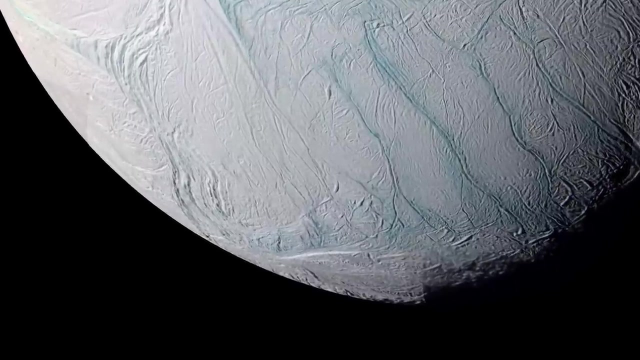 that could possibly support life. With a diameter of 500 kilometers, Enceladus is just too small to sustain a hot core of our radioactive decay. Gravitational squeezing by Saturn explains some of the heating, but the source of the high temperatures detected remains a mystery. 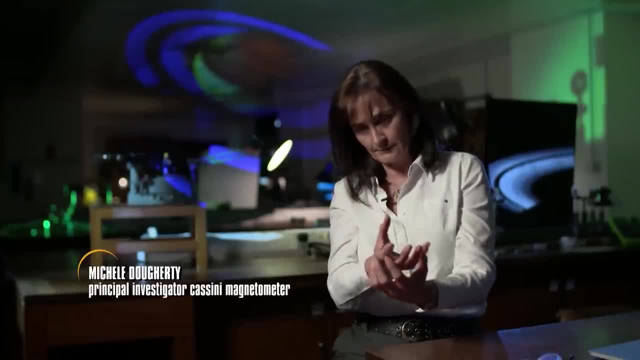 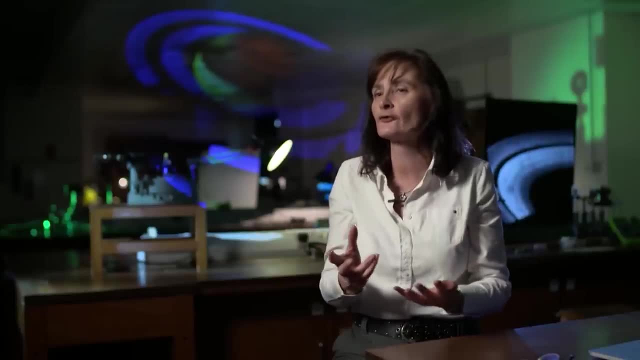 But not only is there liquid water underneath the surface, but there's organic material, there's a heat source. You know when people get excited about the potential for life elsewhere in the solar system. there are four things that you need. You need a heat source, you need liquid water. 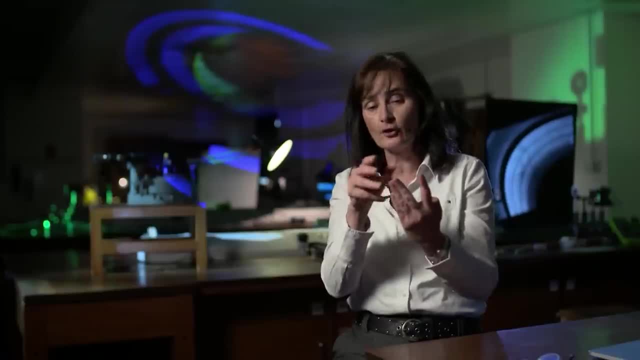 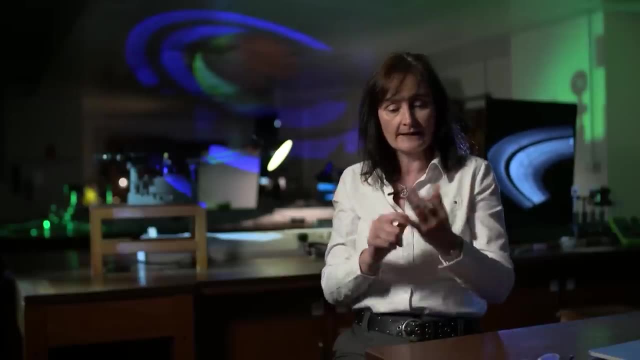 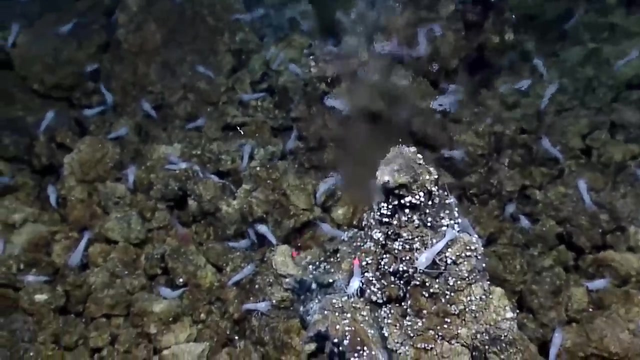 you need organic material and you need those three things to be stable over some period of time so that life could potentially form Enceladus. we've got three. We're not sure about the stability over time yet. In the Earth's deep oceans, hydrothermal vents provide the warmth. 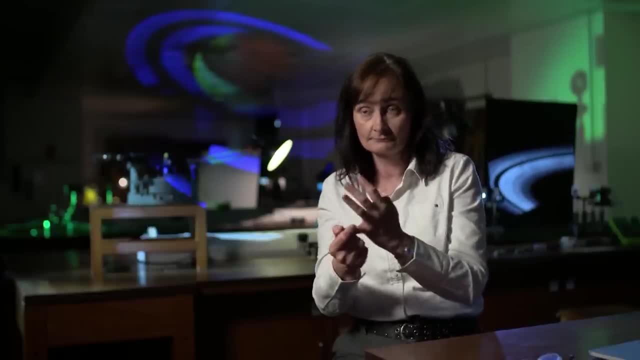 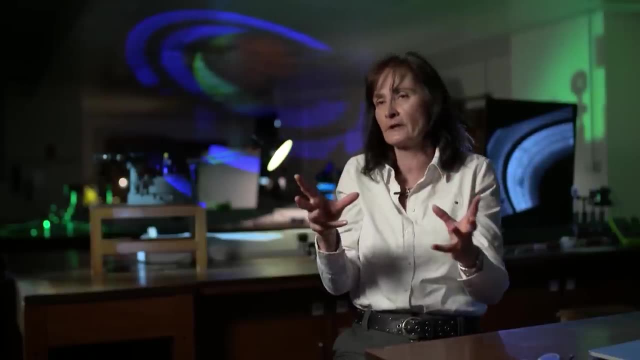 in the solar system. there are four things that you need. You need a heat source, you need liquid water, you need organic material and you need those three things to be stable over some period of time so that life could potentially form At Enceladus. we've got three. 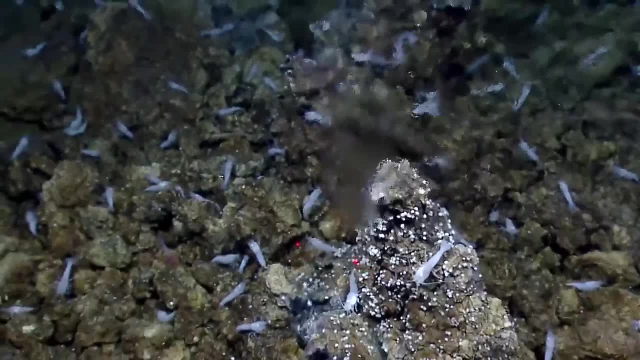 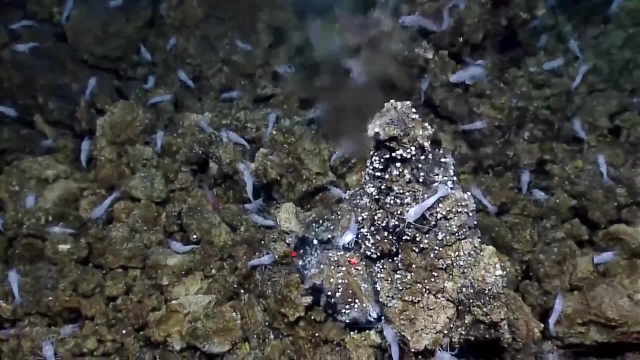 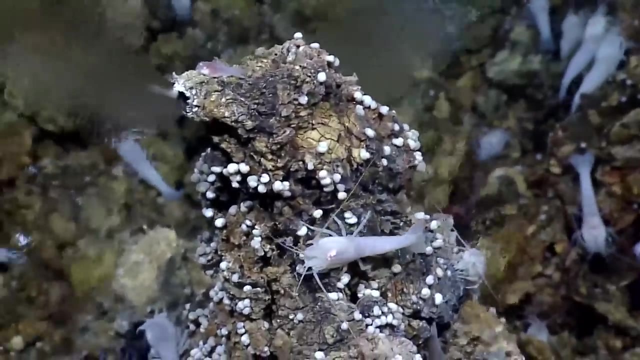 We're not sure about the stability over time. yet In the Earth's deep oceans, hydrothermal vents provide the warmth and nutrition to support life. They may even have been important for the origins of life. Planetary biologists are speculating that the environment in the oceans of Enceladus 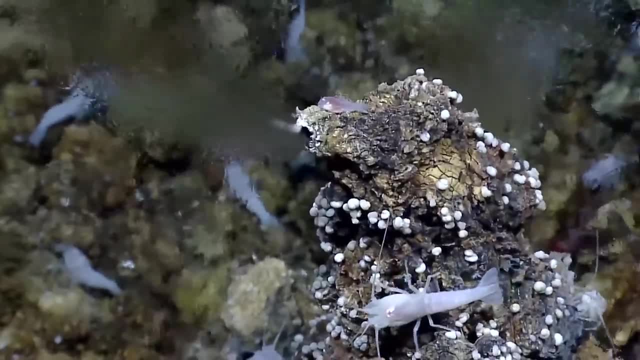 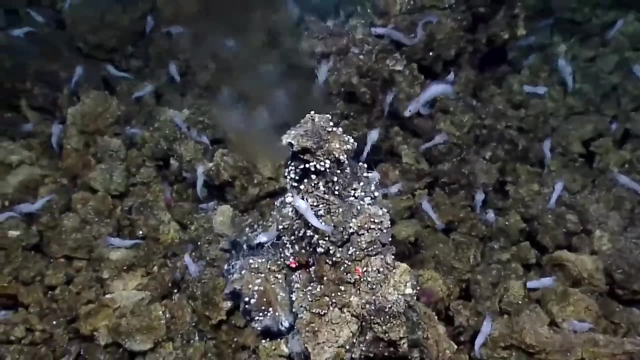 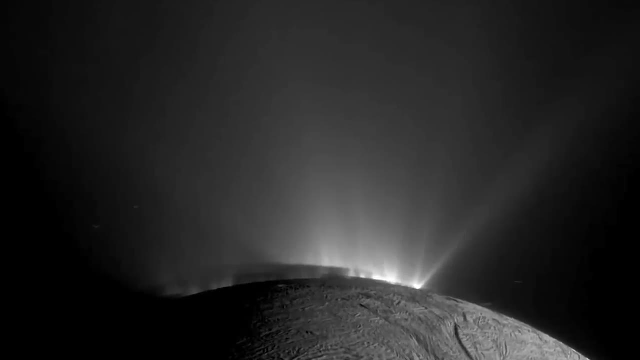 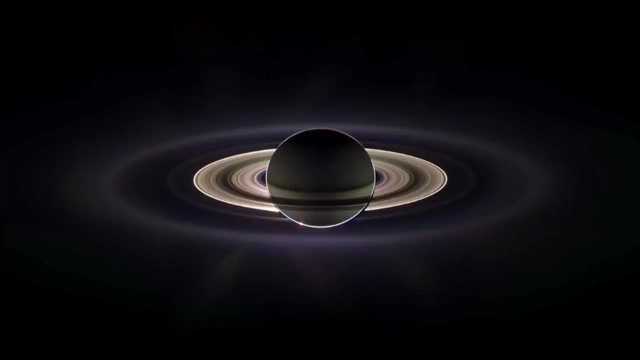 may be the most likely place in the solar system to find some sort of extraterrestrial life. It took a while for Cassini to be in a position where backlighting from the sun allowed the imaging team to capture pictures of the plumes Using a similar technique. 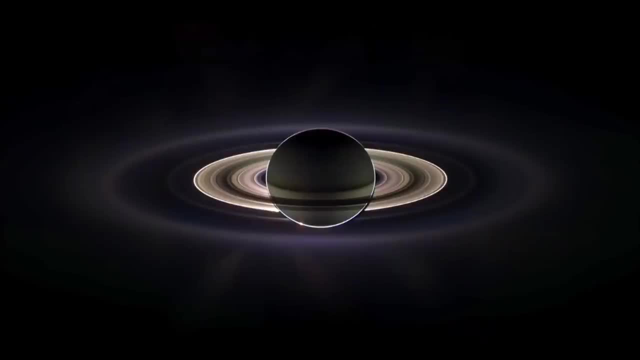 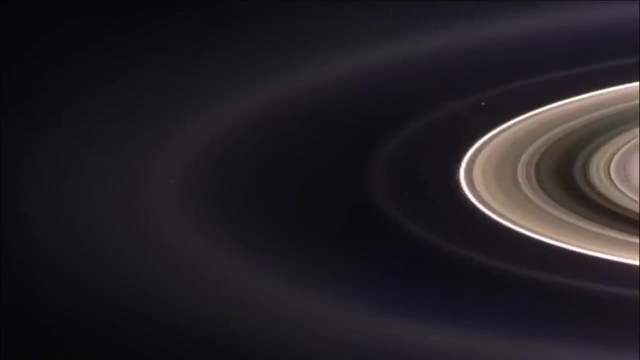 the imaging team took this picture with Saturn directly between Cassini and the sun. It reveals Saturn's E ring, the hazy outermost ring that is usually very difficult to see. The E ring is a result of the plumes from Enceladus. 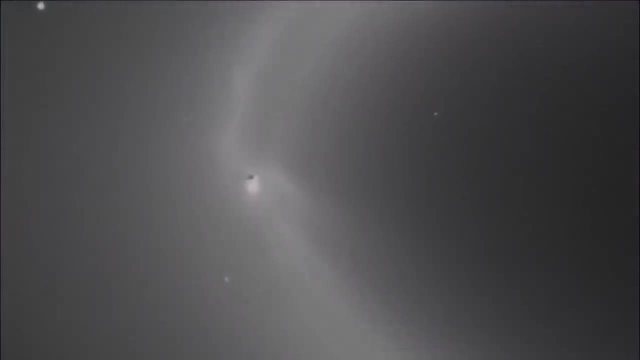 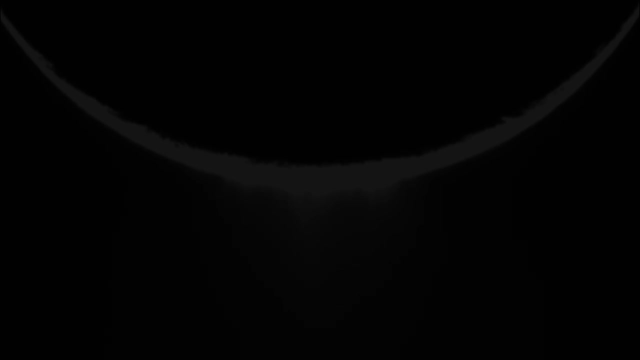 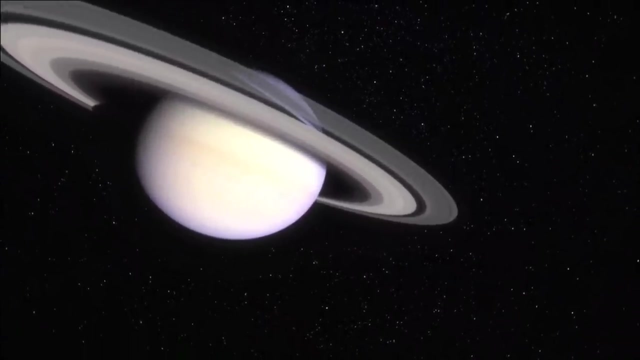 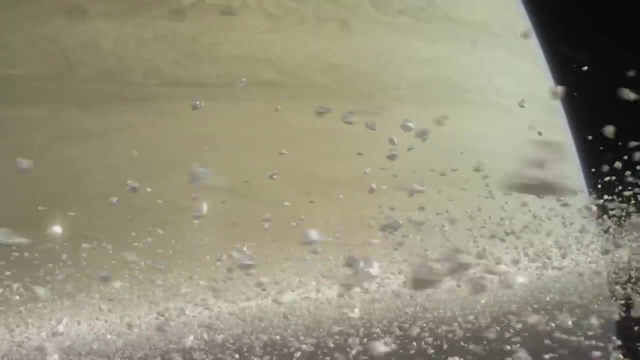 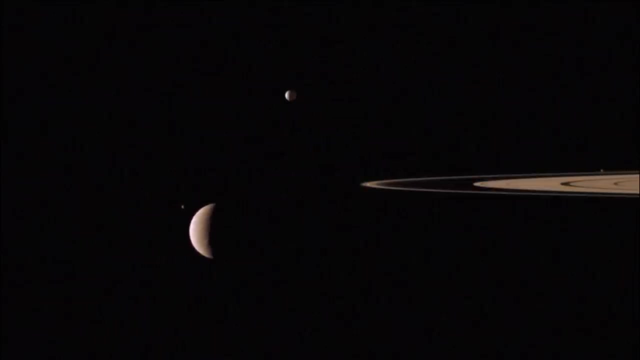 and is constantly replenished by the saltwater eruptions. This is how Saturn looks like in the sun. Saying that Saturn has 62 moons is misleading. Each particle within the ring system could be regarded as a moon. There are the inner large moons and the outer large moons. 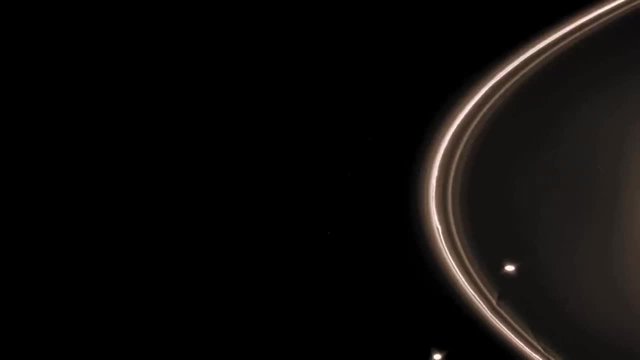 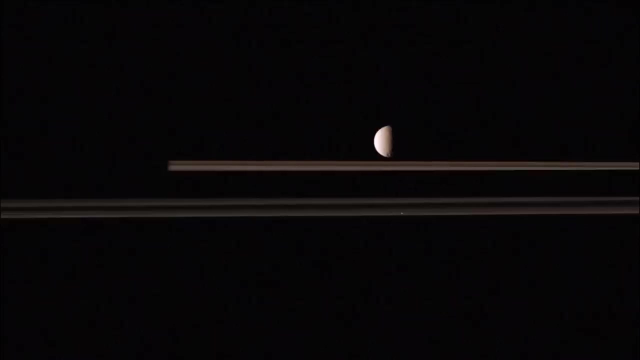 There are the shepherds that shape the rings, There are co-orbitals that exchange orbits And there are even moons that orbit other moons. moons- All are unique. During the Voyager missions, interest in the moons came as something of an afterthought. 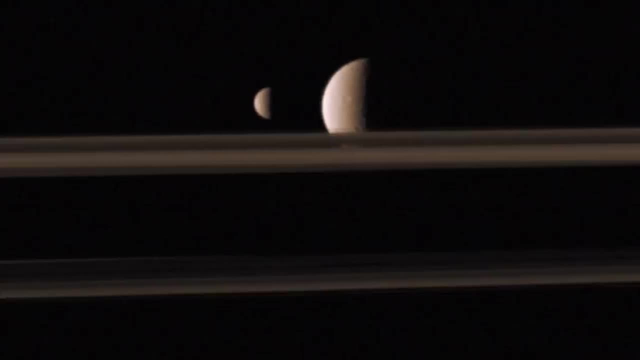 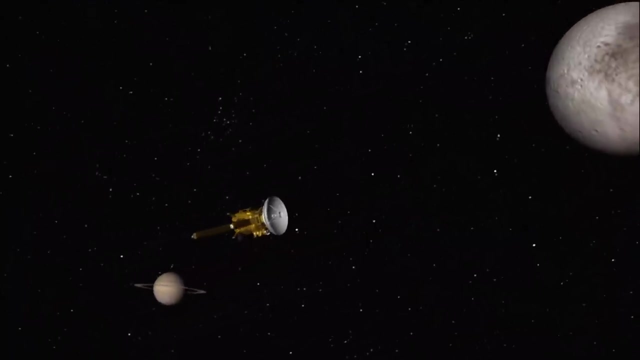 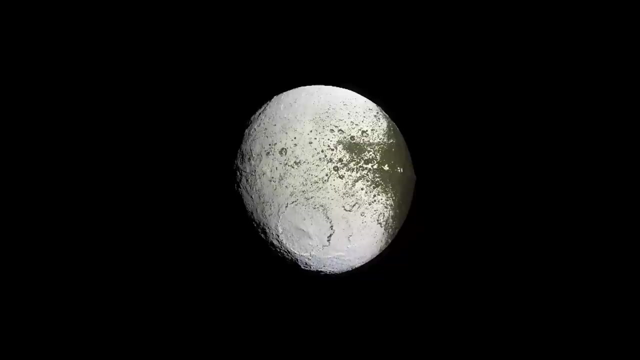 But for Cassini close examination of the moons was planned from the beginning. Iapetus orbits Saturn beyond Titan. It was first observed in 1671 by Giovanni Cassini. He could see it as a dot of light to the west of Saturn but could not see it when it should. 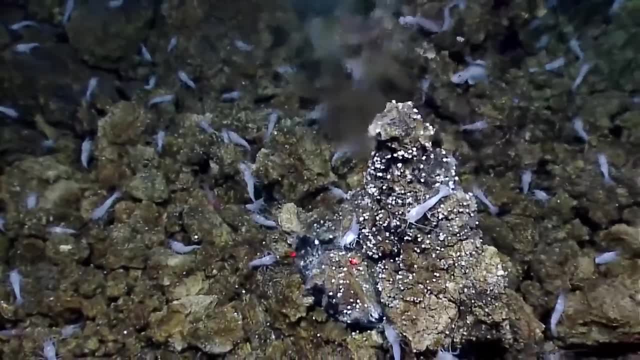 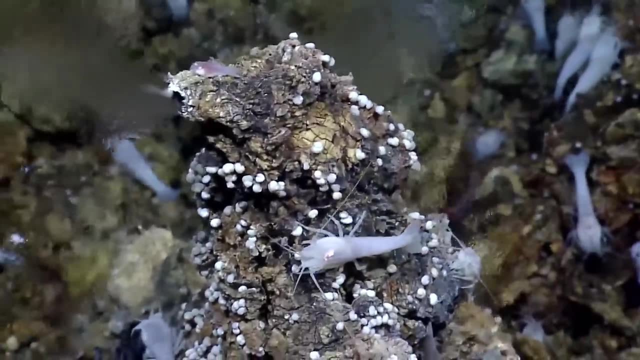 and nutrition to support life. They may even have been important for the origins of life. Planetary biologists are speculating that the environment in the oceans of Enceladus may be the most likely place in the solar system to find some sort of extraterrestrial life. 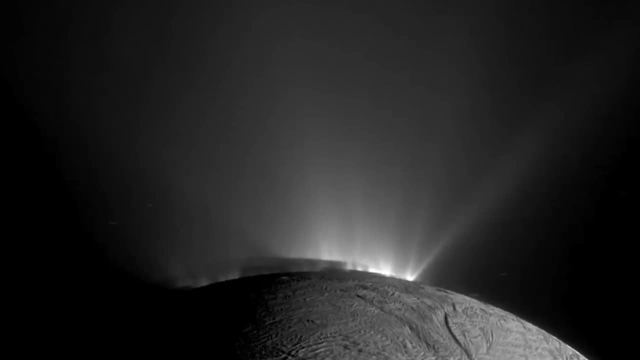 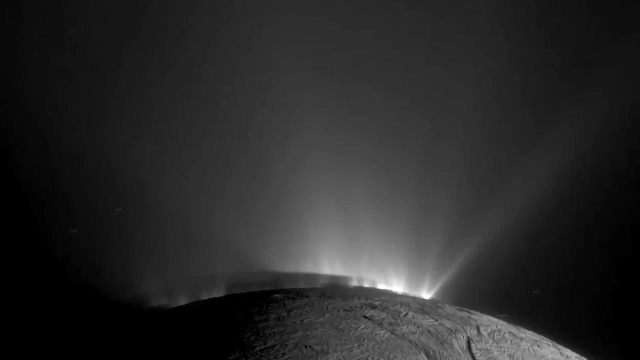 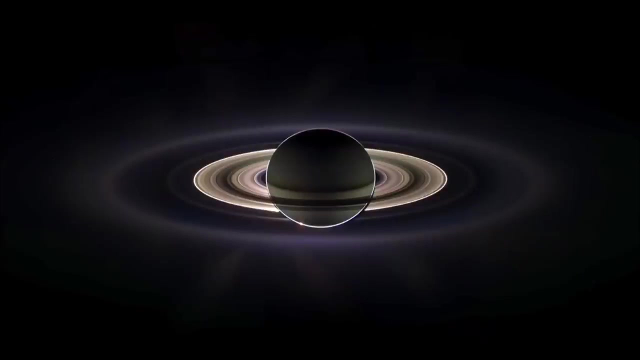 It took a while for Cassini to be in a position where backlighting from the Sun allowed the imaging team to capture pictures of the plumes. Using a similar technique, the imaging team took this picture with Saturn directly between Cassini and the Sun. 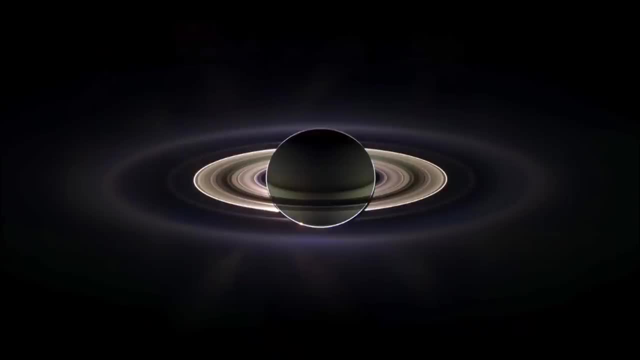 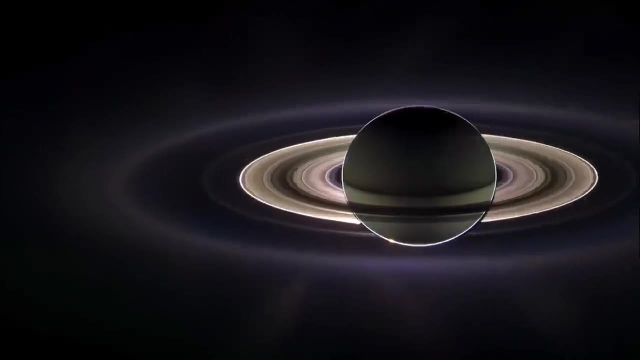 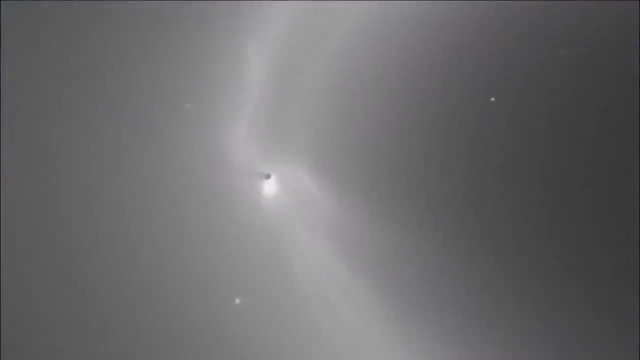 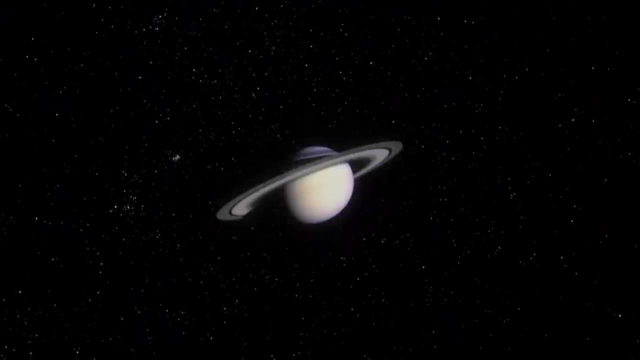 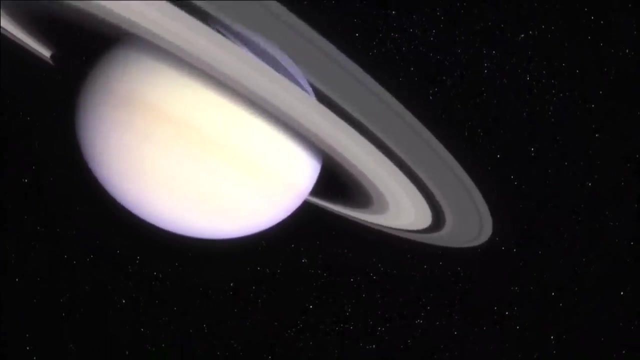 It reveals Saturn's E-ring, the hazy outermost ring that is usually very difficult to see. The E-ring is a result of the plumes from Enceladus and is constantly replenished by the saltwater eruptions. Saying that Saturn has 62 moons is misleading. 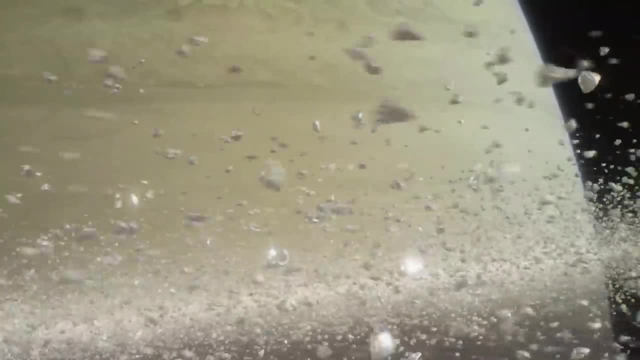 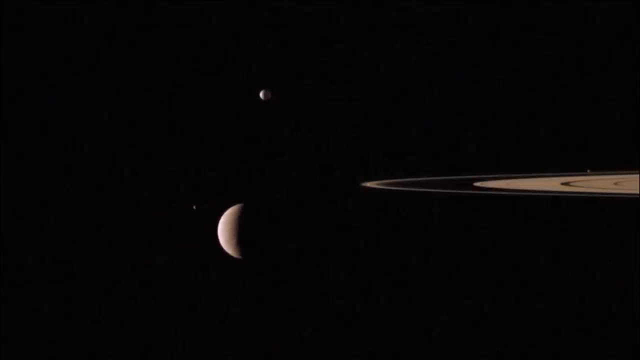 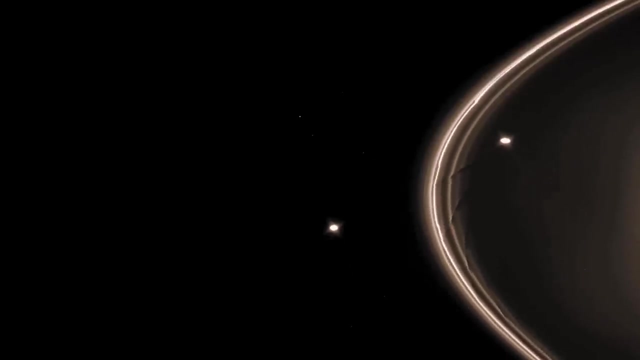 Each particle within the ring system could be regarded as a moon. There are the inner large moons and the outer large moons. There are the shepherds that shape the rings, There are co-orbitals that exchange orbits And there are even moons that orbit other moons. 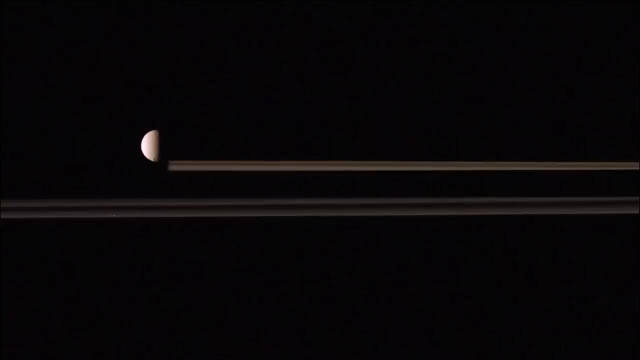 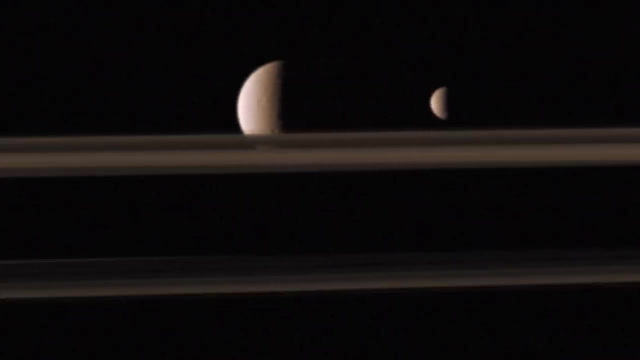 All are unique. During the Voyager missions, interest in the moons came as something of an afterthought, But for Cassini, close examination of the moons was planned from the beginning. Iapetus orbits Saturn beyond Titan. It was first observed in 1671 by Giovanni Cassini. 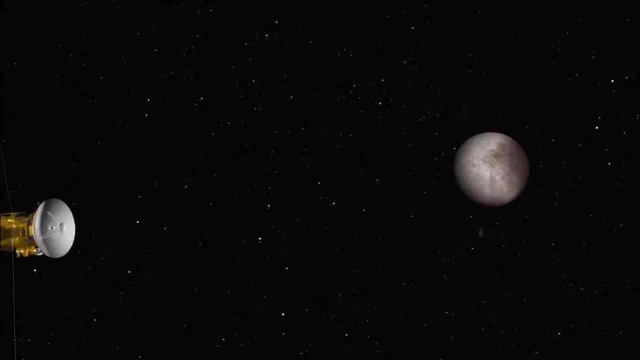 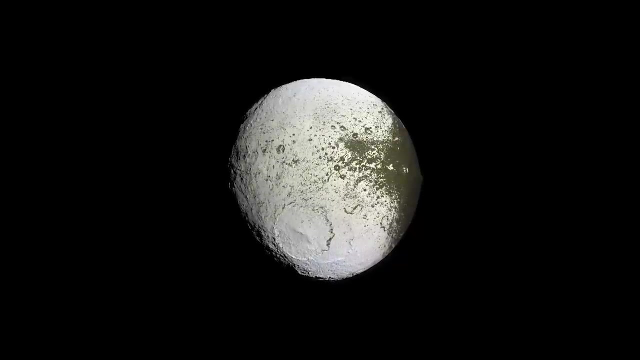 He could see it as a dot of light to the west of Saturn, but could not see it when it should have been to the east. Iapetus has one bright face and one dark one Because the moon is tidally locked to Saturn. 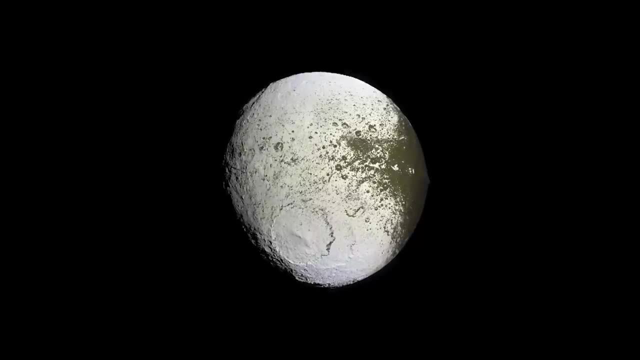 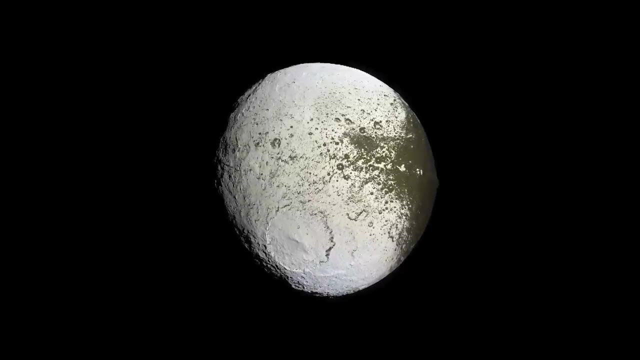 it is always the dark face that leads as it orbits. One theory suggests that it sweeps up debris that spews from Phoebe, a more distant moon. Another feature of Iapetus has scientists baffled. The moon is not the only moon in the world. 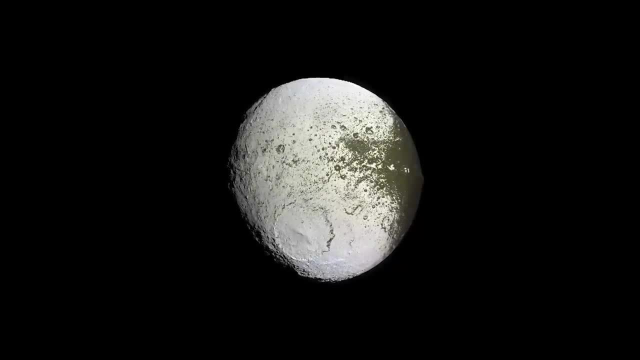 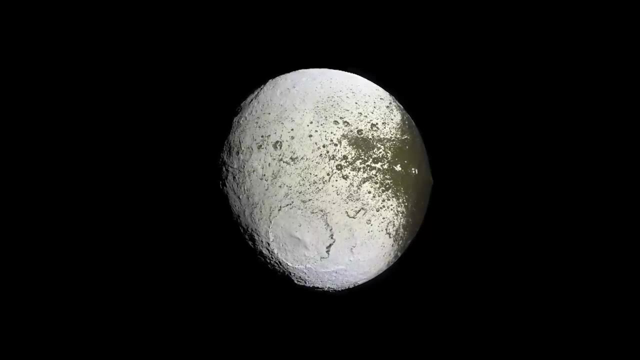 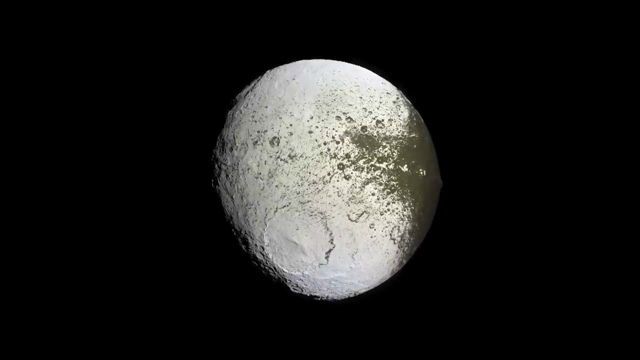 have been to the east. Iapetus has one bright face and one dark one. Because the moon is tidally locked to Saturn, it is always the dark face that leads as it orbits. One theory suggests that it sweeps up debris that spews from Phoebe, a more distant 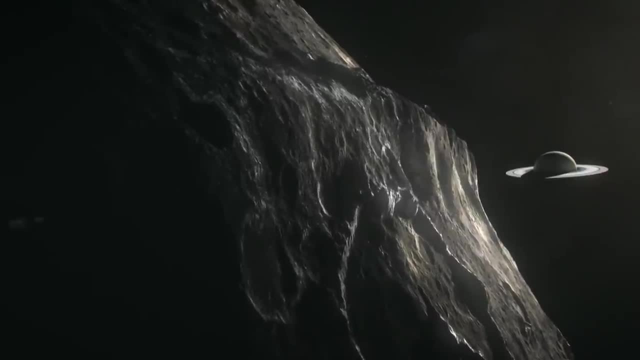 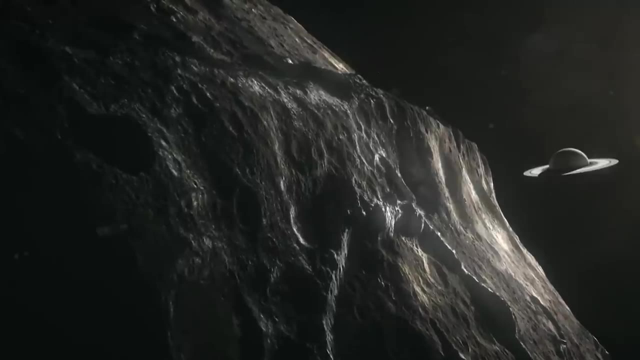 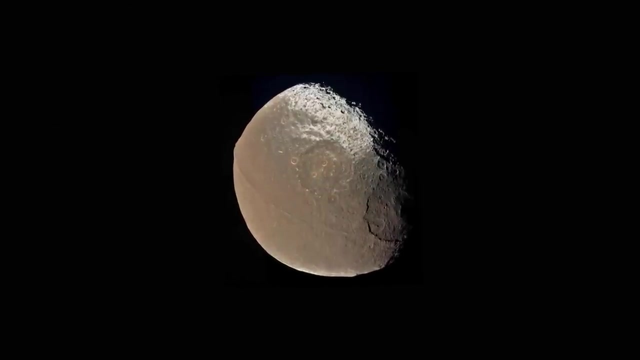 moon. Another feature of Iapetus has scientists baffled A ridge along the equator stretches more than halfway around the moon. It's twice as high as Earth's tallest mountain, With Iapetus being just 1500 kilometres across. the ridge gives Iapetus the appearance of 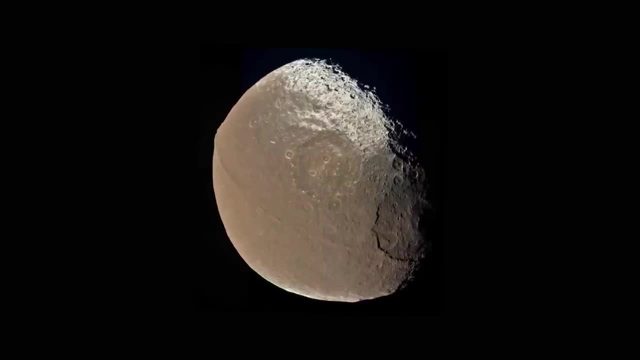 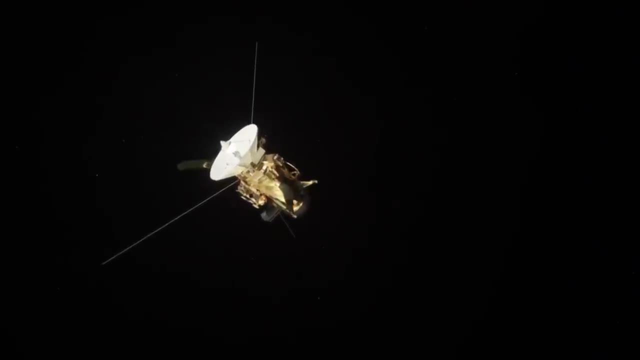 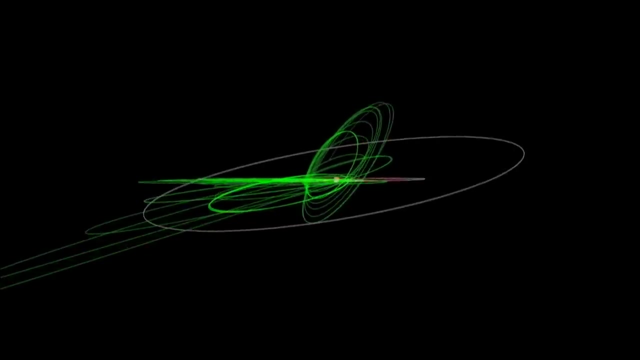 a walnut. Very accurately directed bursts from Cassini's main engine allowed mission engineers to see if the moon was moving at all, and if it was moving at all. and if it was moving at all, Iapetus had the ability to modify the probe's looping orbits, so mission specialists could. 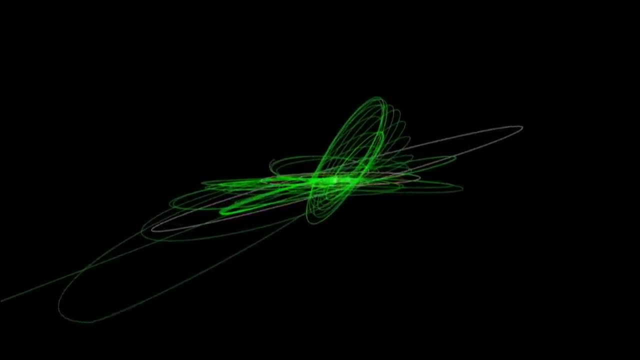 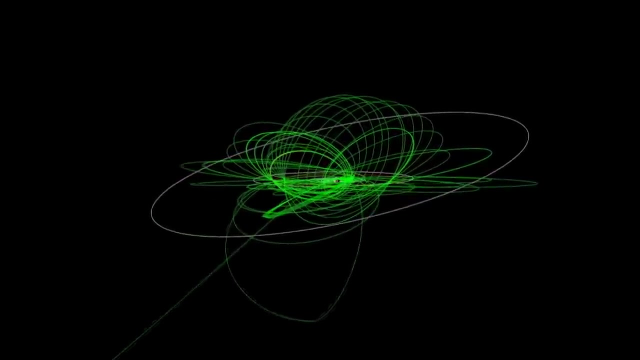 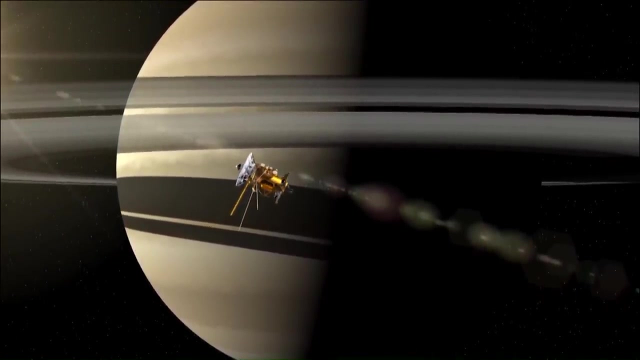 focus on various moons, different areas of the ring system or different parts of Saturn itself. With gravitational assistance from the moons, particularly Titan mission control were able to conserve fuel. The Cassini probe performed so well. it received two mission extensions, but the fuel could. 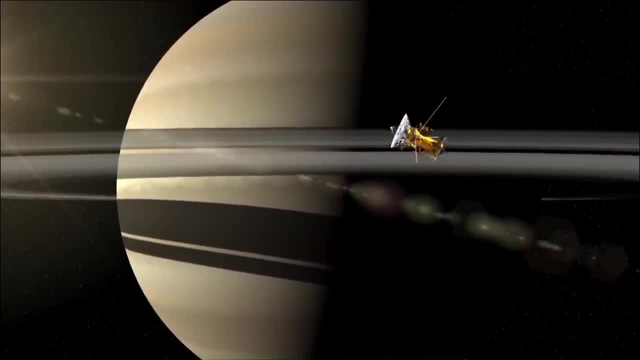 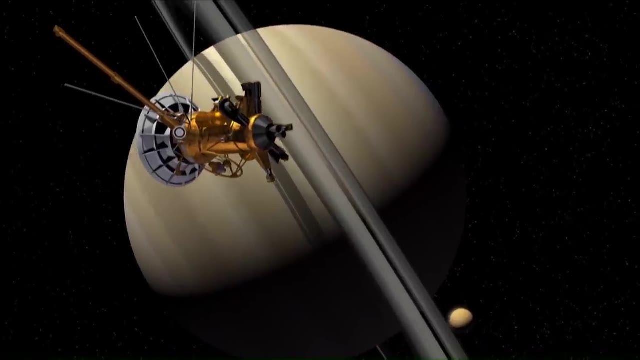 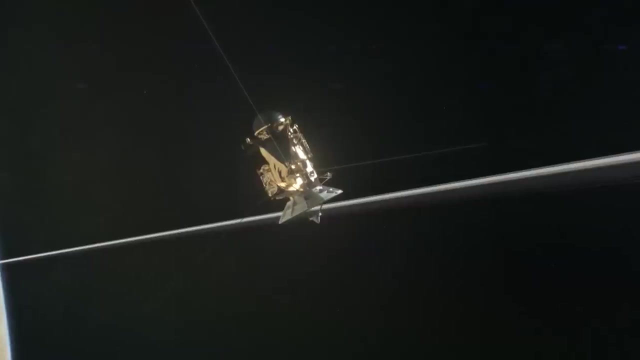 not last forever. Iapetus was the last part of Cassini's mission for its final year at Saturn Late in 2016,, Cassini began a series of polar orbits that would take it close to the outer edge of the rings In what mission specialists called grazing on the rings. the craft's mass spectrometer. 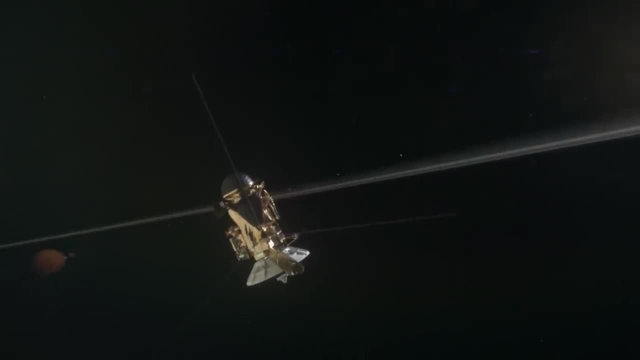 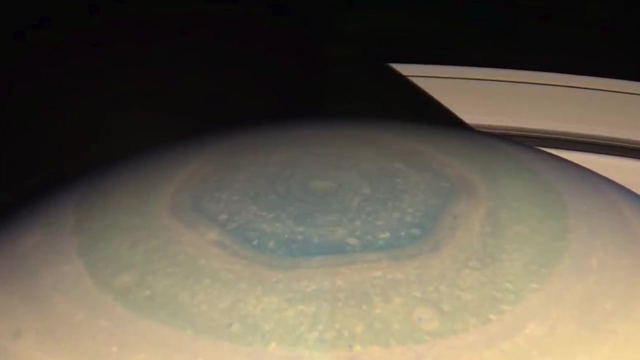 and its cosmic dust analyser would sample particles and gases as it crossed the ring plane In orbit 251, its first pass above Saturn's north pole. Iapetus was the first to reach the ring plane. The mass spectrometer was used to track the Earth's orbit and it was able to almost 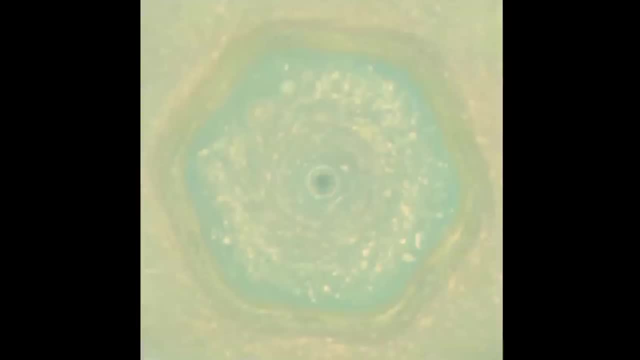 fully detect the current movement. The first time it was ever recorded it was in the North Pole. It recorded the peculiar hexagonal storm that was first hinted at by the Voyagers. The storm, more than twice the diameter of Earth, maintains its hexagonal shape, but its colour changed with the advance of summer. At its centre is a cyclone, shown here in false colour, with red indicating lower cloud and green higher cloud. Winds at its edge blow at 540 km per hour. The wind is blowing at 540 km per hour. 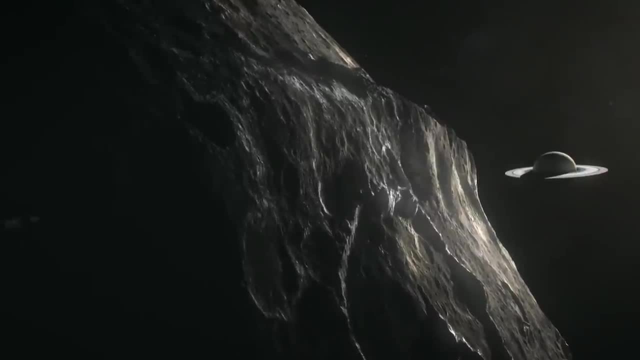 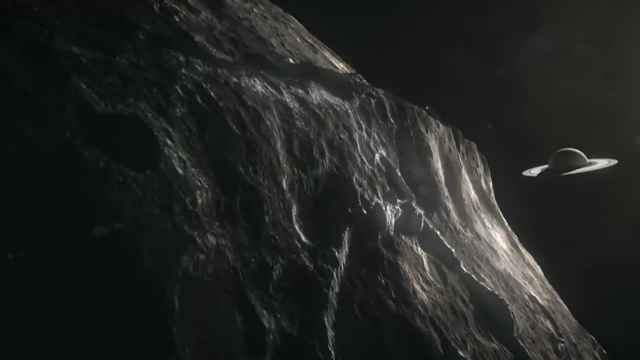 It is the only moon in the world. It is the only moon in the world. It is the only moon in the world. A ridge along the equator stretches more than halfway around the moon. It's twice as high as Earth's tallest mountain. 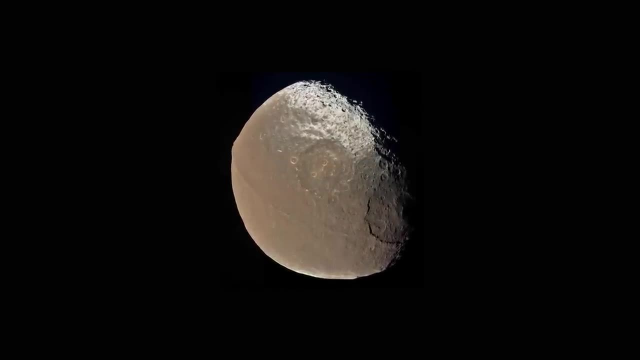 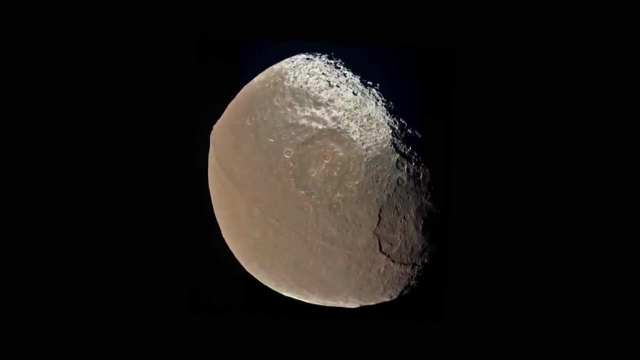 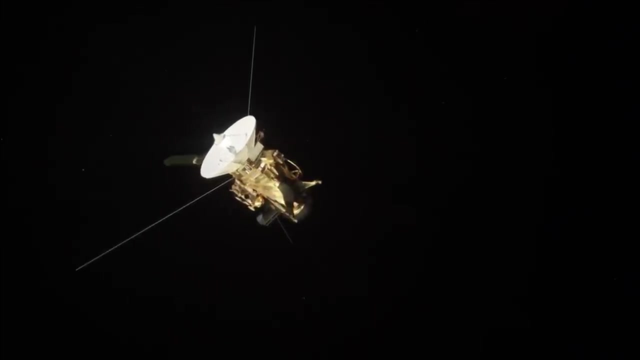 With Iapetus being just 1,500 kilometres across. the ridge gives Iapetus the appearance of a walnut. Very accurately directed bursts from Cassini's main engine allowed mission engineers to modify the probe's looping orbits, so mission specialists could focus on various moons. 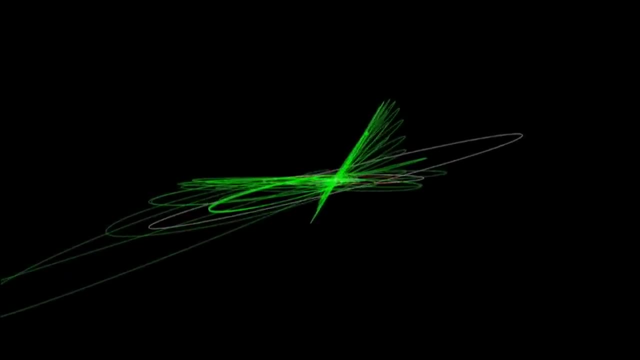 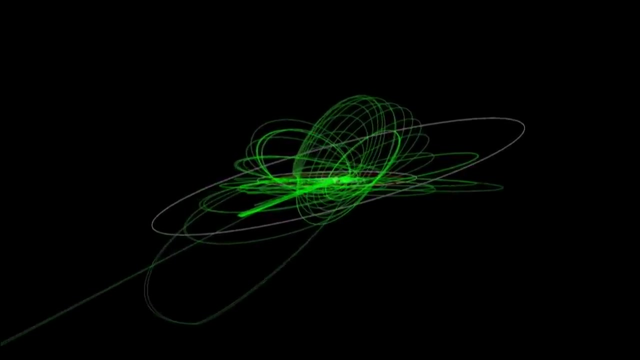 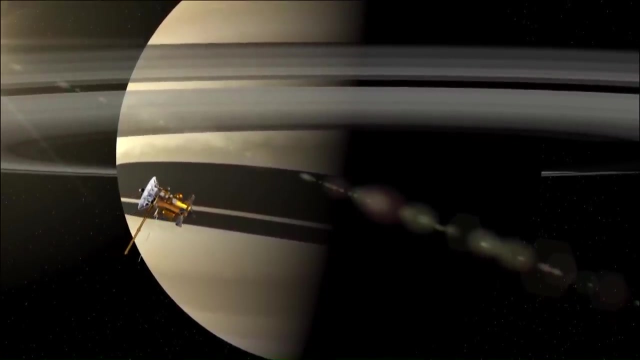 different areas of the ring system or different parts of Saturn itself, With gravitational assistance from the moons, particularly Titan mission control, were able to conserve fuel. The Cassini probe performed so well. it received two mission extensions, But the fuel could not last forever. 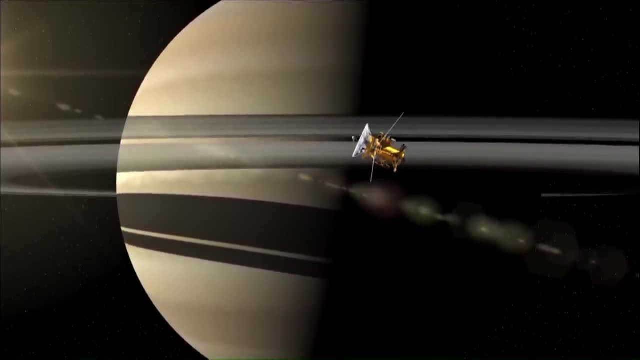 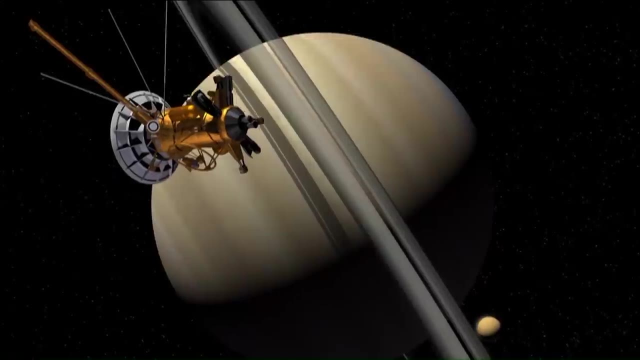 Planners had scheduled the most hazardous part of Cassini's mission for its final year of operation. It was its last year at Saturn Late in 2016,, Cassini began a series of polar orbits that would take it close to the outer edge of the rings. 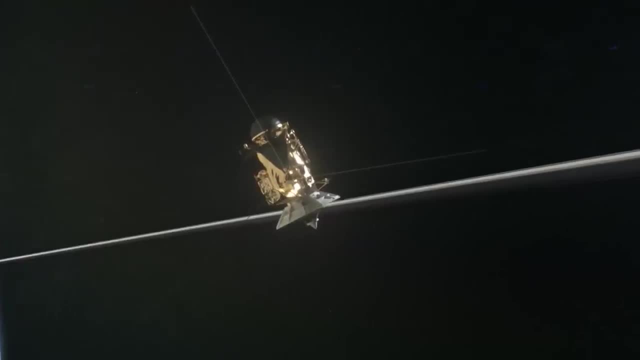 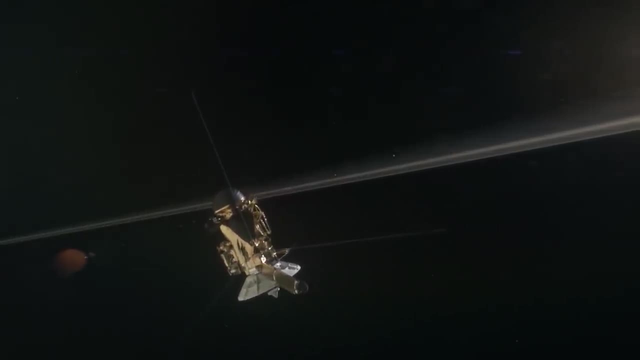 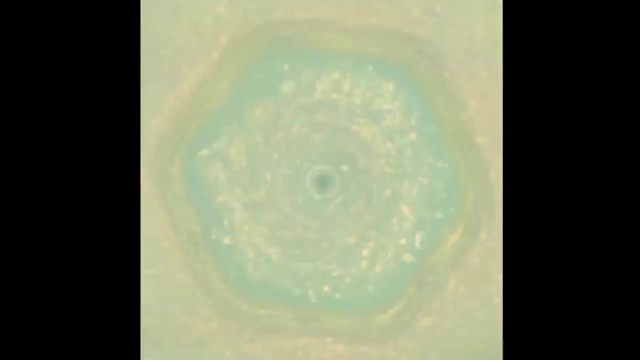 In what mission specialists called grazing on the rings. the craft's mass spectrometer and its cosmic dust analyser would sample particles and gases. as it crossed the ring plane In orbit 251, its first pass above Saturn's north pole, it recorded the peculiar hexagonal storm. that was first hinted at by the Voyagers. The storm, more than twice the diameter of Earth, maintains its hexagonal shape, but its colour changed with the advance of summer. At its centre is a cyclone, shown here in false colour. 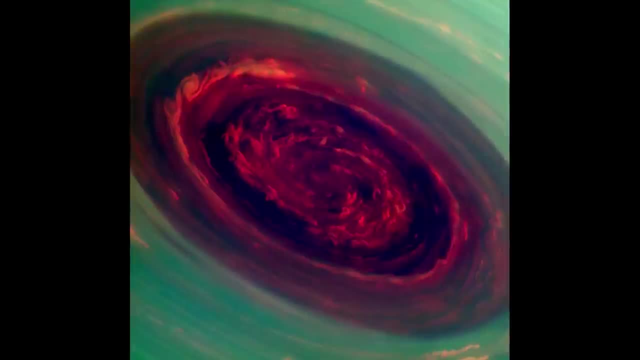 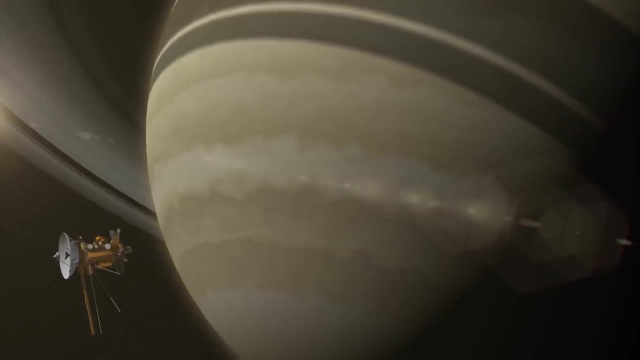 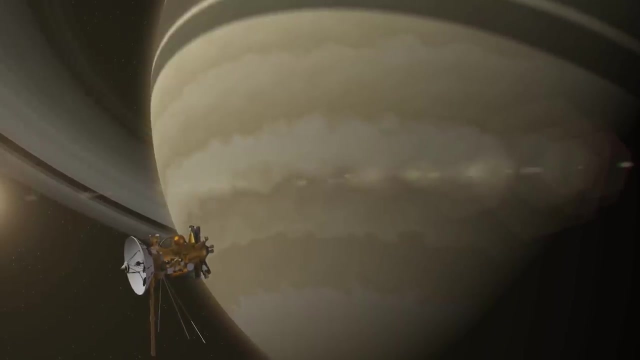 with red indicating lower cloud and green higher cloud. Winds at its edge blow at 540 kilometres per hour. One part of Cassini's dual-technique magnetometer had stopped working early in the mission. Without it, the craft had to do roll manoeuvres from time to time. 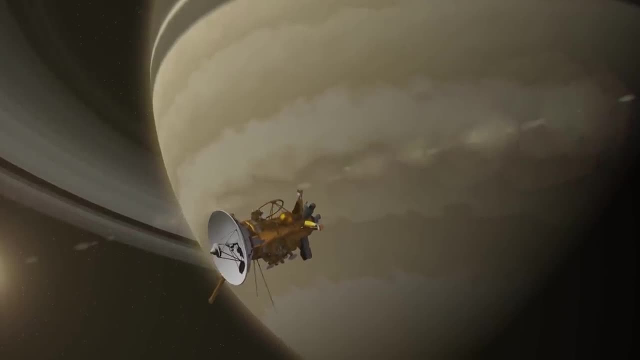 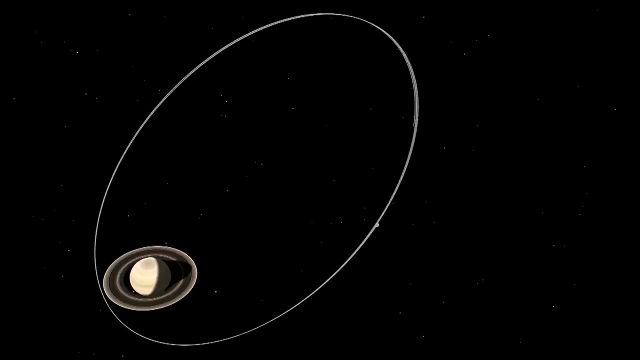 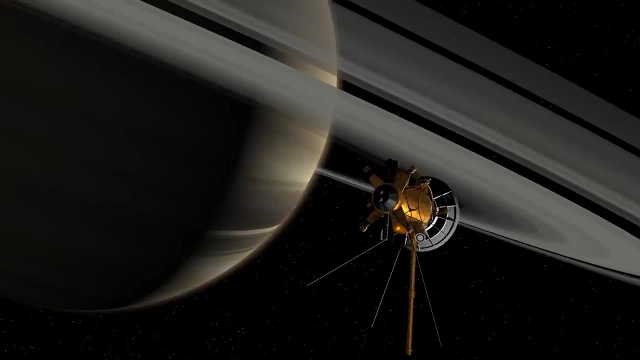 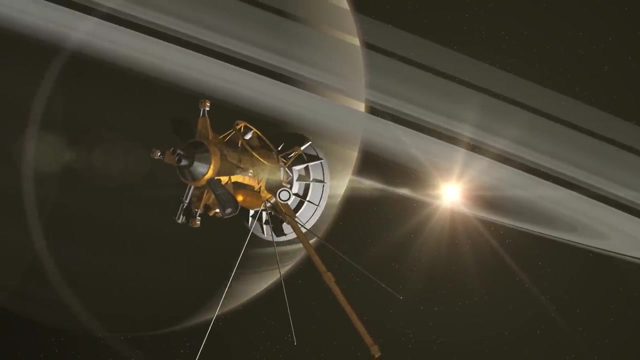 to calibrate the instrument. The spacecraft would make 20 ring-grazing orbits with the work of its instruments mapped out to the second. As the Sun was almost directly behind the rings, Cassini looked for dust clouds. Something is reducing ring particles to fine powder. 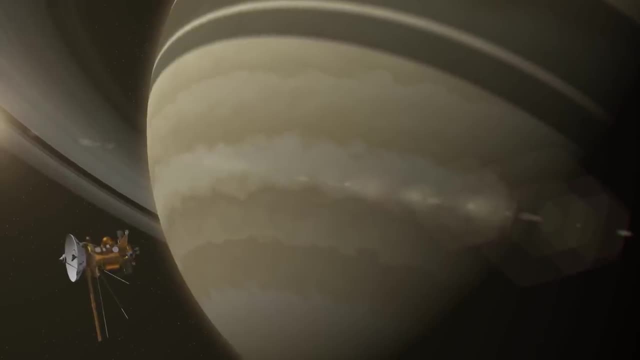 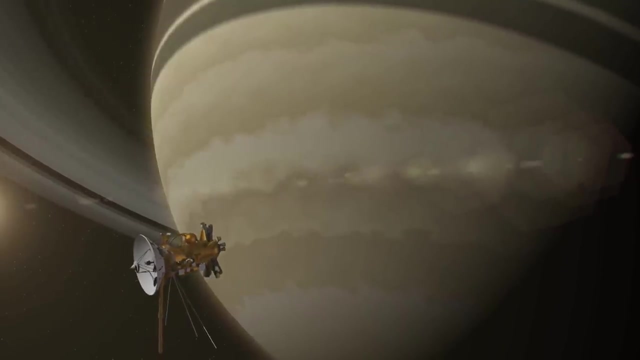 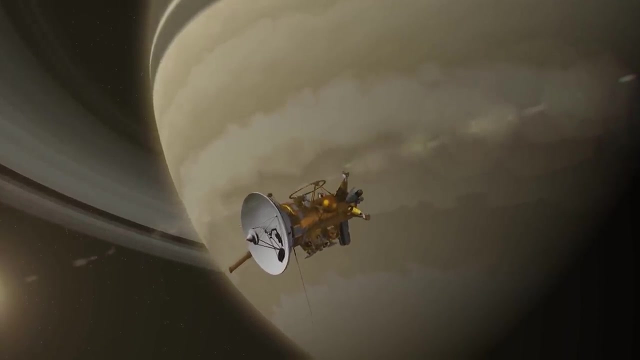 It is the second largest wind in the world. one part of Cassini's dual technique magnetometer had stopped working early in the mission. without it, the craft had to do roll maneuvers from time to time to calibrate the instrument. the spacecraft would make 20 ring raising. 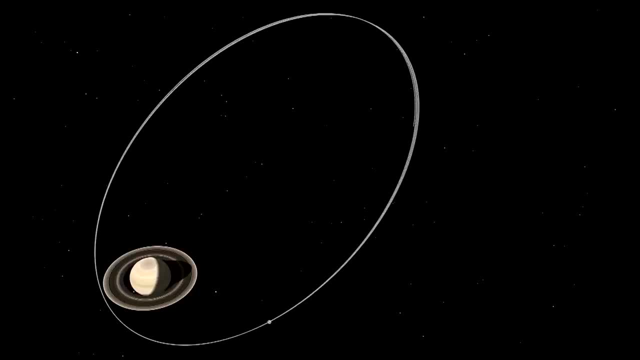 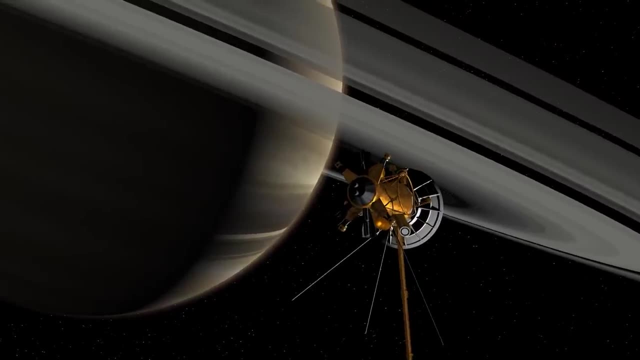 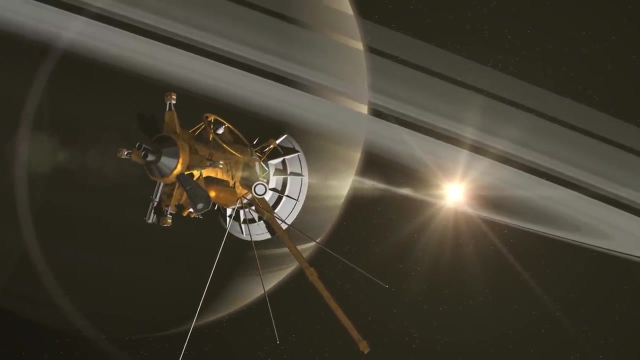 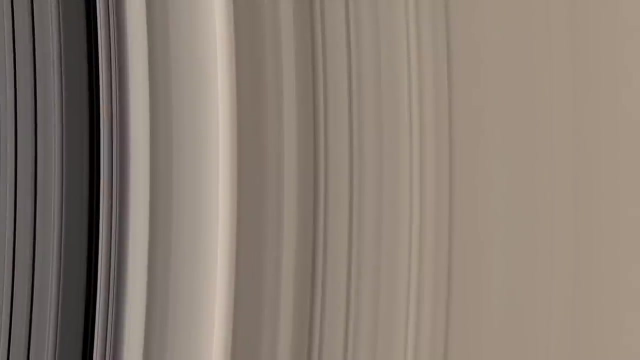 orbits with the work of its instruments mapped out to the second, as the Sun was almost directly behind the rings. Cassini looked for dust clouds. something is reducing ring particles to find powder. Cassini made a number of radio occultation observations with the rings between the spacecraft and earth. three: 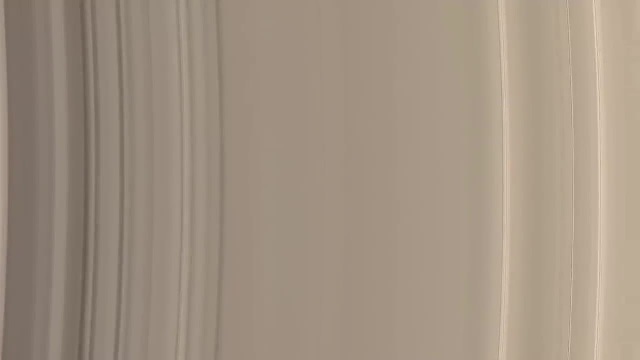 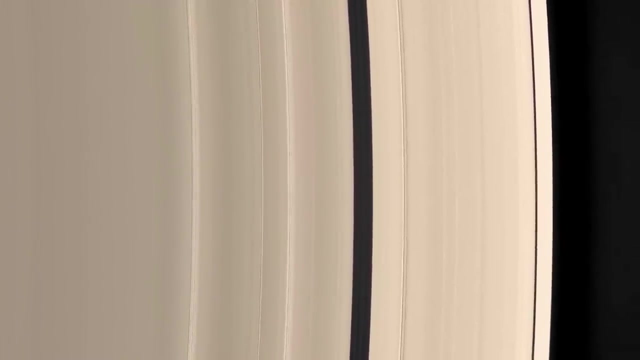 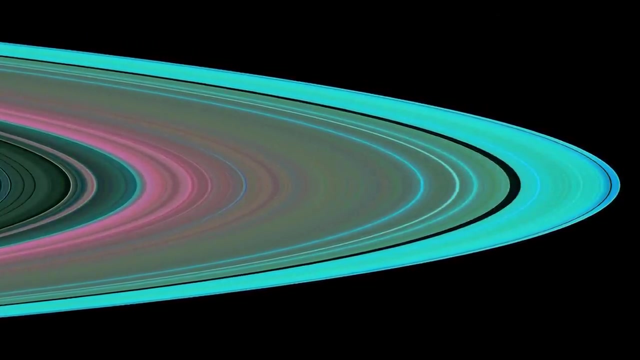 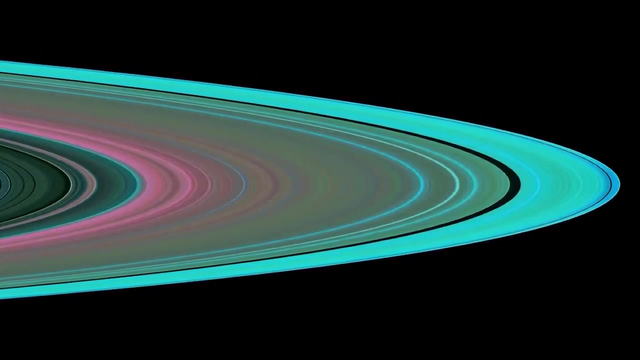 radio signals of differing wavelengths were transmitted simultaneously, allowing the radio science team to build a profile of the ring particles. this false color image of the airing, the outermost of the large bright rings, shows red for particles larger than five centimeters across. green denotes particles smaller than five centimeters, with blue for particles smaller than one. 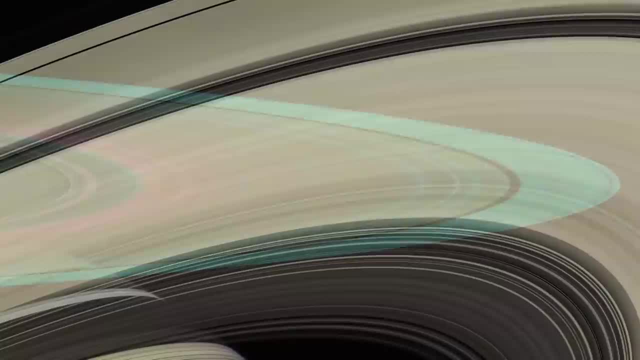 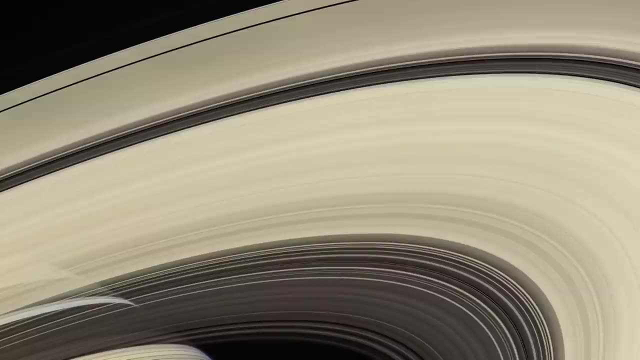 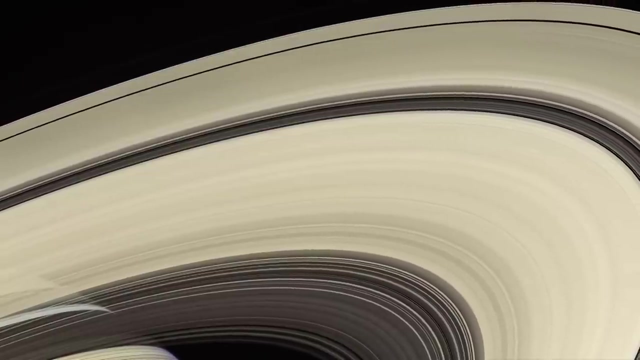 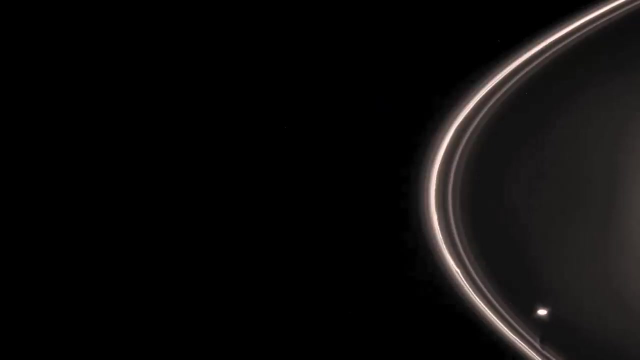 centimeter. the complex gravitational interaction between Saturn, its rings and its moons leads to gaps in very particular places. before Cassini arrived, only 18 moons were known. that number has grown to 62. Prometheus acts as a shepherding moon, limiting the inner edge of Saturn's f-ring, along with Pandora, which orbits outside the 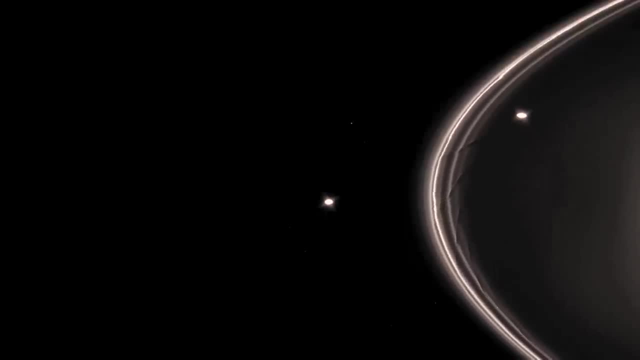 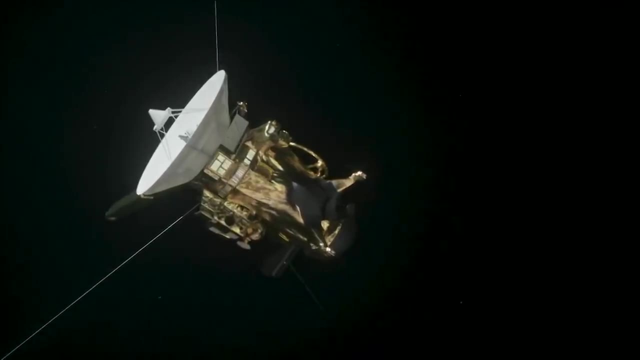 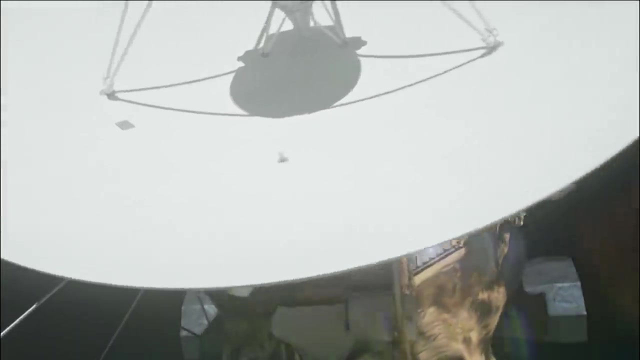 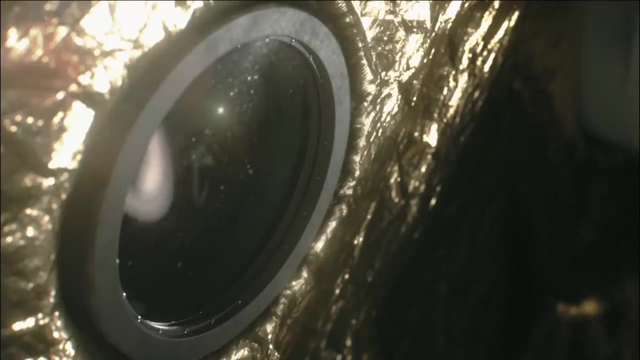 f-ring. the two moons keep the ring narrowly confined. in April 2017, Cassini's orbit was changed for the final phase of its mission. the probe would now loop in the rings, Though it would ultimately mean burning up in Saturn's atmosphere. the information 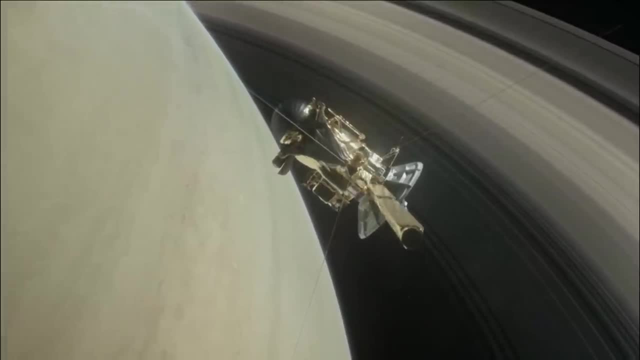 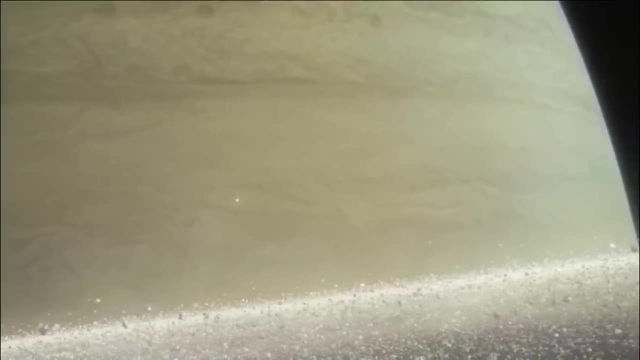 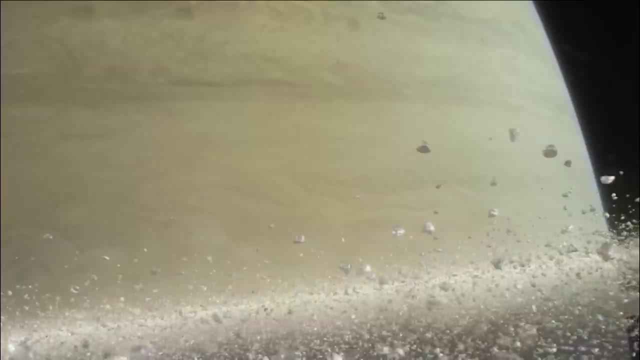 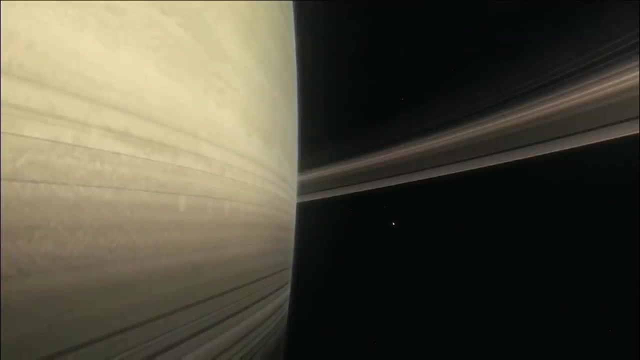 gathered from such close proximity to Saturn and its rings would give a fuller picture of the gas giant. It was decided that intentionally destroying Cassini was preferable to letting it drift without fuel possibly contaminating one of the moons. Cassini's sensors began picking up a stream of ring particles raining down upon Saturn. 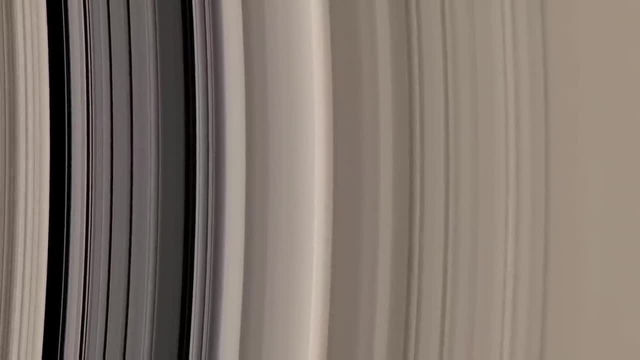 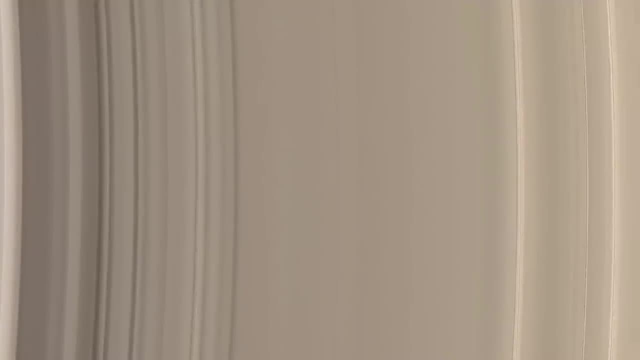 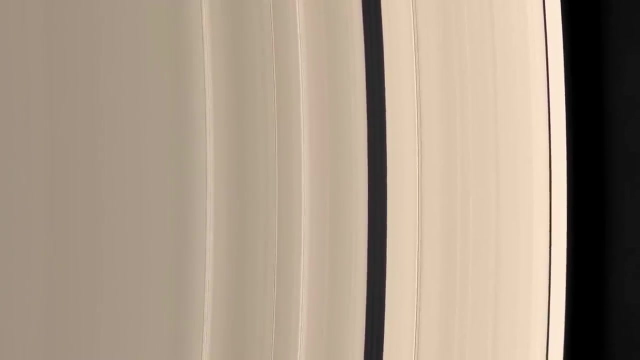 Cassini made a number of radio occultation observations With the rings between the spacecraft and Earth. three radio signals of differing wavelengths were transmitted simultaneously, allowing the radio science team to build a profile of the ring particles. This false-colour image of the A ring 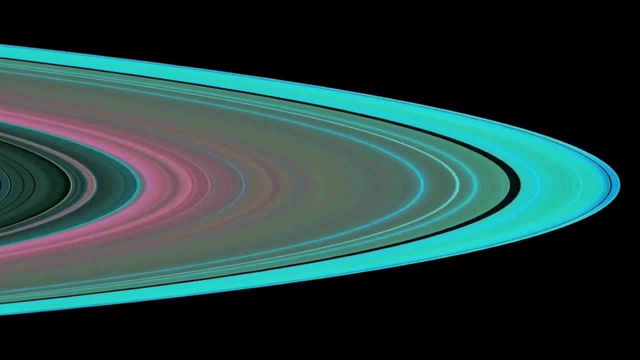 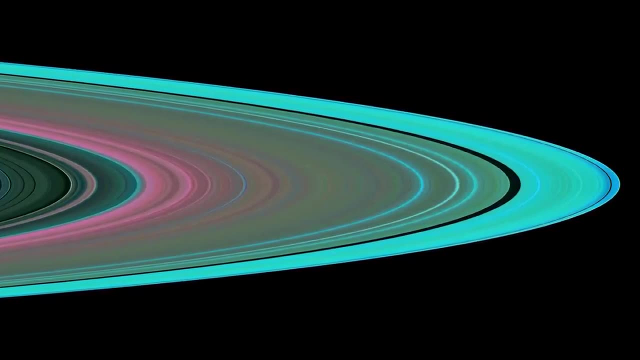 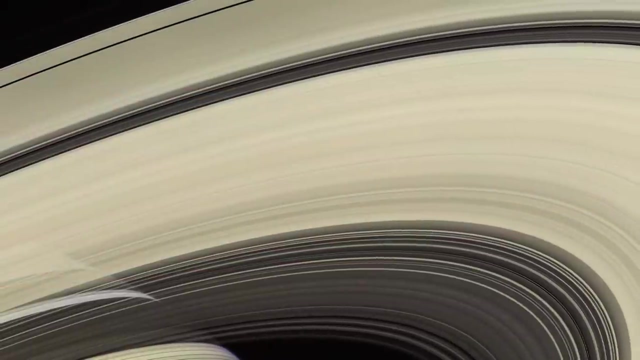 – the outermost of the large bright rings – shows red for particles larger than 5 centimetres across. Green denotes particles smaller than 5 centimetres, with blue for particles smaller than 1 centimetre. The complex gravitational interaction between Saturn. 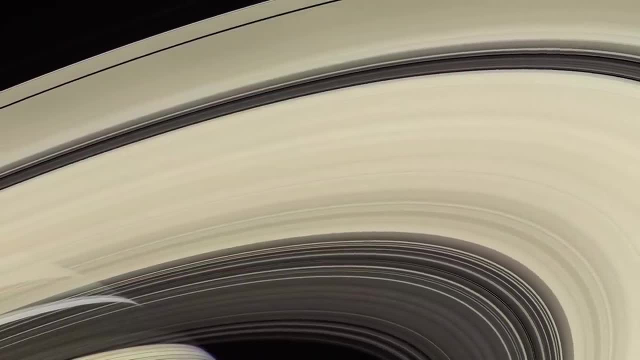 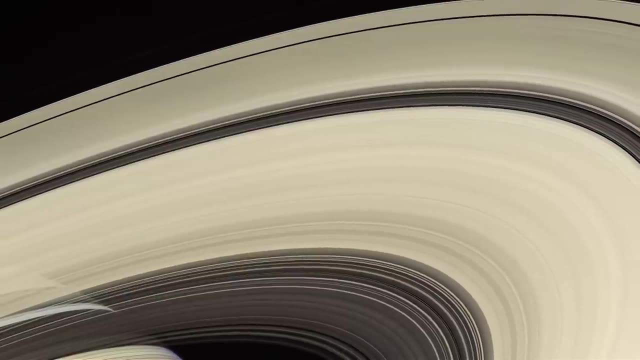 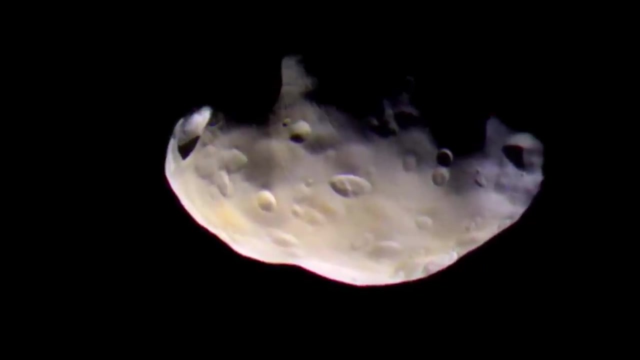 its rings and its moons leads to gaps in very particular places. Before Cassini arrived, only 18 moons were known. That number has grown to 62.. Prometheus acts as a shepherding moon, limiting the inner edge of Saturn's F ring. 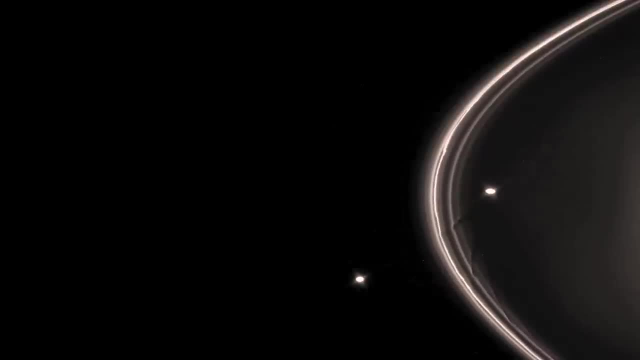 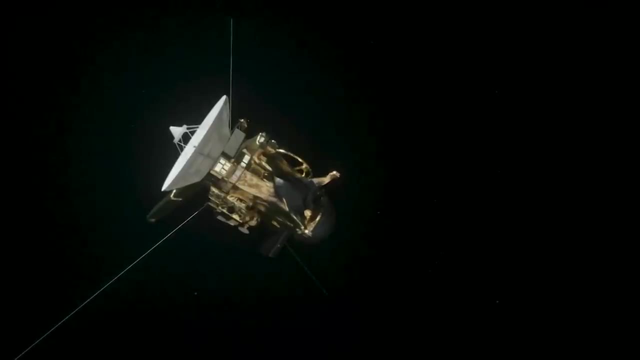 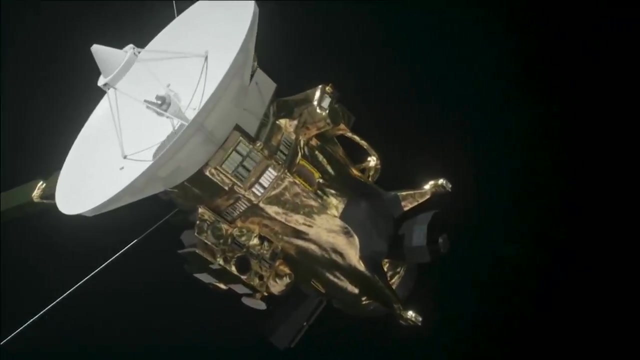 Along with Pandora, which orbits outside the F ring. the two moons keep the ring narrowly confined. In April 2017, Cassini's orbit was changed for the final phase of its mission. The probe would now loop inside the ring. Cassini's orbit would now loop inside the ring. 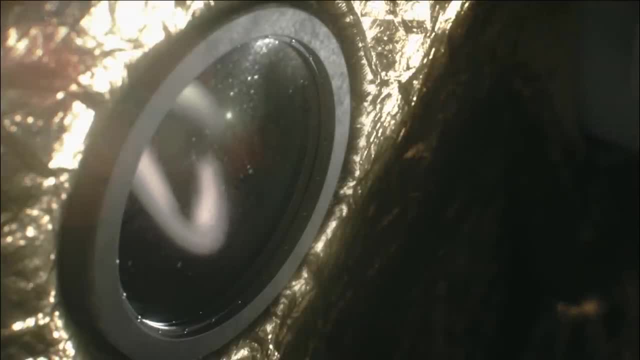 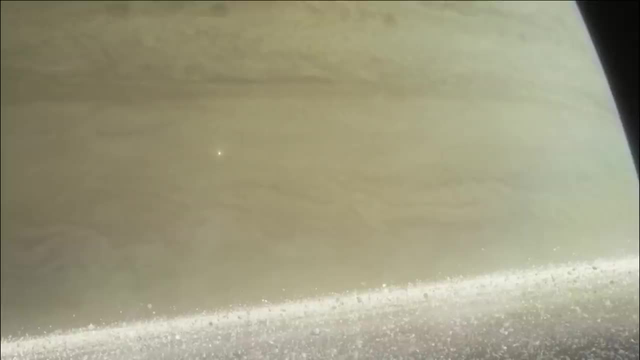 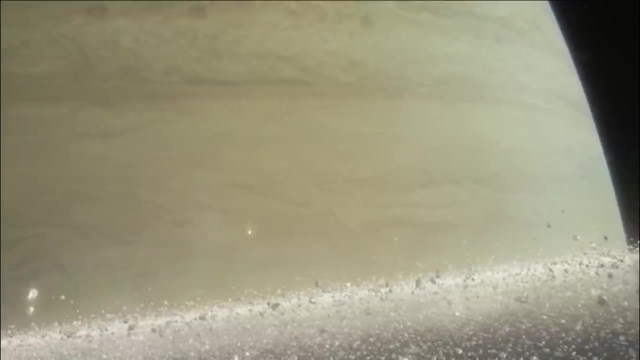 Though it would ultimately mean burning up in Saturn's atmosphere. the information gathered from such close proximity to Saturn and its rings would give a fuller picture of the gas giant. It was decided that intentionally destroying Cassini was preferable to letting it drift without fuel. 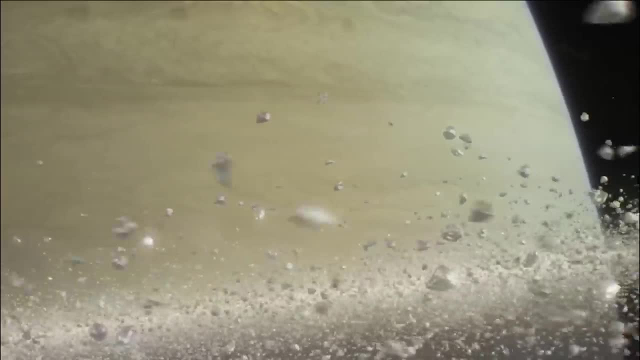 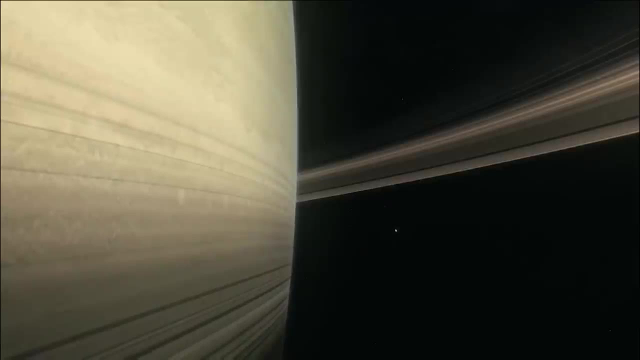 possibly contaminating one of the moons. Cassini's sensors began picking up a stream of ring particles. Cassini's sensors began picking up a stream of ring particles raining down upon Saturn. A continuous shower of ice and dust particles are dragged toward the planet's equator by gravity. 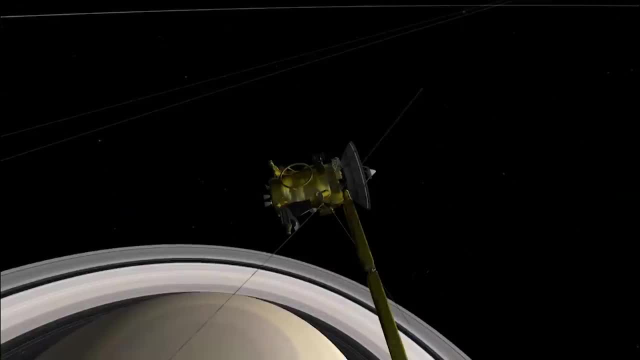 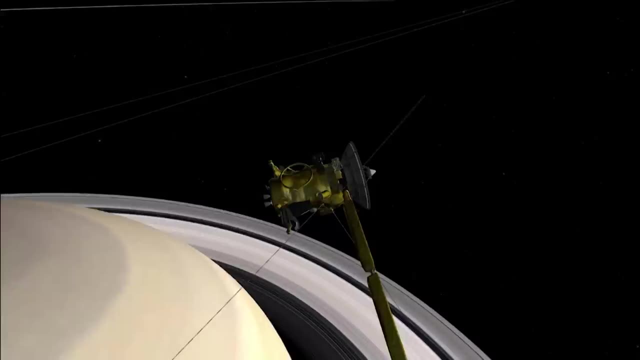 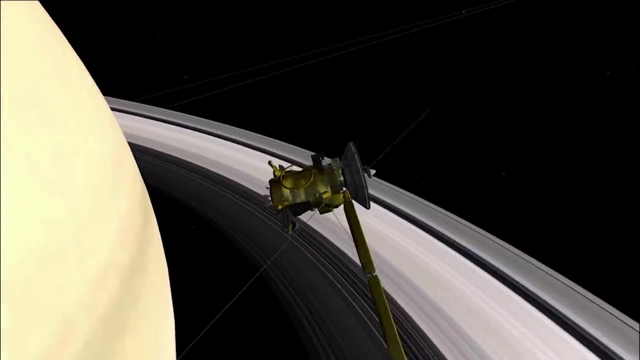 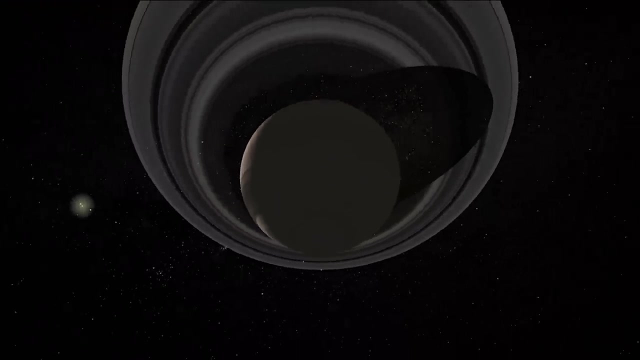 or at higher latitudes. charged ring particles spiral in along magnetic field lines. Every second, 10,000 kilograms of ring rain falls to the surface- the surface. at this rate, the rings will be completely gone in 100 million years. researchers were surprised to discover an electric current flowing between the inner d-ring. 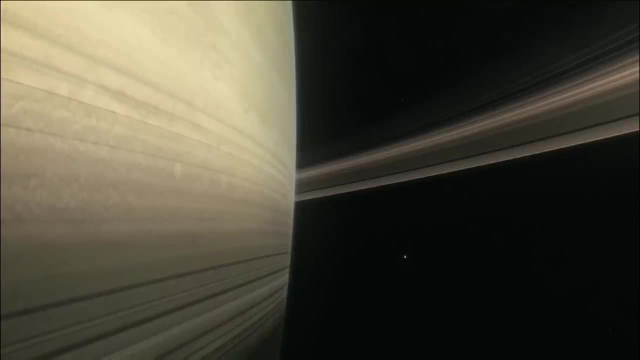 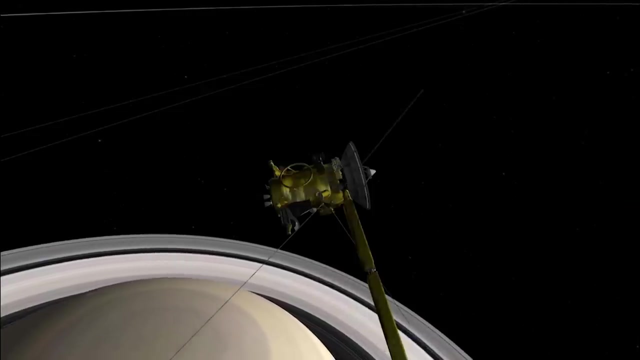 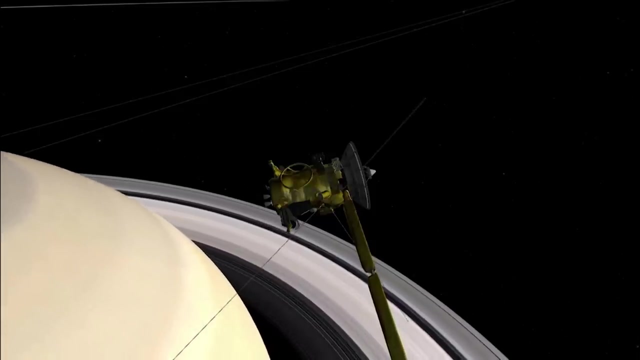 A continuous shower of ice and dust. particles are dragged toward the planet's equator by gravity or at higher latitudes. charged ring particles spiral in along magnetic field lines. Every second, 10,000 kilograms of ring rain falls to the surface. At this rate, the rings 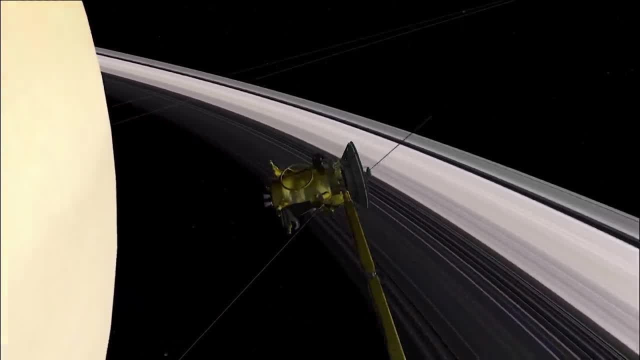 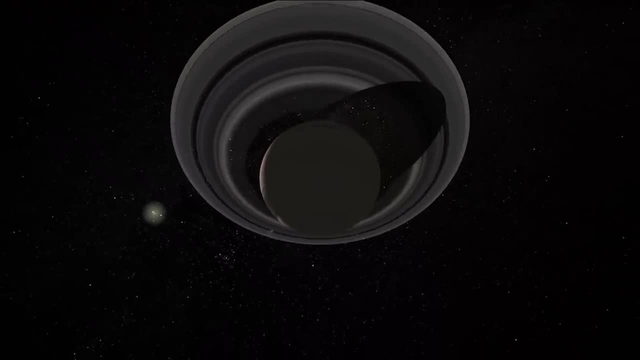 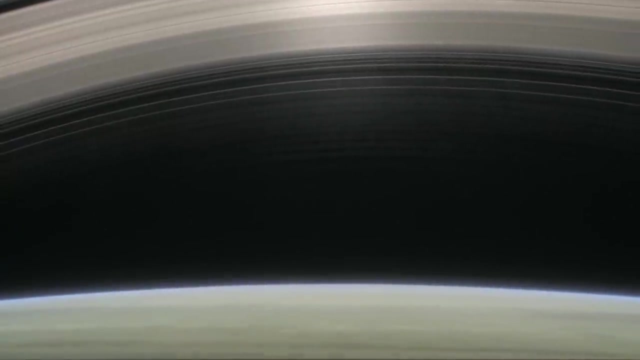 will be completely gone in 100 million years. Researchers were surprised to discover an electric current flowing between the inner D-ring and the upper atmosphere Toward the end of Cassini's close passes of Saturn. the spacecraft began catching the upper edge of the atmosphere. 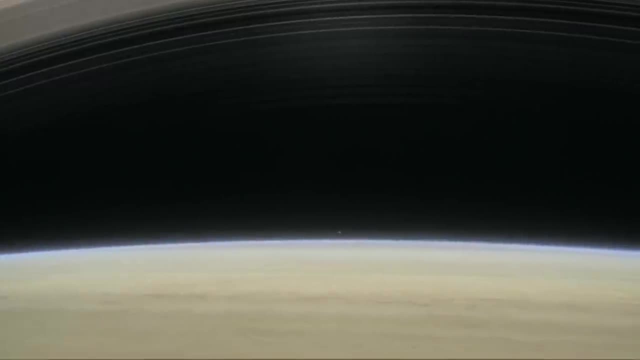 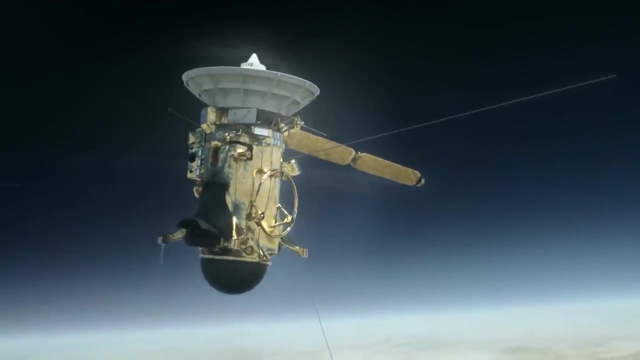 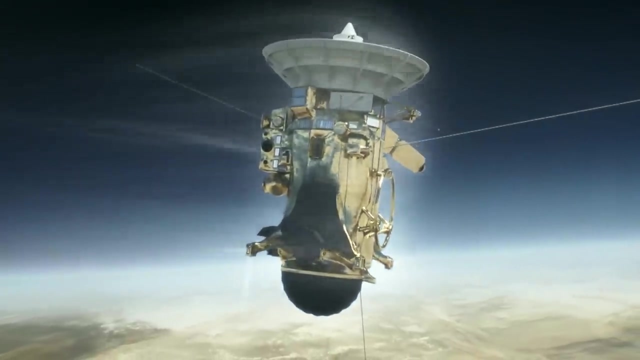 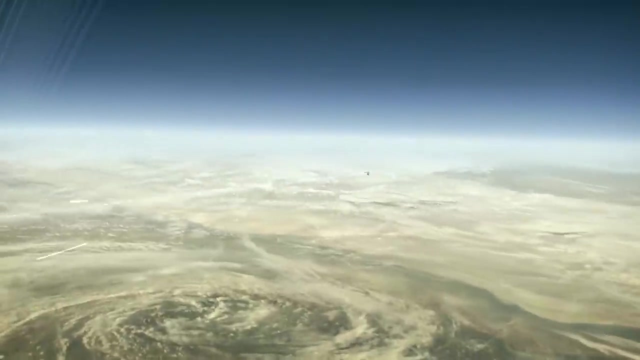 All information had been retrieved from the recorders. Data now was transmitted directly back to Earth, but it relied on the spacecraft's thrusters to stop Cassini from tumbling. keeping its high-gain antenna pointed accurately, The probe's final work was sampling the atmosphere and measuring the offset of Saturn's magnetic 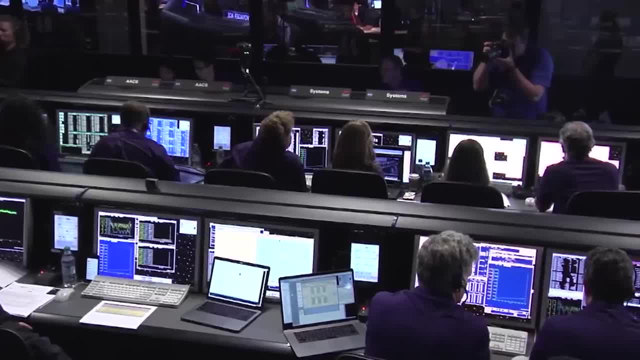 axis. This is VCS-1.. We just had pre-trial data. The probe's final work was sampling the atmosphere and measuring the offset of Saturn's magnetic axis. This is VCS-1.. We just had pre-trial data. The probe's final work was sampling the atmosphere. 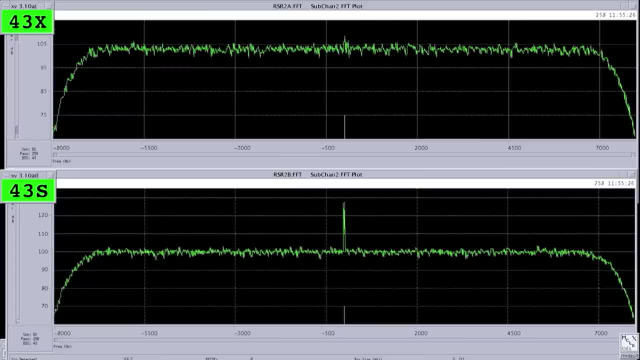 and measuring the offset of Saturn's magnetic axis. This is VCS-1.. We just had pre-trial data. The probe's final work was sampling the atmosphere and measuring the offset of Saturn's magnetic axis. This is VCS-1.. We just had pre-trial data. 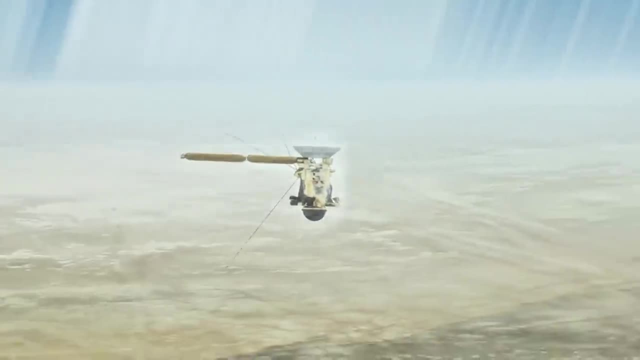 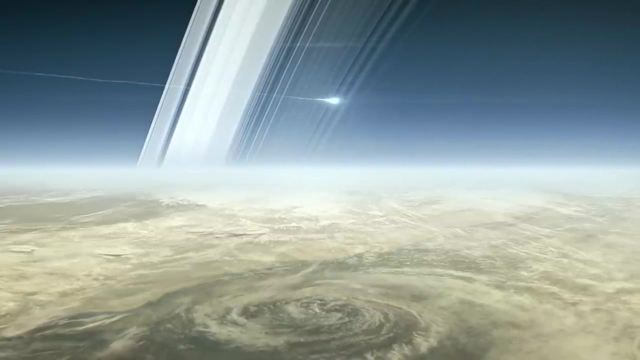 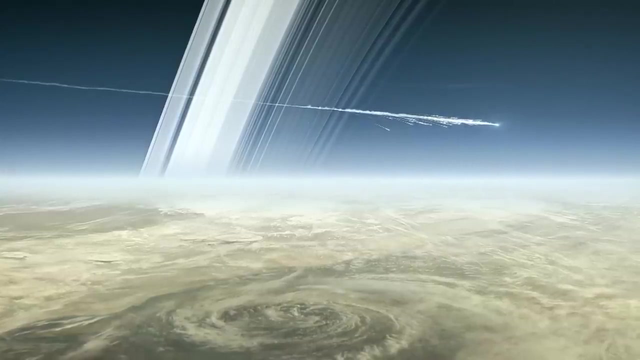 In mission control. there was no more control. The engineers could just monitor the signals sent from Saturn 84 minutes previously. The signal from the spacecraft is gone, and within the next 45 seconds so will be the spacecraft. It will take years to process the data gained from Cassini. As yet, there are no future. 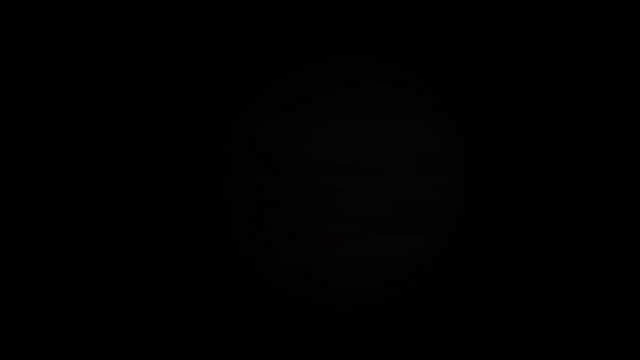 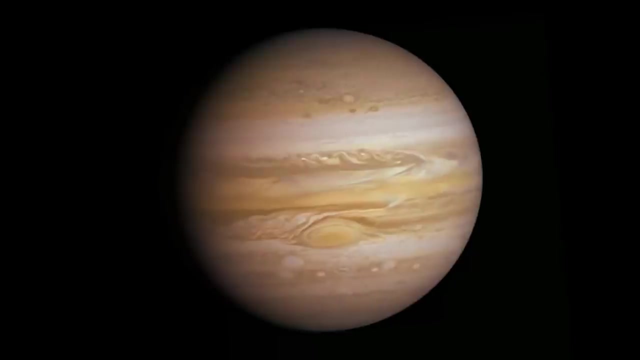 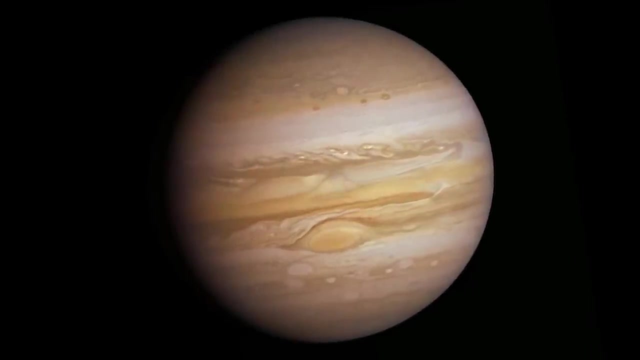 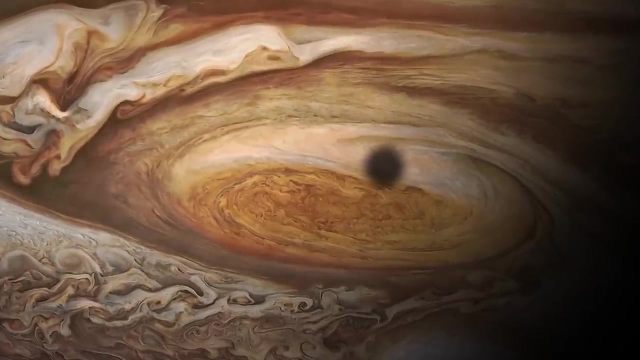 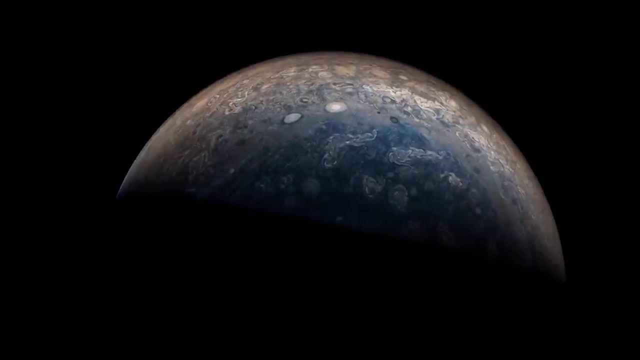 missions to Saturn scheduled. Jupiter is our solar system's largest planet. It's more than twice the mass of all the other planets combined. Its swirling atmosphere moves in bands at different latitudes and its great red spot is thought to be a perpetual storm. Recently, images from a new probe that has flown above 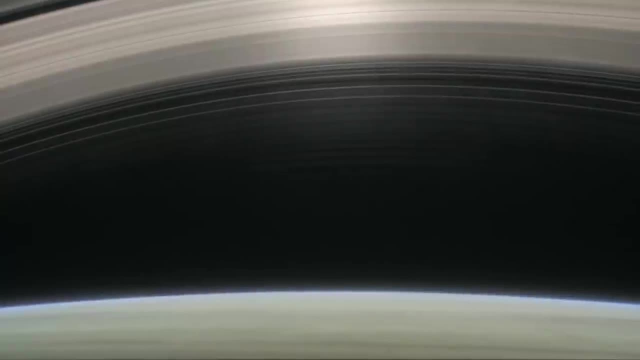 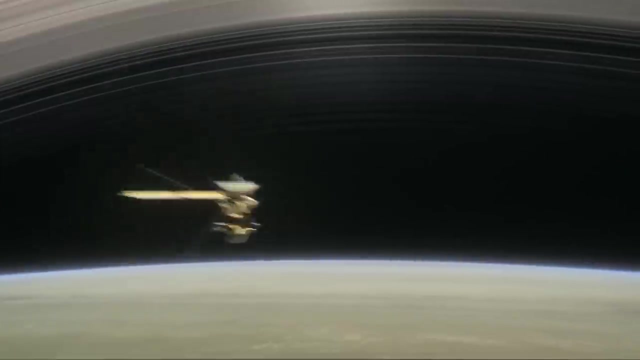 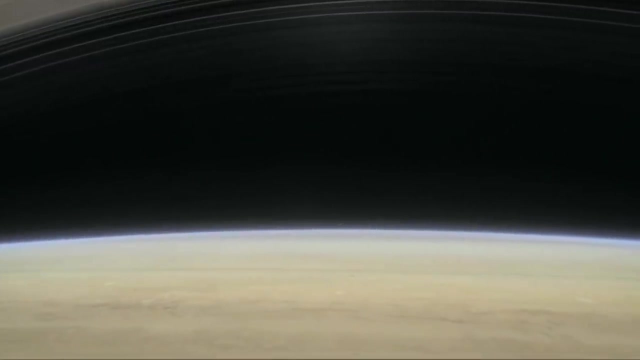 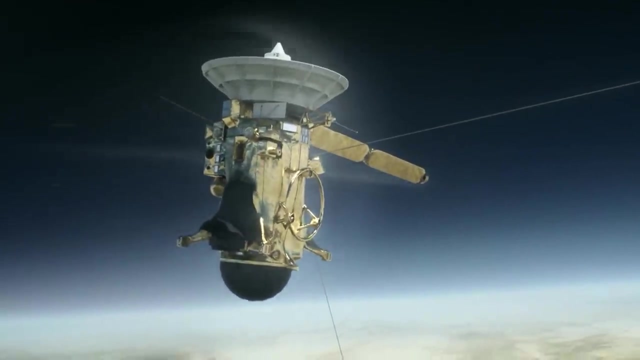 and the upper atmosphere. toward the end of cassini's close passes of saturn, the spacecraft began catching the upper edge of the atmosphere. all information had been retrieved from the recorders. data now was transmitted directly back to earth, but it relied on the spacecraft's thrusters to stop cassini from tumbling. 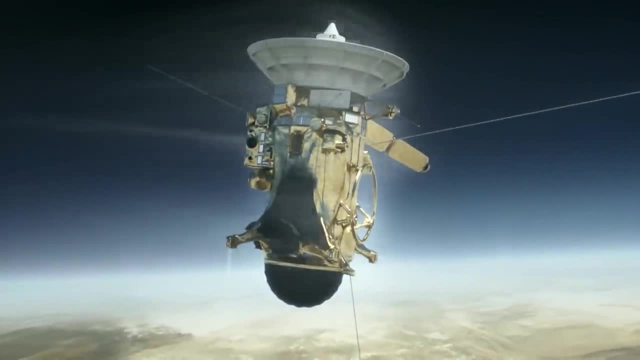 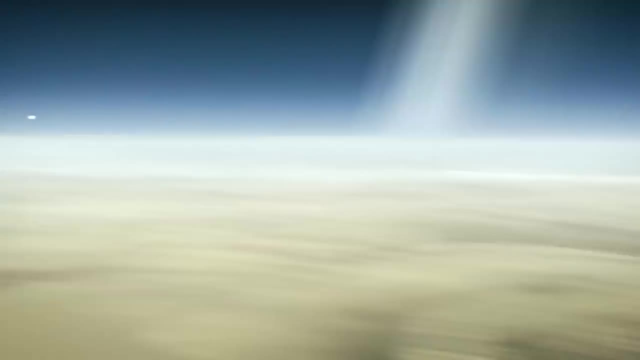 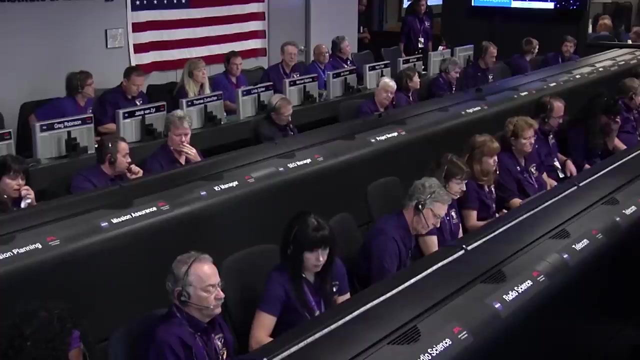 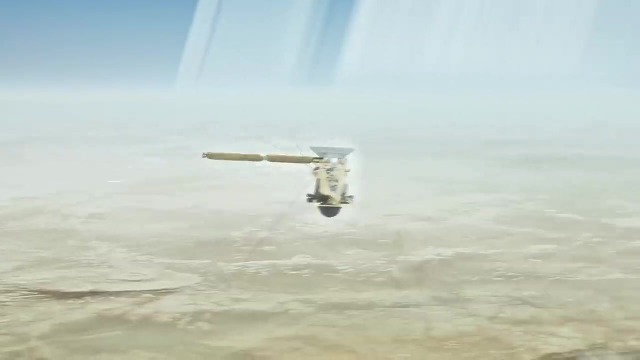 keeping its high gain antenna pointed accurately. the probe's final work was sampling the atmosphere and measuring the offset of saturn's magnetic axis. this is bcs1. we just had transition to high rate in mission control. there was no more control. the engineers could just monitor the signal sent from saturn 84 minutes previously. 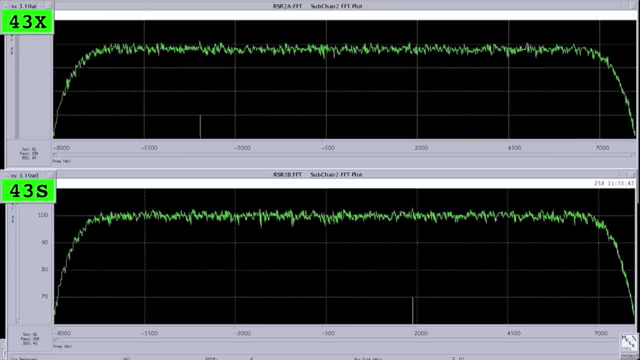 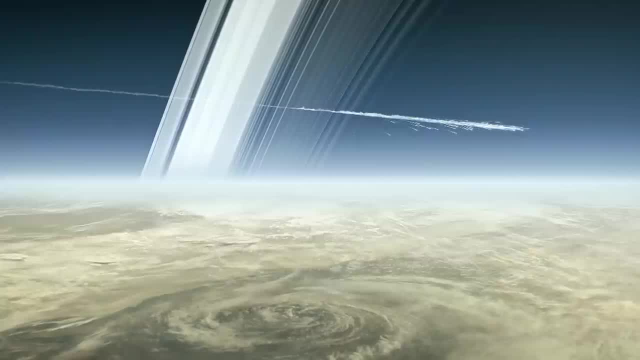 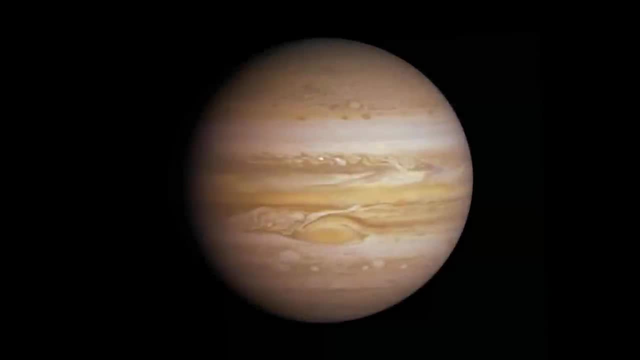 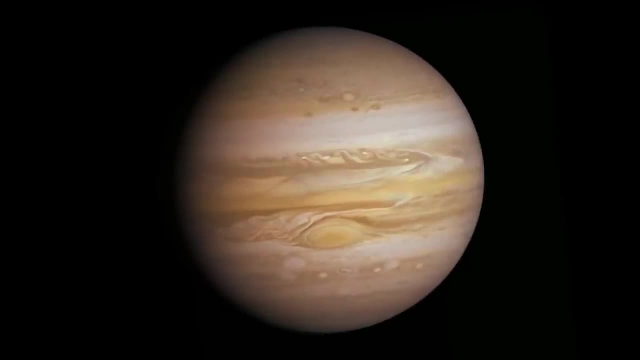 the signal from the spacecraft is gone and within the next 45 seconds so will be the spacecraft. it will take years to process the data gained from cassini. as yet, there are no future missions to saturn scheduled. jupiter is our solar system's largest planet. it's more than twice the mass of all the other planets combined. 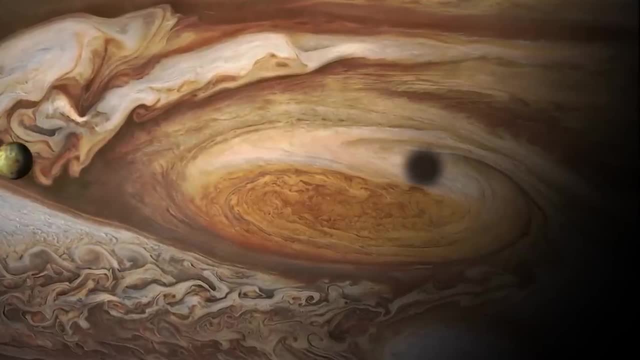 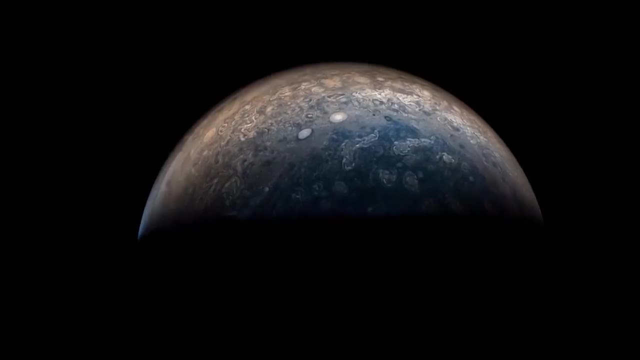 its swirling atmosphere moves in bands at different latitudes and its great red spot is thought to be a perpetual storm. recently, images from a new planet have been found in the atmosphere of the solar system, images from a new probe that has flown above jupiter's poles. 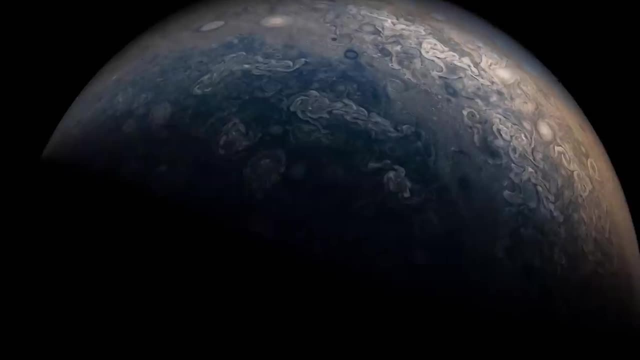 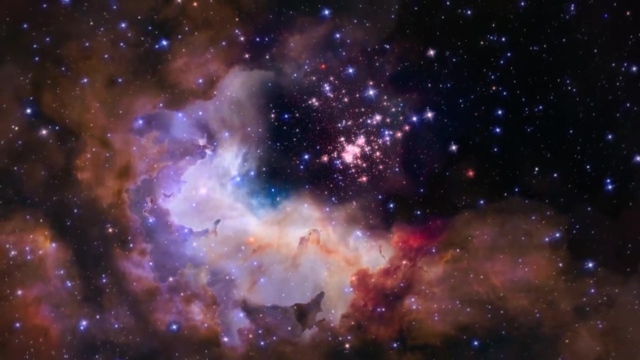 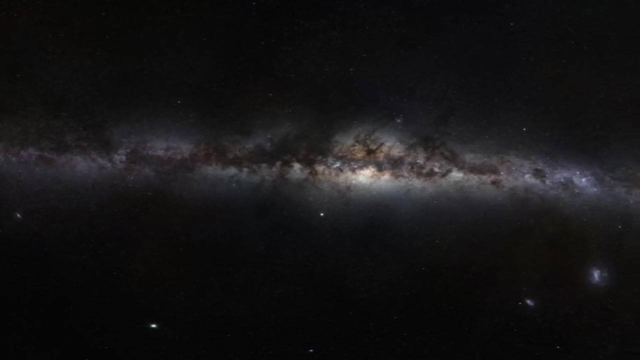 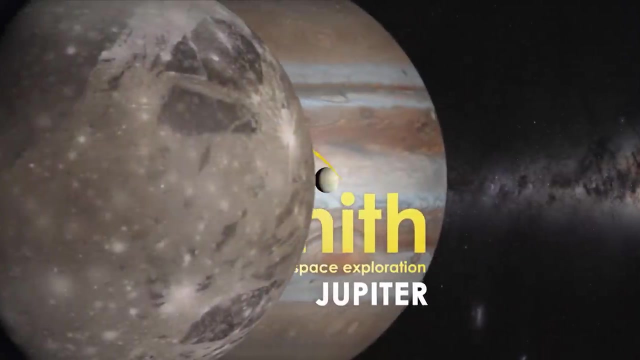 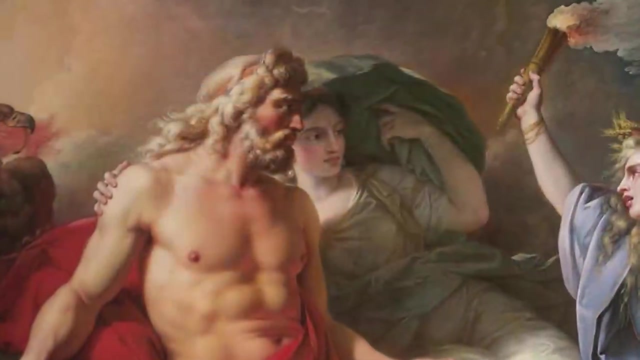 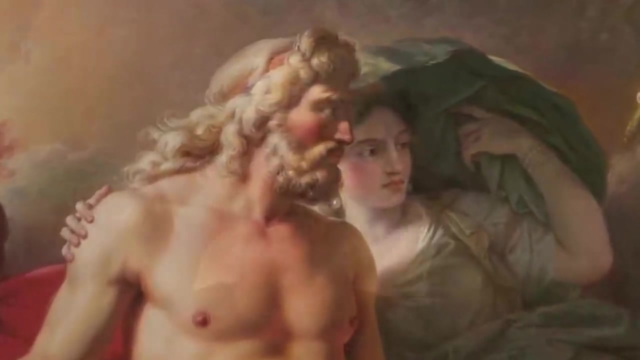 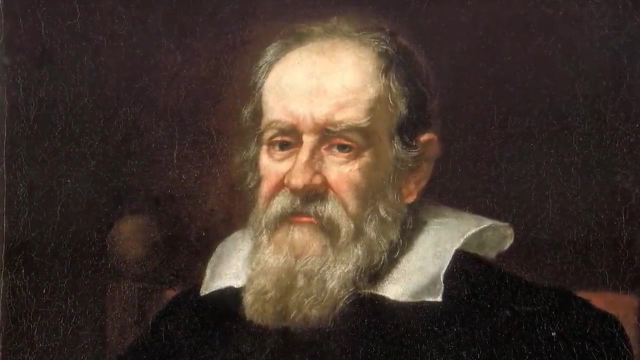 reveal a completely different planet. so the ancient romans knew jupiter as the celestial representation of the king of the gods. in 1610, galileo, using his newly improved telescope, saw jupiter's moons and could see they orbited the planet, evidence that not everything revolved around the earth as the church had declared. 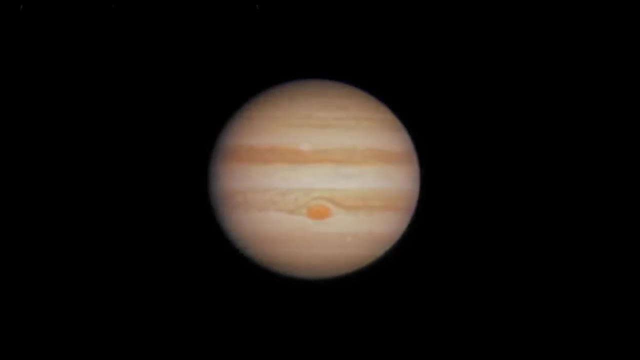 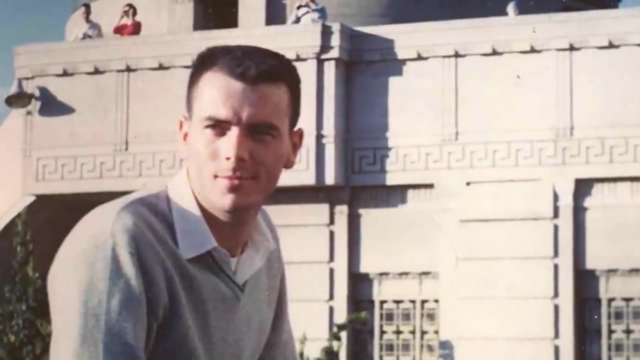 though better telescopes improved our view of jupiter, the solar system is still the same as ever. the solar system is still the same as ever. it was not until 1964 that gary flandro, a graduate student working part-time at nasa's jpl. 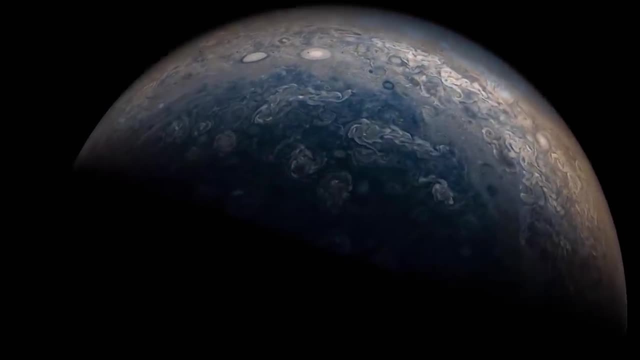 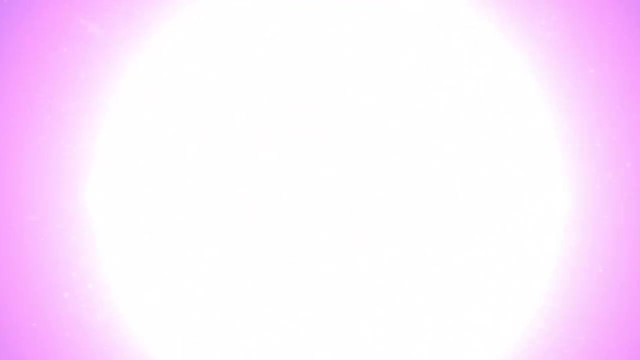 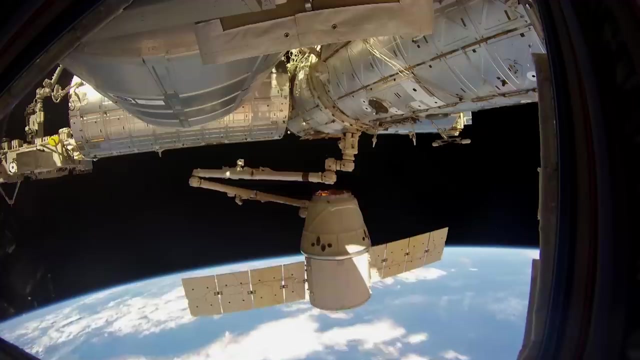 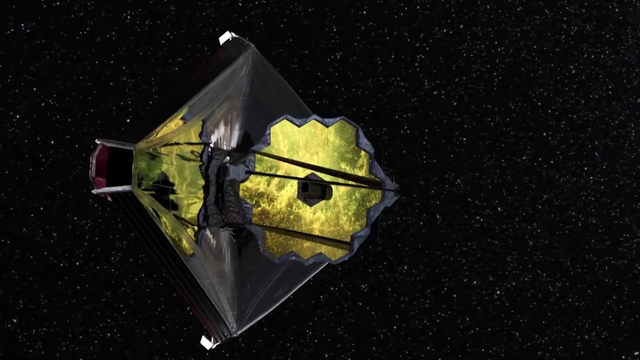 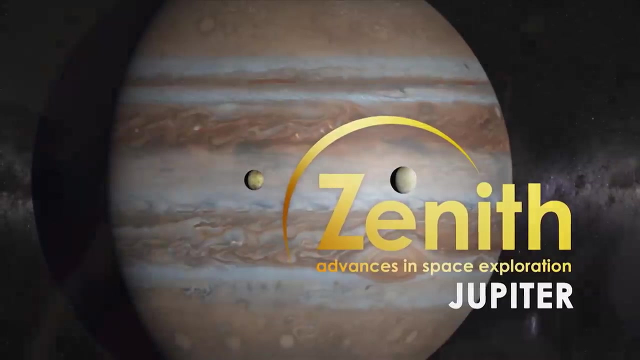 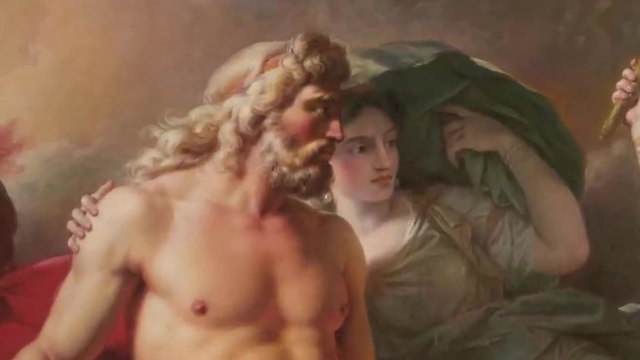 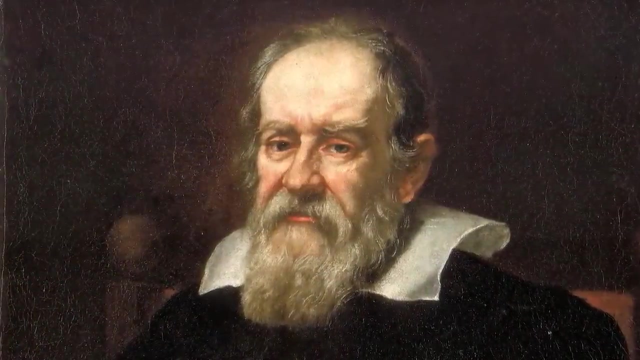 Jupiter's poles reveal a completely different planet. The ancient Romans knew Jupiter as the celestial representation of the king of the gods. In 1610, Galileo, using his newly improved telescope, saw Jupiter's moons and could see they orbited the planet. 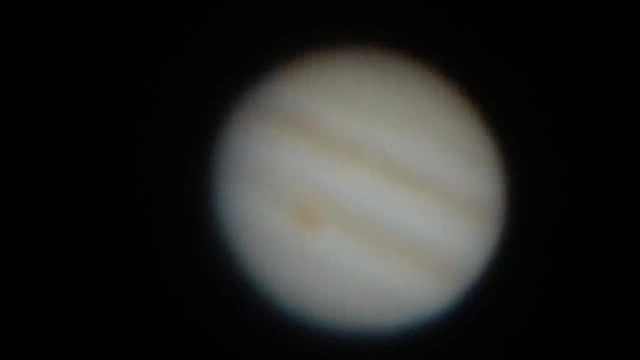 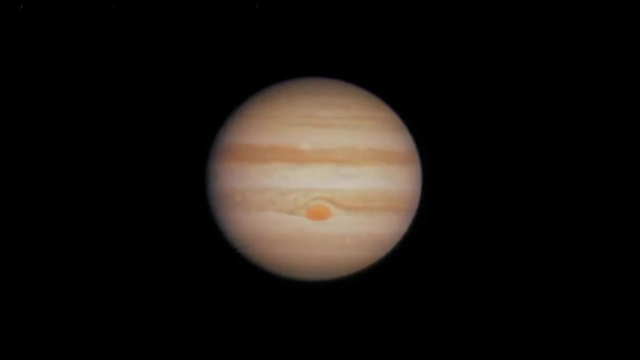 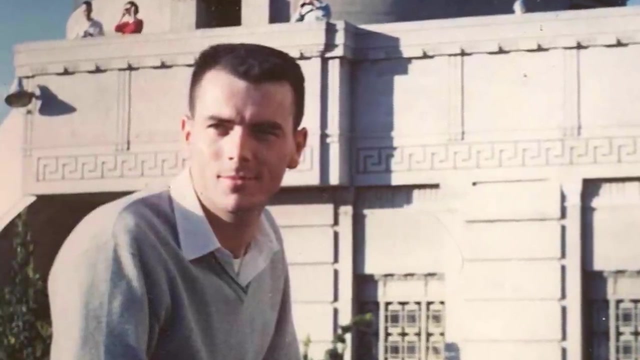 evidence that not everything revolved around the Earth as the Church had declared. Though better telescopes improved our view of Jupiter, it was not until 1964 that Gary Flandro, a graduate student working part-time at NASA's JPL, understood there was a way. 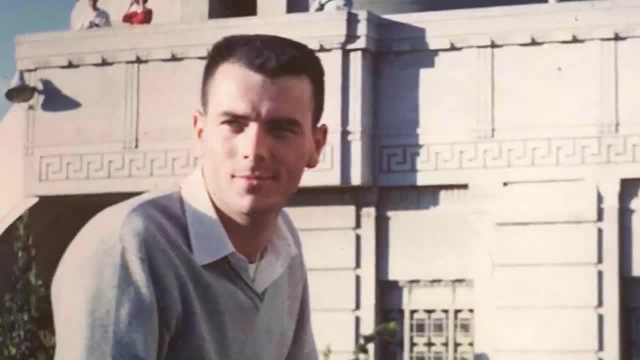 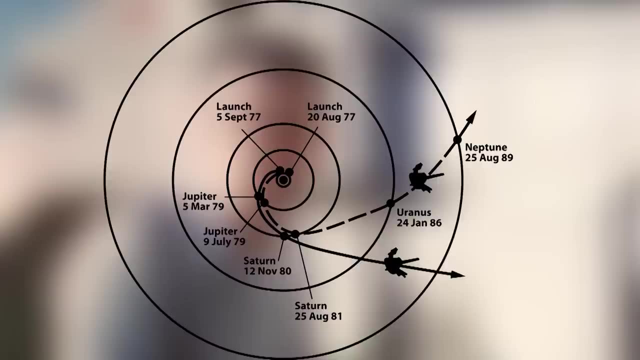 to get a clearer look at Jupiter By plotting the positions of the outer planets. he realised that a rare alignment would enable a spacecraft launched in 1977, to visit Jupiter, Saturn, Uranus and Neptune. NASA jumped at the opportunity and began work on twin craft. 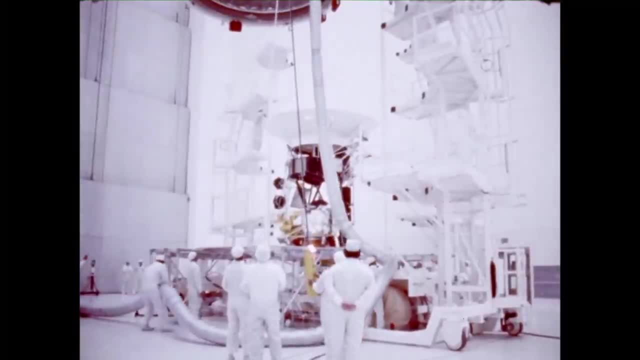 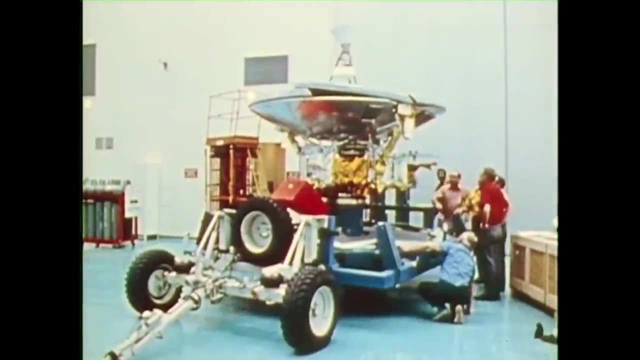 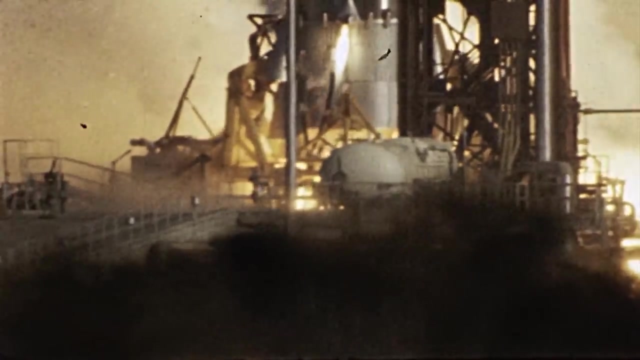 for what was then known as the Planetary Grand Tour. To limit any possibility, two basic spacecraft known as Pioneer 10 and 11, were quickly built. They would go ahead of the Grand Tour missions to send back information about the environment. 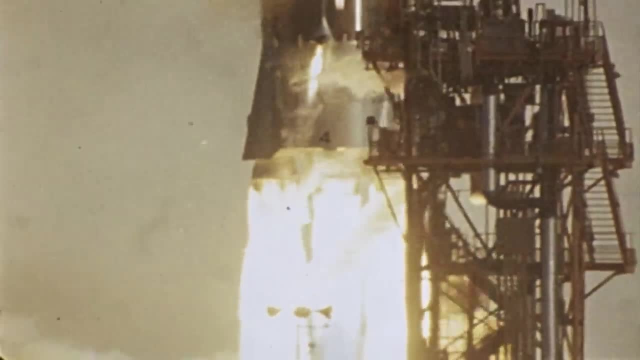 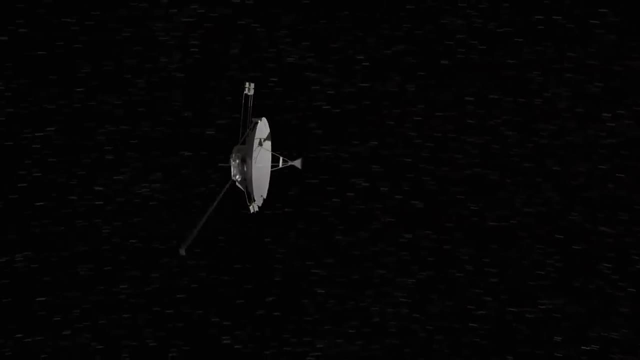 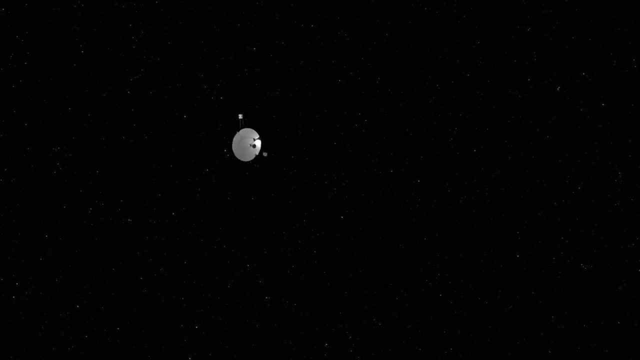 Pioneer 10 was launched toward Jupiter in March 1972.. It was the first spacecraft to cross the asteroid belt that lay between Mars and Jupiter, and because it was a space plane trip, Because it was the first probe on a trajectory that would take it out of the solar system, 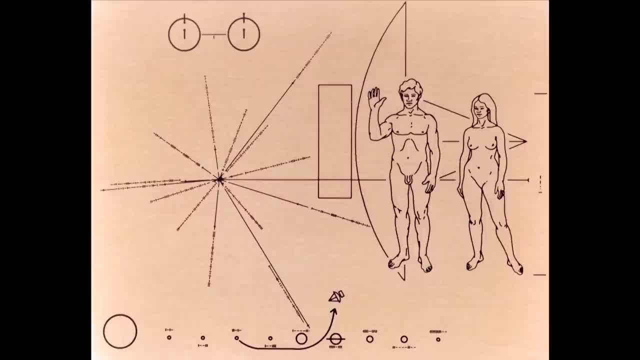 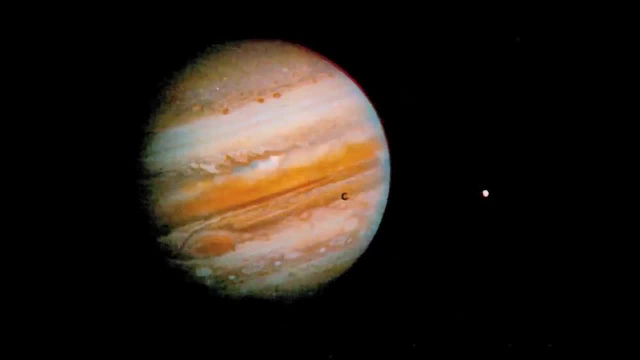 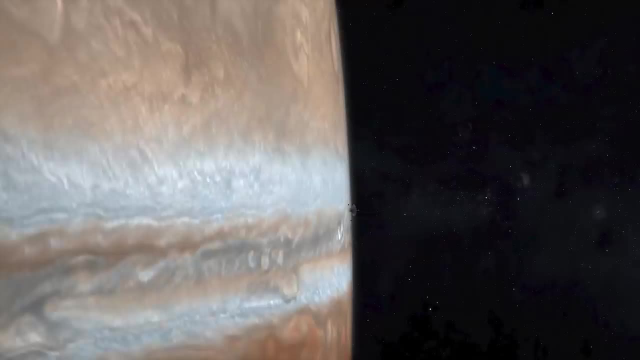 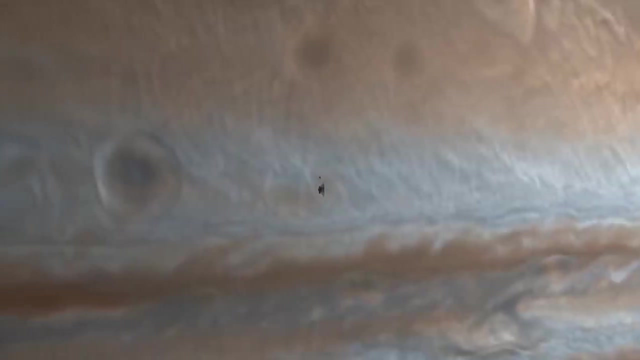 it carried a plaque identifying its origin. By December 1973, Pioneer 10 was sending back pictures of Jupiter clearer than anything that had been seen before. Approaching Jupiter, it encountered levels of ion radiation 10,000 times more intense than the radiation belts surrounding Earth. 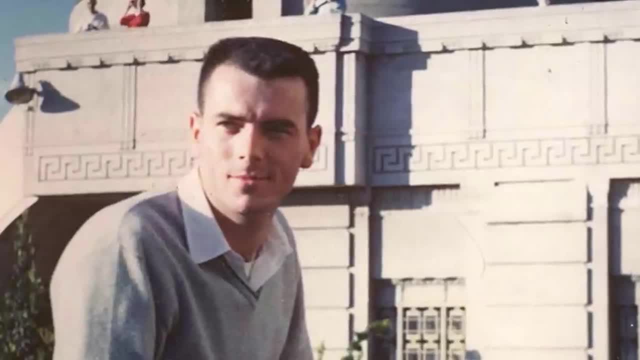 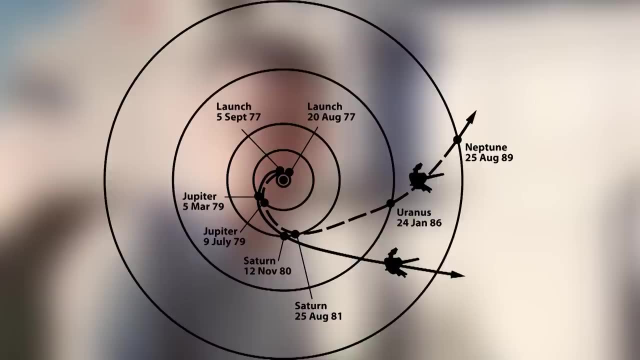 understood there was a way to get a clearer look at jupiter by plotting the positions of the outer planets. he realized that a rare alignment would enable a spacecraft launched in 1977 to visit jupiter, saturn, uranus and neptune. nasa jumped the opportunity and began work on. 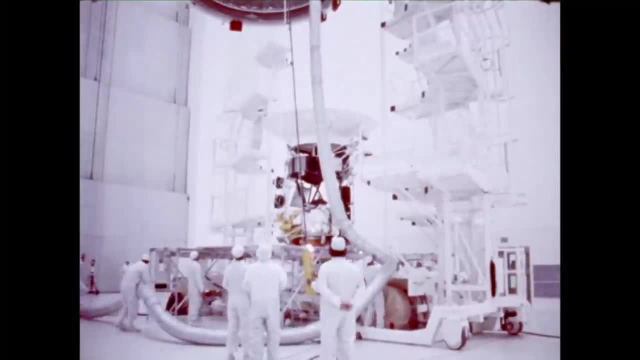 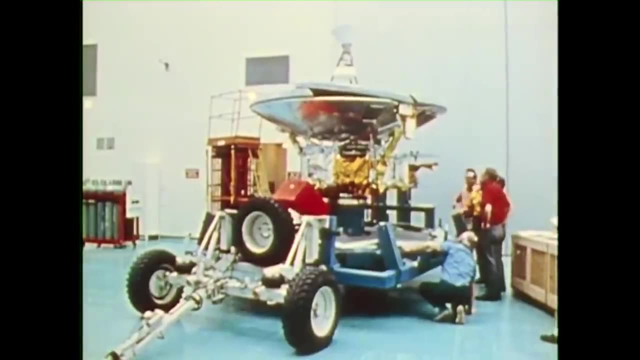 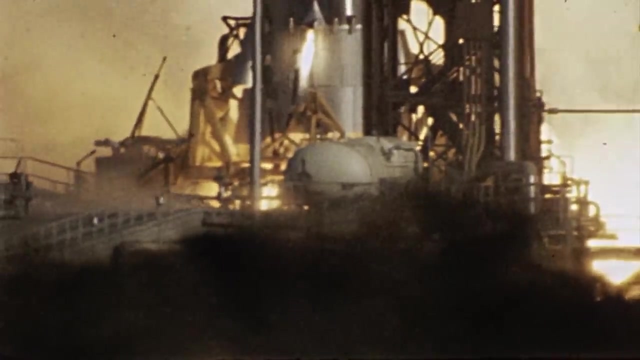 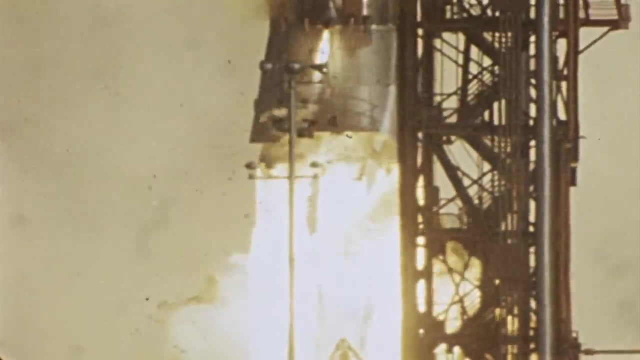 twin craft for what was then known as the planetary grand tour. to limit any surprises, two basic spacecraft known as pioneer 10 and 11 were quickly built. they would go ahead of the grand tour missions to send back information about the environment. pioneer 10 was launched toward jupiter in march. 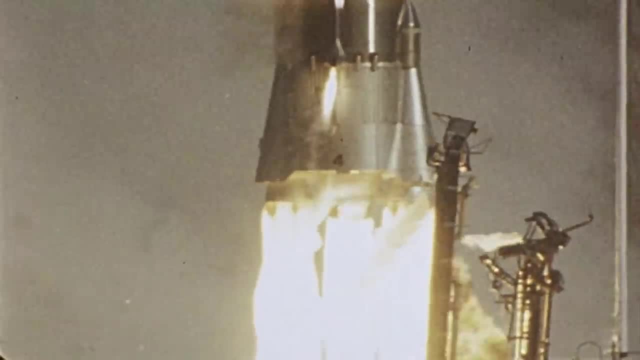 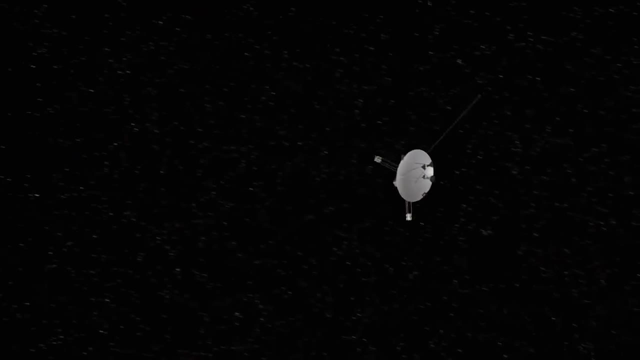 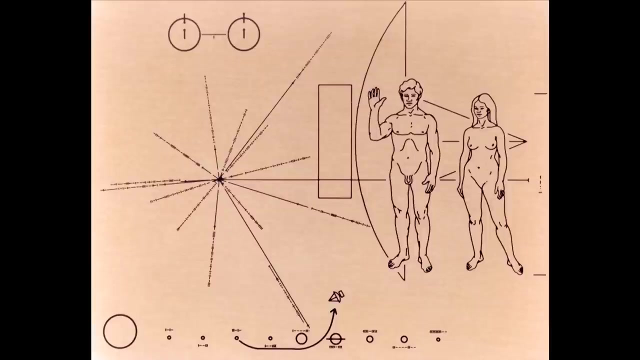 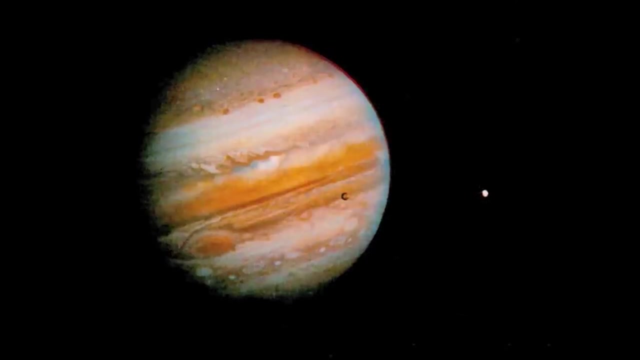 1972, it was the first spacecraft to cross the asteroid belt that lay between mars and jupiter, and because it was the first probe on a trajectory that would take it out of the solar system, it carried a plaque identifying its origin. by december 1973, pioneer 10 was sending back pictures of jupiter clearer than anything that. had been seen. before approaching jupiter, it encountered levels of iron radiation 10 000 times more intense than the radiation belts surrounding earth. as the probe skimmed past the giant planet, it gained speed, leaving earth. pioneer 10 was moving at 51 000 kilometers per hour, departing jupiter. it had more. 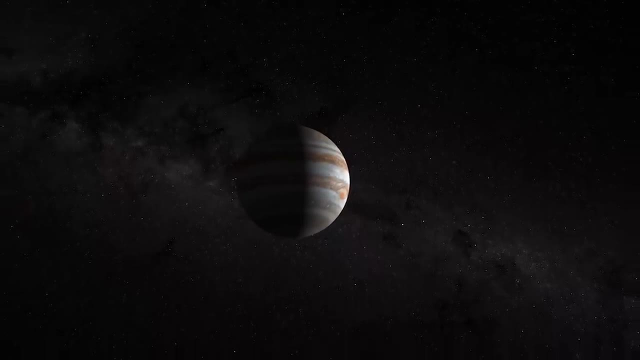 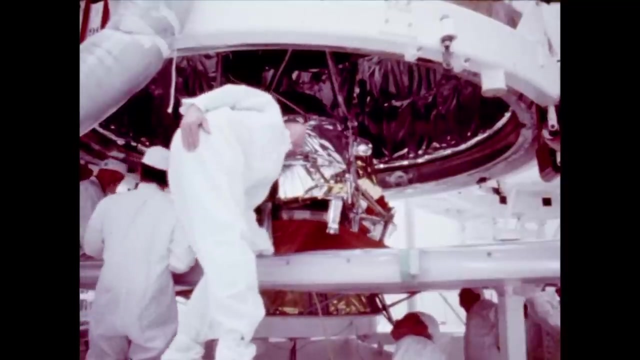 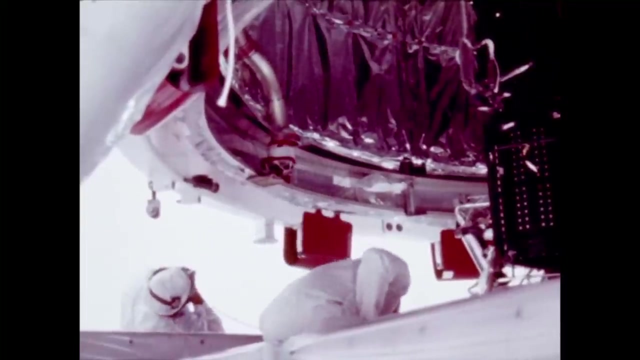 than doubled its speed. this gravitational slingshot effect made the grand tour possible. the grand tour craft, recently renamed voyager 1 and 2, were due to be transferred to cape canaveral for launch integration when news of jupiter's extreme radiation environment came through. 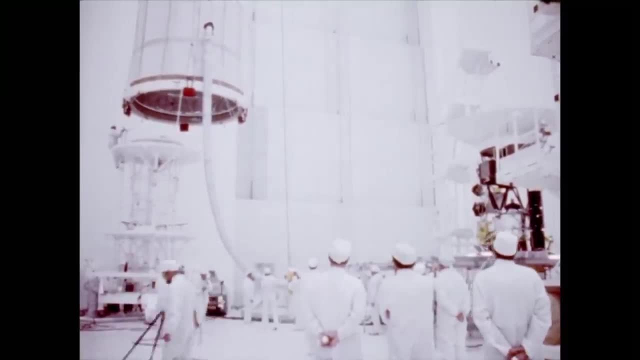 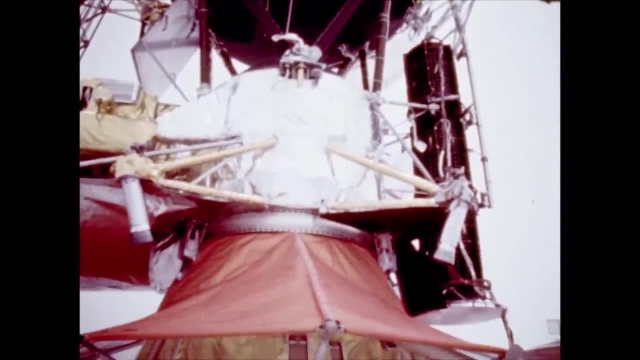 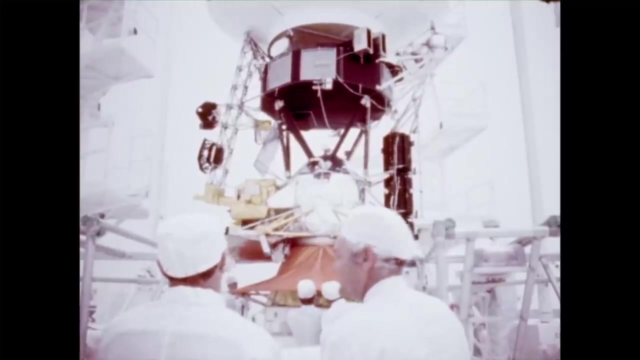 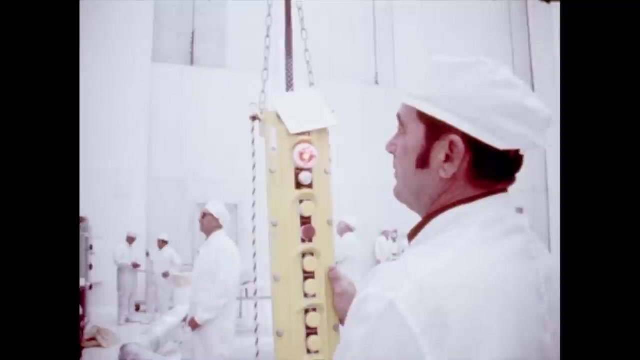 the electron radiation at jupiter had generated false commands within pioneer 10 with the far more sophisticated voyagers. this presented problems. local supermarkets were stripped of their stocks of kitchen aluminum foil, which was then used to shield critical cables. without this last minute alteration, electrical pressures of up to 40 000 volts would have been induced in the voyagers. 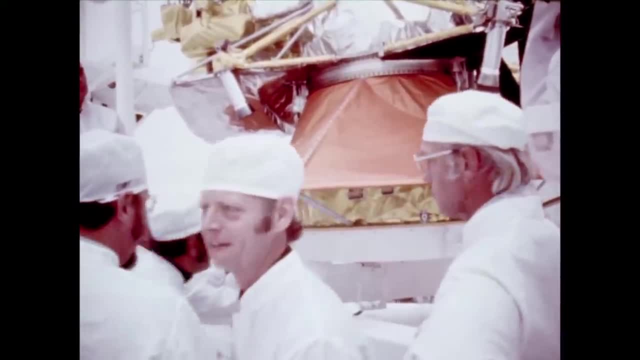 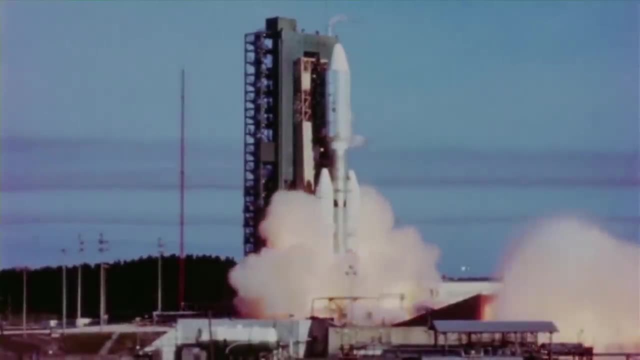 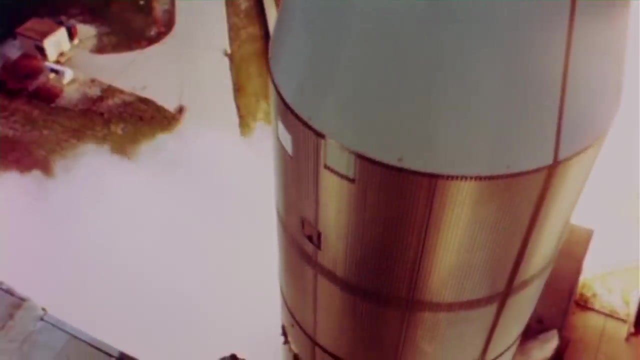 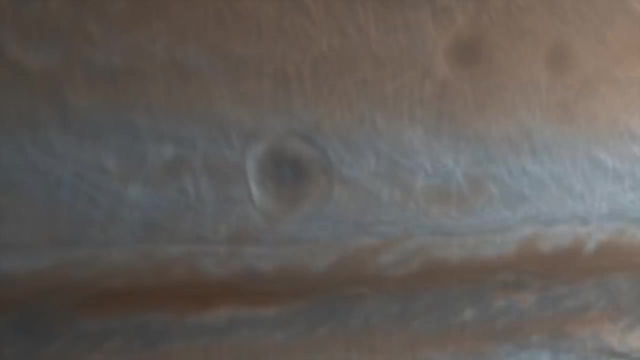 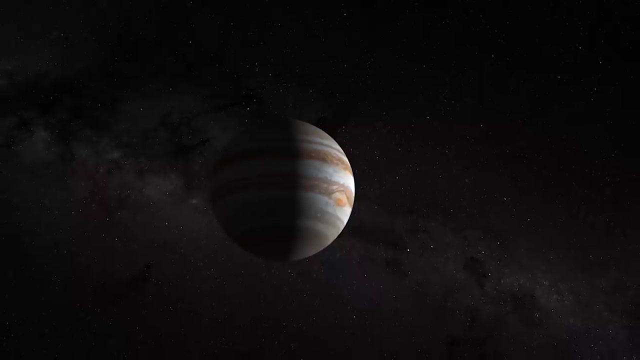 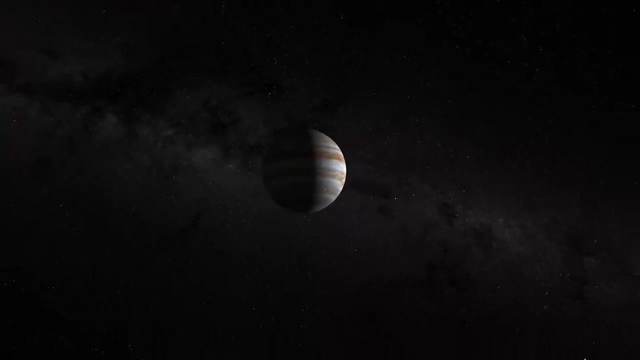 As the probe skimmed past the giant planet, it gained speed, Leaving Earth. Pioneer 10 was moving at 51,000 kilometers per hour. Departing Jupiter, it had more than doubled its speed. This gravitational slingshot effect made the Grand Tour possible. 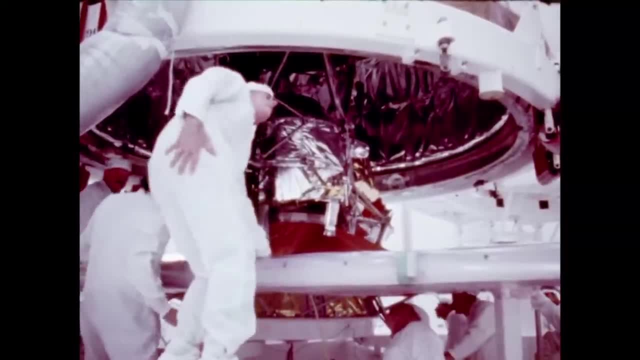 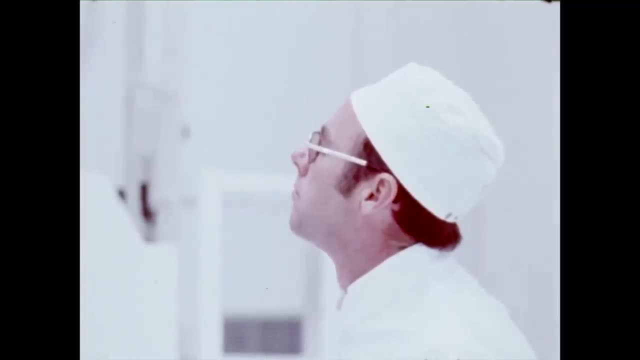 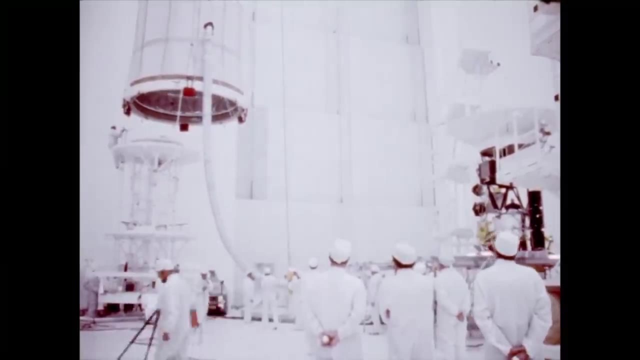 The Grand Tour craft recently renamed- Voyager 1 and 2, were due to be transferred to the Earth. It was also due to Cape Canaveral for launch integration when news of Jupiter's extreme radiation environment came through. The electron radiation at Jupiter had generated false commands within Pioneer 10.. 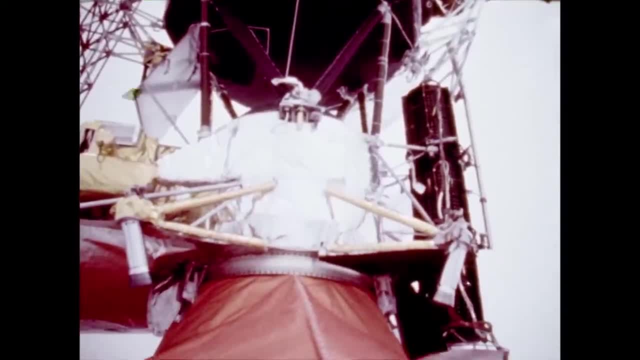 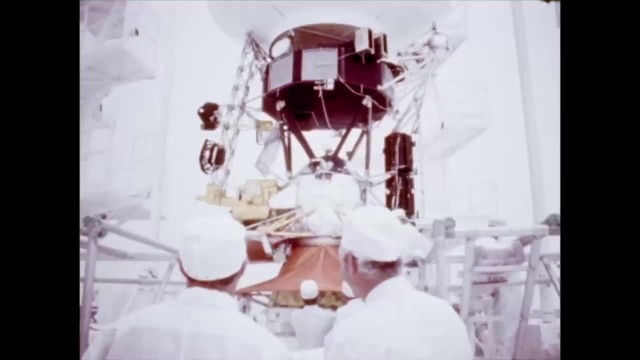 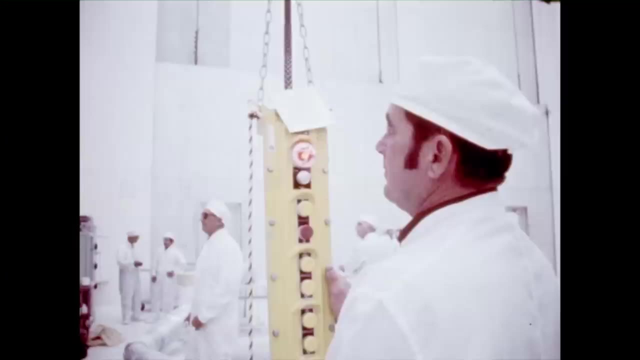 With the far more sophisticated Voyagers. this presented problems. Local supermarkets were stripped of their stocks of kitchen-grade aluminum foil, which was then used to shield critical cables. Without this last-minute alteration, electrical pressures of up to 40,000 volts would have been induced in the Voyager's subsystems as the craft passed. 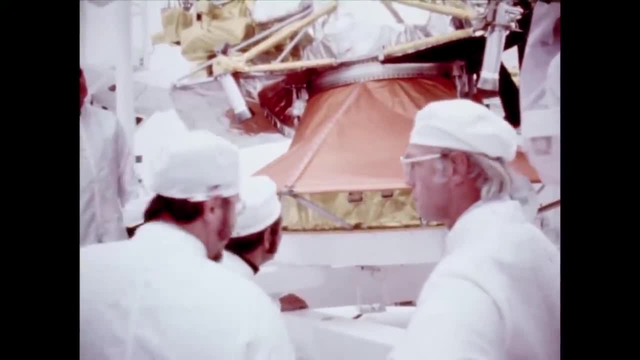 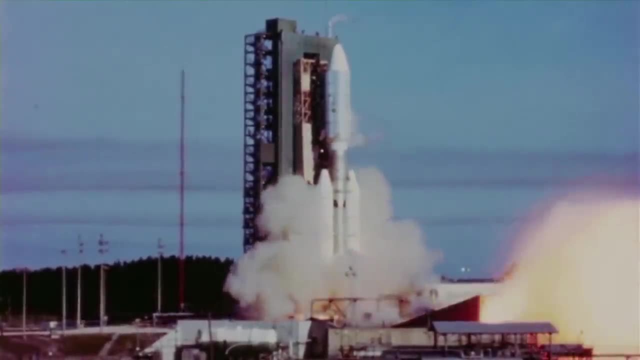 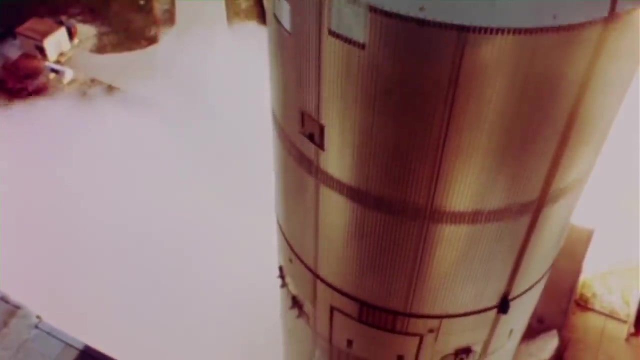 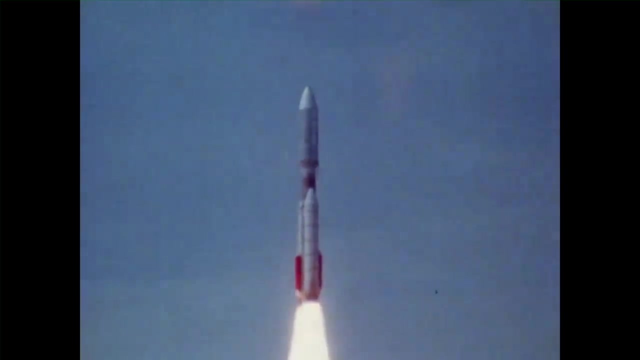 Jupiter Voyager 2 was launched in August 1977.. Its trajectory meant that it could visit Jupiter, Saturn, Uranus and Neptune. Voyager 1 left 16 days later. Its different, faster trajectory only allowed flybys of Jupiter and Saturn and various 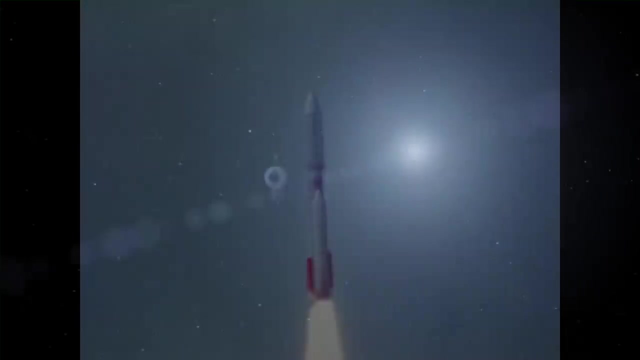 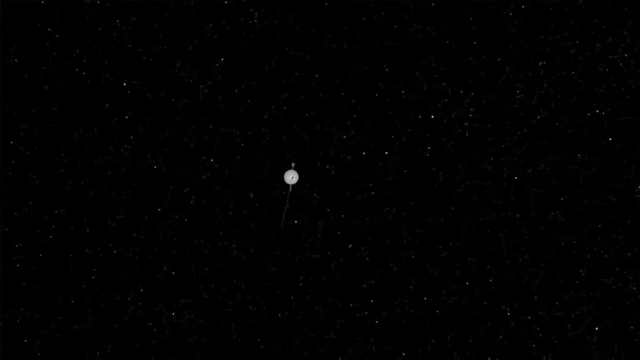 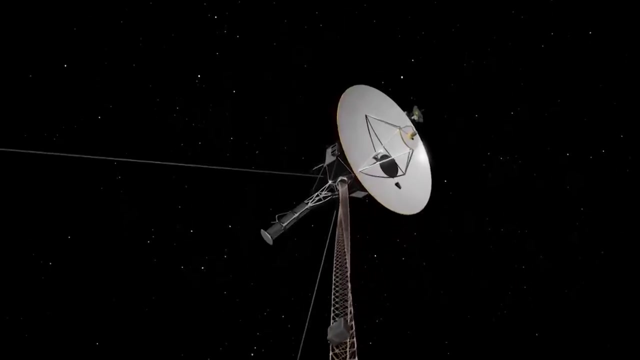 large moons. At the time, the Voyager spacecraft were the most sophisticated probes to be launched, Because they were to operate at huge distances from the Sun. solar panels could not be used as a power source. They were equipped with radioisotope thermoelectric generators, which used the heat from the decay. 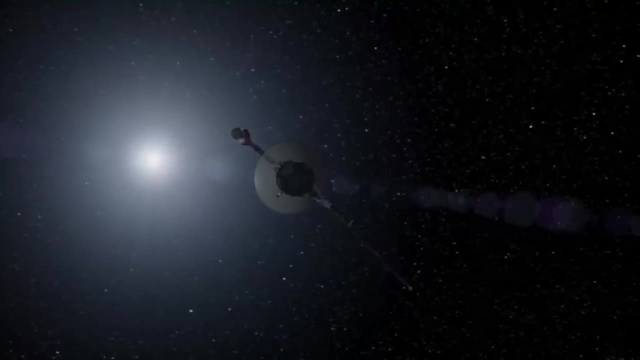 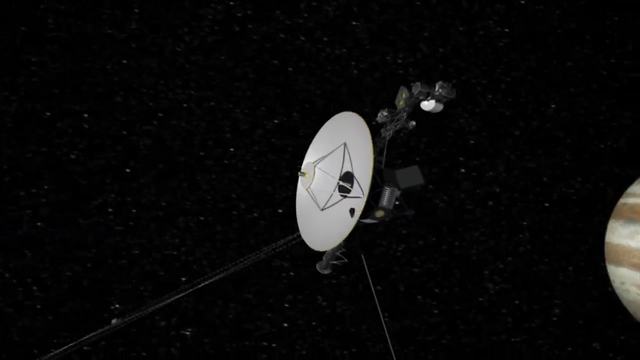 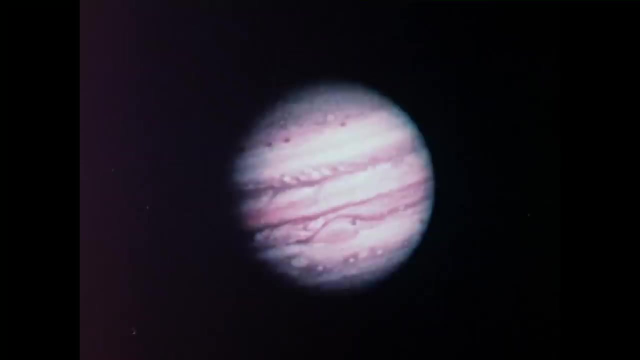 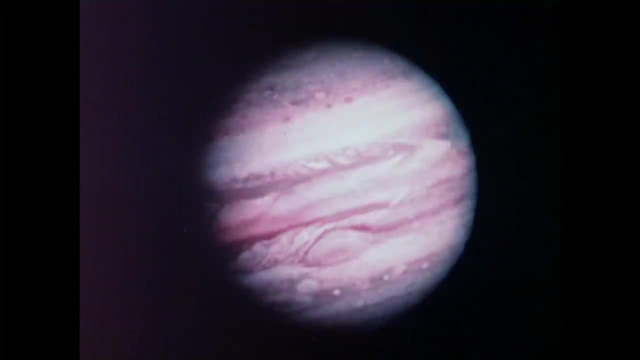 of plutonium-238.. As Voyager 1 approached Jupiter in January 1979, it began sending image sequences that showed a complex and dynamic planet. The planet's giant red spot was revealed as a vast rotating storm. In 1665,, Giovanni Cassini described a permanent spot on Jupiter which was 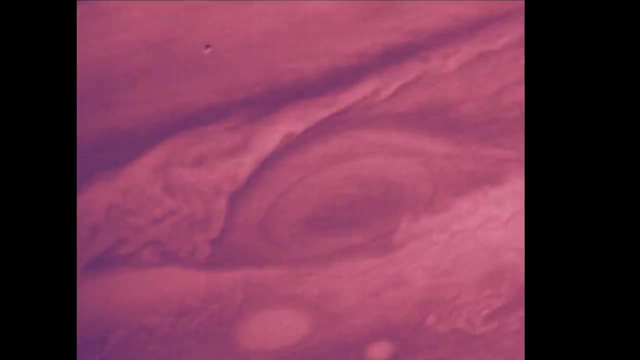 according to him, an extremely red spot. The red spot was the first stone which was regularly observed into the 1700s, But it was not until the late 1800s that Jupiter's spot was described as red. It was not until the late 1800s that the red spot was described as a red spot. 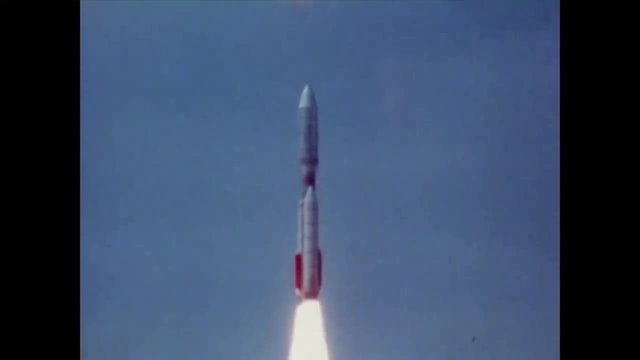 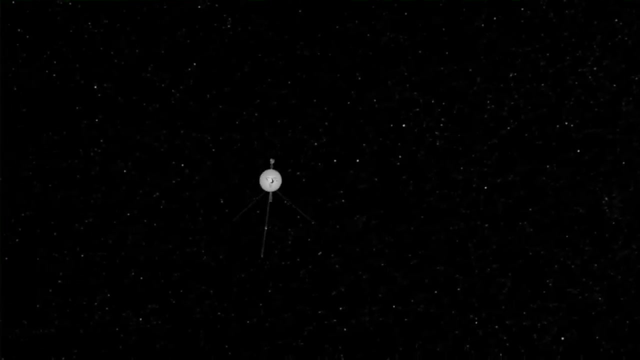 voyager 1 left 16 days later. its different, faster trajectory only allowed flybys of jupiter and saturn and various large moons. at the time, the voyager spacecraft were the most sophisticated probes to be launched because they were to operate at huge distances from the sun. solar panels could not be. 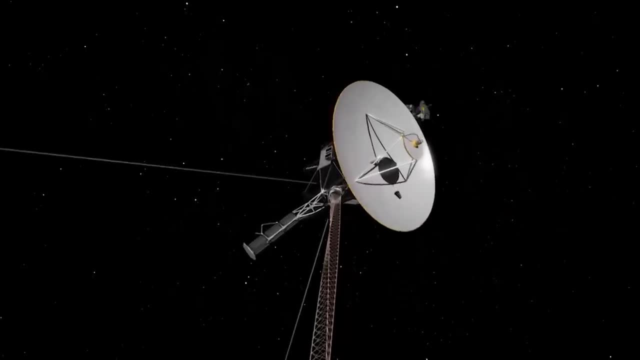 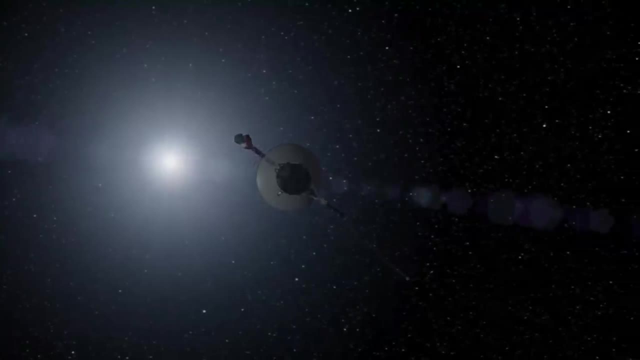 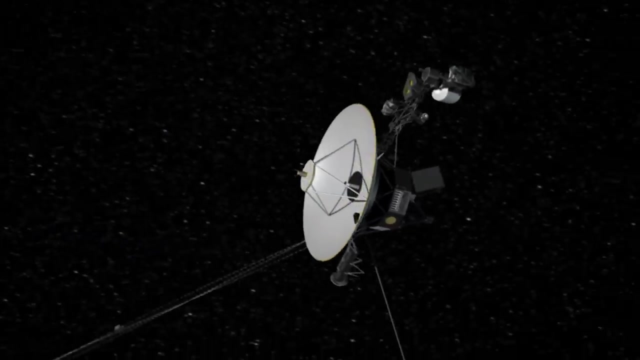 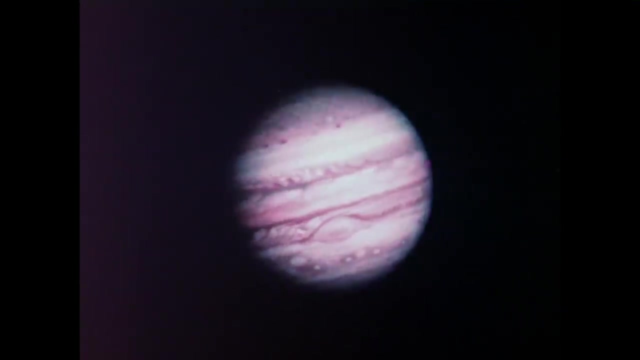 used as a power source. they were equipped with radioisotope thermoelectric generators, which use the heat from the decay of plutonium-238 to generate power. as voyager 1 approached jupiter in january 1979, it began sending image sequences that showed a complex and dynamic planet. 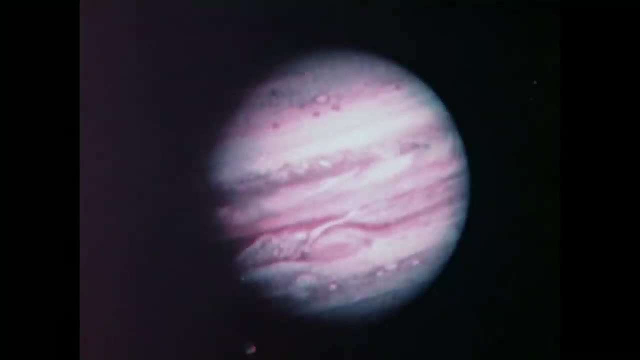 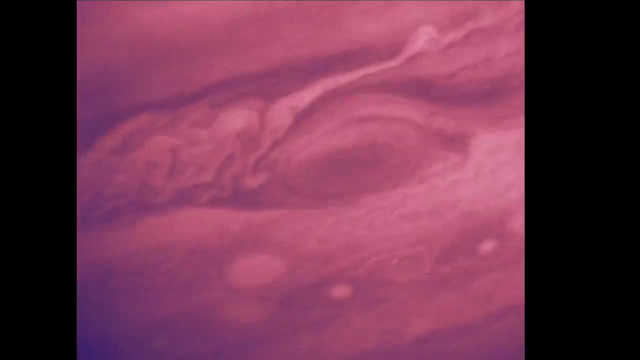 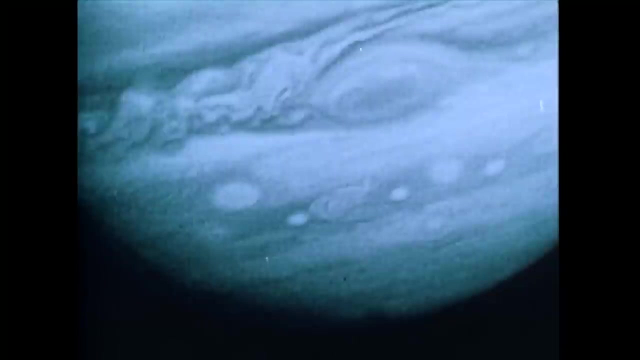 the planet's giant red spot was revealed as a vast rotating storm. in 1665, giovanni cassini described a permanent spot on jupiter which was regularly observed into the 1700s. it was not until the late 1800s that jupiter's spot was described as red. 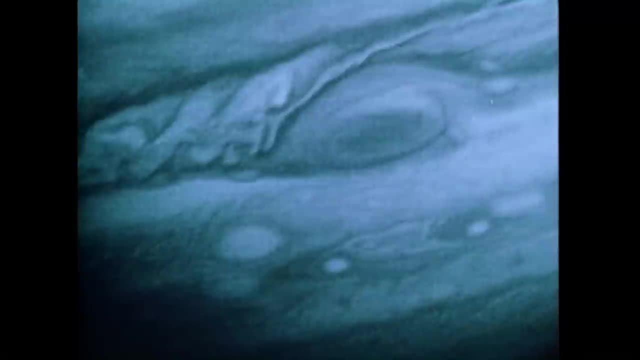 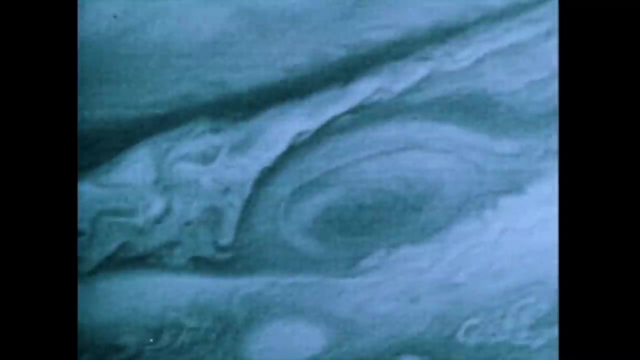 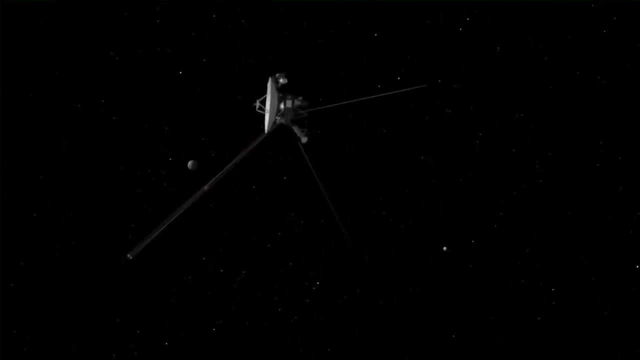 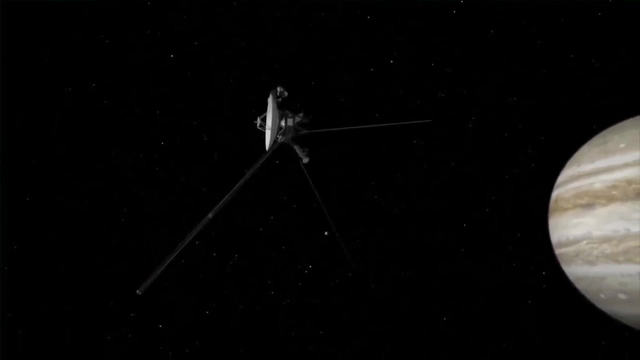 and it's uncertain whether the historic observations of jupiter's spot refer to the same feature or a phenomenon that regularly manifests in jupiter's atmosphere. voyager 1 made its closest approach early in march 1979. as the probe near jupiter, the activity at nasa's jet propulsion laboratory became. 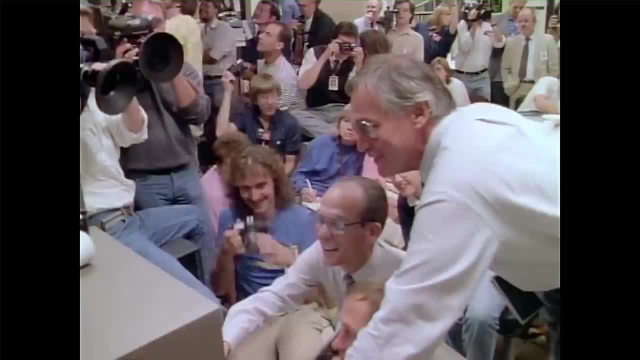 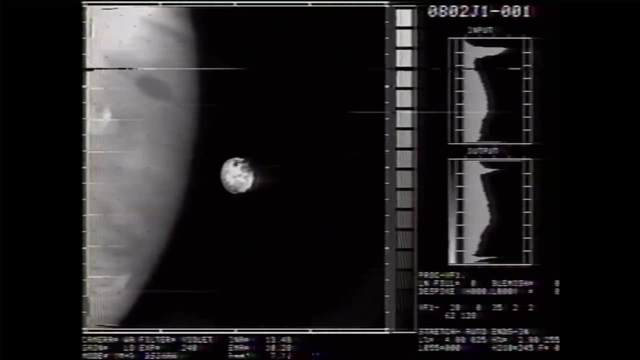 intense. this was the nature of the voyager's flyby missions. there were long, quiet cruise phases between the planets, followed by brief periods when the flow of information from the craft overwhelmed researchers. voyager 1 was one of the biggest contributors to the jupiter project. 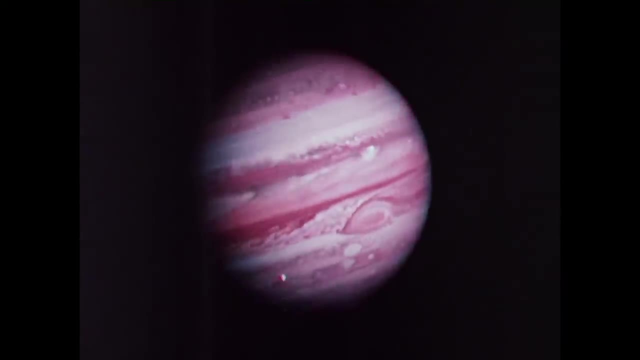 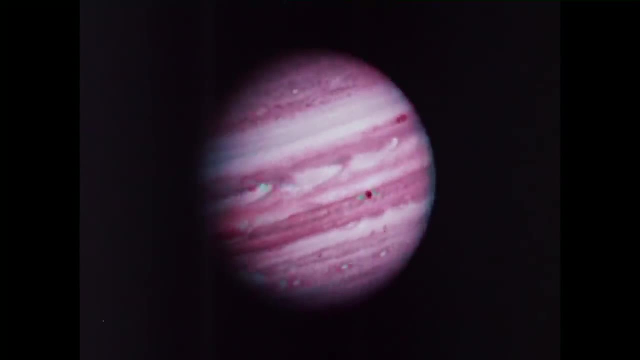 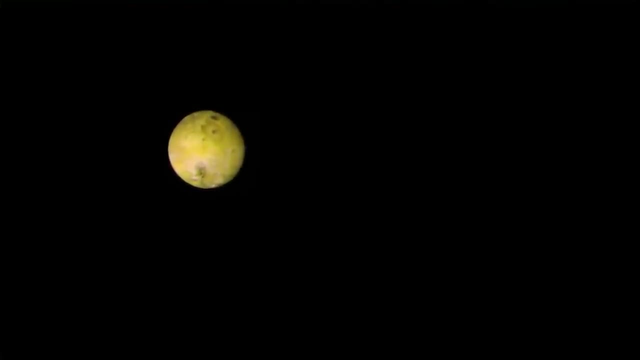 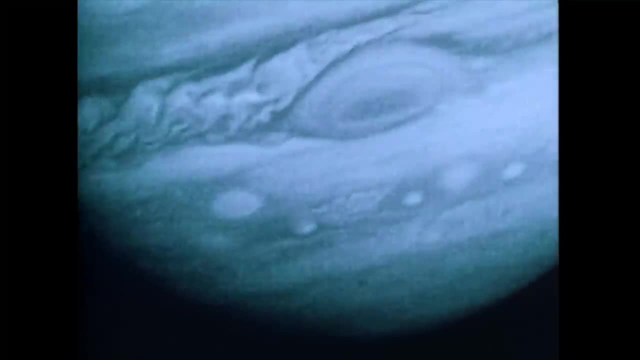 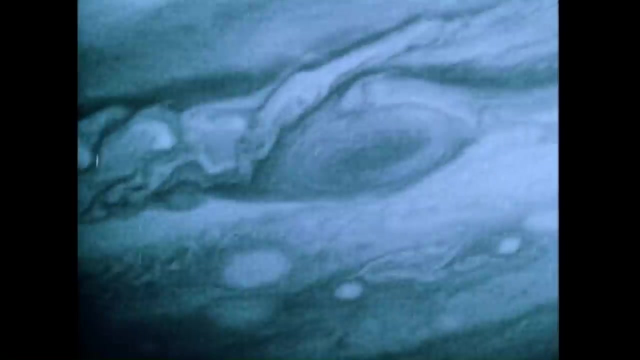 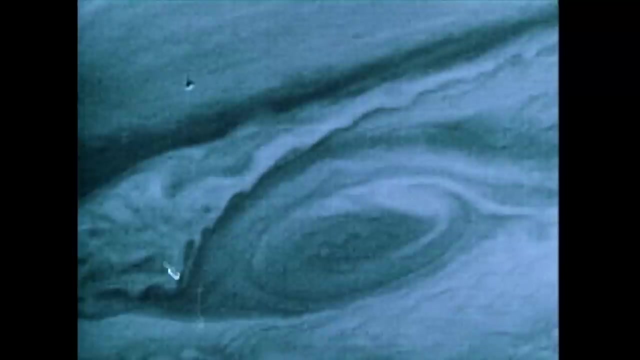 It was not until the late 1800s that the red spot was described as red, And it's uncertain whether the historical observations of Jupiter's spot refer to the same feature or a phenomenon that regularly manifests in Jupiter's atmosphere. Voyager 1 made its closest approach early in March 1979.. 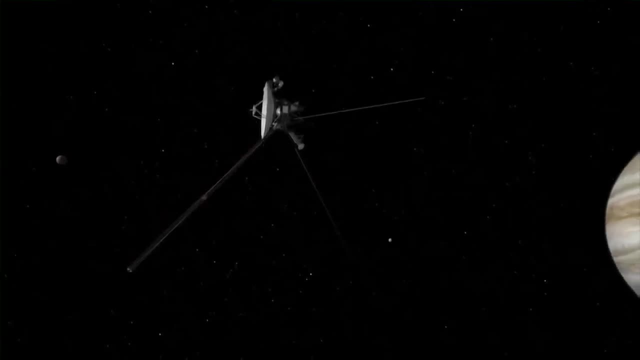 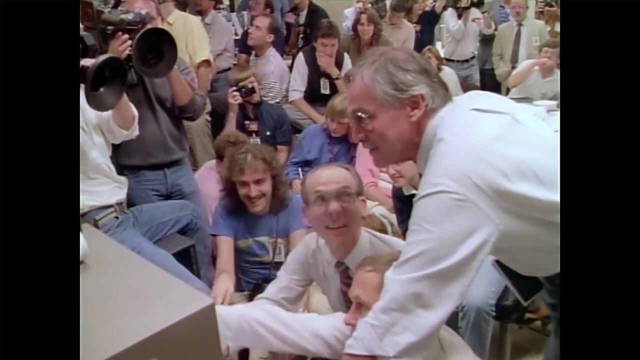 It was launched in September 1979.. It was launched in February 1979.. It was launched in February 1979.. It was launched in February 1979.. As the probe neared Jupiter, the activity at NASA's Jet Propulsion Laboratory became intense. 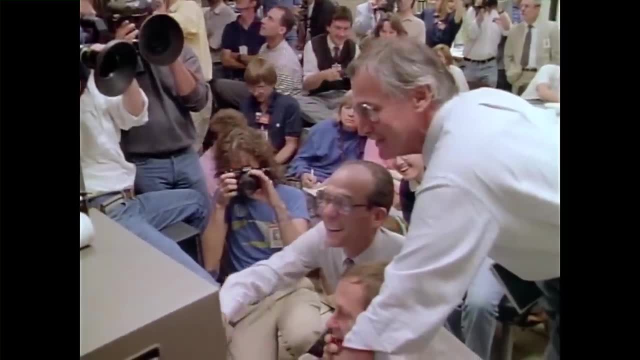 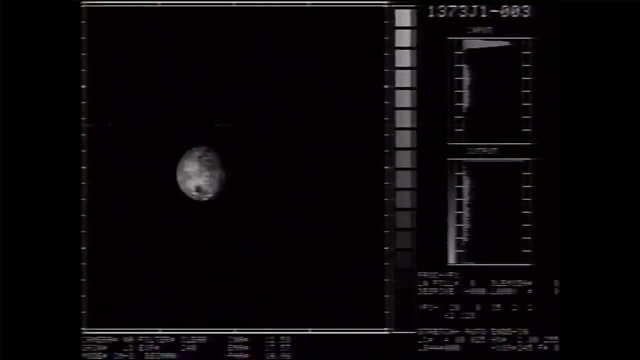 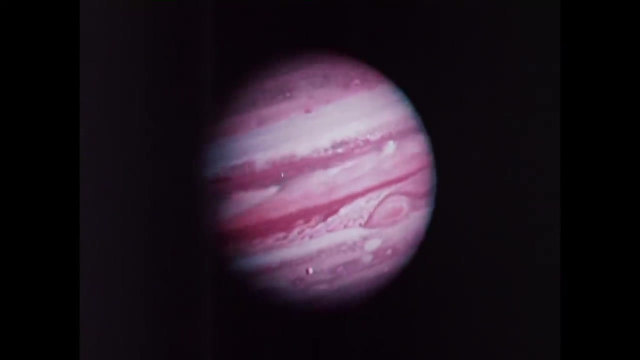 This was the nature of the Voyager's flyby missions. There were long, quiet cruise phases between the planets, followed by brief periods when the flow of information from the craft overwhelmed researchers. One of the biggest contributions made by the Voyagers was the transformation in our understanding of the Galilean moons. 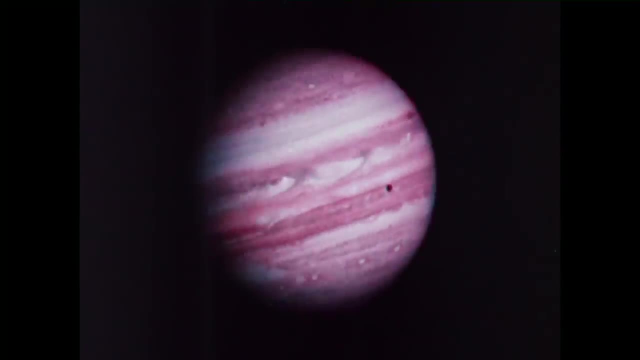 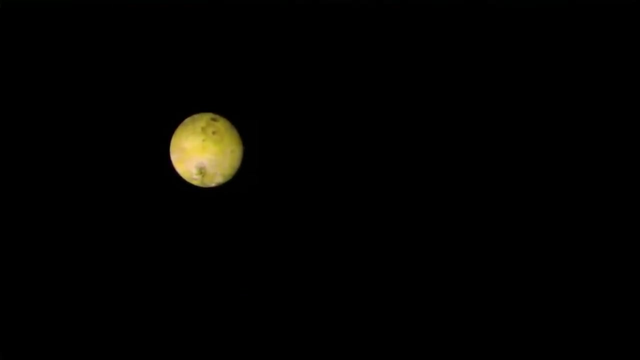 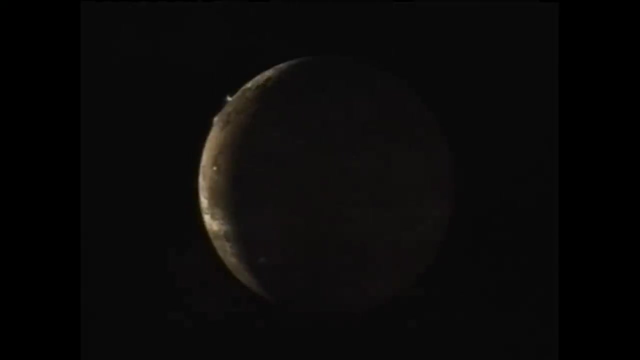 Previously just dots of light. Jupiter's four largest moons were each distinct and completely different. The first surprise was the inner moon, Io. It's a sulphurous yellow in appearance, and one particular long-duration exposure revealed an odd plume. Rather than being a cold dead world. 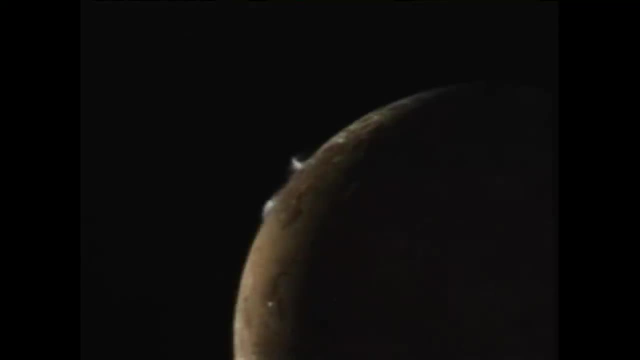 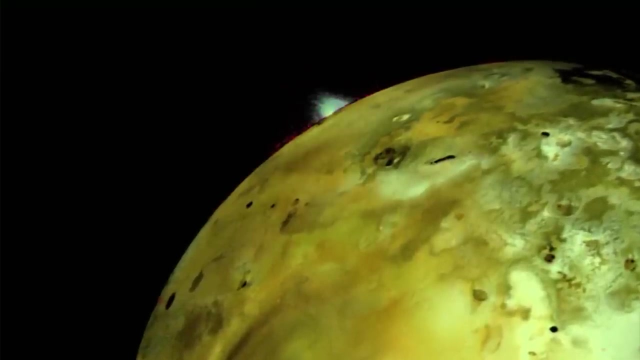 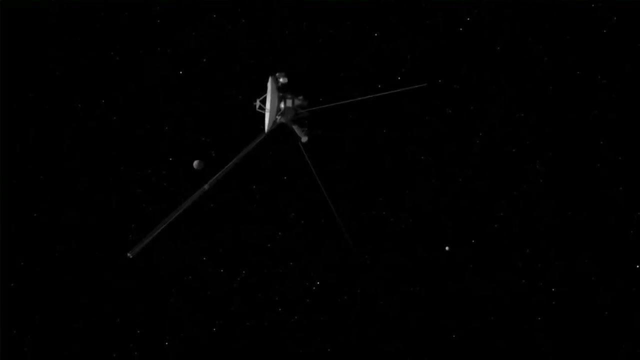 the gravitational squeezing which Io receives from its giant neighbour heats the moon's interior. The plume was a volcanic eruption ejecting material hundreds of kilometres above the surface In July 1979, three months after Voyager 1 had moved beyond Jupiter. 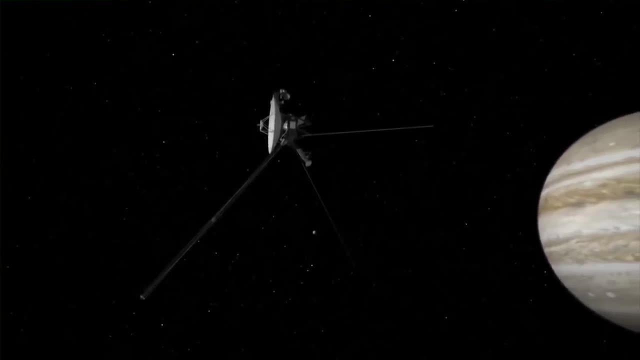 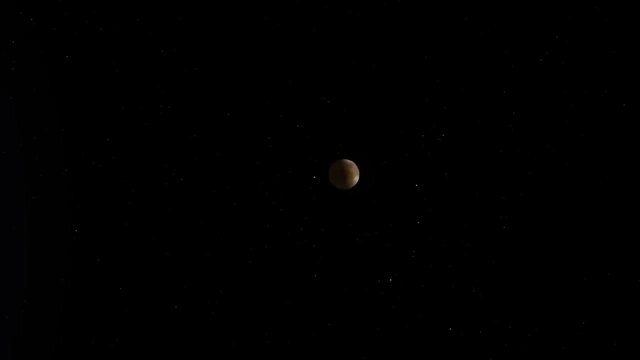 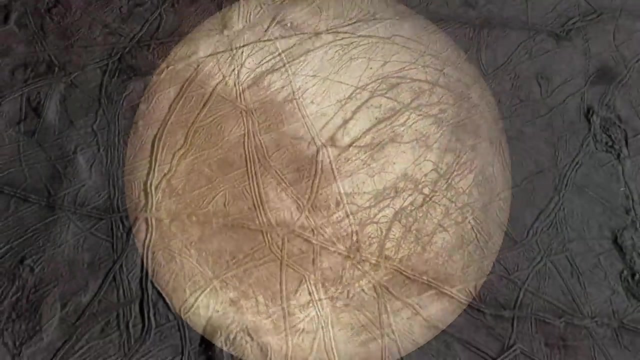 Voyager 2 made its closest approach. It was able to examine different moons more closely than its twin. Europa was the next surprise. It is highly reflective and has the smoothest surface of any body in the solar system. Further observation revealed pressure ridges reminiscent of polar ice flows on Earth. 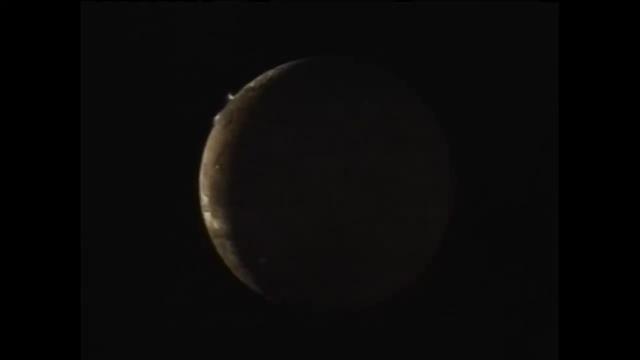 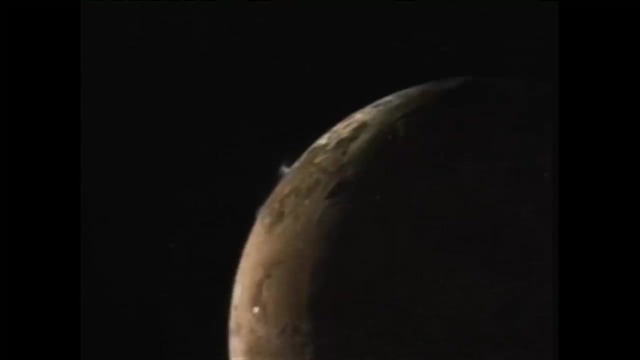 voyager 1 was one of the biggest contributors to the jupiter project. voyager 1 was one of the biggest contributors to the jupiter project. rather than being a cold dead world, the gravitational squeezing IO receives from its giant neighbor heats the moon's interior. the plume was a volcanic. 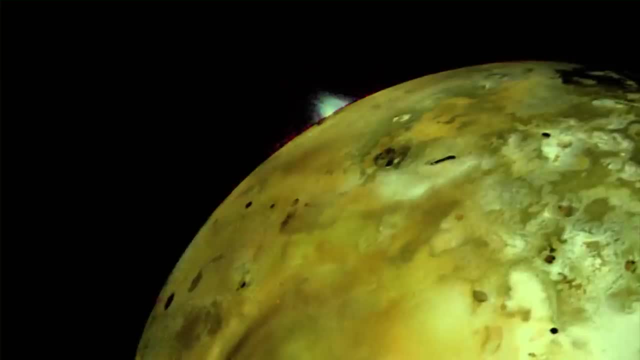 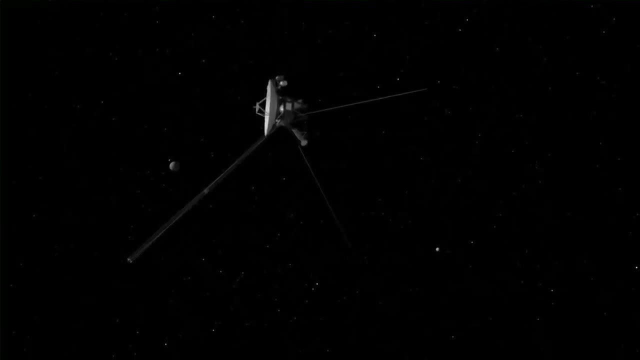 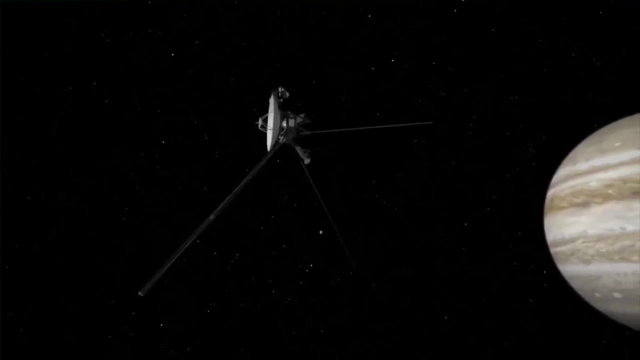 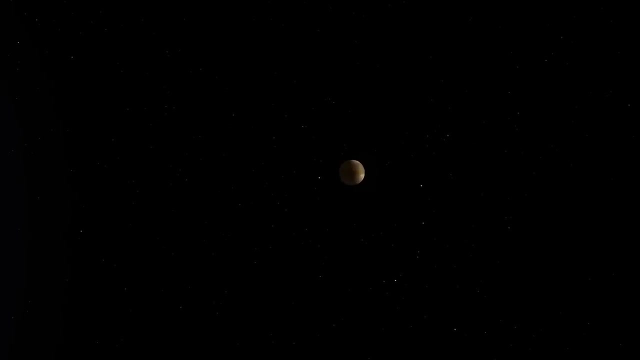 eruption ejecting material hundreds of kilometers above the surface. in July 1979, three months after Voyager 1 had moved beyond Jupiter, Voyager 2 made its closest approach. it was able to examine different moons more closely than its twin. Europa was the next surprise. it is highly reflective and has the smoothest 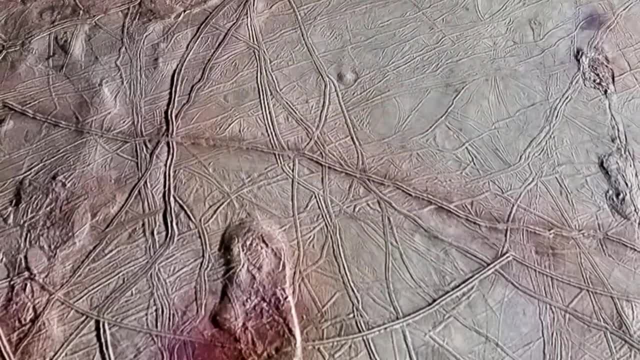 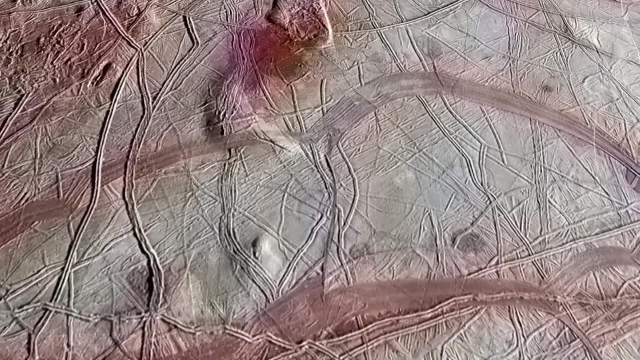 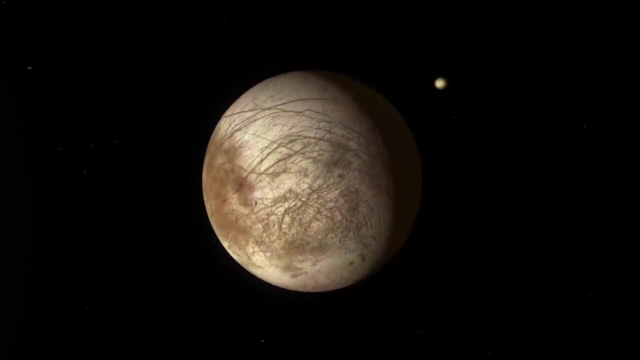 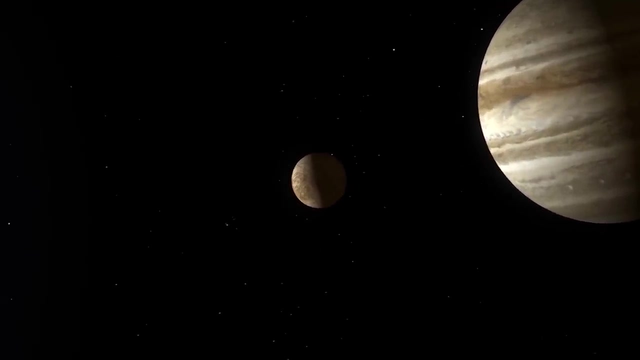 surface of any body in the solar system. further observation revealed pressure ridges reminiscent of polar ice flows on Earth. you, Europa, is a frozen world with a vast ocean beneath a thick crust of ice. like IO, it is heated from within by tidal flexing as Voyager 2 continued towards. 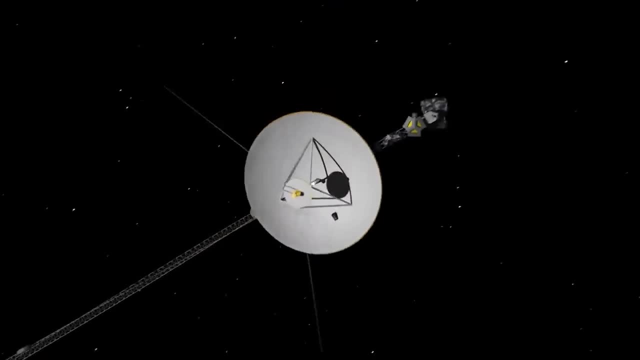 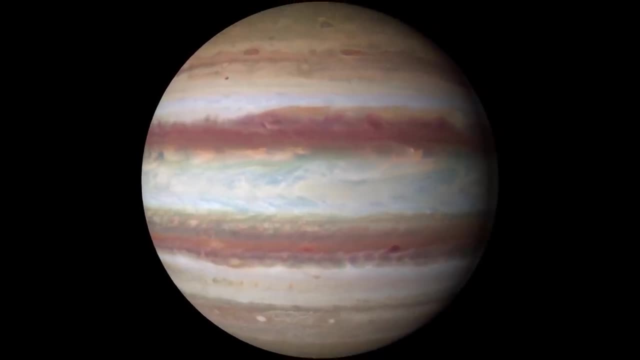 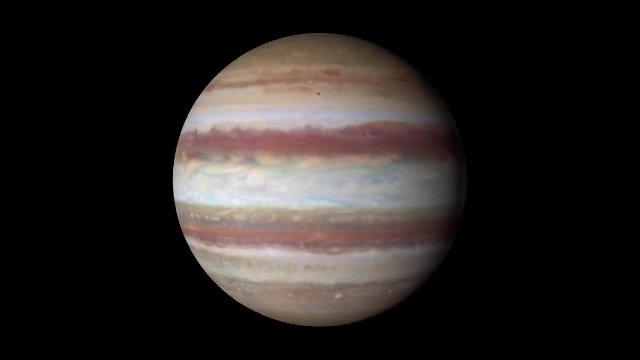 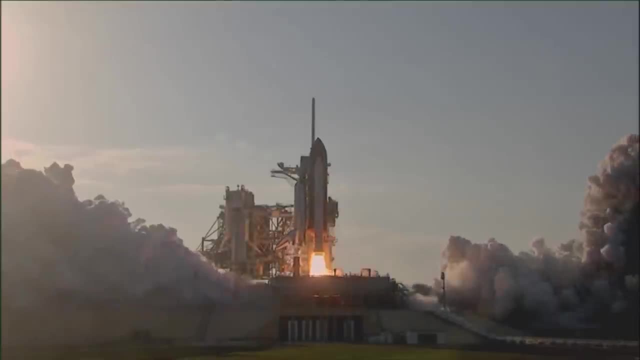 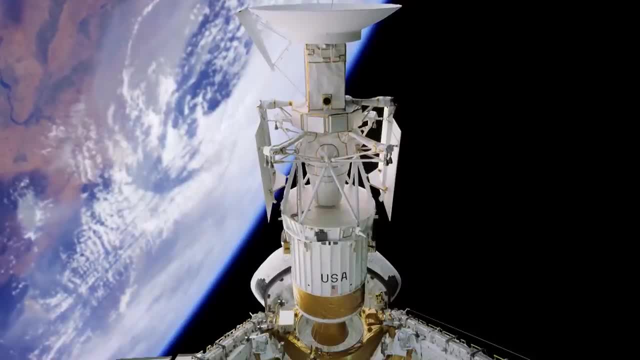 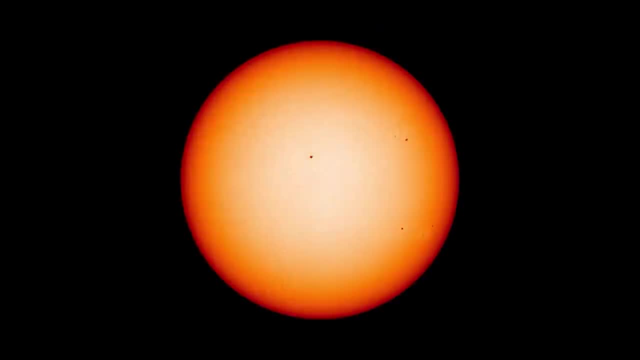 In October 1990, the space shuttle Discovery lifted the European Ulysses spacecraft to low Earth orbit. From there it was boosted on a mission to observe the Sun, but first it would pass Jupiter. All the planets orbit the Sun in the same direction. 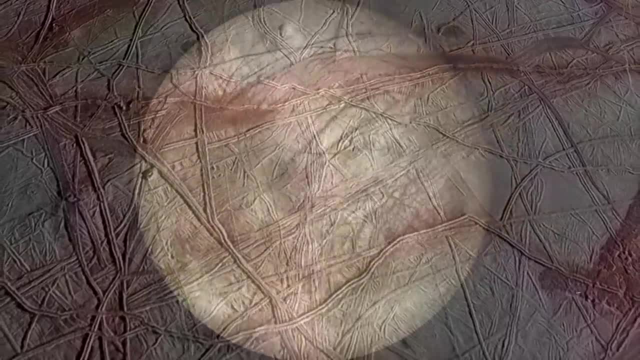 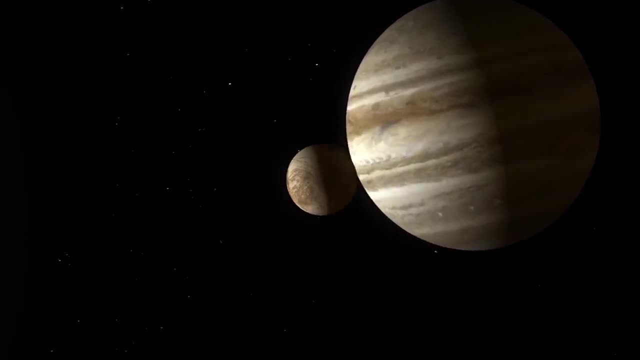 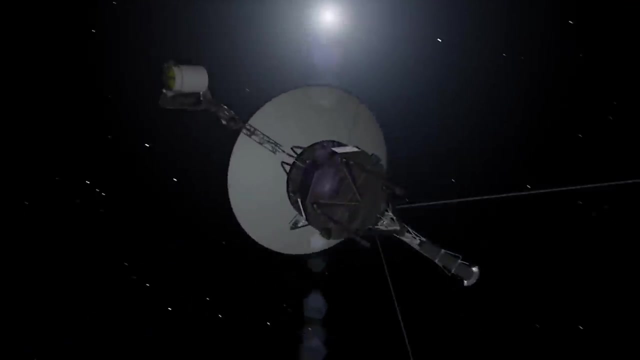 Europa is a frozen world with a vast ocean beneath a thick crust of ice. Like Io, it is heated from within by tidal flexing. As Voyager 2 continued towards Saturn, planetary researchers were left with large amounts of raw data about Jupiter still to be processed. 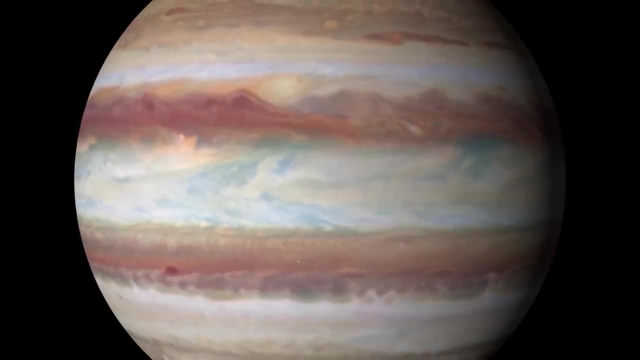 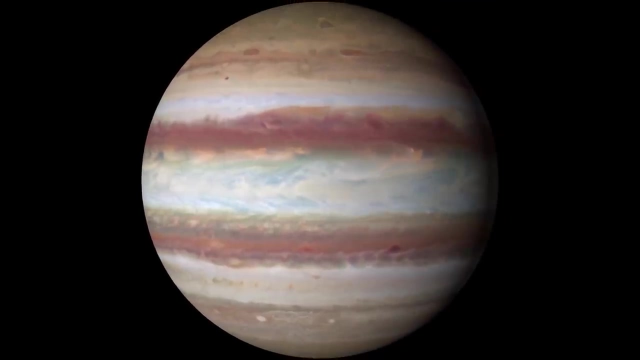 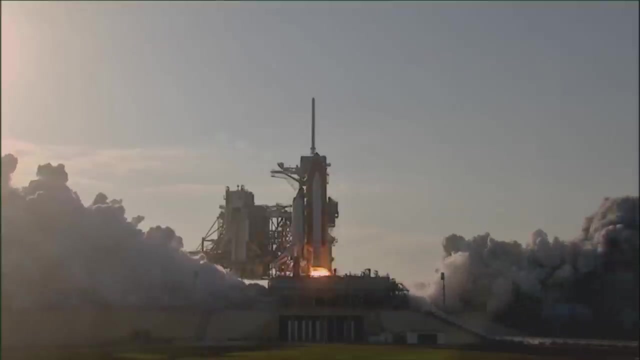 The Voyager missions left us with a basic view of the Jovian system, but they had raised more questions than they were able to answer. It would be more than ten years before Jupiter received another visitor from Earth Mission and liftoff of Discovery. 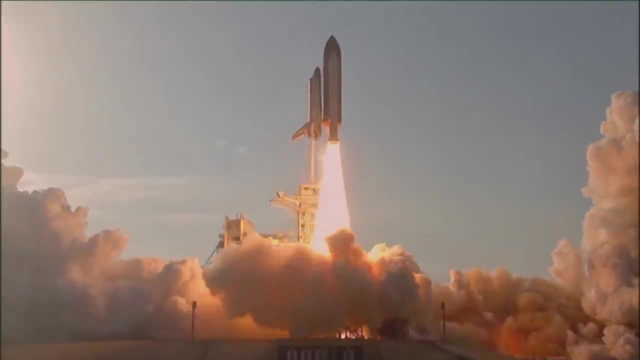 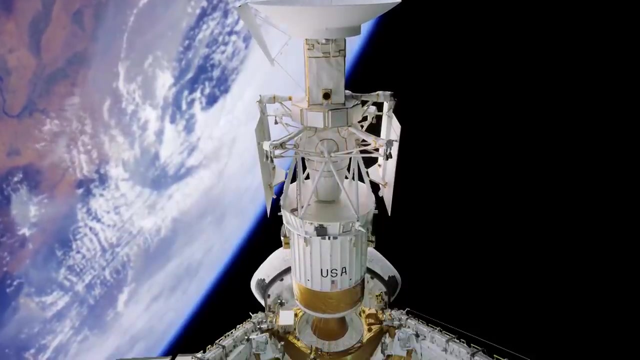 and the Ulysses spacecraft bound for the polar regions of the Sun. In October 1990, the Space Shuttle Discovery lifted the European Ulysses spacecraft to low Earth orbit. From there it was boosted on a mission to observe the Sun. 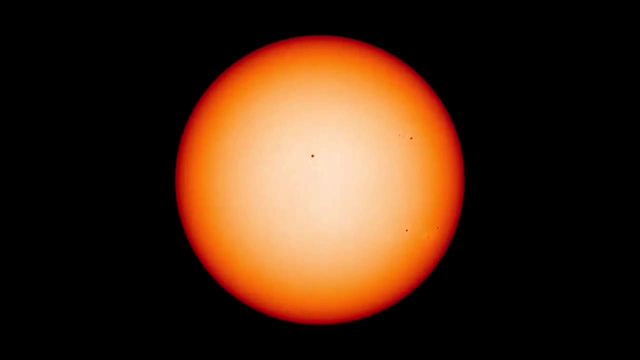 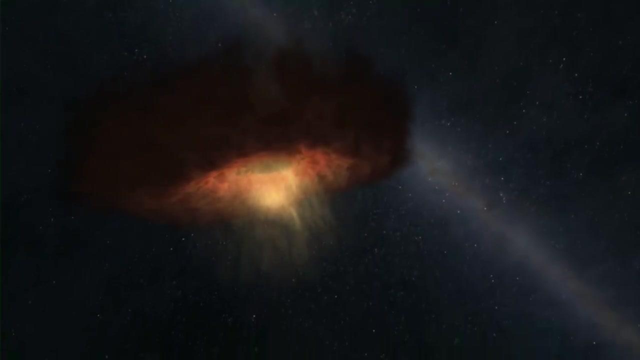 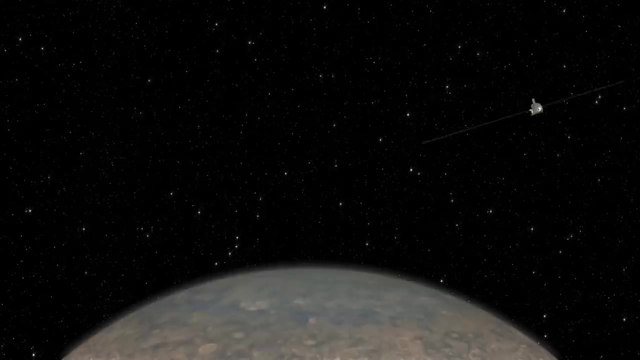 But first it would pass Jupiter. All the planets orbit the Sun in the same direction, in roughly the same plane. This is called the ecliptic, and it developed from the spinning disk of dust and gas that formed our solar system. The designers of the Ulysses spacecraft wanted to see the Sun from an orbit above its poles. 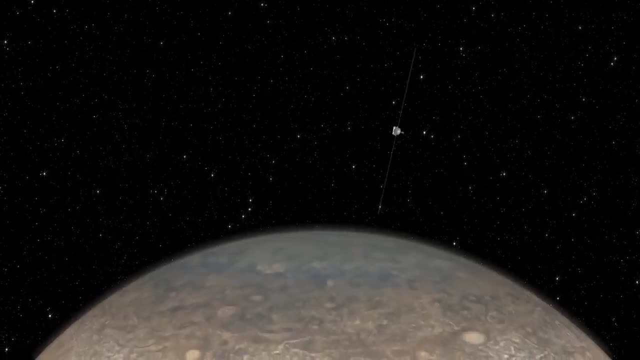 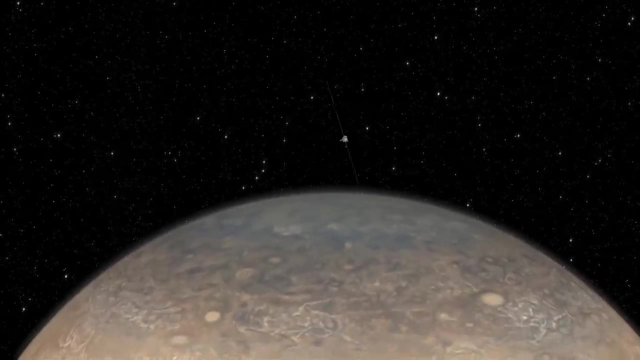 Jupiter's extreme gravitation was used to bend the probe's flight path out of the ecliptic so it could make north-south orbits of the Sun. The probe was also used to observe the Earth's orbit. Ulysses was not the only probe to take advantage of Jupiter's gravity. 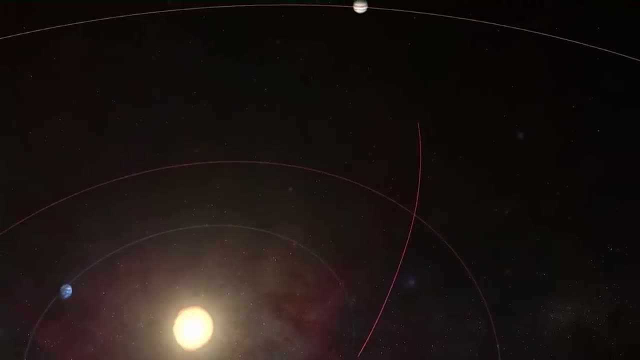 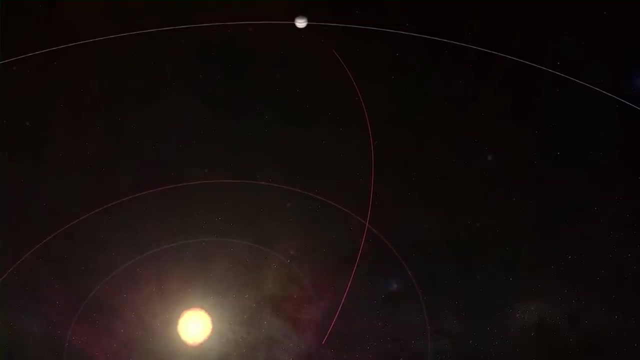 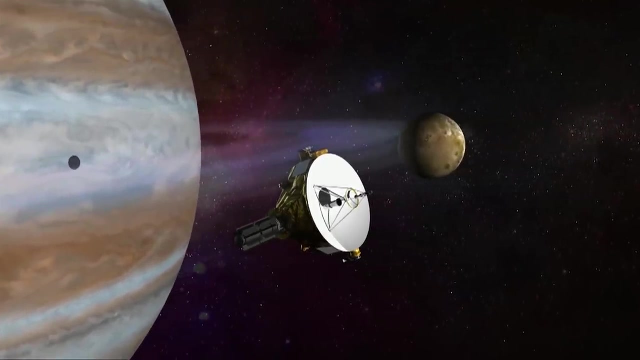 Both the Cassini probe to Saturn, launched in 1997,, and the New Horizons probe to Pluto, launched in 2006,, were able to reduce their flight times by years. with Jupiter flybys, These probes were able to make meaningful observations. 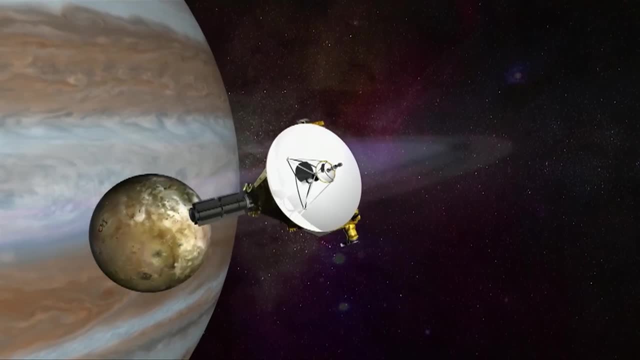 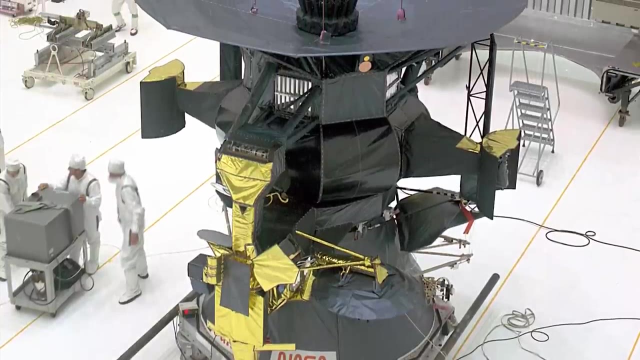 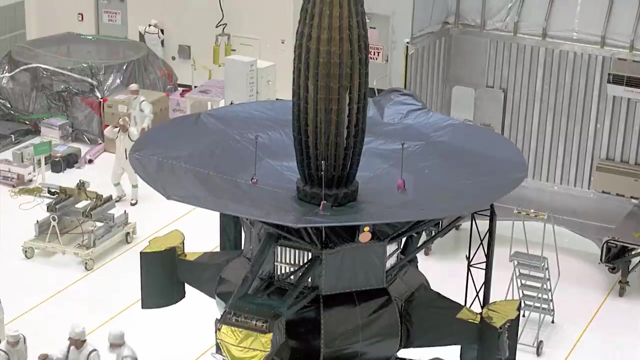 while passing the giant planet, In the clean rooms of the Jet Propulsion Laboratory, a new probe was taking shape. Galileo would be the first spacecraft to go into orbit around Jupiter. Its 4.8-metre antenna was folded like an umbrella. 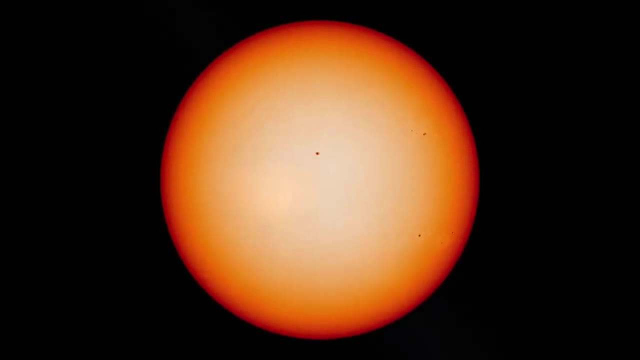 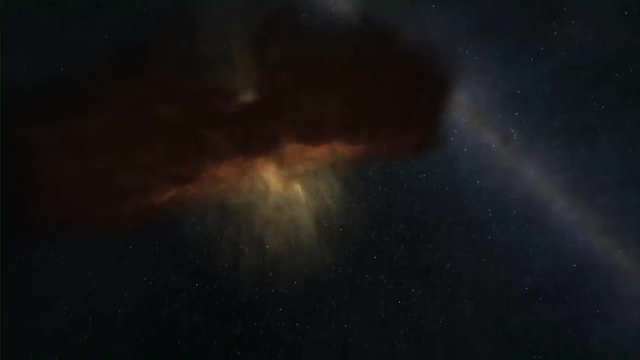 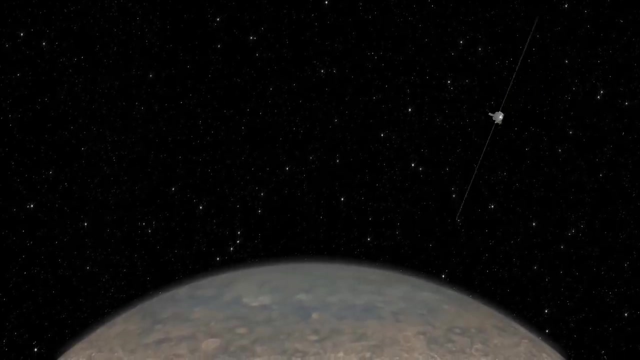 in roughly the same plane. This is called the ecliptic, and it developed from the spinning disk of dust and gas that formed our solar system. The designers of the Ulysses spacecraft wanted to see the Sun from an orbit above its poles. 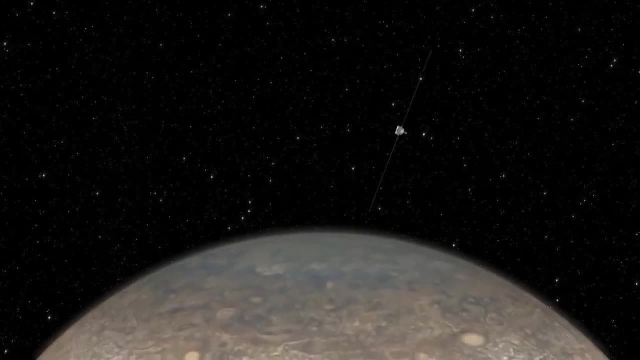 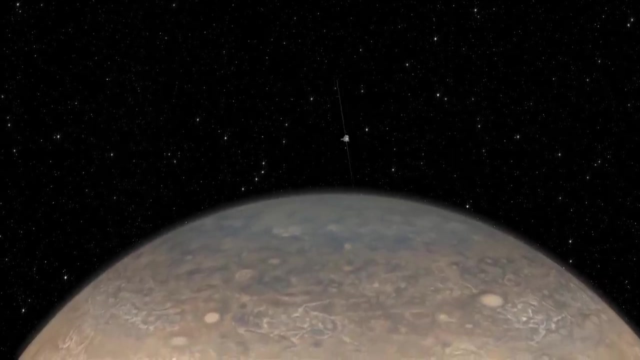 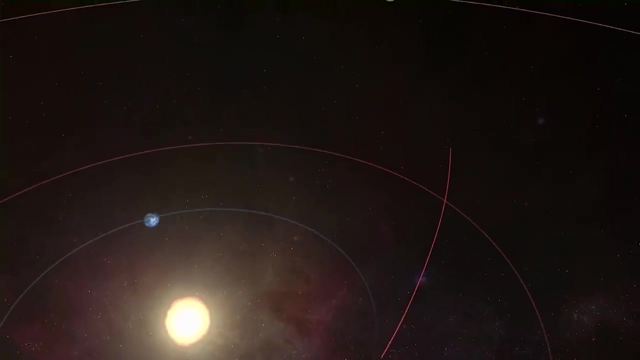 Jupiter's extreme gravitation was used to bend the probe's flight path out of the ecliptic so it could make north-south orbits of the Sun. Ulysses was not the only probe to take advantage of Jupiter's gravity. Both the Cassini probe to Saturn, launched in 1997,. 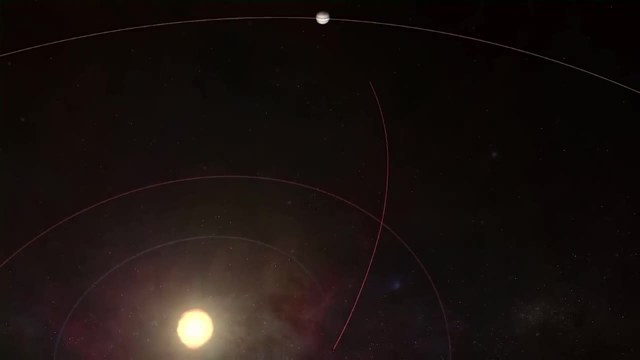 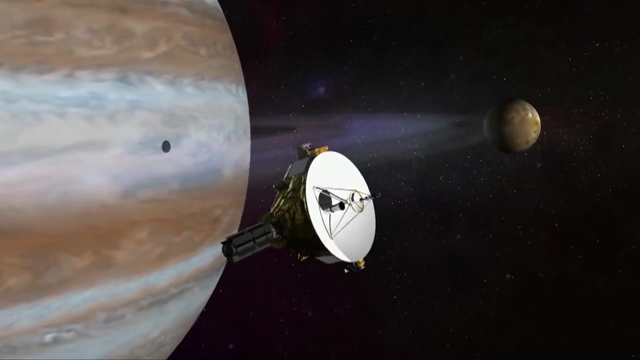 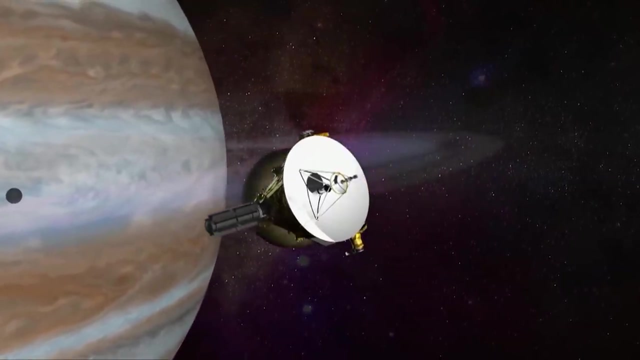 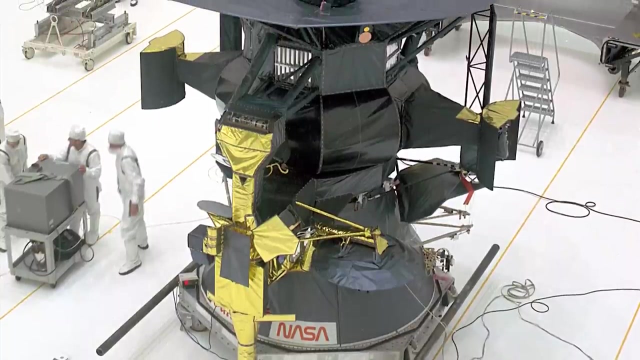 and the New Horizons probe to Pluto, launched in 2006,, were able to reduce their flight times by years. with Jupiter flybys, These probes were able to make meaningful observations while passing the giant planet In the clean rooms of the Jet Propulsion Laboratory. 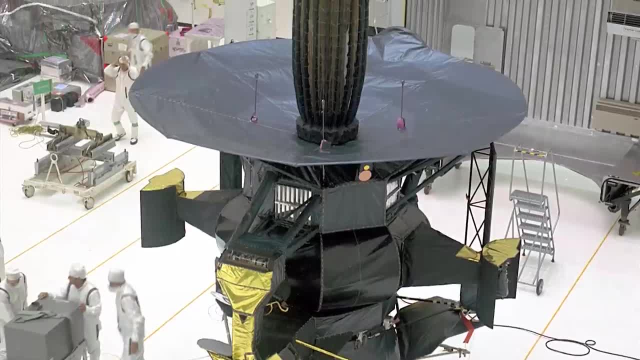 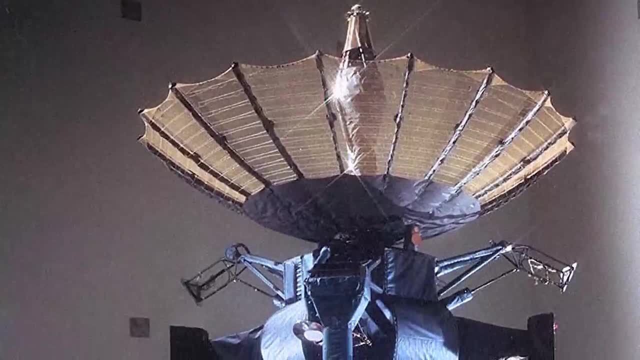 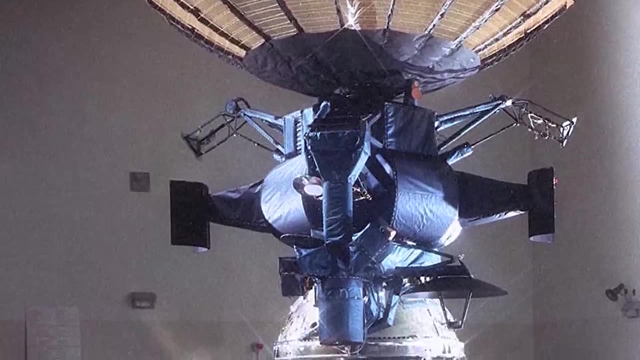 a new probe was taking shape. Galileo would be the first spacecraft to go into orbit around Jupiter. Its 4.8-metre antenna was folded like an umbrella, only to be deployed when safely on the way to Jupiter, Originally scheduled to launch in 1986,. 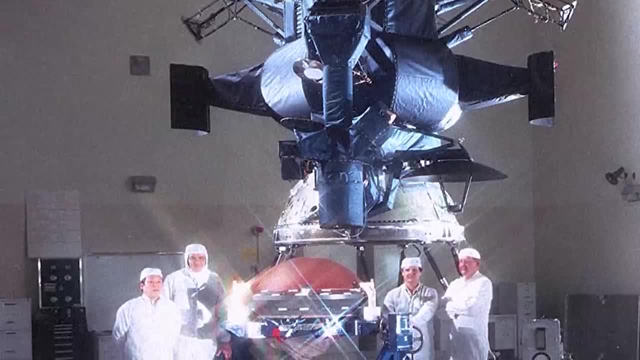 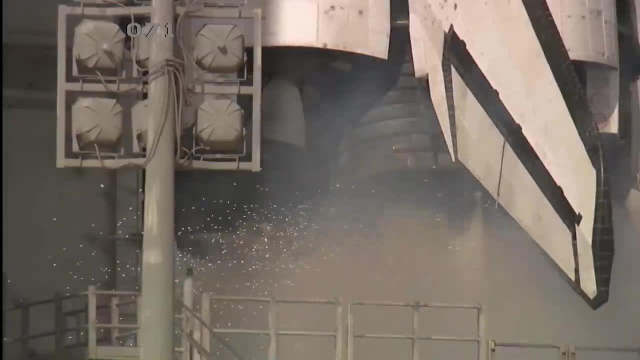 it sat in storage for years after the Space Shuttle Challenger exploded. The probe was launched on the Earth's surface in 2008.. It launched aboard Space Shuttle Atlantis in October 1989.. It launched aboard Space Shuttle Atlantis in October 1989. 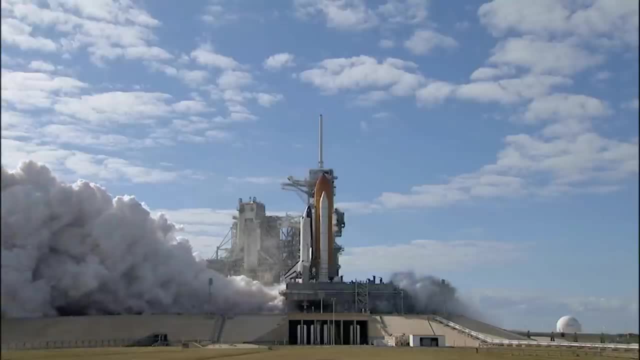 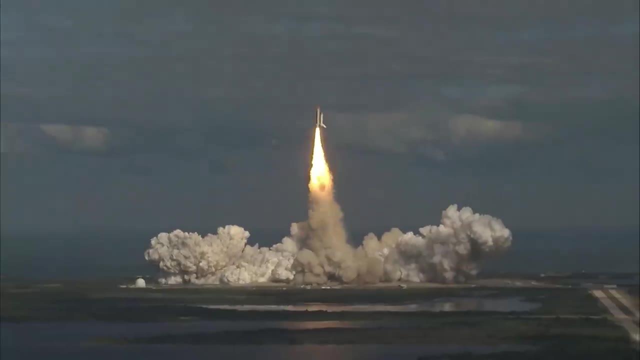 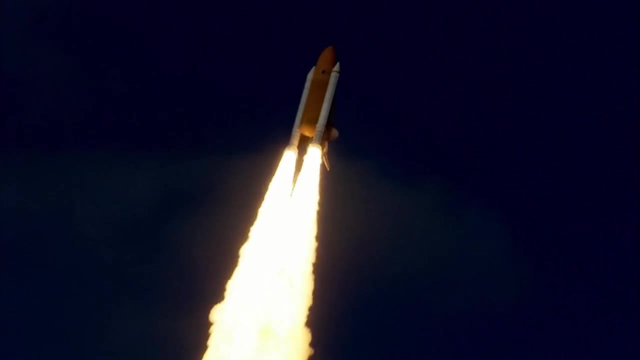 5, 4,, 3, 2, 1.. We have ignition and liftoff of Atlantis and the Galileo spacecraft bound for Jupiter. New rules governing shuttle launches meant a change in the booster to push Galileo out of Earth orbit. 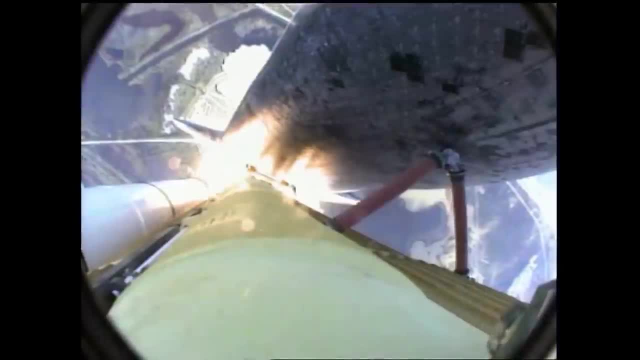 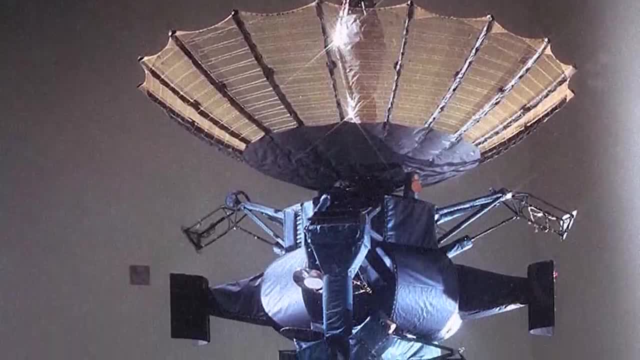 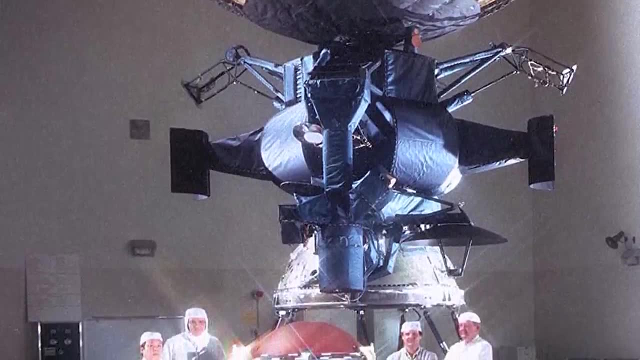 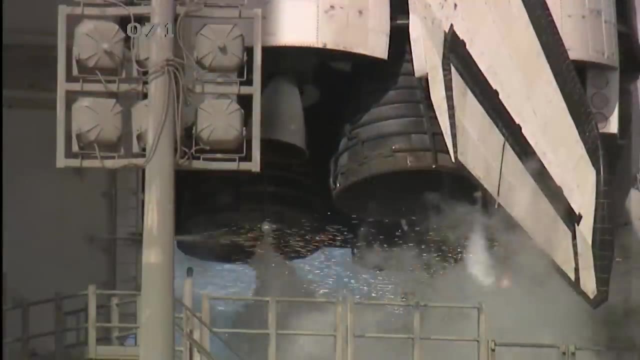 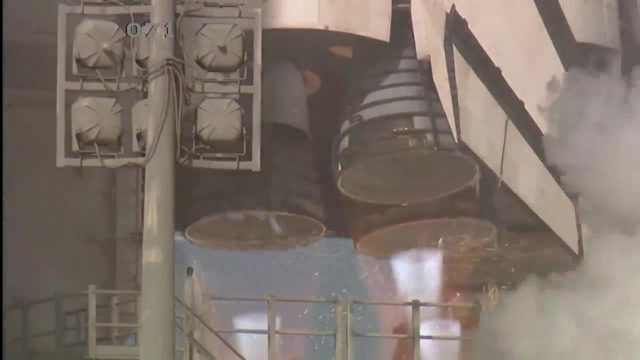 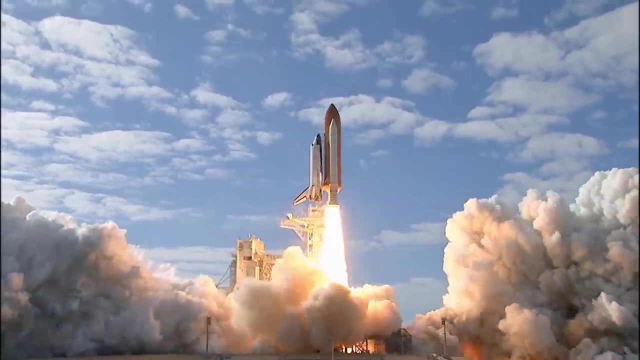 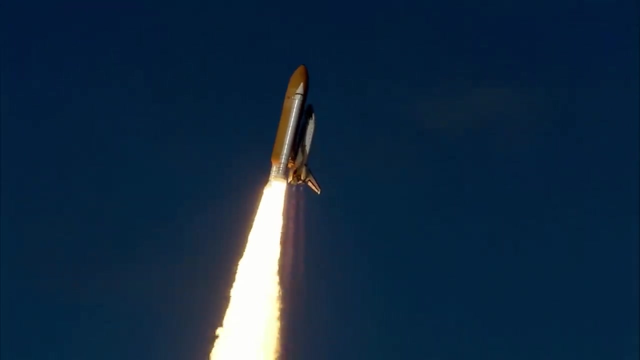 only to be deployed when safely on the way to Jupiter. Originally scheduled to launch in 1986, it sat in storage for years after the Space Shuttle Challenger exploded, It launched aboard Space Shuttle Atlantis in October 1989. New rules governing shuttle launches meant a change in the booster. 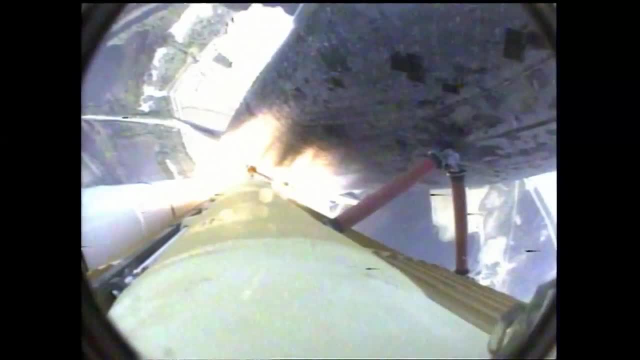 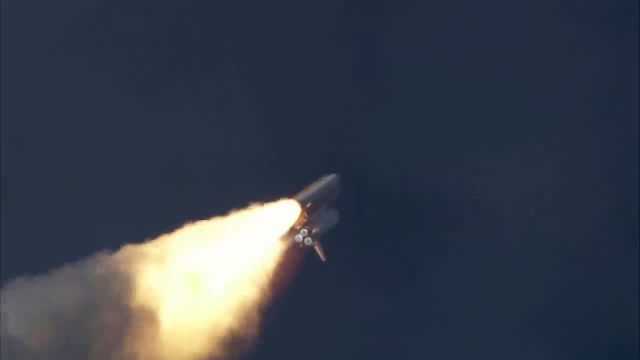 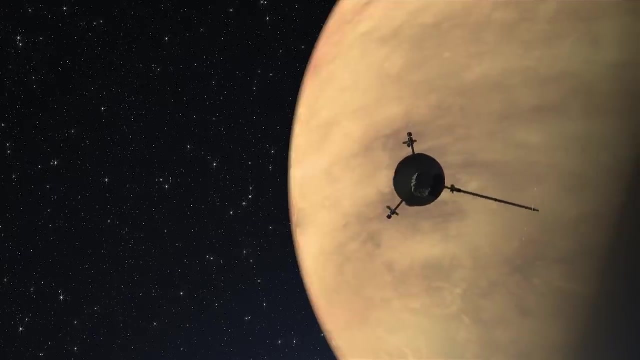 to push Galileo out of Earth orbit. The less powerful solid-fuel upper stage now stipulated sent Galileo toward Venus for a gravity assist. The new flight path meant Galileo was travelling to a hotter part of the Solar System. It was decided to keep the heat-sensitive antenna furled. 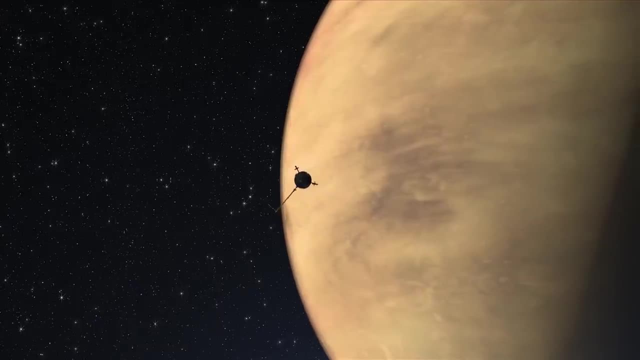 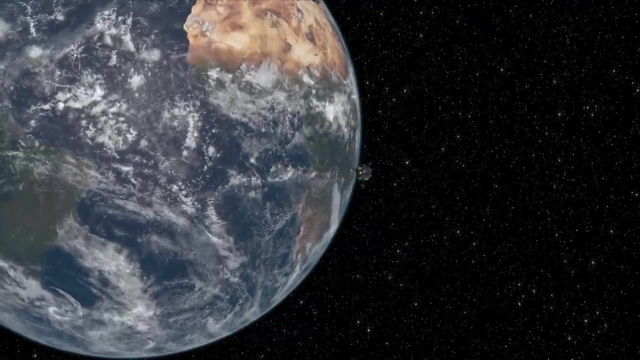 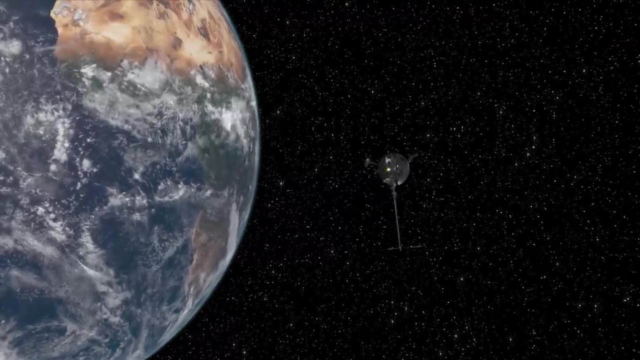 until after the spacecraft looped back past Earth. Galileo made two close passes of Earth orbit, each time gaining more speed. Its first pass was in December 1990, more than a year after its launch. A further year on when it passed Earth again, 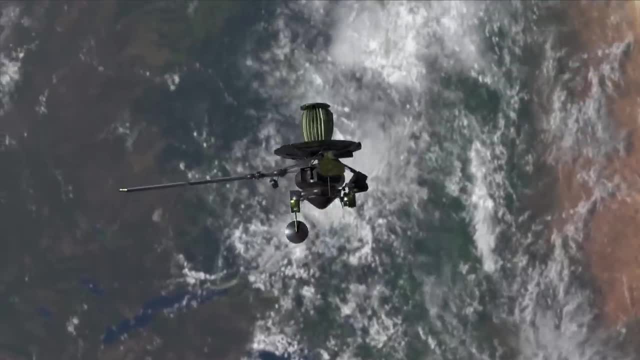 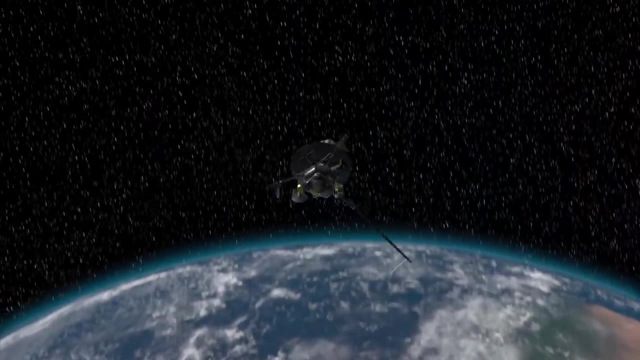 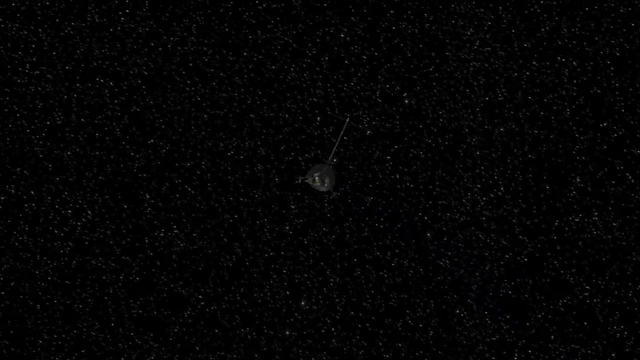 the high-gain antenna was only partially open. After months of trying different techniques to deploy the antenna mission, engineers concluded that long periods in storage had caused lubricant at the tips of the antenna's ribs. to dissipate, Researchers would rely on Galileo's smaller antenna. 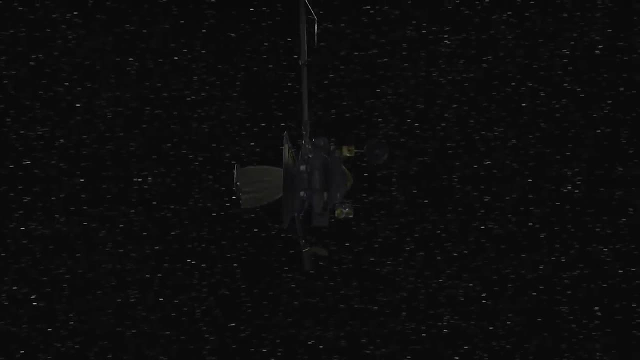 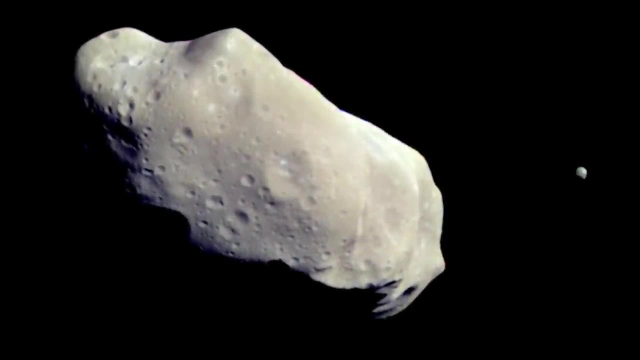 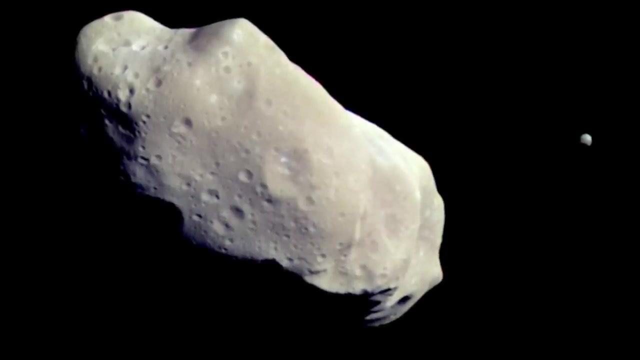 with data delivered at slower rates. During the cruise to Jupiter, Galileo encountered several asteroids. This is Ida, the first asteroid we've learnt of, with its own moon, Dactyl, In July 1995, while it was still six months away. 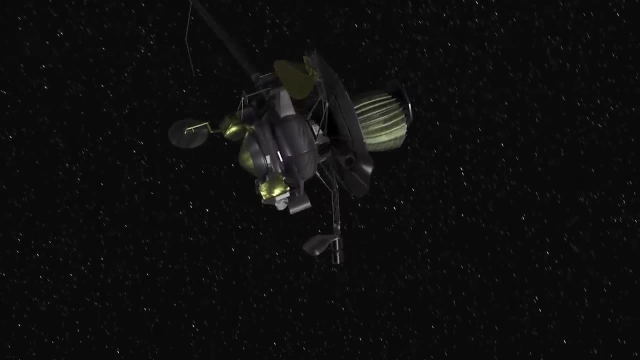 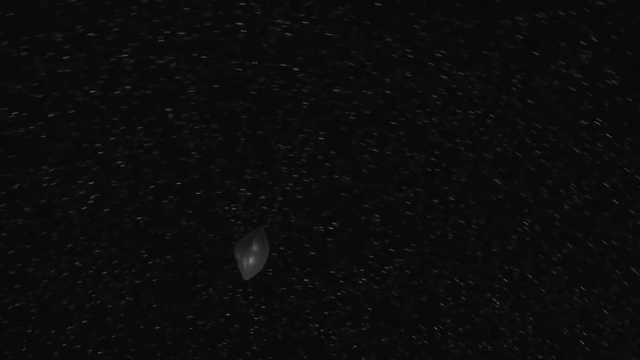 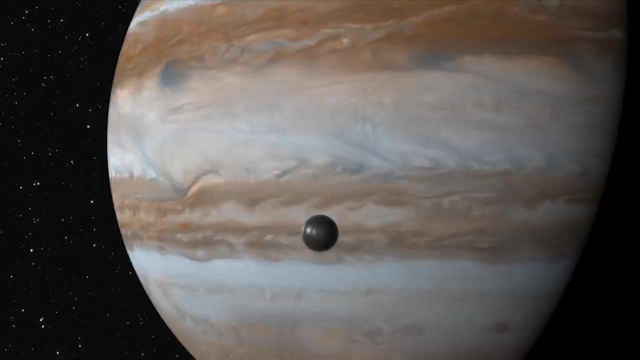 from its closest encounter with Jupiter, Galileo engineered a new satellite. It ejected a small probe designed to enter the atmosphere and sample its chemical composition. The probe lasted for an hour in Jupiter's atmosphere. The data was relayed to Galileo and recorded for subsequent transmission back to Earth. 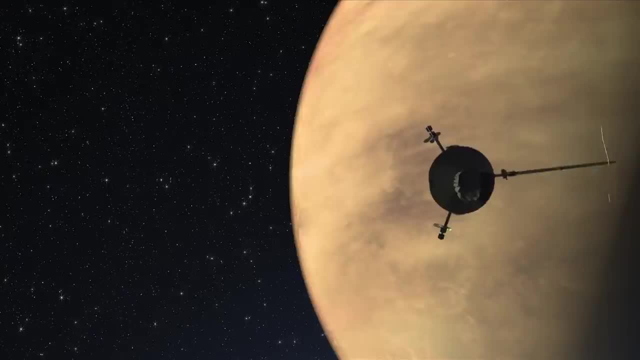 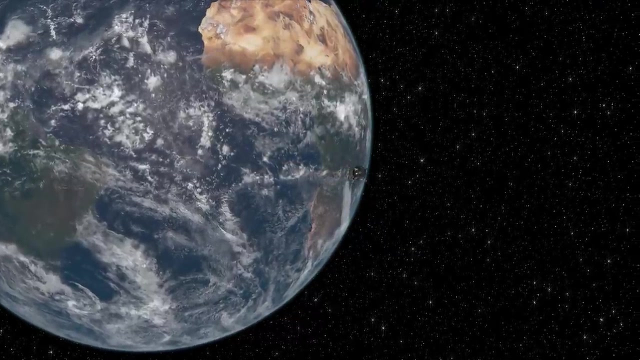 The new flight path meant Galileo was travelling to a hotter part of the solar system. It was decided to keep the heat-sensitive antenna furled until after the spacecraft looped back past Earth. Galileo made two close passes of Earth, each time gaining more speed. 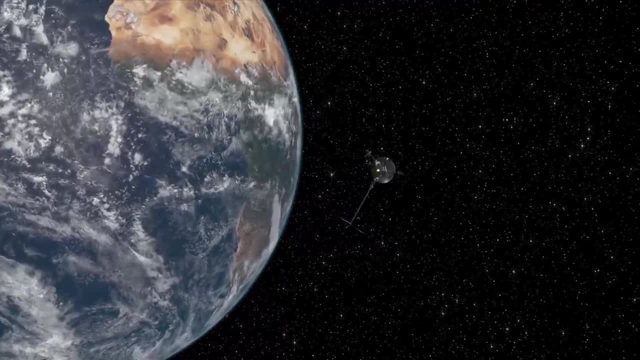 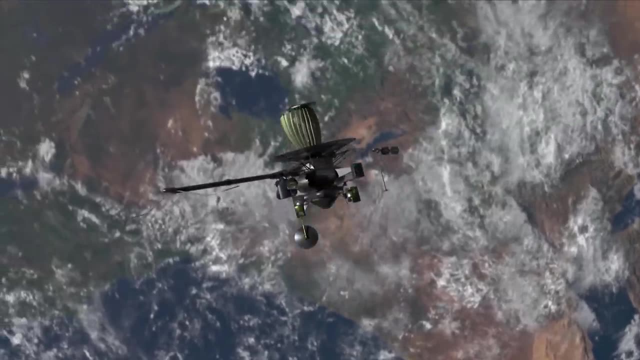 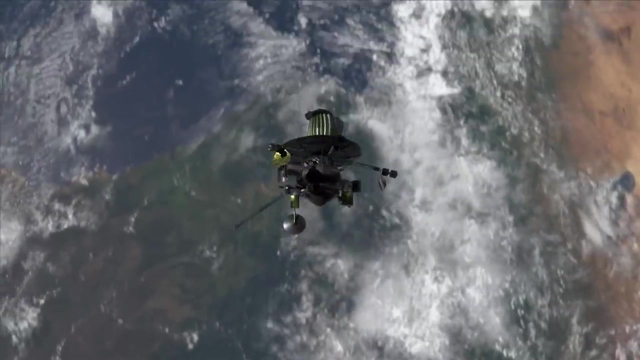 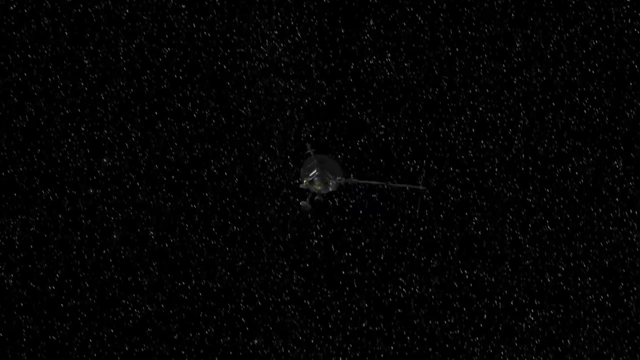 Its first pass was in December 1990, more than a year after its launch. A further year on, when it passed Earth again, the high-gain antenna was only partially open. After months of trying different techniques to deploy the antenna mission, engineers concluded that long periods in storage had caused lubricant at the tips of the antenna's ribs to dissipate. 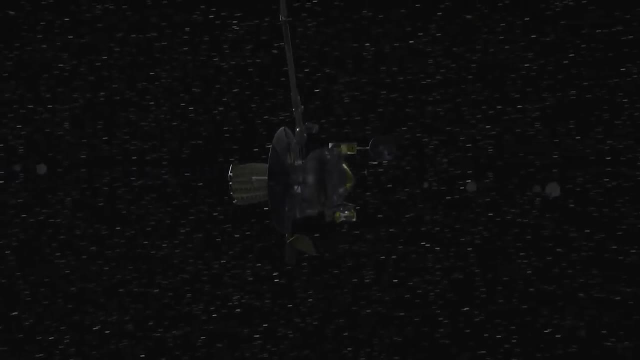 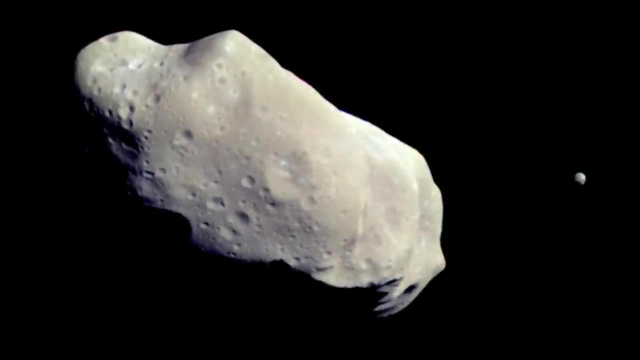 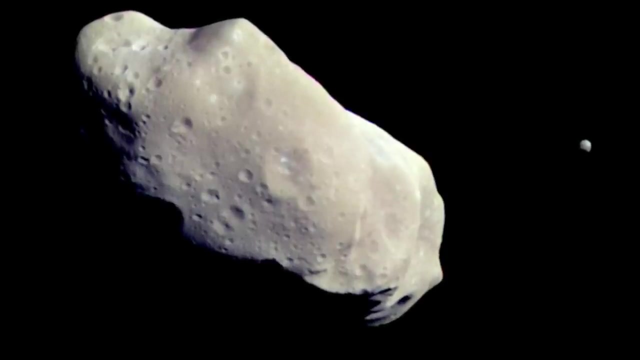 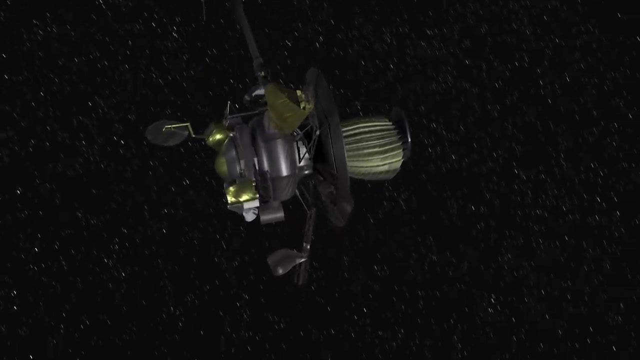 Researchers would rely on Galileo's smaller antenna, with data delivered at slower rates. During the cruise to Jupiter, Galileo encountered several asteroids. This is Ida, the first asteroid we've learnt of, with its own moon, Dactyl, In July 1995, while it was still six months away from its closest encounter with Jupiter. 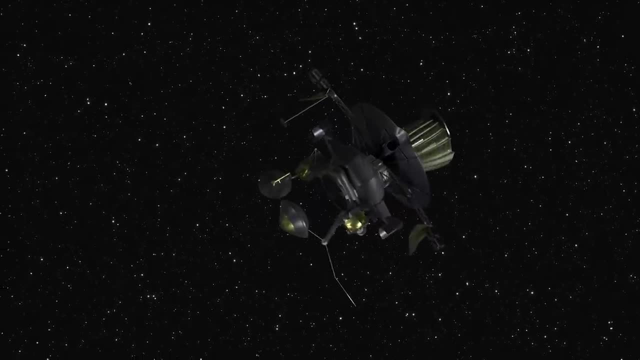 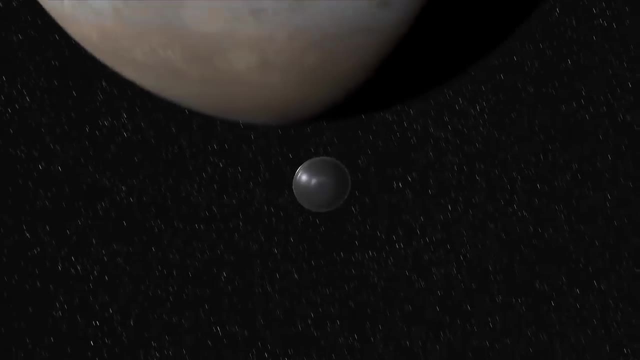 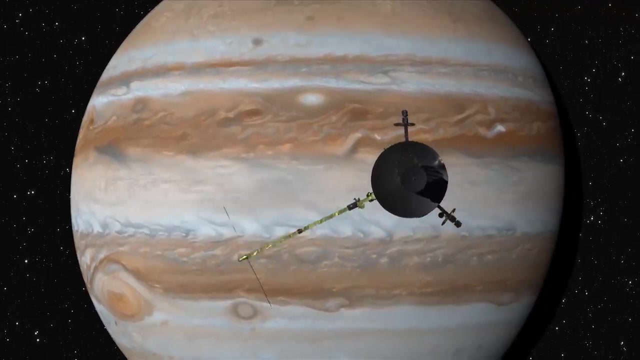 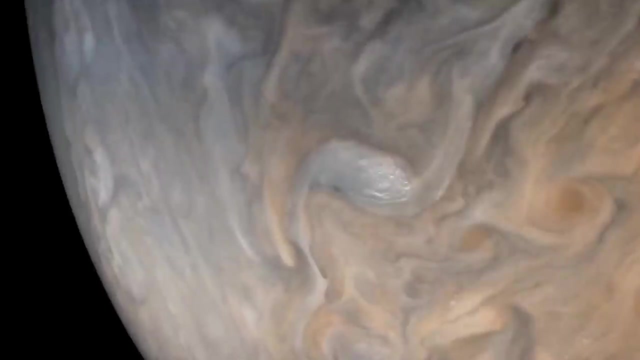 Galileo ejected a small probe designed to enter the atmosphere and sample its chemical composition. The probe lasted for an hour in Jupiter's atmosphere. The data was relayed to Galileo and recorded for subsequent transmission back to Earth. Its analysis revealed hardly any water vapour, which was unexpected. 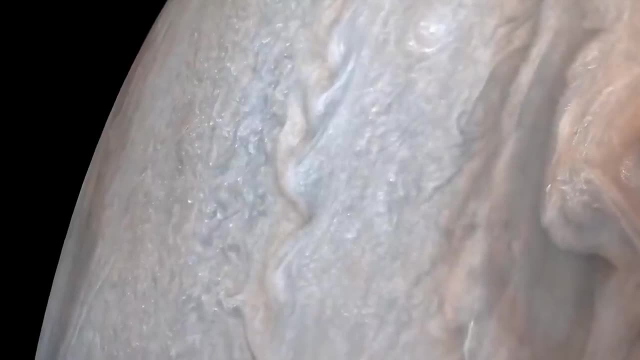 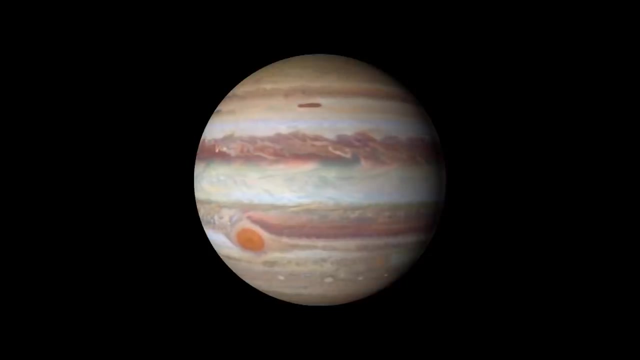 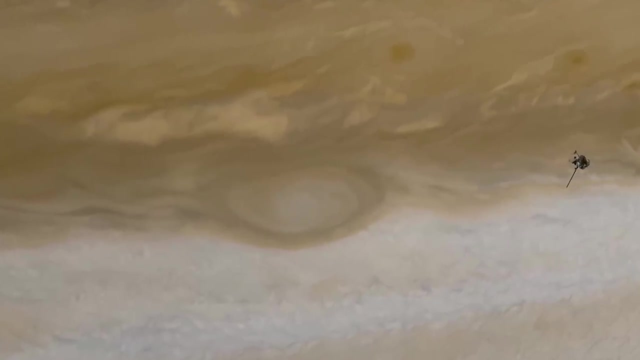 and other elements, particularly helium, were detected at far lower levels than predicted. The probe experienced areas of extreme heat and cold, suggesting heat is being released from the planet's interior Slightly more than an hour after transmission from the probe ceased, Galileo began its orbit insertion burn. 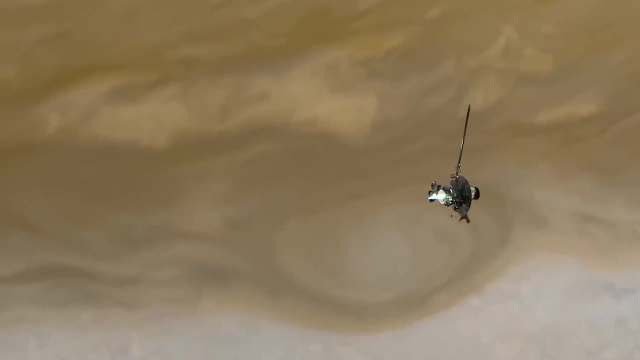 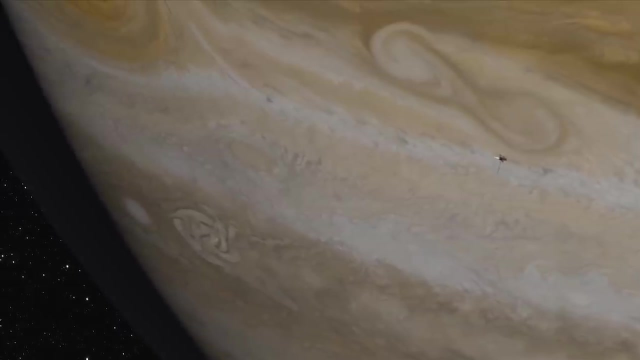 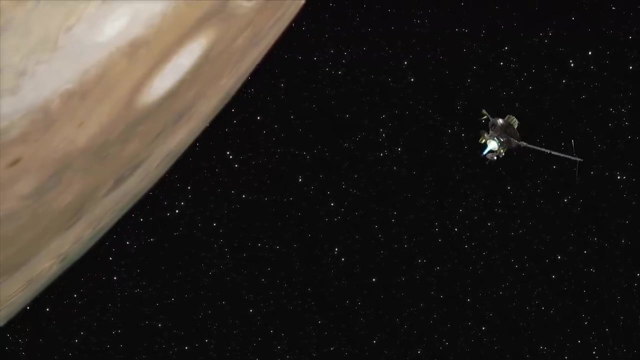 Its engine had to operate for 49 minutes to put it into a highly elliptical equatorial orbit. But this orbit would be altered with another burn at its high point. Mission designers were acutely aware of the high radiation environment, and the second burn would lift Galileo above the extreme radiation at its closest approach. 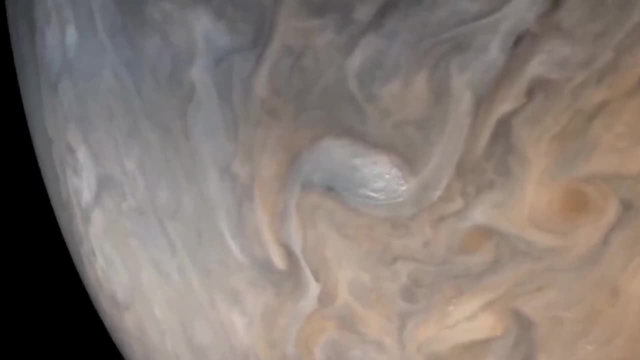 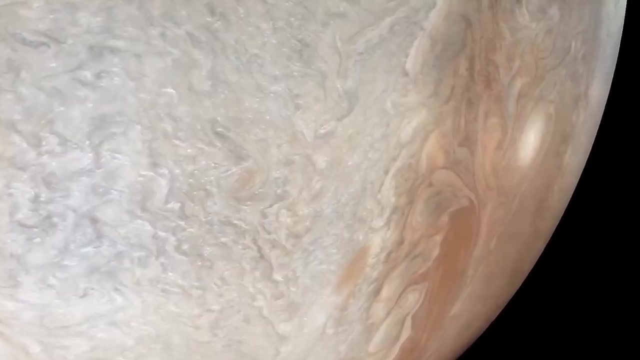 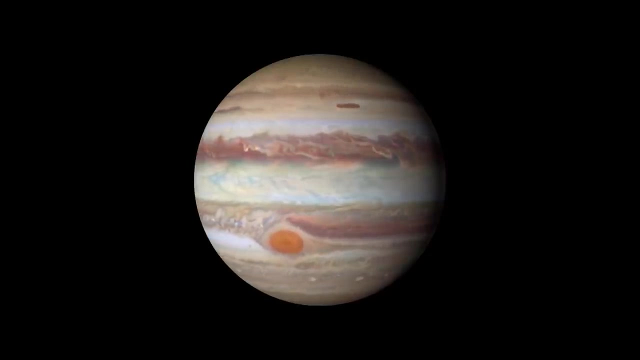 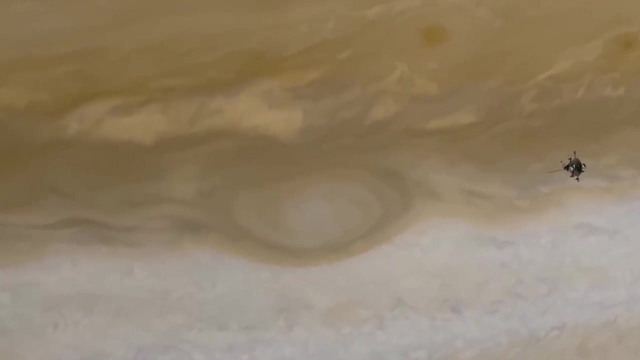 Its analysis revealed hardly any water vapour, which was unexpected, and other elements, particularly helium, were detected at far lower levels than predicted. The probe experienced areas of extreme heat and cold, suggesting heat is being released from the planet's interior Slightly more than an hour after transmission from the probe ceased. 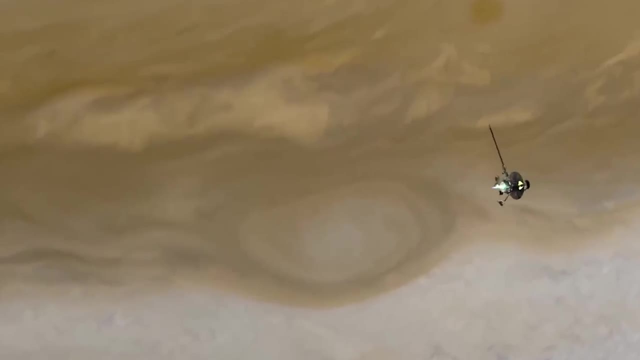 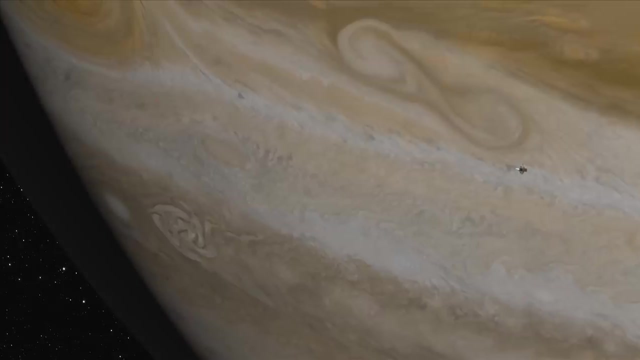 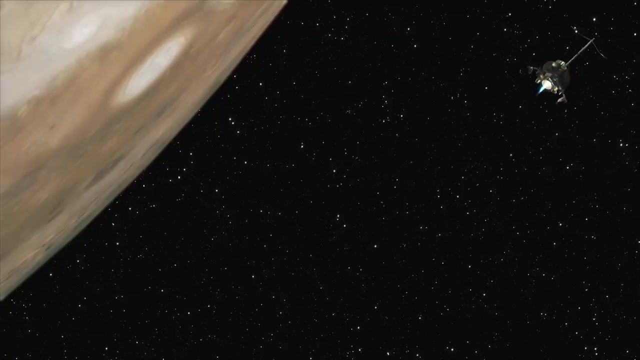 Galileo began its orbit insertion burn. Its engine had to operate for 49 minutes to put it into a highly elliptical equatorial orbit, But this orbit would be altered with another burn at its high point. Mission designers were acutely aware of the high radiation environment. 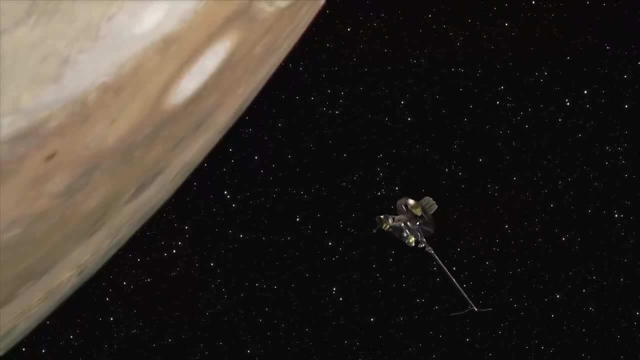 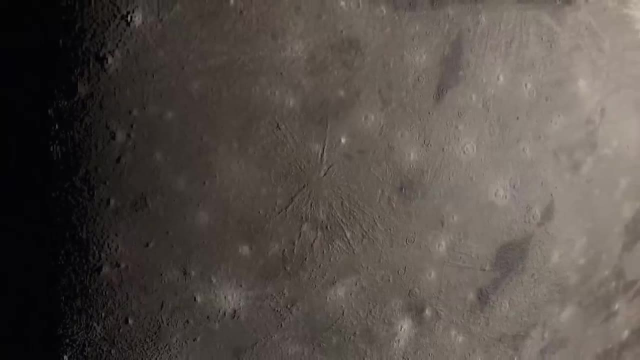 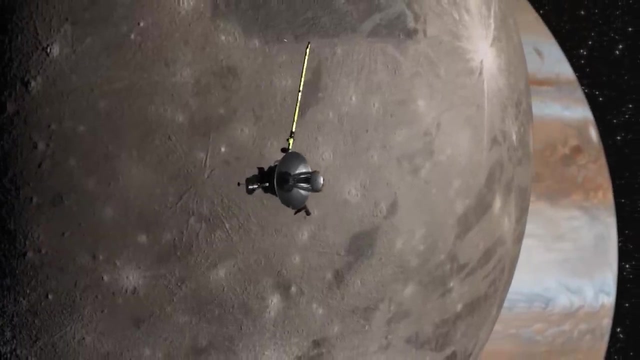 and the second burn would lift Galileo above the extreme radiation at its closest approach. Galileo's initial orbit eventually delivered a close approach to Ganymede, Jupiter's largest moon. During this orbit, engineers were trying to understand damage to the spacecraft's vital tape recorder. 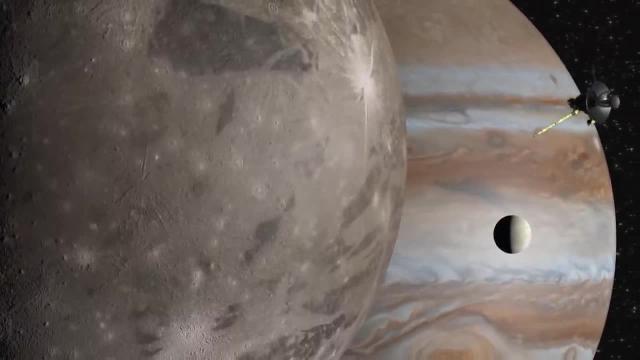 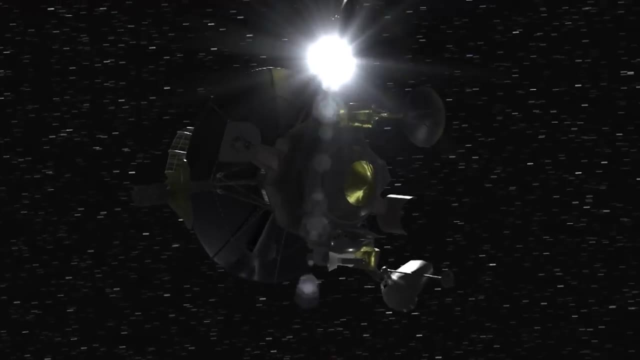 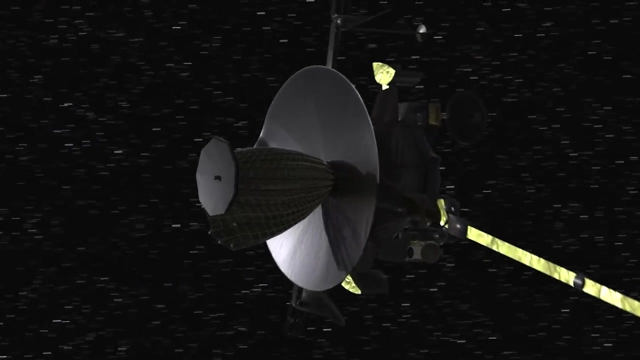 Without its high-gain antenna, the recorder was essential for slow replay of data recorded during the brief close encounters. It had been stuck in rewind for 15 hours and tape had been degraded. Light-emitting diodes: key elements in the recorder's control system. 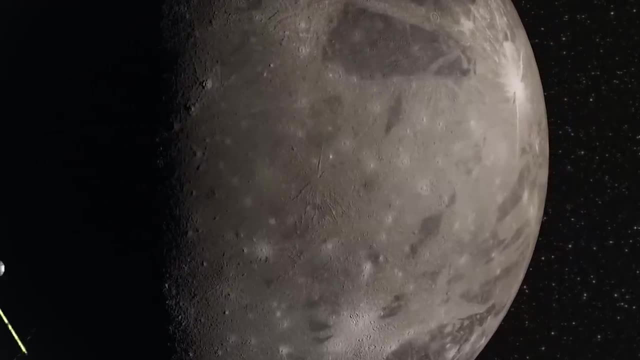 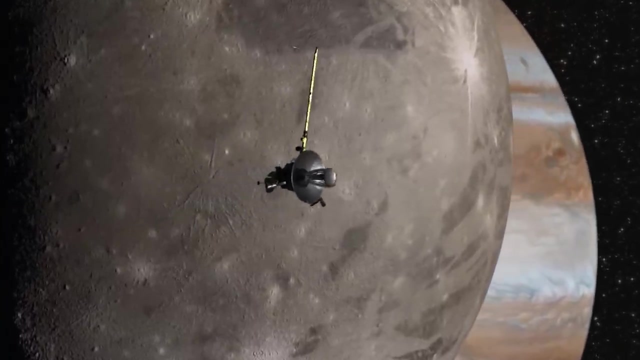 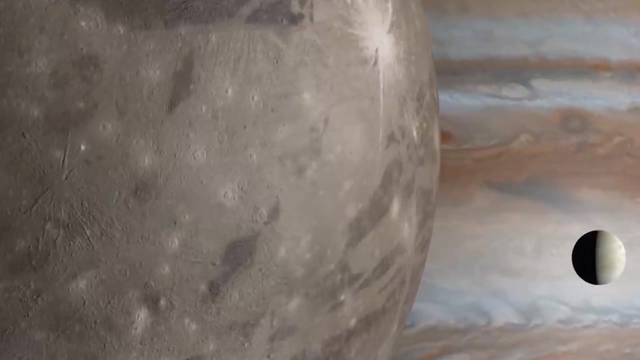 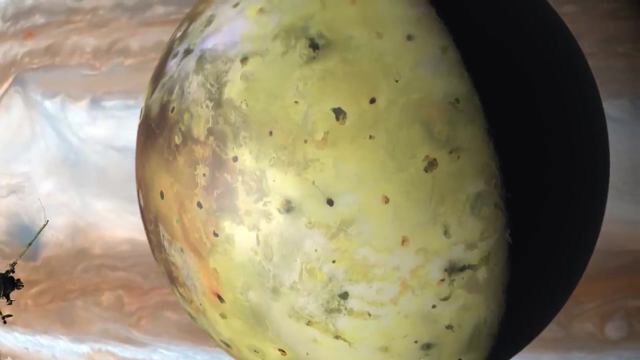 had acquired radiation defects. The second orbit also passed Ganymede Galileo discovered it's the only moon in the solar system with a significant magnetic field. It also has an ocean sandwiched between two layers of ice. Galileo's orbits would be slightly varied. 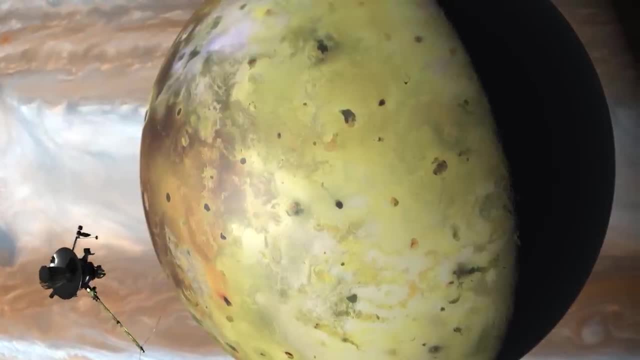 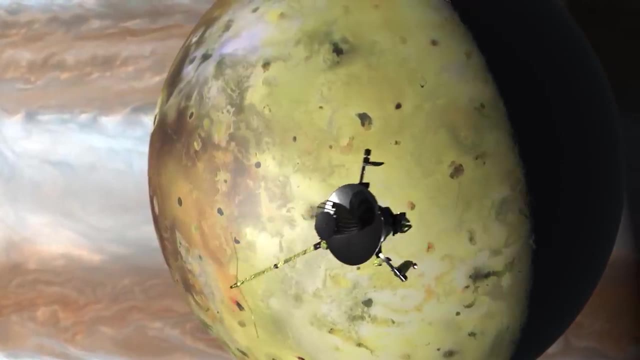 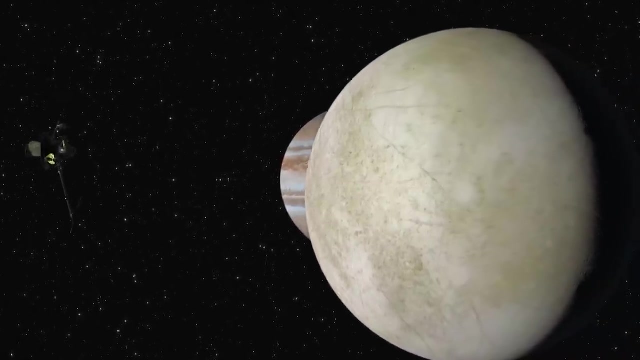 so that it could make close approaches to different Jovian moons. But the equatorial orbits needed to reach the moons also took the craft through hotspots in Jupiter's radiation belts. With the observations made by the Voyagers, the moon Europa was of particular interest to the Galileo team. 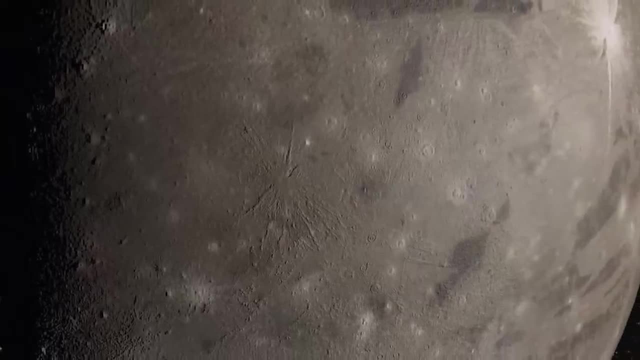 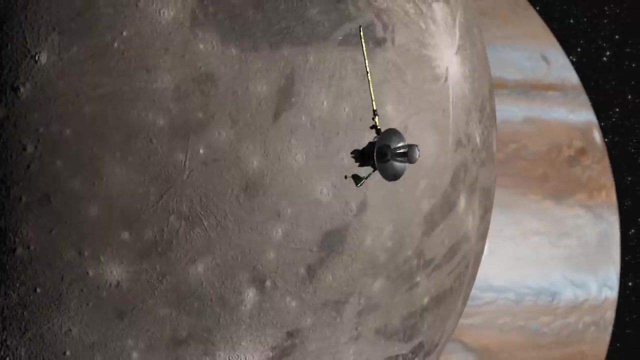 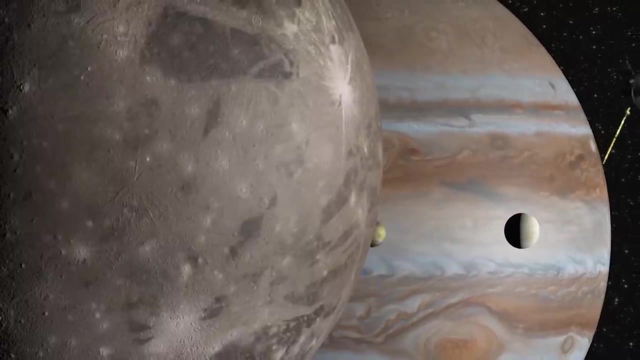 Galileo's initial orbit eventually delivered a close approach to Ganymede, Jupiter's largest moon. During this orbit, engineers were trying to understand damage to the spacecraft's vital tape recorder. Without its high-gain antenna, the recorder was essential for slow replay of data recorded during the brief close encounter. 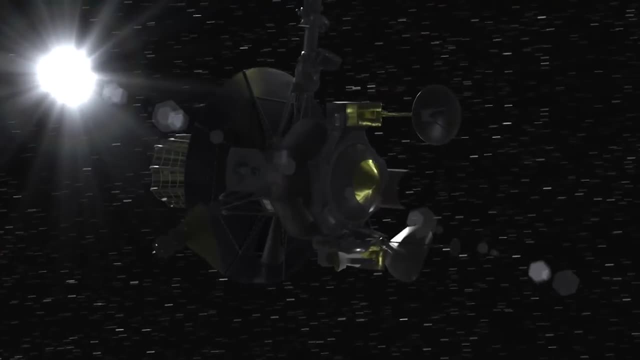 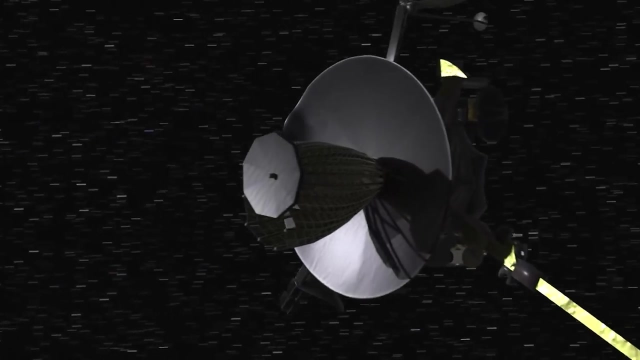 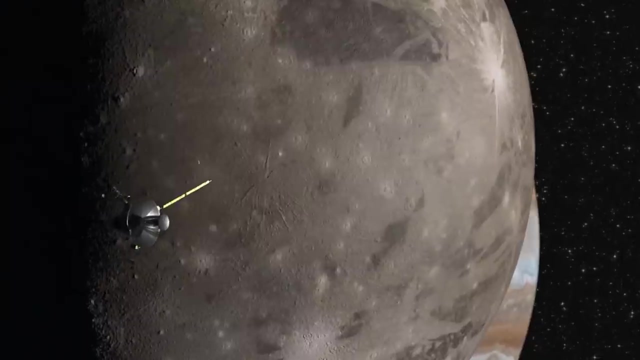 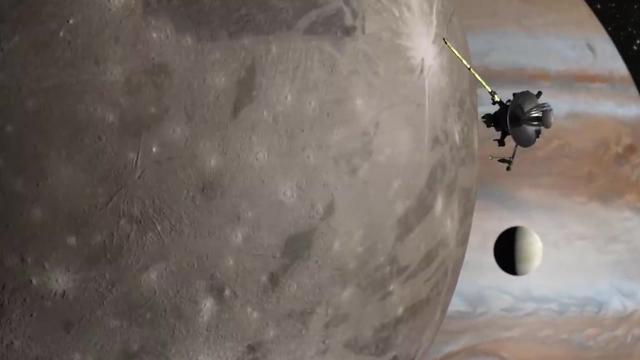 It had been stuck in rewind for 15 hours and tape had been degraded. Light-emitting diodes- key elements in the recorder's control system- had acquired radiation defects. The second orbit also passed Ganymede. Galileo discovered it's the only moon in the solar system with a significant magnetic field. 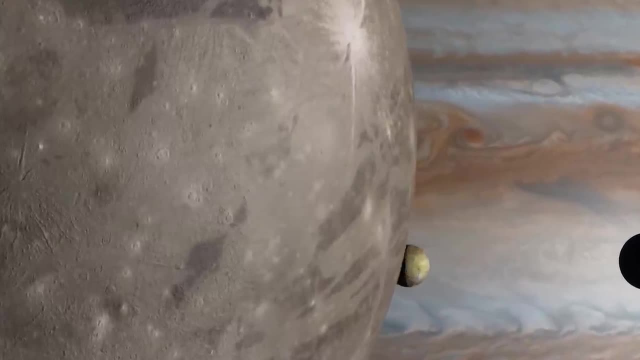 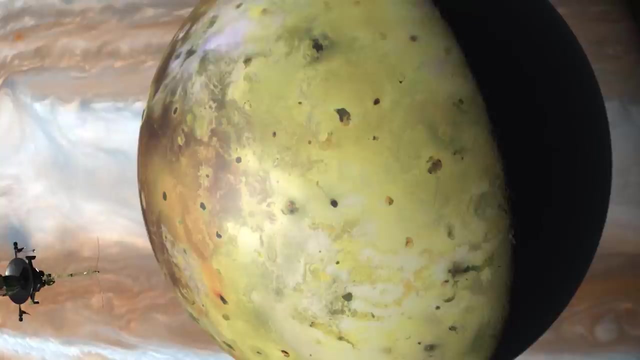 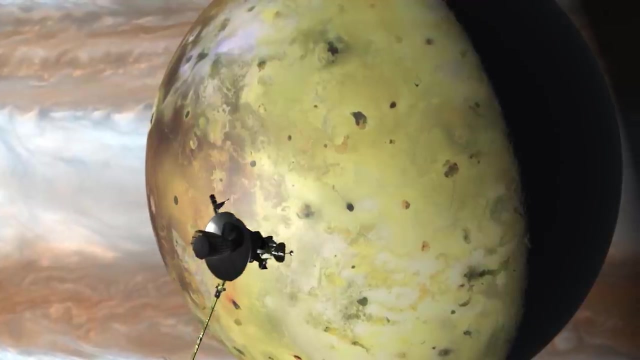 It also has an ocean sandwiched between two layers of ice. Galileo's orbits would be slightly varied so that it could make close approaches to different Jovian moons, But the equatorial orbits needed to reach the moons also took the craft through hotspots in Jupiter's radiation belts. 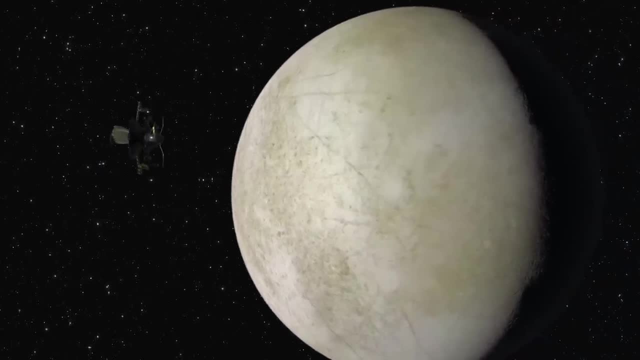 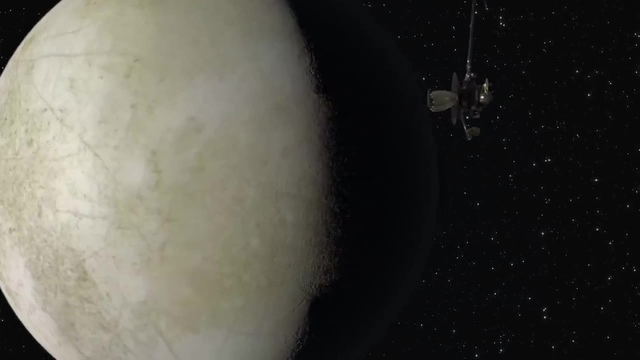 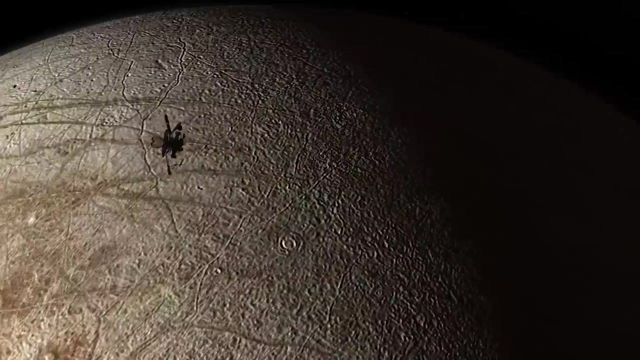 With the observations made by the Voyagers, the moon Europa was of particular interest to the Galileo team. Data from several instruments agreed that a salty ocean exists beneath Europa's surface ice. Later examination of the Galileo datasets revealed plasma wave and magnetic field information. 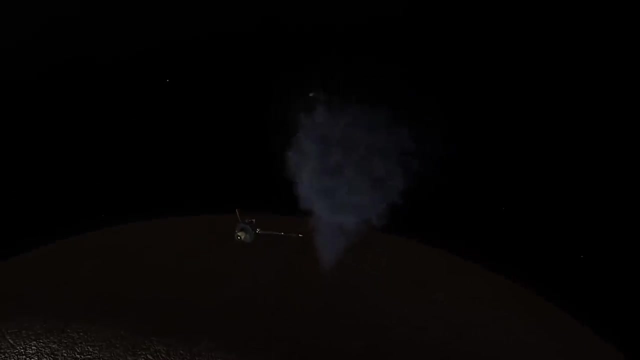 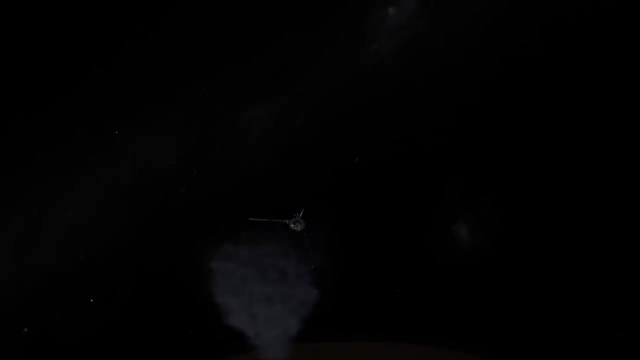 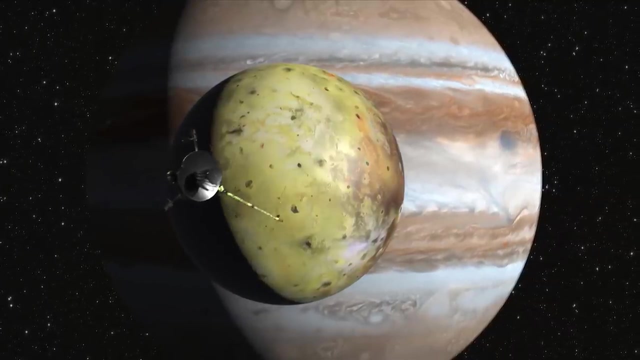 showing that plumes of water vapor were erupting from cracks in the surface. Europa has more water than Earth, which makes it a possible home to life. Europa is already known to have volcanic activity, But Galileo saw tides in the moon's solid surface of more than 100 meters. 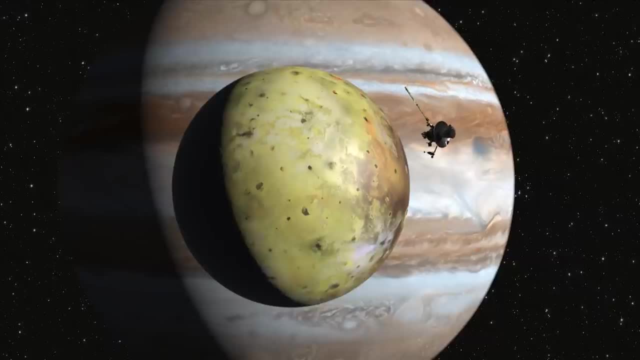 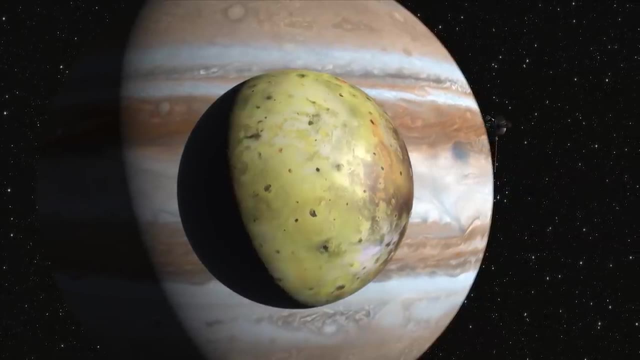 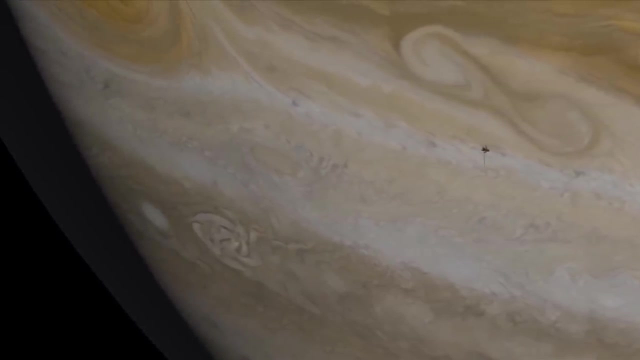 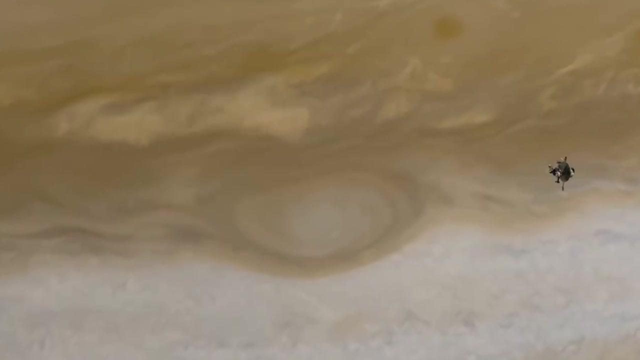 The temperatures generated by this gravitational distortion of Io make its numerous volcanoes hotter than anything found on Earth. During its eight years at Jupiter, Galileo completed 35 orbits, filling out our limited picture of the Jovian system. This was never an easy mission. 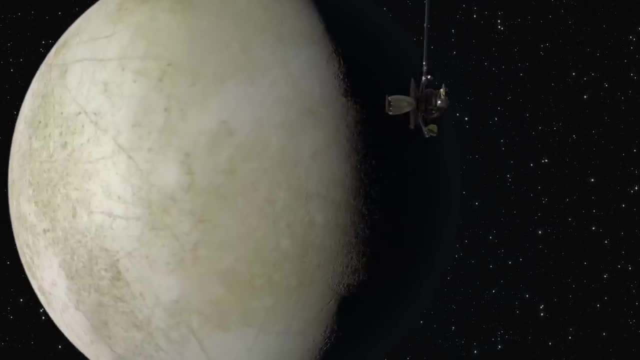 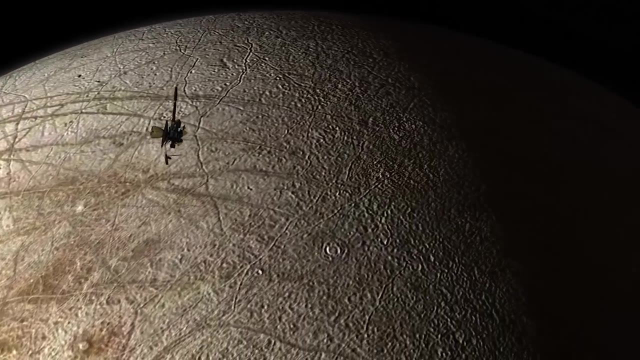 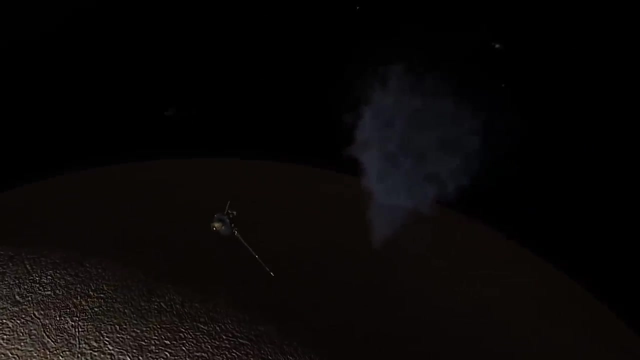 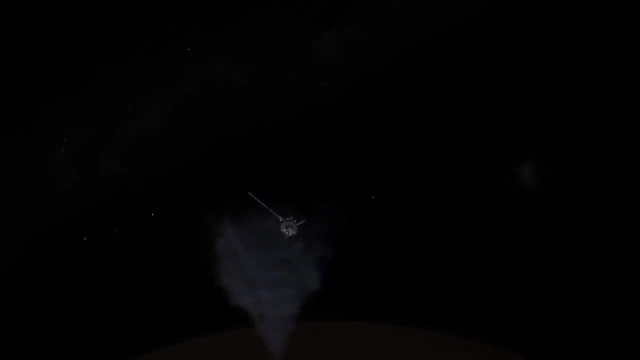 Data from several instruments agreed that a salty ocean exists beneath Europa's surface ice. Later examination of the Galileo data sets revealed plasma wave and magnetic field information showing that plumes of water vapor were erupting from cracks in the surface. Europa has more water than Earth. 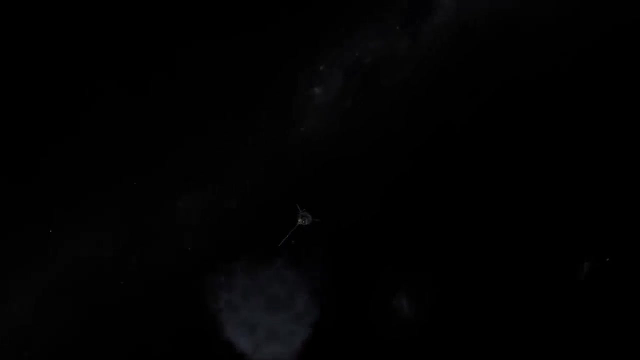 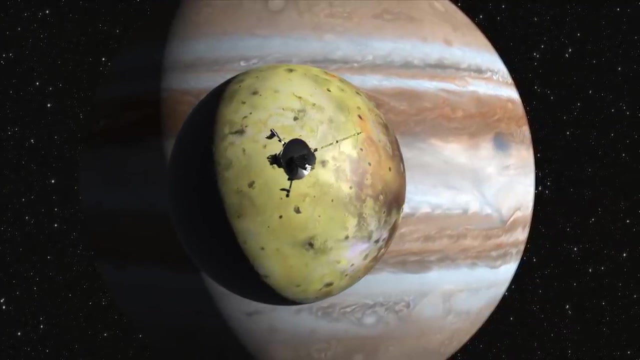 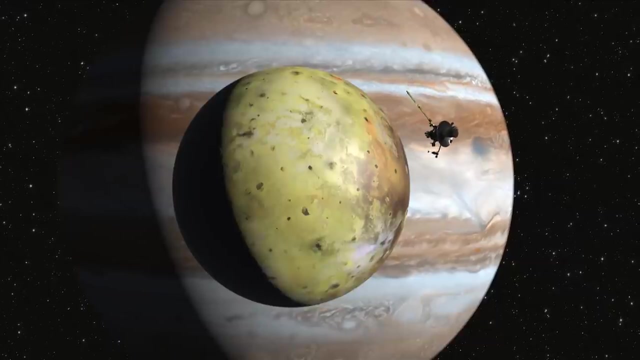 which makes it a possible home to life. Io was already known to have volcanic activity, but Galileo saw tides in the moon's solid surface of more than 100 meters. The temperatures generated by this gravitational distortion of Io make its numerous volcanoes hotter than anything found on Earth. 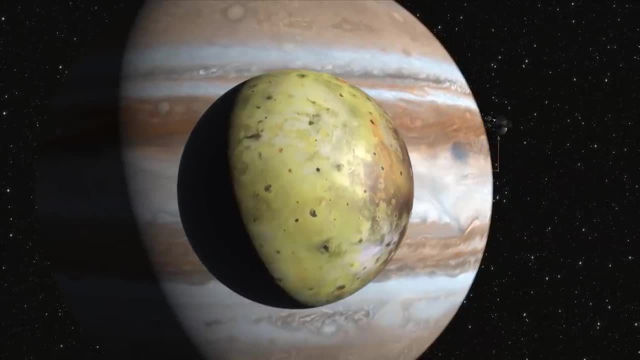 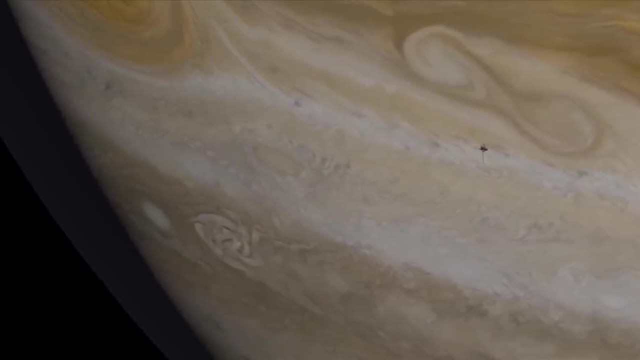 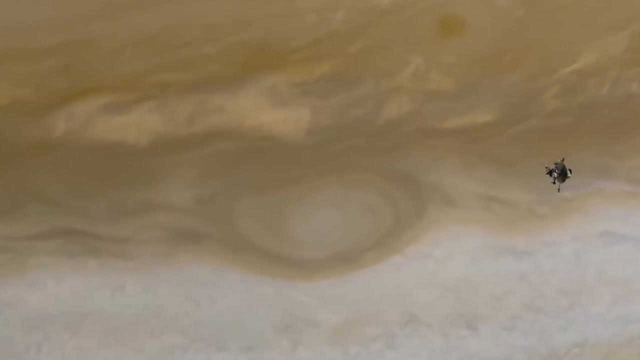 This is the first time Galileo has been able to do this. During its eight years at Jupiter, Galileo completed 35 orbits, filling out our limited picture of the Jovian system. This was never an easy mission. Galileo was a robust spacecraft. 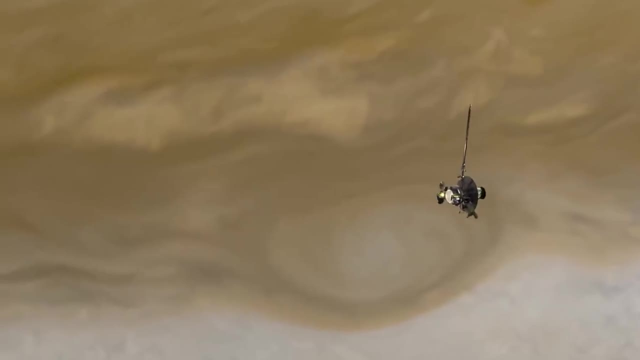 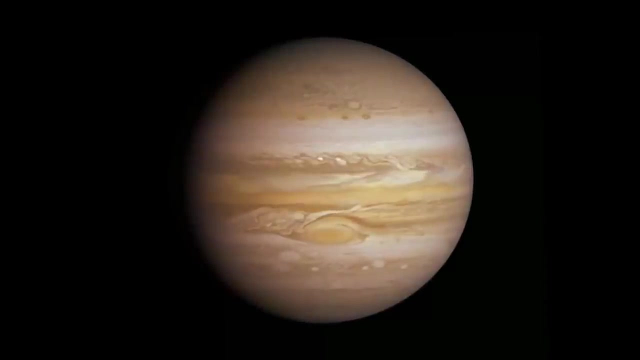 but the radiation environment stressed all the subsystems, and engineers were constantly having to find workarounds for the frequent breakdowns Galileo suffered. Instruments showed increased noise when near Jupiter, and current leakages caused by radiation led to several resets of the onboard computer. 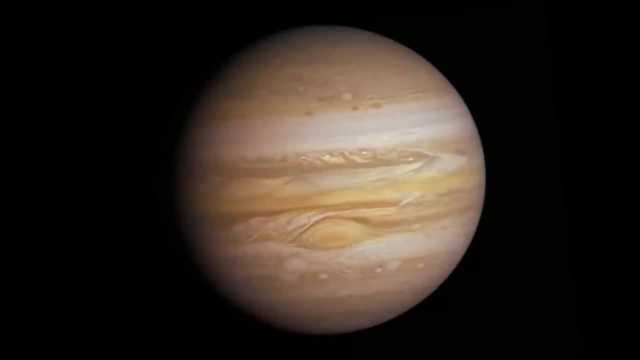 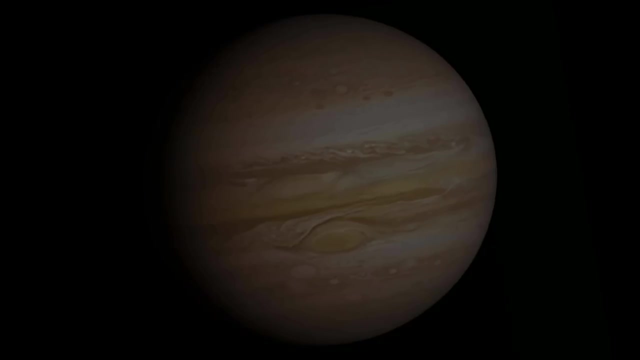 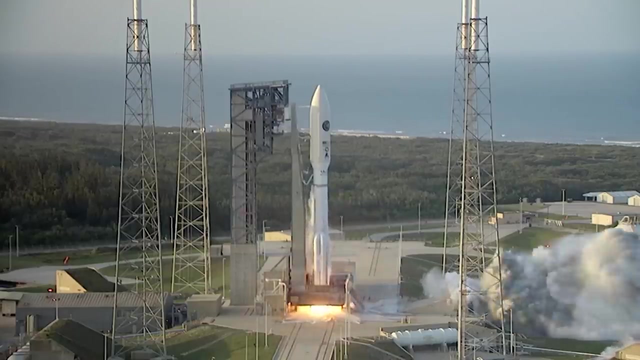 with crucial loss of data. Software changes enabled the computer to recognize these resets and to recover by itself. Information learned would lead to changes in the way the next Jupiter spacecraft was designed. Four, three, two, one. Ignition and liftoff of the Atlas V with Juno. 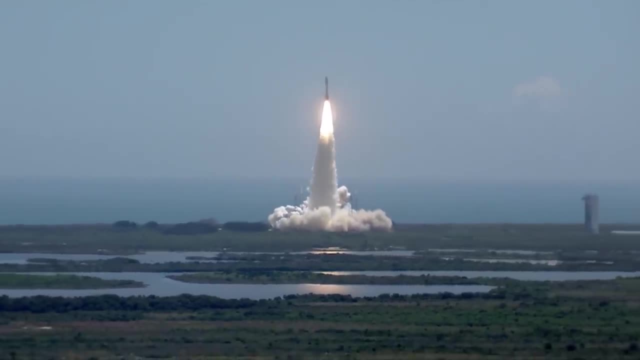 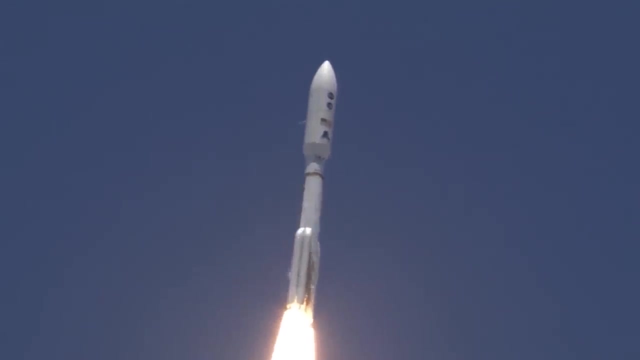 on a trek to Jupiter. In August 2011,, Juno began a journey to Jupiter that would last almost five years. Its mission parameters would be very different to Galileo's: It would ignore the moons and focus exclusively on Jupiter. Spacecraft design saw crucial electrical changes. 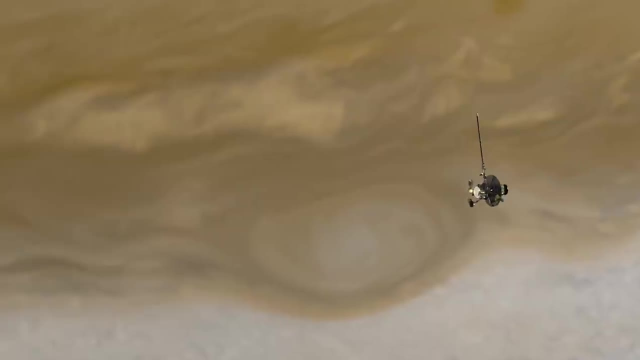 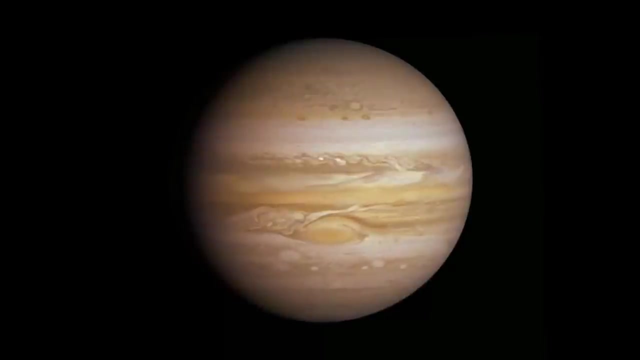 Galileo was a robust spacecraft, but the radiation environment stressed all the subsystems and engineers were constantly having to find workarounds for the frequent breakdowns Galileo suffered. Instruments showed increased noise when near Jupiter, and current leakages caused by radiation led to several resets of the onboard computer. 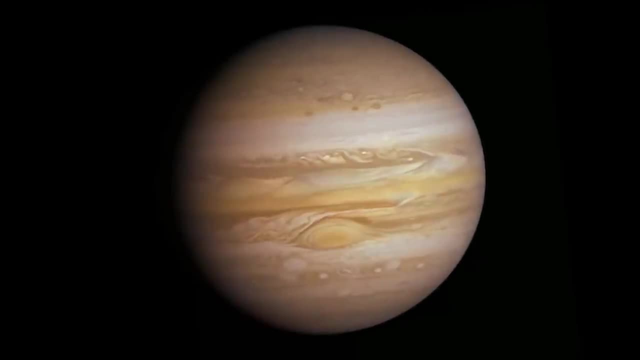 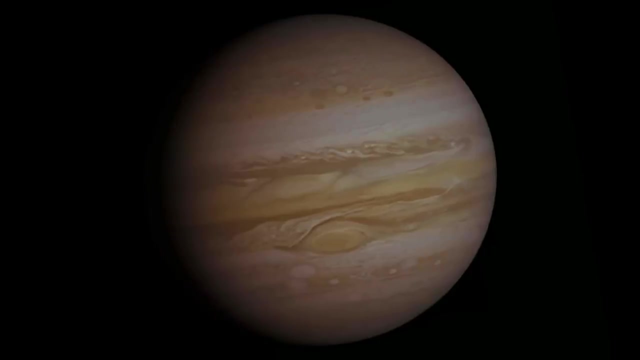 with crucial loss of data, Software changes which enabled the computer to recognize these resets and to recover by itself. Information learned would lead to changes in the way the next Jupiter spacecraft was designed. 5,, 4,, 3,, 2, 1.. 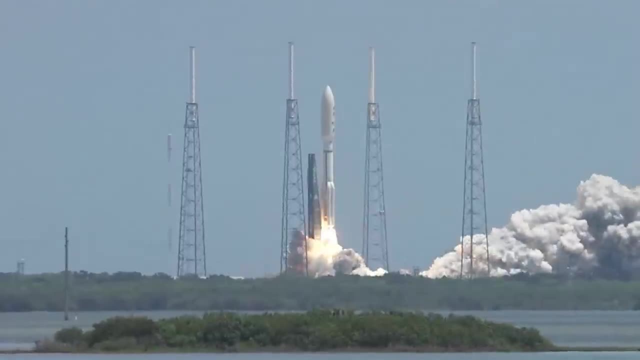 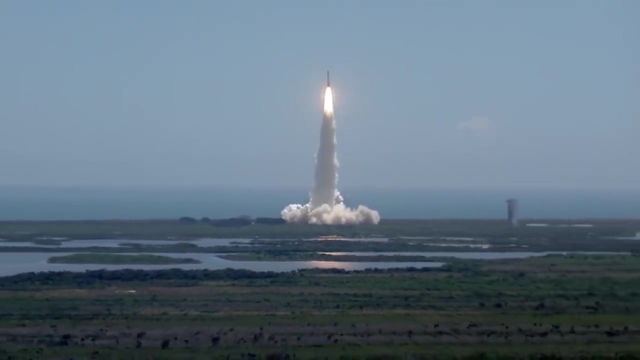 Ignition and liftoff of the Atlas V with Juno on a trek to Jupiter. In August 2011,, Juno began a journey to Jupiter that would last almost five years. Its mission parameters would be very different to Galileo's. 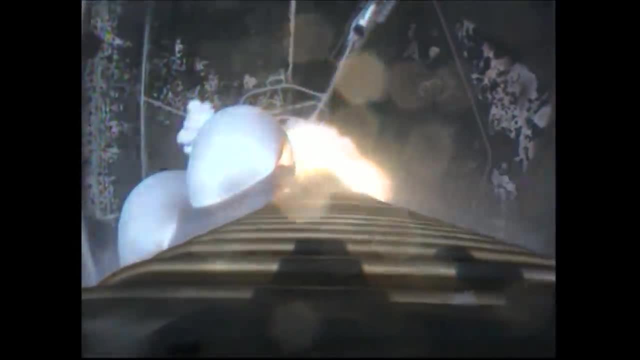 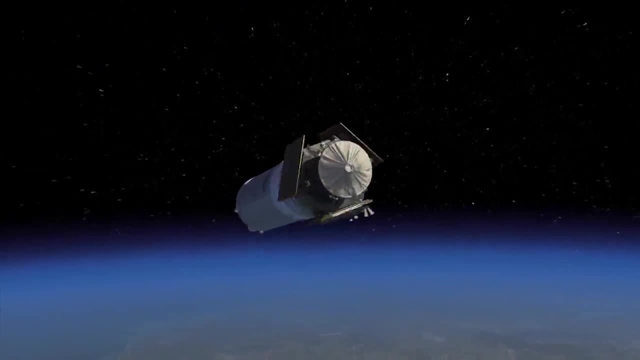 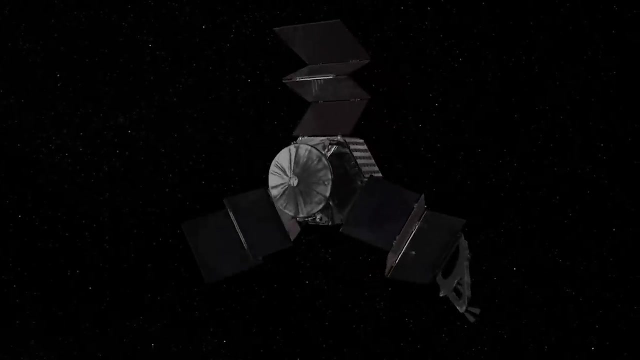 It would ignore the moons and focus exclusively on Jupiter. Spacecraft design saw crucial electronics shielded within a thick titanium vault and, rather than a plutonium power source, Juno would rely on solar panels. The Sun's intensity at Jupiter is roughly 5%. 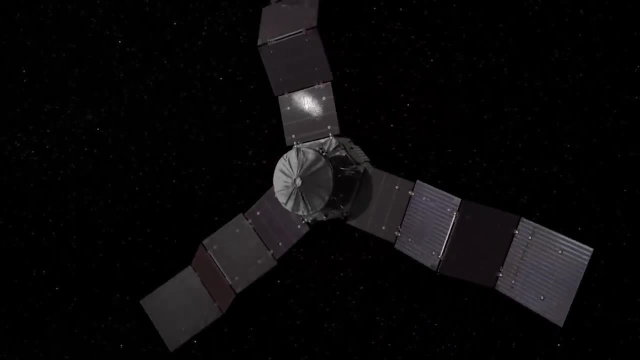 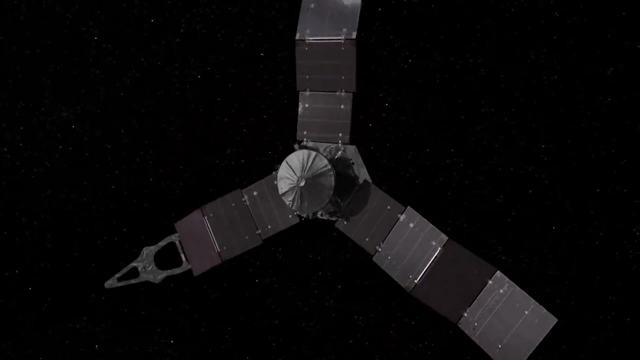 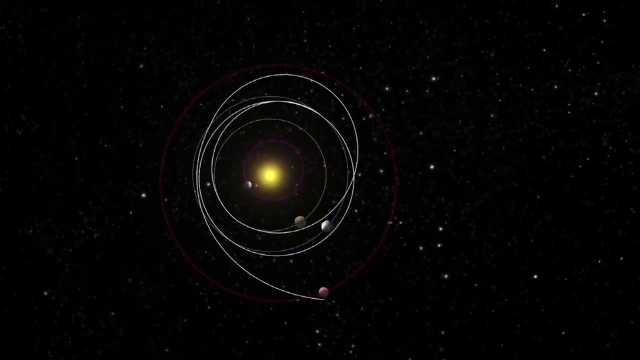 of what it is at Earth, so the panels are huge. A shortage in stocks of plutonium-238 led to the change in power sources. Juno followed a looping orbit that took it beyond Mars before swooping back to Earth for a gravitational boost. 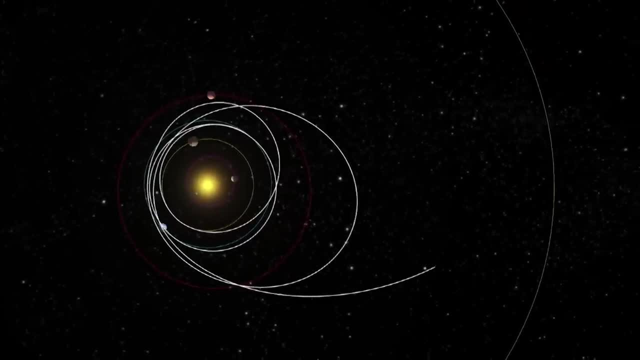 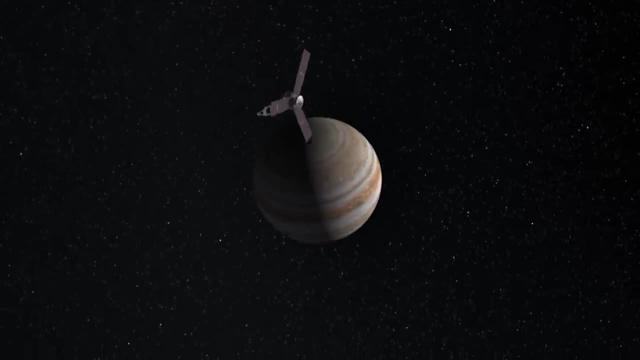 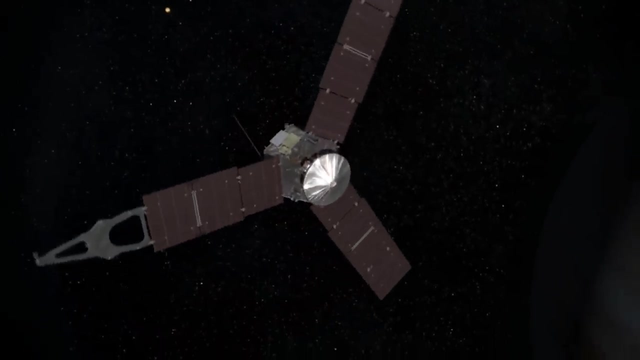 that added 14,000 kilometers per hour to its velocity, sending it on to Jupiter. Juno approached Jupiter on a path that took it above the planet's north pole. It was destined for a north-south orbit. This would see it pass beneath the severest sections. 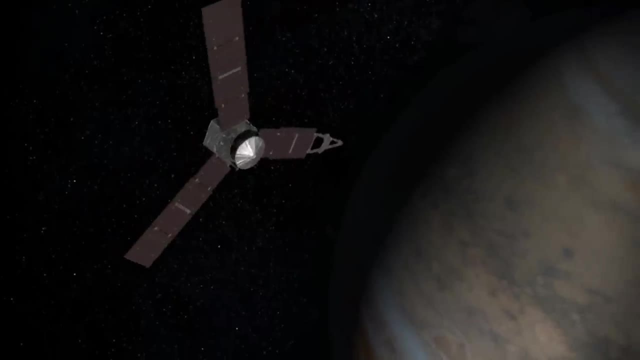 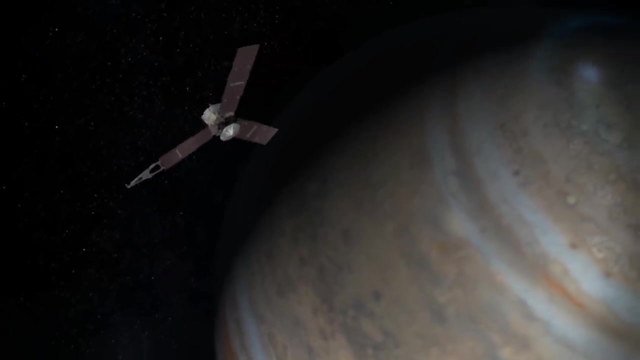 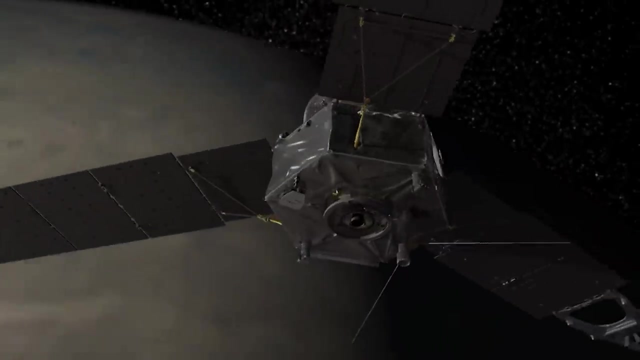 of the planet's radiation belts that extend out from Jupiter's equator. Four days before its closest approach, Mission Control sent a command that initiated the craft's autopilot. On July, the 4th 2016,, Juno began an engine burn. 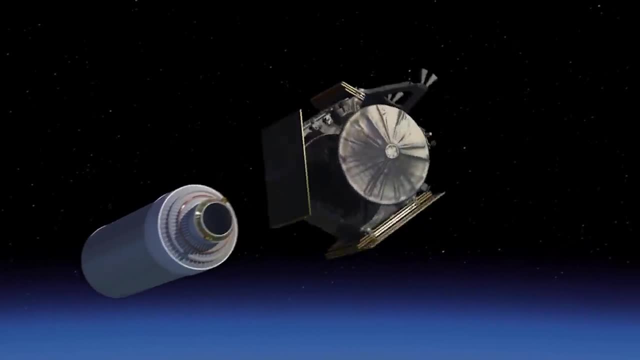 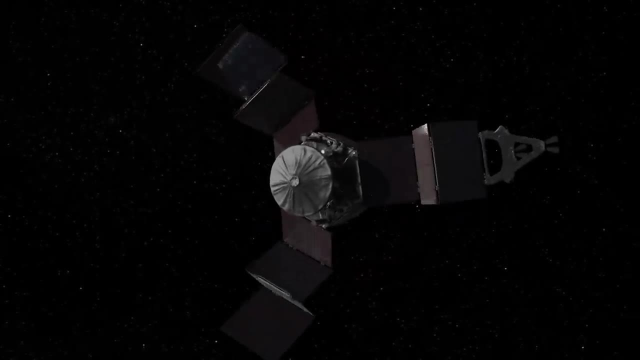 in its electronics shielded within a thick titanium vault, and rather than a plutonium power source, Juno would rely on solar panels. The Sun's intensity at Jupiter is roughly 5% of what it is at Earth, so the panels are huge. 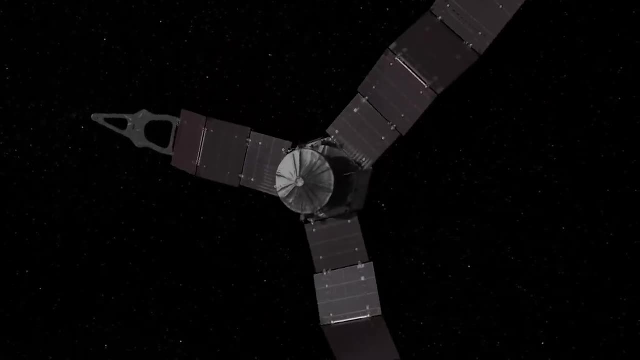 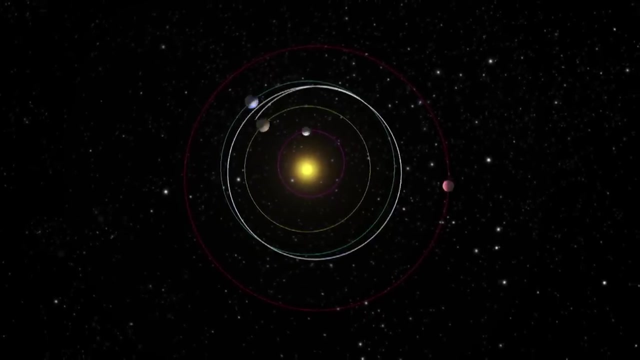 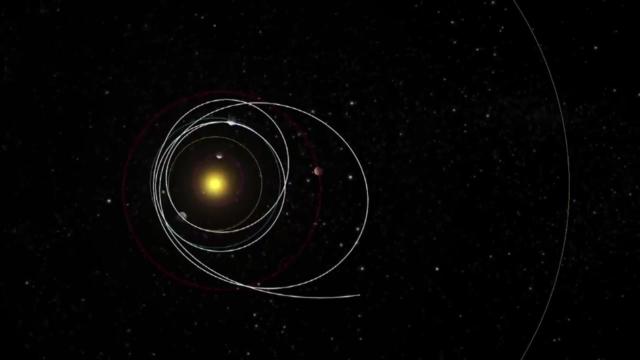 A shortage in stocks of plutonium-238 led to the change in power sources. Juno followed a looping orbit that took it beyond Mars before swooping back to Earth for a gravitational boost that added 14,000 km per hour to its velocity. 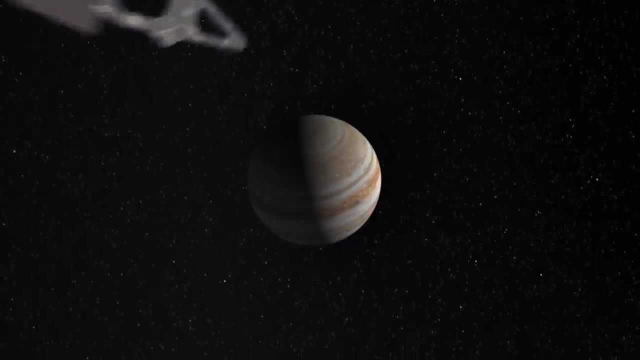 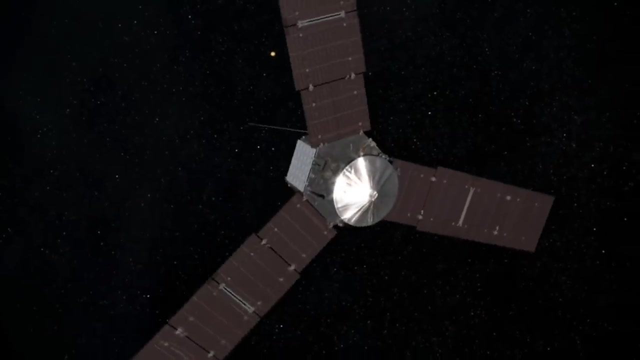 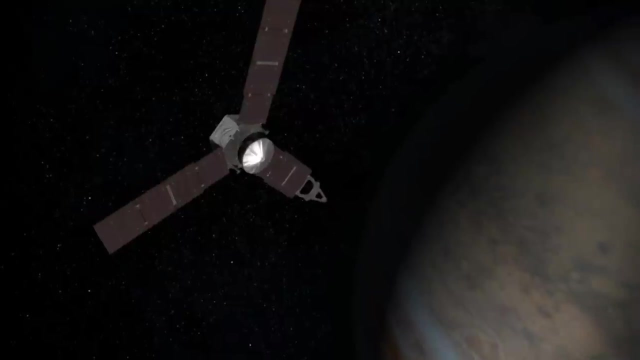 sending it on to Jupiter. Juno approached Jupiter on a path that took it above the planet's north pole. It was destined for a north-south orbit. This would see it pass beneath the severest sections of the planet's radiation belts that extend out from Jupiter's equator. 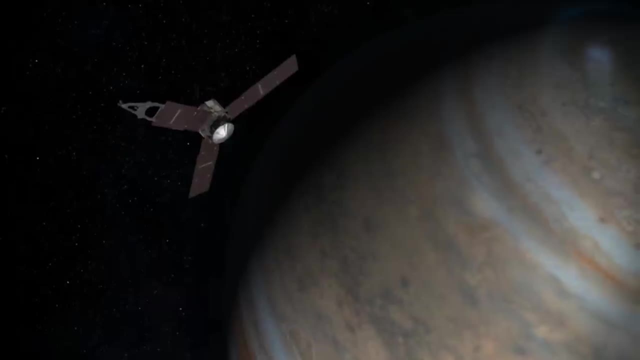 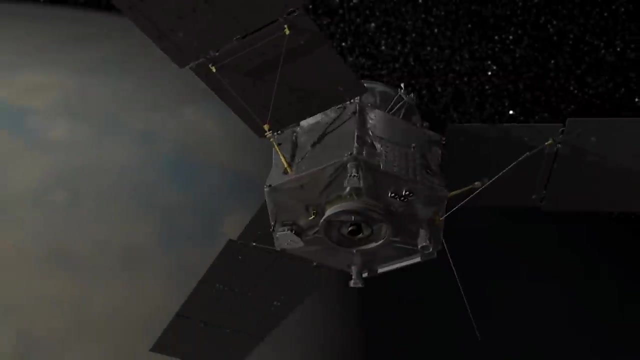 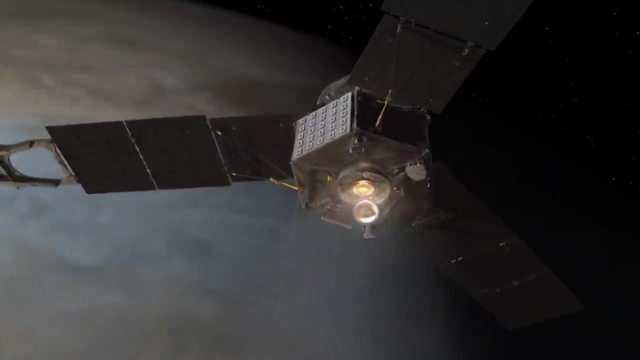 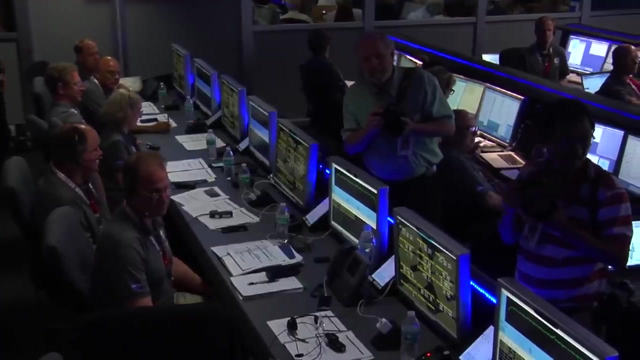 Four days before its closest approach, Mission Control sent a command that initiated the craft's autopilot. On July 4th 2016, Juno began an engine burn that would insert it into a 53-day orbit. 48 minutes later, Mission Control at JPL received tones. 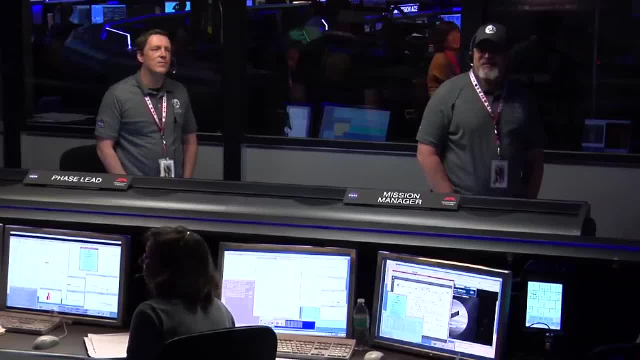 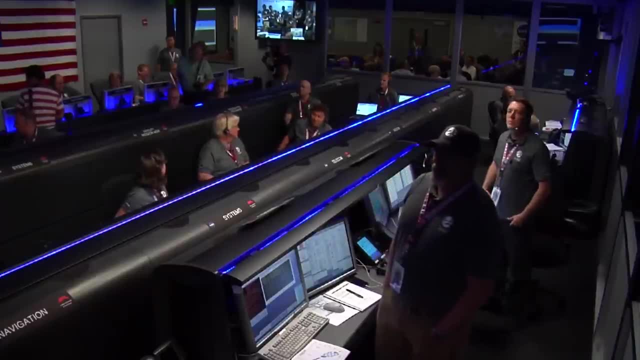 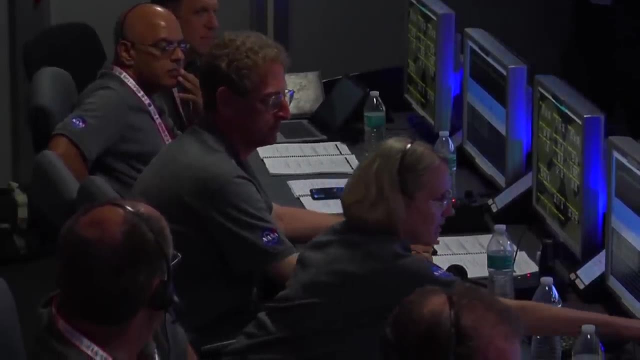 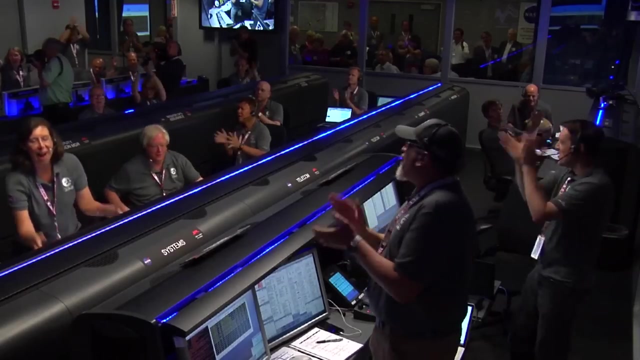 verifying that Juno had started the mission. It started its deceleration maneuver. It was a tense 35-minute wait from the system's engineers before confirmation came through that Juno had performed exactly as intended For the Juno scientists and engineers. 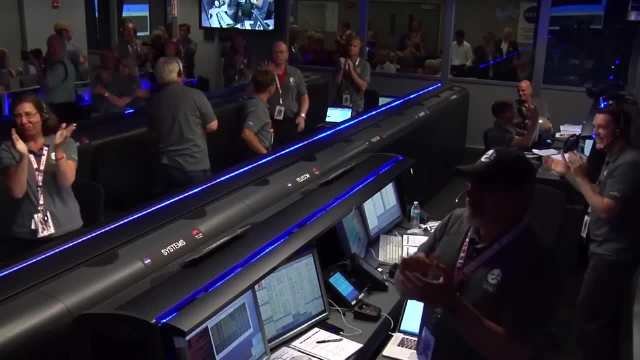 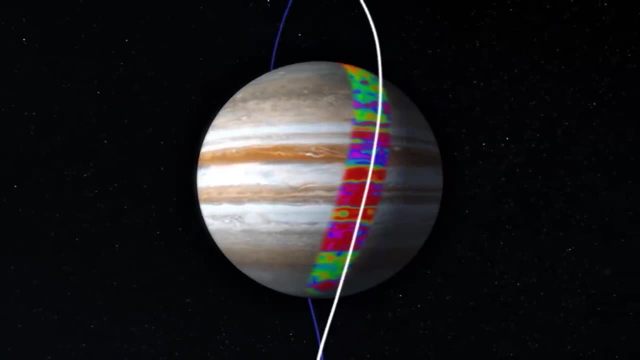 it was a relief that things were going to plan. Roger, don't move, Juno, Juno. Juno is equipped with a suite of instruments capable of penetrating Jupiter's thick cloud. The polar orbit allows Juno to compile a three-dimensional map of the upper atmosphere. 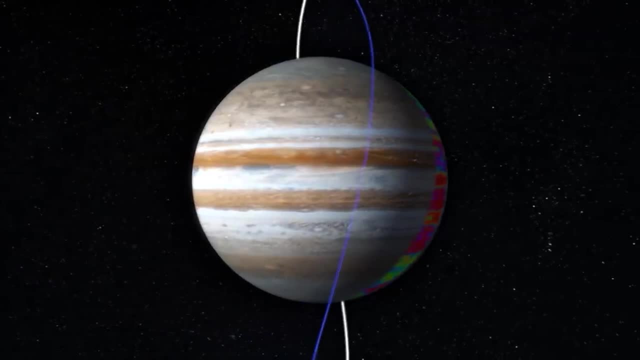 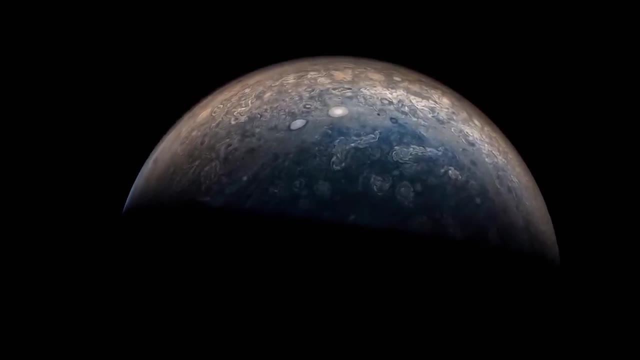 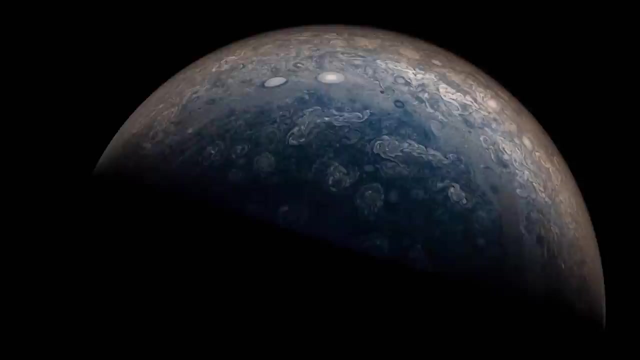 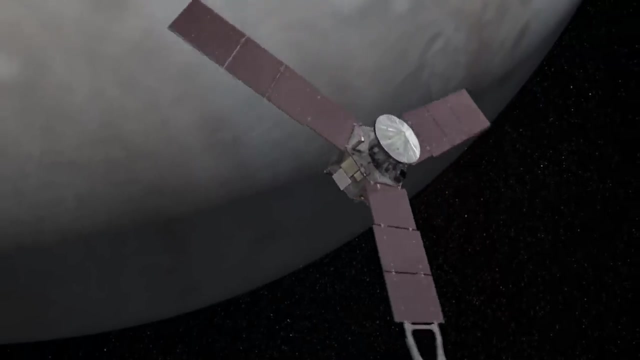 building a picture of the entire planet as it rotates. The images of Jupiter from this new perspective appeared to come from a different planet. Researchers were stunned. It was planned that Juno would only make two 53-day orbits and then change to a series of 14-day orbits. 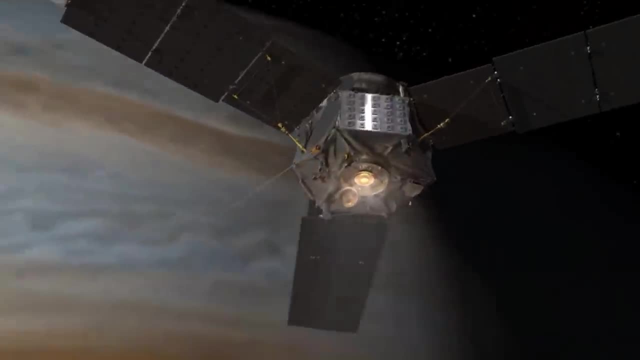 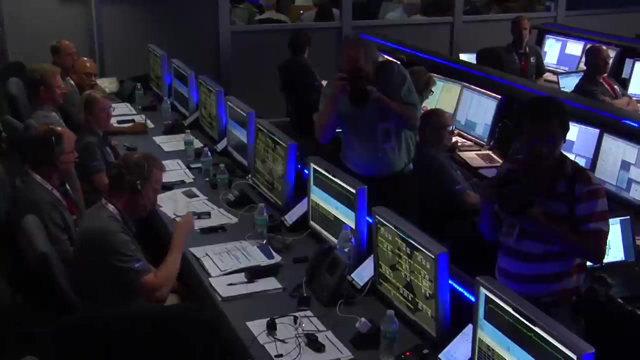 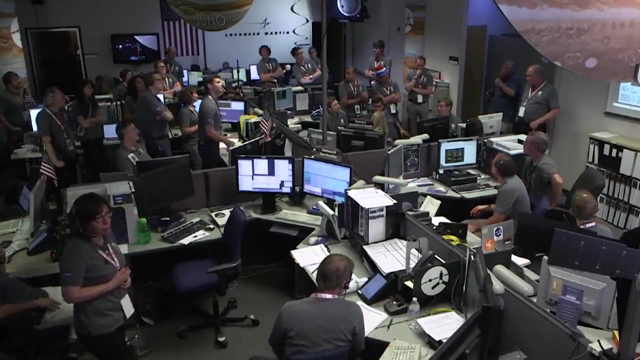 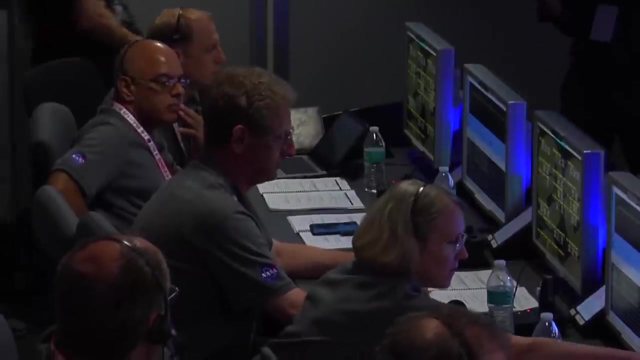 that would insert it into a 53-day orbit. 48 minutes later, Mission Control at JPL received tones verifying that Juno had started its deceleration maneuver. It was a tense 35-minute wait from the system's engineers before confirmation came through that Juno had performed exactly as intended. 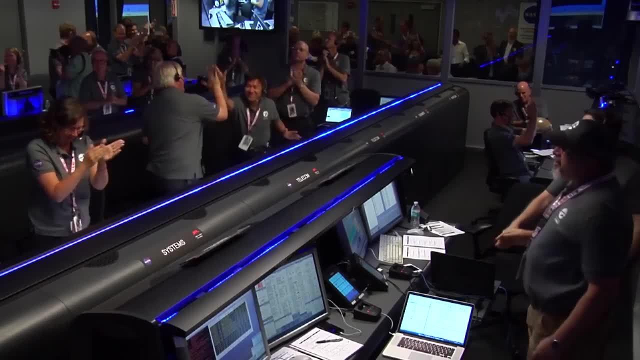 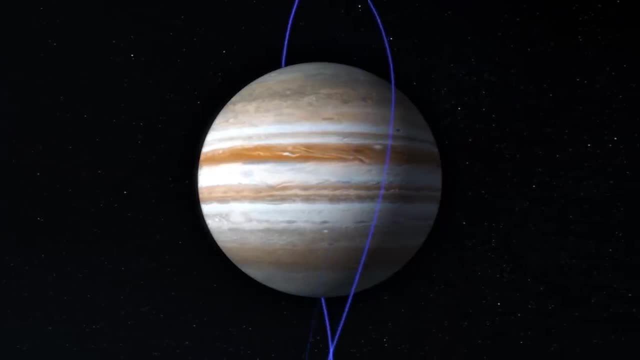 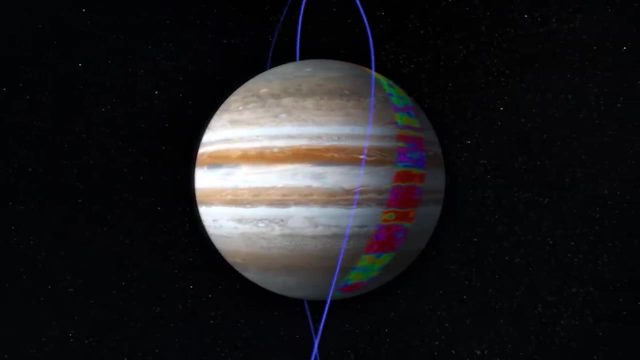 For the Juno scientists and engineers, it was a relief that things were going to plan. Juno is equipped with a suite of instruments capable of penetrating Jupiter's thick cloud. The Polar Orbit allows Juno to compile a three-dimensional map of the upper atmosphere. 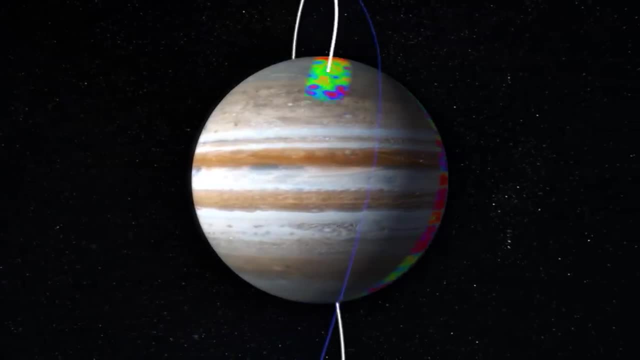 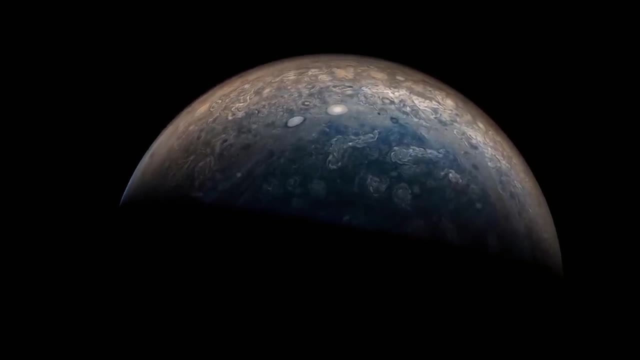 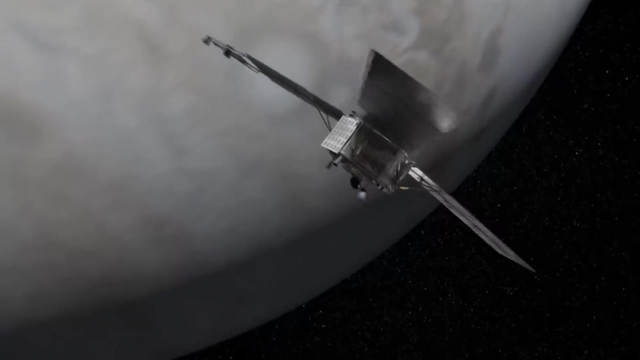 building a picture of the entire planet as it rotates. The images of Jupiter from this new perspective appeared to come from a different planet. Researchers were stunned. It was planned that Juno would only make two 53-day orbits and then change to a series of 14-day orbits. 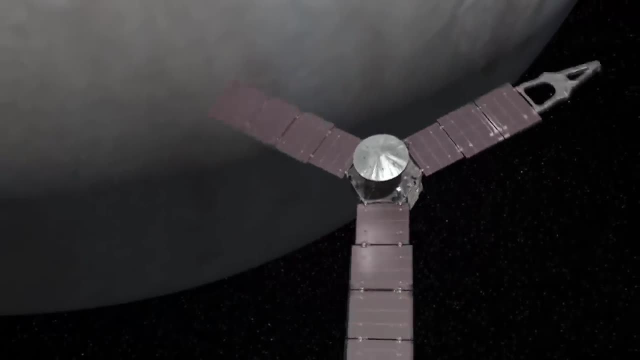 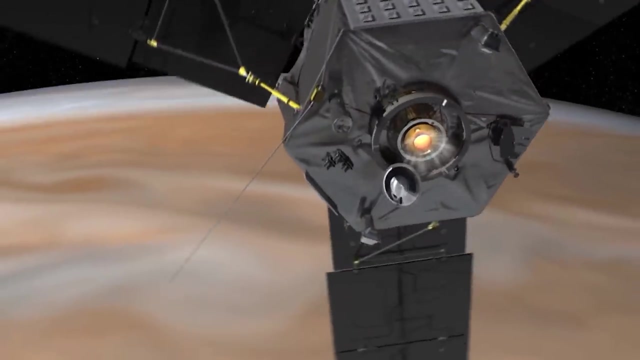 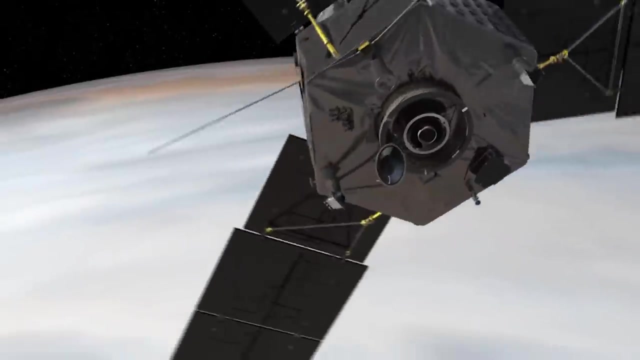 that would speed up the sampling rate. The spacecraft's main engine is fueled by hydrazine and nitrogen tetroxide, which ignite spontaneously when mixed. The propellant and oxidizer are forced out by a bladder of expanding helium As Juno was finishing its second orbit. 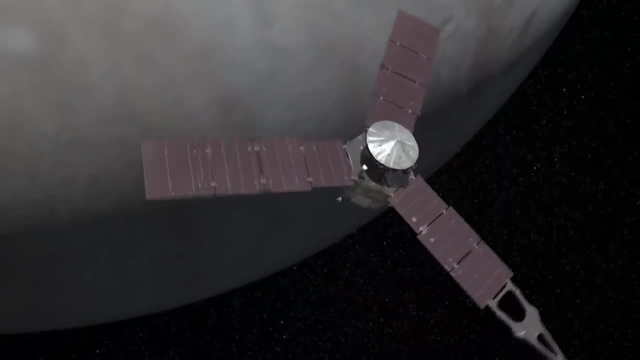 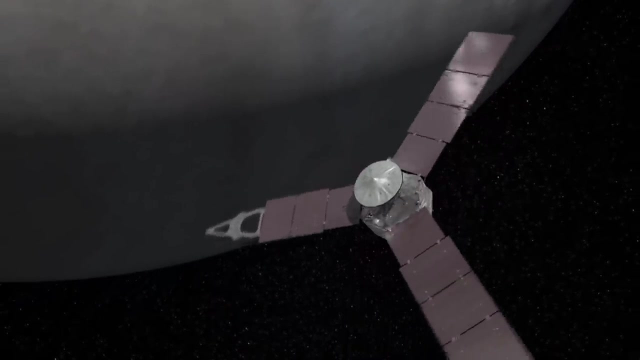 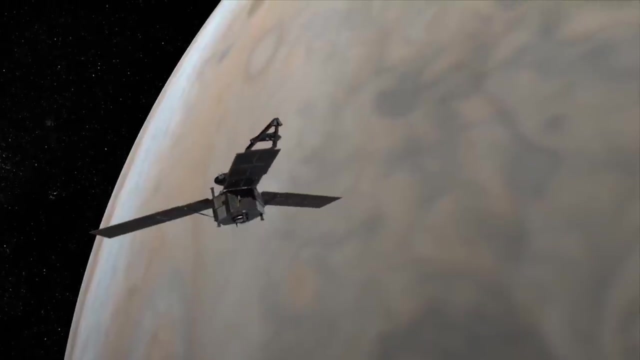 the helium valves were not responding correctly, so it was decided to maintain the original orbit. A mission extension has been granted to allow for the longer orbits Juno continues to follow. Within a day of the helium valve problem, Juno went into safe mode. 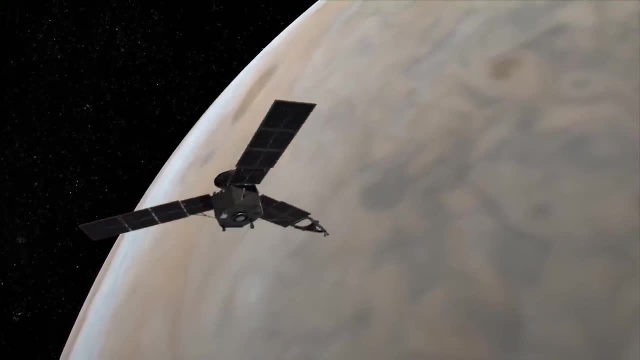 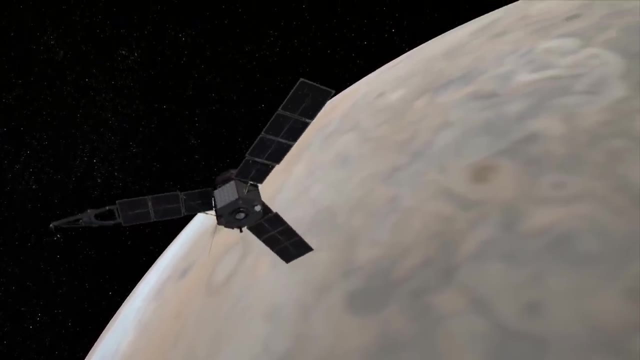 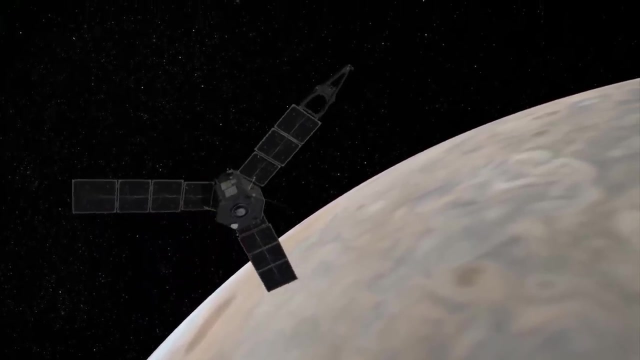 All instruments went offline and data was lost. It appeared to be similar to the difficulties experienced by Galileo, but engineers traced the issue to a data transfer problem from one specific instrument and the spacecraft remains healthy. Jupiter's axis is tilted at only three degrees. 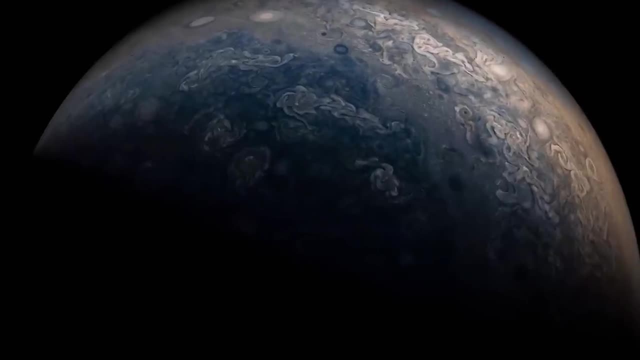 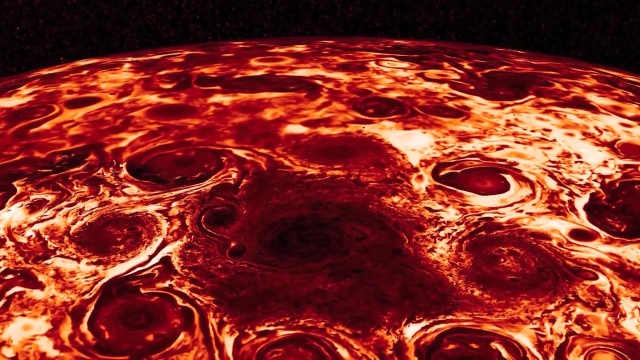 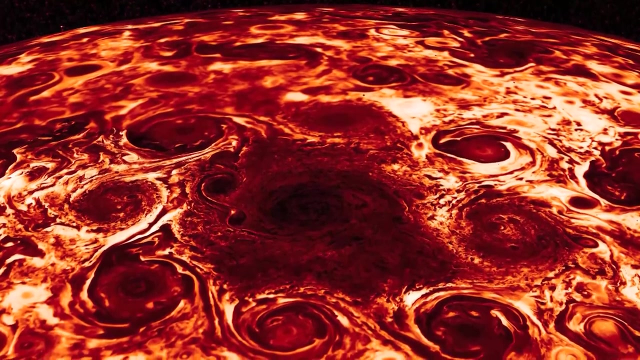 making even an oblique view of the poles near impossible until Juno arrived. When, viewed in the infrared, researchers saw a complex arrangement of storms at both the poles. At the north pole, a central vortex is surrounded by eight anticyclones. 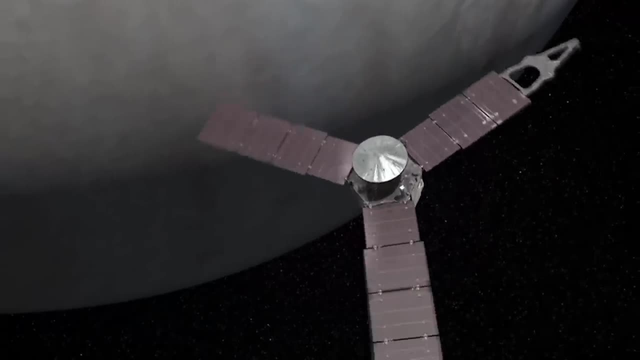 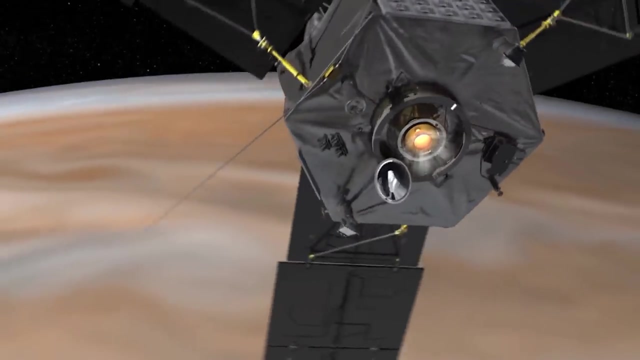 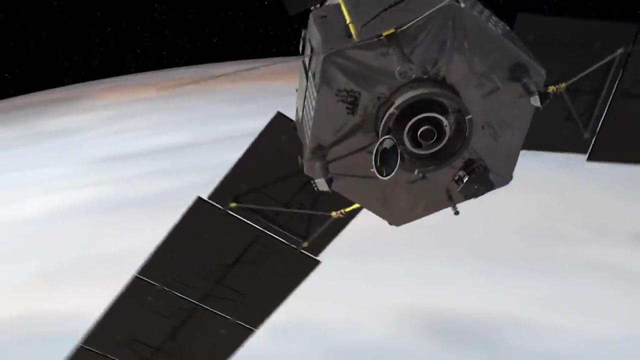 that would speed up the sampling rate. The spacecraft's main engine is fueled by hydrazine and nitrogen tetroxide, which ignite spontaneously when mixed. The propellant and oxidizer are forced out by a bladder of expanding helium As Juno was finishing its second orbit. 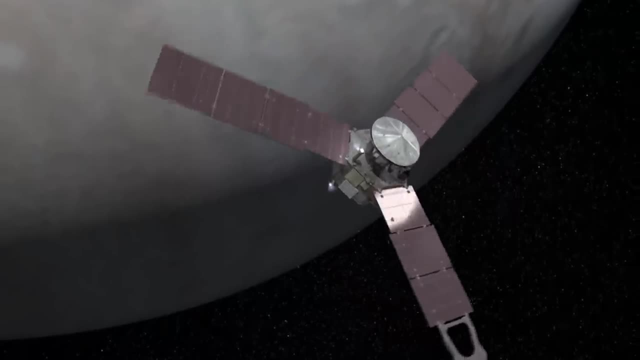 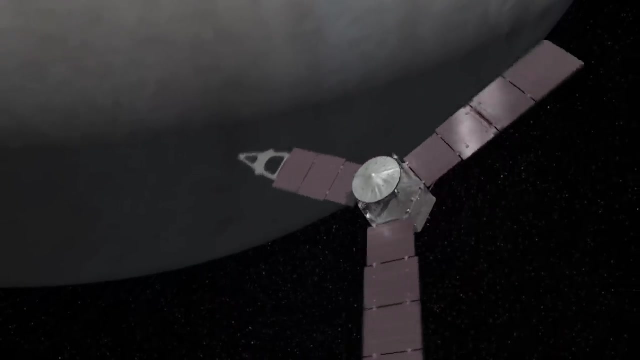 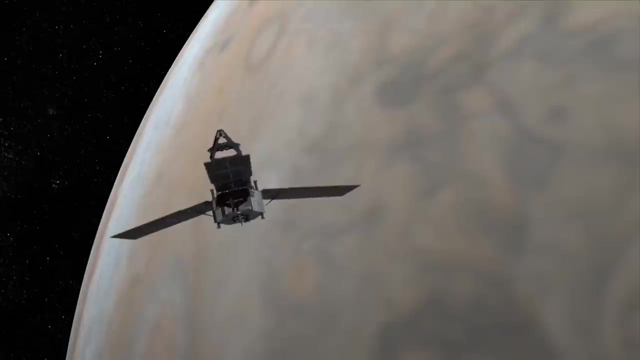 the helium valves were not responding correctly, so it was decided to maintain the original orbit. A mission extension has been granted to allow for the longer orbits Juno continues to follow. Within a day of the helium valve problem, Juno went into safe mode. 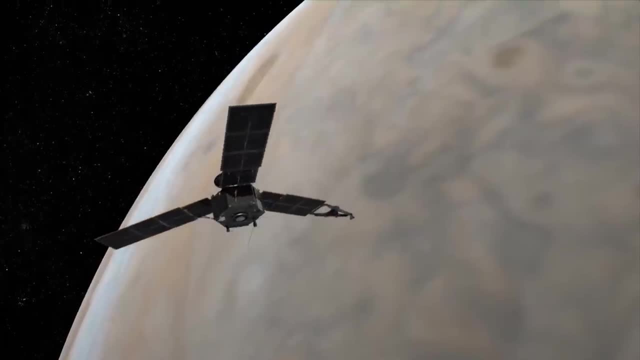 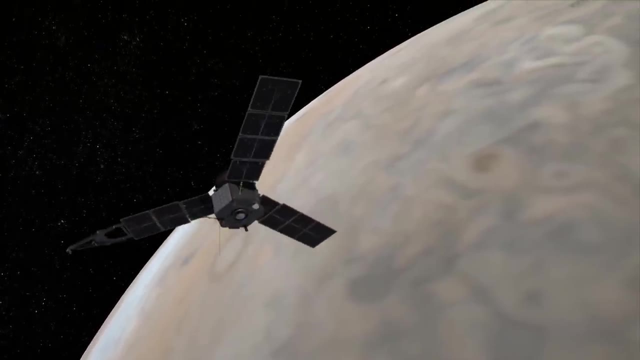 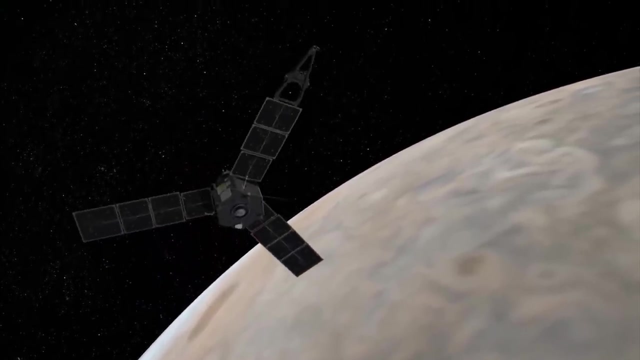 All instruments went offline and data was lost. It appeared to be similar to the difficulties experienced by Galileo, but engineers traced the issue to a data transfer problem from one specific instrument and the spacecraft remains healthy. Jupiter's axis is tilted at only three degrees. 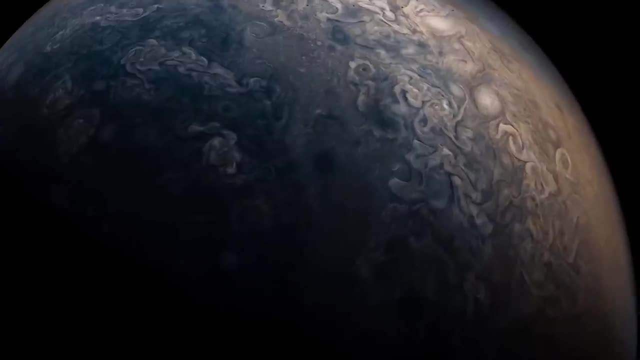 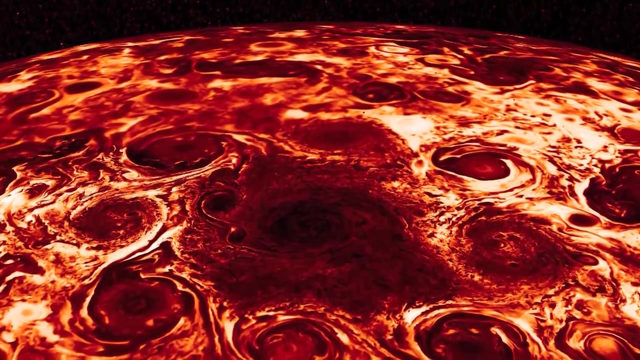 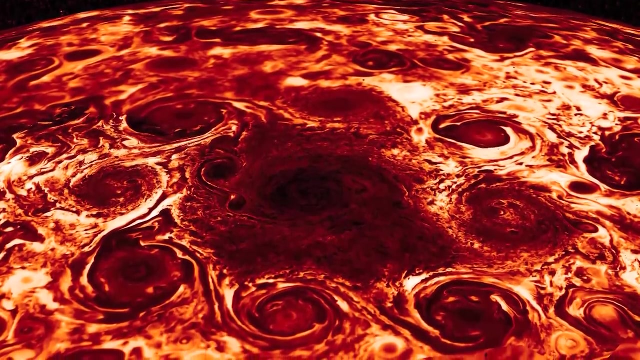 making even an oblique view of the poles near impossible until Juno arrived. When, viewed in the infrared, researchers saw a complex arrangement of storms at both the poles. At the north pole, a central vortex is surrounded by eight anticyclones. 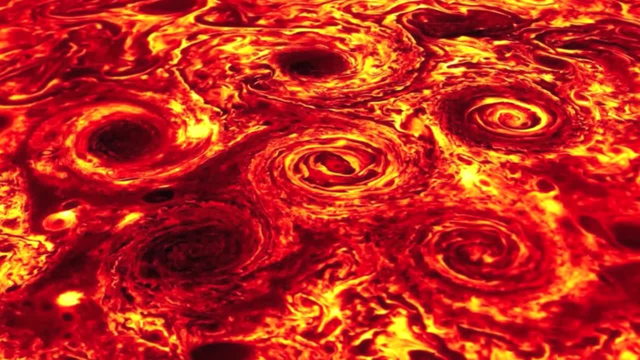 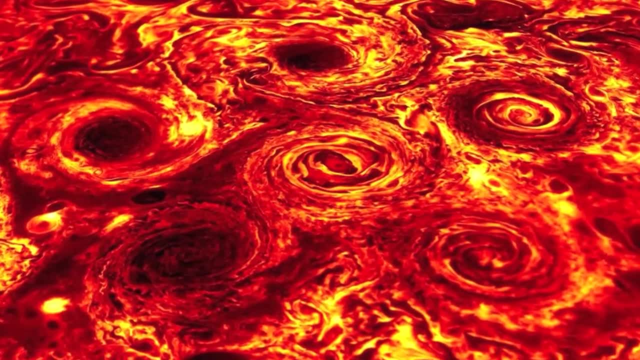 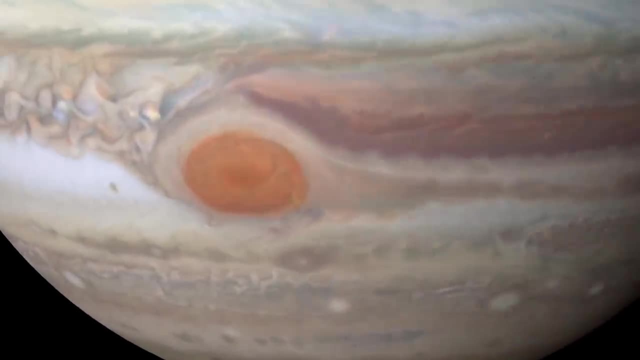 At the south pole, five anticyclones surround the central storm. Scientists do not understand why the storms, all rotating in the same direction, do not obliterate each other. On its seventh close pass of Jupiter, Juno flew directly over the giant red spot. 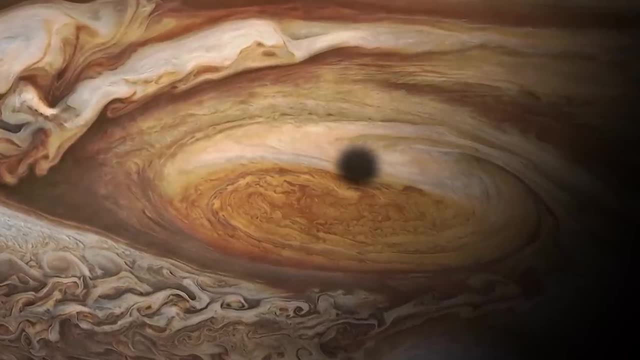 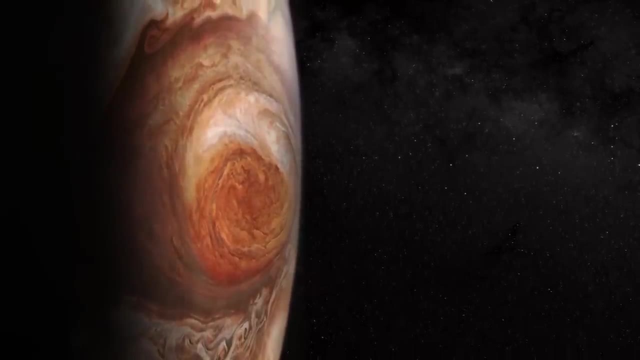 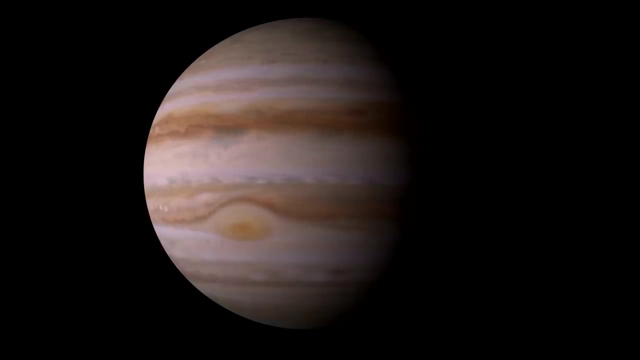 Its microwave radiometer was able to map the heat distributions at varying levels down to 350 kilometers. The red spot is a giant storm and Juno was able to see much higher temperatures at the deepest levels. they could penetrate With no geographic features as on Earth. 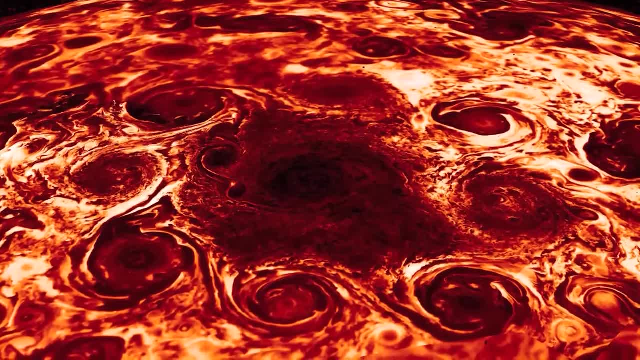 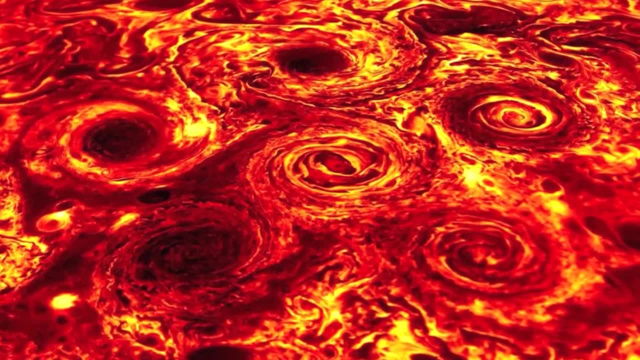 At the south pole, five anticyclones are surrounded by eight anticyclones. At the south pole, five anticyclones surround the central storm. Scientists do not understand why the storms, all rotating in the same direction, do not obliterate each other. 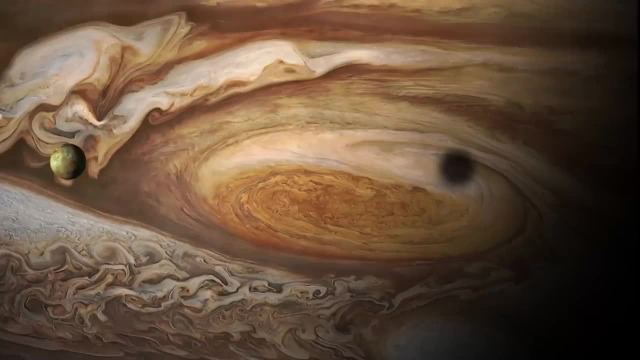 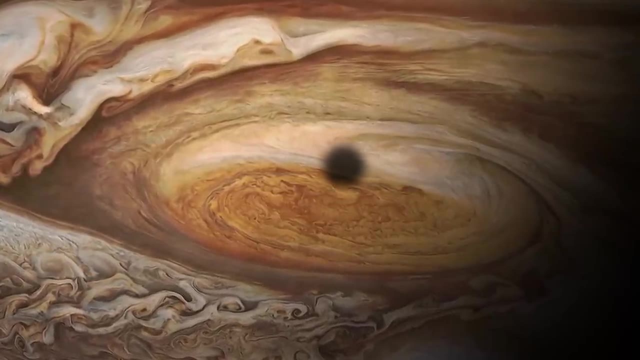 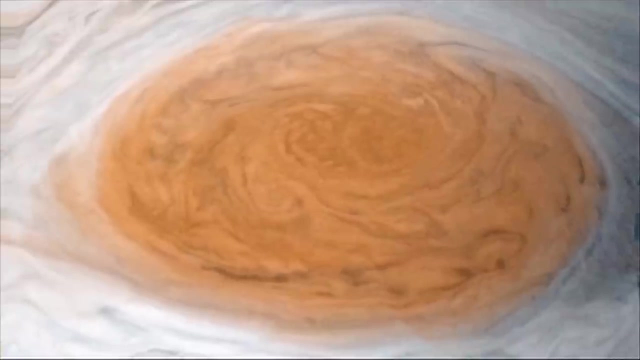 On its seventh close pass of Jupiter, Juno flew directly over the giant red spot. Its microwave radiometer was able to map the heat distributions at varying levels down to 350 kilometers. The red spot is a giant storm and Juno was able to see much higher temperatures. 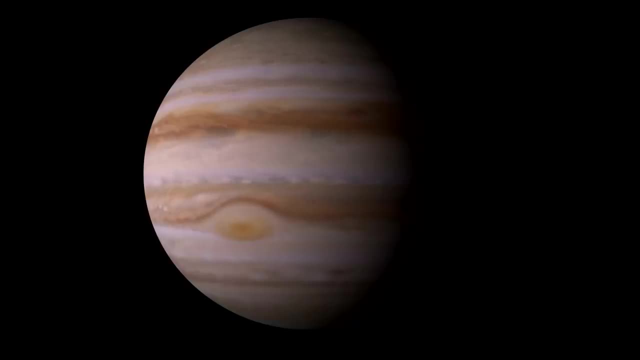 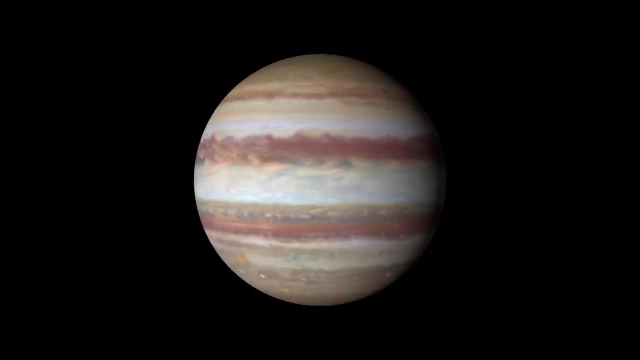 at the deepest levels they could penetrate With no geographic features. as on Earth, there is nothing on Jupiter against which storms can dissipate. The great red spot remains firmly 22 degrees below the equator, yet it appears to have drifted around the planet at least ten times. 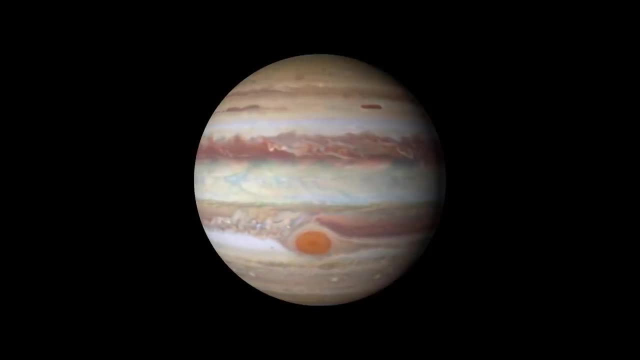 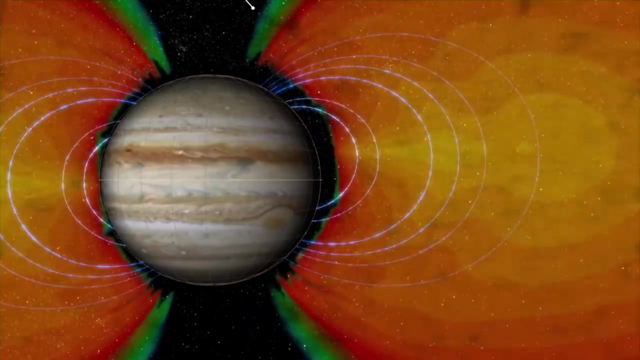 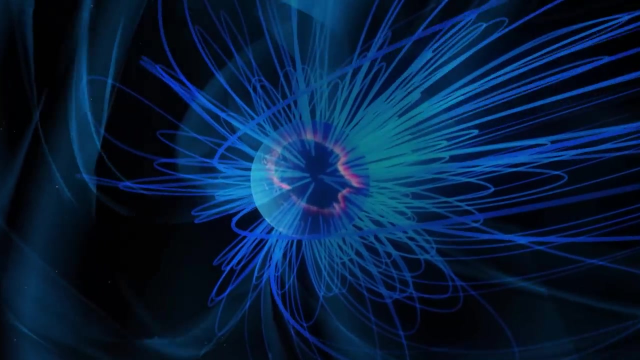 since reliable observations began. Jupiter's magnetosphere is huge. It traps charged particles in bands stretching out to vast distances. This gives sensitive electronics on orbiting spacecraft like Juno big problems. It was assumed that Jupiter's magnetosphere was generated, like Earth's, by dynamo action. 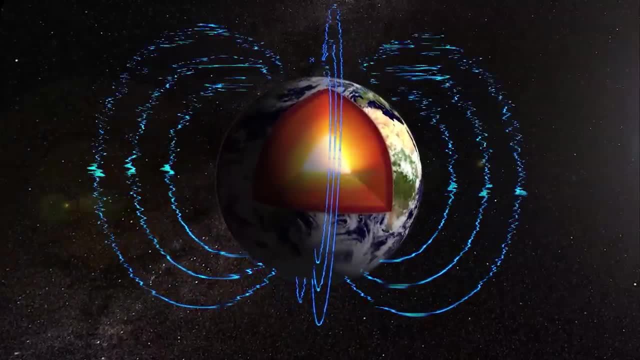 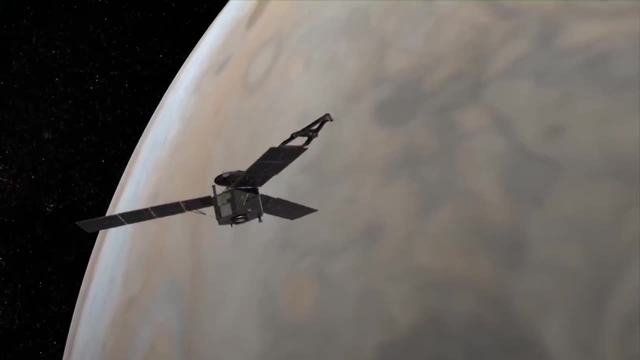 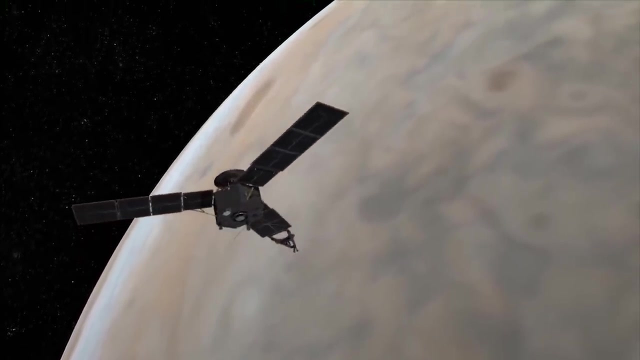 the convective movement of an electrically conductive fluid deep within. So far, results from Juno suggest that this is not the case. The lumpy nature of Jupiter's magnetic field points to an atmospheric source: The giant auroras at the poles. 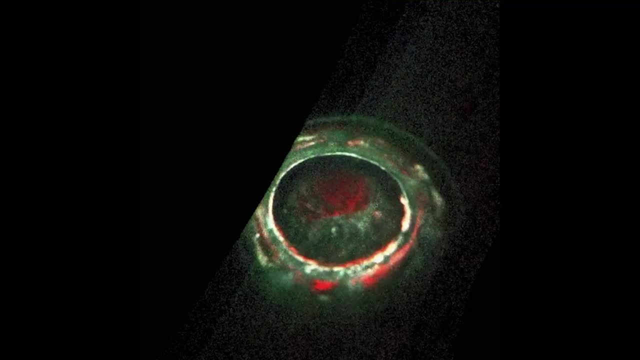 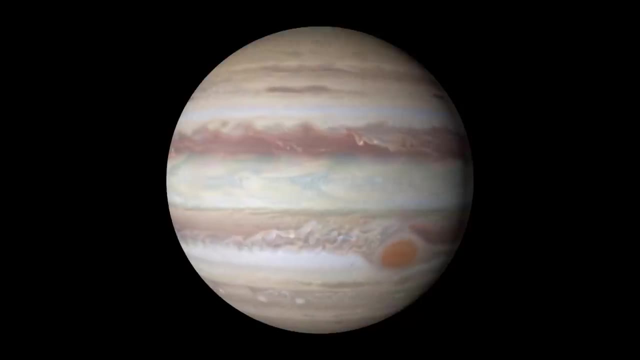 also seem to come from a different mechanism than here on Earth. By focusing on the composition of the gas giant, researchers are hoping to gather clues about conditions at the formation of the solar system, While the Earth has been continuously changed by tectonic forces. it is thought that Jupiter remains very similar in composition to the cloud of gas and dust from which the solar system was formed. At the end of its mission, Juno will be sent on a collision course with Jupiter to avoid any possible contamination of the delicate moons. 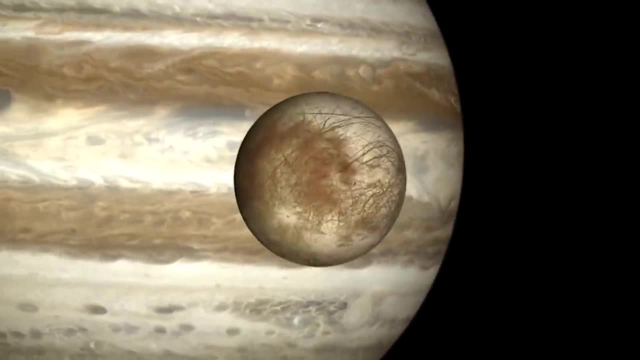 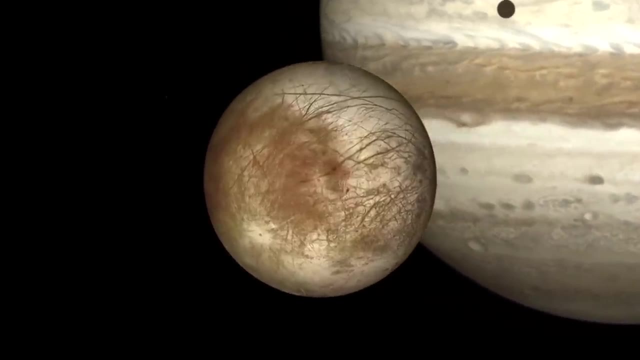 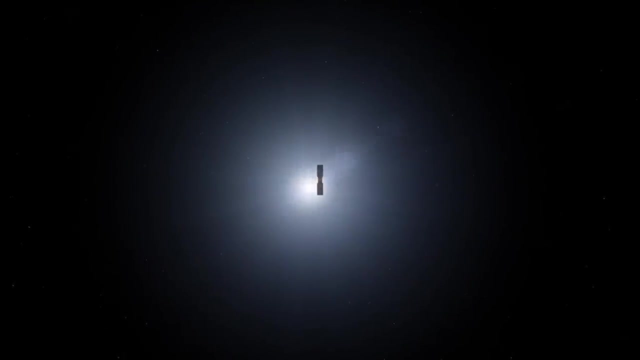 The next mission to the Jovian system will focus on Europa as the most likely place after Earth to harbor some form of life. Known as Europa Clipper, it's scheduled to launch in 2022.. Like Juno, it will be solar-powered. 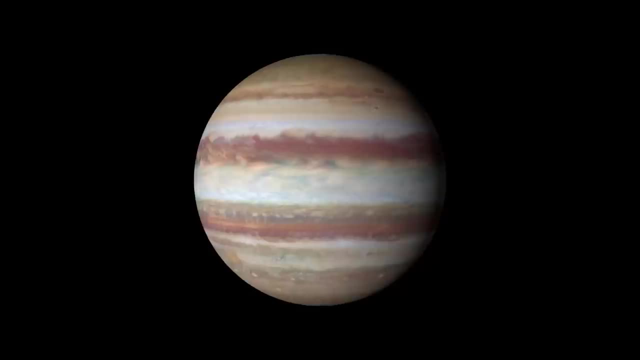 there is nothing on Jupiter against which storms can dissipate. The great red spot remains firmly 22 degrees below the equator, Yet it appears to have drifted around the planet at least ten times since reliable observations began. Jupiter's magnetosphere is huge. 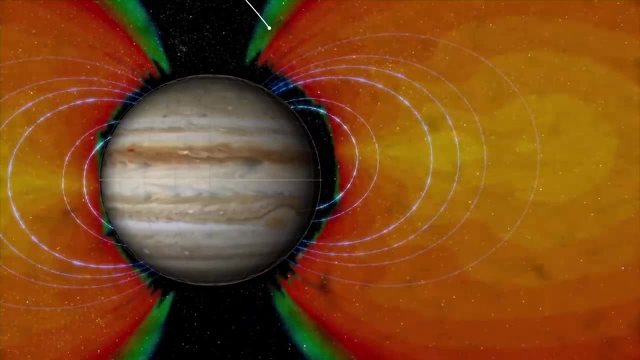 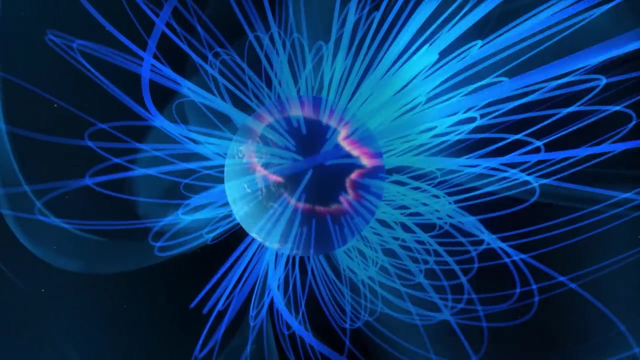 It traps charged particles in bands stretching out to vast distances. This gives sensitive electronics on orbiting spacecraft like Juno big problems. It was assumed that Jupiter's magnetosphere was generated, like Earth's, by dynamo action, the convective movement of an electrically conductive fluid deep within. 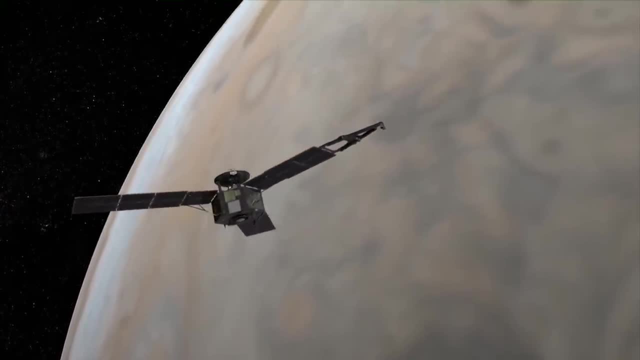 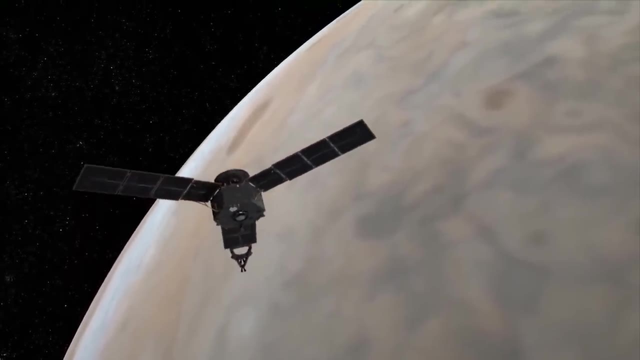 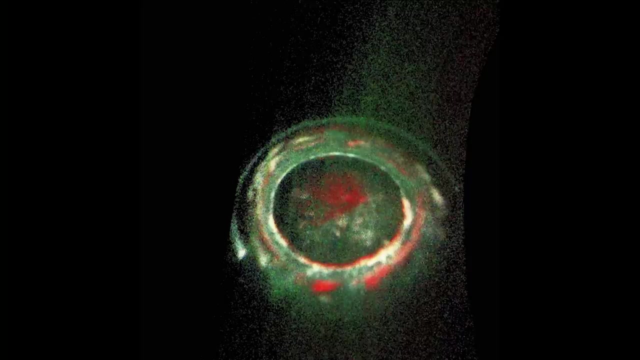 So far, results from Juno suggest that this is not the case. The lumpy nature of Jupiter's magnetic field points to an atmospheric source. The giant auroras at the poles also seem to come from a different mechanism than here on Earth, By focusing on the composition of the gas giant. 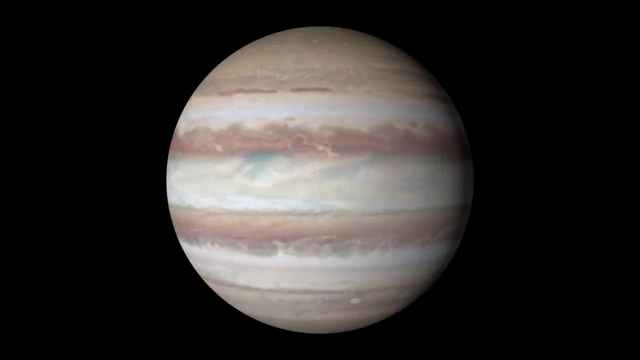 researchers are hoping to gather clues about conditions at the formation of the solar system. While the Earth has been continuously changed by tectonic forces, it is thought that Jupiter remains very similar in composition to the cloud of gas and dust from which the solar system was formed. 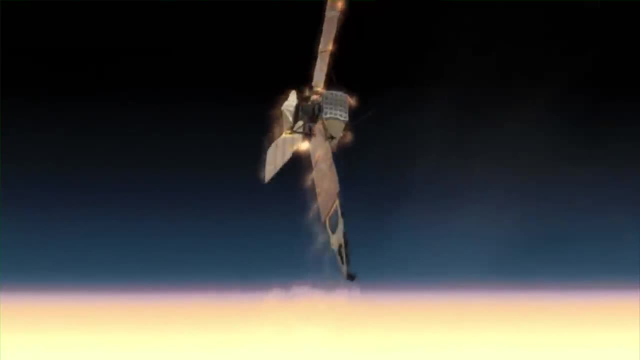 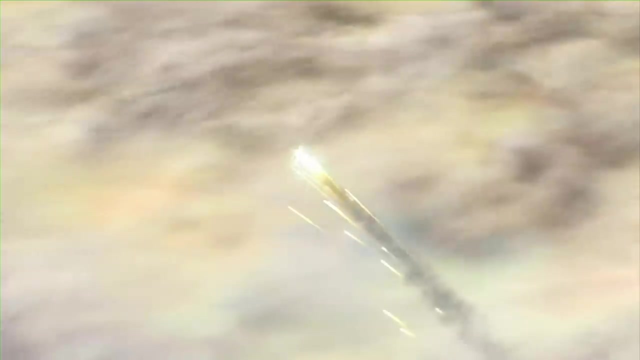 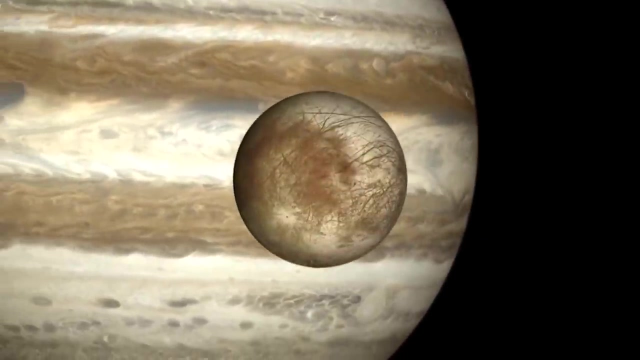 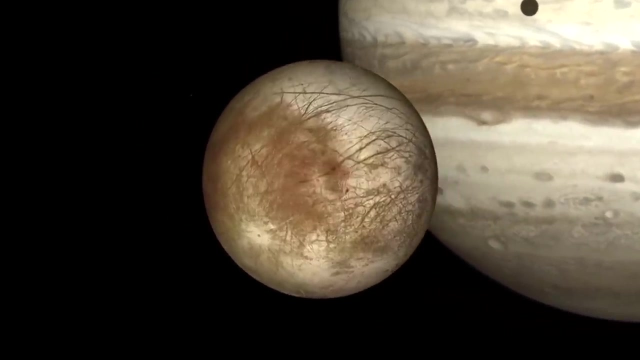 At the end of its mission, Juno will be sent on a collision course with Jupiter to avoid any possible contamination of the delicate moons. The next mission to the Jovian system will focus on Europa as the most likely place after Earth to harbour some form of life. 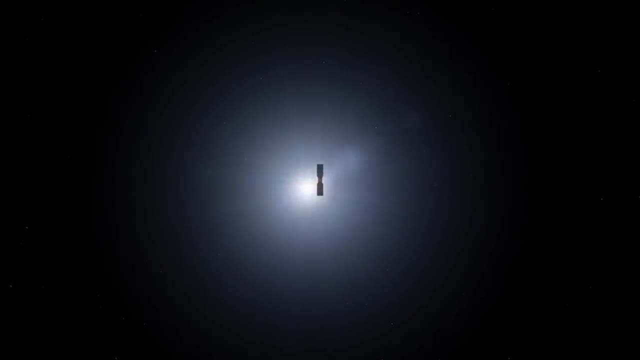 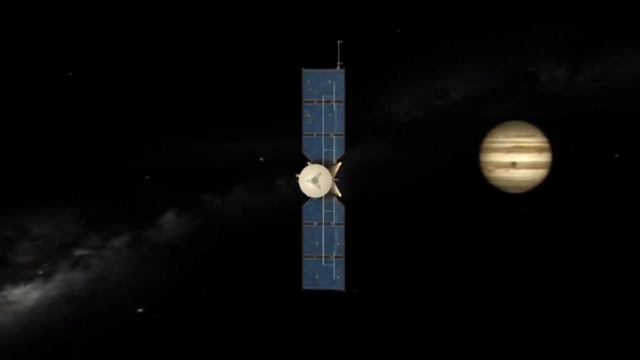 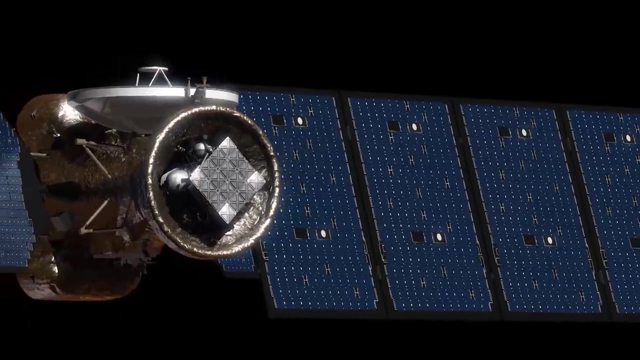 Known as Europa Comet. the Clipper is scheduled to launch in 2022.. Like Juno, it will be solar-powered and its elliptical orbit of Jupiter will see it fly over Europa every two weeks. Early concepts for the mission called for the inclusion of a lander. 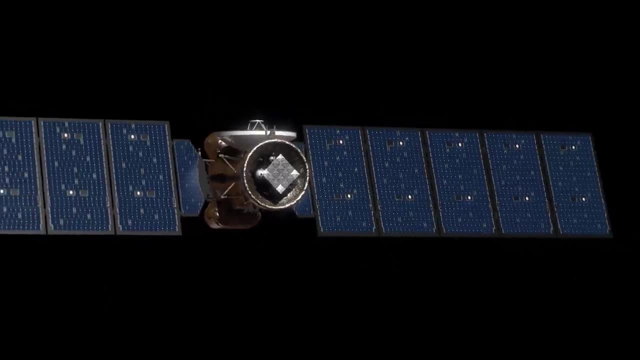 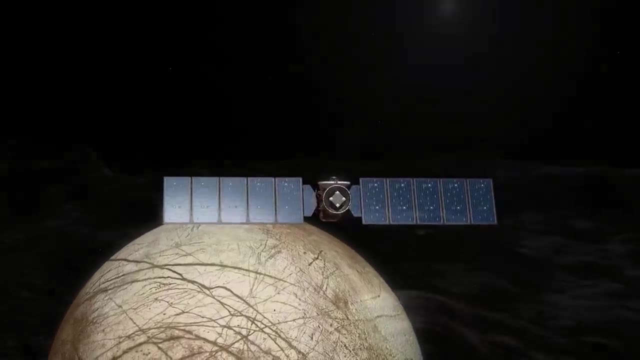 but this idea was soon rejected as premature because more needs to be learned about the surface of the icy moon. Europa's ice crust is thought to be at least 19 kilometres thick. Accurate measurements need to be made If thin areas can be found. 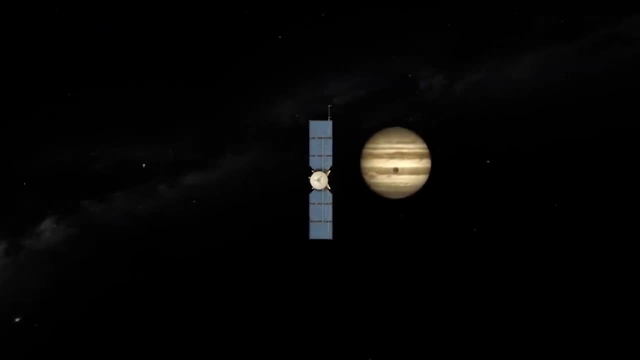 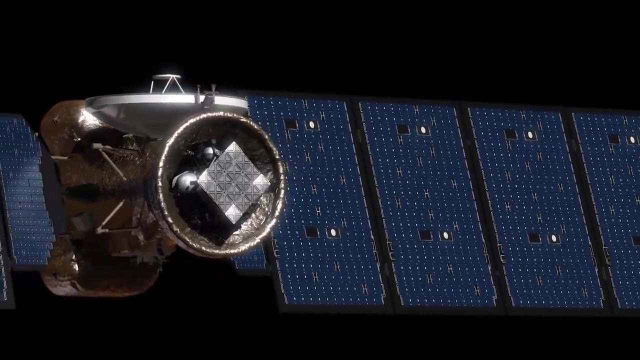 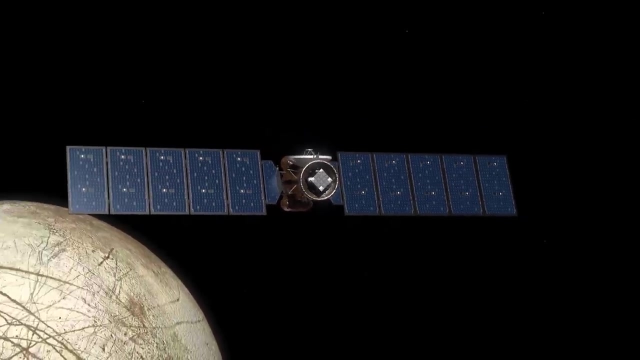 and its elliptical orbit of Jupiter will see it fly over Europa every two weeks. Early concepts for the mission called for the inclusion of a lander, but this idea was soon rejected as premature, because more needs to be learned about the surface of the icy moon. 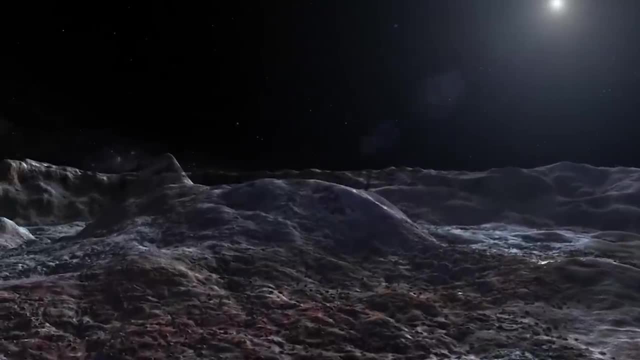 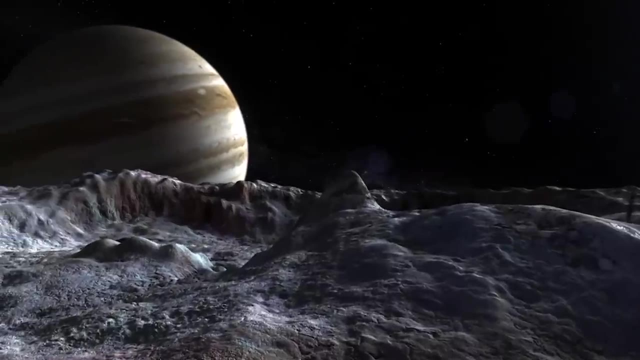 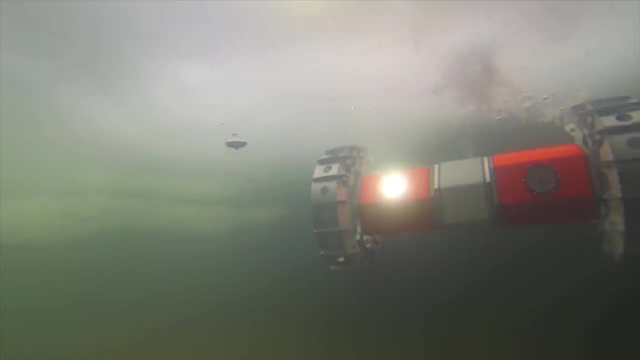 Though Europa's ice crust is thought to be at least 19 kilometers thick, accurate measurements need to be made. If thin areas can be found, then future missions may be able to access the ocean that lies beneath. Concepts for under-ice explorers are in development. 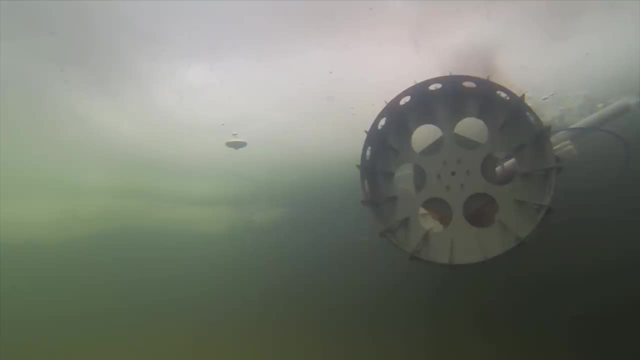 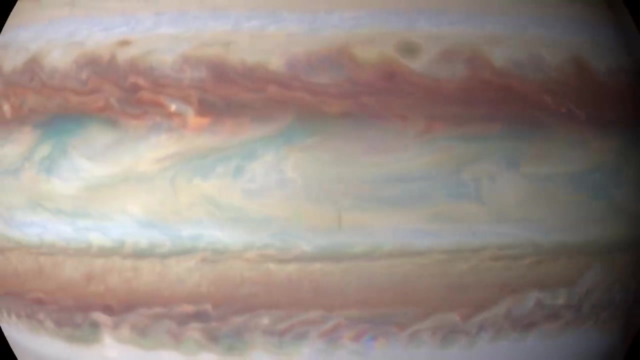 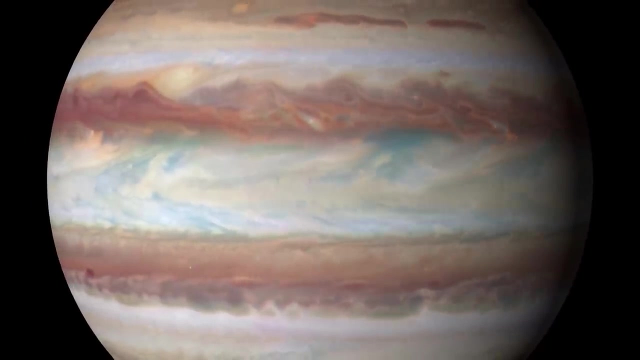 and we can expect other missions to focus on other moons. As the largest planet, Jupiter's influence on the rest of the solar system is profound. It has more than twice the mass of every other planet combined. All other planets' orbits are affected by Jupiter's gravitation. 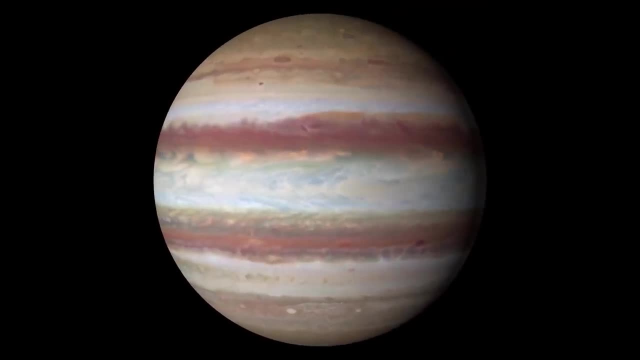 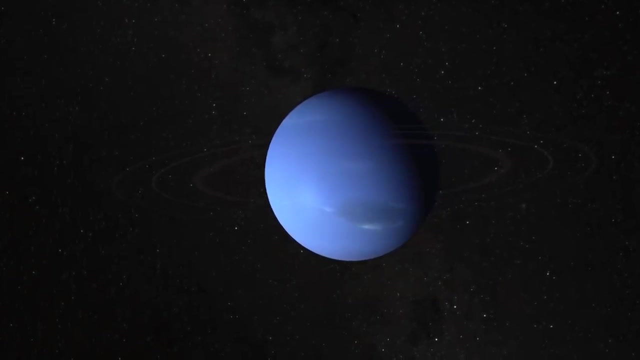 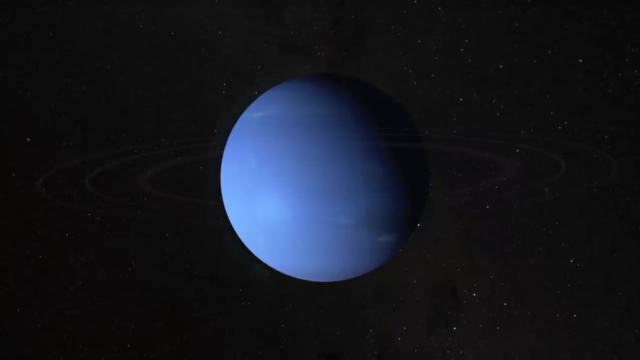 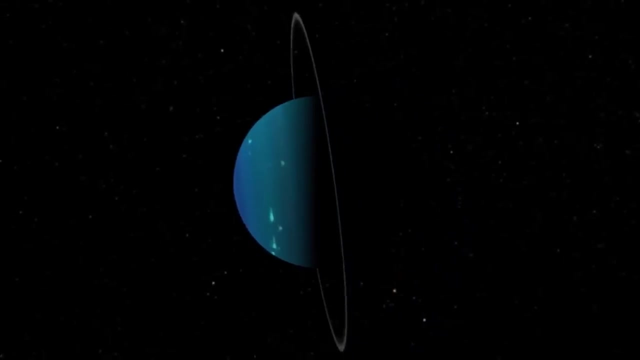 There is still much to learn about Jupiter. Some of our solar system's planets have been visited by scientific probes less frequently than others. The outer gas giants Uranus and Neptune are so distant they're hard to reach. Uranus is 20 times further from the Sun than Earth. 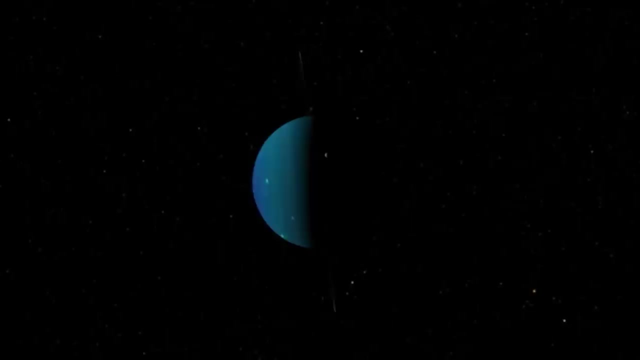 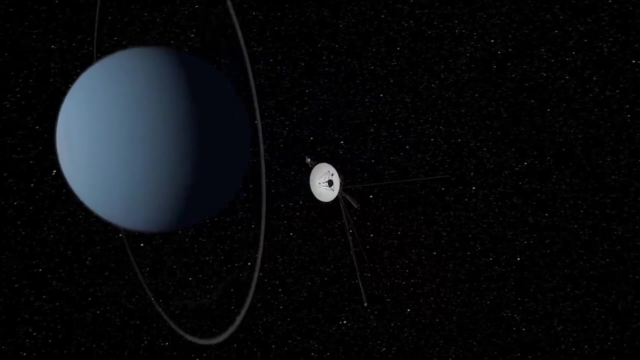 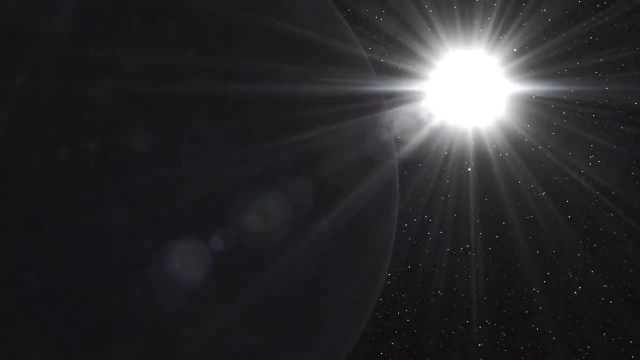 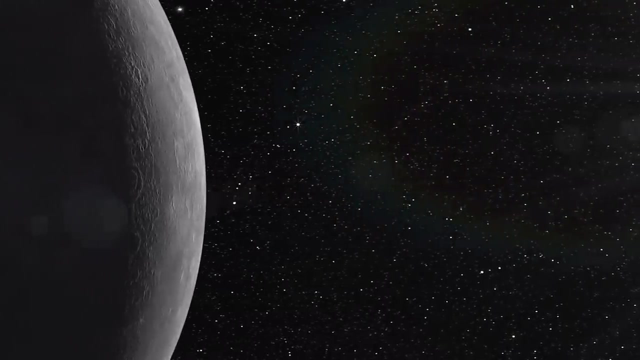 while Neptune is 30 times further. Both have only been seen at close range by NASA's Voyager 2 spacecraft. Mercury is so close to the Sun that any probe sent in its direction must take a circuitous path to offset the Sun's immense gravitational influence. 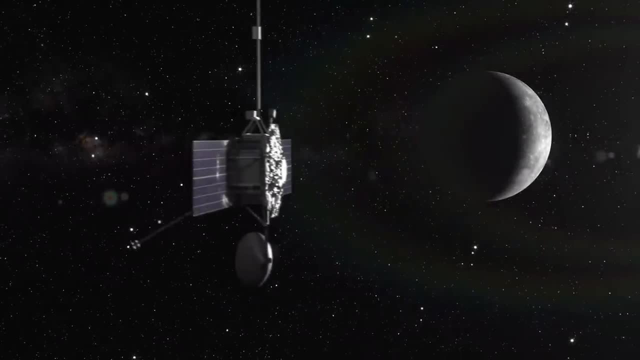 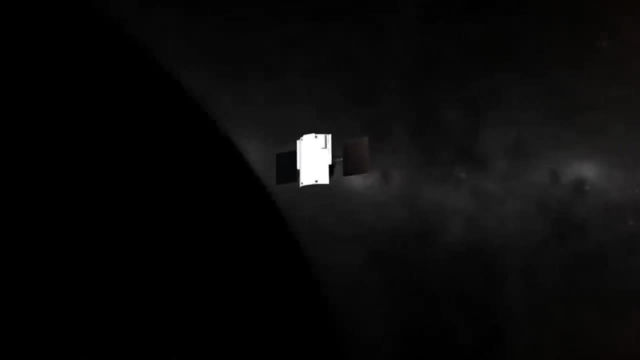 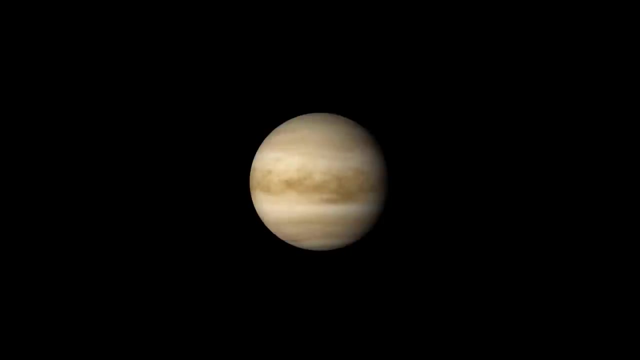 The Mariner 10 probe flew past Mercury in 1973, and the MESSENGER probe went into orbit around Mercury in 2011.. Venus presents different problems. Though it's our closest planetary neighbour and easier for spacecraft to reach, dense cloud hides its features. 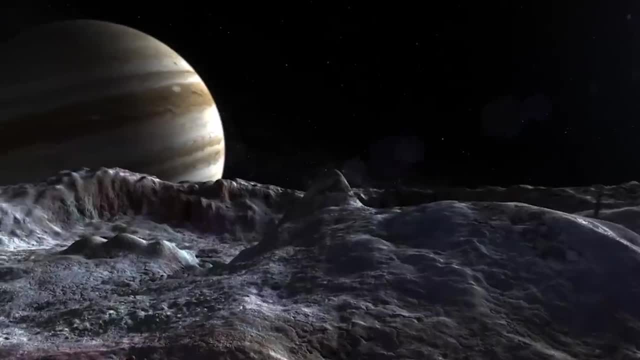 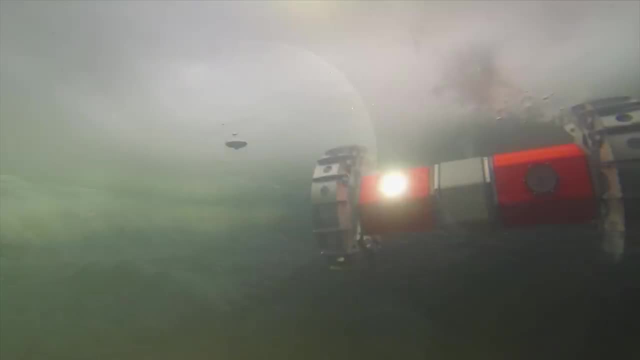 then future missions may be able to access the ocean that lies beneath. Concepts for under-ice explorers are in development, and we can expect other missions to focus on other moons. As the largest planet, Jupiter's influence on the rest of the solar system is profound. 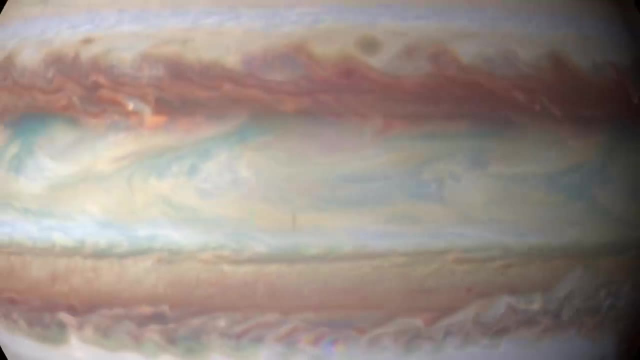 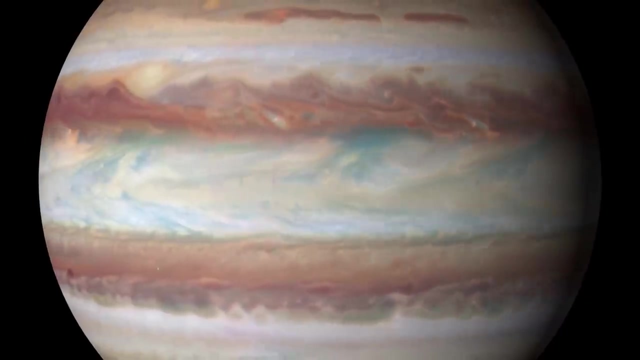 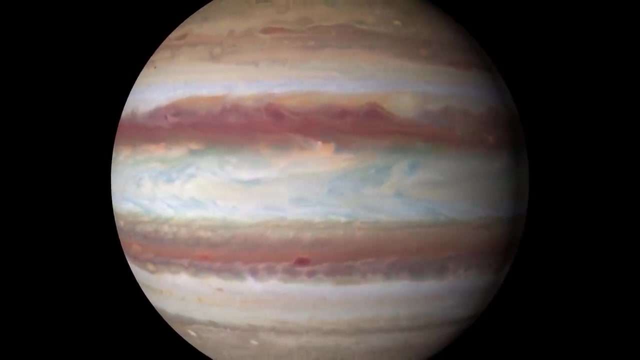 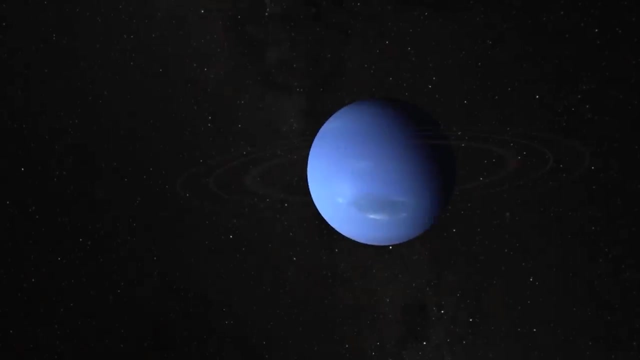 It has more than twice the mass of every other planet combined. All other planets' orbits are affected by Jupiter's gravitation. There is still much to learn about Jupiter. Some of our solar system's planets have been visited by scientific probes less frequently than others. 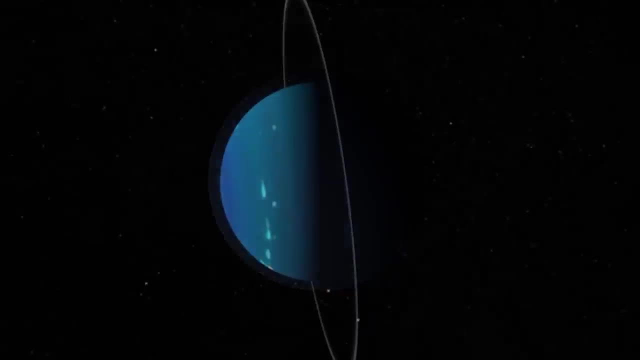 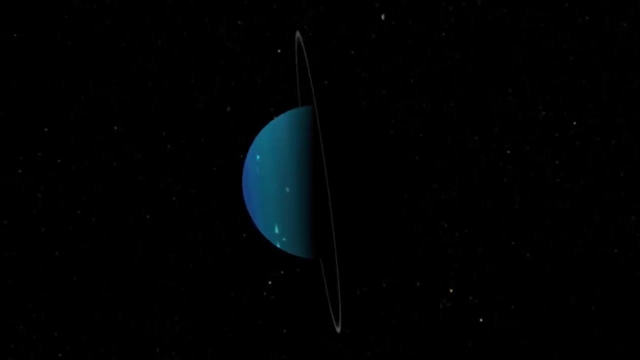 The outer gas giants Uranus and Neptune are so distant they're hard to reach. Uranus is 20 times further from the Sun than Earth, while Neptune is 30 times further. Both have only been seen at close range by NASA's Voyager 2 spacecraft. 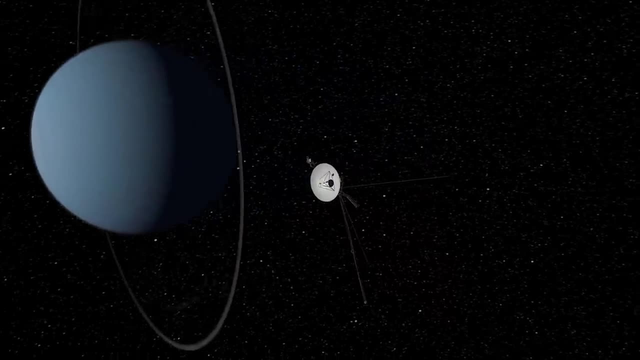 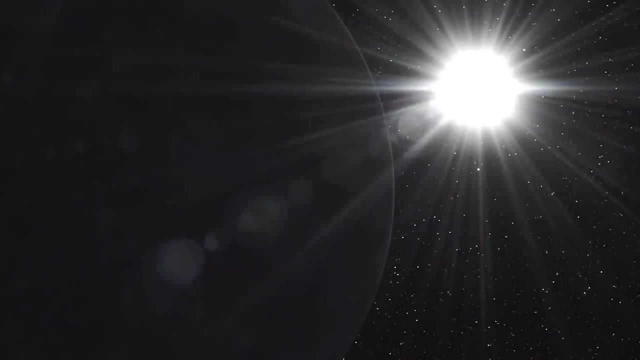 Mercury is so close to the Sun that any probe sent in its direction must take a circuitous path to offset the Sun's immense gravitational influence. The Mariner 10 probe flew past Mercury in 1973. It was the first probe sent in its direction. 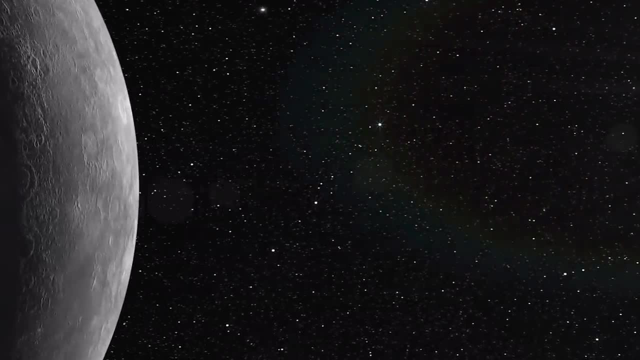 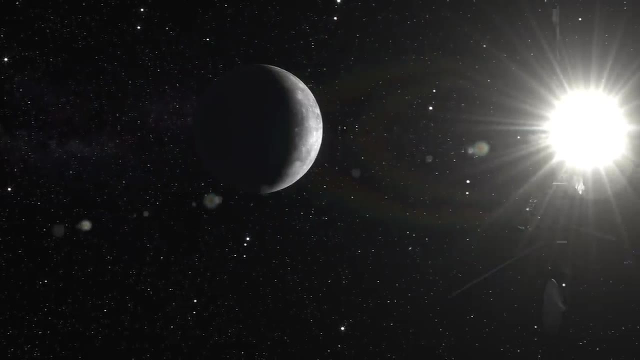 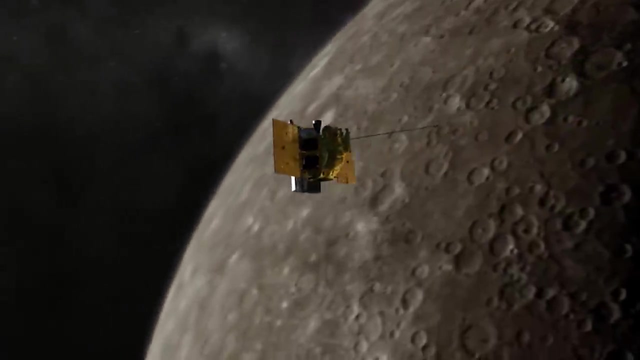 to take a circuitous path to offset the Sun's immense gravitational influence. The Mariner 10 probe flew past Mercury in 1973. And the MESSENGER probe went into orbit around Mercury in 2011.. Venus presents different problems. 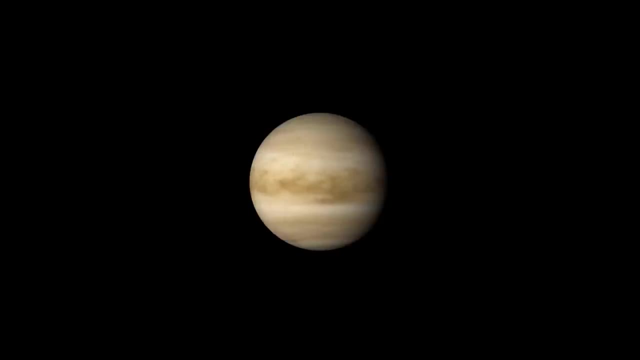 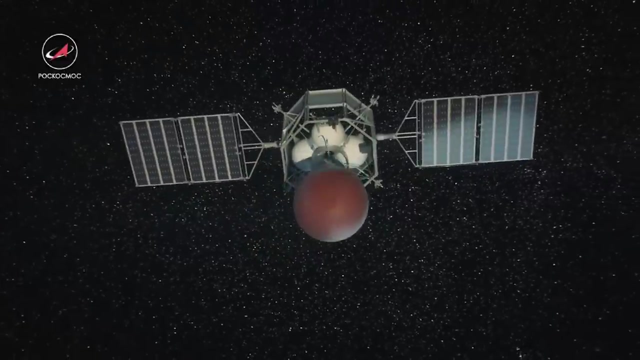 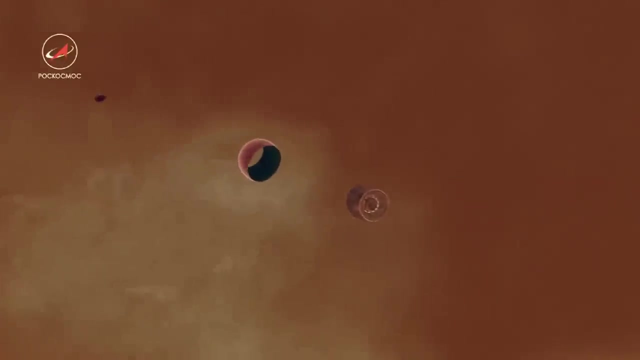 Though it's our closest planetary neighbour and easier for spacecraft to reach, dense cloud hides its features and its surface has hellish conditions and its surface has hellish conditions. The Russian Venera craft have landed, but in the hostile environment they could only survive for minutes. 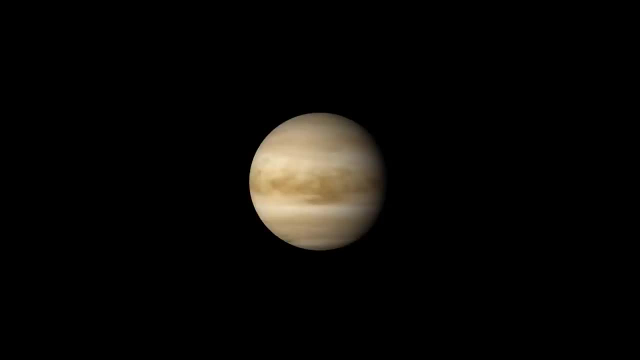 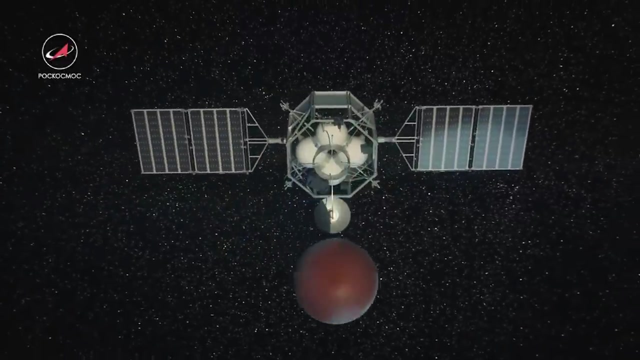 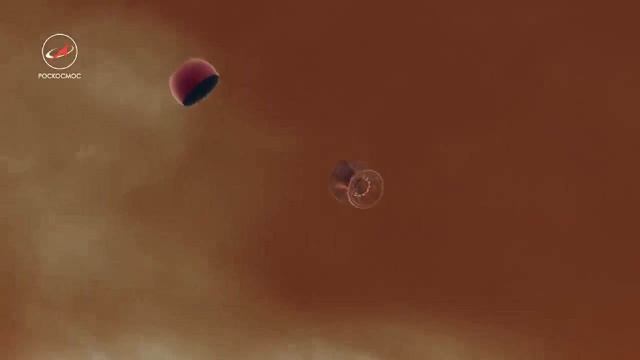 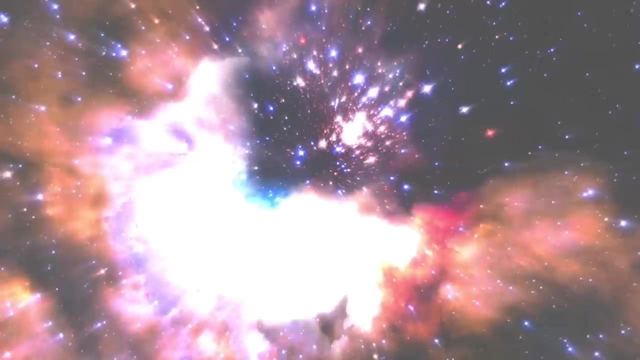 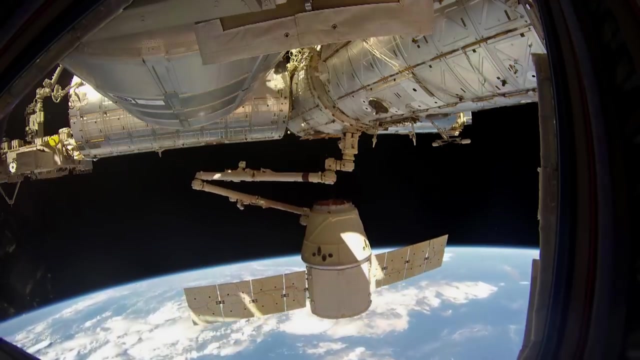 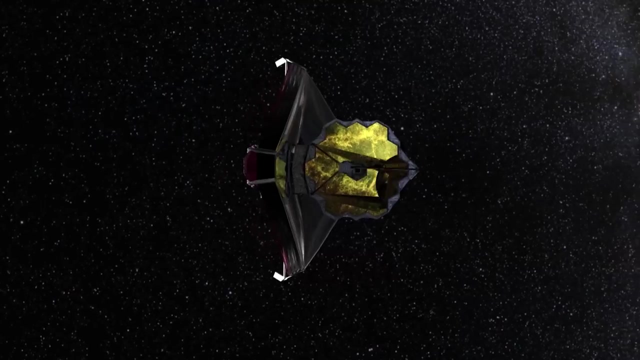 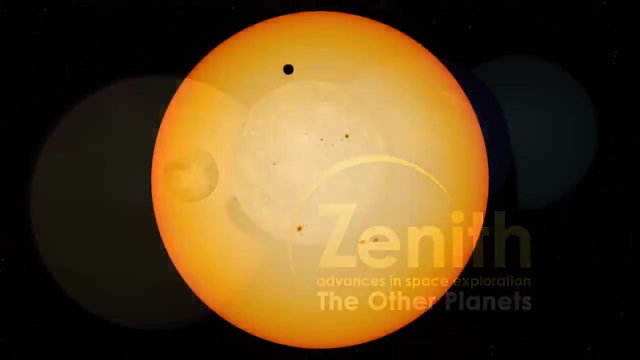 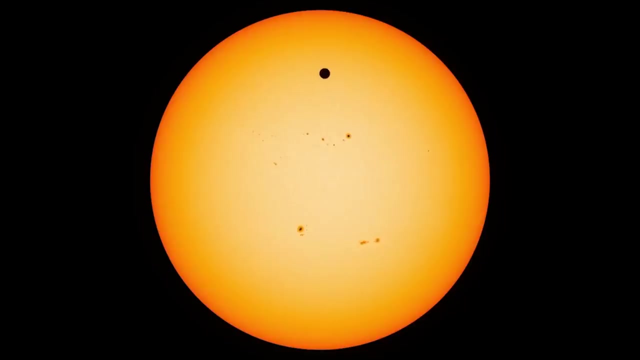 and its surface has hellish conditions. The Russian Venera craft have landed, but in the hostile environment they could only survive for minutes. NASA Jet Propulsion Laboratory, California Institute of Technology. roughly twice every century the planet Venus passes between the Earth and the Sun. Called the transit of Venus. it was closely observed in 1769.. Astronomers realised that careful timing of Venus's passage across the face of the Sun would allow them to calculate the distance to the Sun, which in turn would unlock far more accurate methods of navigation. 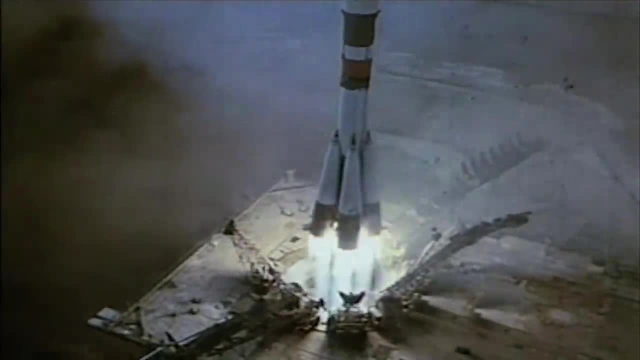 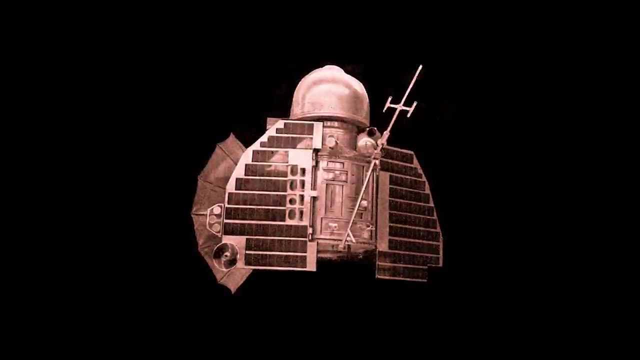 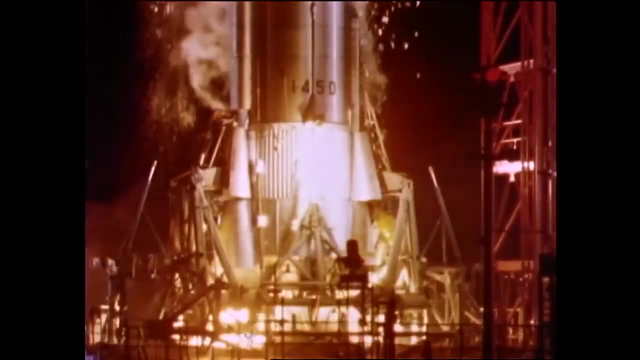 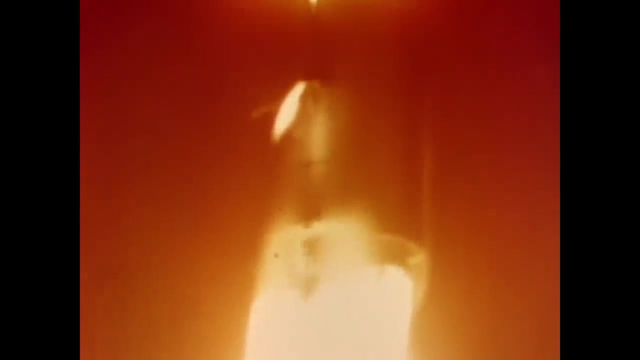 In 1961, the Soviet Union launched Venera 1, the first Venus probe. It passed Venus as intended, but mission control had lost contact with it. The following year, NASA launched Mariner 1 to Venus. We're not on trajectory. 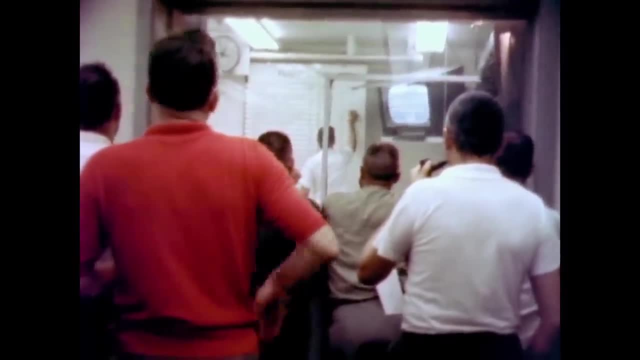 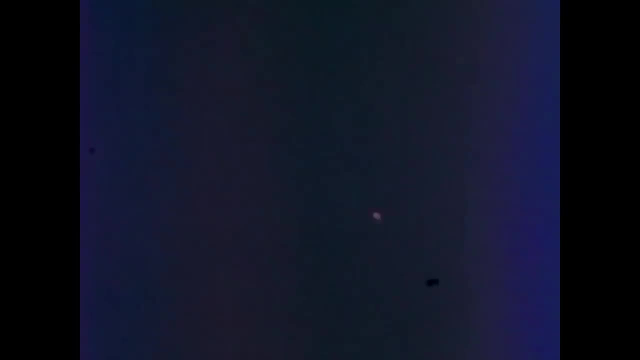 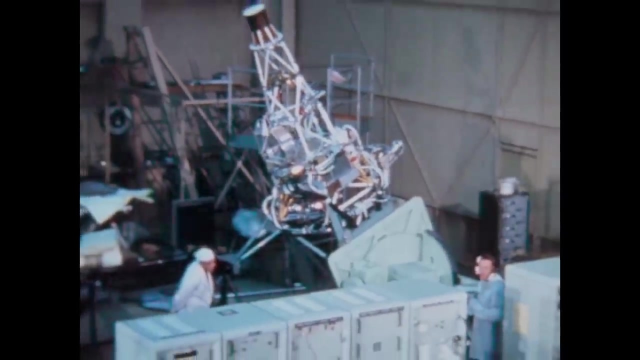 A coding error led to control problems with the launcher Destruct command. It was destroyed minutes after lift-off. This one apparently blew up Because convenient launch opportunities were limited, because convenient launch opportunities only occur in 18-month cycles. NASA had a second probe ready to launch. 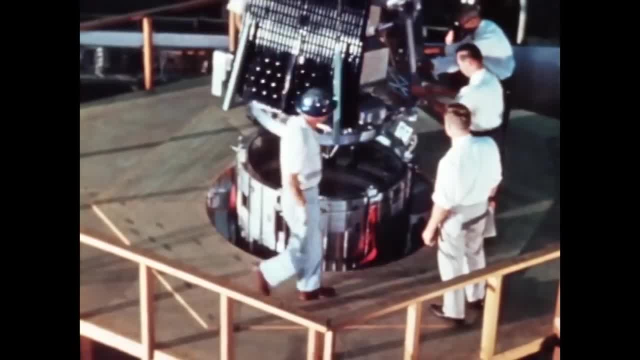 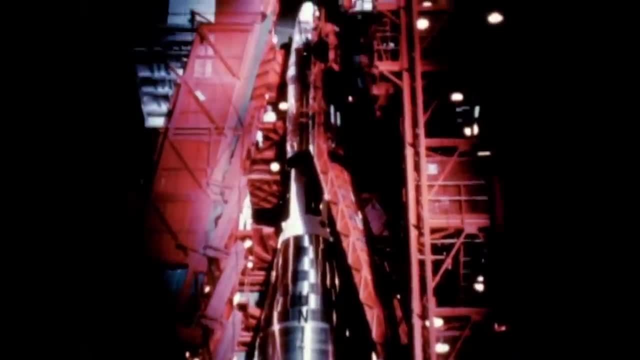 Mariner 2 was essentially a ranger spacecraft designed to go to the Moon. These were the early days of the space race and the United States was desperate to catch up with the Soviet Union. Lead times were short and the Jet Propulsion Laboratory 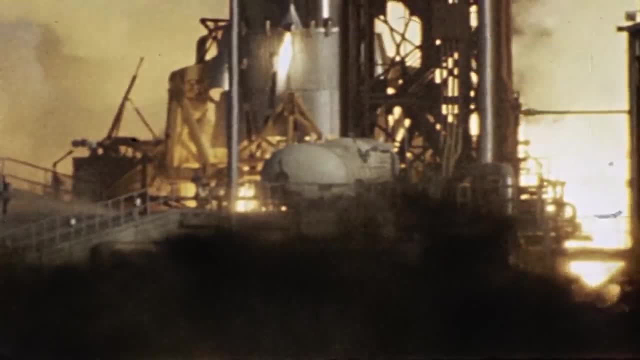 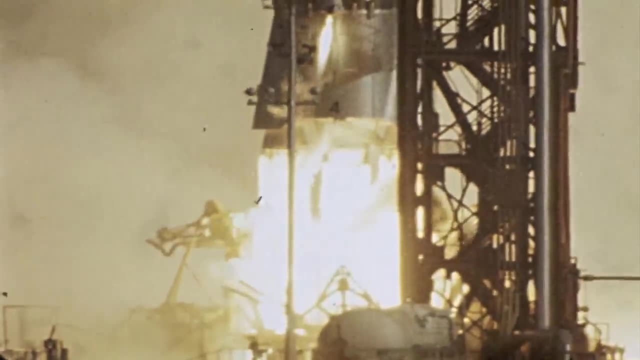 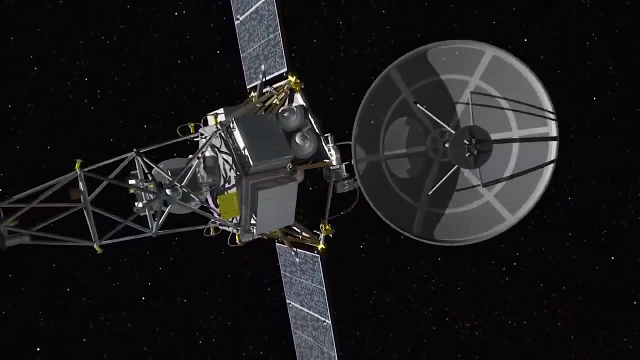 did not have time to complete its original design. In August 1962, Mariner 2 was launched. The ranger spacecraft launched toward the Moon had all failed. Mariner 2, on its way to Venus was functioning, but its transmissions were weak. 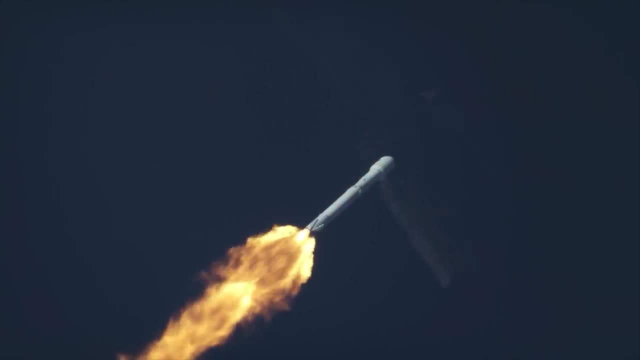 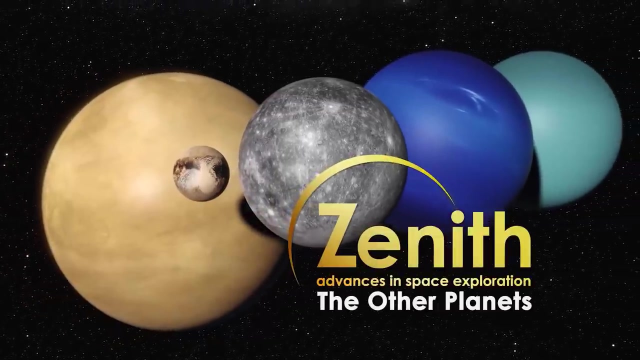 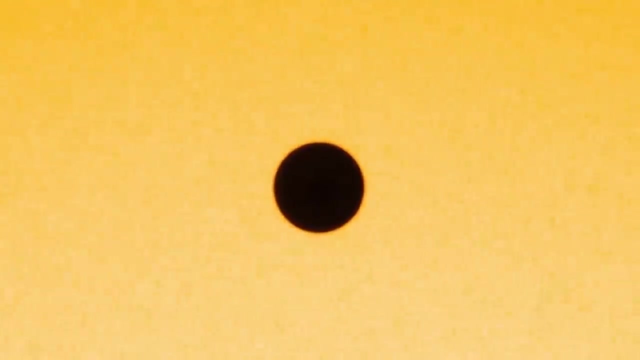 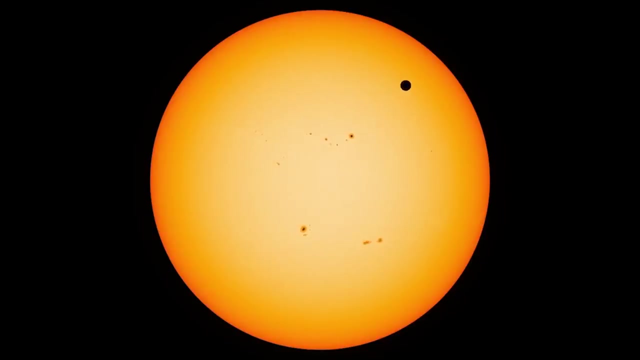 but in the hostile environment they could only survive for minutes. Roughly twice every century the planet Venus passes between the Earth and the Sun. Called the transit of Venus, it was closely observed in 1769.. Astronomers realised that careful timing. 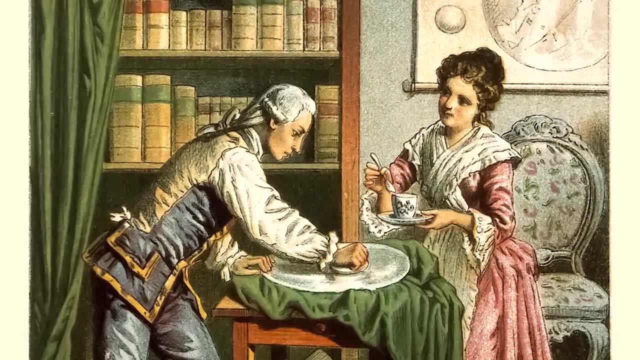 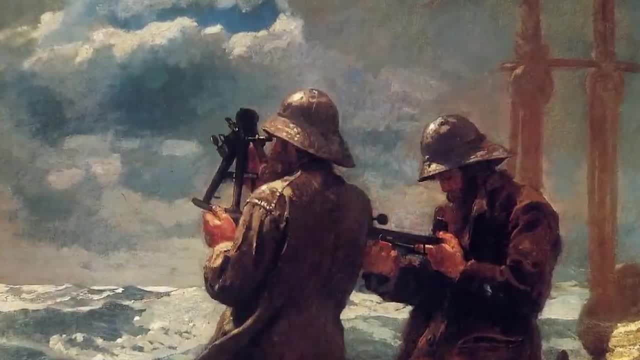 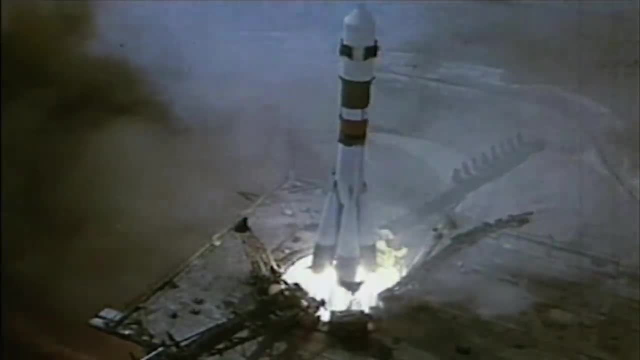 of Venus' passage across the face of the Sun would allow them to calculate the distance to the Sun, which in turn would unlock far more accurate methods of navigation. In 1961, the Soviet Union launched Venera 1, the first Venus probe. 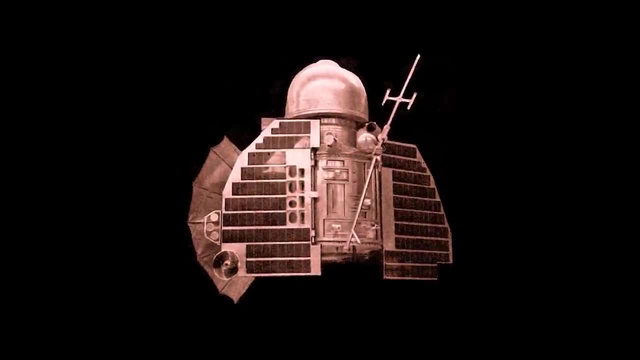 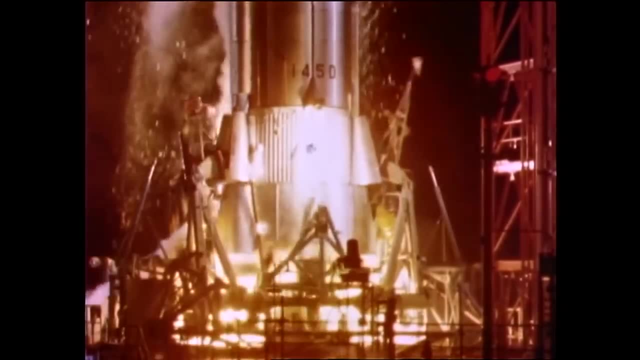 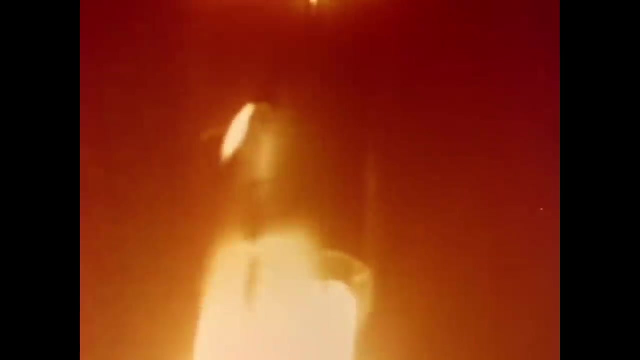 It passed Venus as intended, but mission control had lost contact with it. but mission control had lost contact with it. The following year, NASA launched Mariner 1 to Venus. We're not on trajectory. A coding error led to control problems with the launcher. 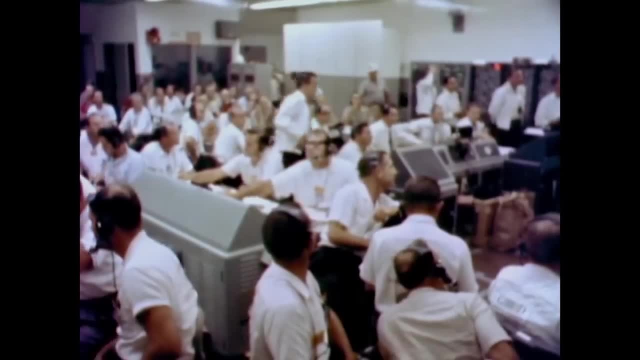 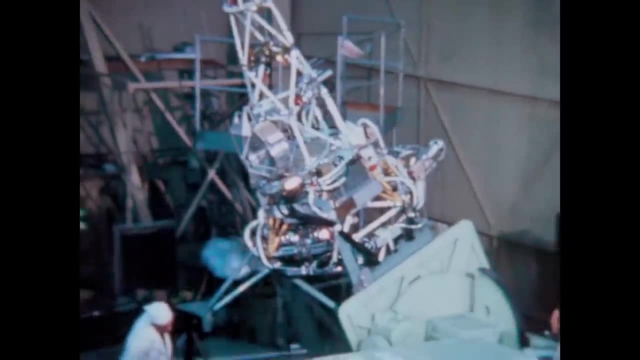 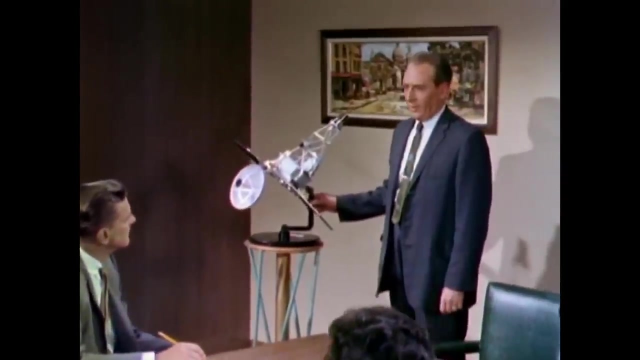 A coding error led to control problems with the launcher Destruct command. It was destroyed minutes after liftoff. This one apparently blew up Because convenient launch opportunities, Because convenient launch opportunities only occur in 18-month cycles- NASA had a second probe ready to launch. 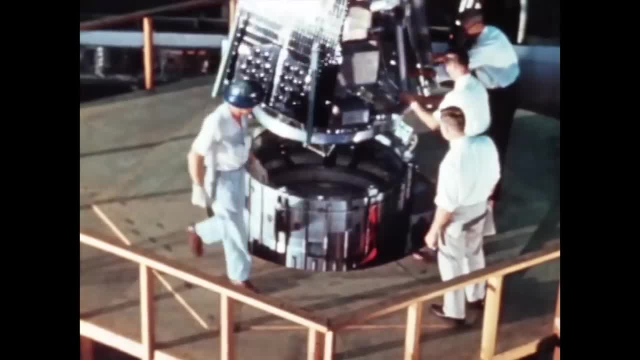 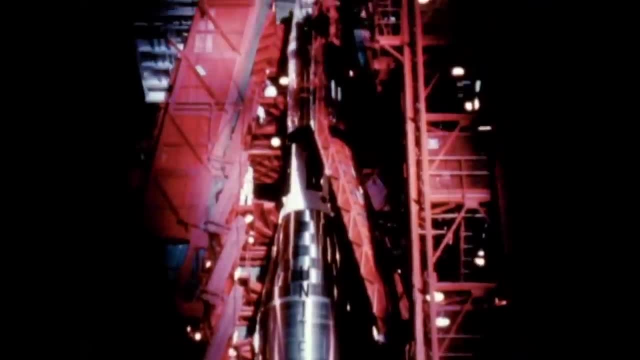 Mariner 2 was essentially a ranger spacecraft designed to go to the Moon. These were the early days of the space race and the United States was desperate to catch up with the Soviet Union. Lead times were short and the Jet Propulsion Laboratory 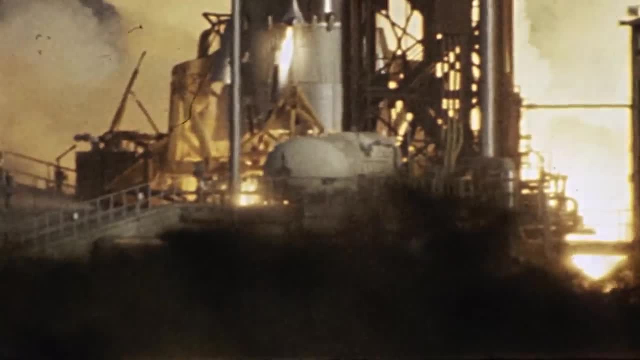 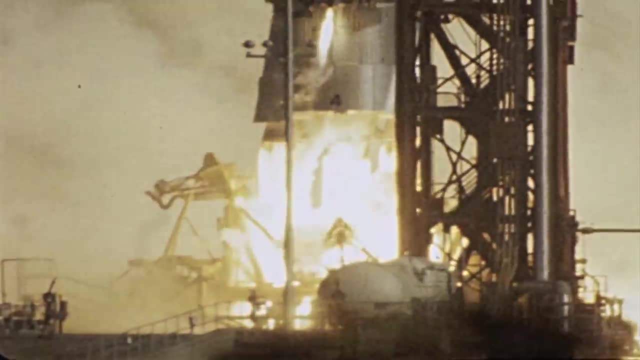 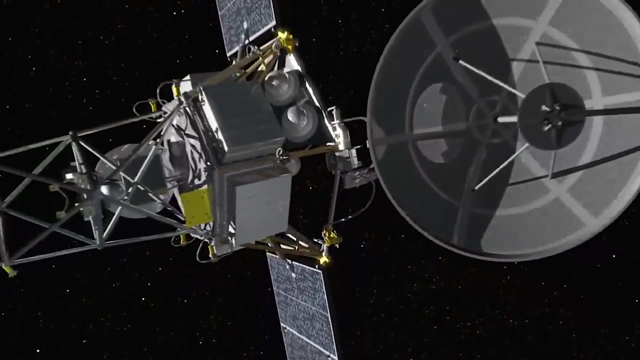 did not have time to complete its original design. In August 1962, Mariner 2 was launched. In August 1962, Mariner 2 was launched. In August 1962, Mariner 2 was launched. The ranger spacecraft launched toward the Moon. 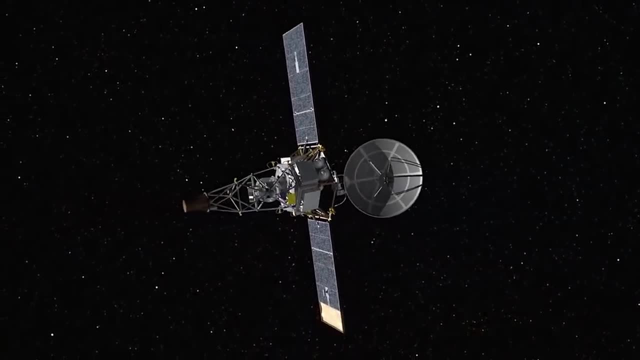 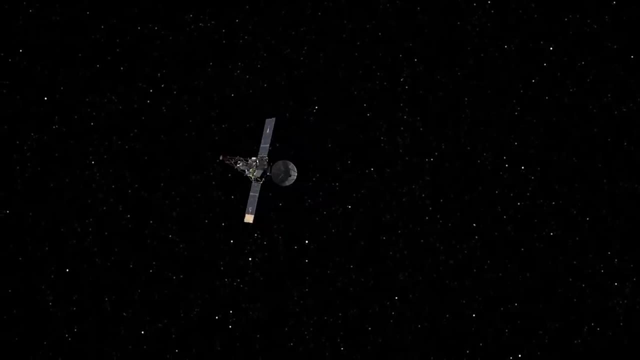 had all failed. Mariner 2, on its way to Venus was functioning, but its transmissions were weak and, due to a launch anomaly, it was off course. it was off course After a week. instructions for a complex course correction. 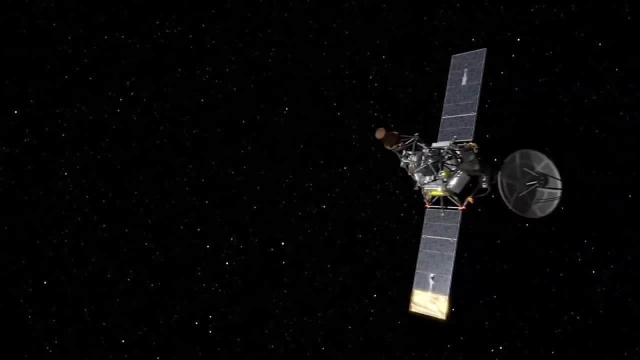 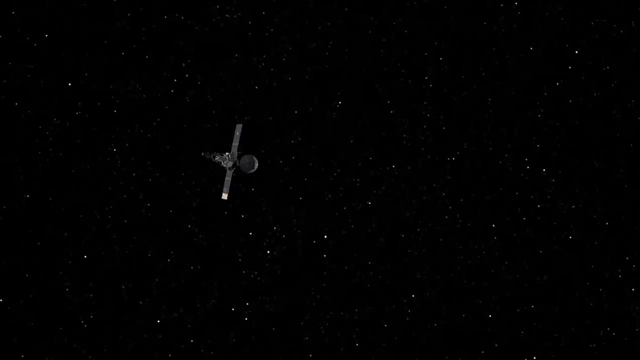 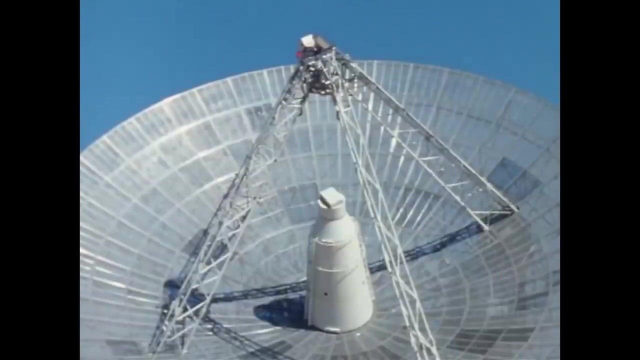 and, due to a launch anomaly, it was off course. After a week, instructions for a complex course correction were sent to NASA. About an hour later, Mariner executed the maneuver, which involved a roll turn followed by a pitch turn and finally a main engine burn. 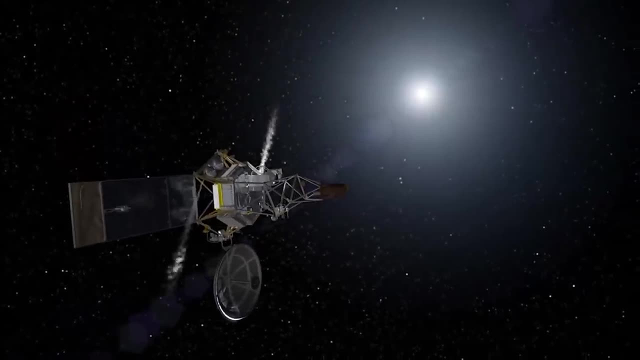 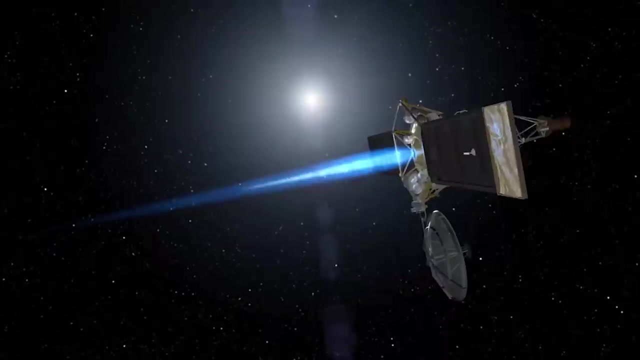 It worked well, but several days later the craft lost lock on the Sun and the Moon and the spacecraft was shut down. This was the first time the spacecraft had ever been shut down. It was the first time the spacecraft had ever been shut down. 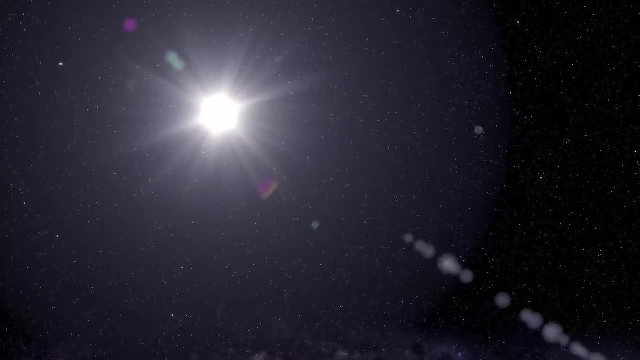 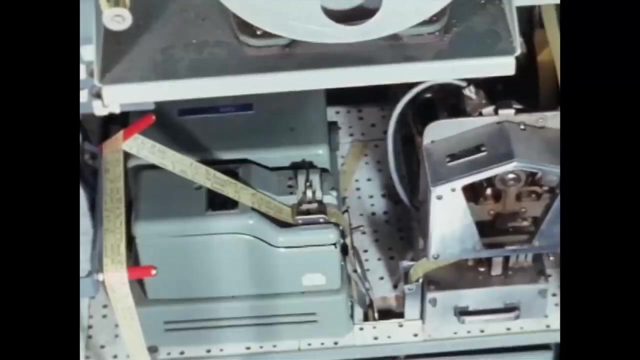 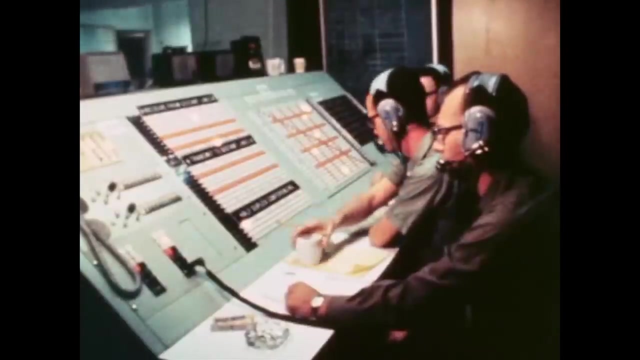 The spacecraft lost lock on the Sun and the Earth, its two attitude reference points. It corrected itself before ground control could diagnose the problem. Next, the signal strength increased to its normal level, but a short in a solar panel left it low on power. 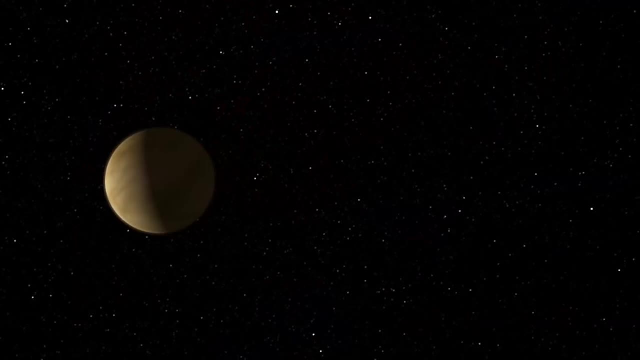 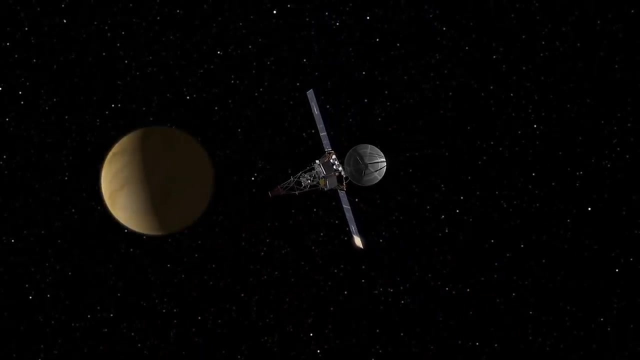 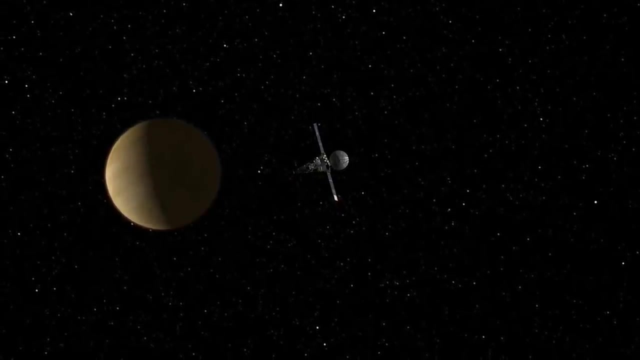 At this time, although both America and the Soviet Union had been sending probes toward the planets, nothing had succeeded. Mariner 2 lost several planetary sensors and it began to overheat. It continued limping toward Venus, but some of the spacecraft's problems 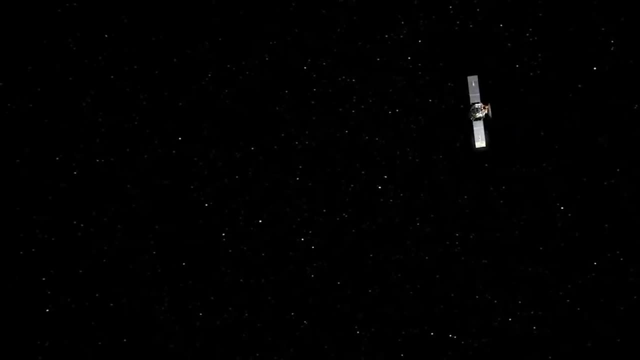 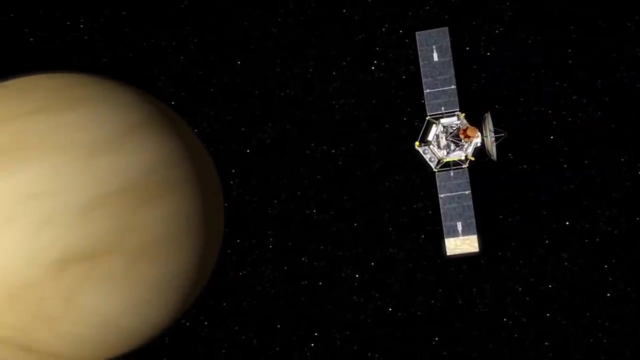 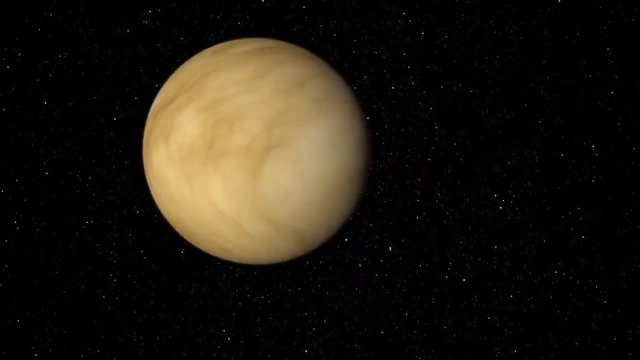 were solving themselves. Mariner 2 was now close enough to the Sun that it could function effectively on just one solar panel. It passed slightly less than 35,000 kilometers above Venus's cloud tops, It could detect no planetary magnetic field and it recorded temperatures. 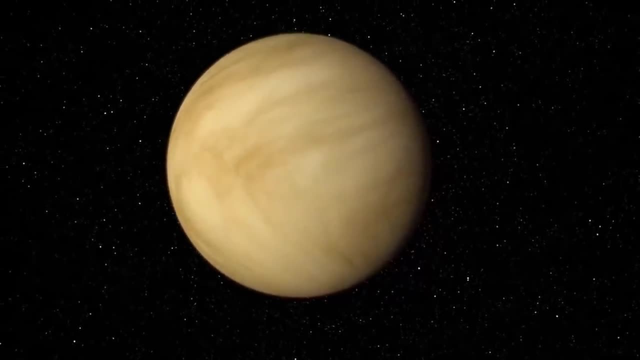 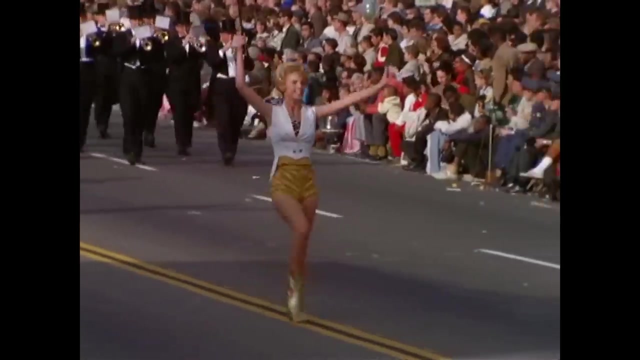 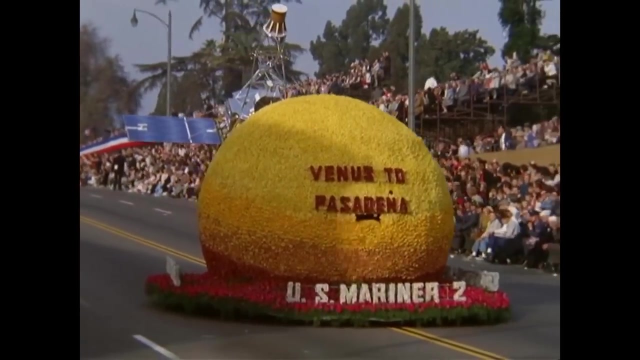 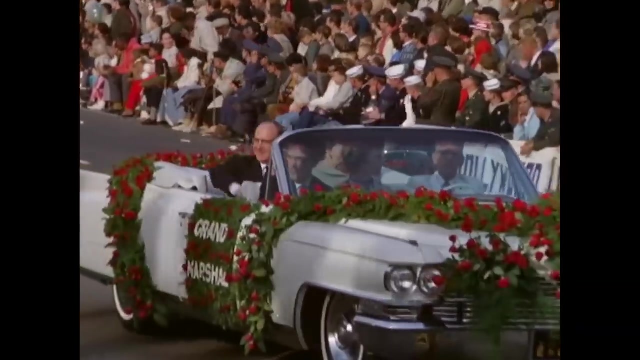 across the planet, approaching 500 degrees Kelvin. Clearly, landing on the surface would present problems, But America wanted to focus on their first real success in space, finally doing something that the Soviets had not. Mariner 2 was the first successful interplanetary probe. 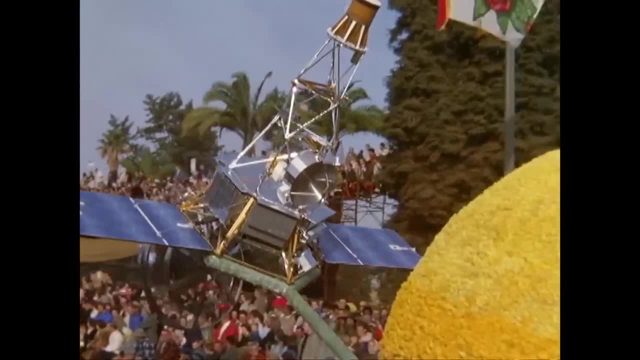 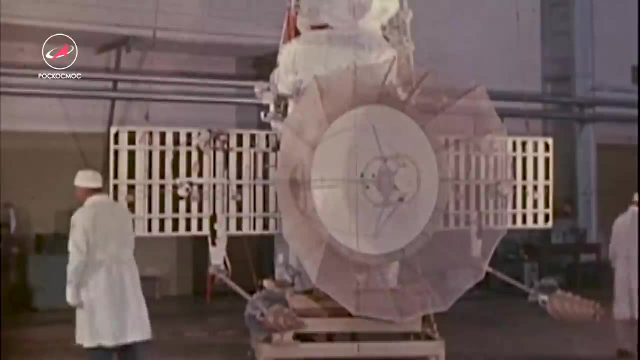 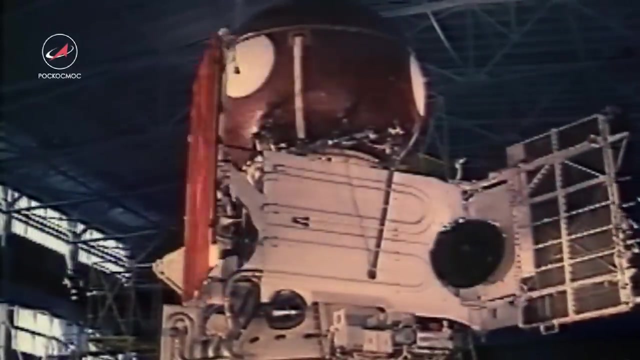 and in California, the home of JPL, they celebrated. The next major advances in the exploration of Venus were made by the Soviet Union. The objective of the Venera series was to land on the surface of Venus. Designers understood that not only were the surface temperatures, 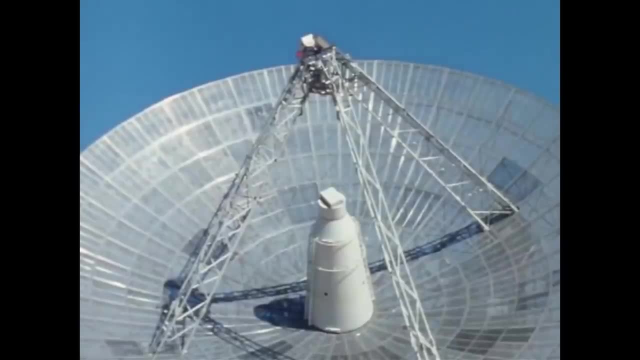 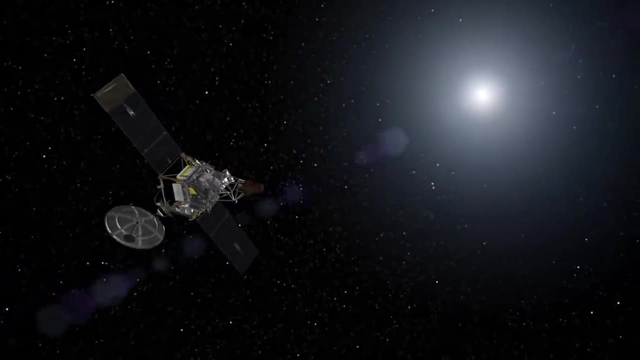 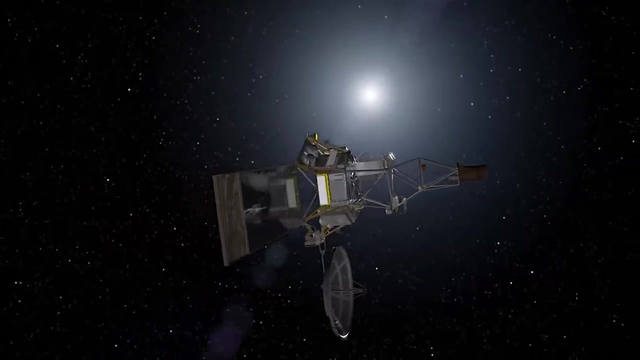 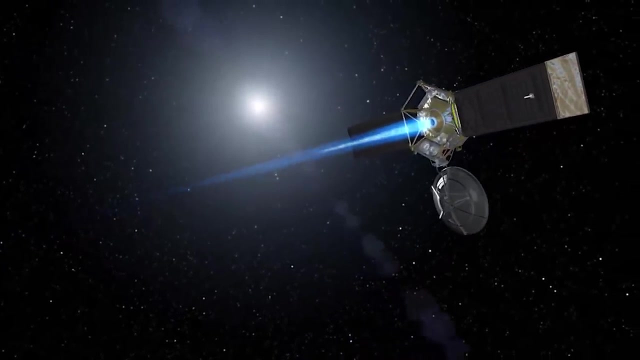 were transmitted to the spacecraft. about an hour later, Mariner executed the manoeuvre, which involved a roll turn, followed by a pitch turn and finally a main engine burn. it worked well, but several days later the craft lost lock on the Sun and the Earth. its two attitude reference points. 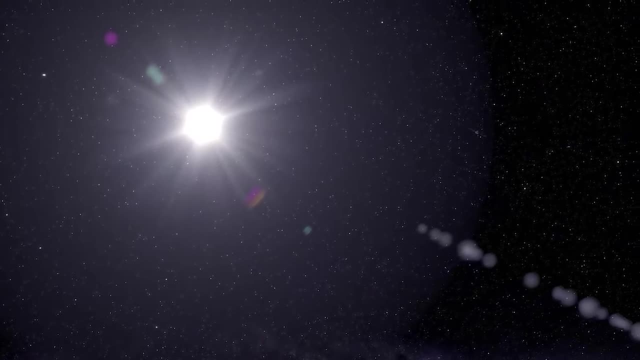 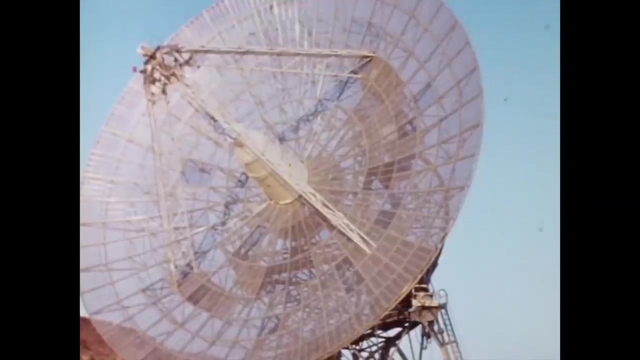 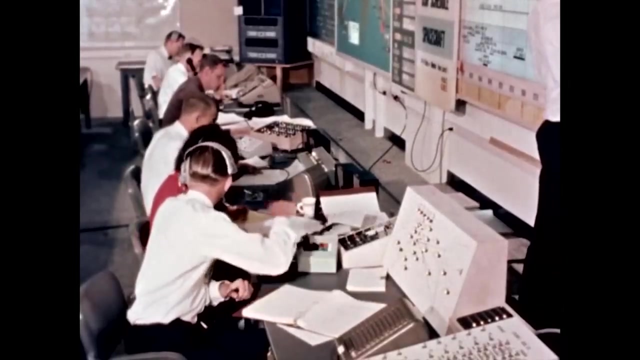 it corrected itself before ground control could diagnose the problem. next, the signal strength increased to its normal level, but a short in a solar panel left it low on power. at this time, although both America and the Soviet Union had been sending probes toward the planets, nothing had succeeded. 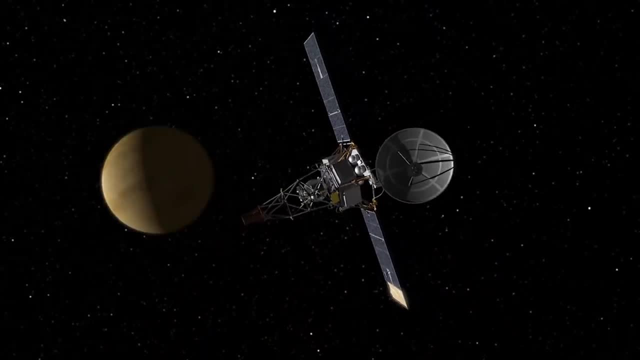 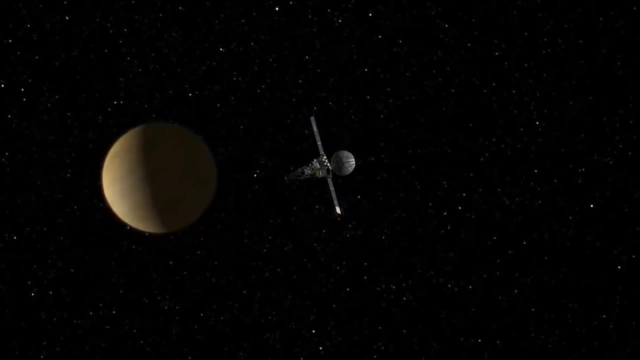 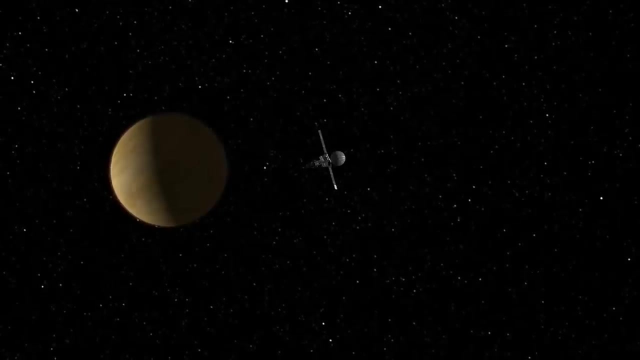 Mariner 2 lost several telemetry sensors and it began to overheat. the first time the probe was sent to the Earth it continued limping toward Venus, but some of the spacecraft's problems were solving themselves. Mariner 2 was now close enough to the Sun that it could function effectively on just one solar panel. 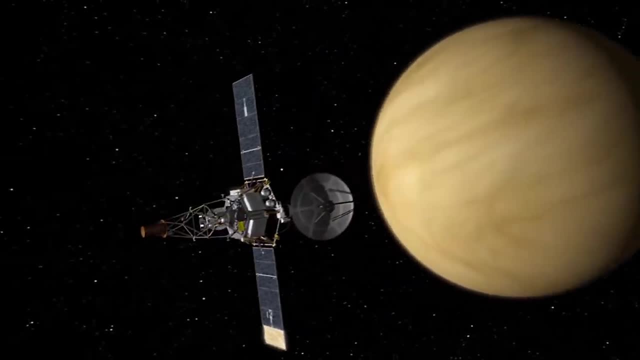 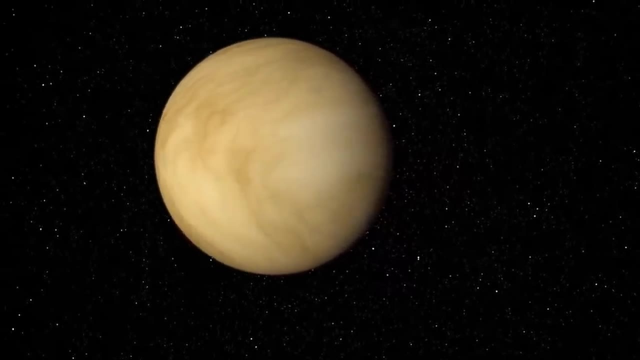 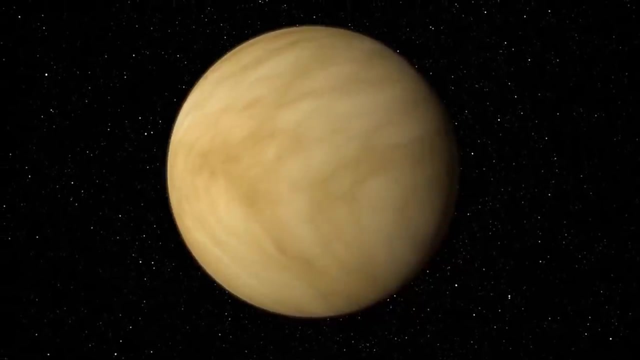 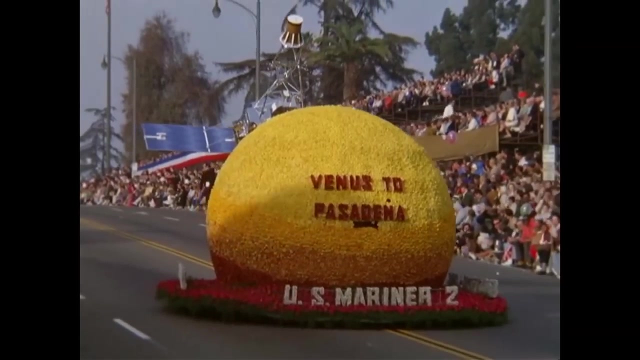 it passed slightly less than 35,000 kilometres above Venus' cloud tops. it could detect no planetary magnetic field and it recorded temperatures across the planet approaching 500 degrees Kelvin. clearly, landing on the surface would present problems, but America wanted to focus on their first real success in space. 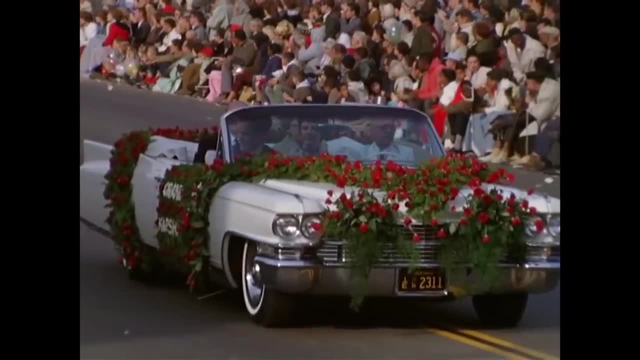 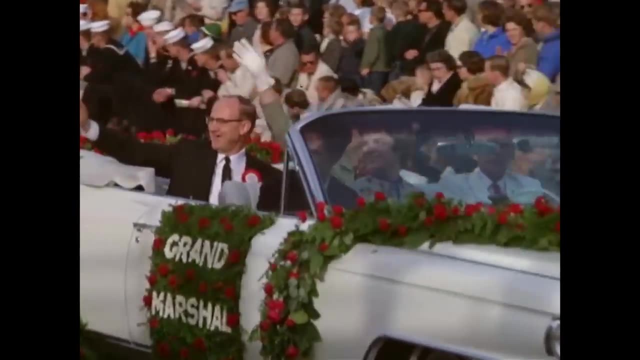 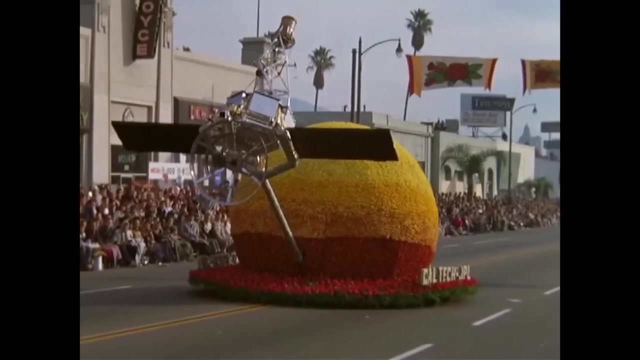 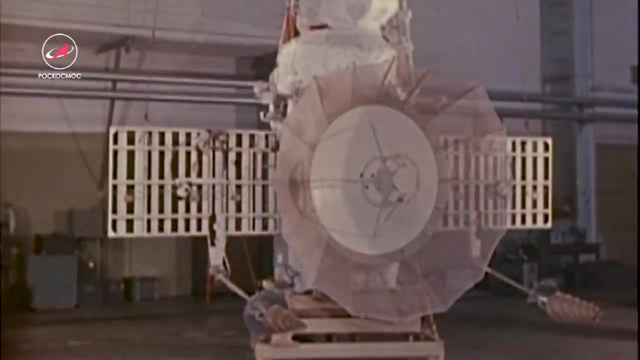 finally doing something that the Soviets had not. Mariner 2 was the first successful interplanetary probe and in California, the home of JPL, they celebrated. the next major advances in the exploration of Venus were made by the Soviet Union. the objective of the Venera series was to land on the surface of Venus. 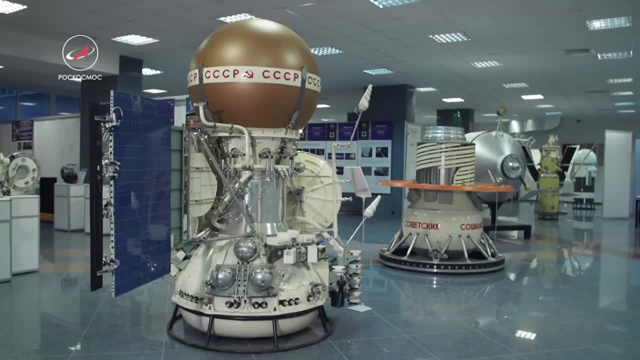 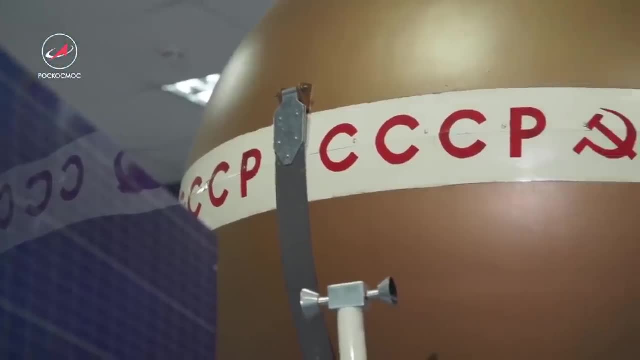 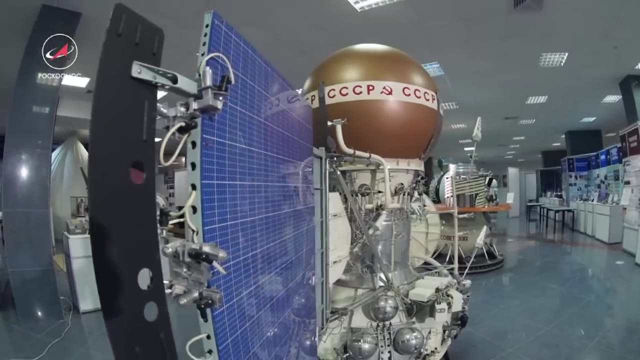 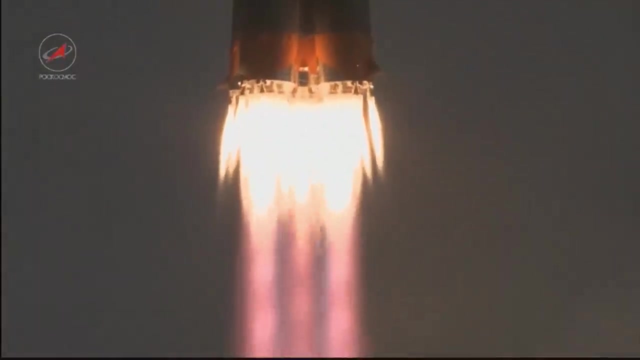 designers understood that not only were the surface temperatures hot enough to melt lead, but that the atmospheric pressure was many times that of Earth. the landers they built looked more like diving bells than spacecraft. in June 1967, Venera 4 was launched. the vehicle consisted of a carrier craft. 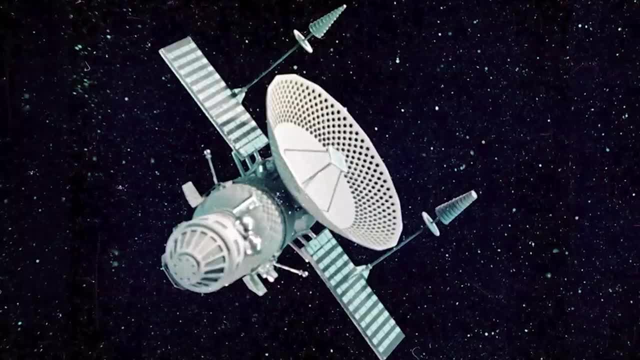 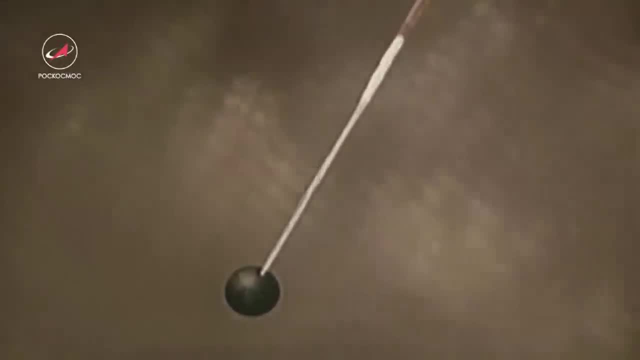 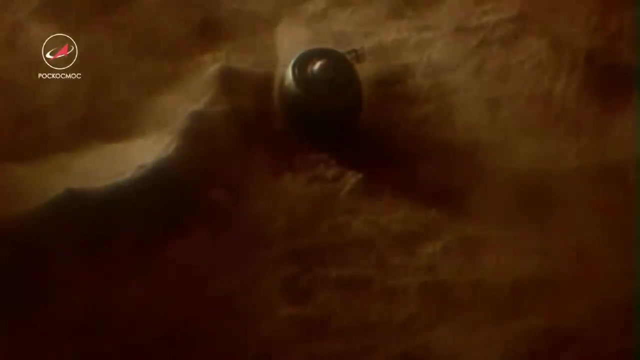 with instruments used during the cruise phase to Venus and a spherical landing module that could communicate independently. after entry into the atmosphere, Venera 4's parachute opened. it sent back data for 93 minutes, but stopped 28 kilometers above the surface yet its electronics hadn't been overwhelmed by the heat. 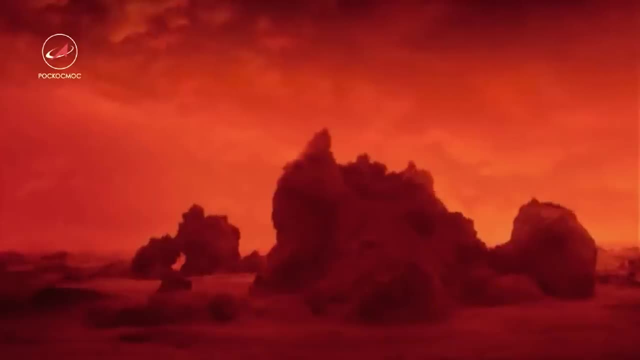 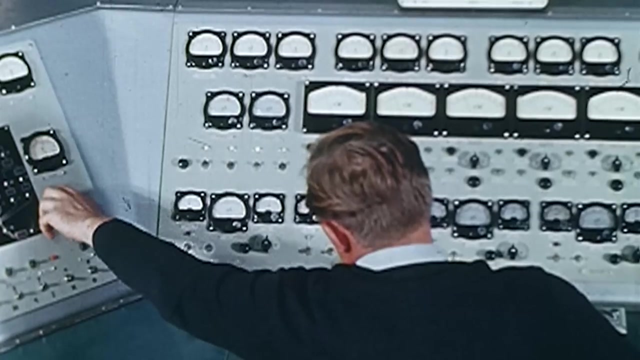 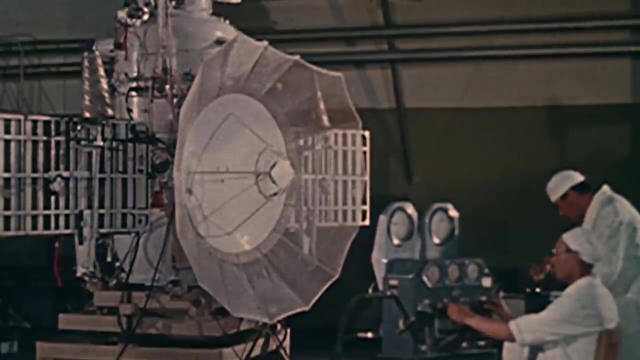 it had simply run out of power. extrapolations from its final measurements showed a surface temperature of 500 degrees Celsius and a pressure of 75 atmospheres, far higher than anyone expected. the Venera program strengthened its landers and fitted smaller parachutes to reduce descent time. 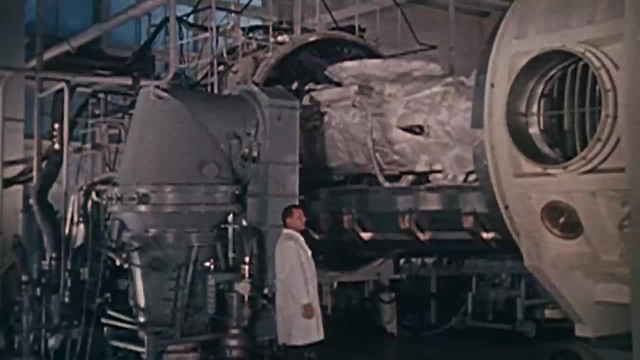 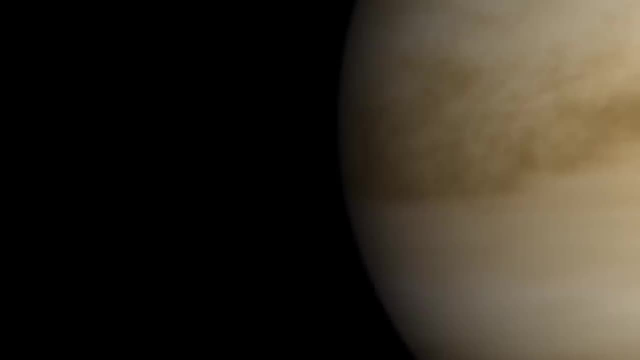 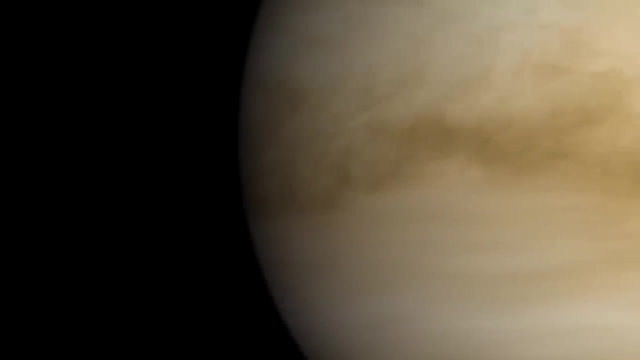 launched in January 1969, Venera 5 and 6 learned more about the chemical makeup of the atmosphere, but neither remained functioning at the surface. the Venera series continued refining the technology and making incremental improvements to mission duration, adding to the knowledge about Venus. 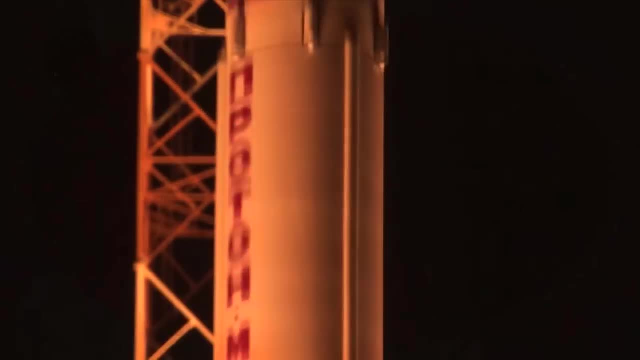 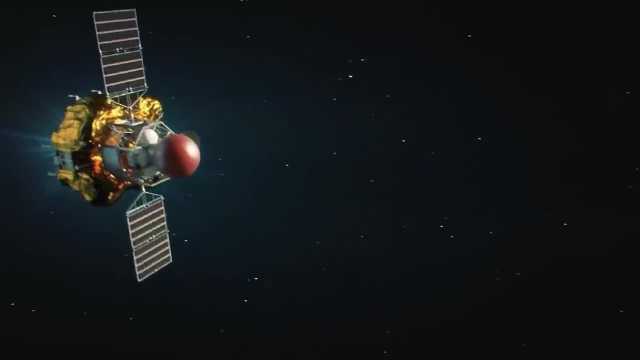 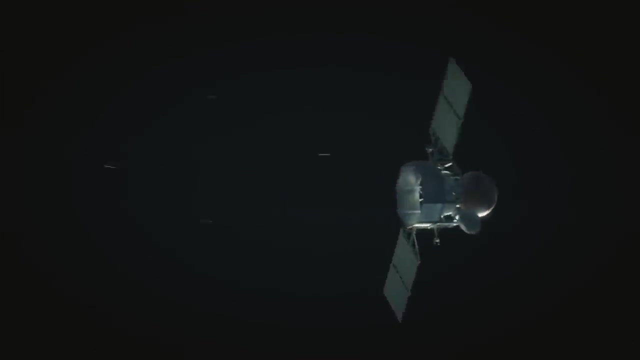 Venera 5 was launched in 1975. in 1975, Venera 9 was launched. it was a new design consisting of an orbiter-lander combination, with the orbiter able to act as a relay station for signals transmitted from the surface. 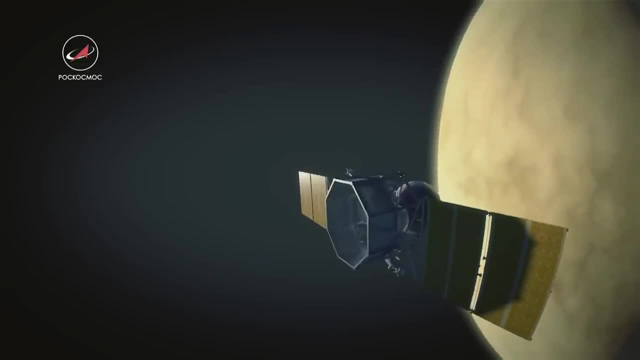 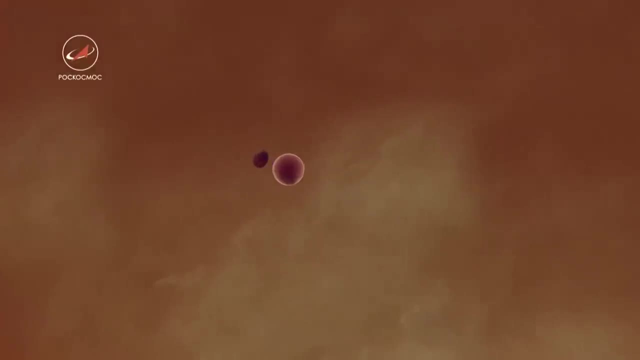 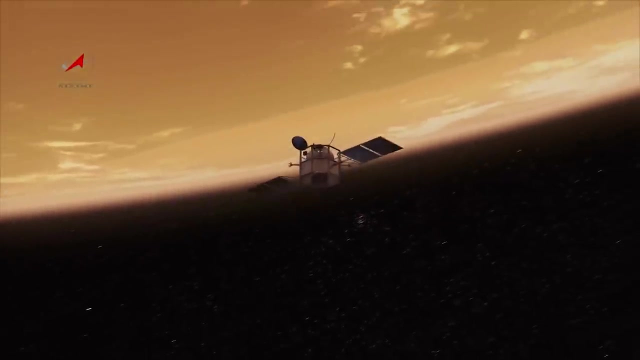 four months after launch, the orbiter and the lander, encased in a spherical shell, separated. it entered the atmosphere two days later, while the mother craft became the first probe to go into orbit around Venus, photographing parts of the surface in ultraviolet. the new lander had a ring shield. 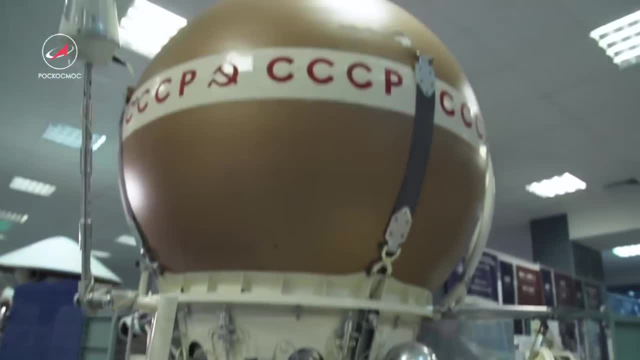 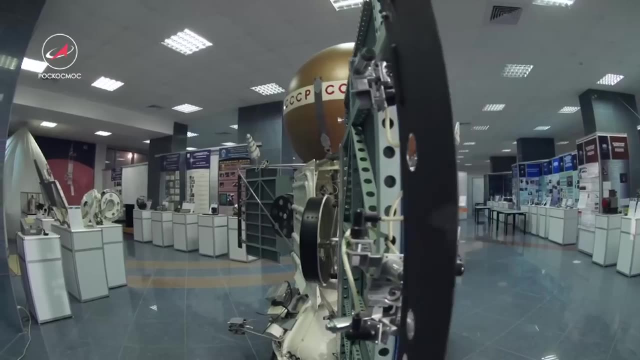 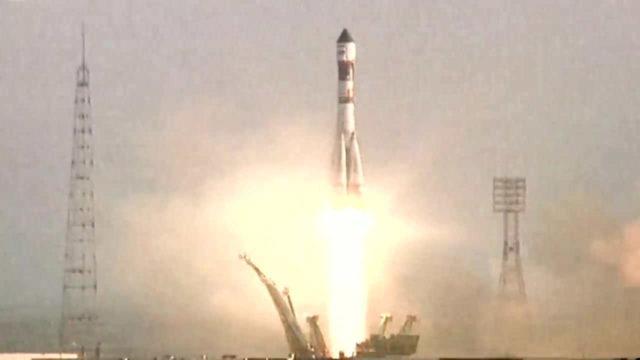 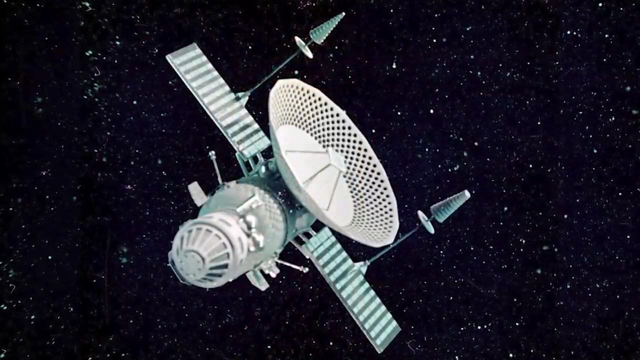 hot enough to melt lead, but that the atmospheric pressure was many times that of Earth. The landers they built looked more like diving bells than spacecraft. In June 1967, Venera 4 was launched. The vehicle consisted of a carrier craft. 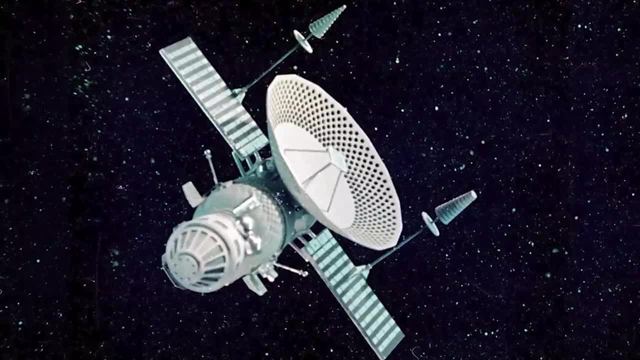 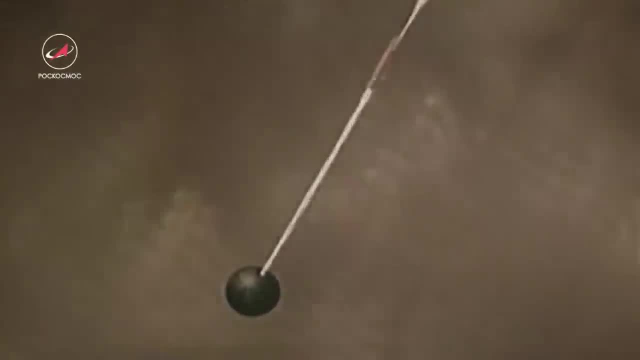 with instruments used during the cruise phase to Venus and a spherical landing module that could communicate independently After entering into the atmosphere. Venera 4's parachute opened. It sent back data for 93 minutes, but stopped 28 kilometers above the surface. 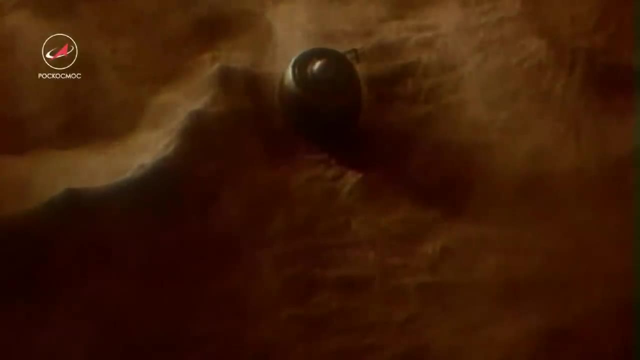 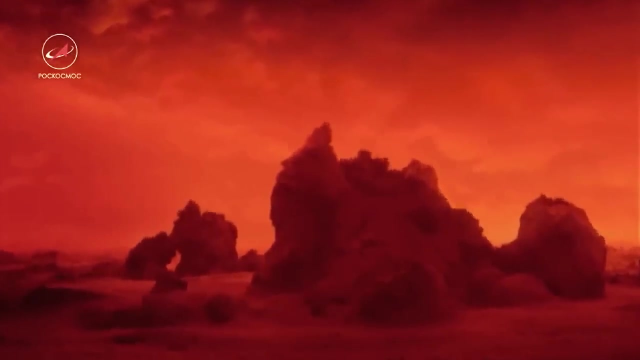 Yet its electronics hadn't been overwhelmed by the heat, it had simply run out of power. Extrapolations from its final measurements showed a surface temperature of 500 degrees Celsius and a pressure of 17 degrees Fahrenheit. A pressure of 75 atmospheres. 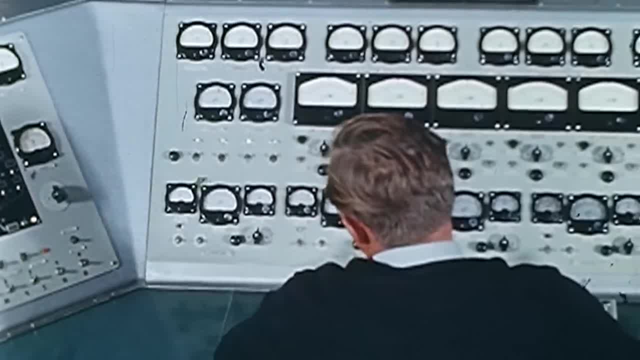 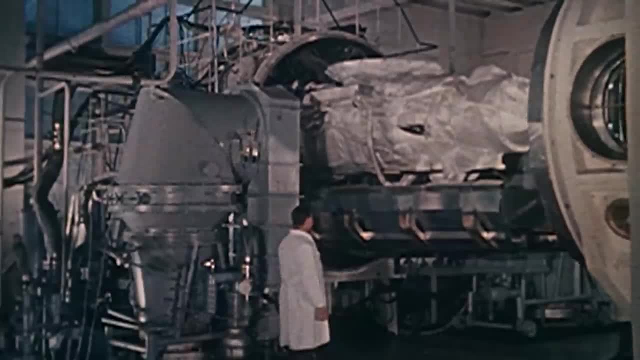 far higher than anyone expected. The Venera program strengthened its landers and fitted smaller parachutes to reduce descent time. Launched in January 1969, Venera 5 and 6 learned more about the chemical makeup of the atmosphere. 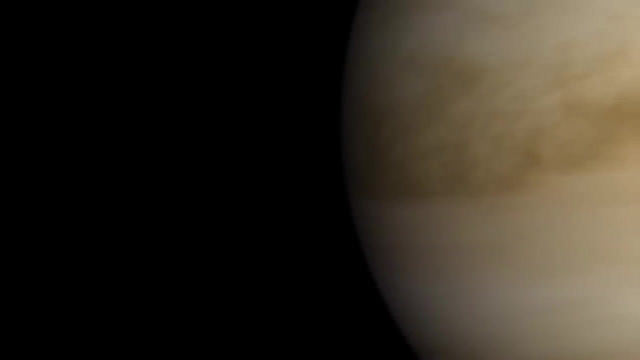 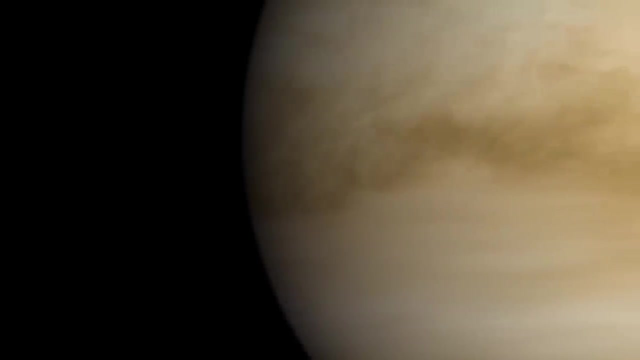 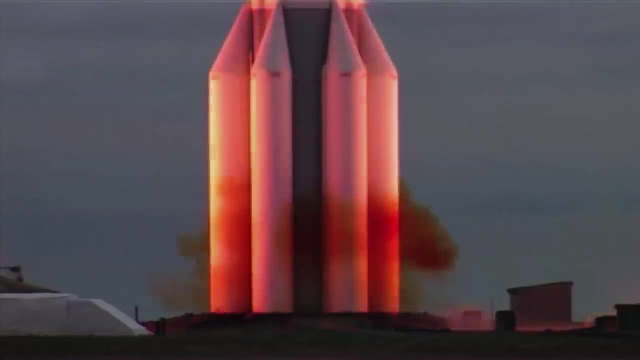 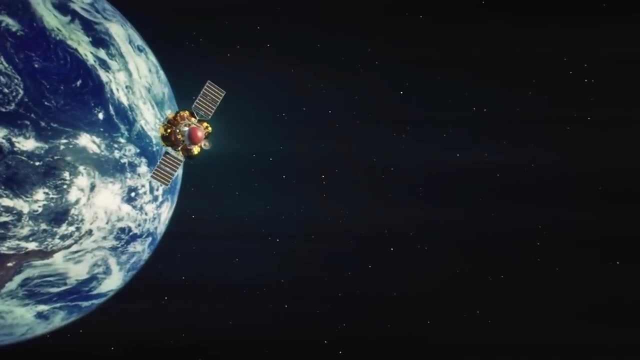 but neither remained functioning at the surface. The Venera series continued refining the technology and making incremental improvements to mission duration, adding to the knowledge about Venus. In 1975, Venera 9 was launched. It was a new design. 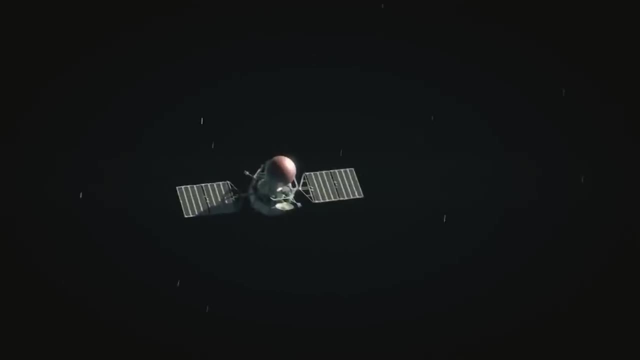 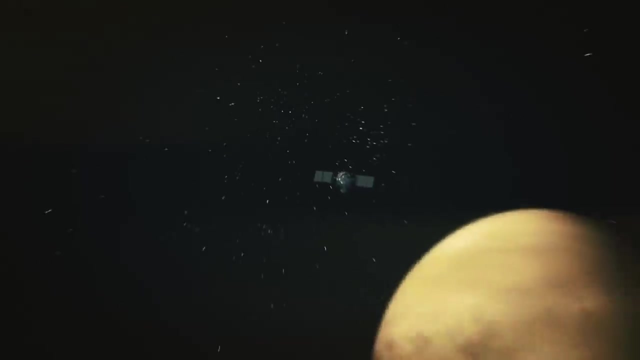 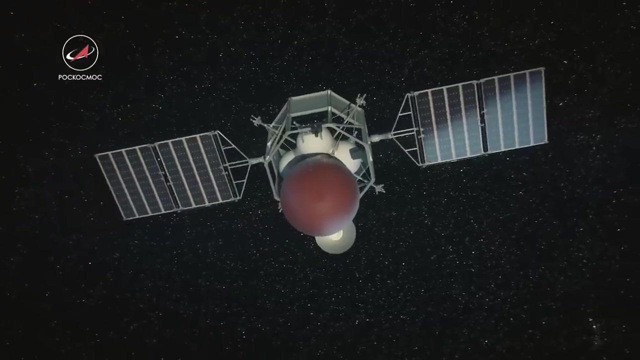 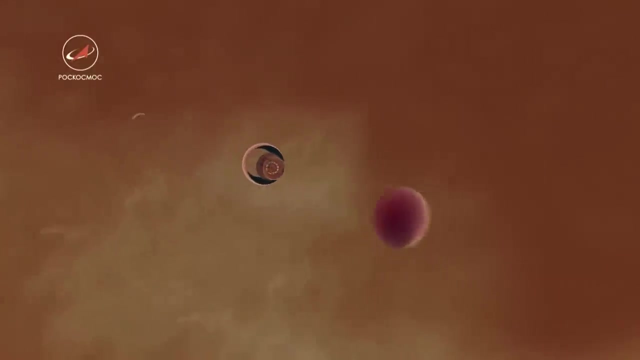 consisting of an orbiter-lander combination, with the orbiter able to act as a relay station for signals transmitted from the surface. Four months after launch, the orbiter and the lander, encased in a spherical shell, separated. It entered the atmosphere two days later. 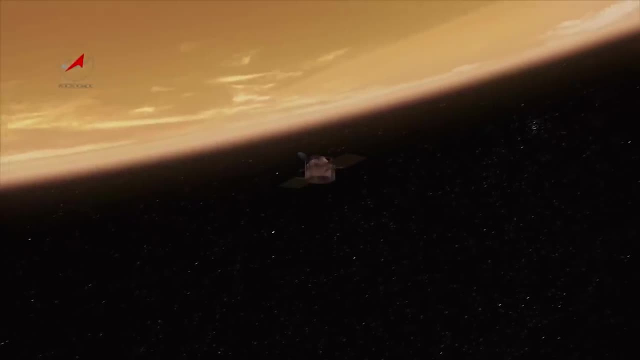 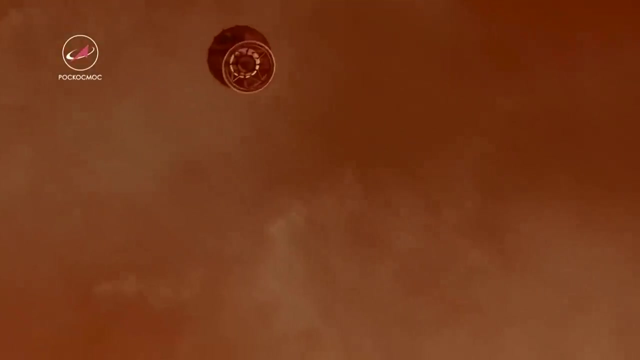 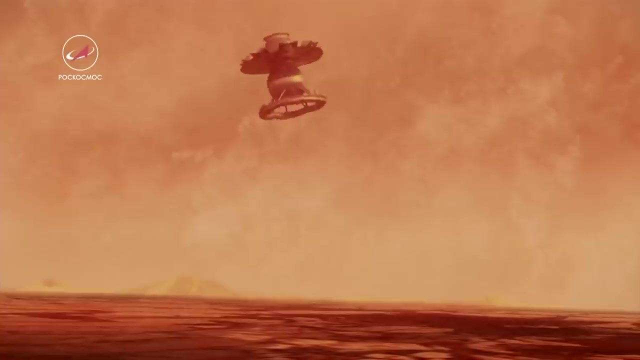 while the mother craft became the first probe to go into orbit around Venus, photographing parts of the surface in ultraviolet. The new lander had a ring shield that could replace a parachute during the latter stages of the descent through the dense atmosphere. Venera 9 transmitted the first black and white pictures. 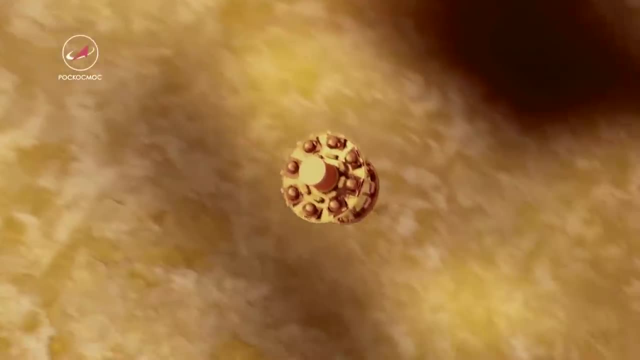 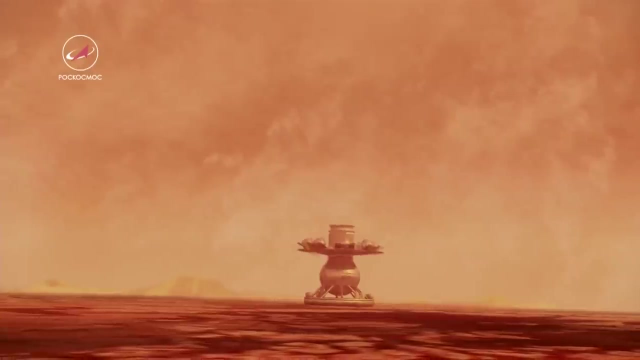 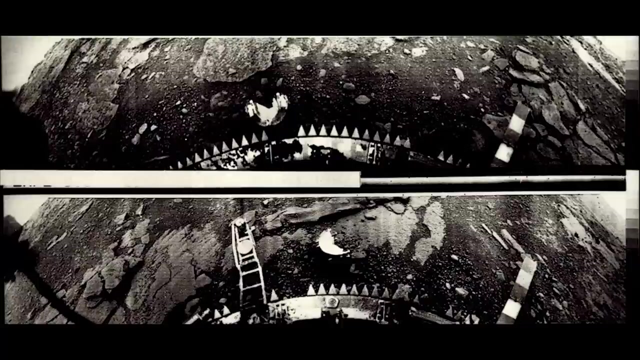 that could replace a parachute during the latter stages of the descent through the dense atmosphere. Venera 9 transmitted the first black and white pictures from the surface, though a design fault meant a second camera could not eject its lens cap. three days later, and two thousand kilometers away, 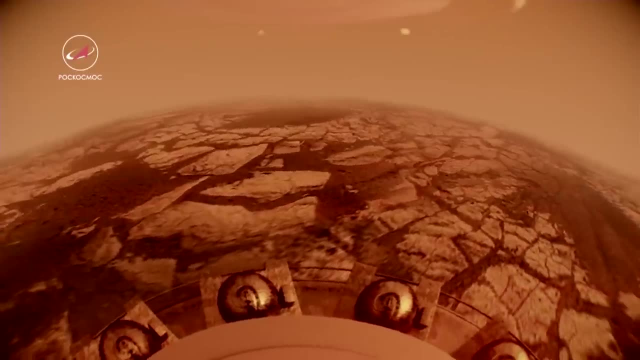 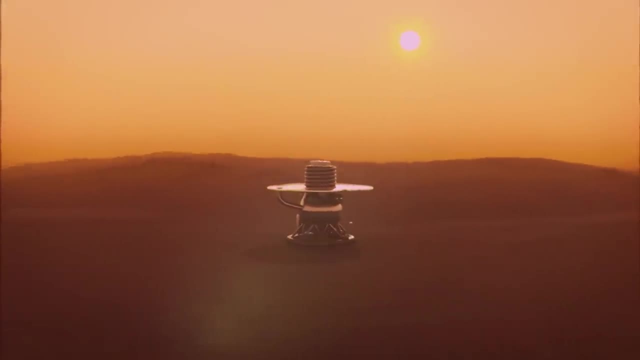 a twin craft, Venera 10, landed. it took pictures too, but the same design fault left a lens cap stuck in place. both landers had been pre-cooled while still in space and circulating cooling fluid kept the craft operating on the blistering surface. 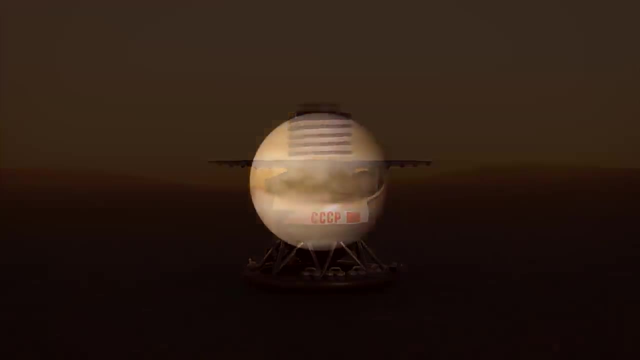 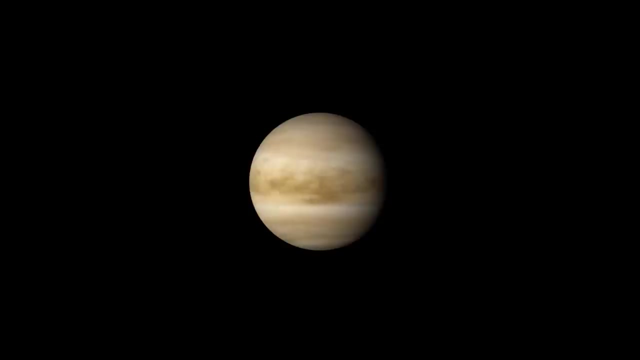 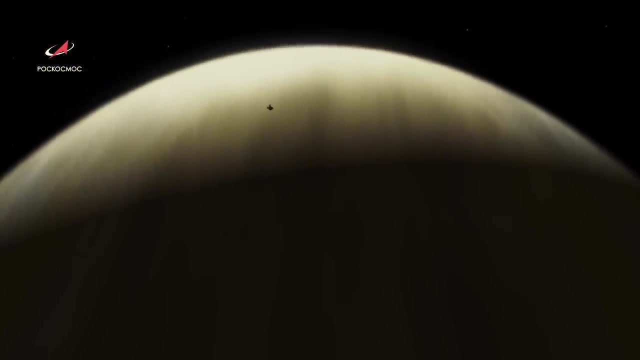 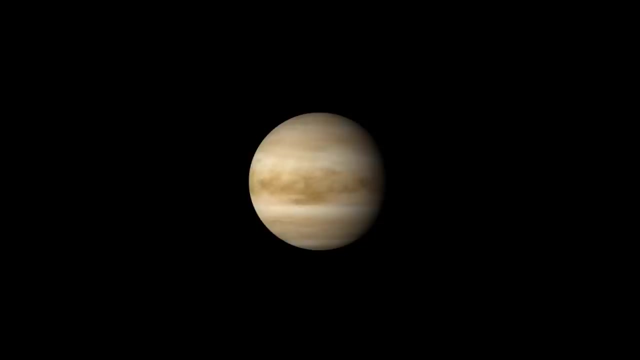 for more than an hour. in 1983, two more Venera craft arrived at Venus equipped with synthetic aperture radar. they made the first serious attempt to map the surface beneath the cloud layer. over eight months they mapped from the north pole down to 30 degrees north. 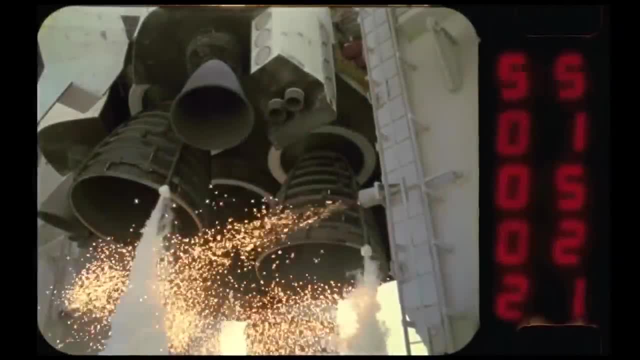 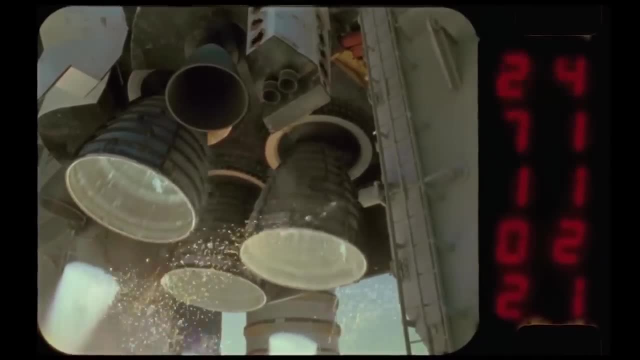 to 10 degrees south and from the south pole to the south pole, to the south pole and from the south pole they could see the entire sky and the entire sky. Nasa had taken a minor role in the early exploration of Venus, but in 1989. 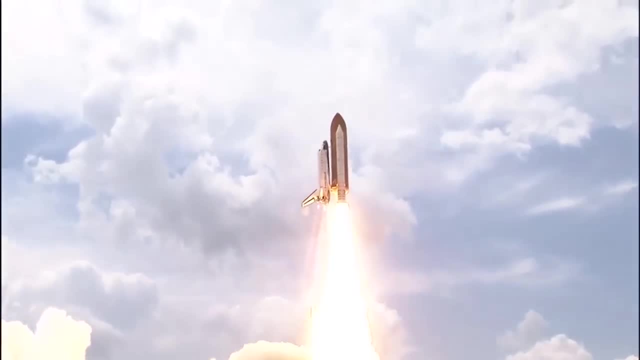 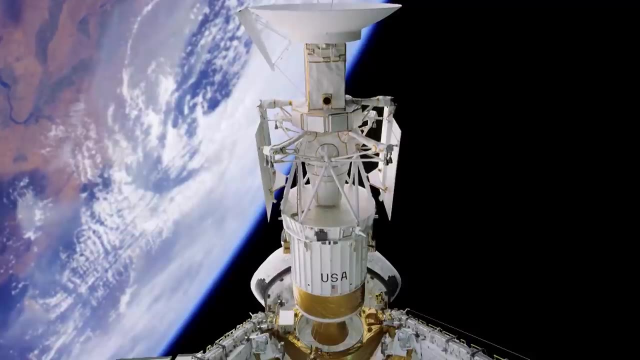 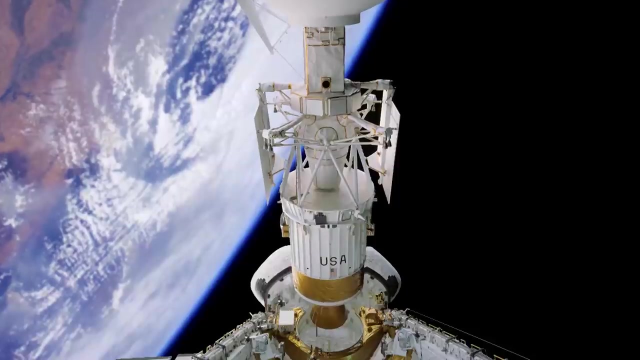 the space shuttle Atlantis lifted off, carrying the Magellan probe. Magellan was bound for Venus, like the Venera craft before it craft before it, Magellan would use radar to map the surface of the planet. it was the first interplanetary spacecraft launched from the Space Shuttle. 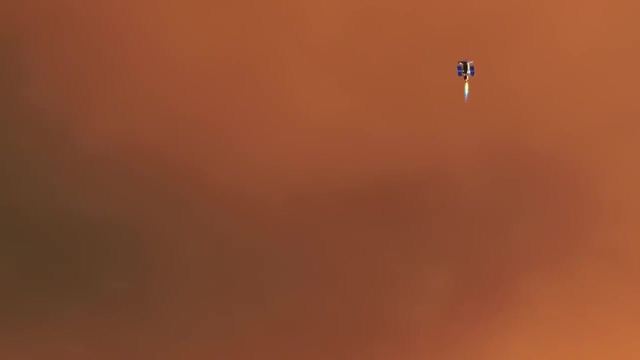 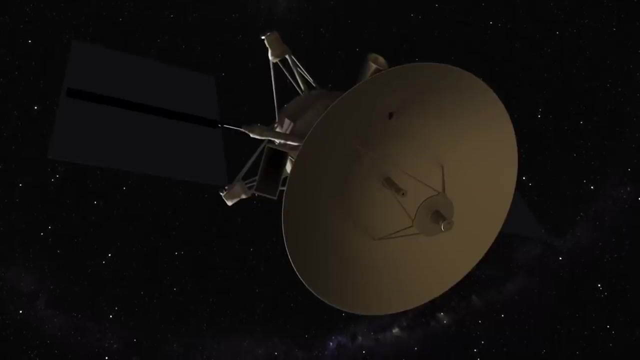 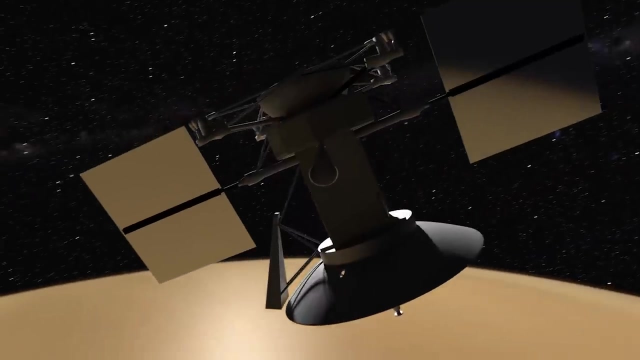 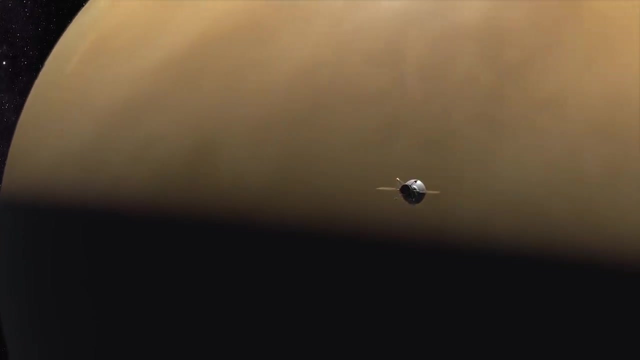 following the cruise of 15 months, Magellan arrived at Venus and entered an elliptical orbit. to keep costs down, the probe had been built from an agglomeration of spare parts left over from previous NASA missions. after some software problems, it began mapping. the images it relayed remained the highest. 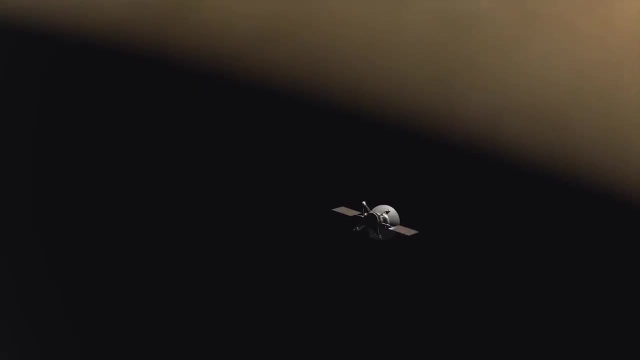 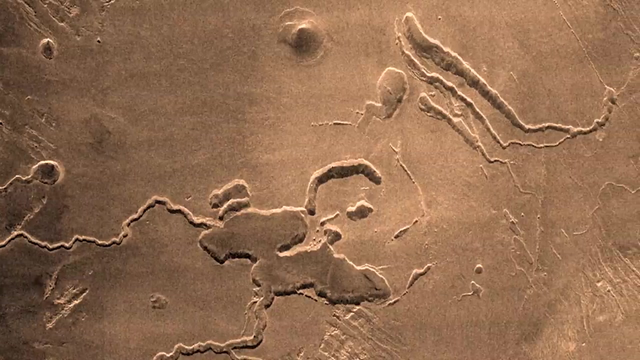 resolution pictures we have of the surface of Venus. pictures of low volcanic blisters emerged and lava channels were evidence of an extremely active surface. the thick atmosphere has prevented all but the largest meteors reached the surface of the planet and the surface of the planet has been. 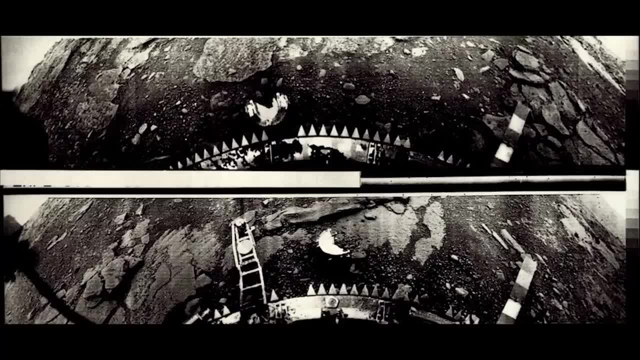 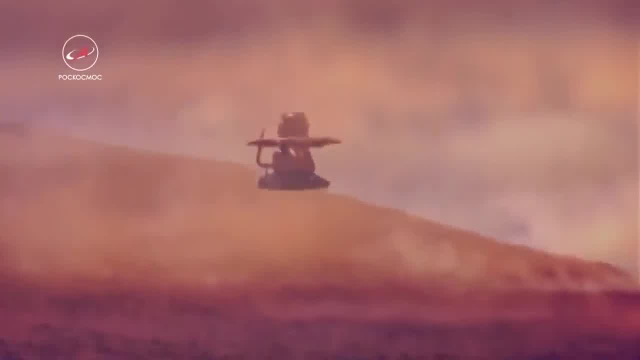 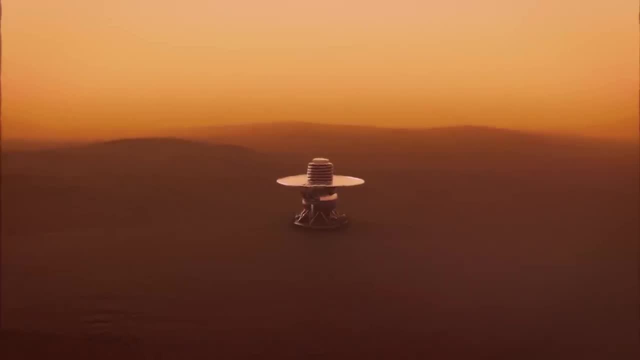 from the surface, though a design fault meant a second camera could not eject its lens cap. Three days later, and 2,000 kilometers away, a twin craft- Venera 10,- landed. It took pictures too, but the same design fault left a lens cap stuck in place. 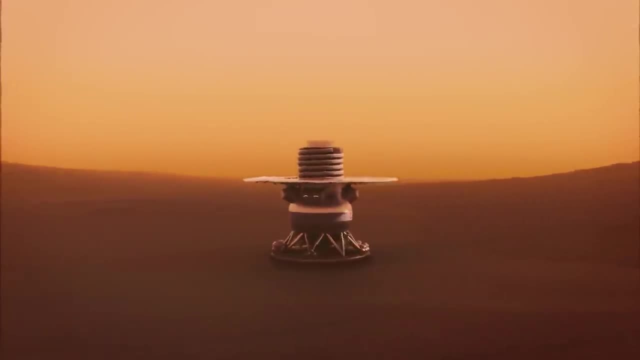 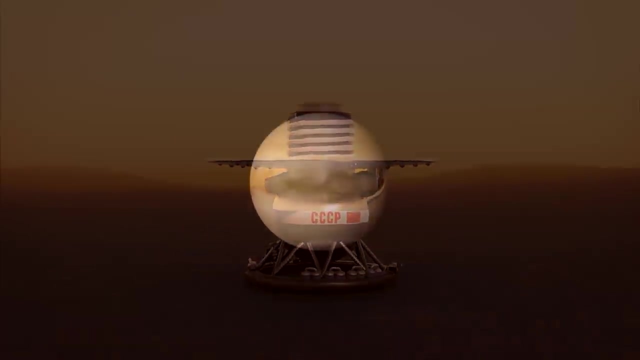 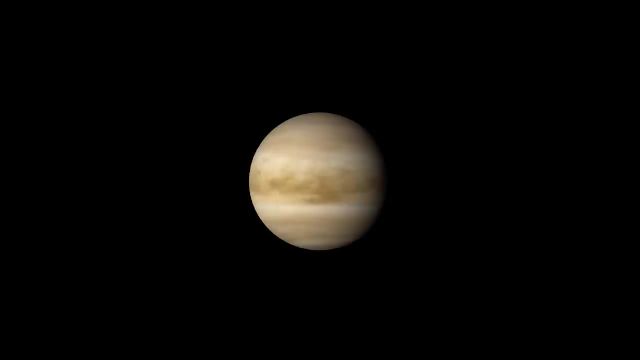 Both landers had been pre-cooled while still in space, and circulating cooling fluid kept the craft operating on the blistering surface for more than an hour. In 1983, two more Venera craft arrived at Venus Equipped with synthetic aperture radar. 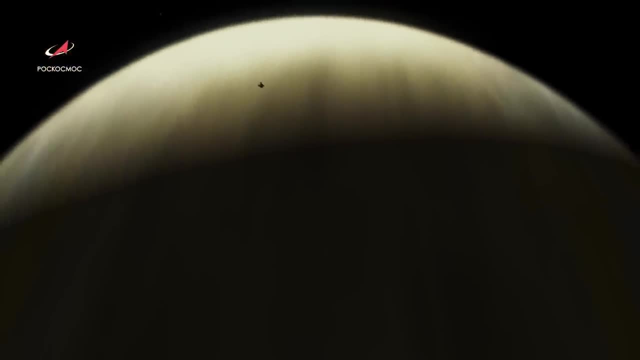 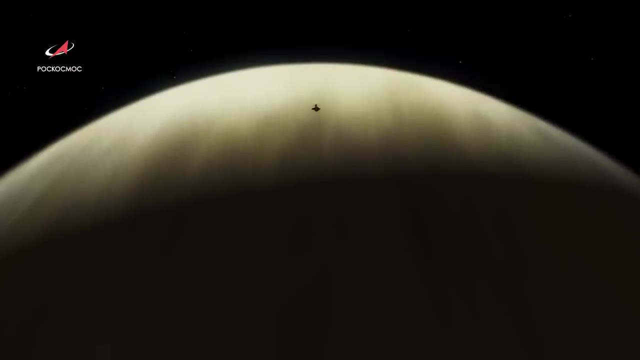 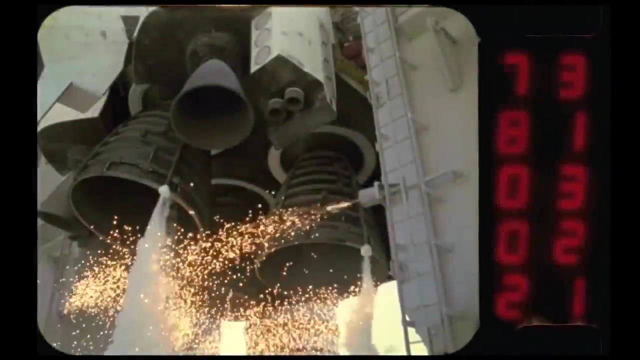 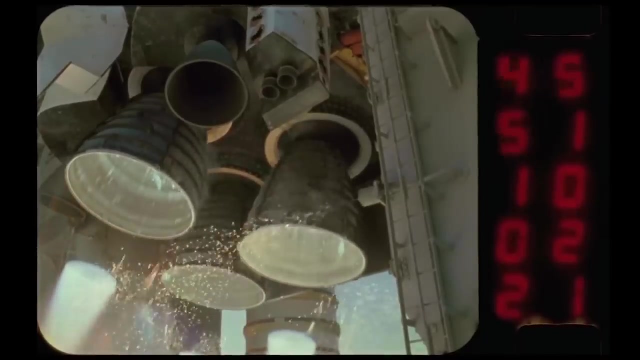 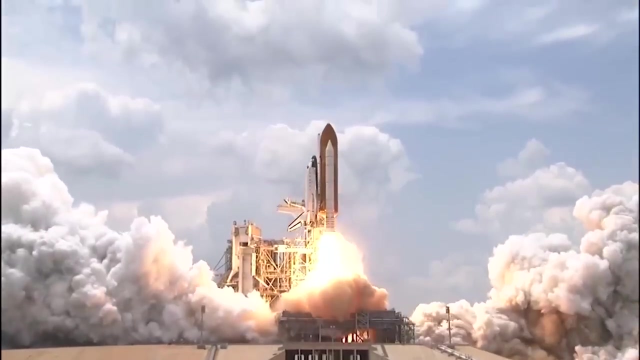 they made the first serious attempt to map the surface beneath the cloud layer. Over eight months they mapped from the North Pole down to 30 degrees north. NASA had taken a minor role in the early exploration of Venus, But in 1989,. 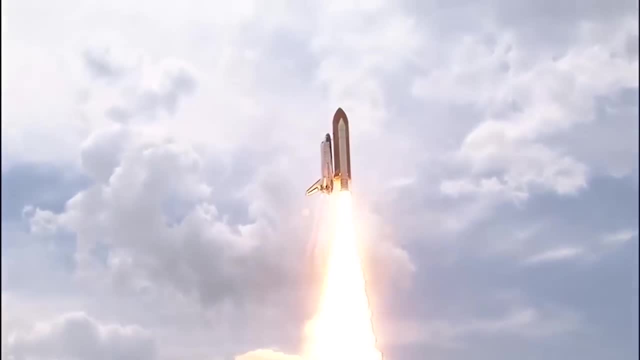 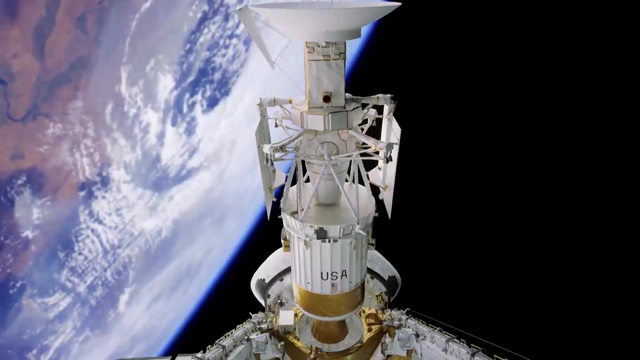 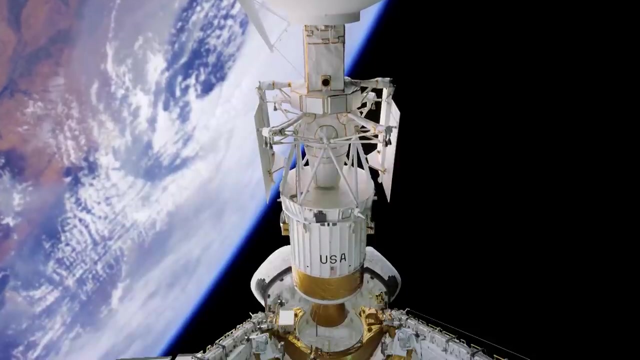 the space shuttle Atlantis lifted off, carrying the Magellan probe. Magellan was bound for Venus. Like the Venera craft before it, Magellan would use radar to map the surface of the planet. It was the first interplanetary spacecraft launched from the space shuttle. 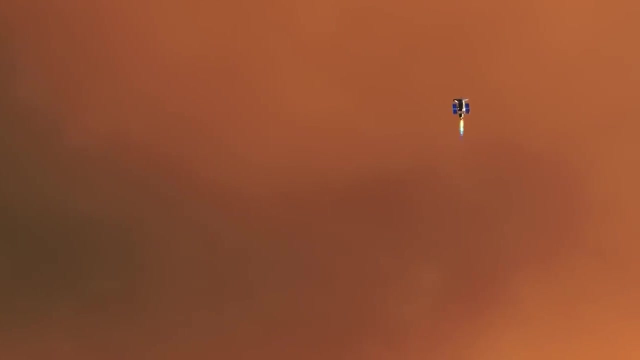 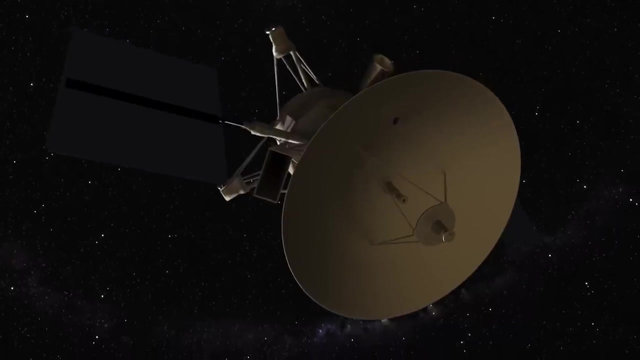 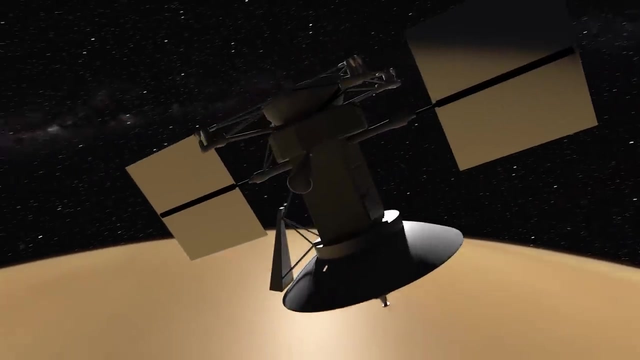 Following a cruise of 15 months, Magellan arrived at Venus and entered an elliptical orbit. To keep costs down, the probe had been built from an agglomeration of spare parts left over from previous NASA missions. After some software problems. 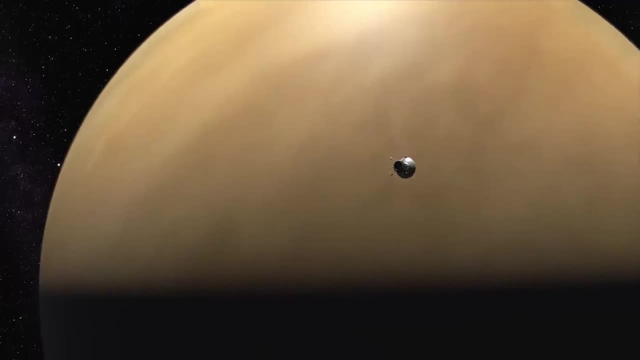 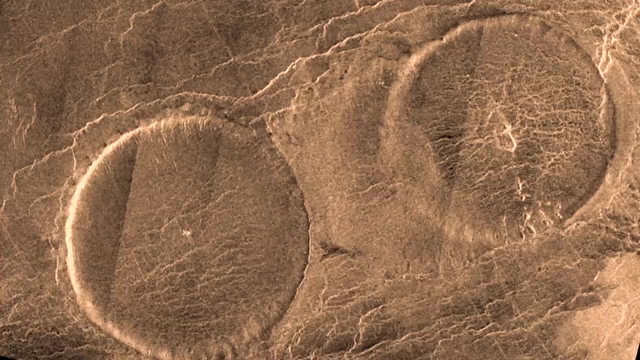 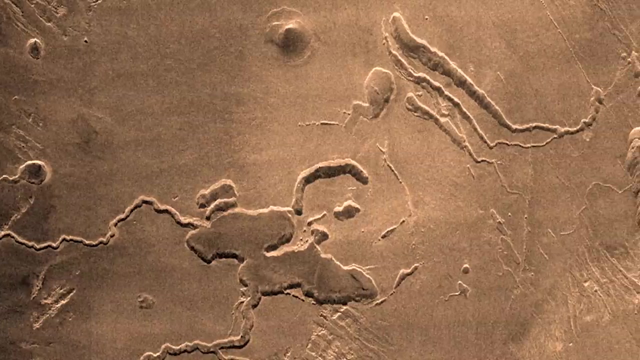 it began mapping. The images it relayed remained the highest resolution pictures we have of the surface of Venus, Pictures of low volcanic blisters emerged and lava channels were evidence of an extremely active surface. The thick atmosphere has prevented all but the largest meteors. 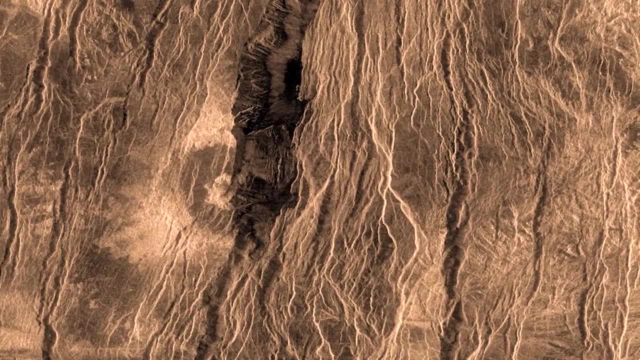 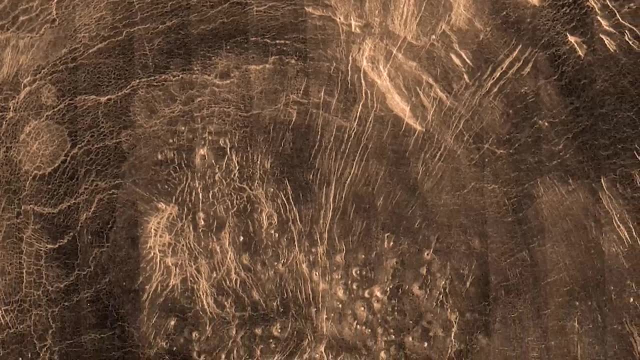 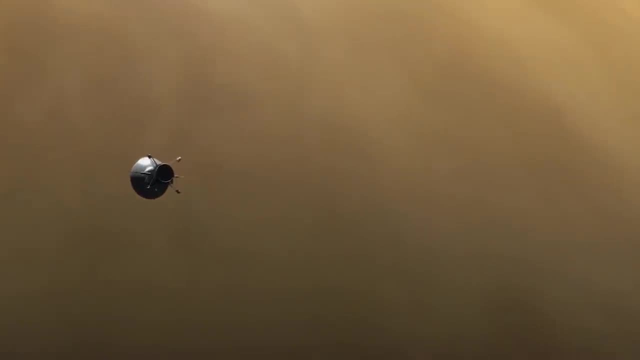 reaching Venusian ground and few impact craters were visible, Yet evidence of plate tectonics that sculpts the Earth's surface was not obvious. After mapping Venus, Magellan changed its orbit and plotted the planet's gravitational anomalies On Venus. 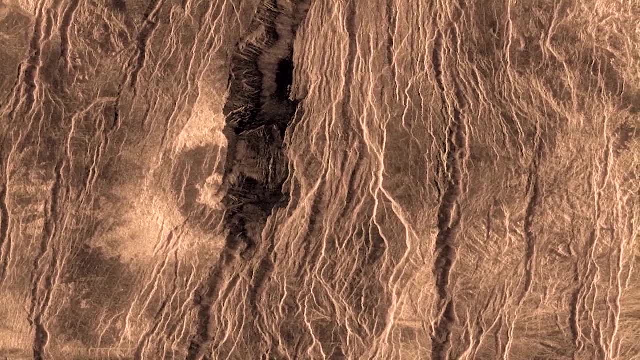 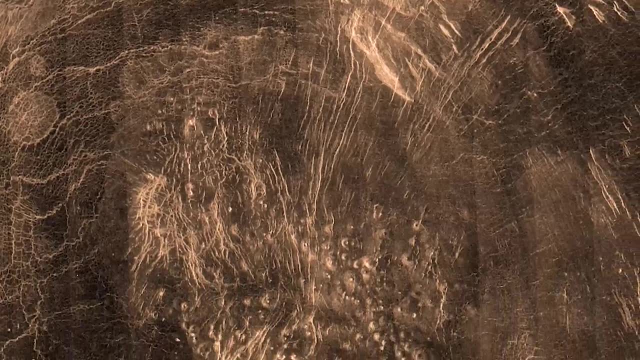 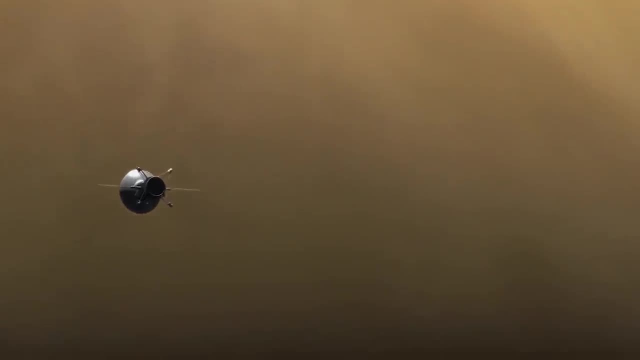 reaching Venusian ground and few impact craters were visible. yet evidence of plate tectonics that sculpts the Earth's surface was not obvious. after mapping Venus, Magellan changed its orbit and plotted the planet's gravitational anomalies on Venus localized changes in gravity. 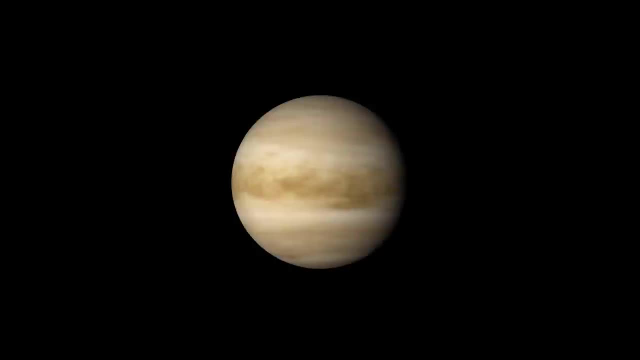 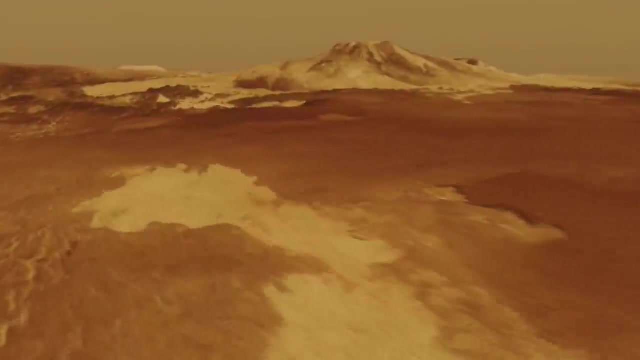 correspond to surface features on Earth. this is not the case. a A new naked picture of Venus emerged. The surface appears to have been completely remade around half a billion years ago. Yet while volcanoes and lava channels are common features on Venus, Magellan could not find evidence. 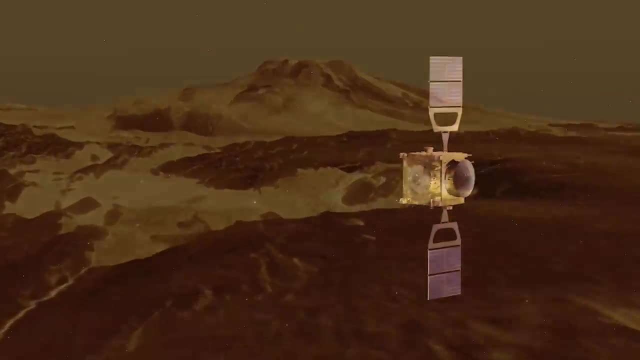 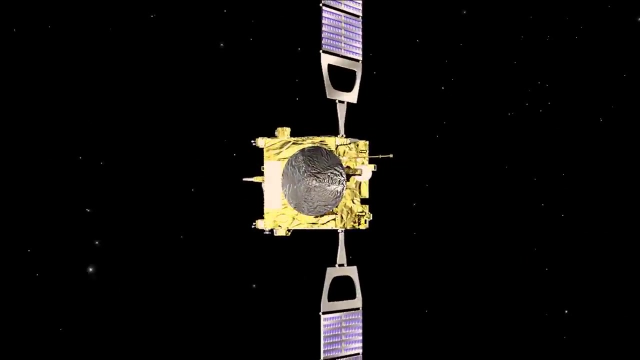 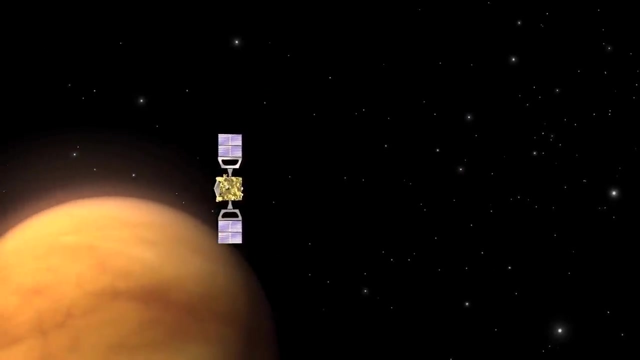 that volcanic activity still happens on the planet. In 2006,, the European Space Agency's Venus Express went into orbit around Venus. Its focus was the long-term analysis of the planet's atmosphere. During its eight-year mission, it registered a sharp rise. 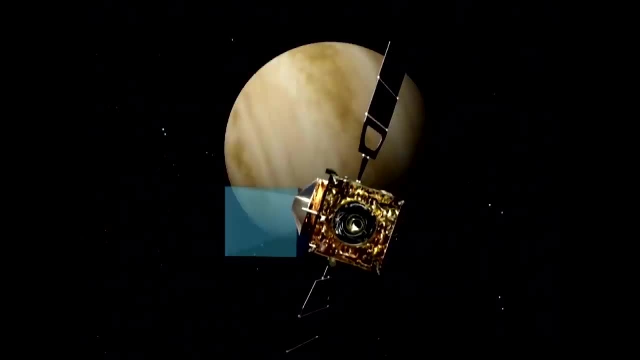 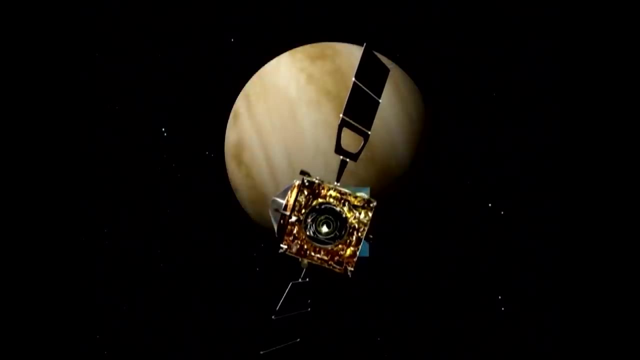 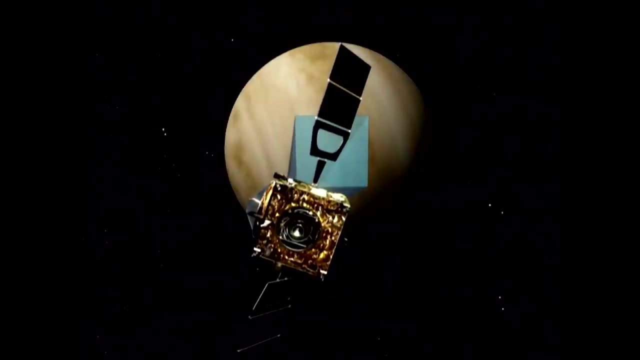 in the atmosphere's sulfur dioxide. This could be due to changes in wind patterns, but it could also be a sign of volcanic activity. Researchers also saw increases in infrared radiation coming from three different volcanic locations. More circumstantial evidence of current volcanic activity. 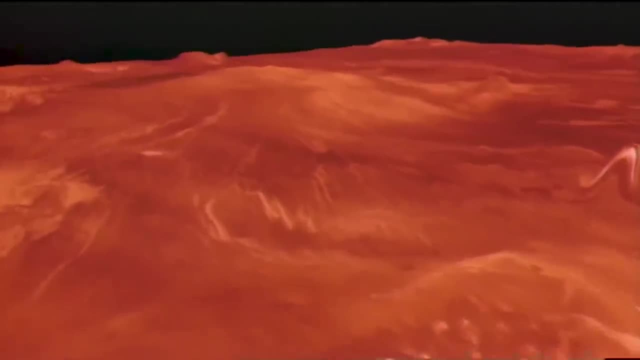 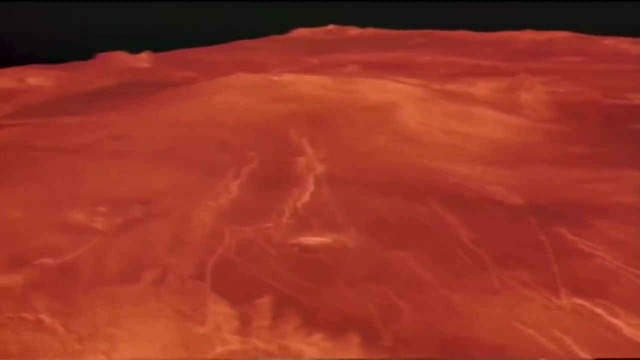 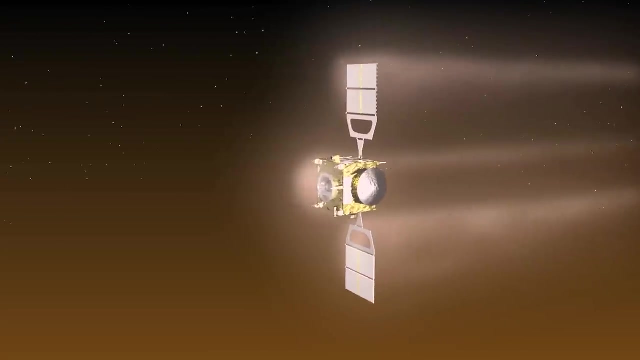 Finally, the infrared team saw short-term temperature changes that fluctuated over just a few days. It appears that volcanoes may still be active on Venus. The mission ended in 2015 with a series of swoops into the upper atmosphere that verified unexpected ripples in the mesosphere. 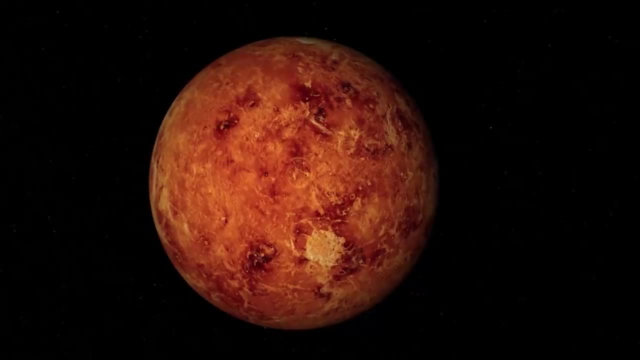 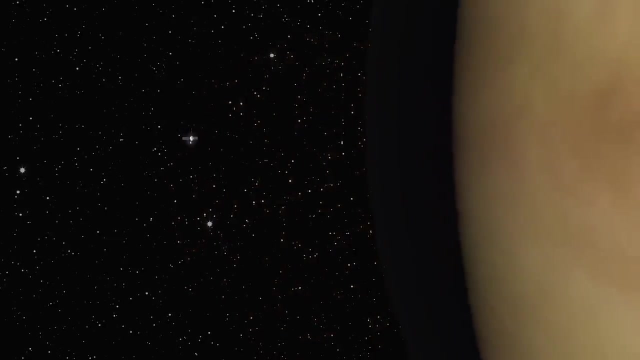 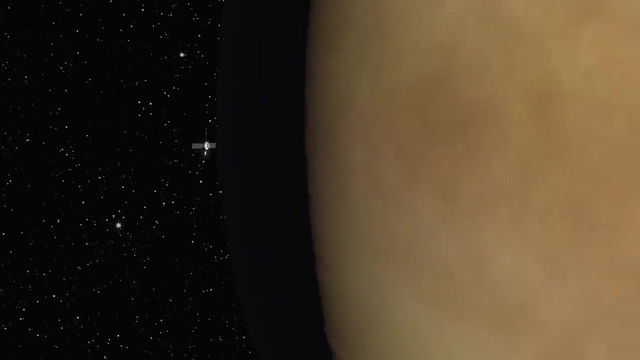 Very little in the way of Venus exploration has happened since Venus Express. Though elaborate plans exist for future missions to Venus, nothing at this stage has been funded. Yet many missions still pass close to Venus to use its gravitation to alter their flight paths. 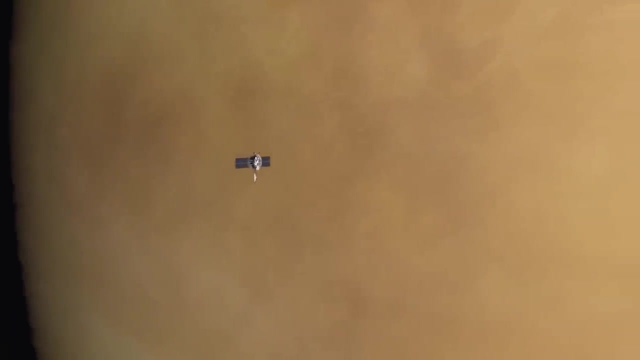 In 1974, Mariner 10 was the first spacecraft ever to use the gravitational slingshot effect on Venus. It was the first spacecraft ever to use the gravitational slingshot effect on Venus, Yet many missions still pass close to Venus. 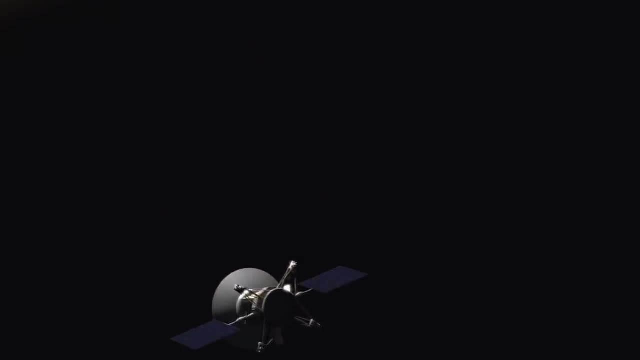 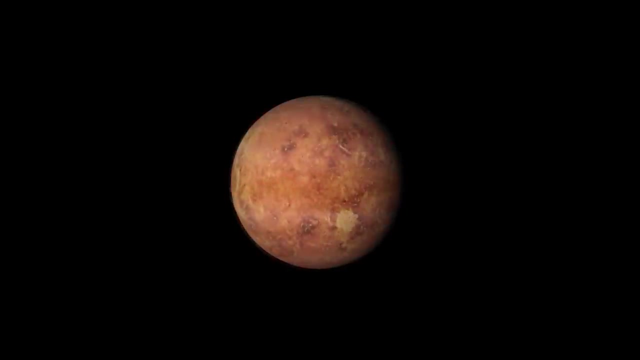 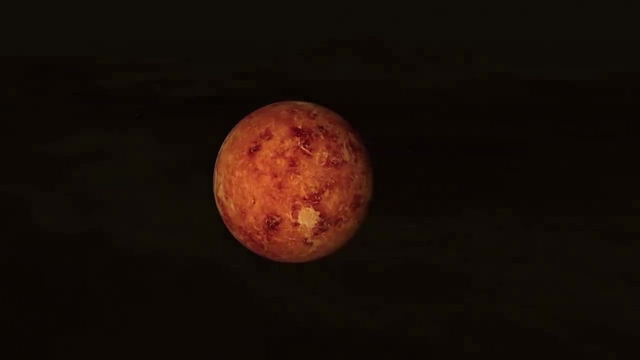 localized changes in gravity correspond to surface features On Earth. this is not the case. A new naked picture of Venus emerged. The surface appears to have been completely remade around half a billion years ago. Yet while volcanoes and lava channels are common features on Venus, 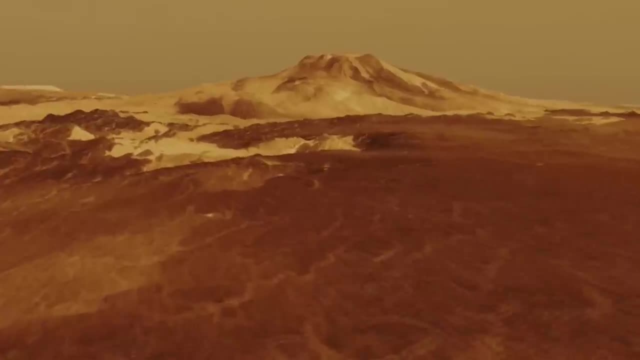 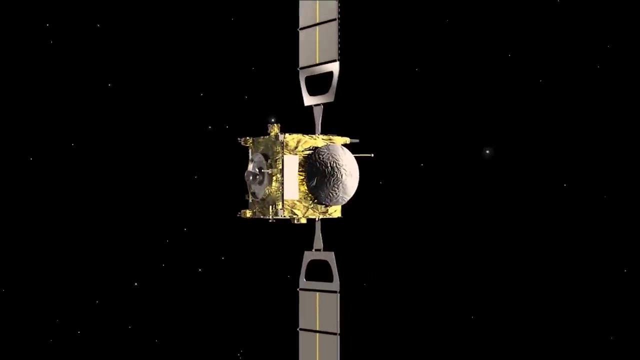 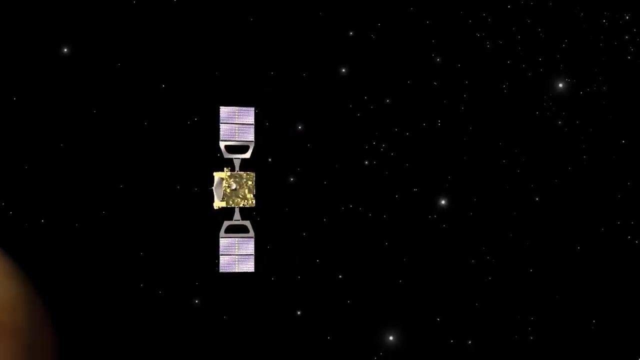 Magellan could not find evidence that volcanic activity still happens on the planet. In 2006,, the European Space Agency's Venus Express went into orbit around Venus. Its focus was the long-term analysis of the planet's atmosphere During its eight-year mission. 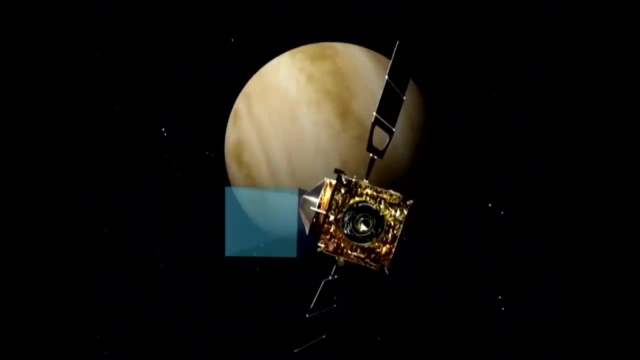 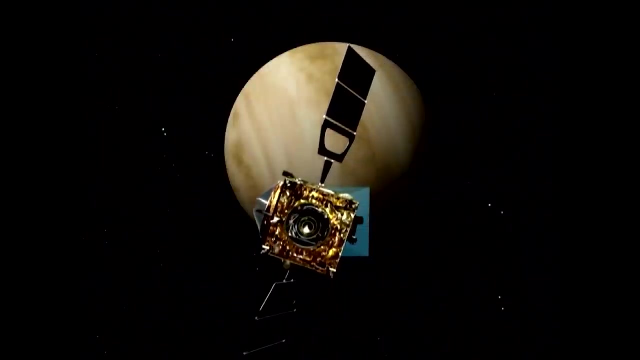 it registered a sharp rise in the atmosphere's sulfur dioxide. This could be due to changes in wind patterns, but it could also be a sign of volcanic activity. Researchers also saw increases in infrared radiation coming from three different volcanic locations. More circumstantial evidence. 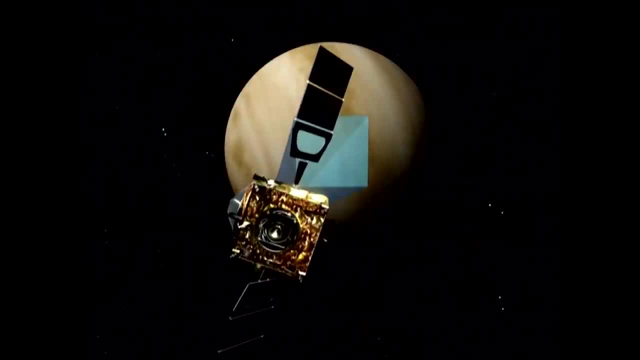 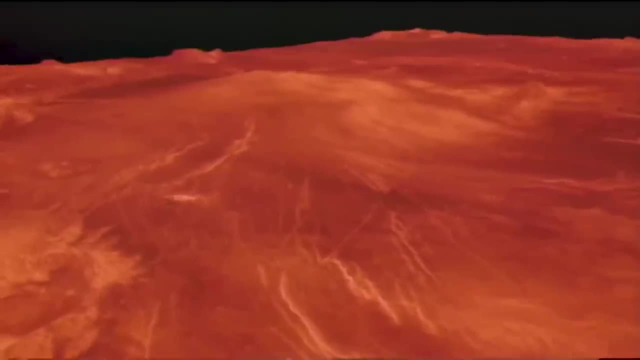 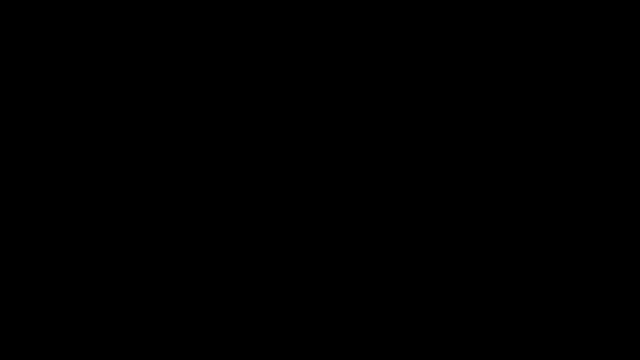 of current volcanic activity. Finally, the infrared team saw short-term temperature changes that fluctuated over just a few days. It appears that volcanoes may still be active on Venus. The mission ended in 2015 with a series of swoops into the upper atmosphere. 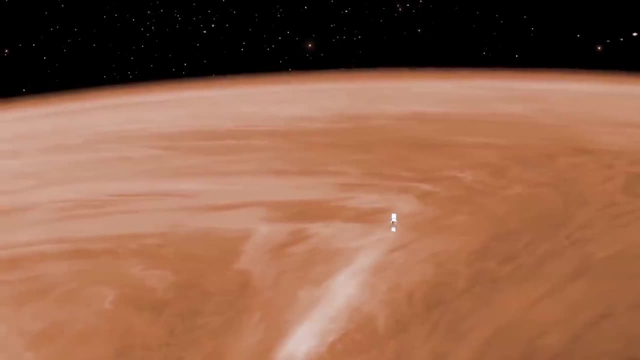 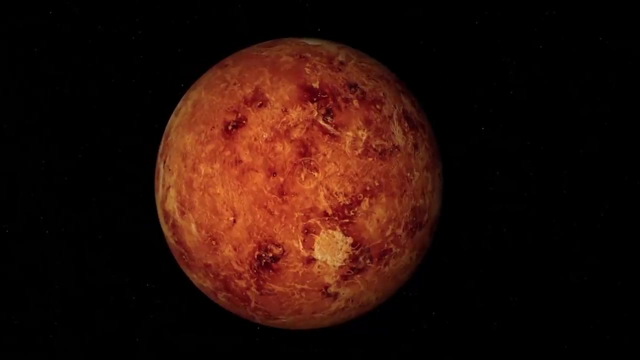 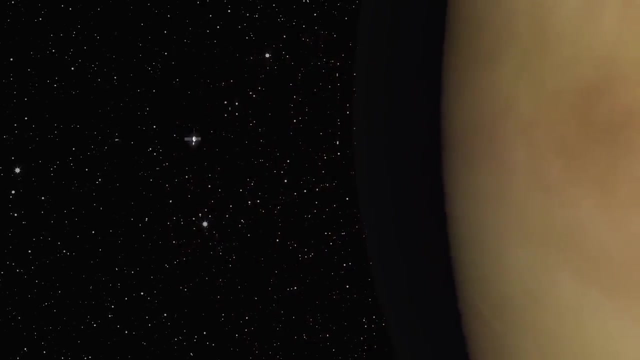 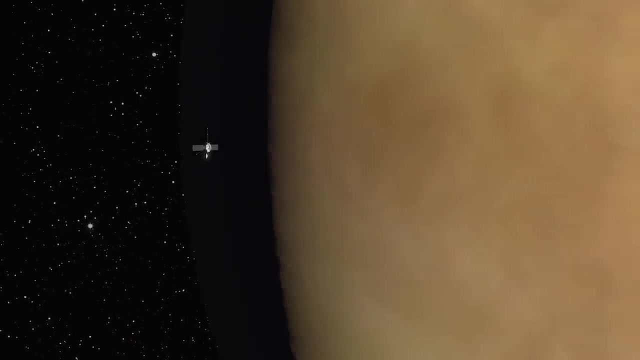 that verified unexpected ripples in the mesosphere. Very little in the way of Venus exploration has happened since Venus Express. Though elaborate plans exist for future missions to Venus, nothing at this stage has been funded. Yet many missions still pass close to Venus to use its gravitation to alter their flight paths. 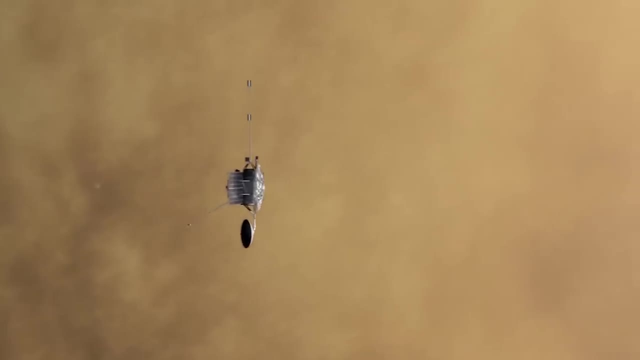 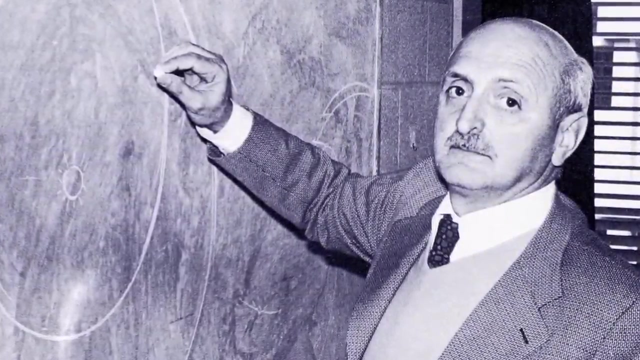 In 1971, Mariner 10 was the first spacecraft ever to use the gravitational slingshot effect on its way to Mercury. Italian mathematician Giuseppe Colombo devised the maneuver as a way to save fuel and to fly past Mercury not once. 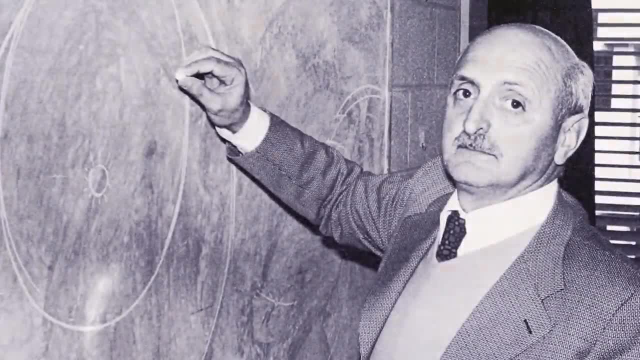 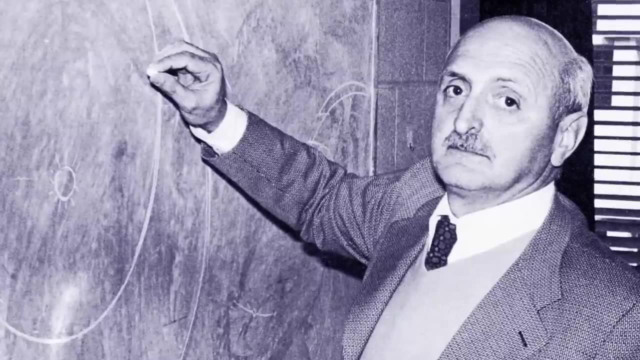 Yet many missions still pass close to Venus. Yet many missions still pass close to Venus. Yet many missions still pass close to Venus. Italian mathematician Giuseppe Colombo devised the maneuver as a way to save fuel and to fly past Mercury not once, but several times. 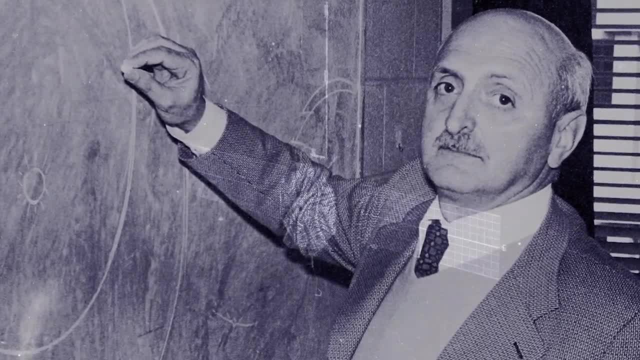 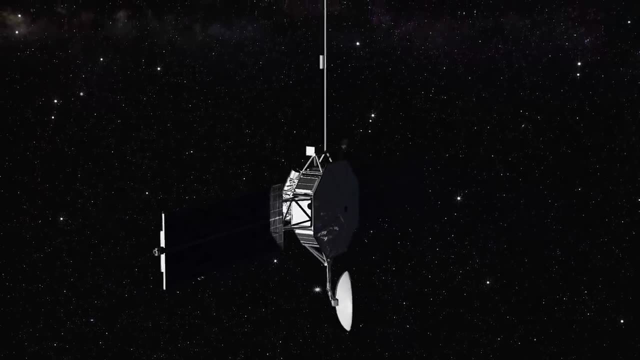 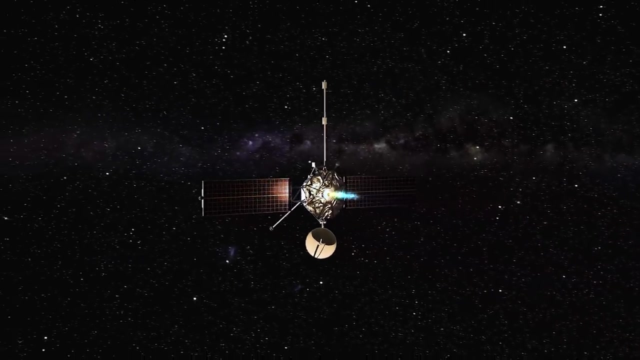 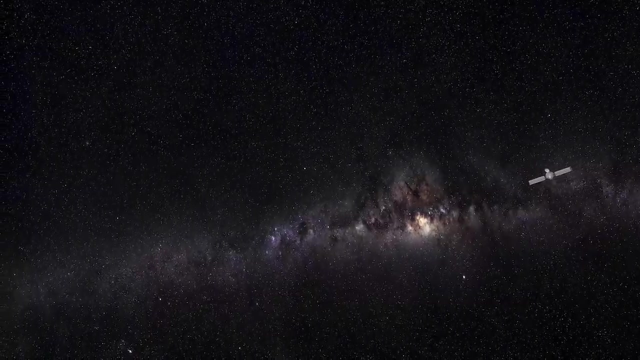 The technique is now commonplace. 10 days after launch, Mariner 10 executed instructions for a routine course correction. This appeared to go well, but after the burn, when the craft attempted to reorient itself, there was a problem. Mariner 10 knew where it was pointing. 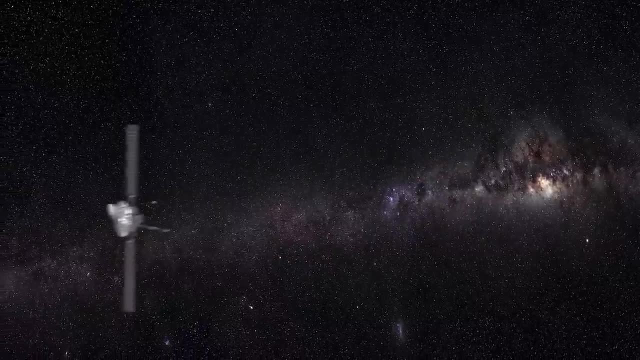 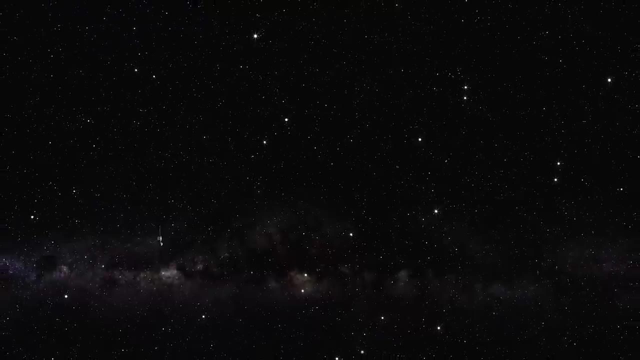 because its tracking sensor could lock onto the star Canopus, but a flake of paint that had come from the spacecraft was confusing the system. An automated backup procedure found Canopus again, but flaking paint was an issue for the rest of the mission. 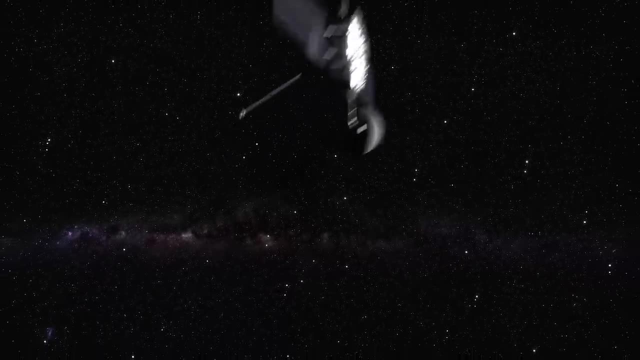 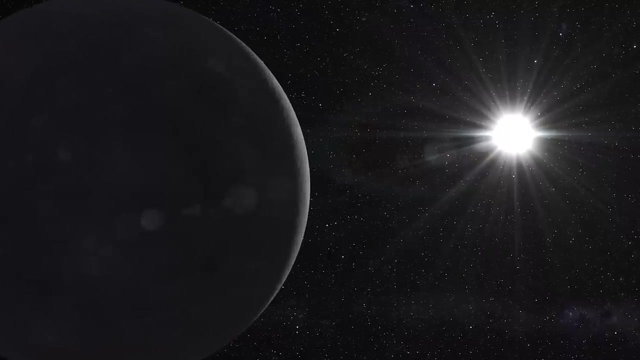 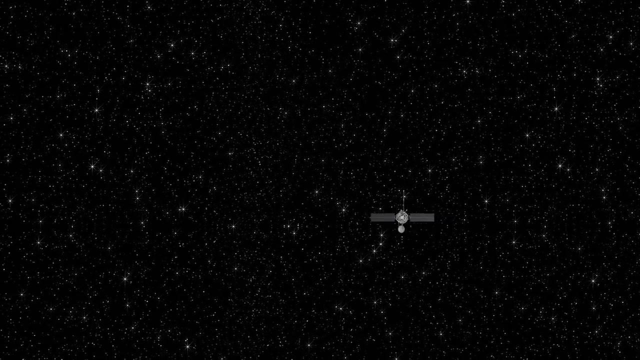 To reach Mercury, a spacecraft must approach the Sun, and its immense gravity presents a problem. Voyages to outer planets are constantly slowed by solar gravity, but with the inner planets, a spacecraft constantly accelerates. Mariner 10 used Venus's gravity to reduce its speed. 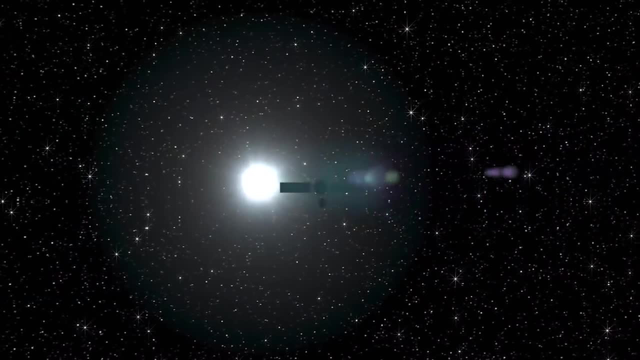 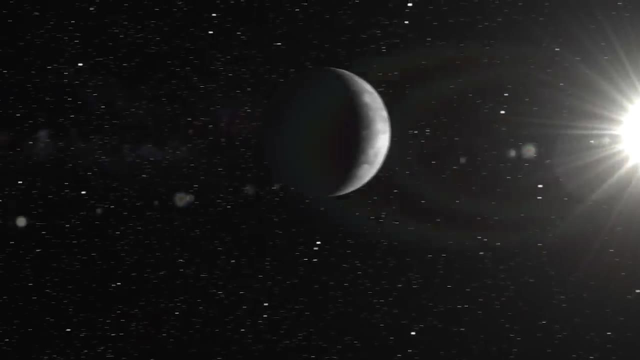 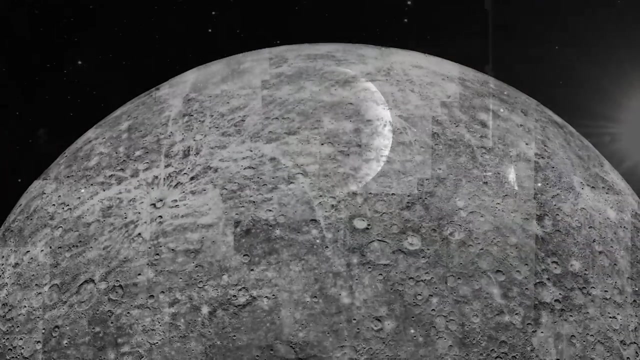 and it approached Mercury at an acute angle. Mariner 10 did not have enough fuel to go into orbit around Mercury, but its sun-centred path allowed the probe to make three close passes. Its first pass revealed a moon-like planet with a heavily cratered surface. 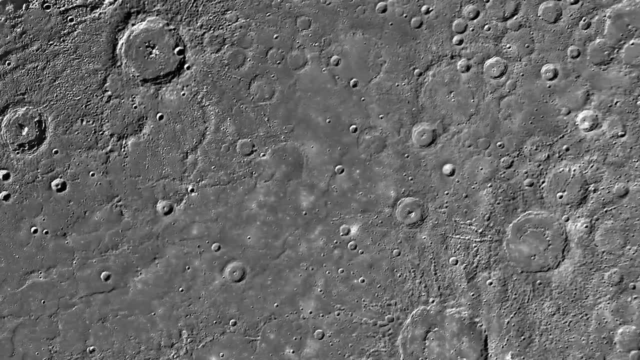 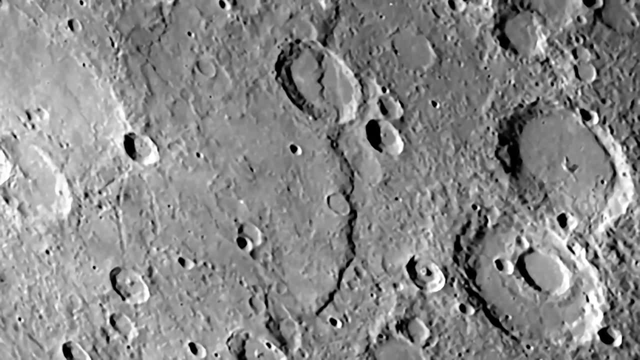 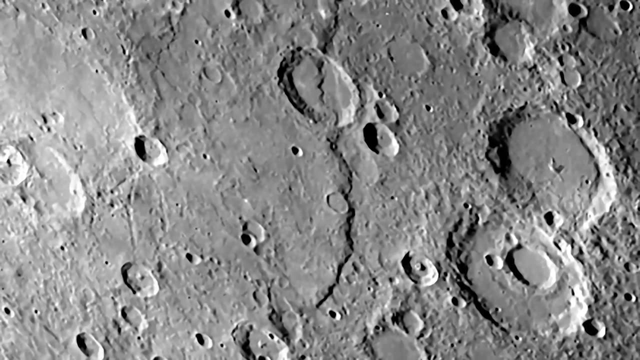 Though Mercury is the smallest planet, it's the most dense. It has a large iron-rich core. Prominent escarpments were seen Here. Discovery Scarp cuts through two craters. It falls three kilometres. It's thought that these cliffs are the result of cooling and shrinking of the core. 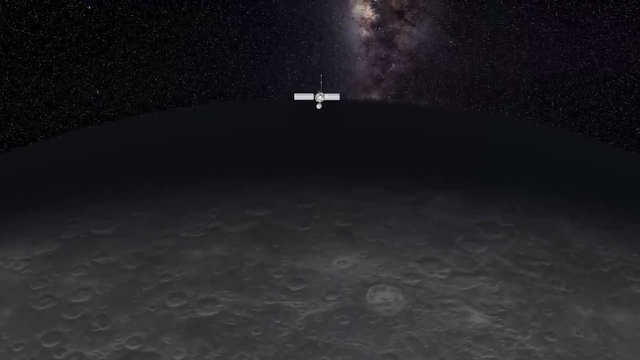 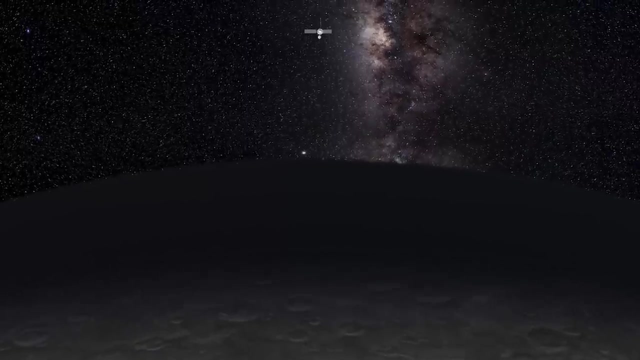 Mariner 10 continued to suffer technical problems. Its tape recorder kept sticking. There were restrictions in the rates of data transmission and limited attitude control meant flight engineers were using solar pressure on the high-speed aircraft. They had to use a high-gain antenna and solar panels to compensate. 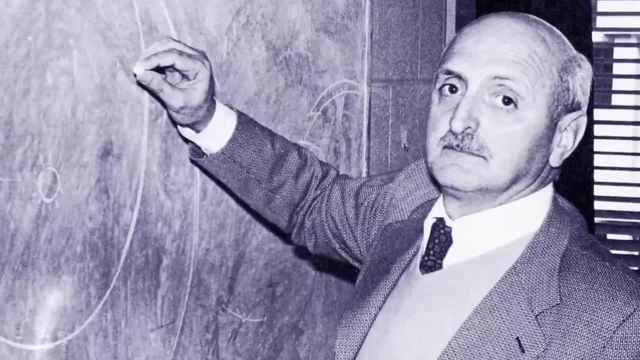 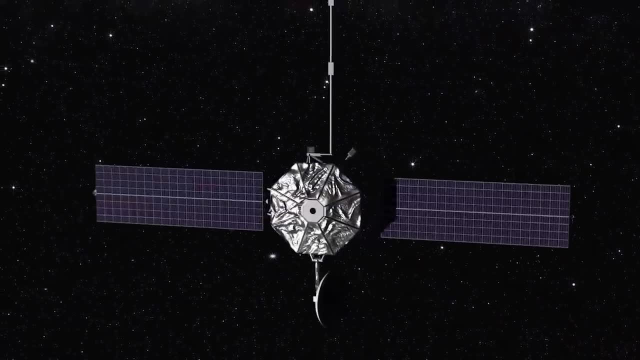 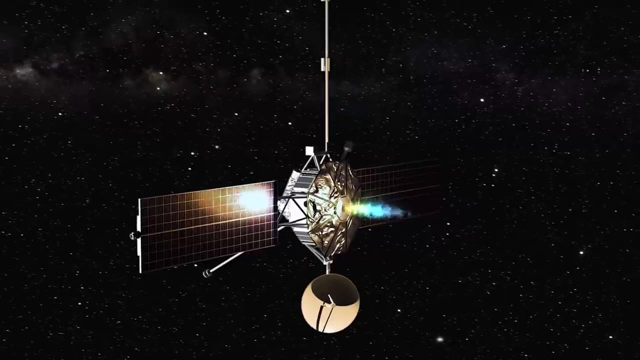 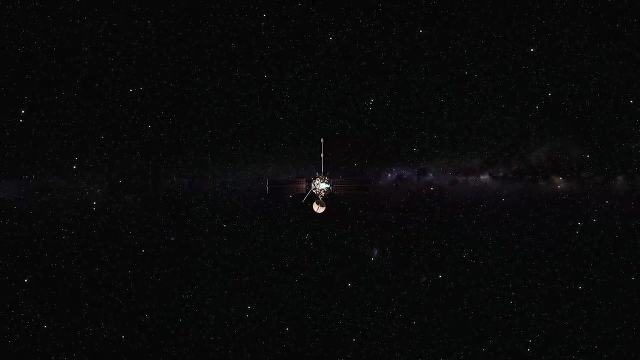 but several times. The technique is now commonplace. Ten days after launch, Mariner 10 executed instructions for a routine course correction. This appeared to go well, But after the burn, when the craft attempted to reorient itself, there was a problem. 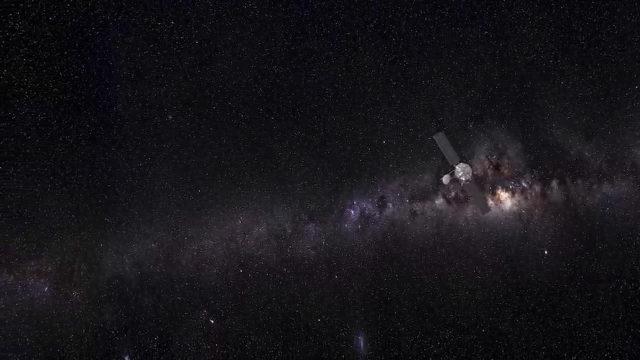 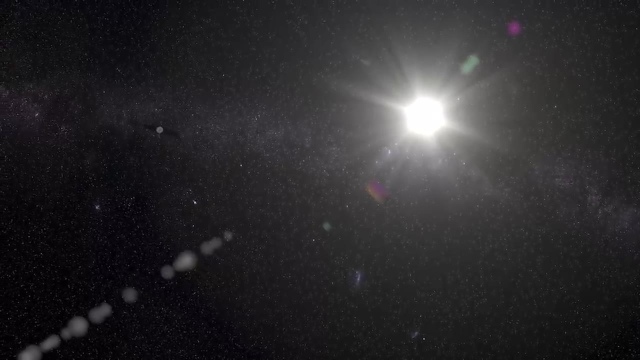 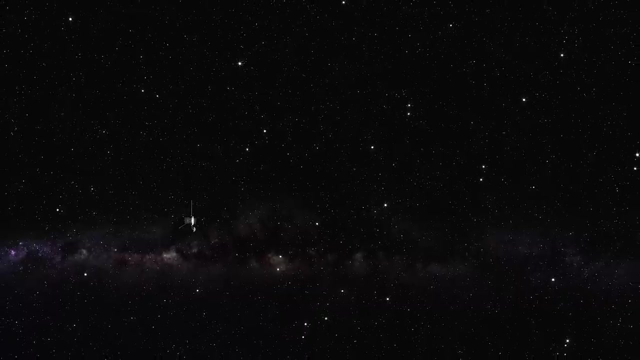 Mariner 10 knew where it was pointing because its tracking sensor could lock onto the star Canopus, But a flake of paint that had come from the spacecraft was confusing the system. An automated backup procedure found Canopus again, but flaking paint was an issue for the rest of the mission. 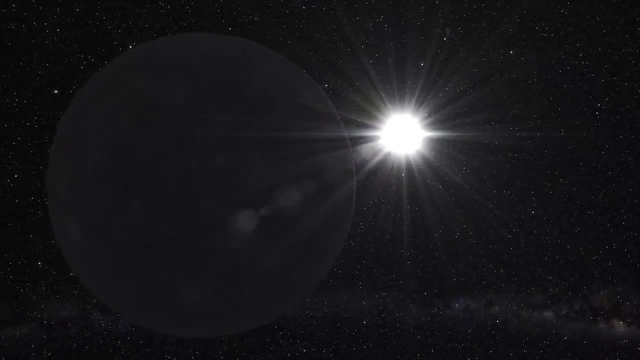 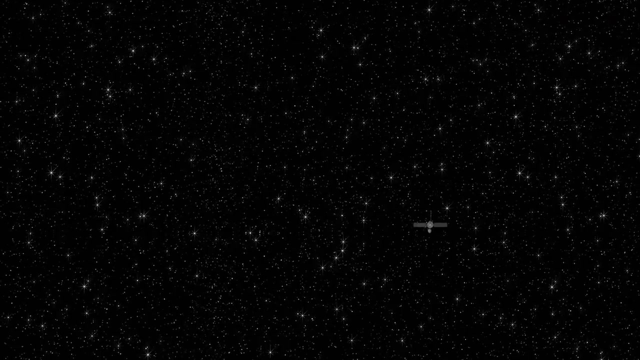 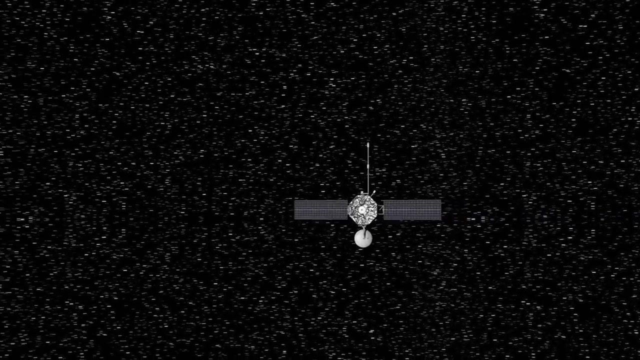 To reach Mercury, a spacecraft must approach the Sun, and its immense gravity presents a problem. Voyages to outer planets are constantly slowed by solar gravity, But with the inner planets, a spacecraft constantly accelerates. Mariner 10 used Venus's gravity. 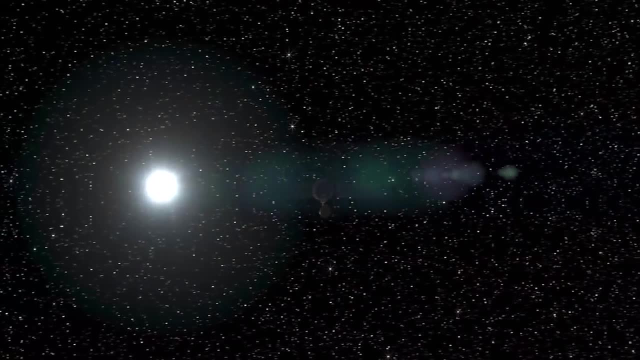 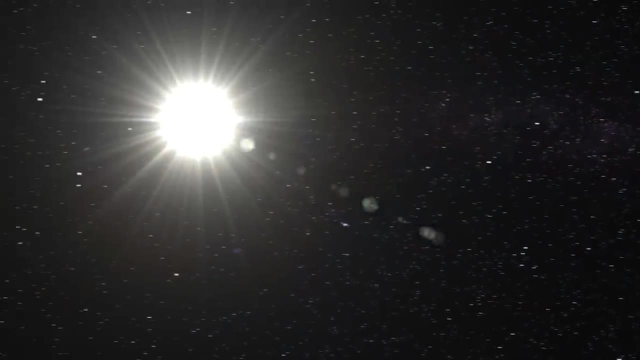 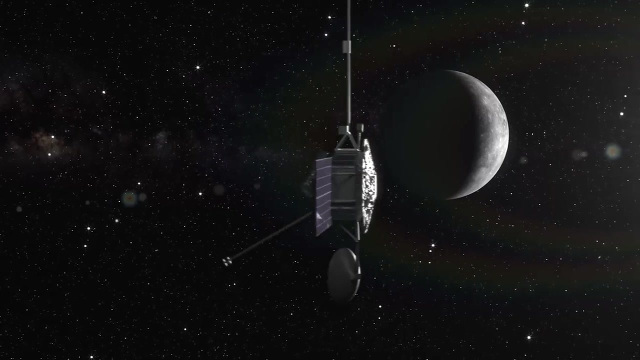 to reduce its speed and it approached Mercury at an acute angle. Mariner 10 did not have enough fuel to go into orbit around Mercury, but its Sun-centered path allowed the probe to make three close passes. Its first pass revealed a moon-like planet. 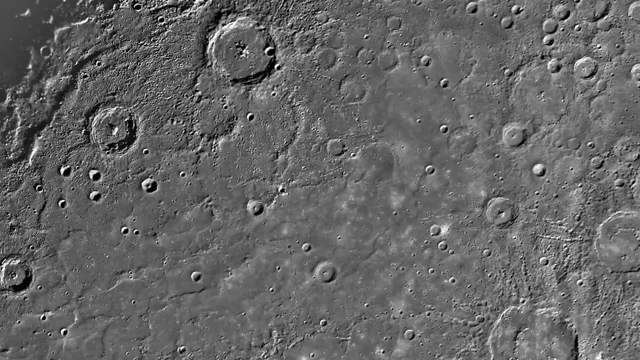 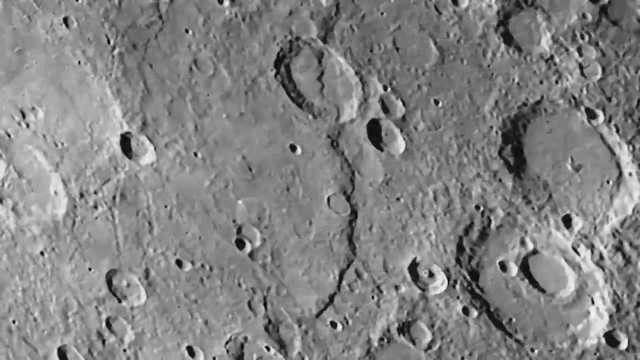 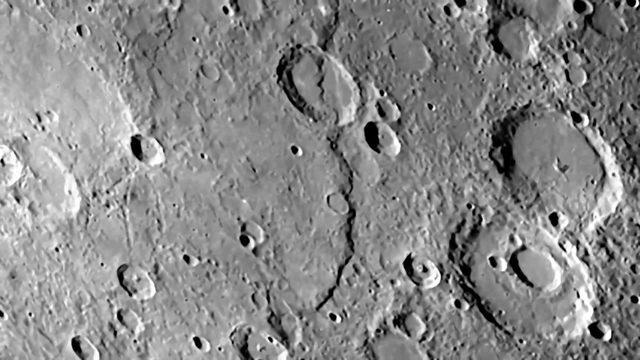 with a heavily cratered surface. Though Mercury is the smallest planet, it's the most dense. It has a large iron-rich core. Prominent escarpments were seen Here. Discovery Scarp cuts through two craters. It falls three kilometers. 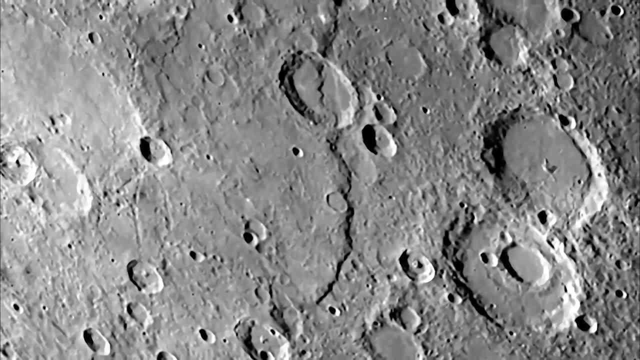 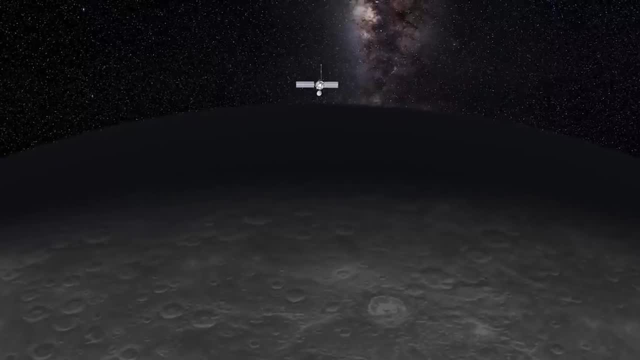 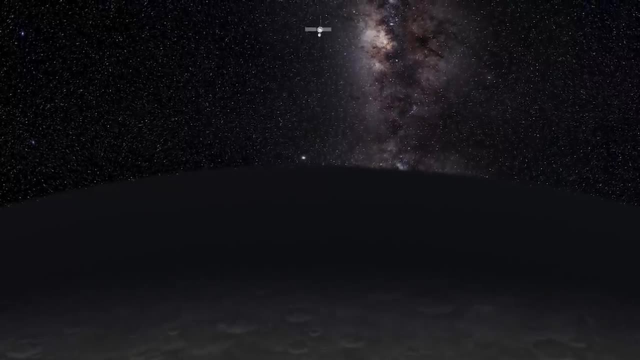 It's thought that these cliffs are the result of cooling and shrinking of the core. Mariner 10 continued to suffer technical problems. Its tape recorder kept sticking. There were restrictions in the rates of data transmission And limited attitude control meant flight engineers were using solar pressure. 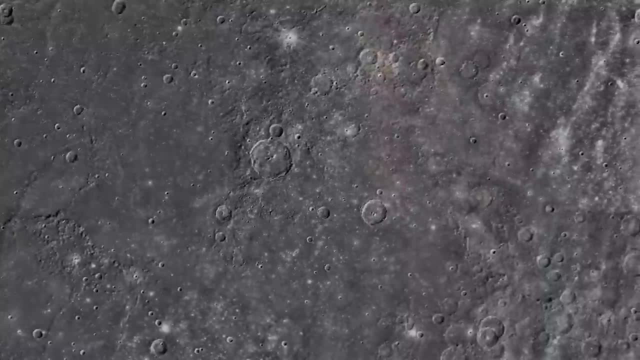 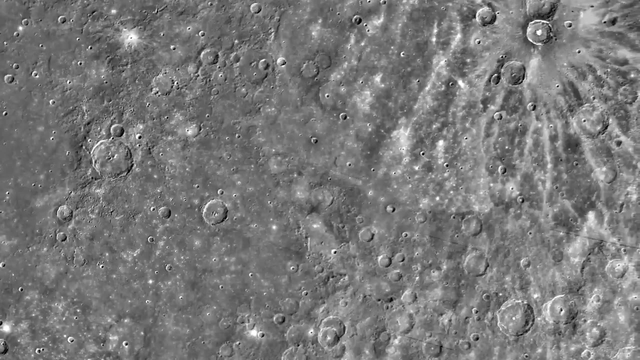 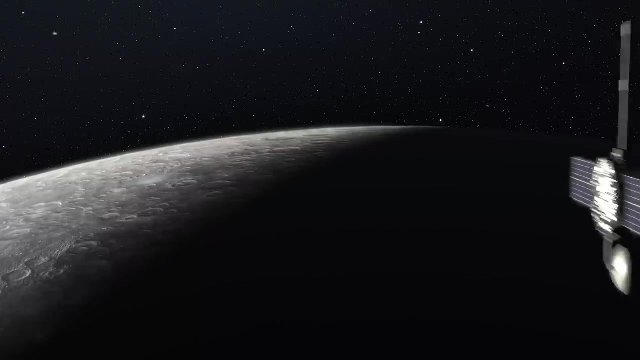 on the high-gain antenna and solar panels to compensate. Yet the mission continued. Mariner 10 could only map about 45% of Mercury's surface, as the same hemisphere faced the Sun during each of its passes, Mariner 10 discovered a very thin atmosphere. 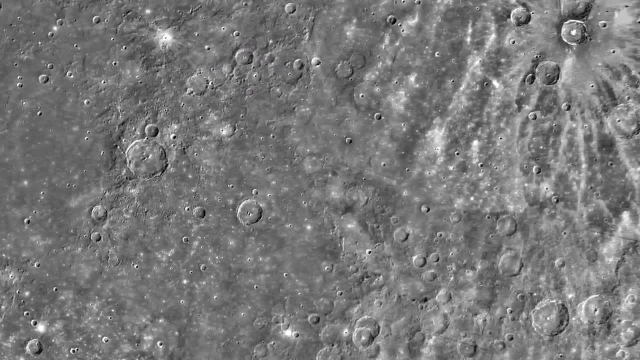 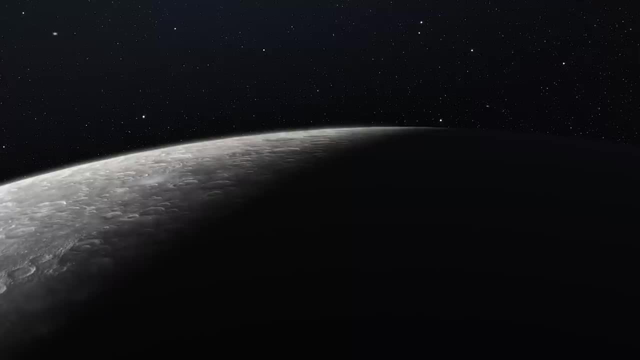 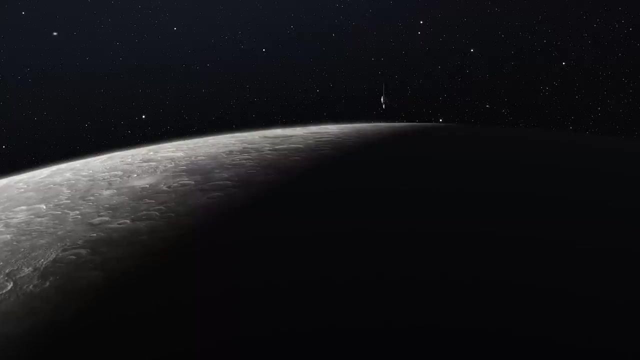 Yet the mission continued. Mariner 10 could only map about 45% of Mercury's surface, as the same hemisphere faced the sun. during each of its passes, Mariner 10 discovered a very thin atmosphere, primarily of helium. Several months after its third and final pass of Mercury, it ran out of fuel. 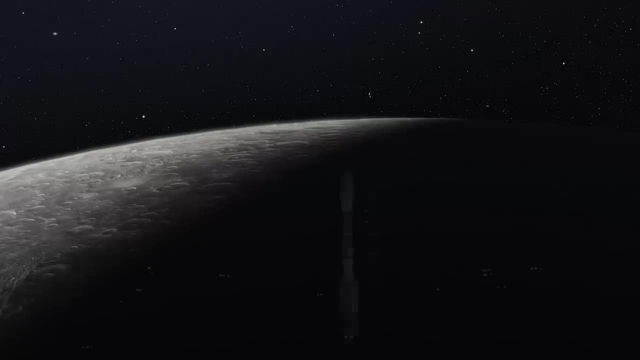 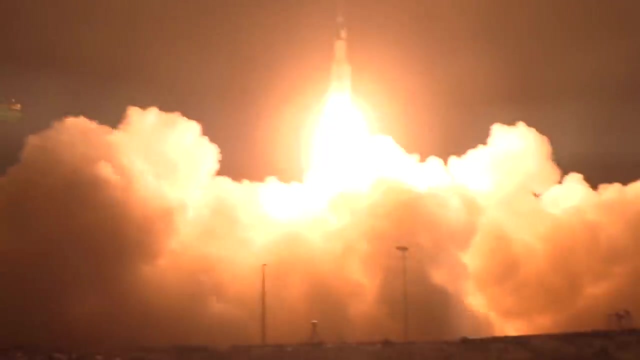 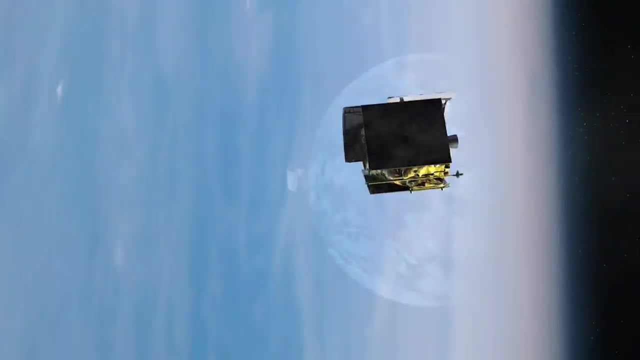 It still orbits the sun Main engine. start Two, One And zero. It was more than 30 years before the next mission to Mercury In 2004,. MESSENGER was launched. It was designed to go into orbit around Mercury. 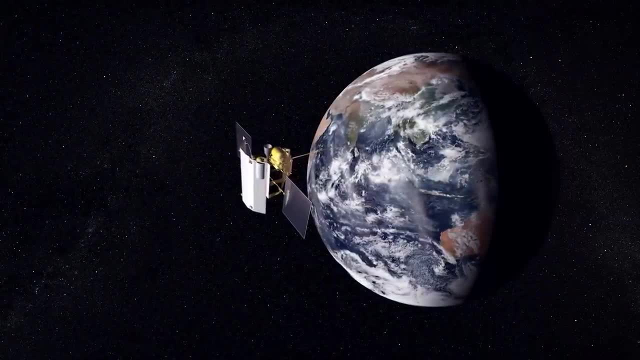 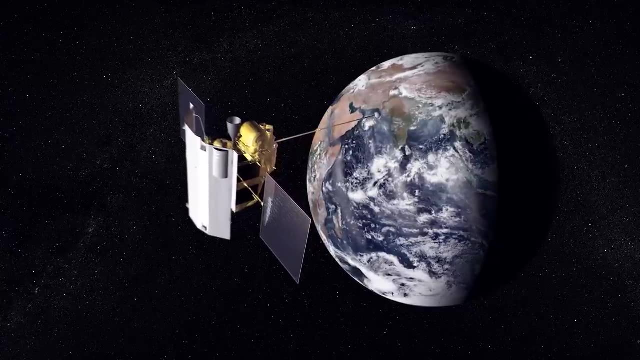 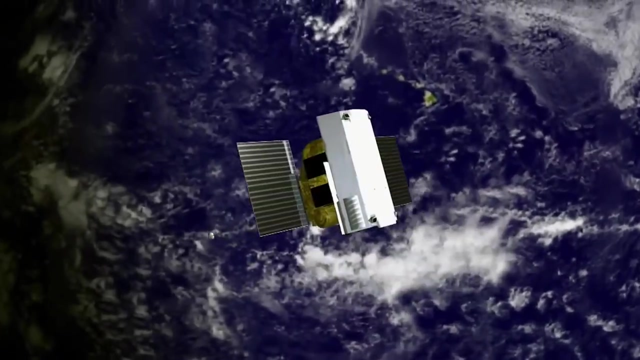 which presented a number of design constraints. It featured a large woven ceramic sunshield, but it did not have a dish antenna. It would rely on a phased array that could be electronically pointed. After a year in space, MESSENGER was back at Earth. 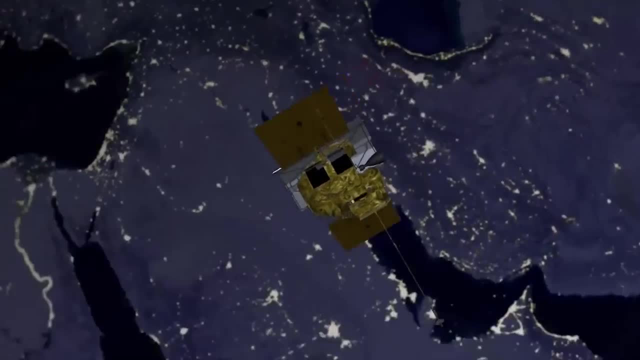 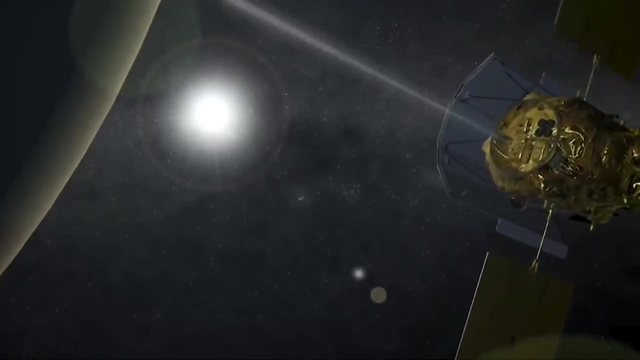 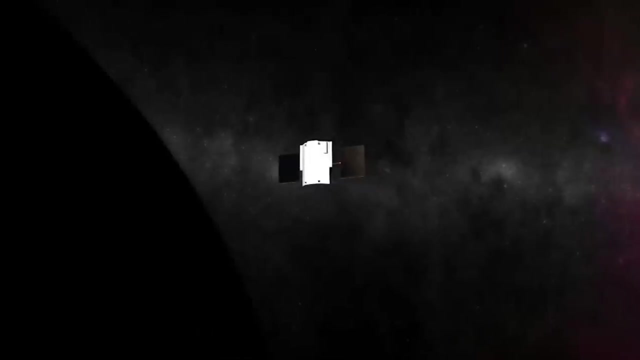 using its gravitation to modify its orbit. Even though it was not a large spacecraft, it had a powerful engine for course corrections and orbit insertion. It continued on to pass Venus twice, to lose speed as it drew closer to the sun. Three and a half years after launch. 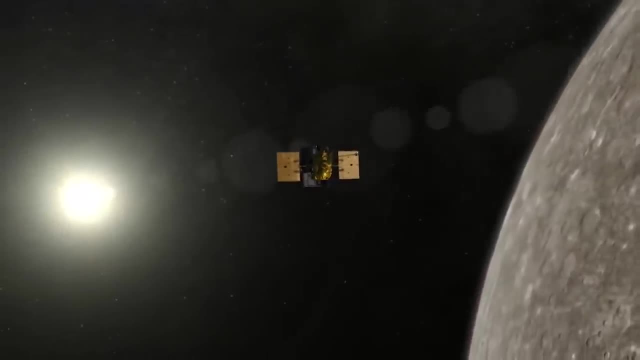 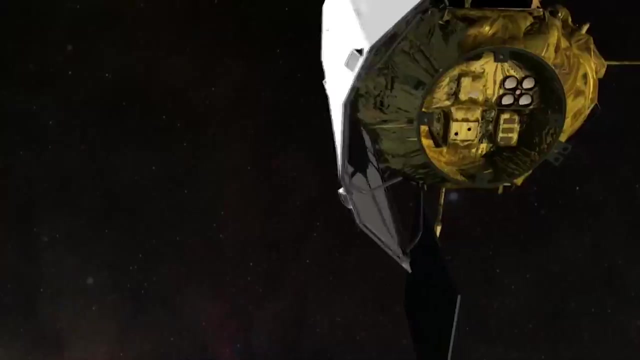 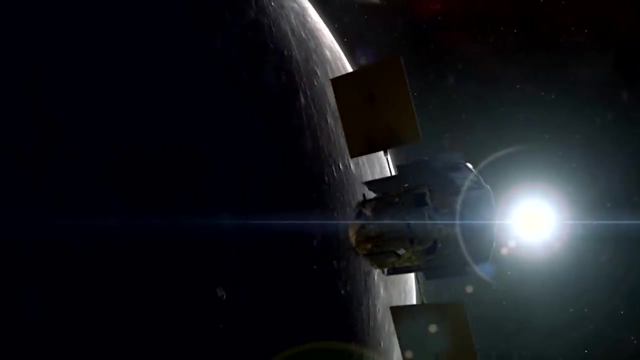 MESSENGER approached Mercury, but this was not the end of its journey. The probe made two more passes of Mercury before finally going into orbit after almost seven years in space Mission. engineers had the extra problem of always requiring the probe's sunshield to be pointed toward the sun. 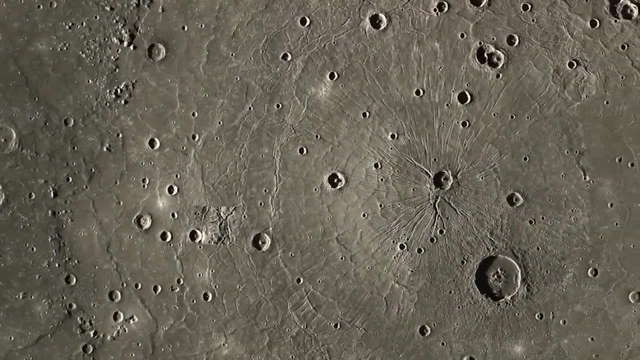 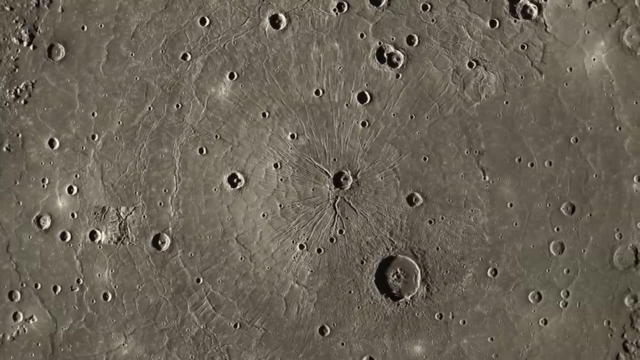 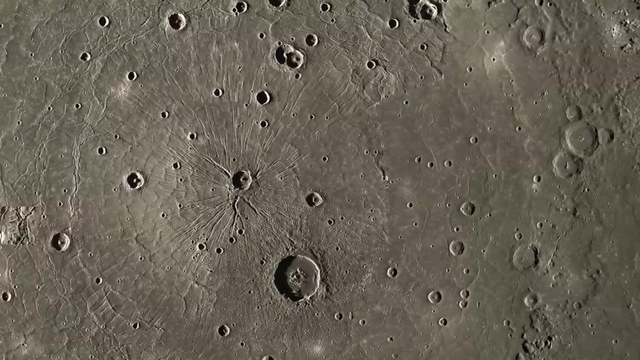 Because it was in orbit, MESSENGER was able to complete the mappings started by Mariner 10.. The planet's dominant feature is the Caloris basin. It's an ancient crater more than 1,500 kilometers across. Mariner 10 saw some of the area. 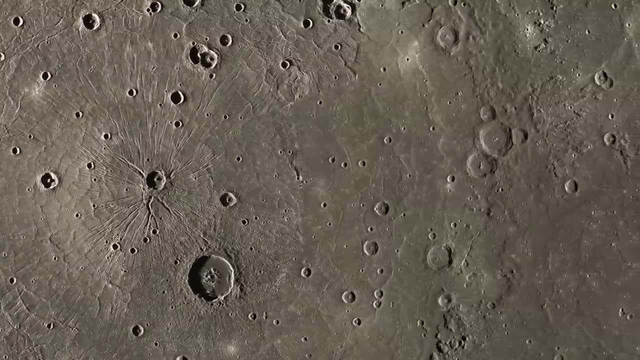 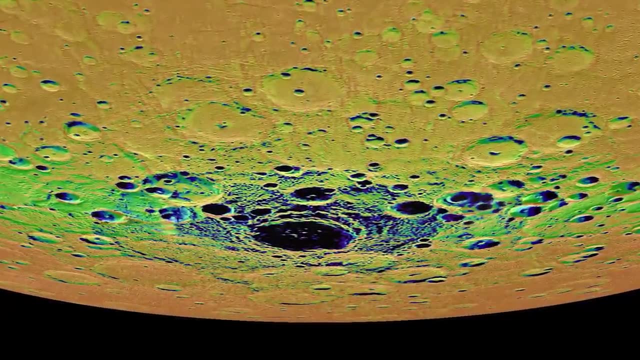 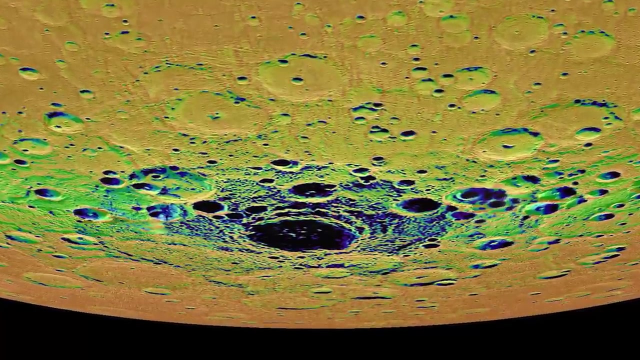 but the rest had been in darkness. This map of the southern polar region uses color to represent illumination. Because Mercury's axis is not tilted, sunlight cannot penetrate deep craters near the poles. It was in these areas that MESSENGER discovered substantial amounts of water ice. 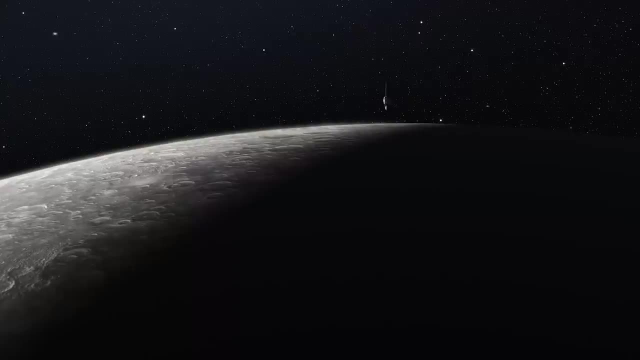 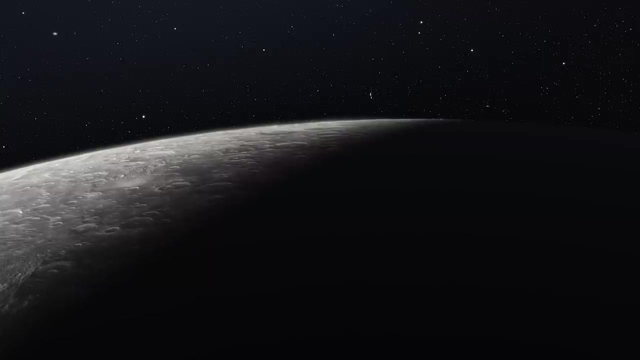 primarily of helium. Several months after its third and final pass of Mercury, it ran out of fuel. It still orbits the Sun Main engine, start Two one, and It was more than 30 years before the next mission to Mercury. In 2004,, MESSENGER was launched. It was designed to go into orbit around Mercury, which presented a number of design constraints. It featured a large woven ceramic sun shield, but it did not have a dish antenna. It would rely on a phased array. 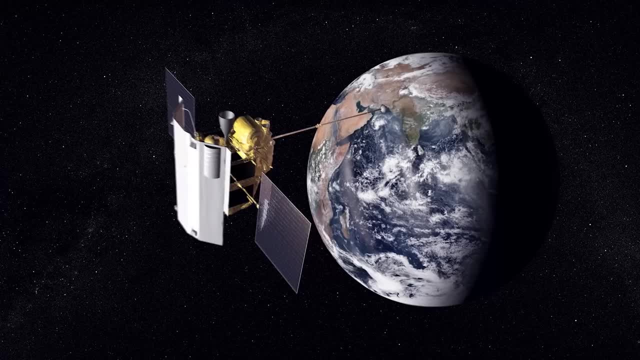 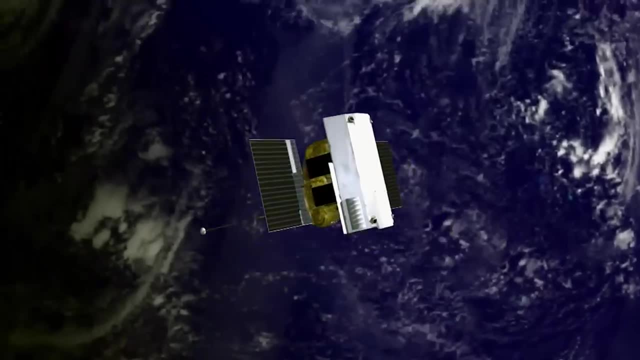 that could be electronically pointed. After a year in space, MESSENGER was back at Earth, using its gravitation to modify its orbit. Even though it was not a large spacecraft, it had a powerful engine for course corrections and orbit insertion. 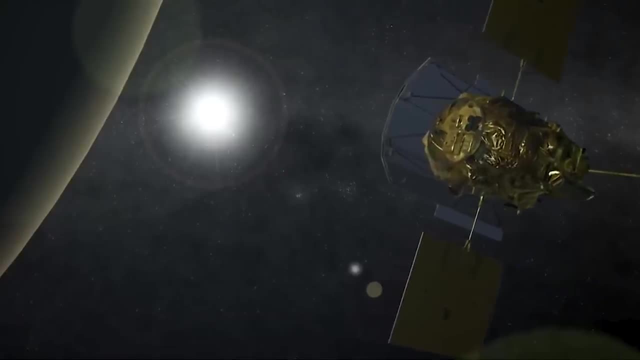 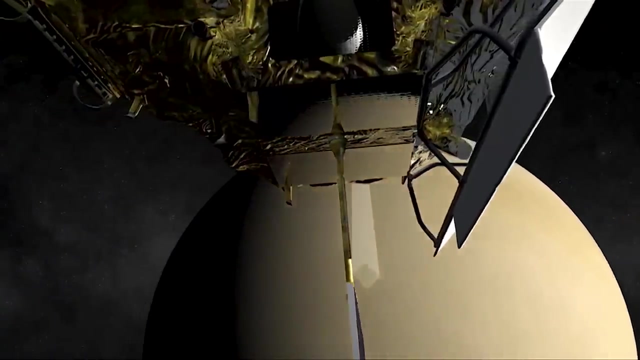 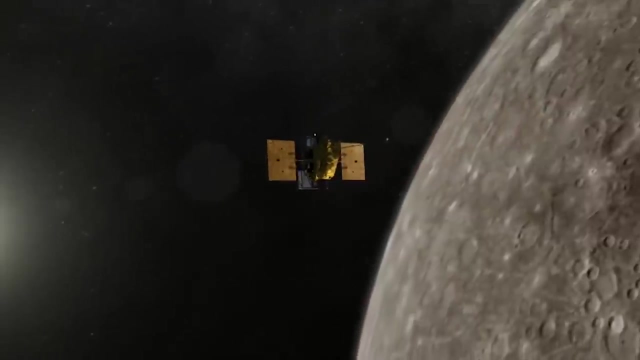 The MESSENGER was the first MESSENGER to be launched. It continued on to pass Venus twice, to lose speed as it drew closer to the Sun. Three and a half years after launch, MESSENGER approached Mercury, but this was not the end of its journey. 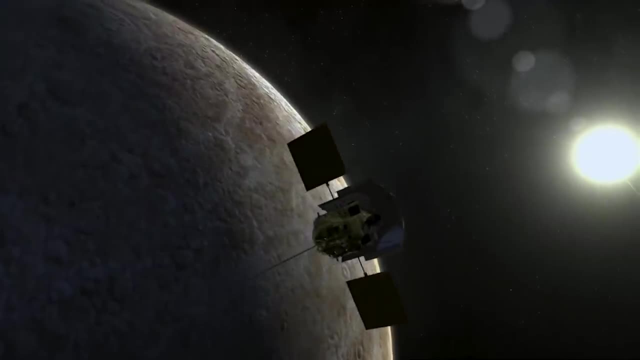 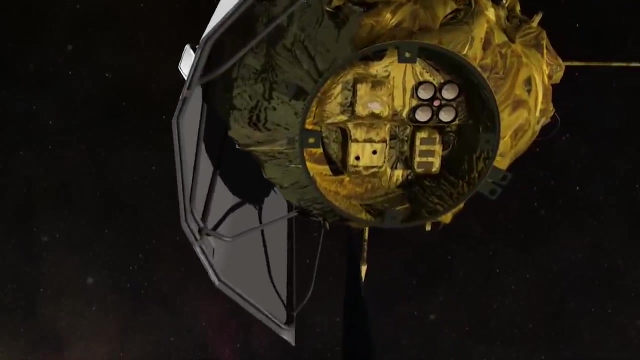 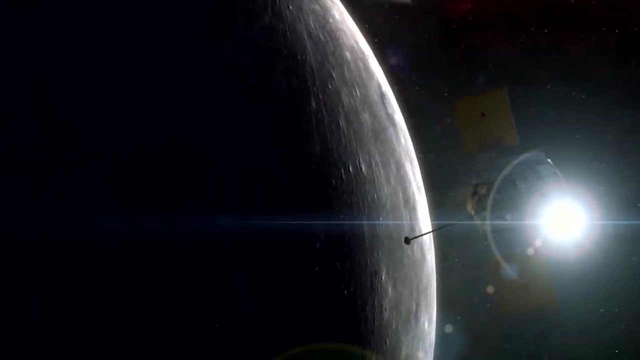 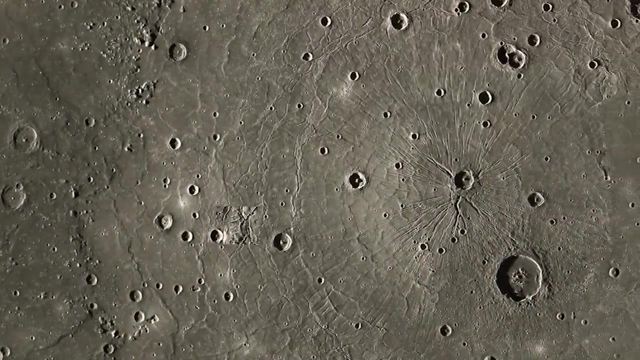 The probe made two more passes of Mercury before finally going into orbit after almost seven years in space Mission. engineers had the extra problem of always requiring the probe's sun shield to be pointed toward the Sun Because it was in orbit. MESSENGER was able to complete the mapping. 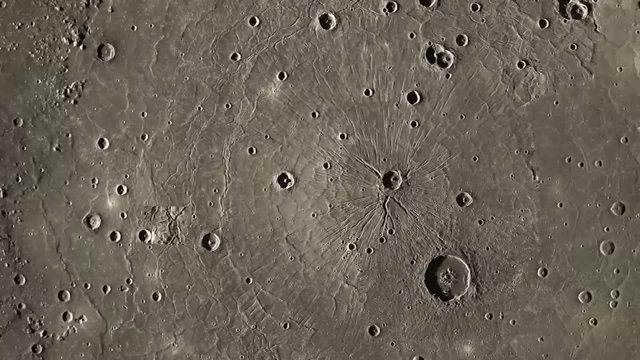 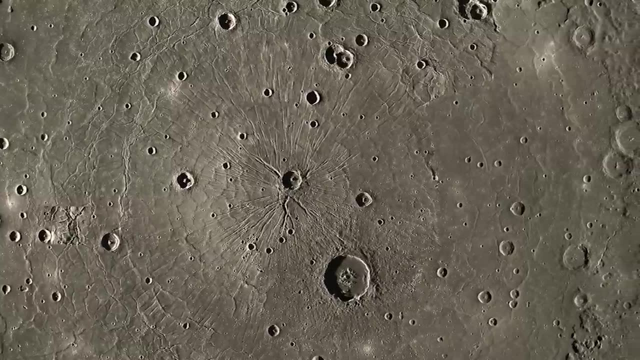 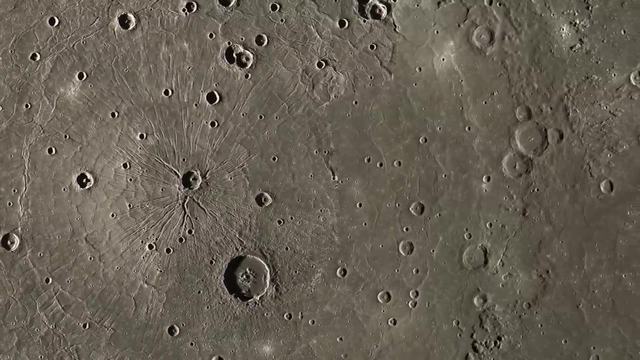 started by Mariner 10.. The planet's dominant feature is the Caloris Basin. It's an ancient crater more than 1,500 kilometres across. Mariner 10 saw some of the area, but the rest had been in darkness. This map of the southern polar region. 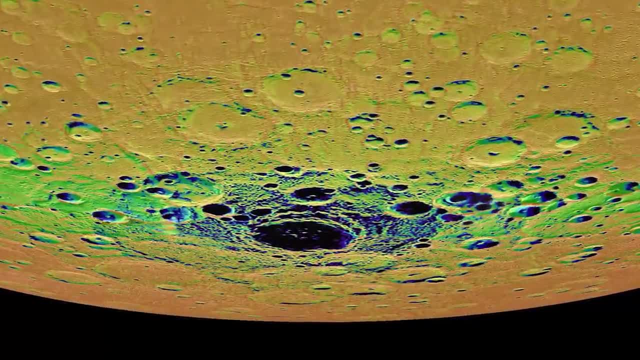 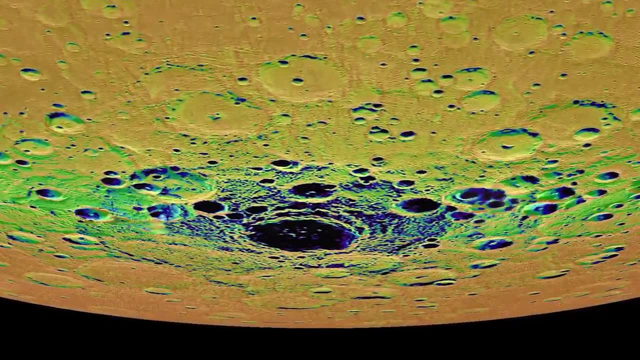 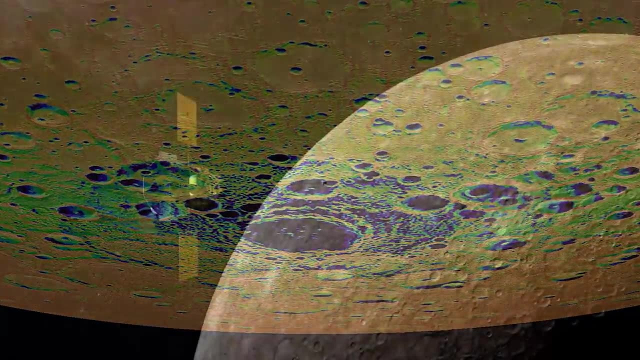 uses colour to represent illumination. Because Mercury's axis is not tilted, sunlight cannot penetrate deep craters near the poles. It was in these areas that MESSENGER discovered substantial amounts of water ice. MESSENGER received several mission extensions, but in 2015,. 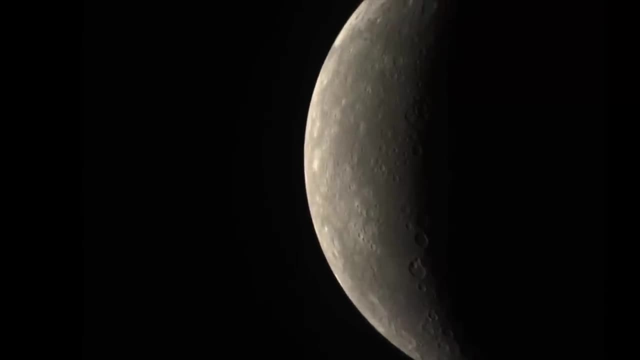 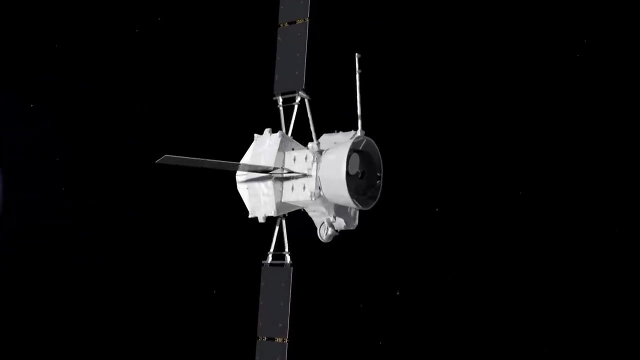 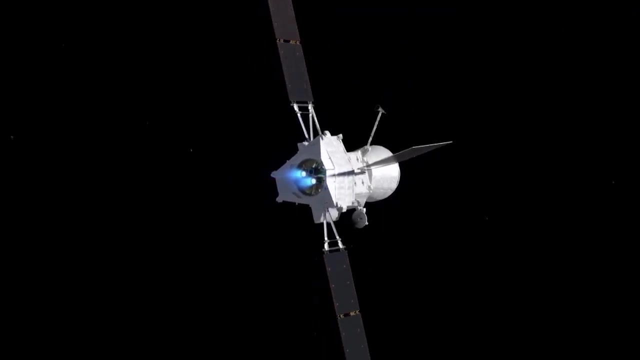 it crashed into Mercury after running out of fuel. A new mission is already on its way to Mercury, BepiColombo, named after the designer of Mariner 10's trajectory. It's a joint effort between JAXA, the Japanese space agency. 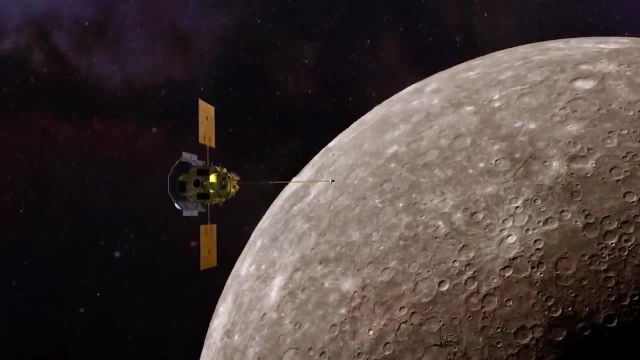 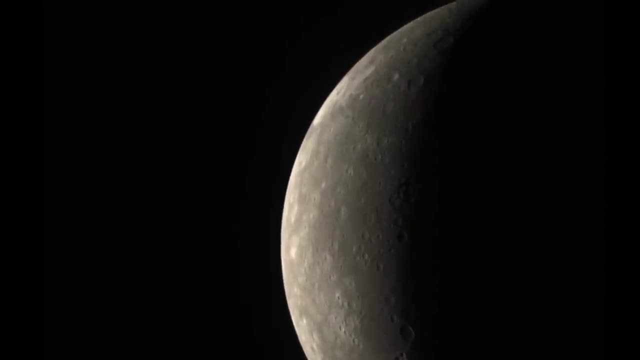 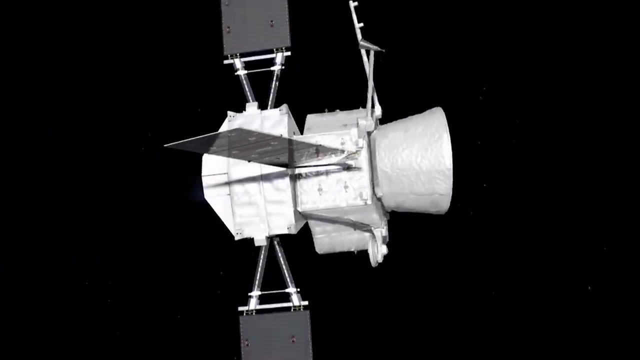 MESSENGER received several mission extensions, but in 2015 it crashed into Mercury after running out of fuel. A new mission is already on its way to Mercury, BepiColombo, named after the designer of Mariner 10's trajectory. 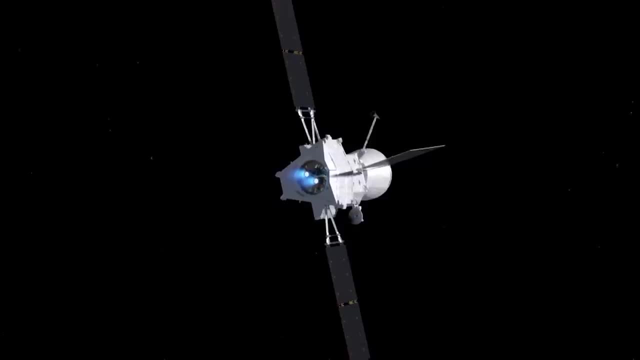 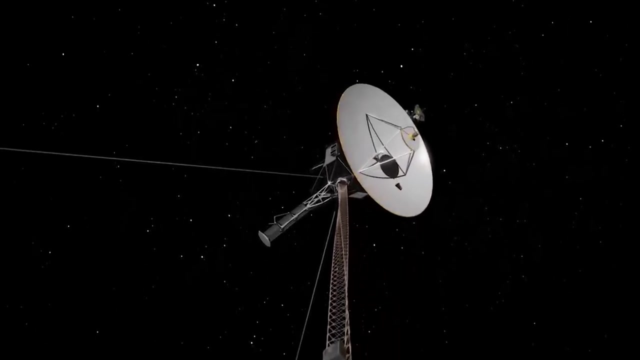 It's a joint effort between JAXA, the Japanese space agency, and the European Space Agency. It will take seven years to reach Mercury. The Voyager 2 spacecraft is the only probe to have made close approaches to the two outer ice giants. 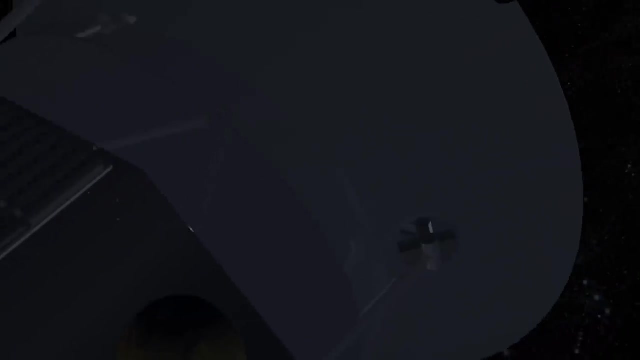 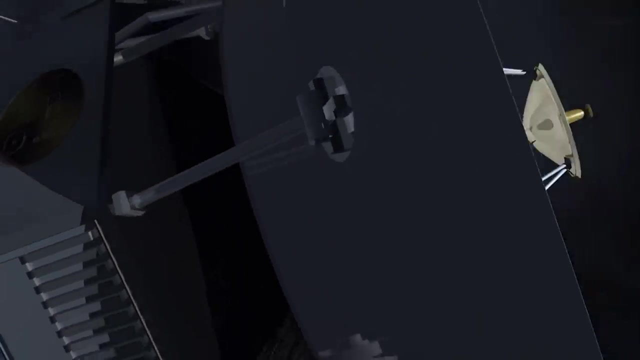 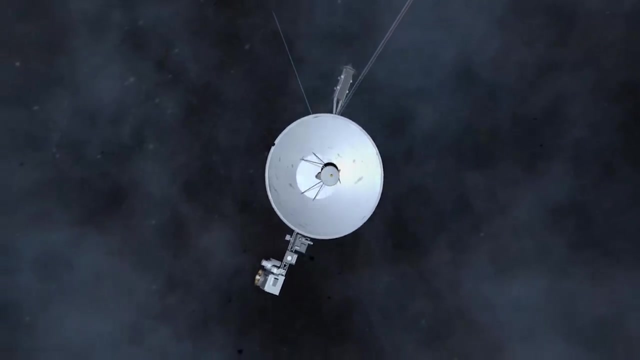 Uranus and Neptune. Launched in 1977 with its twin Voyager 1,, it was able to take advantage of a rare alignment of the four outer planets, enabling it to make close observations of each one. In 1986, Voyager approached Uranus. 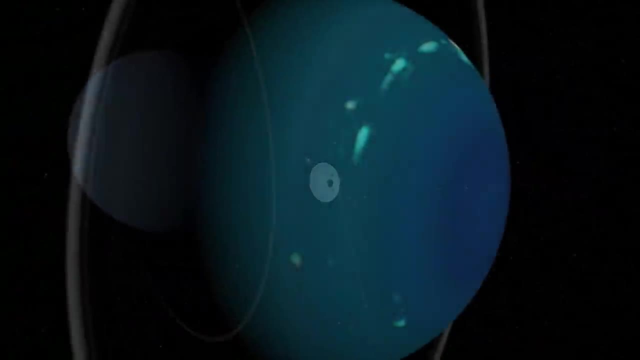 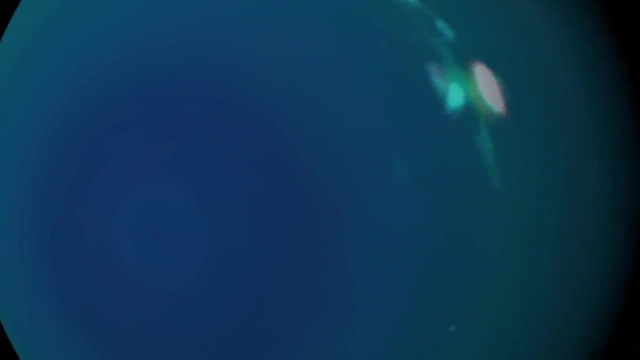 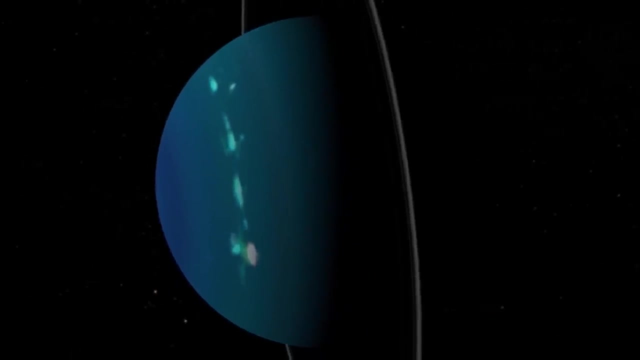 In the distant past, it must have been hit by another massive body that knocked its axis sideways. Uranus has an east and a west pole, and for half its orbit one side sees continual sun, while the other remains in darkness. It has rings which follow its north-south equator. 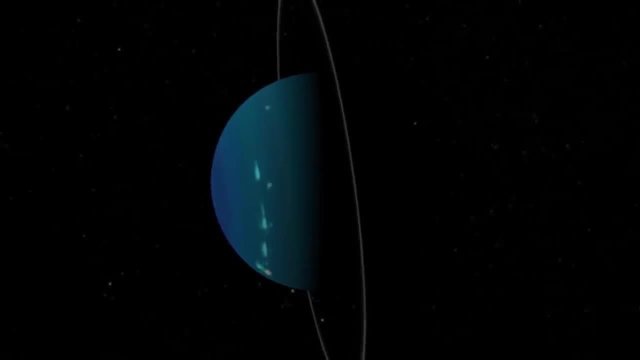 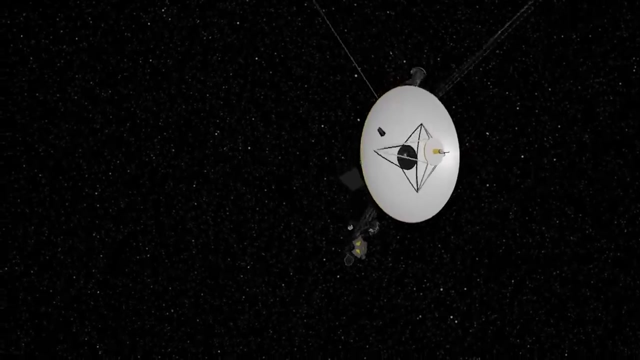 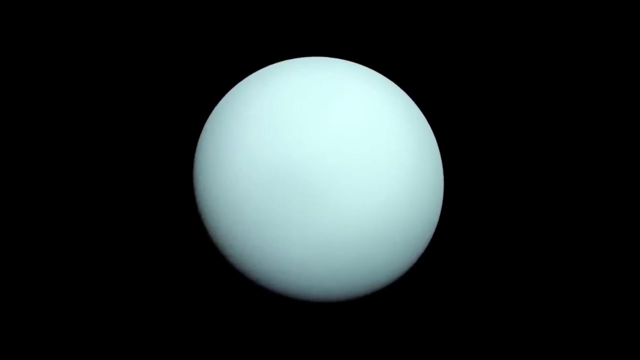 Voyager 2 discovered 11 new moons and a misaligned magnetic field. Images that the Voyager captured showed Uranus as a bland, featureless planet, But this was because Uranus was a small, tiny planet on this planet. But this was because of its particular season. 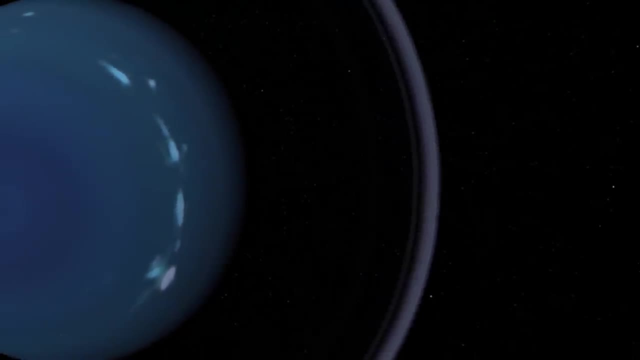 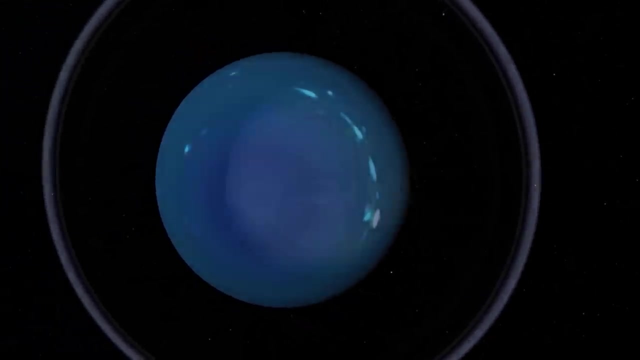 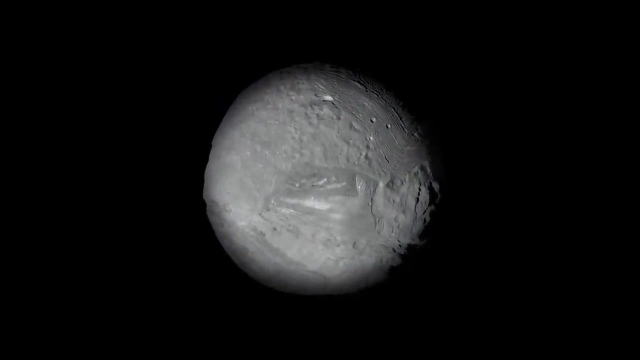 With images from the Hubble Space Telescope, we now know that at certain times, clouds and planetary weather appear in the atmosphere. Uranus's largest moon, Miranda, was observed in detail for the first time, So chaotic is its surface that researchers thought. 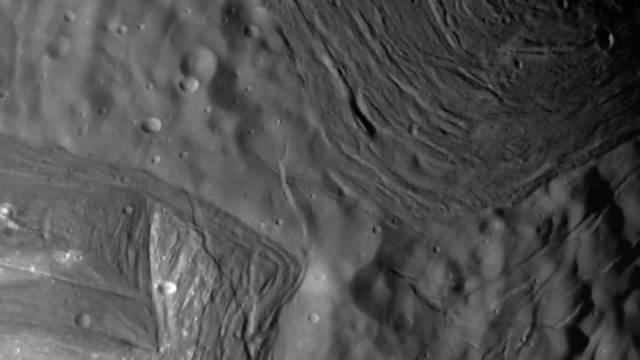 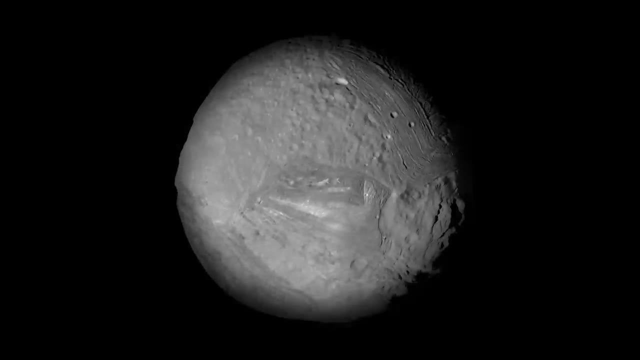 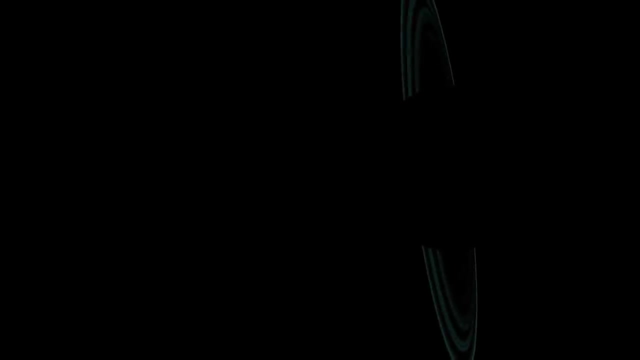 that it must have been blown apart by some cosmic impact, with fragments reforming. Now it's thought that tectonic forces initiated by the gravitation of Uranus are responsible for the moon's jumbled appearance, As Voyager 2 left Uranus. 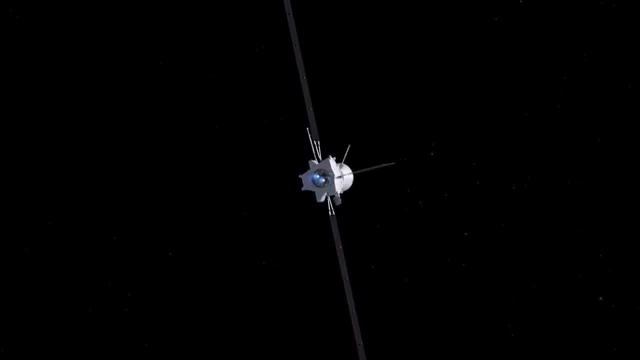 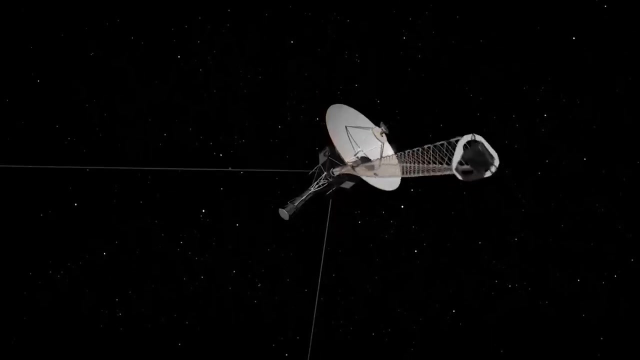 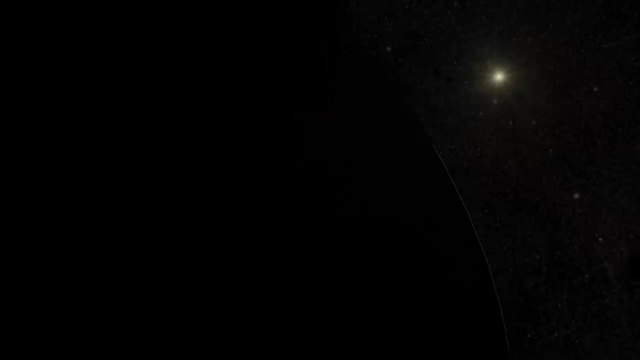 and the European Space Agency. It will take seven years to reach Mercury. The Voyager 2 spacecraft is the only probe to have made close approaches to the two outer ice giants Uranus and Neptune, Launched in 1977 with its twin Voyager 1,. 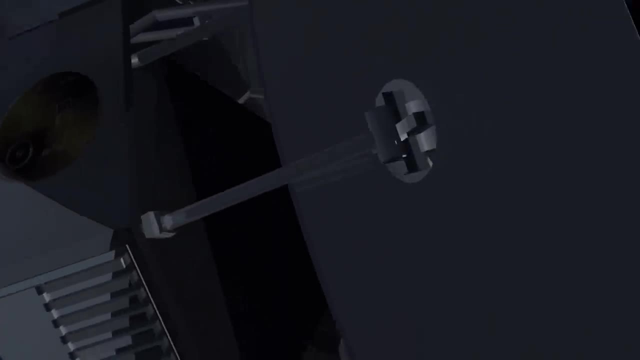 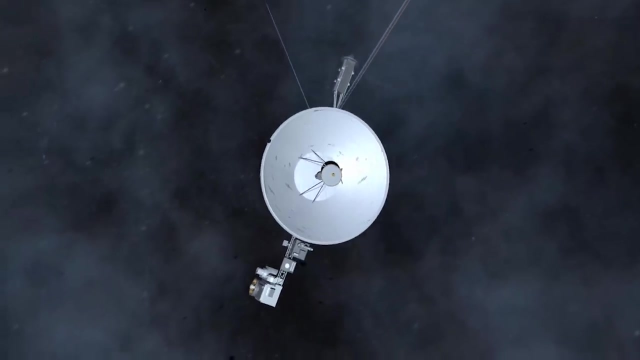 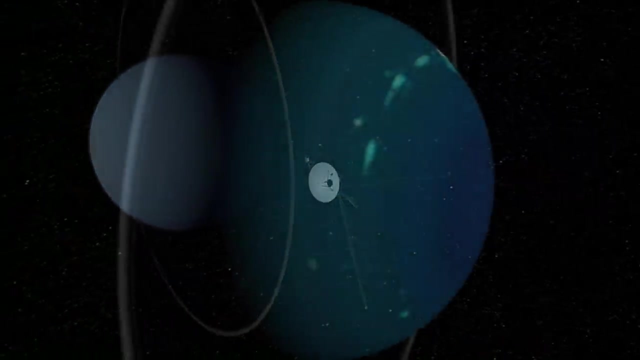 it was able to take advantage of a rare alignment of the four outer planets, enabling it to make close observations of each one. In 1986, Voyager approached Uranus. In the distant past, it must have been hit by another massive body that knocked its axis sideways. 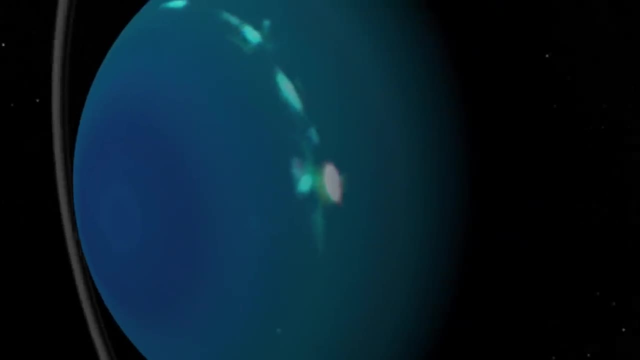 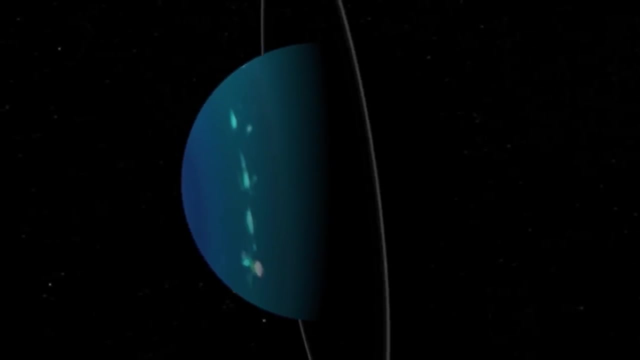 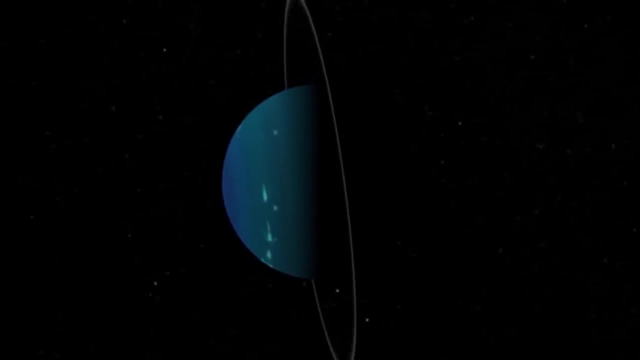 Uranus has an east and a west pole and for half its orbit, one side sees continual sun, while the other remains in darkness. It has rings which follow its north-south equator. Voyager 2 discovered 11 new moons and a misaligned magnetic field. 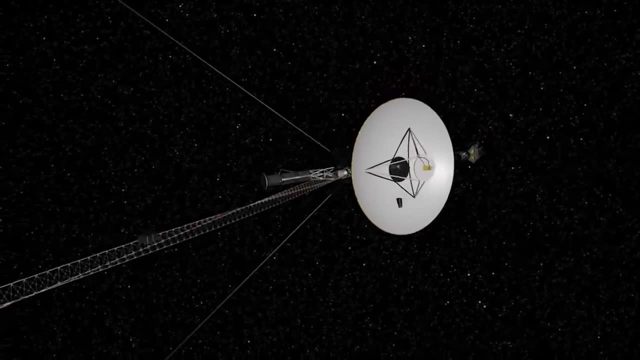 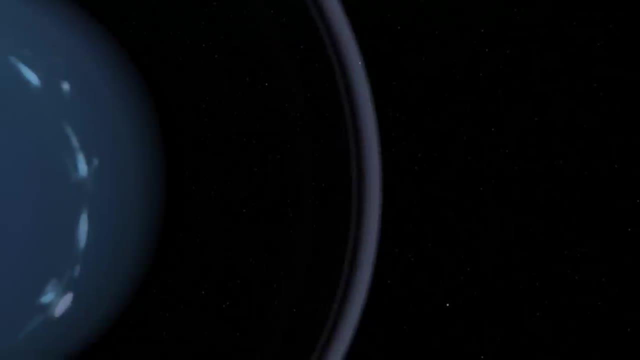 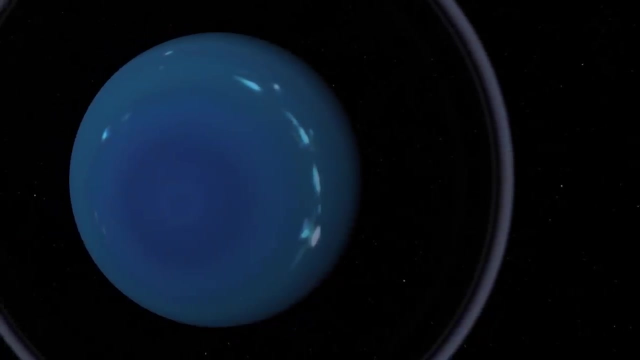 Images that the Voyager captured showed Uranus as a bland, featureless planet, But this was because of its particular season. With images from the Hubble Space Telescope, we now know that at certain times, clouds and planetary weather appear in the atmosphere. Uranus's largest moon, Miranda. 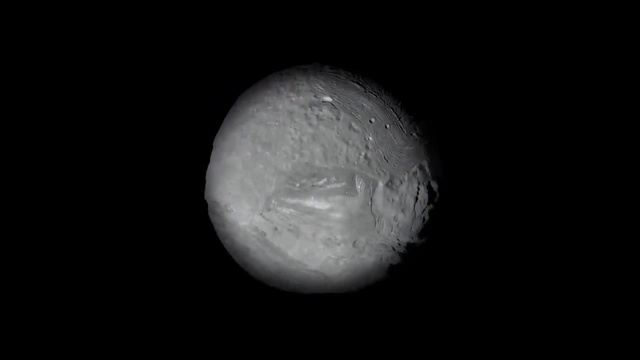 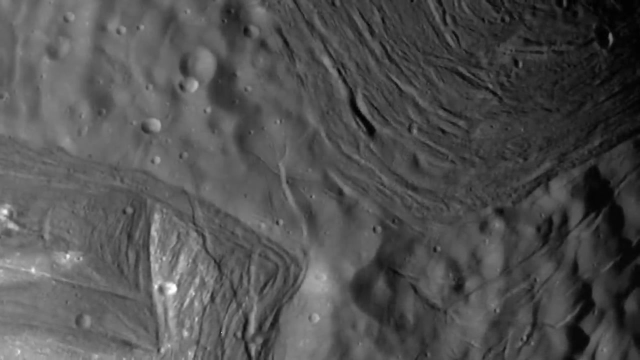 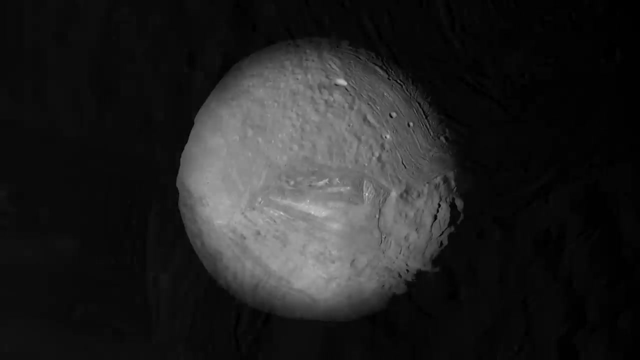 was observed in detail for the first time. So chaotic is its surface that researchers thought that it must have been blown apart by some cosmic impact, with the fragments reforming. Now it's thought that tectonic forces initiated by the gravitation of Uranus. 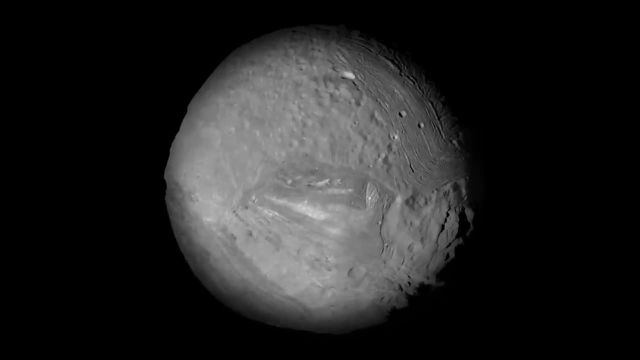 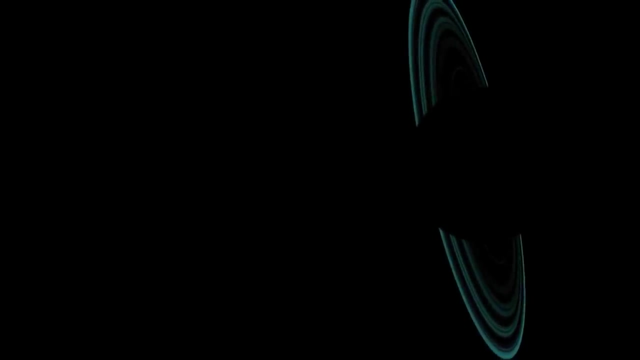 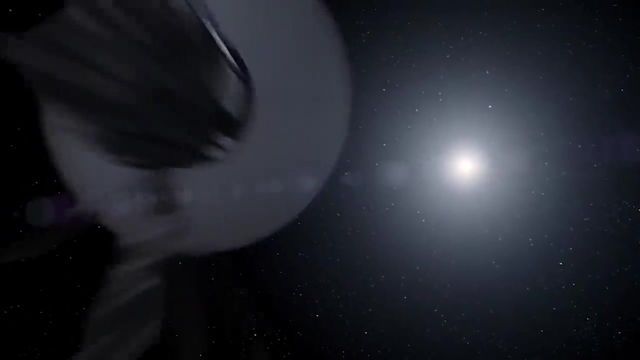 are responsible for the moon's jumbled appearance. As Voyager 2 left Uranus, backlighting from the sun revealed two new rings encircling the planet. The spacecraft was now heading toward Neptune, the solar system's last planet. In the three years it would take to get there. 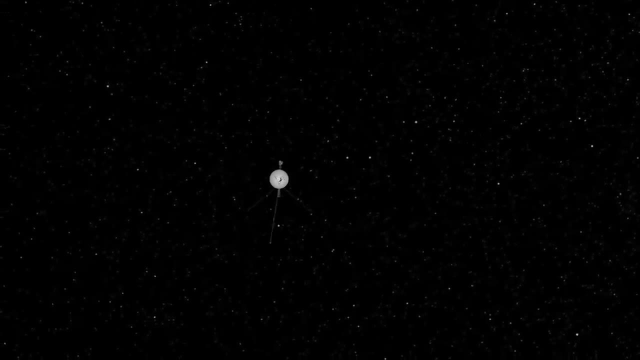 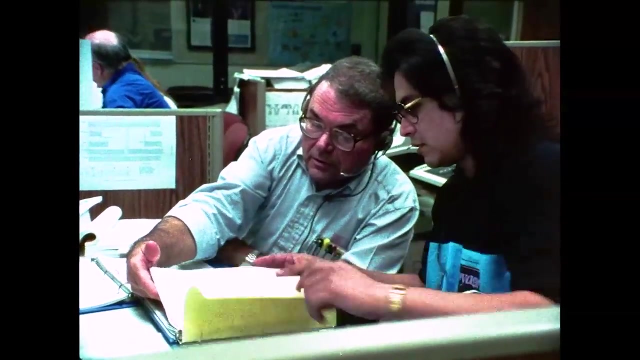 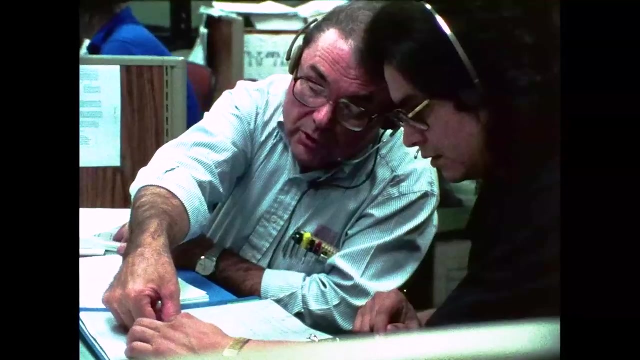 ground, engineers began preparing for unique challenges. Neptune is 30 times further from the sun than the Earth, and the light intensity is one-thousandth what it is here. For photography, time exposures would be necessary, Yet Voyager 2 was travelling so fast. 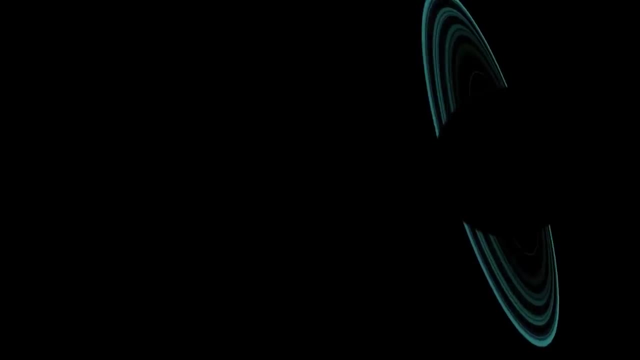 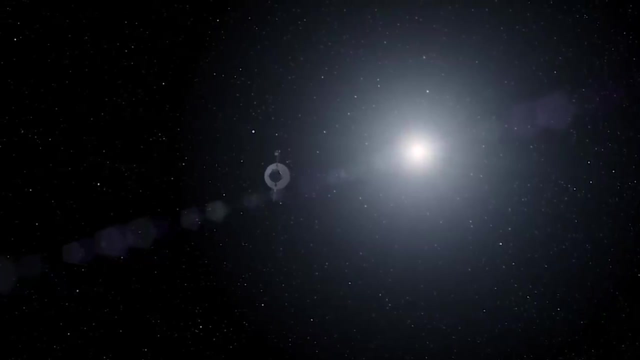 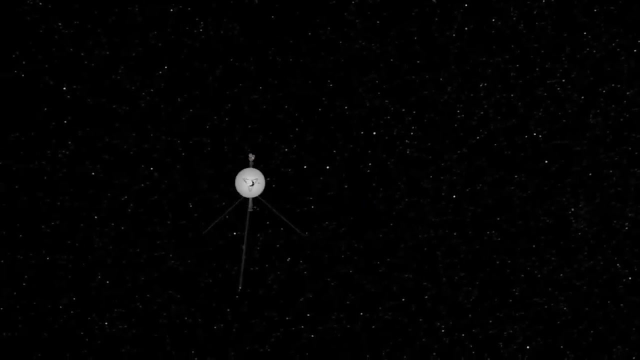 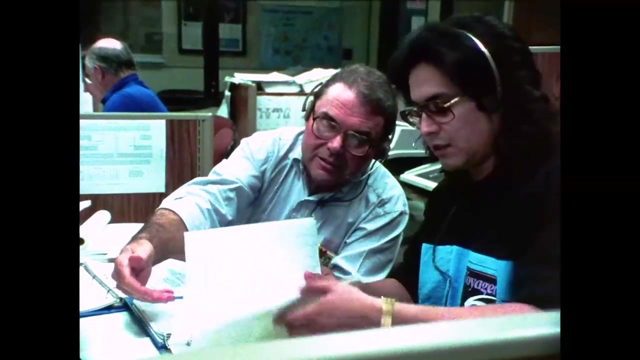 backlighting from the sun revealed two new rings encircling the planet. The spacecraft was now heading toward Neptune, the solar system's last planet. In the three years it would take to get there, ground engineers began preparing for unique challenges. Neptune is 30 times further from the sun than the Earth. 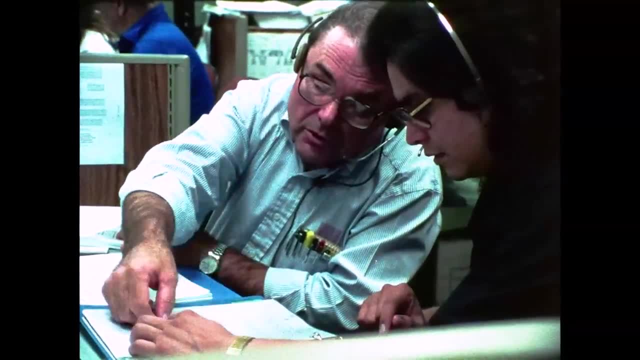 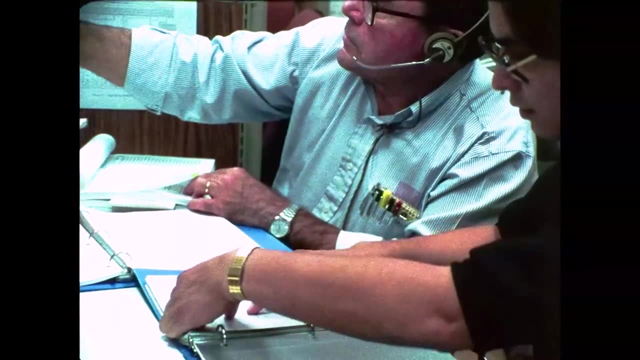 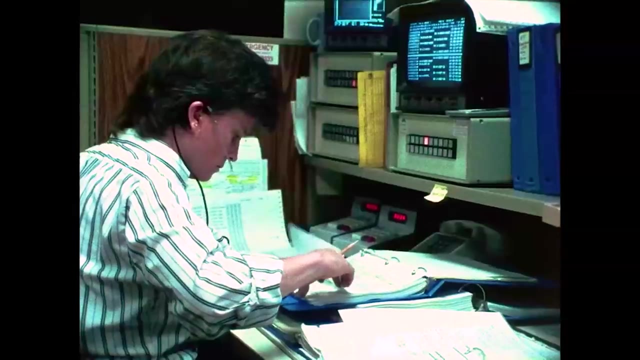 and the light intensity is one thousandth what it is here For photography, time exposures would be necessary. Yet Voyager 2 was travelling so fast that images would smear without special preparation. Engineers calculated just how much the craft would have to swivel. 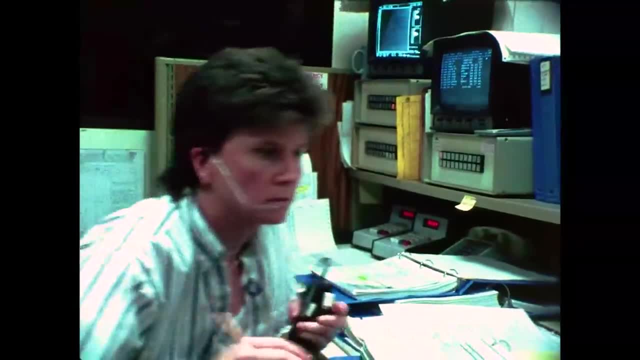 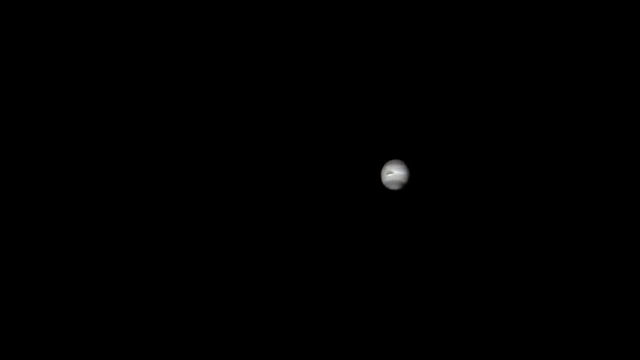 while exposures were made to compensate for the probe's movement. In June 1989, Voyager 2 began returning distant images of Neptune Across the world. people had realised that the data sent back to Earth by this spacecraft was transforming our understanding of the solar system. 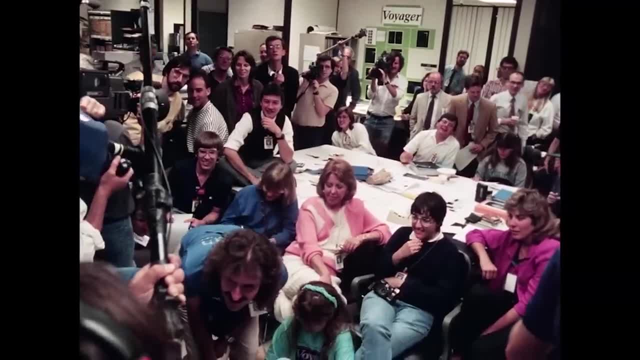 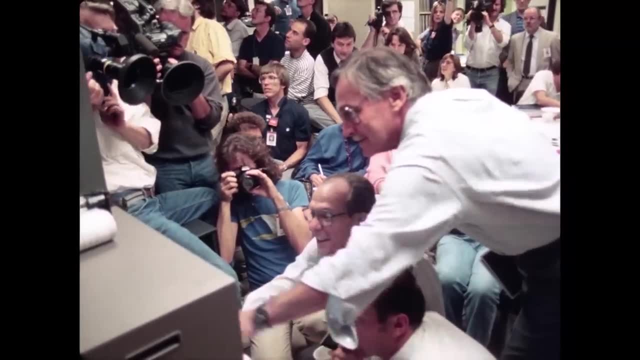 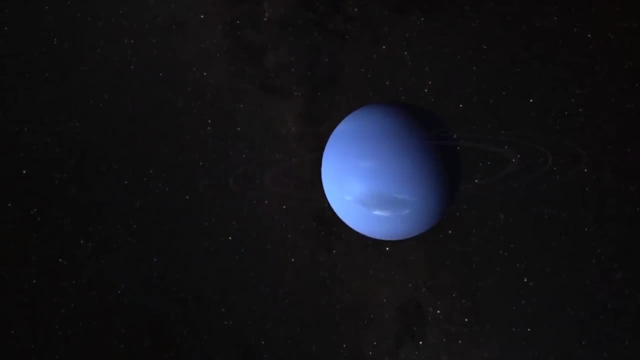 This was before the Internet age. Researchers at the Jet Propulsion Laboratory clustered around TV sets to watch as data and images came in line by line. Neptune is a more conventional planet. Its axial tilt is 30 degrees and it revolves in the same direction as Earth. 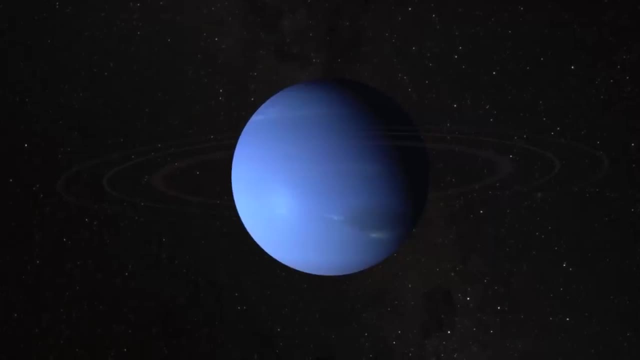 While Neptune is slightly heavier than its fellow ice giant Uranus, it has a slightly smaller diameter And though it is further from the sun than its neighbour, Neptune emits more heat than Uranus. The planet has an internal heat source that drives more dynamic weather patterns. 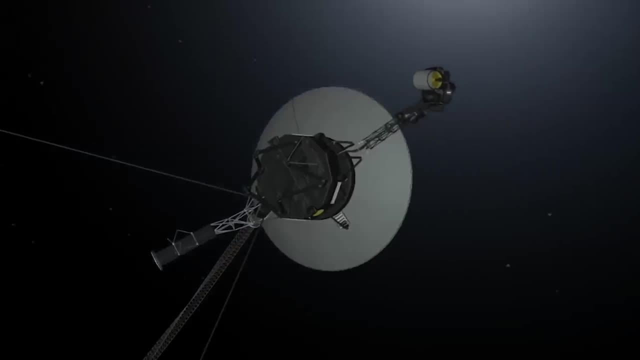 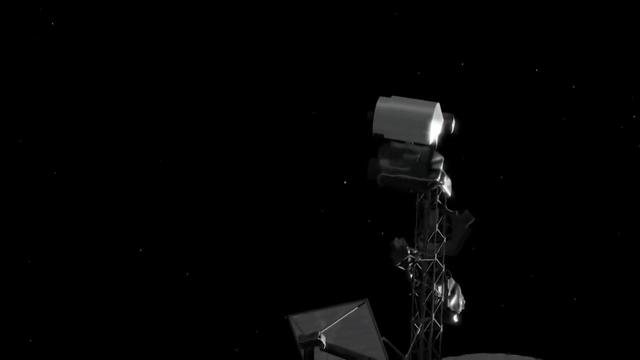 The Earth's solar system. Neptune is the only one with a solar system that is as fast as the Earth. Voyager 2 measured wind speeds at Neptune in excess of 2,000 kilometres per hour, the fastest in the solar system. There were cirrus clouds in the atmosphere. 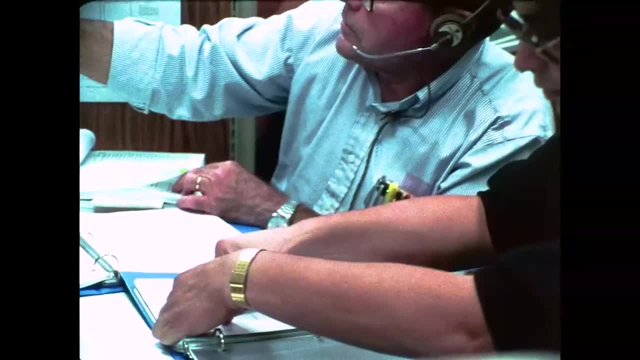 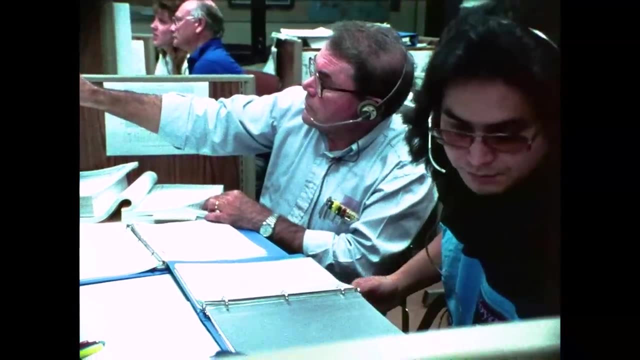 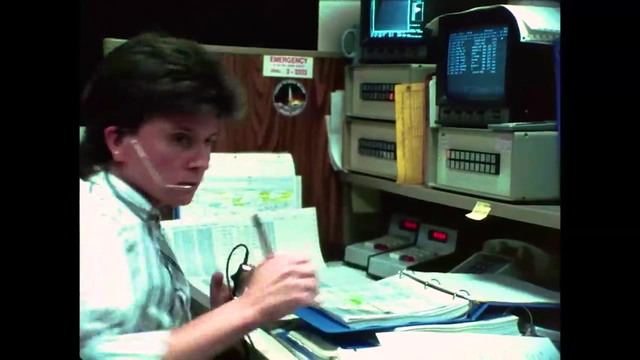 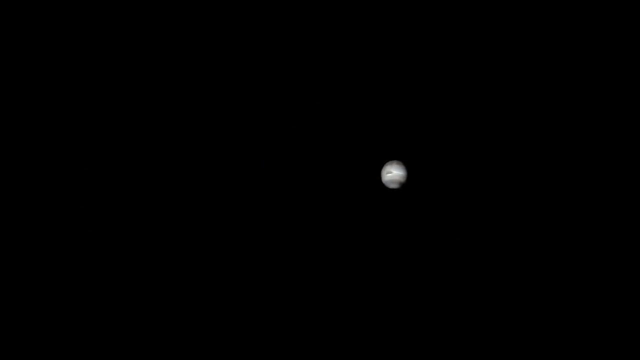 that images would smear without special preparation. Engineers calculated just how much the craft would have to swivel while exposures were made to compensate for the probe's movement. In June 1989, Voyager 2 began returning distant images of Neptune Across the world. people had realised. that the data sent back to Earth by this spacecraft was transforming our understanding of the solar system. The first time Voyager 2 was sent back to Earth was in the early 1980s. This was before the Internet age. Researchers at the Jet Propulsion Laboratory. 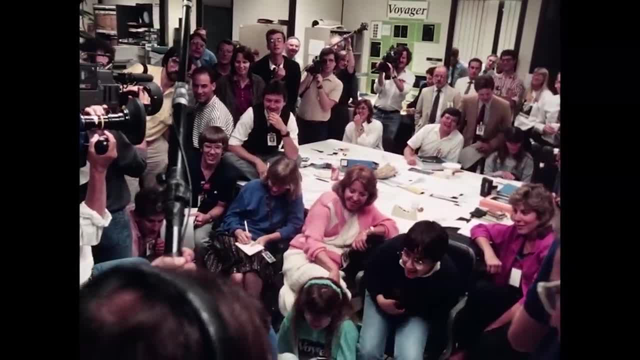 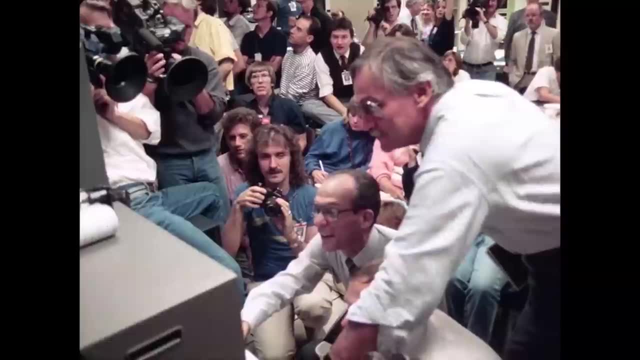 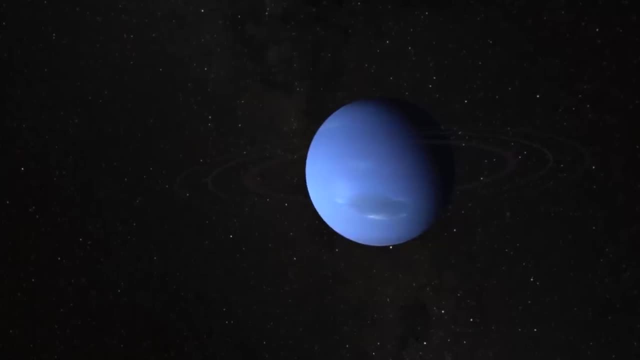 clustered around TV sets to watch as data and images came in line by line. Neptune is a more conventional planet than Uranus. Its axial tilt is 30 degrees and it revolves in the same direction as Earth, While Neptune is slightly heavier than its fellow ice giant Uranus. 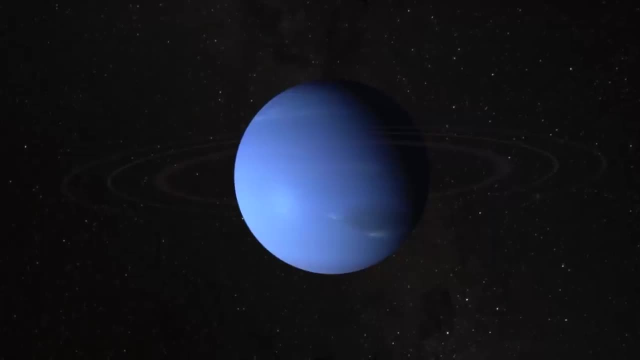 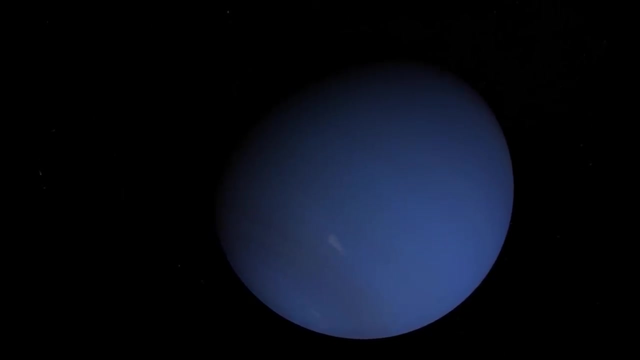 it has a slightly smaller diameter And though it is further from the Sun than its neighbour, Neptune emits more heat than Uranus. The planet has an internal heat source that drives more dynamic weather patterns. Voyager 2 measured wind speeds at Neptune in the early 1980s. It was the first time that Neptune emitted more heat than Uranus. It was the first time that Neptune emitted more heat than Uranus. It was in excess of 2,000 km per hour, the fastest in the solar system. There were cirrus clouds in the atmosphere. 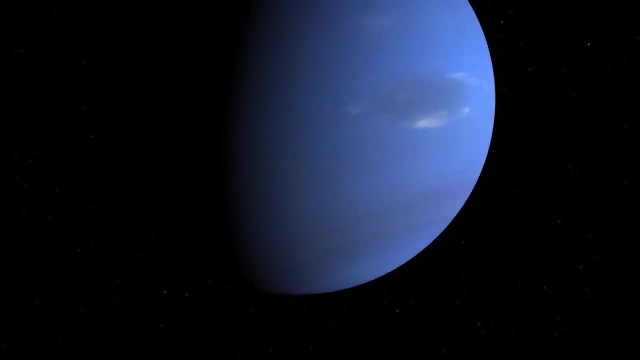 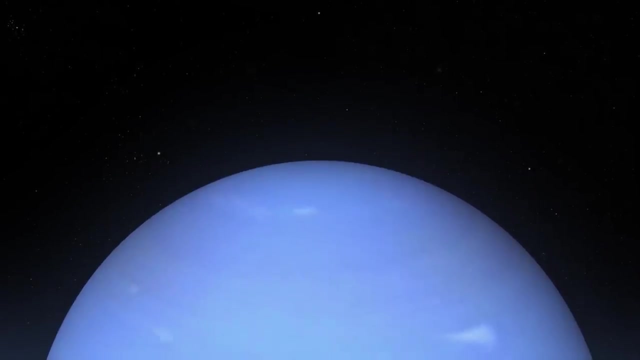 and the probe recorded pictures of a great dark spot, similar to Jupiter's Great Red Spot. It was an anticyclone in the southern hemisphere as large as the Earth. In 1994, when Hubble tried to find the same feature, it had disappeared. 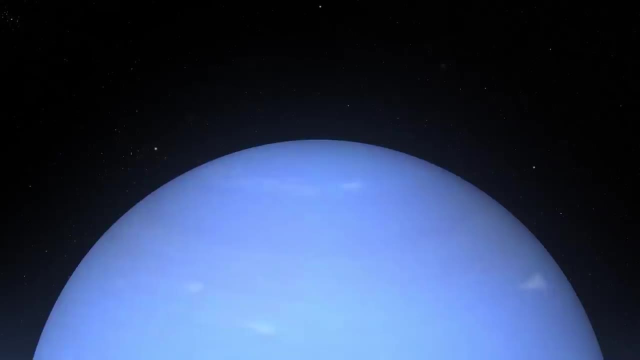 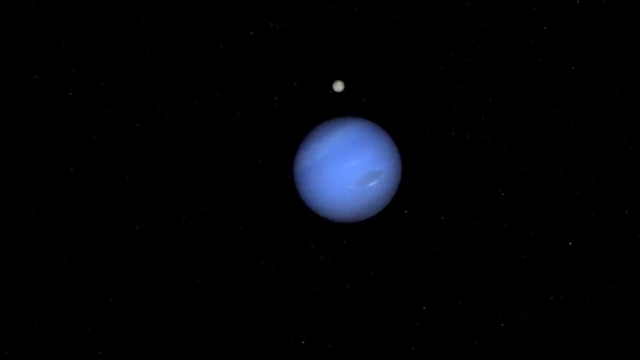 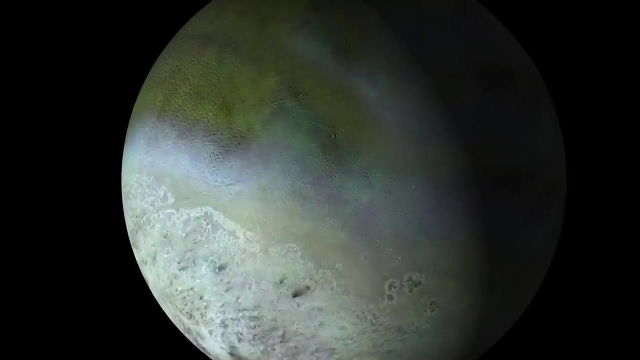 But a new dark spot was forming in the northern hemisphere. Voyager 2's last observations within the solar system were of Neptune's largest moon, Triton. Unlike all other moons in the solar system, Triton has a retrograde orbit, indicating that it was not formed. 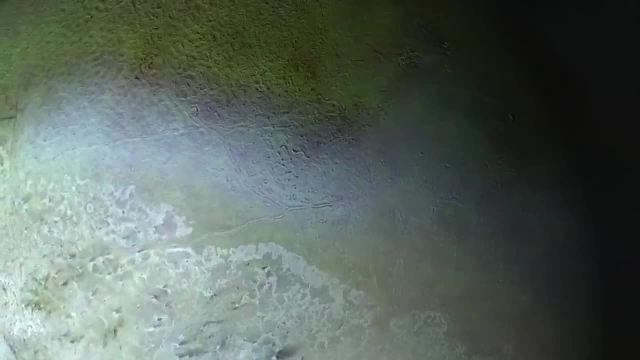 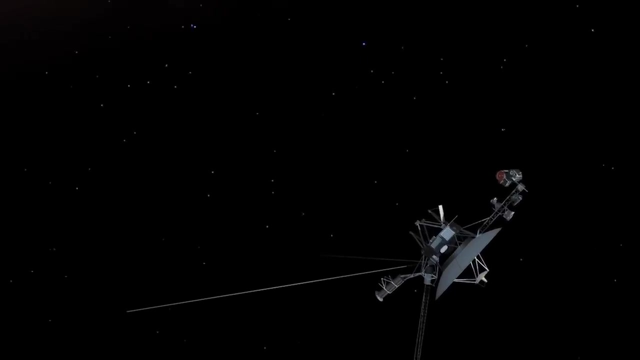 at the same time as the planet, but that it had been captured. The moon was not formed at the same time as the planet, but that it had been captured. As Voyager 2 moved beyond the planets, its cameras were switched off to save power. 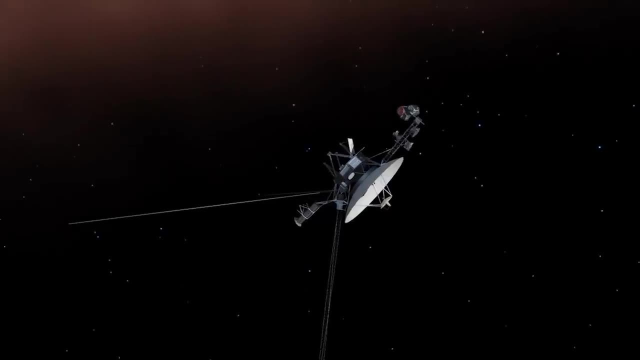 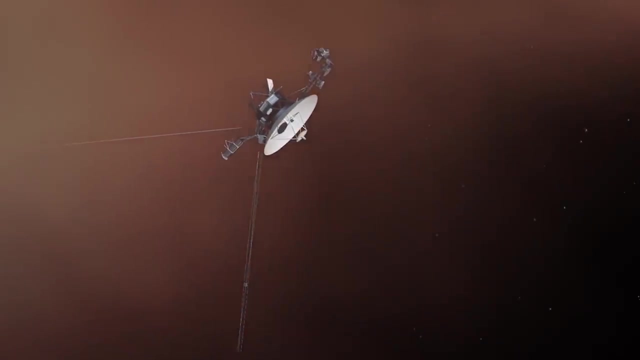 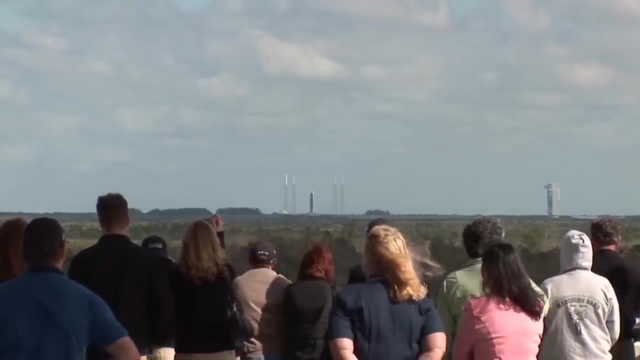 Both Voyagers continue away from the solar system, measuring the influence of the solar wind. This remains the only mission to the ice giants. On January 19th 2006, an Atlas V was launched. It was the second most powerful rocket in the solar system. 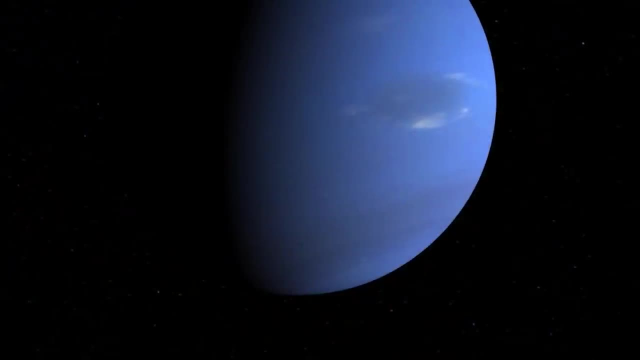 and the probe recorded pictures of a great dark spot, similar to Jupiter's Great Red Spot. It was an anticyclone in the southern hemisphere as large as the Earth. In 1994, when Hubble tried to find the same feature, it had disappeared. 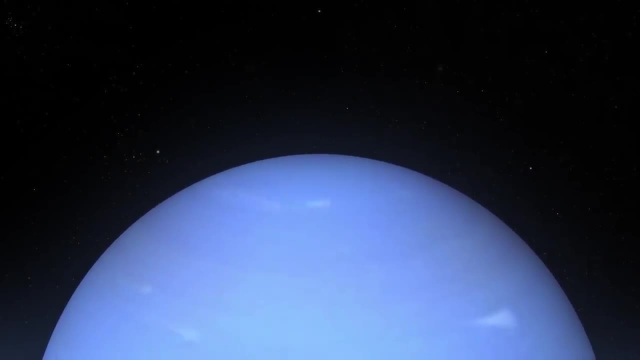 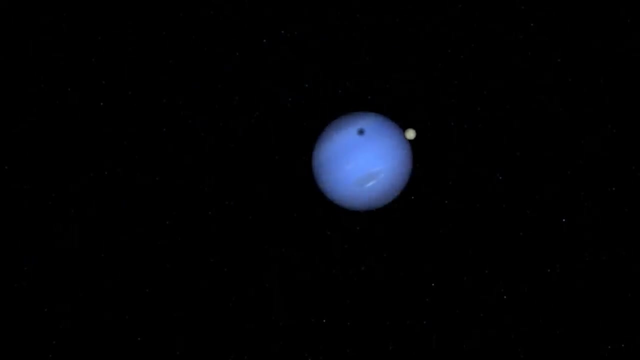 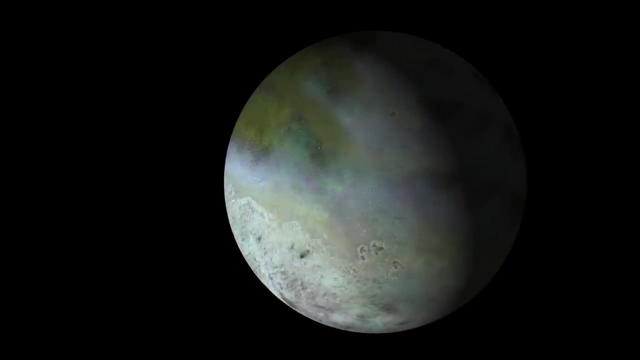 but a new dark spot was forming in the northern hemisphere. Voyager 2's last observations within the solar system were of Neptune's largest moon, Triton. Unlike all other moons in the solar system, Triton has a retrograde orbit, indicating that it was not formed at the same time as the planet. 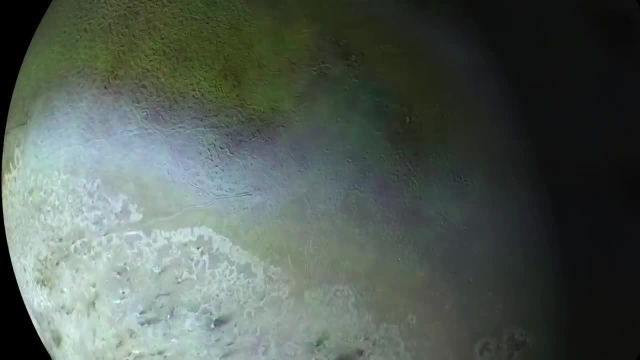 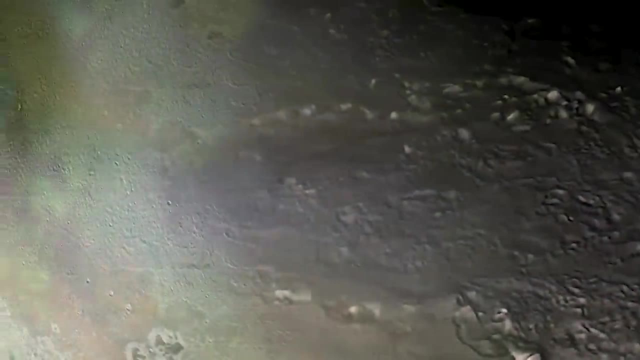 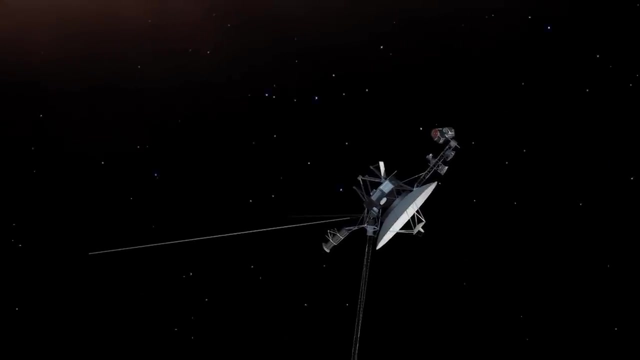 but was formed at the same time as the Earth. This means that not only did it move beyond the planet, but that it had been captured. As Voyager 2 moved beyond the planets, its cameras were switched off to save power. Both Voyagers continue away from the solar system. 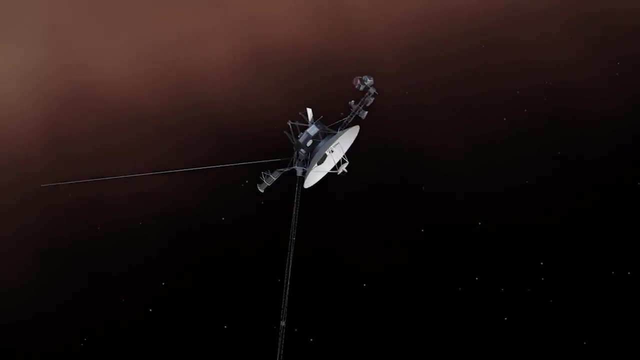 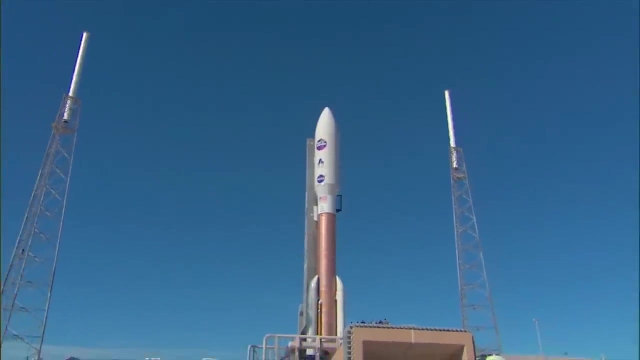 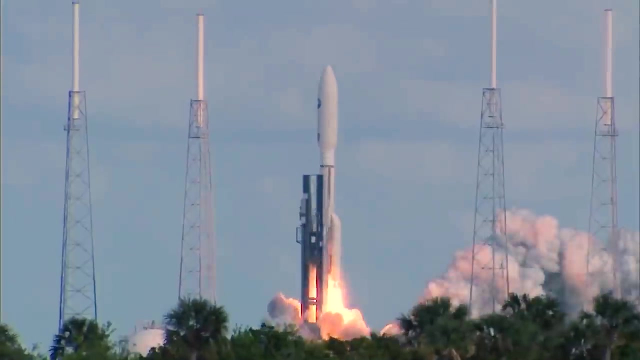 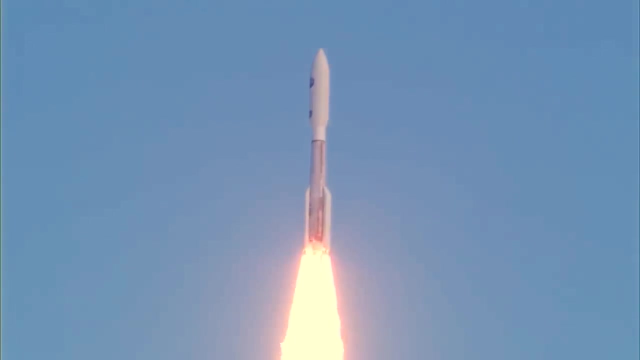 measuring the influence of the solar wind. This remains the only mission to the ice giants. On January 19th 2006, an Atlas V was launched. It was a very powerful rocket with an unusually small payload. New Horizons left Earth orbit faster than any other probe. 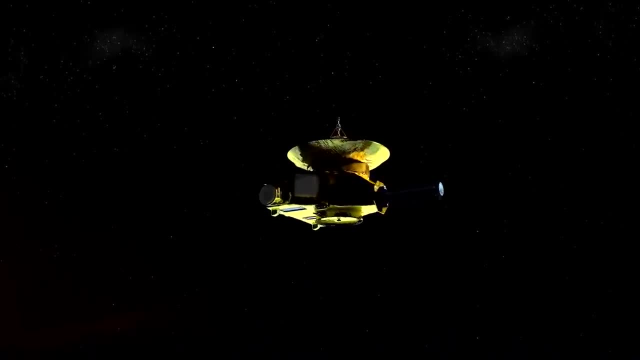 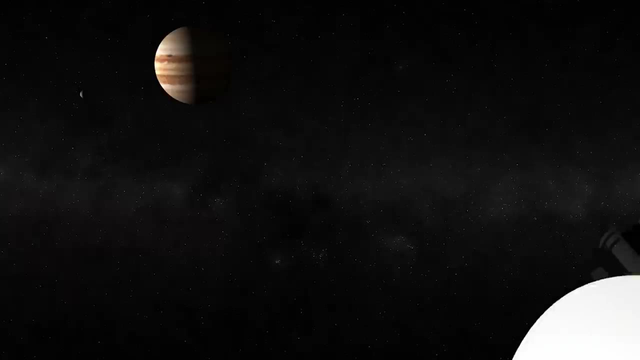 It was headed for the Kuiper belt at the outer edge of the solar system, in particular Pluto. In a little more than a year, New Horizons reached Jupiter, where it received a gravitational assist that cut three years from its flight time to Pluto. 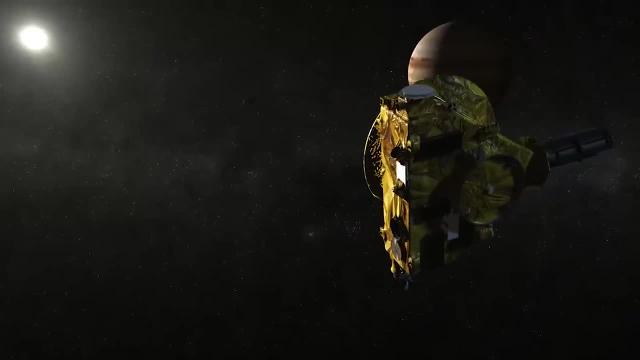 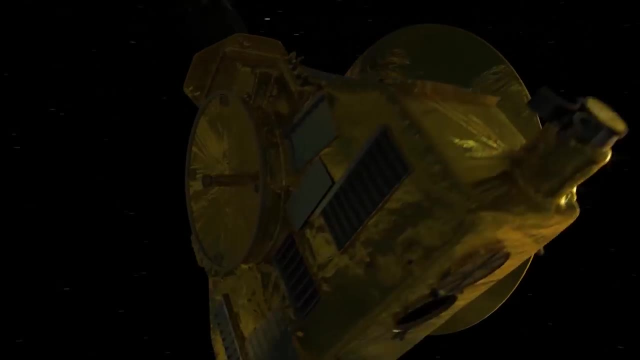 After it passed Jupiter, the spacecraft went into hibernation, simply sending an all's-well transmission once a week. It took New Horizons more than nine years to reach Jupiter. It was the first time in the history of space that New Horizons reached Jupiter. 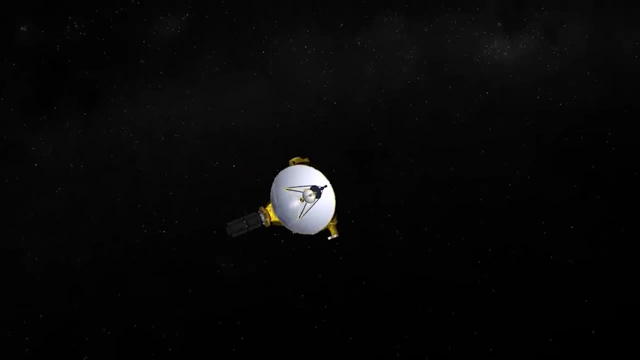 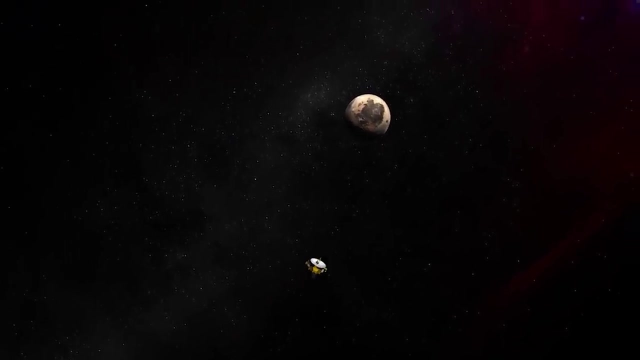 It took New Horizons more than nine years to reach Pluto. Since it had departed, Pluto had lost its status as a planet. With the discovery of more objects of similar size in the Kuiper belt, it was decided that to be a planet. 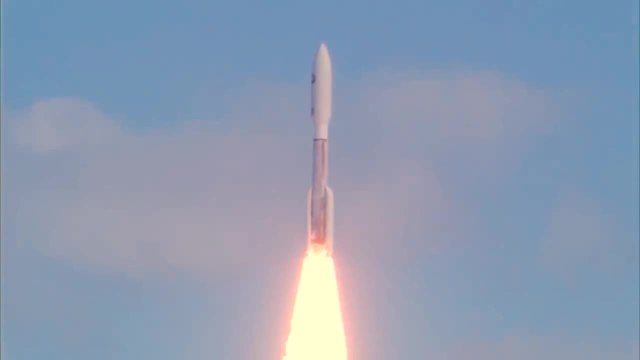 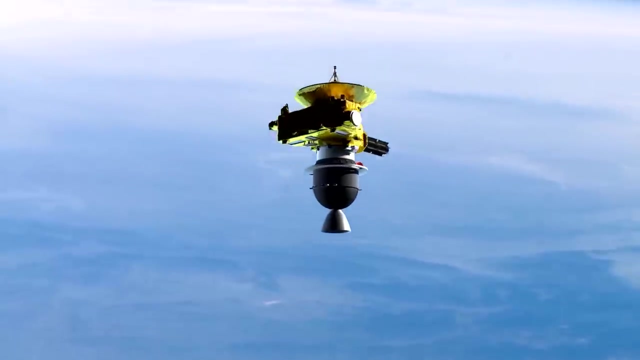 It was a very powerful rocket with an unusually small payload. It was a very powerful rocket with an unusually small payload. New Horizons left Earth orbit faster than any other probe. It was headed for the Kuiper belt, at the outer edge of the solar system. 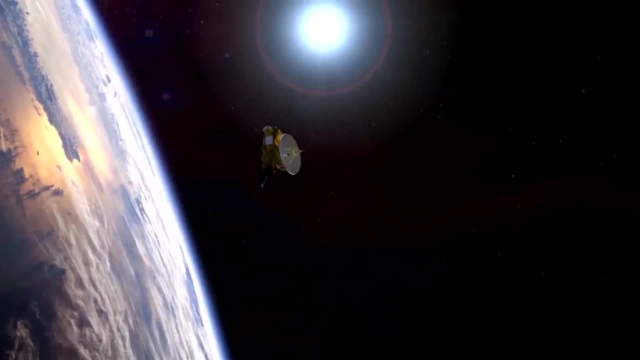 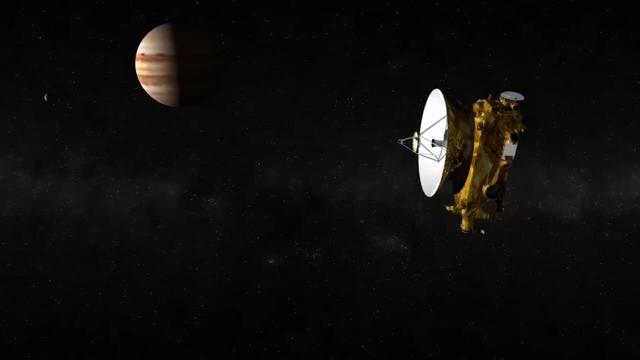 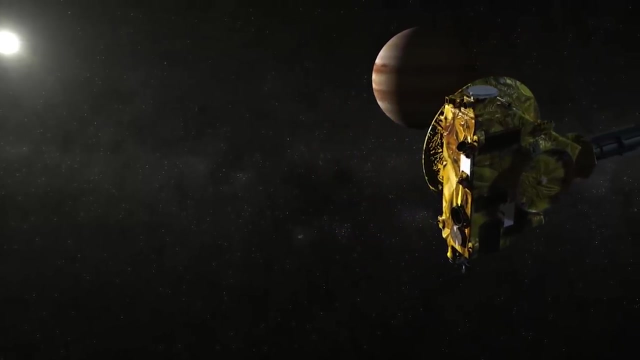 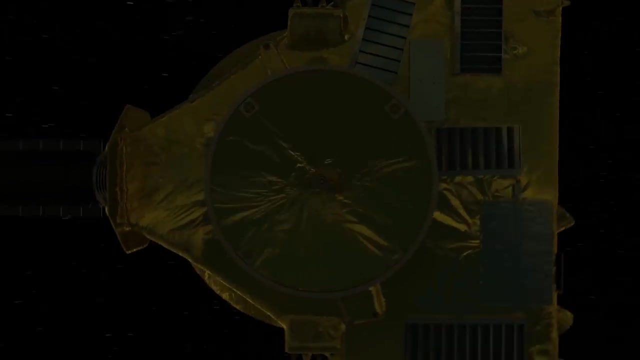 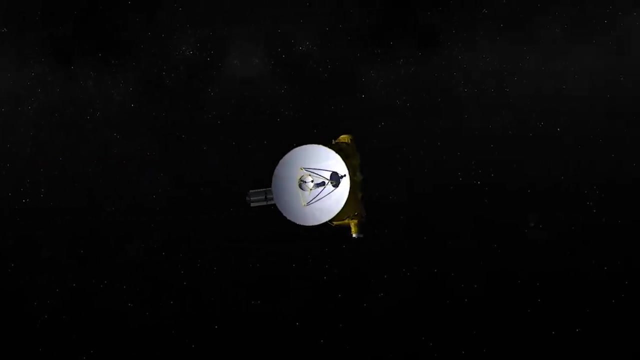 in particular Pluto, In a little more than a year reached Jupiter, where it received a gravitational assist that cut three years from its flight time to Pluto. after it passed Jupiter, the spacecraft went into hibernation, simply sending an all's-well transmission once a week. it took New Horizons more than nine years. 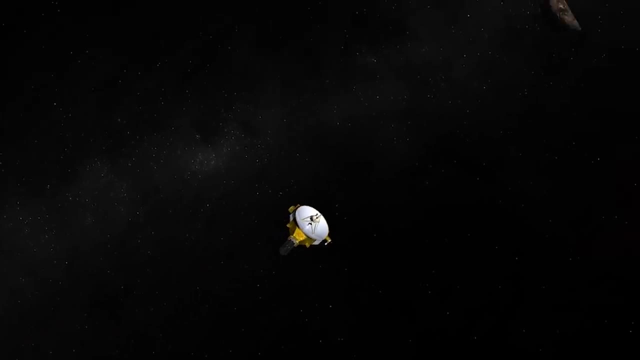 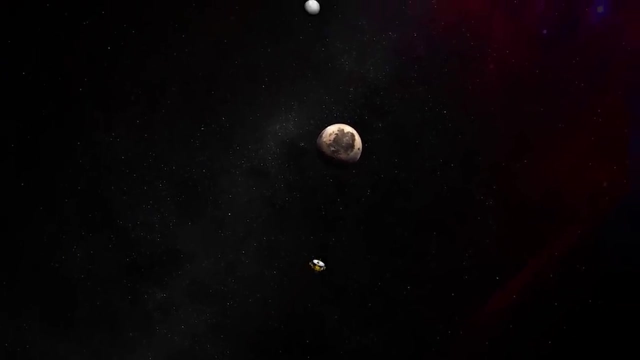 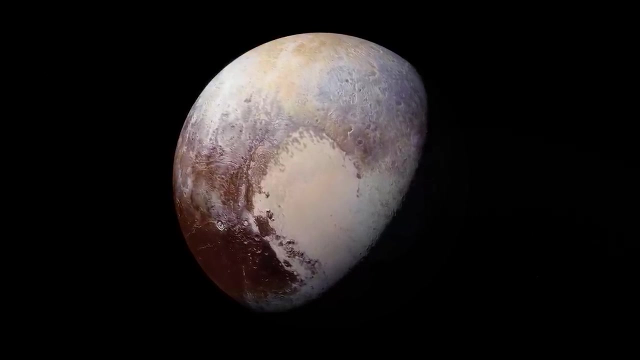 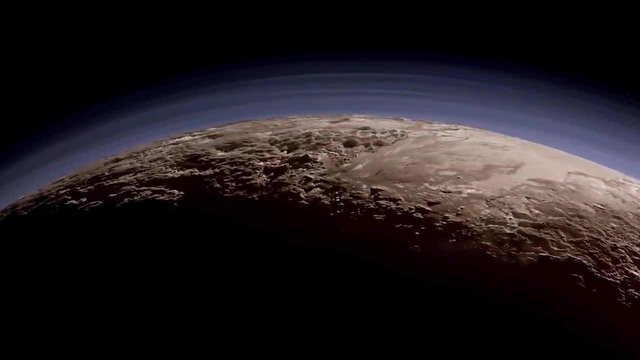 to reach Pluto. since it had departed. Pluto had lost its status as a planet with the discovery of more objects of similar size in the Kuiper belt. it was decided that to be a planet, a body had to clear its orbit. Pluto's features surprised everyone. here was a living planet shaped by tectonic. 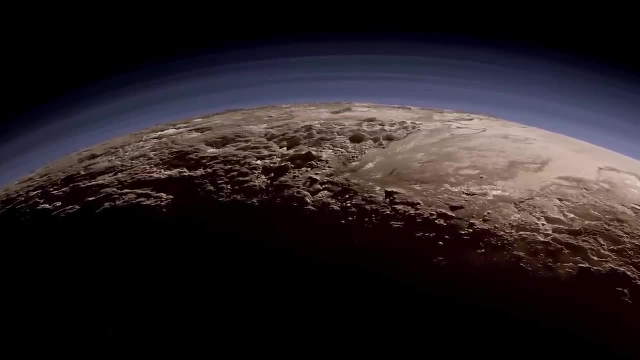 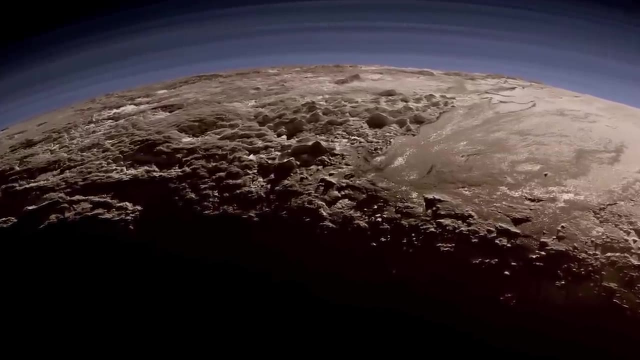 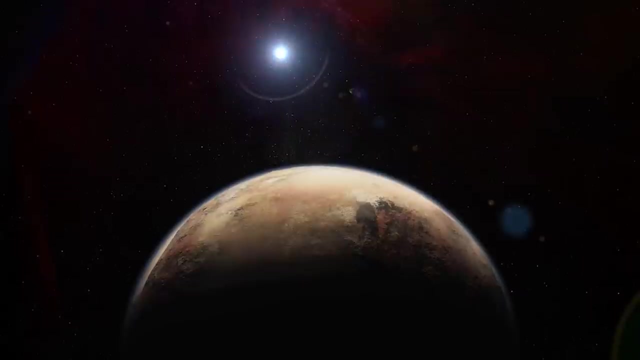 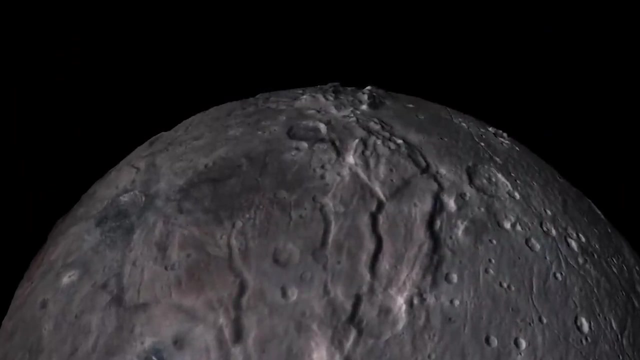 forces. but instead of rock, the mountains were made of ice and frozen methane, and Pluto has a thin atmosphere mainly of nitrogen. the probe continued on over Karen, Pluto's largest moon. its icy surface has deep canyons and some evidence suggests that it has ice volcanoes. Karen is about. 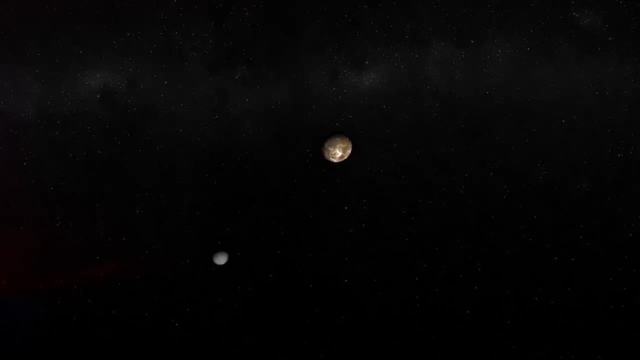 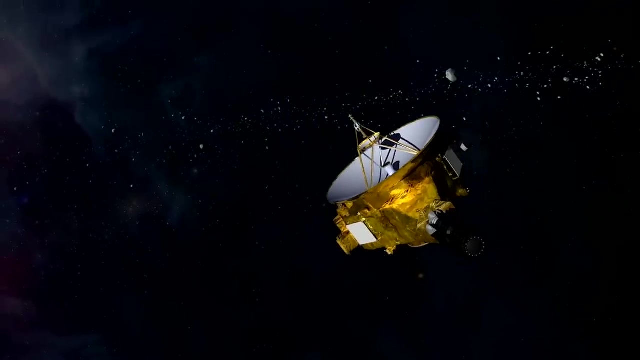 half the size of Pluto and the two orbit each other from Pluto. car would appear motionless in the sky as the New Horizons probe sped away from Pluto's probe, sped away from Pluto's probe, sped away from Pluto's probe, sped away from Pluto into deep space, it began the slow process of transmitting it's recorded. 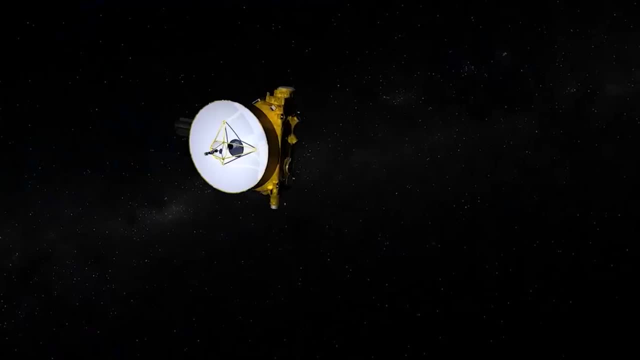 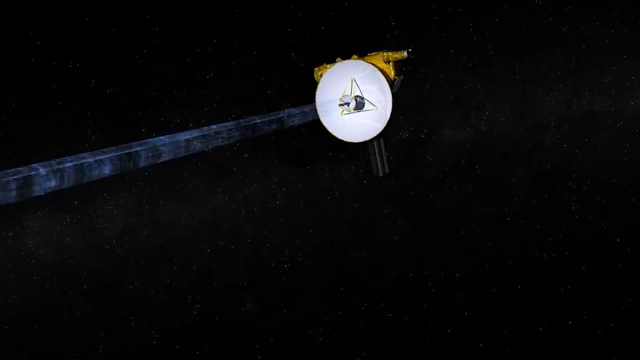 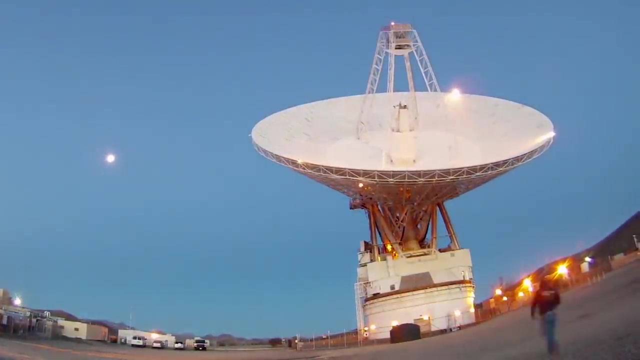 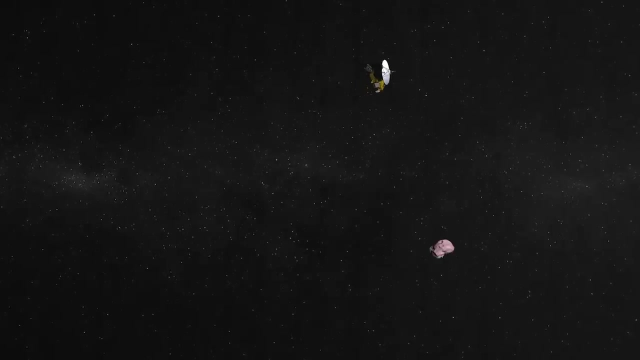 back to the earth at these distances. it take signals four-and-a-half hours to reach Earth, with data coming in at one kilobit per second. it took four hundred sixty nine days for all the fallumph of information to be received back on us early in 2019. 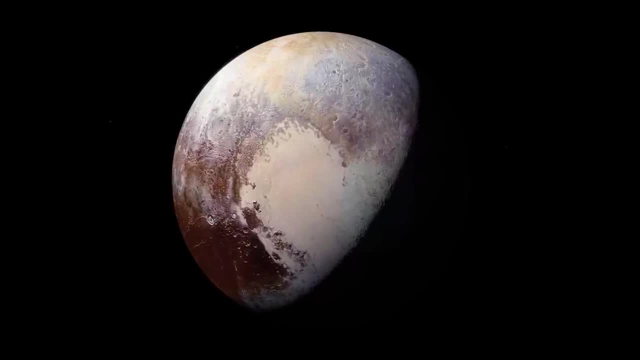 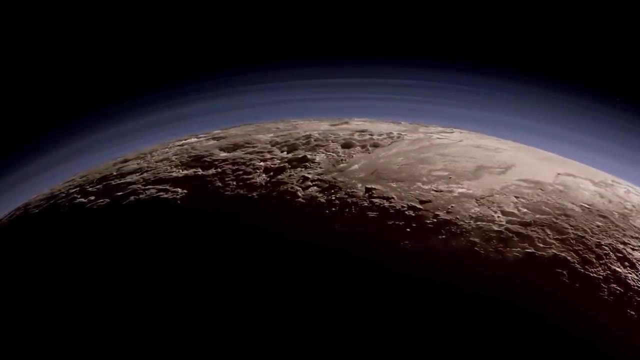 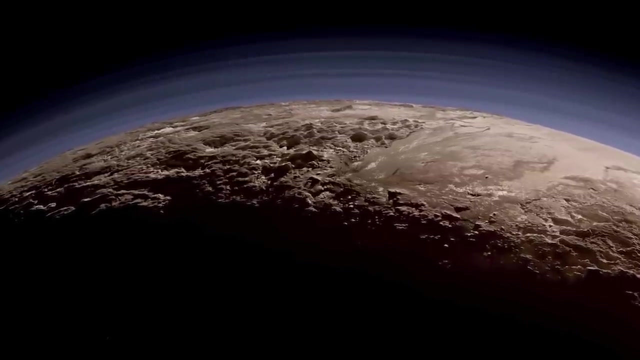 a body had to clear its orbit. Pluto's features surprised everyone. Here was a living planet shaped by tectonic forces, but instead of rock, the mountains were made of ice and frozen methane, And Pluto has a thin atmosphere mainly of nitrogen. 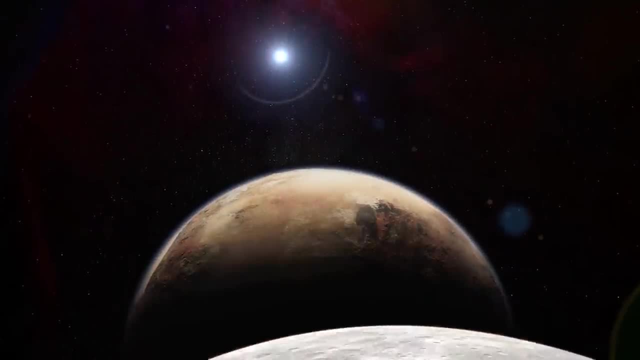 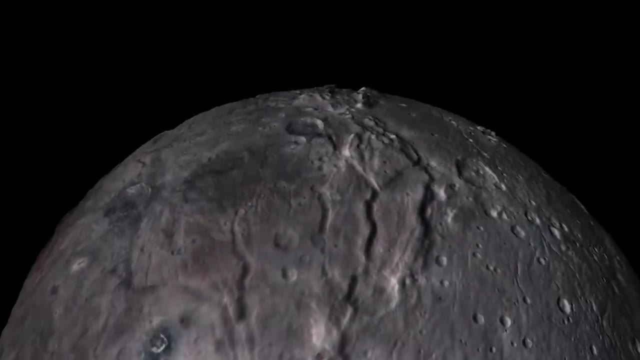 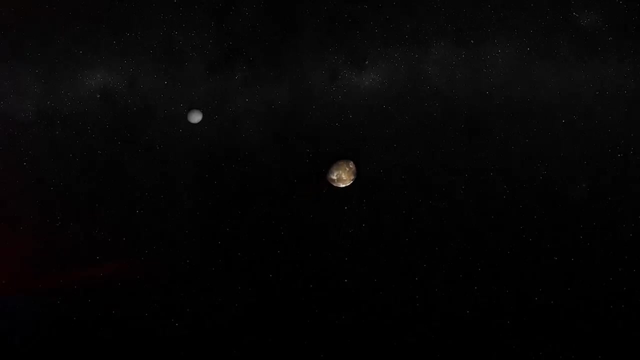 The probe continued on over Charon, Pluto's largest moon. Its icy surface has deep canyons and some evidence suggests that it has ice volcanoes. Charon is about half the size of Pluto and the two orbit each other From Pluto. 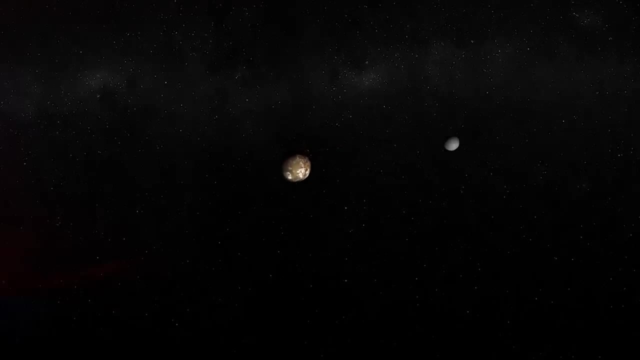 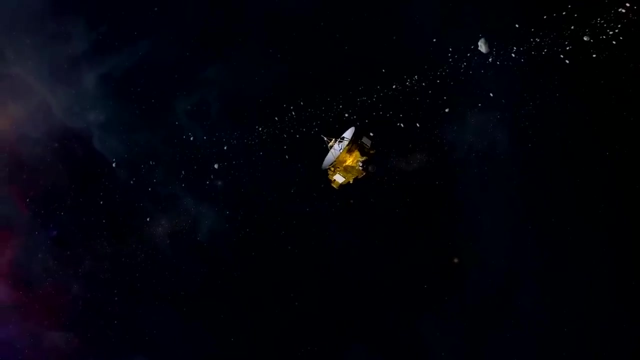 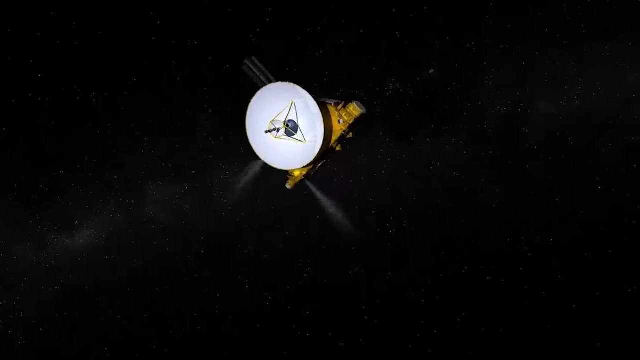 Charon would appear motionless in the sky. As the New Horizons probe sped away from Pluto into deep space, it began the slow process of transmitting its recorded data back to the Earth. At these distances it takes signals four and a half hours. 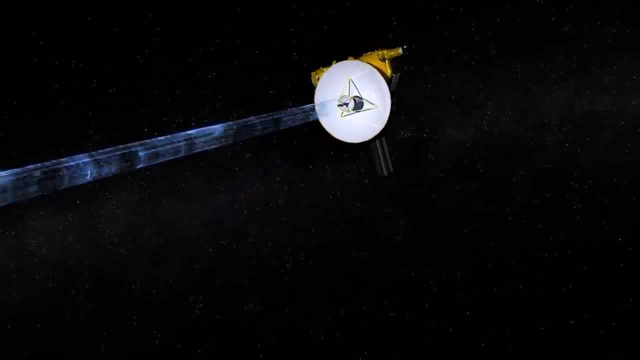 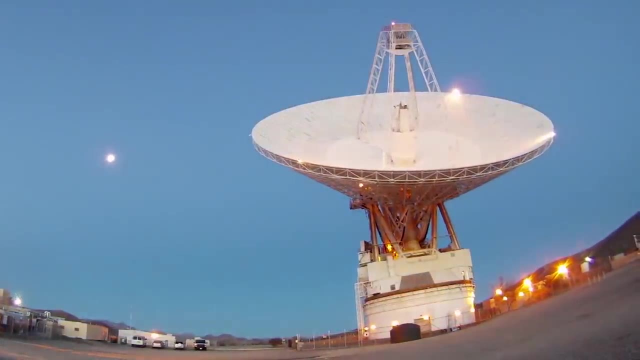 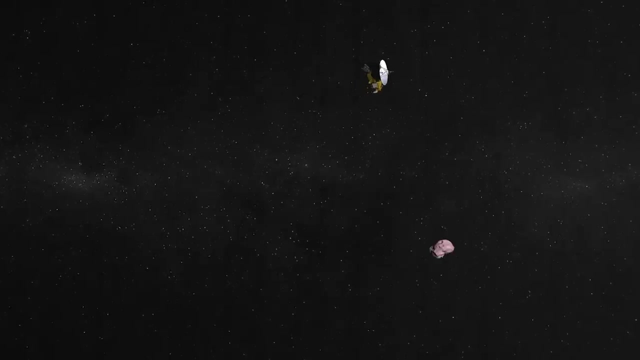 to reach Earth. with data coming in at one kilobit per second, It took 469 days for all the Pluto information to be received back on Earth. Early in 2019, New Horizons passed trans-Neptunian object Altima Thule. 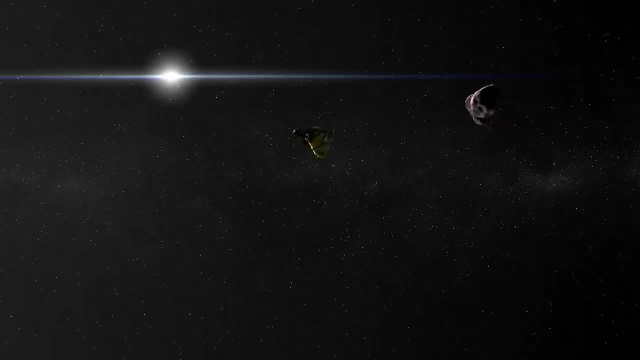 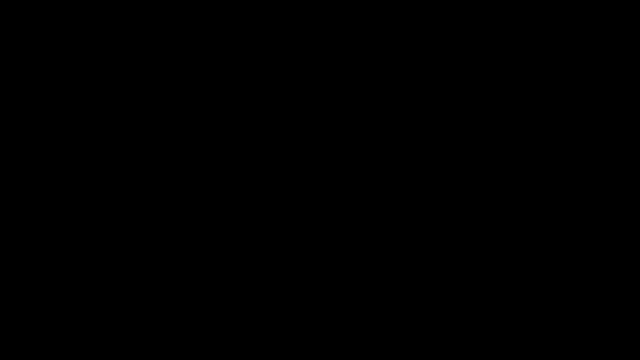 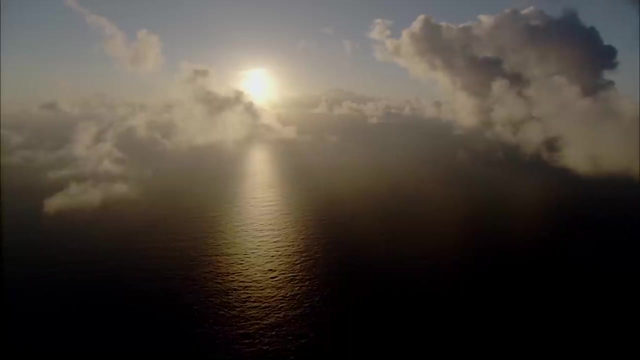 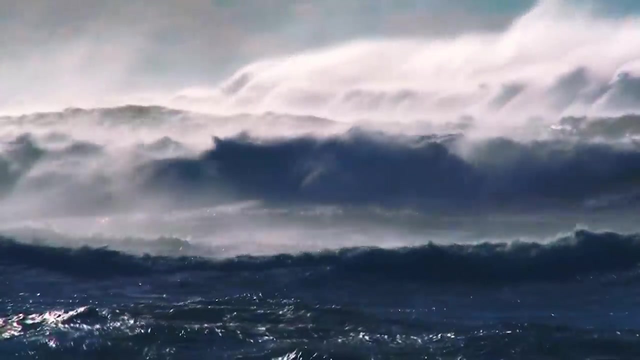 And with a mission extension, it continues exploring the outer reaches of the solar system. The Earth is our home. Our natural environment results from complex relations between the sun, the oceans and the atmosphere. The polar ice and the tropical heat represent the extremes. 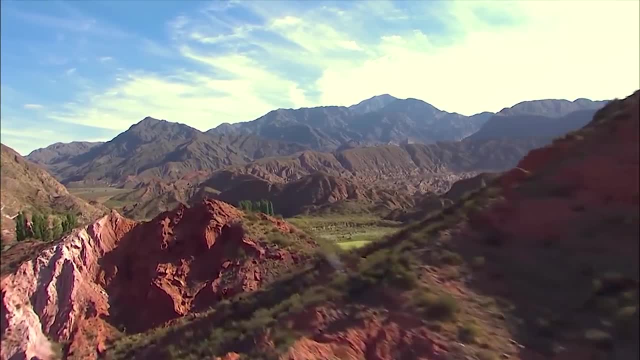 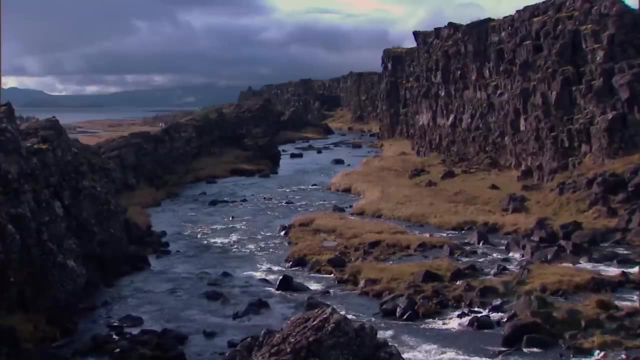 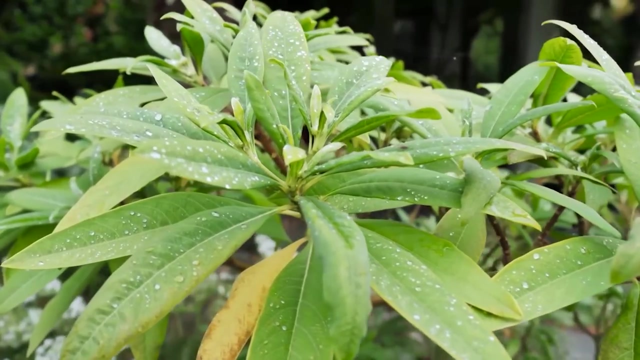 of our planet's climate. In reality, this is a very narrow temperature band, completely different from any other planet we've observed. The stability of the Earth's environment has allowed life to emerge, and life has changed the planet As far as we know. 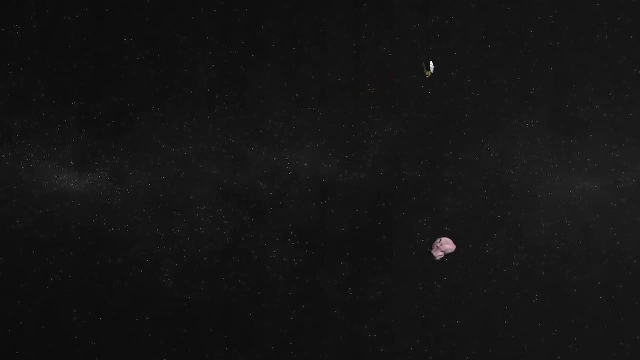 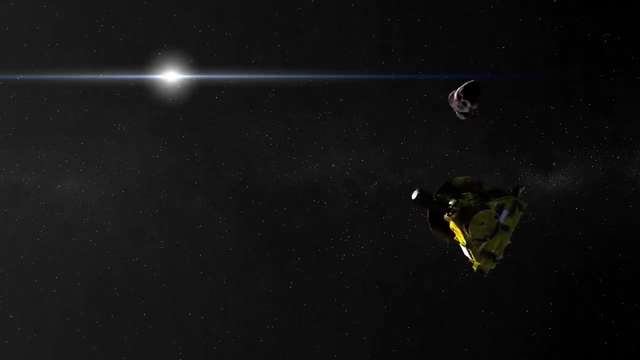 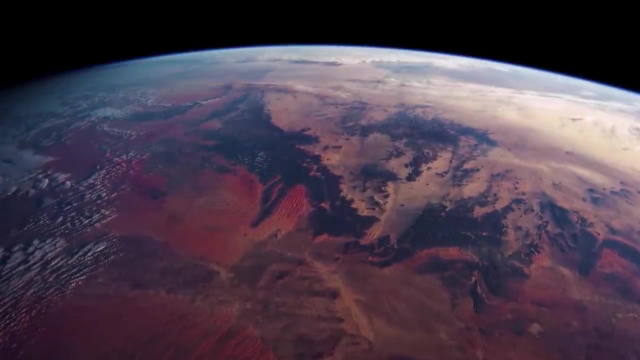 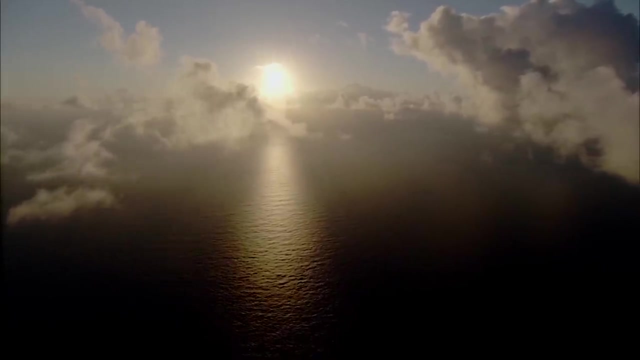 New Horizons passed trans-Neptunian object Ultima Thule And, with a mission extension, it continues exploring the outer reaches of the solar system. The Earth is our home. Our natural environment results from complex relations between the sun, the oceans and the atmosphere. 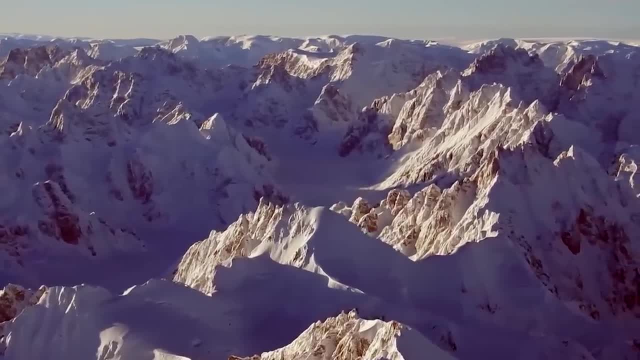 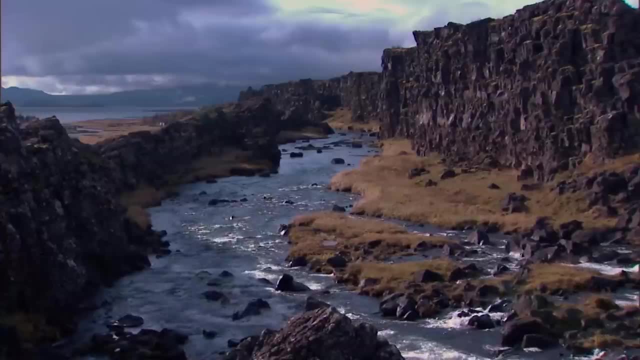 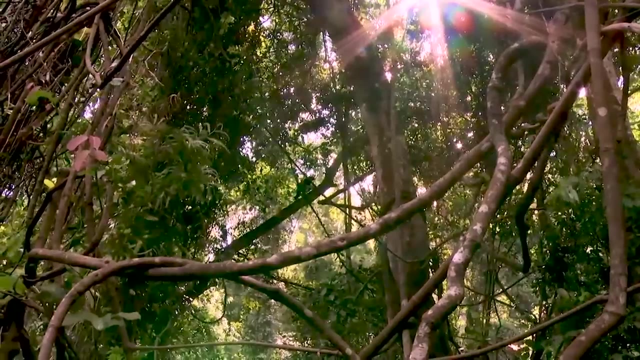 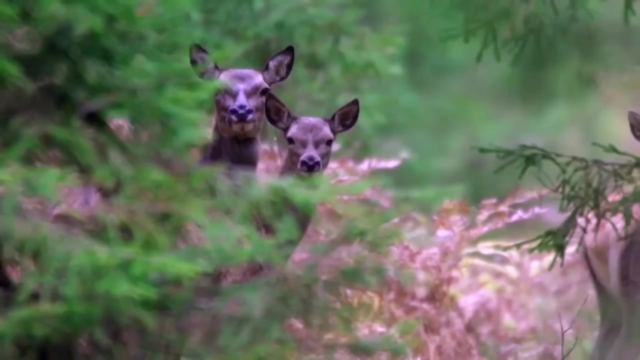 The polar ice and the tropical heat represent the extremes of our planet's climate. In reality, this is a very narrow temperature band, completely different from any other planet we've observed. The stability of the Earth's environment has allowed life to emerge, and life has changed the planet. 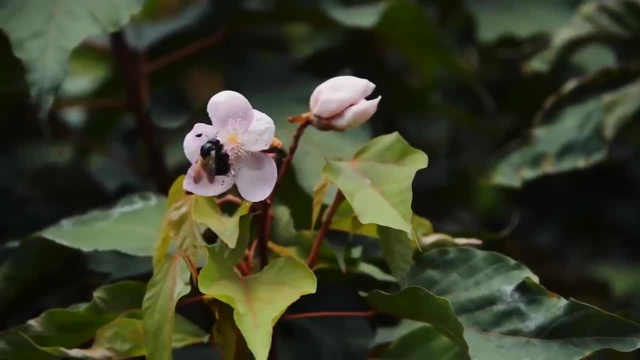 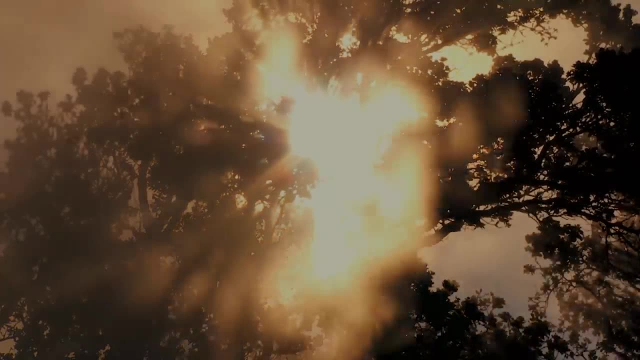 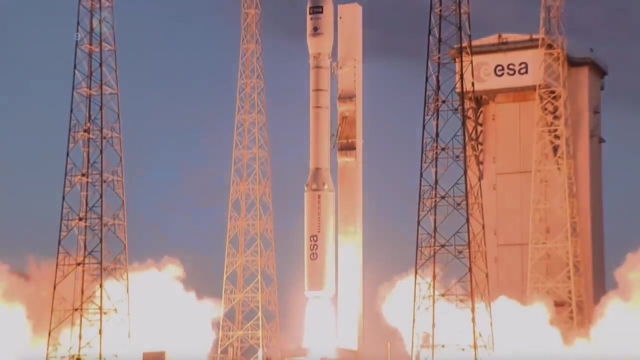 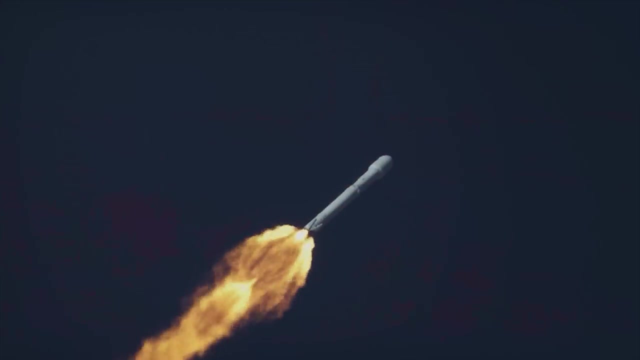 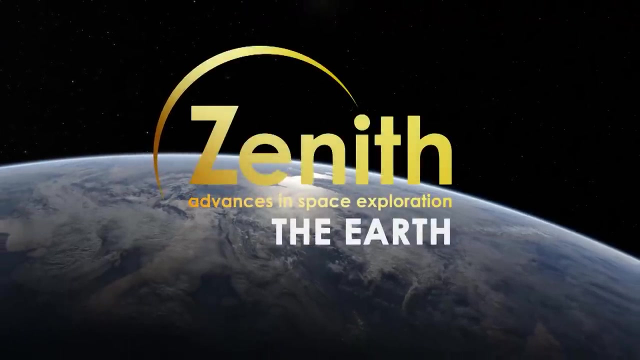 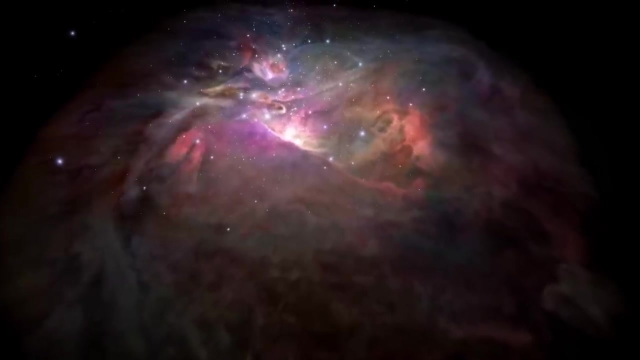 As far as we know, the Earth's climate has changed. The Earth is the only planet in the universe to have given rise to life. The Orion Nebula is a vast cloud of gas and dust in the Orion constellation. It's a place where new stars are being created. 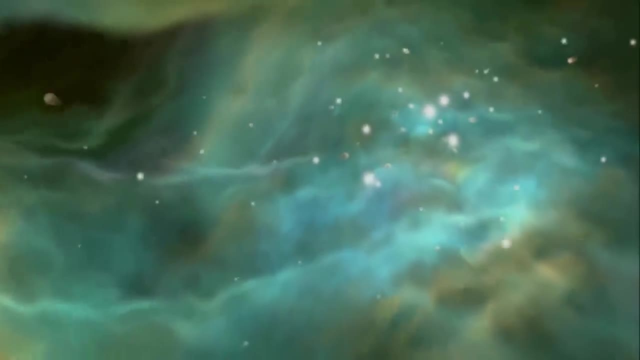 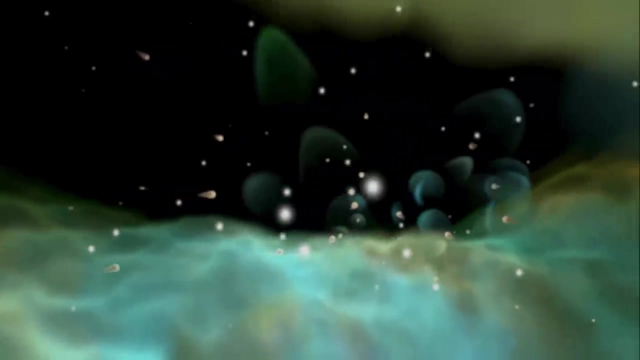 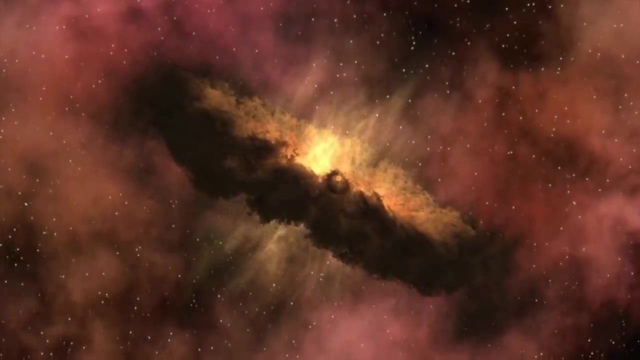 As part of the nebula, condenses, it separates into clumps. As each clump contracts under its own gravitation, it begins to swirl, flattening into a disk. They're called protoplanetary disks or propylids. In the center of a propylid, as the molecules are squeezed together, 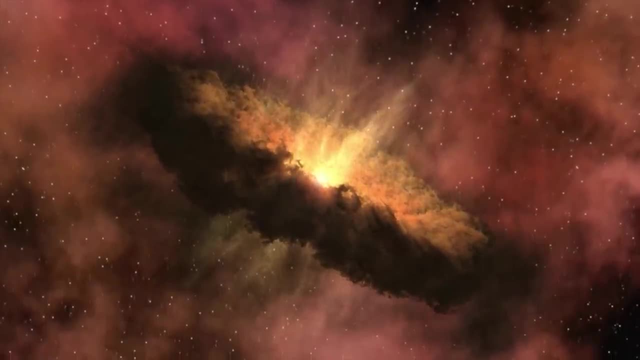 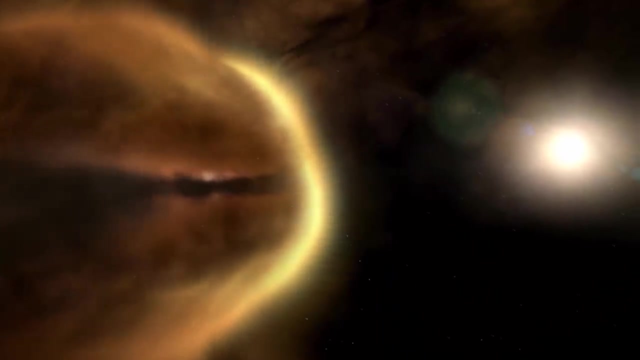 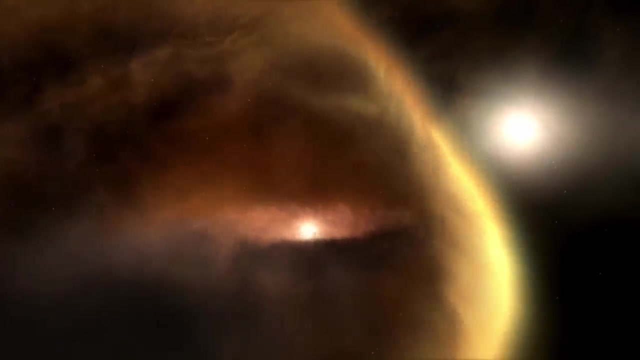 a fusion reaction begins and a star ignites. Some propylids occurring close to an established star shine brightly under the influence of their neighbor. While this makes them easier to observe, the glowing gas and dust is being stripped away by the stellar winds from the adjacent star. 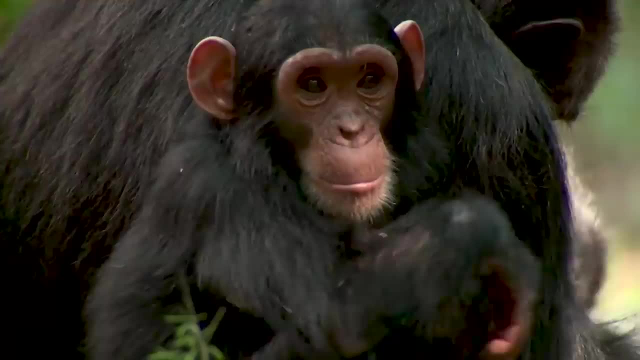 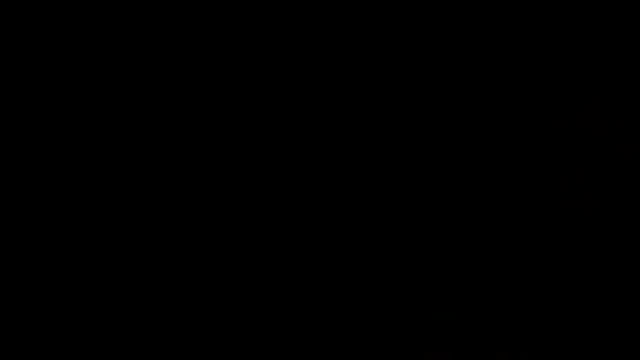 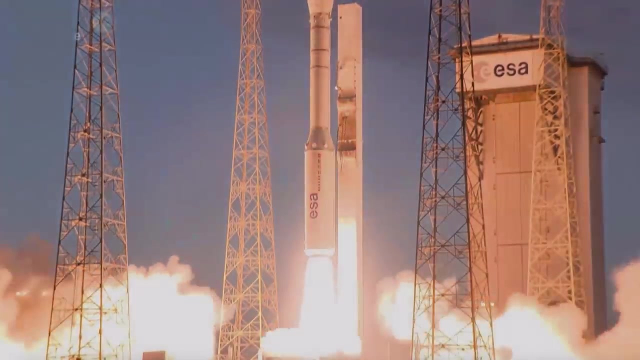 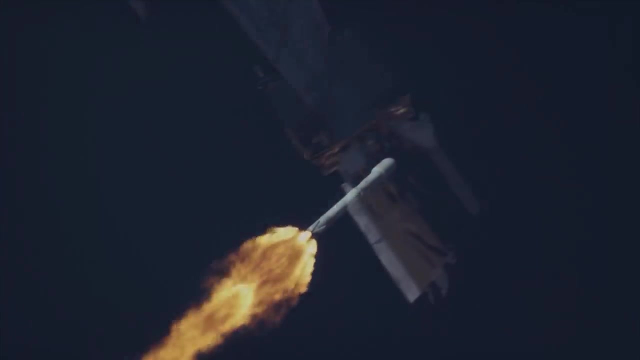 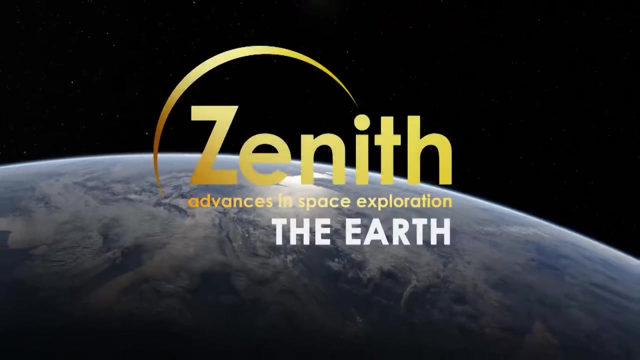 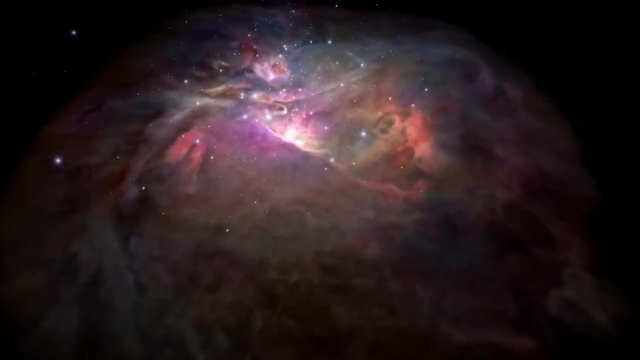 the Earth is the only planet in the universe to have given rise to life. The Orion Nebula is a vast cloud of gas and dust. in the Orion constellation, It's a place where new stars are being created. The Orion Nebula is a vast cloud. 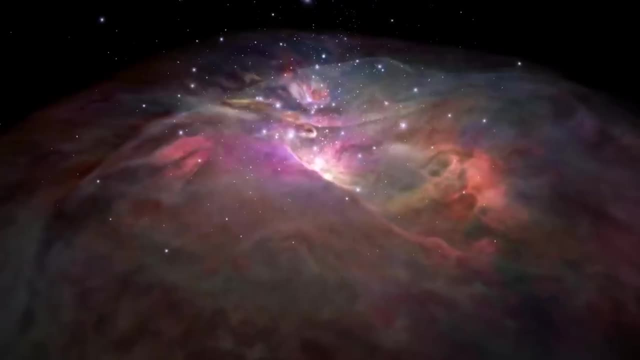 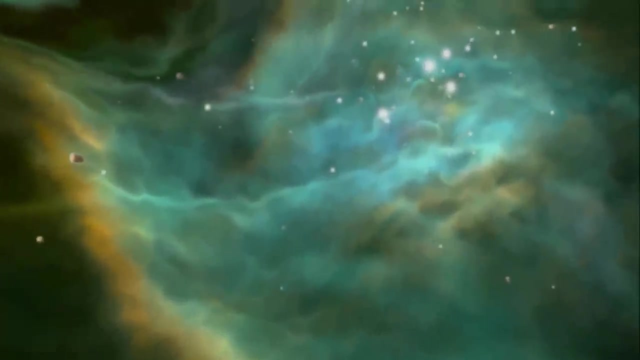 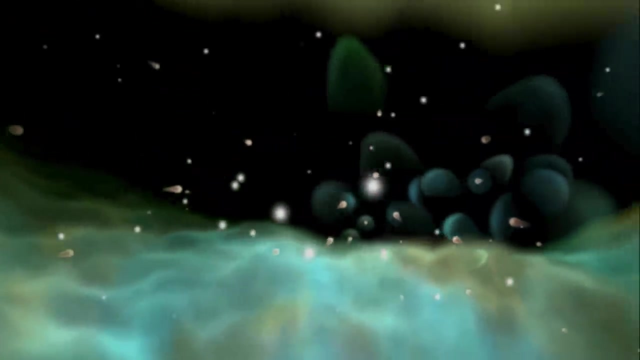 of gas and dust in the Orion constellation. It's a place where new stars are being created. As part of the nebula condenses, it separates into clumps. As each clump contracts under its own gravitation, it begins to swirl. 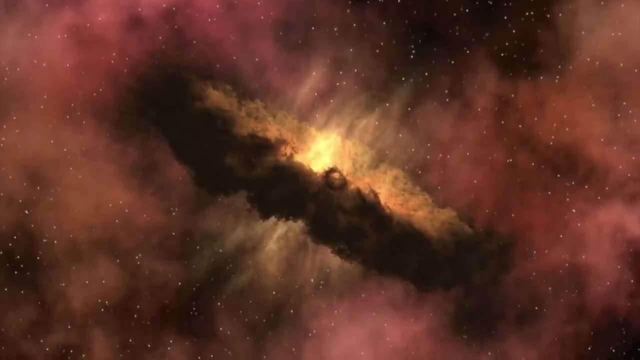 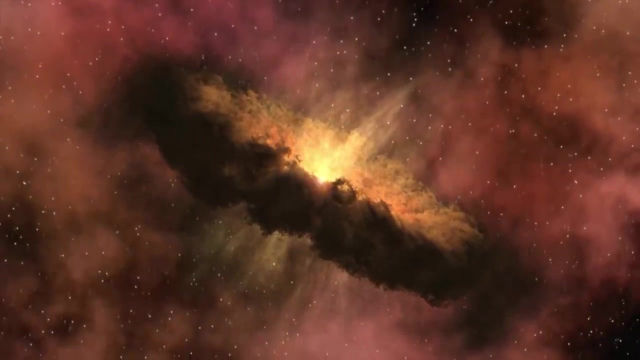 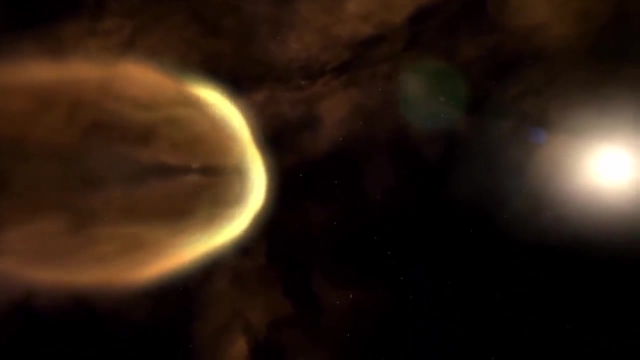 flattening into a disk. They're called protoplanetary disks or proplyds. In the center of a proplyd, as the molecules are squeezed together, a fusion reaction begins and a star ignites. The particles close to an established star. 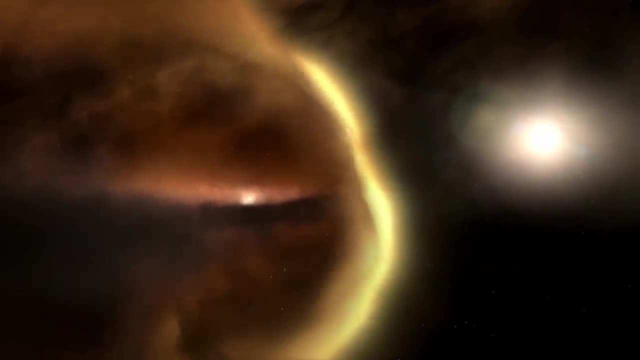 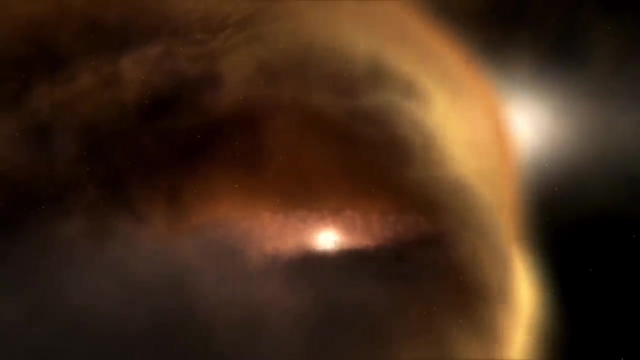 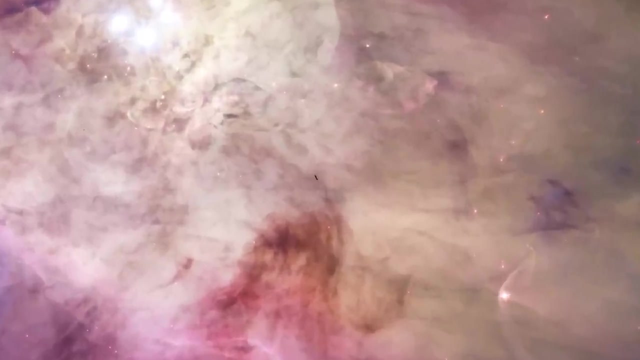 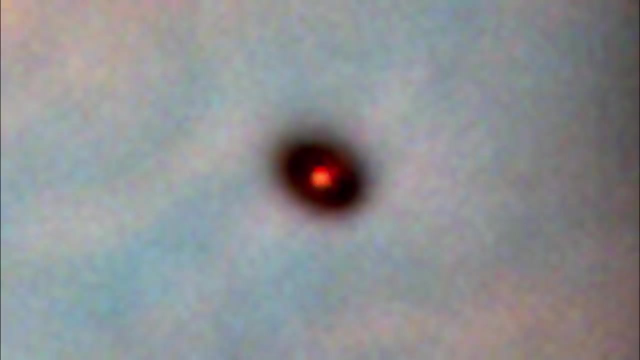 shine brightly under the influence of their neighbor. While this makes them easier to observe, the glowing gas and dust is being stripped away by the stellar winds from the adjacent star. Dark proplyds only observable as silhouettes maintain their surrounding ring of gas and dust. 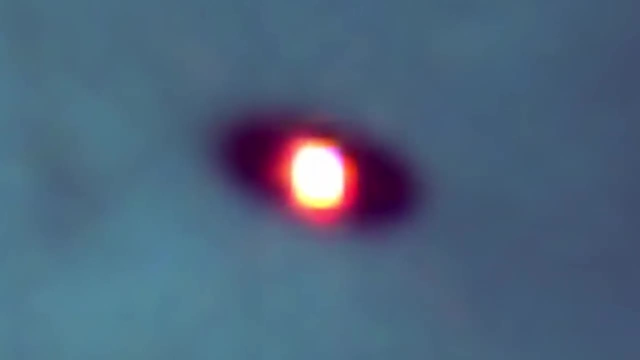 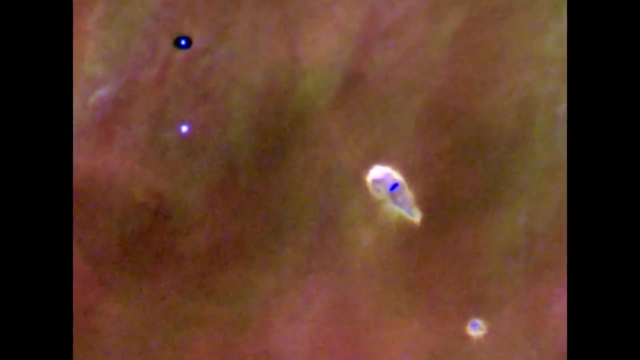 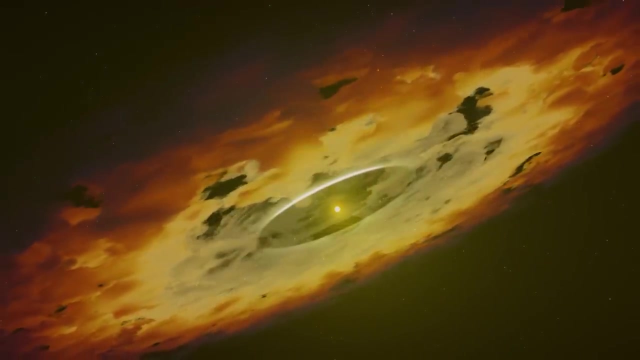 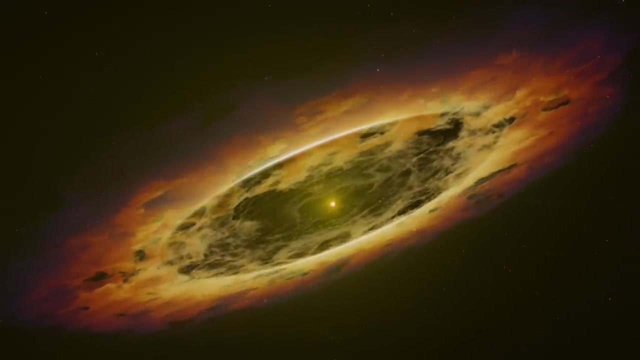 The Hubble Space Telescope has recorded numerous examples of this process, enough for astronomers to understand that the formation of planets is commonplace. This is how our own Sun started its life 4.6 billion years ago, But the planets would take longer to emerge. 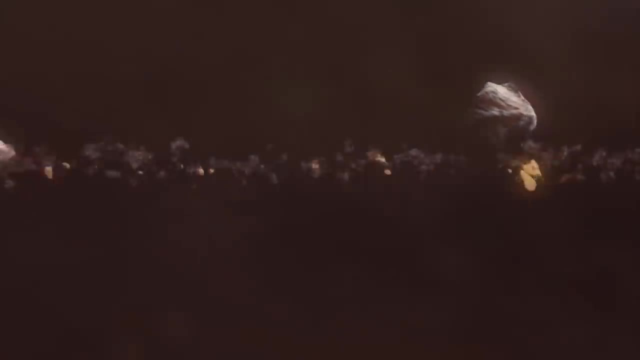 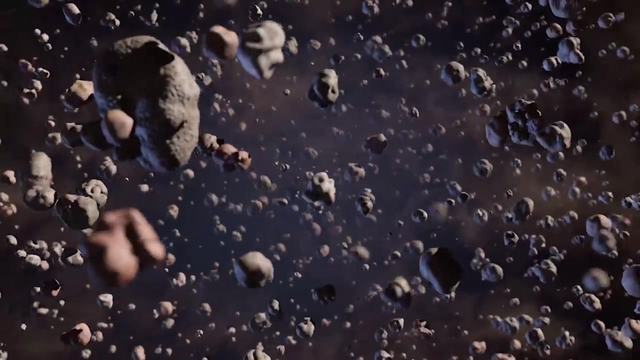 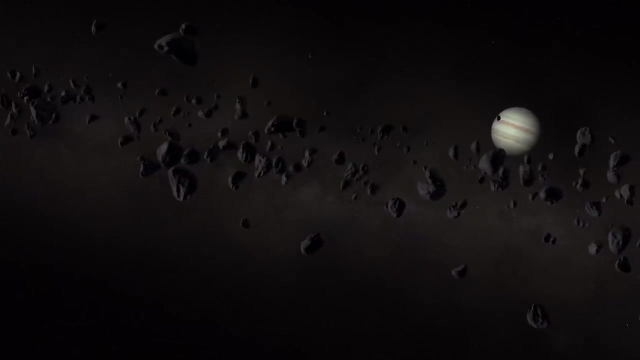 All grains within the disk began accreting, forming planetesimals. The larger a clump became, the stronger its gravitational attraction, in turn leading to more rapid growth. An early version of Jupiter would have been the first to coalesce, completely clearing its orbit. Around a core of heavy metal and rock, and mainly of hydrogen, was compressed by its strong gravitation. Any solid surface lay beneath thousands of kilometers of liquid gas. Our observations of exoplanets have revealed Jupiter-sized gas giants orbiting close to their stars. Astronomers believe the young Jupiter would have begun a track toward the Sun, dragging asteroids and comets in with it. But Jupiter's inward path reversed as it was pushed into an orbital resonance with the emerging Saturn. Not all of the objects forming in the early solar system. 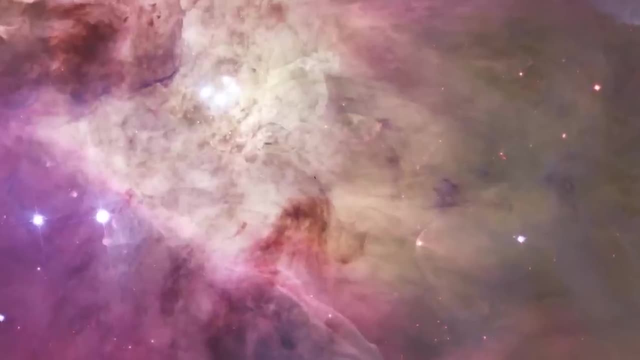 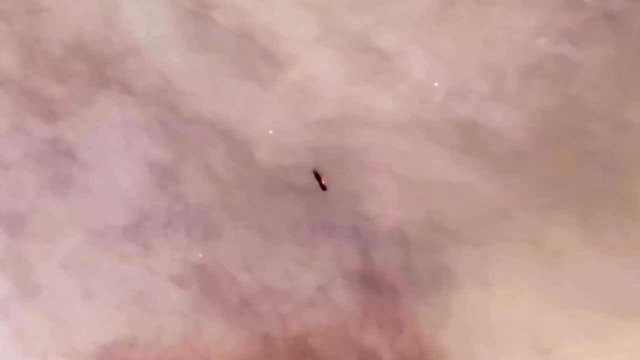 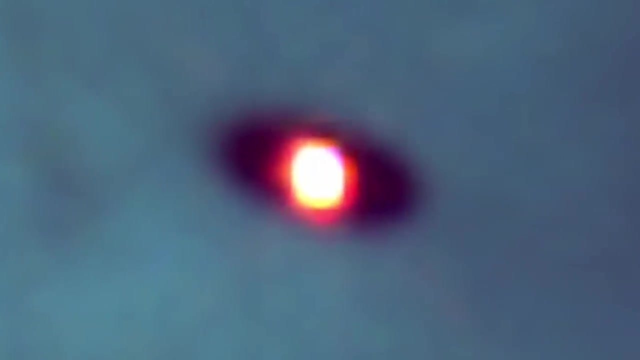 Dark propylids, only observable as silhouettes, maintain their surrounding ring of gas and dust. As the system matures, this stellar debris will form a planetary system. The Hubble Space Telescope has recorded numerous examples of this process, enough for astronomers to understand that the formation of planets is commonplace. 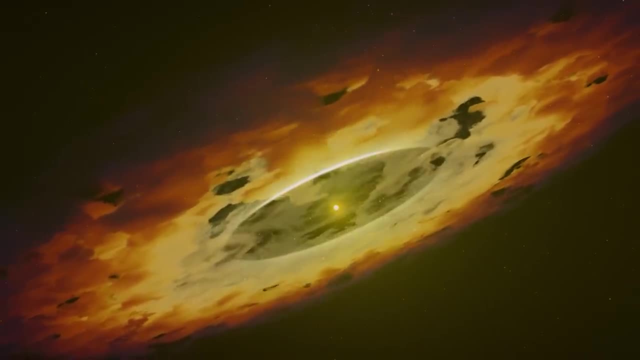 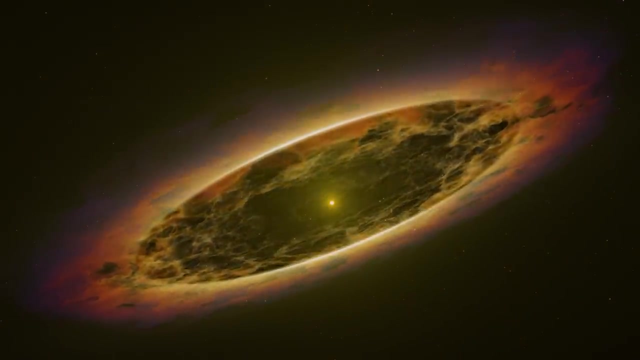 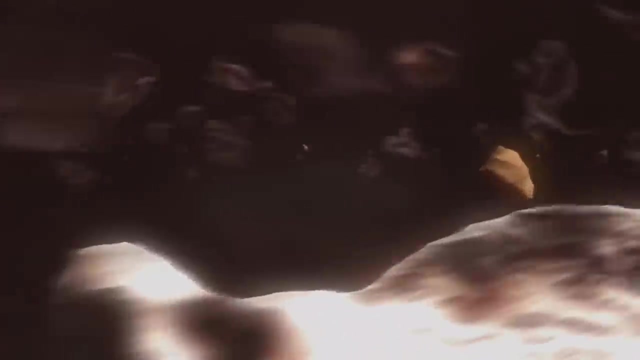 This is how our own sun started its life 4.6 billion years ago, But the planets would take longer to emerge. Small grains within the disk began accreting, forming planetesimals. The larger a clump became, the stronger its gravitational attraction. 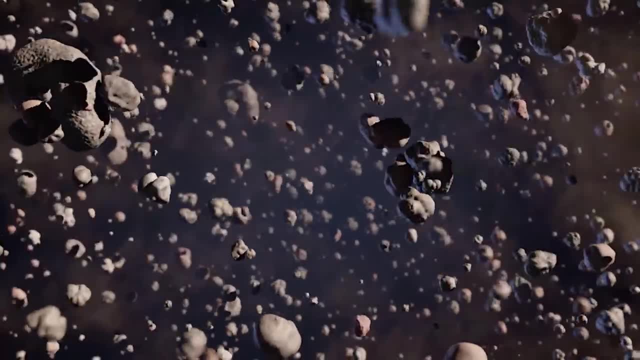 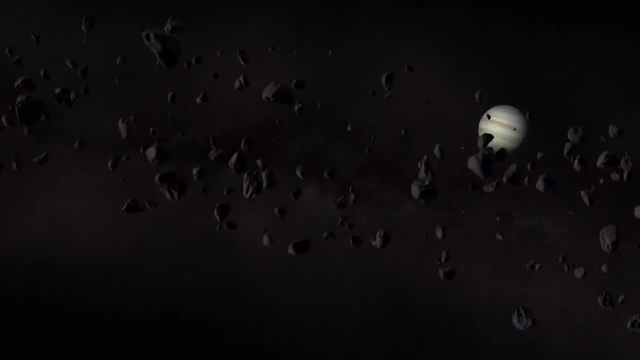 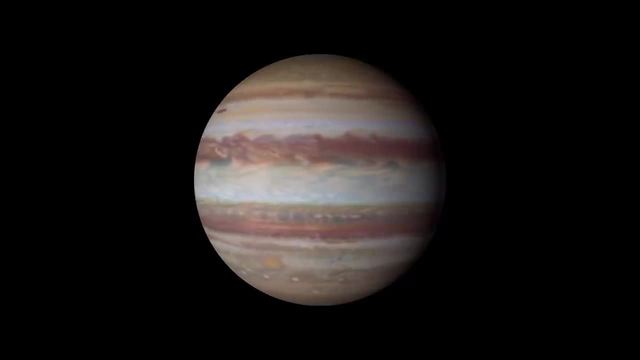 in turn leading to more rapid growth. An early version of Jupiter would have been the first to coalesce, completely, clearing its orbit Around a core of heavy metal and rock. Jupiter's atmosphere, mainly of hydrogen, was compressed by its strong gravitation. Any solid surface lay beneath thousands of kilometers of liquid gas. Our observations of exoplanets have revealed Jupiter-sized gas giants orbiting close to their stars. Astronomers believe the young Jupiter would have begun a track toward the sun, dragging asteroids and comets in with it. But Jupiter's inward path reversed as it was pushed into an orbital resonance with the emerging Saturn. Not all of the objects forming in the early solar system stayed orbiting the sun. Smaller objects passing a planet would be deflected by the stronger gravitation. 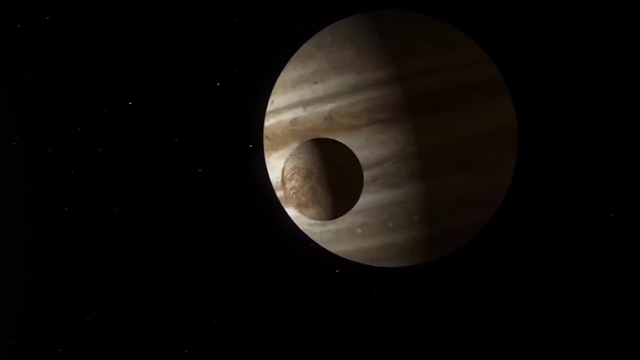 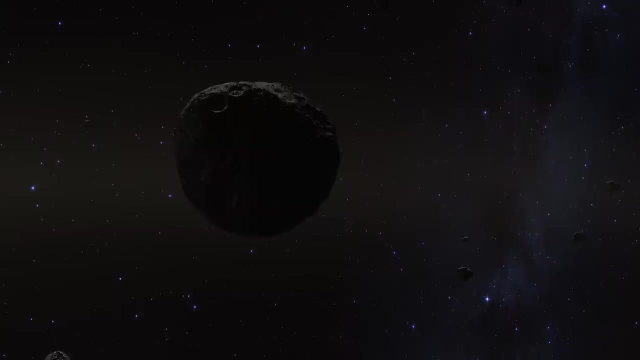 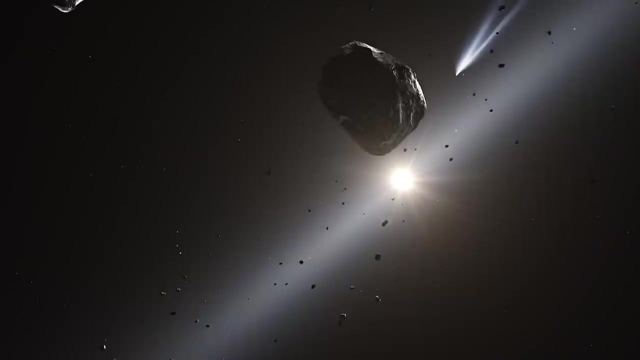 or even captured, becoming a moon. It is thought that there were up to 20 smaller planets orbiting in the inner solar system, from which the four remaining terrestrial planets were formed. At this time, collisions in the developing planetary system were common. 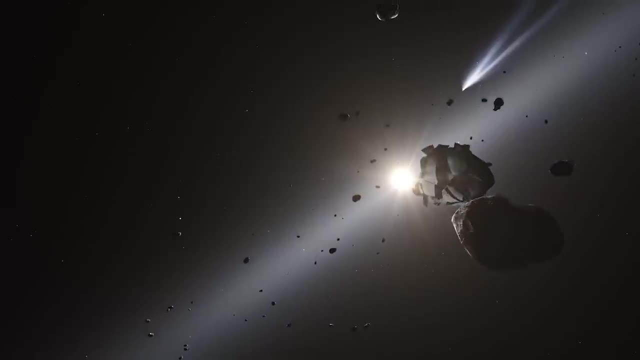 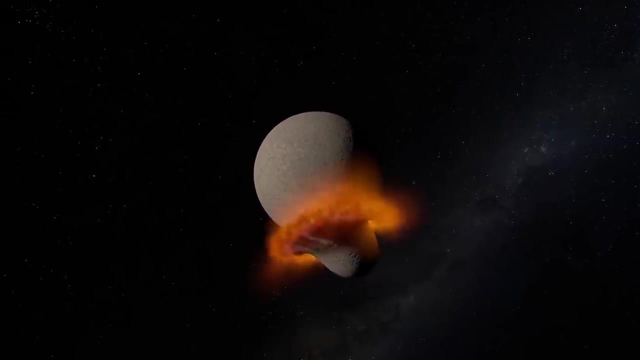 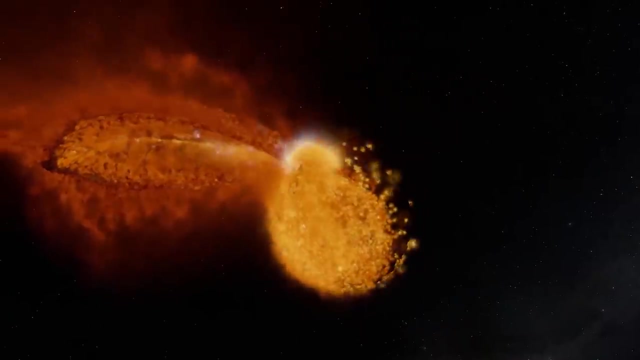 and evidence from the Apollo moon rocks suggests an impact between the early Earth and an ancestor of our moon was important in our planet's evolution. The Earth has a larger-than-expected iron core and gravitational analysis of the moon suggests its core is lighter than expected. A collision between the bodies would explain the moon's loss of much of its heavy material to the more massive Earth. The impact was a glancing blow that set the Earth rapidly spinning. with a five-hour day, The moon that we know coalesced from the multiverse. 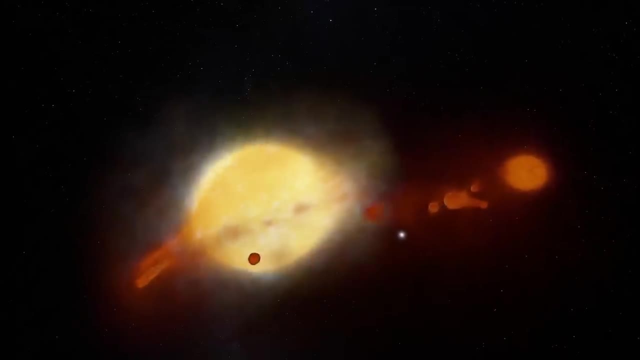 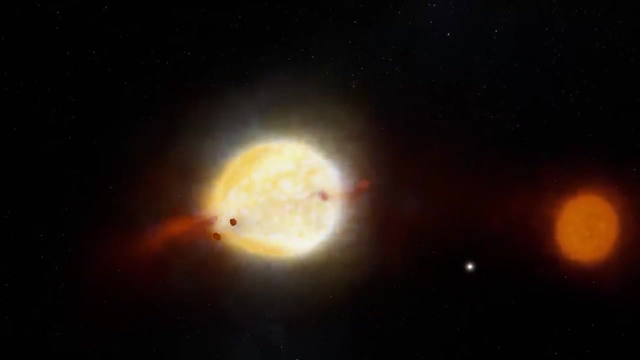 is the one that was the most active on the planet and the one that was more active in the solar system. Although the moon is the largest in the solar system, it is closer in mass to its parent planet than any other moon. The stabilizing effect that the moon has upon the Earth's rotation is significant. 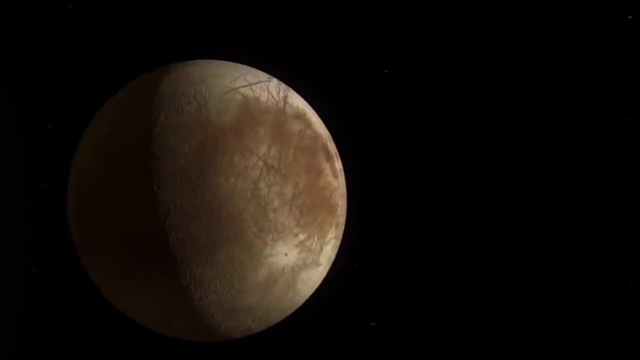 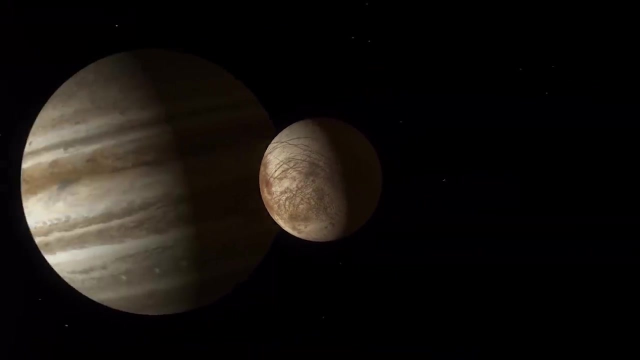 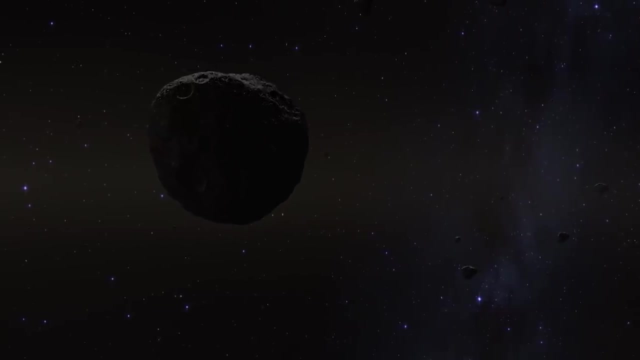 stayed orbiting the Sun. Smaller objects passing a planet would be deflected by the stronger gravitation or even captured, becoming a moon. It is thought that there were up to 20 smaller planets orbiting in the inner solar system, from which the four remaining terrestrial planets were formed At this time. collisions in the developing planetary system were common and evidence from the Apollo moon rocks suggest an impact between the early Earth and an ancestor of our Moon was important in our planet's evolution. The Earth has a larger than expected. core and gravitational analysis of the Moon suggests its core is lighter than expected. A collision between the bodies would explain the Moon's loss of much of its heavy material to the more massive Earth. The impact was a glancing blow that set the Earth rapidly spinning. with a five-hour day. The Moon that we know coalesced from the molten debris. Although our Moon is not the largest solar system, it is closer in mass to its parent planet than any other Moon. The stabilizing effect that the Moon 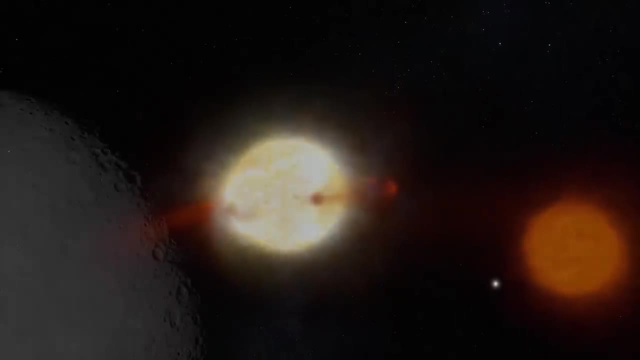 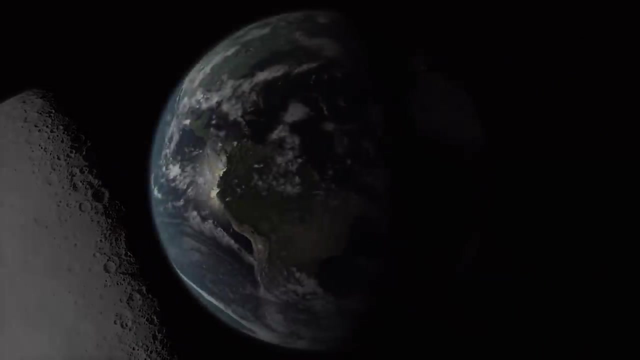 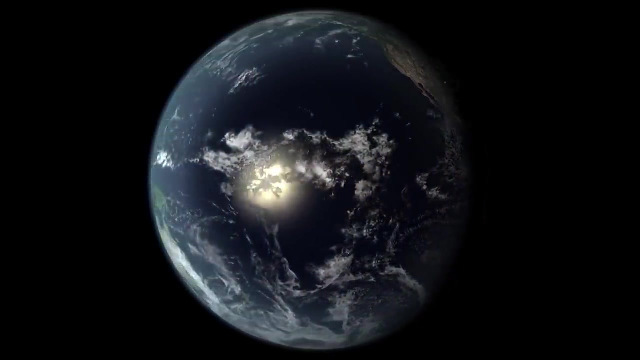 has upon the Earth's rotation is significant. Over long periods, the Earth's axis will vary by as much as one degree. Without the Moon's influence, this variation could be as much as 85 degrees, with drastic implications for the climate's stability. 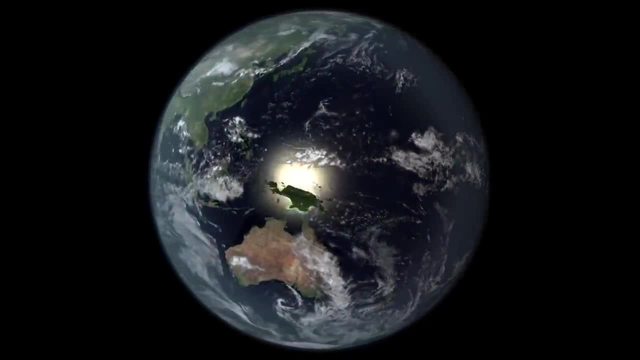 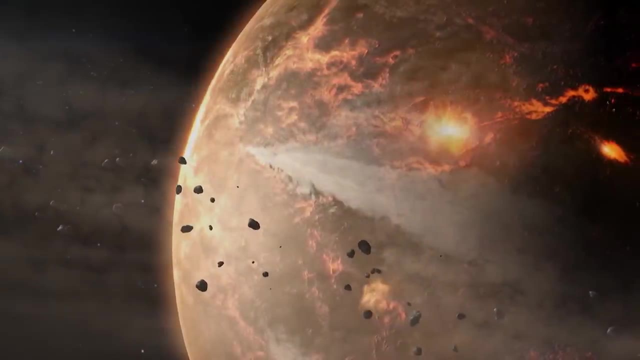 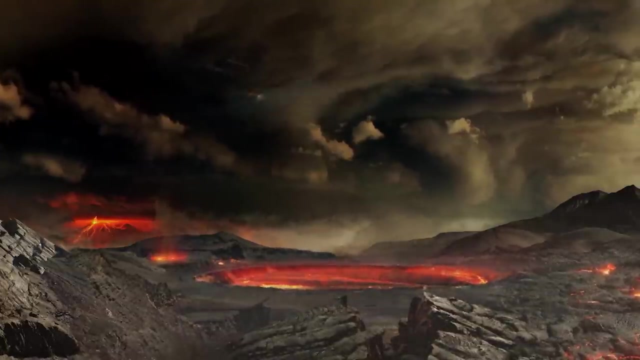 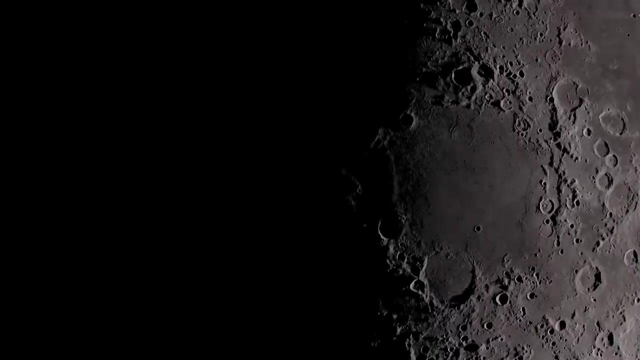 The debris in the early solar system was cleared by the planets in a period called the Heavy Bombardment. The emerging Earth was peppered with asteroids and comets delivering water necessary for life. While tectonic forces erased the bombardment scars from Earth, the Moon, 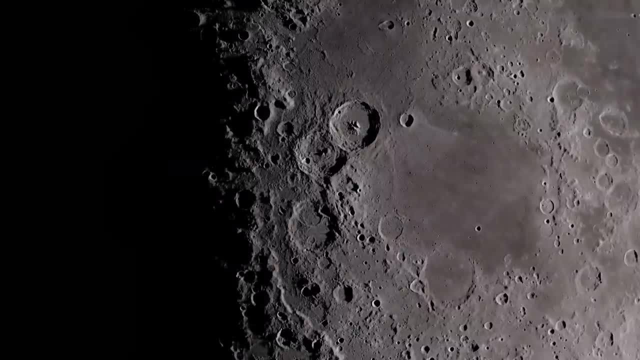 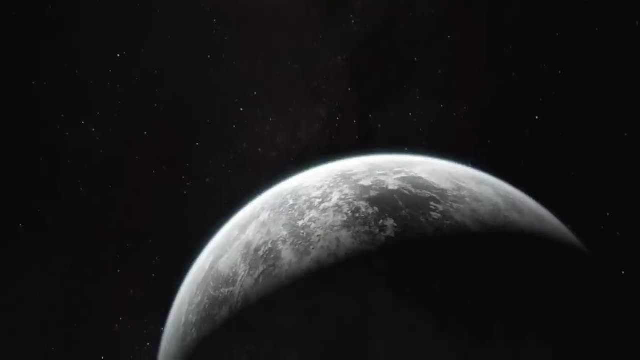 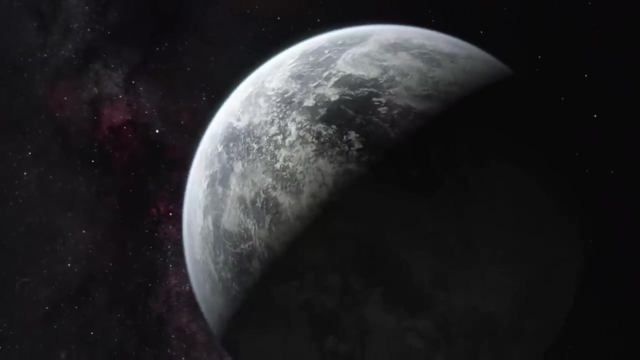 which endured the same travails, is still covered with craters. When chaos in the developing solar system settled down, the young Earth was in a unique position. The Earth's distance from the Sun was just right for the abundance of water on the planet to exist. 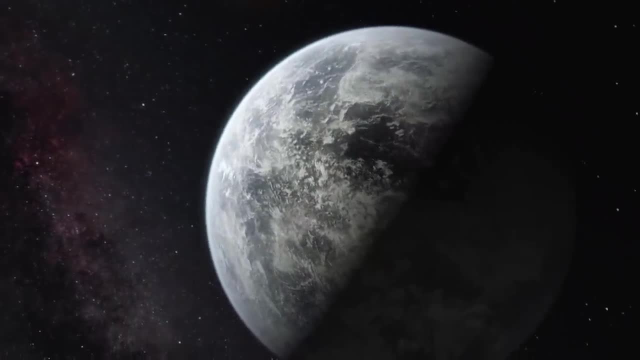 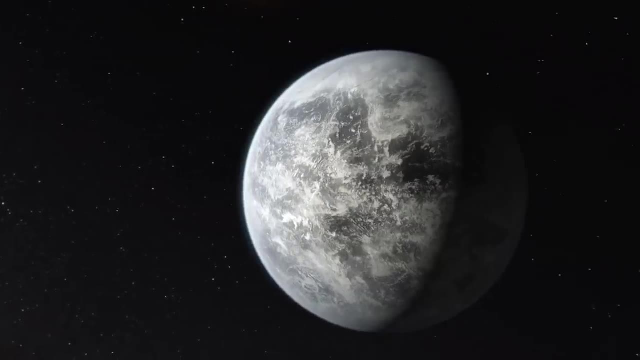 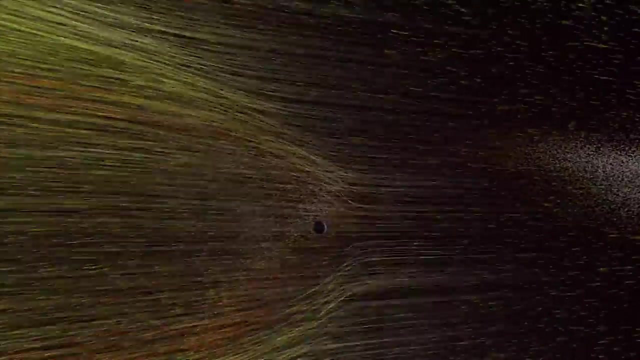 in liquid form. As the Moon had drifted away, the planet's rapid rotation had slowed and the Sun's heat was evenly shared across the surface. The Earth's large metallic core, combined with the planet's rotation, meant that a magnetic field stretched out around the planet. 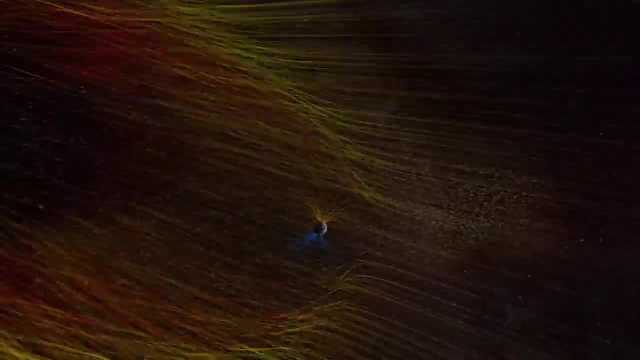 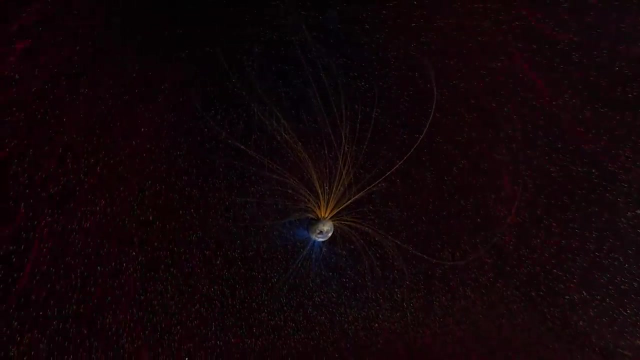 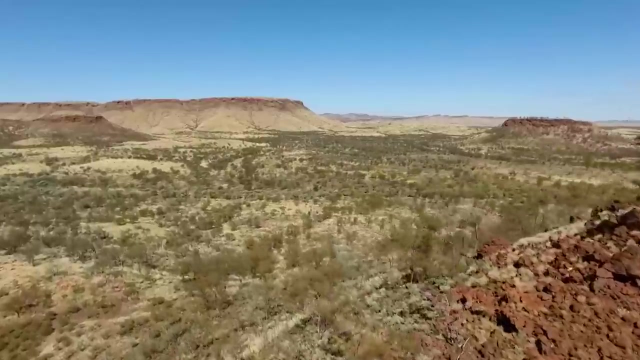 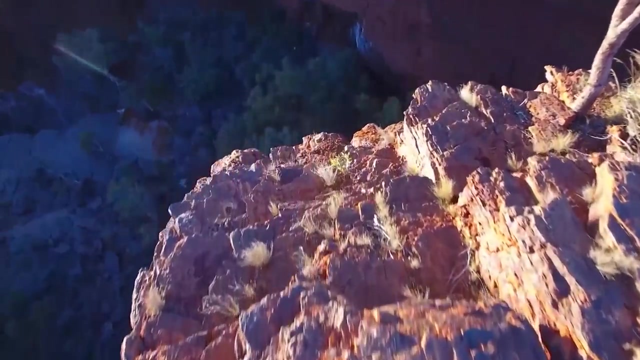 deflecting the charged solar wind and protecting the surface from extremes of solar radiation In a hostile universe. the Earth was a uniquely benign environment. The geological record shows that around 2.7 billion years ago oxygen began occurring in the atmosphere. The vast iron ore regions 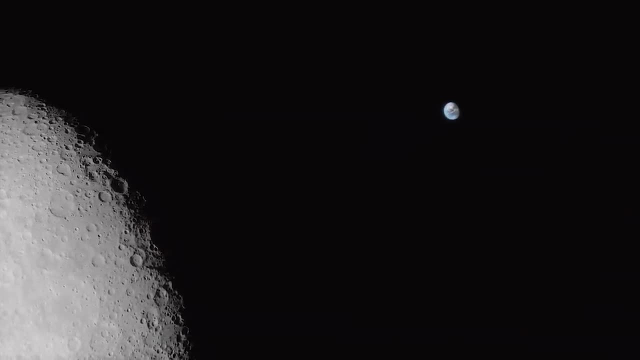 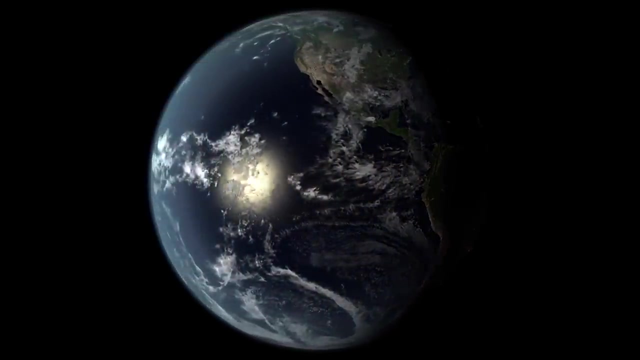 Over long periods, the Earth's axis will vary by as much as 1 degree. Without the moon's influence, this variation could be as much as 85 degrees, with drastic implications for the climate's stability. The debris in the early solar system. 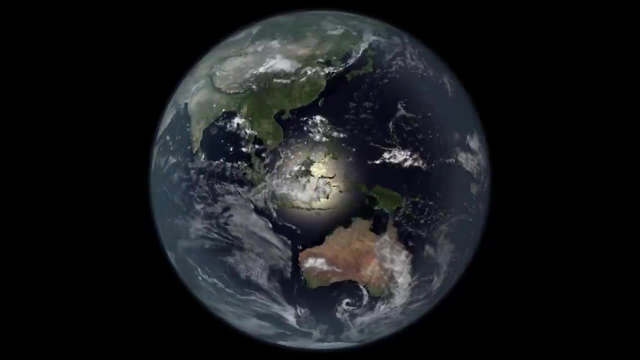 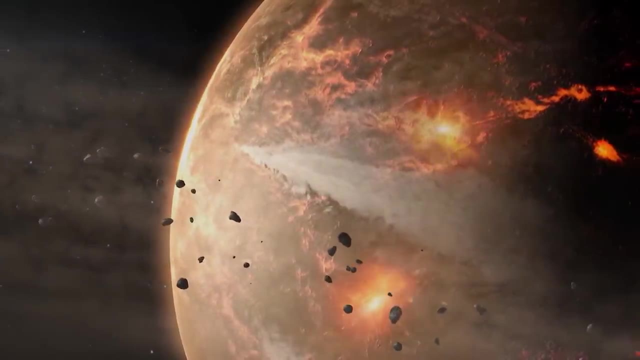 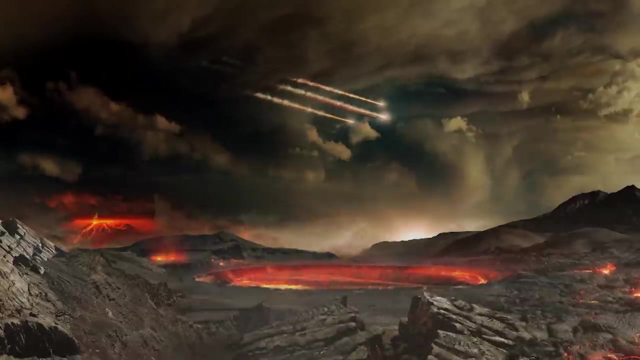 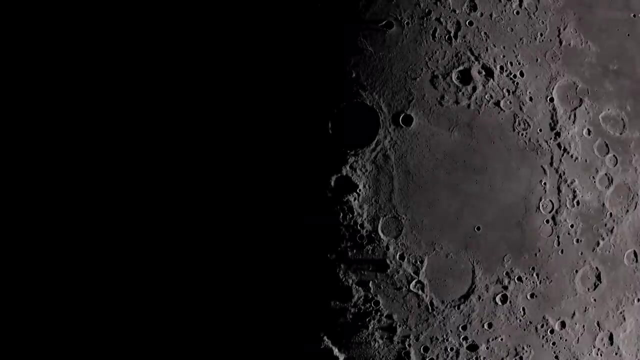 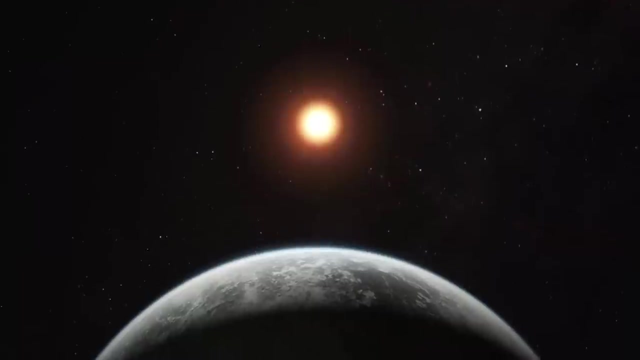 was cleared by the planets in a period called the heavy bombardment. the emerging earth was peppered with asteroids and comets, delivering water necessary for life. while tectonic forces erased the bombardment scars from Earth, the moon, which endured the same travails, is still covered with craters. when chaos and the developing solar system settled down, the young earth was in a unique position. the Earth's distance from the Sun was just right for the abundance of water on the planet to exist in liquid form. as the moon had drifted away, the planets, rapid rotation had slowed and the Sun's heat was evenly shared across the surface. 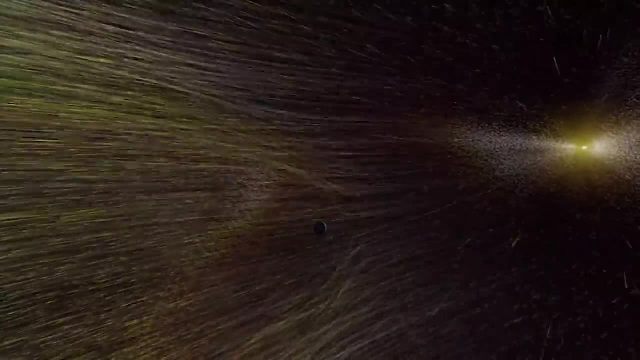 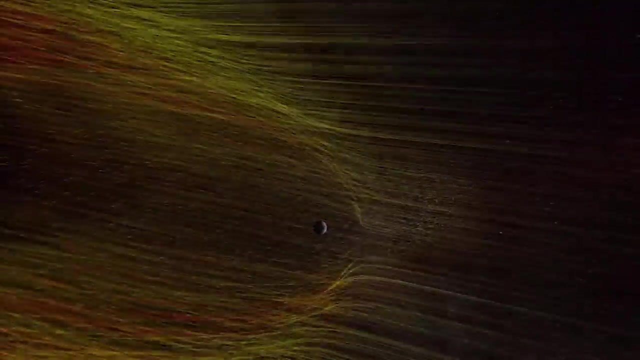 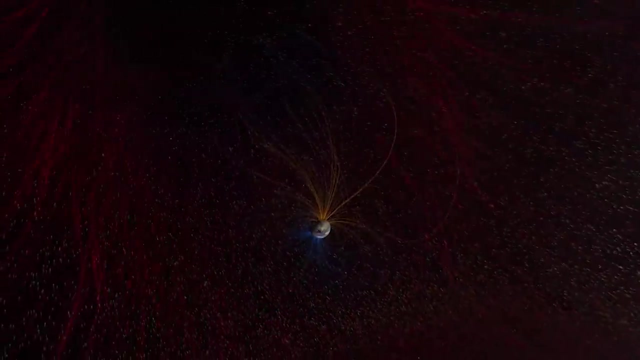 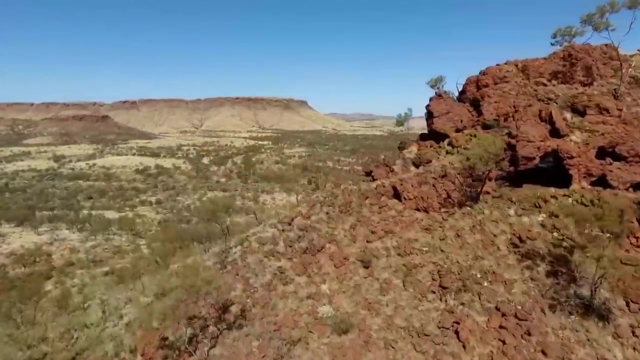 you. the Earth's large metallic core, combined with the planet's rotation, meant that a magnetic field stretched out around the planet, deflecting the charged solar wind and protecting the surface from extremes of solar radiation. in a hostile universe, the earth was a uniquely benign environment. the geological record shows that around 2.7 billion years ago, oxygen was. 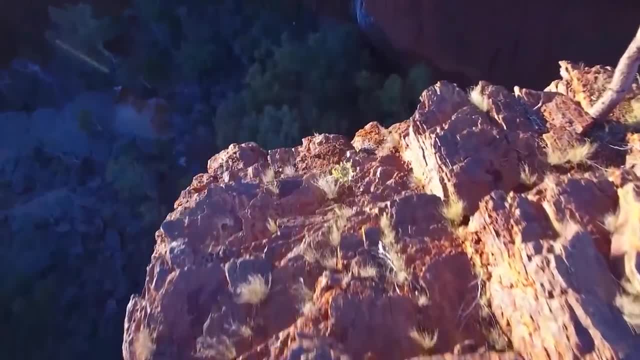 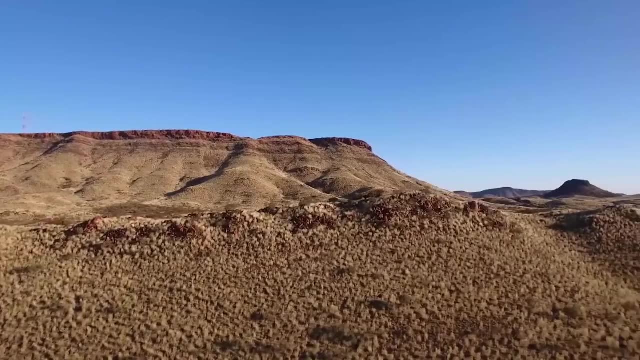 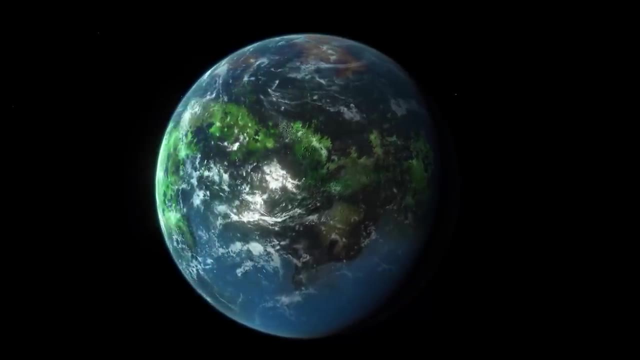 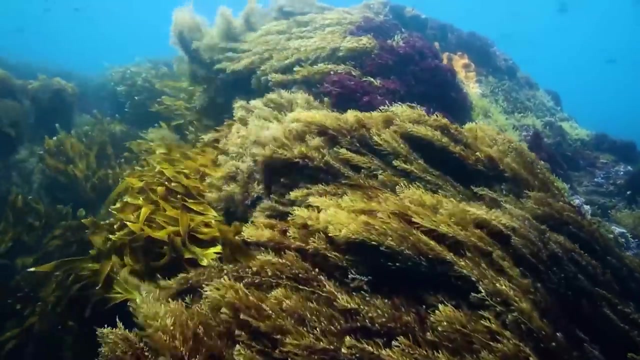 ini altitude in the atmosphere. the vast iron ore regions of Western Australia were formed as iron in the oceans reacted with the new abundance of oxygen to form iron oxide. in Bangor, plant life was using the Sun and calm micron carbon dioxide looks a bit Waldøre. each living field was apart from the surface by powderJack Sharp. the way oxygen was formed as iron in the oceans reacted with neu abundance of oxygen to form iron oxide. simple plant life was using the sunlight and carbon dioxide to live and it produced highly reactive oxygen as a waste product. aş sesigrit perspektive들. 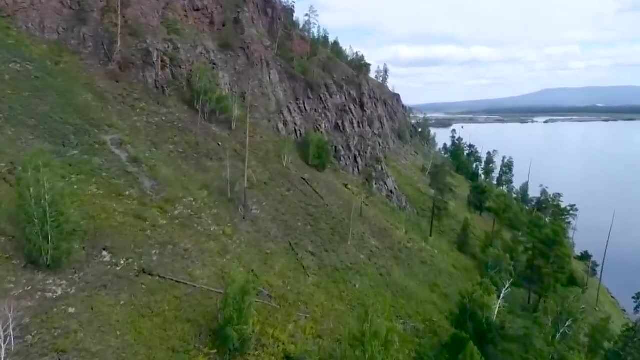 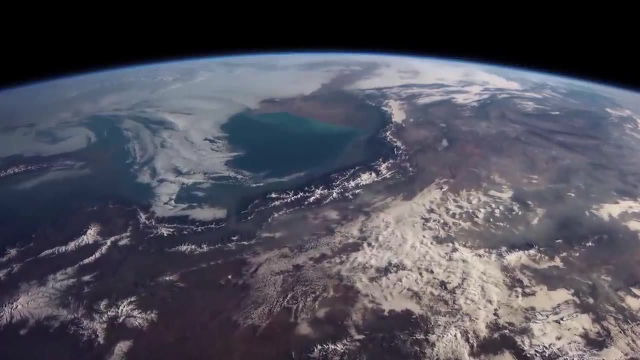 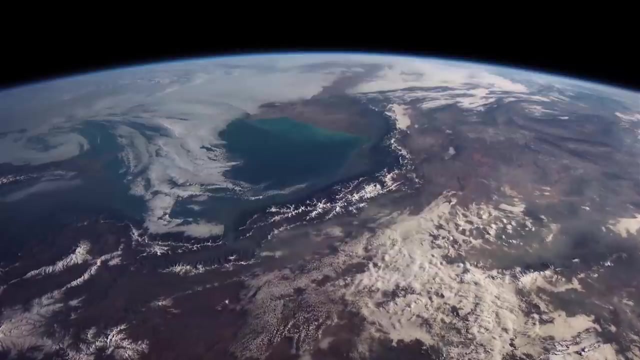 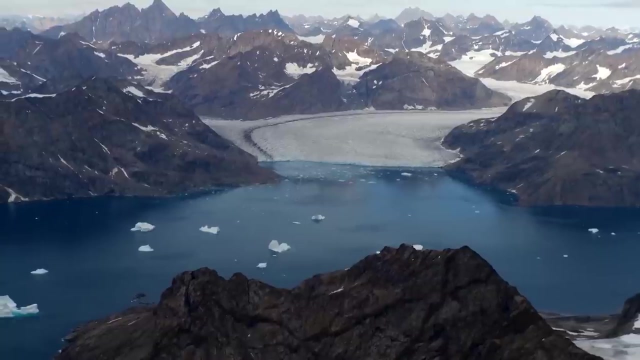 resusa pasadovensja, completely transforming the planet. the change in the atmosphere had other dramatic consequences. oxygen stripped much of the highly insulating gases from the air, drastically cooling the earth. a sequence of ice ages began, though there is an abundance of evidence showing planetary glaciation punctuated by warm. 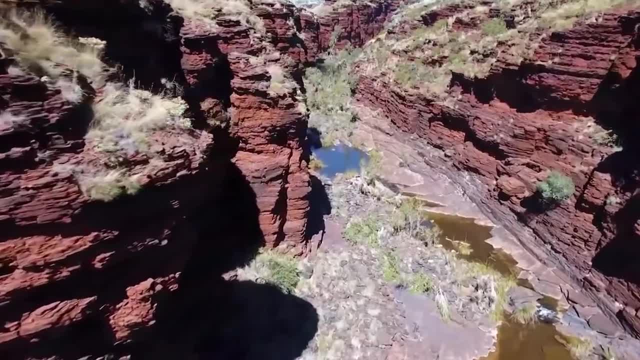 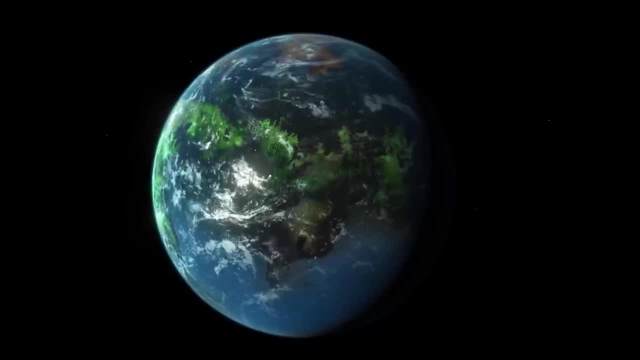 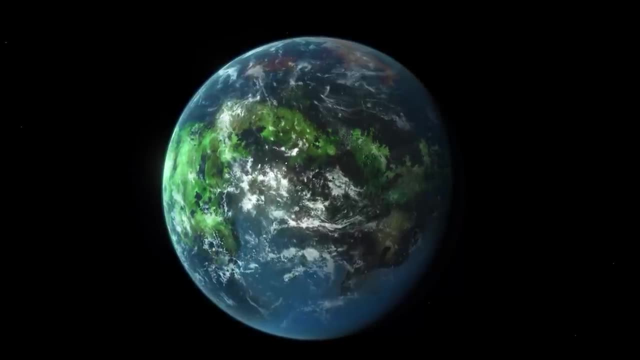 of Western Australia formed as iron in the oceans reacted with the new abundance of oxygen to form iron oxide. Simple plant life was using the sunlight and carbon dioxide to live and it produced highly reactive oxygen as a waste product. This enabled more complex life to emerge. 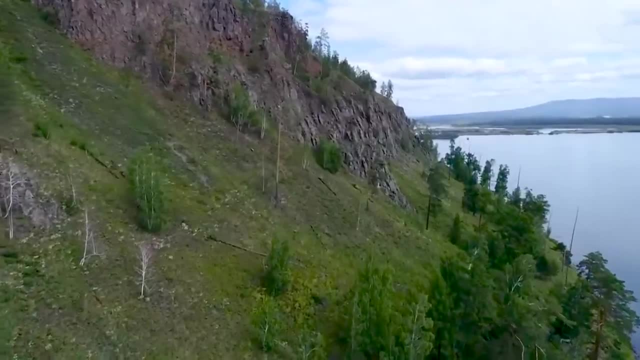 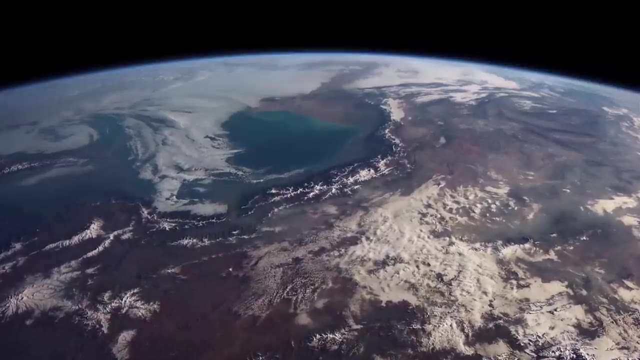 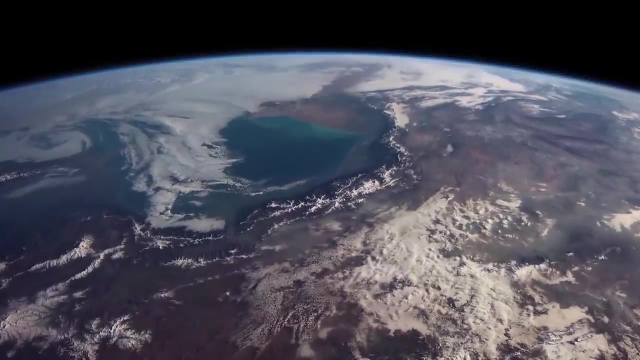 building an intricate web of interrelated plants and animals, completely transforming the planet. The change in the atmosphere had other dramatic consequences. Oxygen stripped much of the highly insulating gases from the air, drastically cooling the Earth. A sequence of ice ages began. Though there is an abundance, 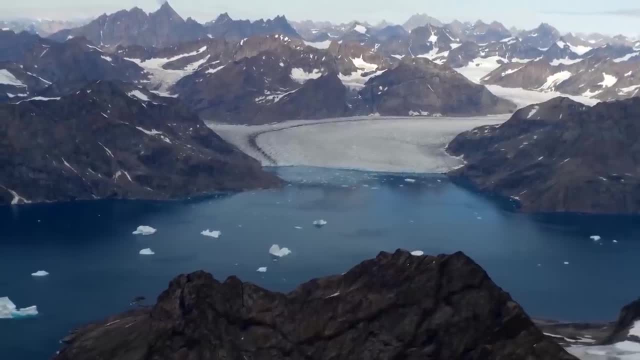 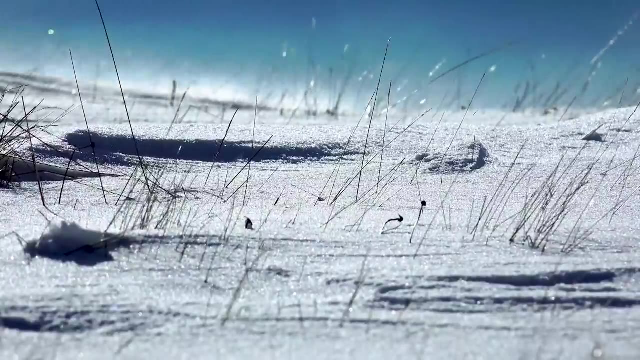 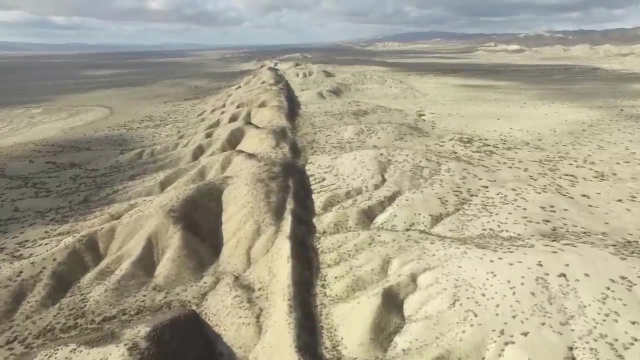 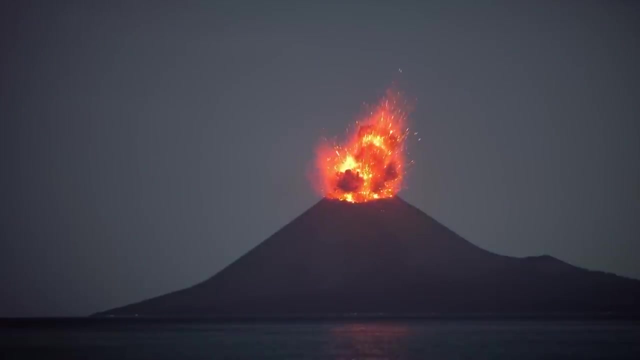 of evidence showing planetary glaciation punctuated by warm periods. the factors triggering these cycles are complex. Fault lines are clues to the movement of continents, leading to diversions of ocean currents, the effect of volcanic activity on the atmosphere and changes in the direction. 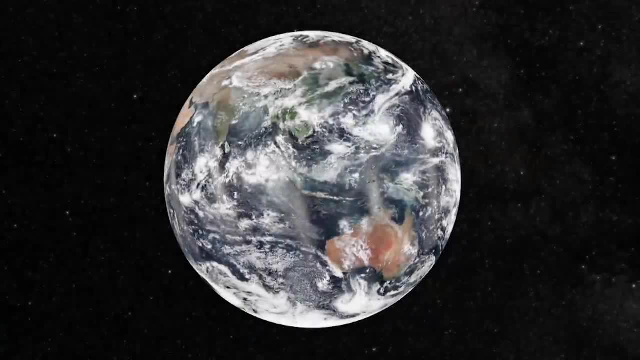 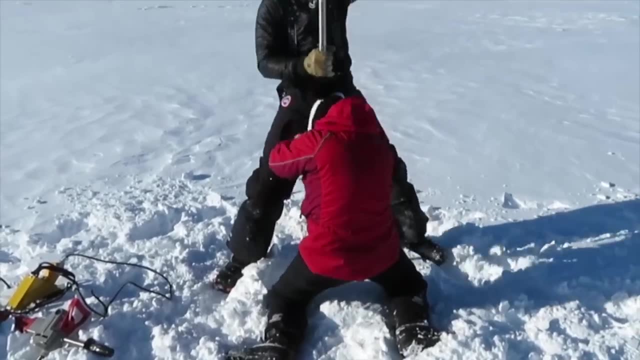 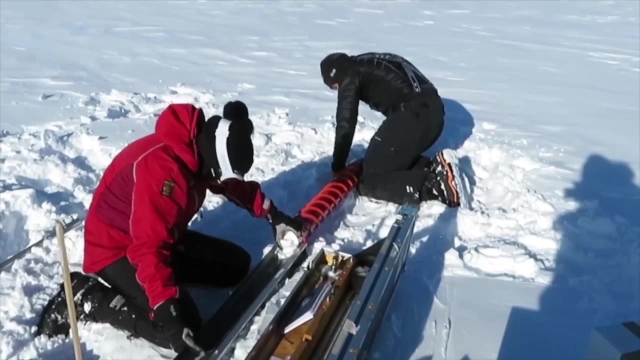 of the Earth's axis with regard to our planet's elliptical orbit around the Sun, all contributors to long-term fluctuations in the Earth's climate. Analysis of ice cores deposited in the Antarctic is an accurate way to see how the composition of the atmosphere has changed. 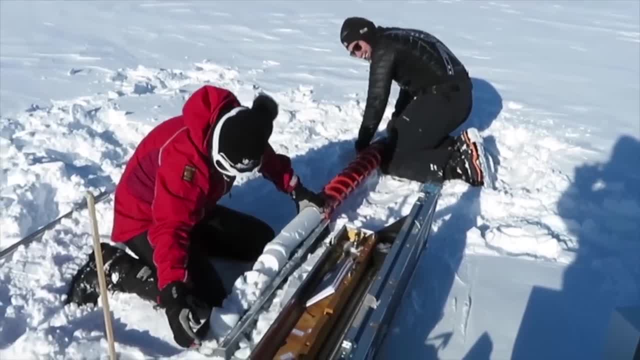 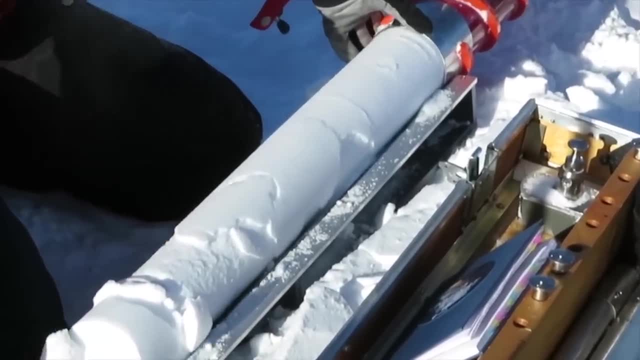 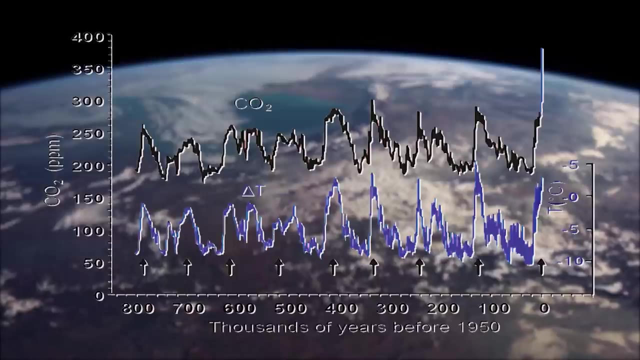 over the previous 800,000 years. Bubbles of air caught between snowflakes, before being rigidly trapped as the snow becomes ice, can be accurately sampled. One thing is clear: Carbon dioxide reaches a peak of around 270 parts per million during the warm periods. 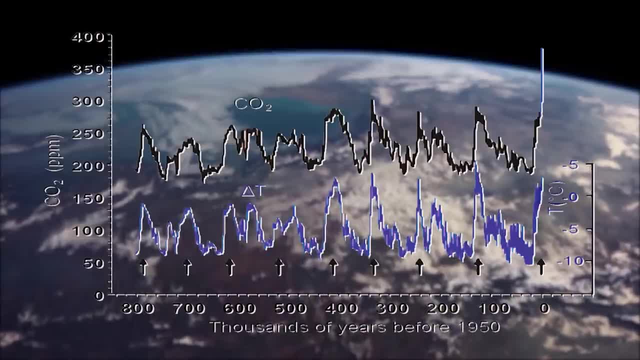 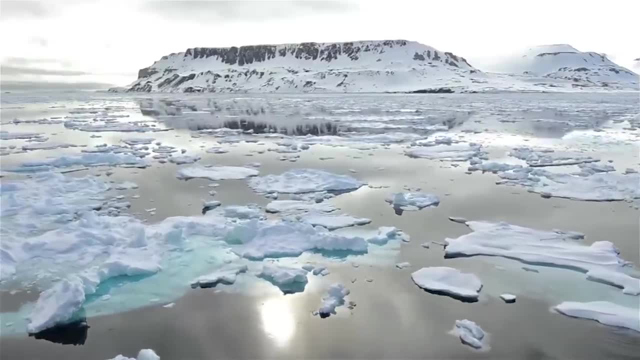 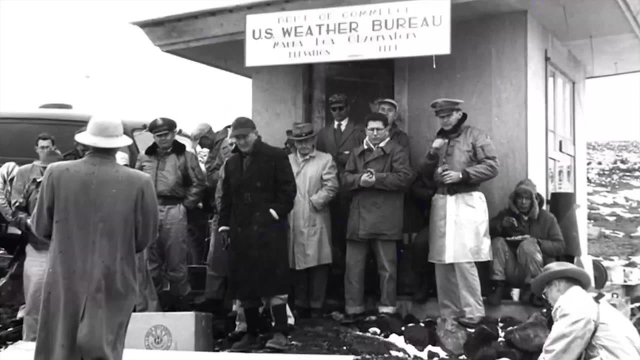 and drops to approximately 170 parts per million when glaciation is at its greatest. But from this data it's hard to know if extra CO2 causes the warming or the warming leads to extra CO2.. In 1958, Dave Keeling. 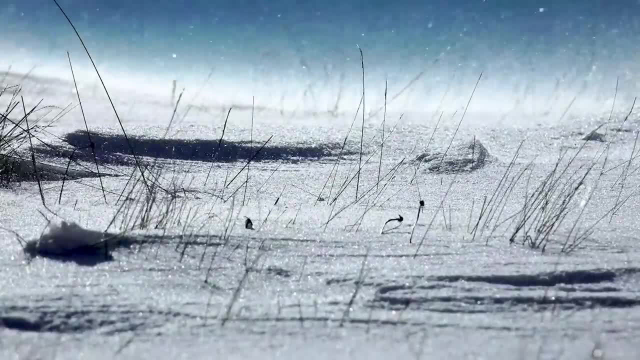 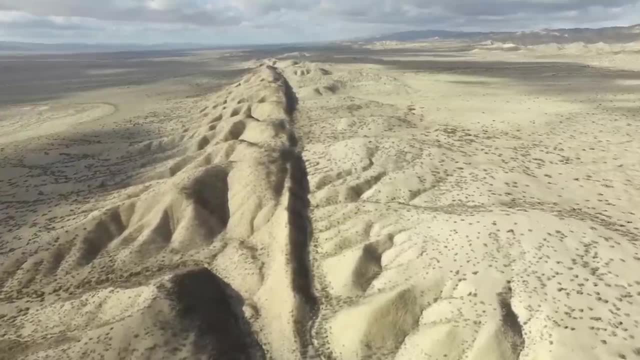 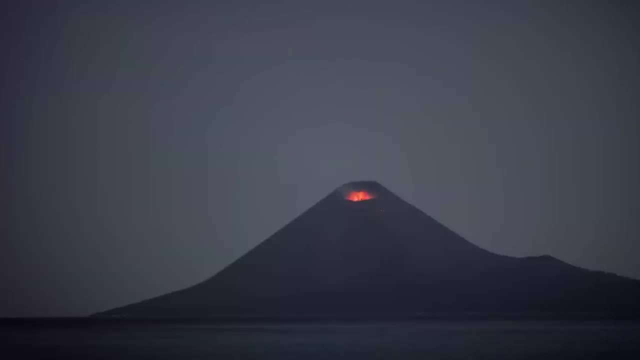 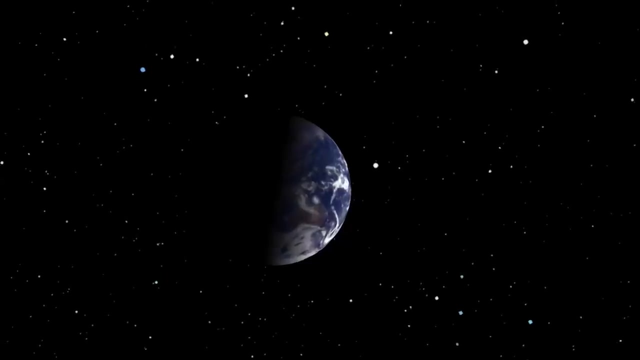 periods. the factors triggering these cycles are complex: fault lines are clues to the movement of continents, leading to diversions of ocean currents, the effect of volcanic activity on the atmosphere and changes in the direction of the Earth's axis with regard to our planet's elliptical orbit around the Sun. 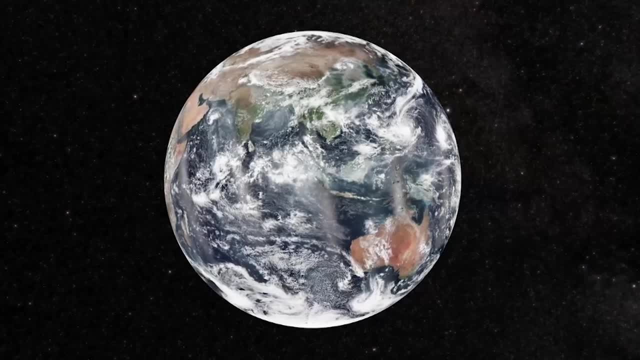 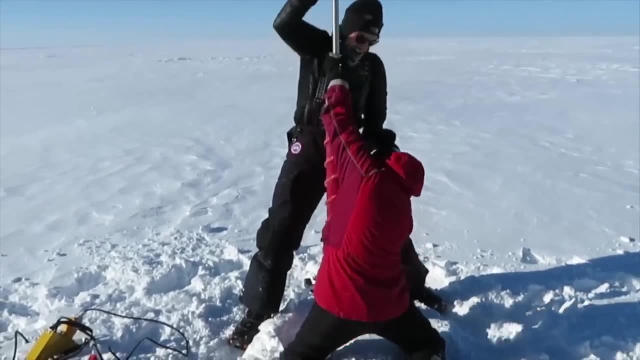 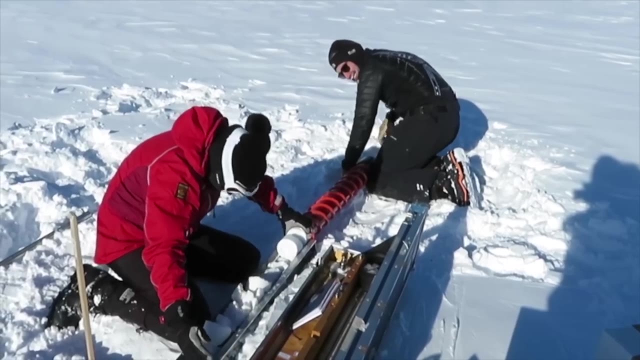 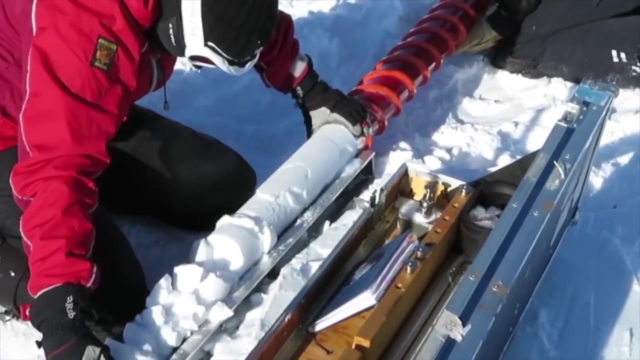 all contributors to long-term fluctuations in the Earth's climate. analysis of ice cores deposited in the Antarctic or Greenland is an accurate way to see how the composition of the atmosphere has changed over the previous 800,000 years. bubbles of air caught between snowflakes before being rigidly. 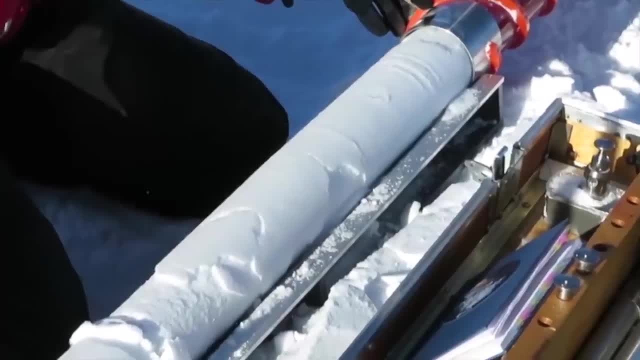 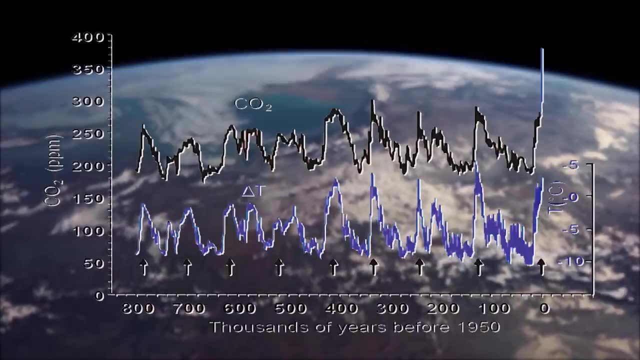 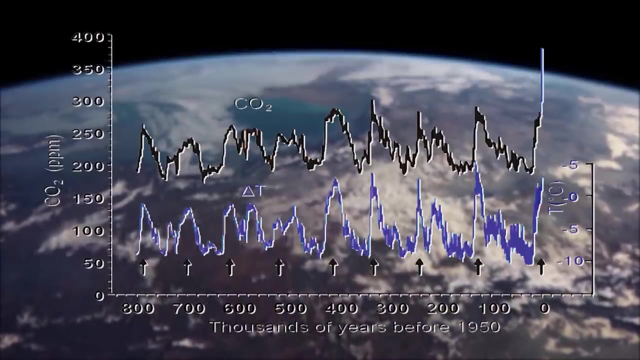 trapped as the snow becomes ice can be accurately sampled. one thing is clear: carbon dioxide reaches a peak of around 270 parts per million during the warm periods and drops to approximately 170 parts per million when glaciation is at its greatest. but from this data it's hard to 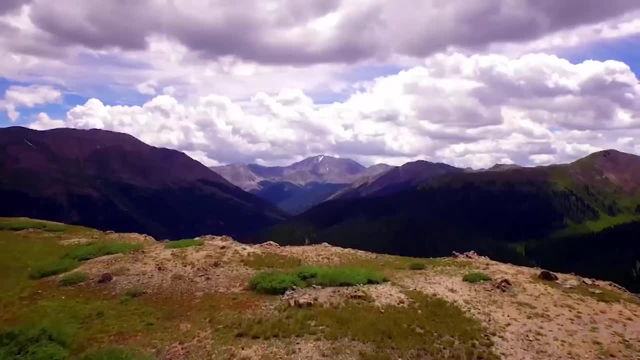 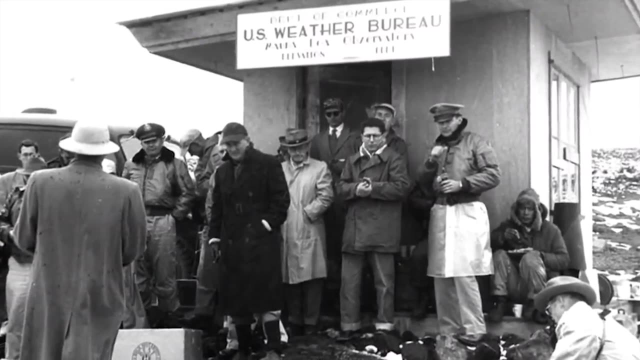 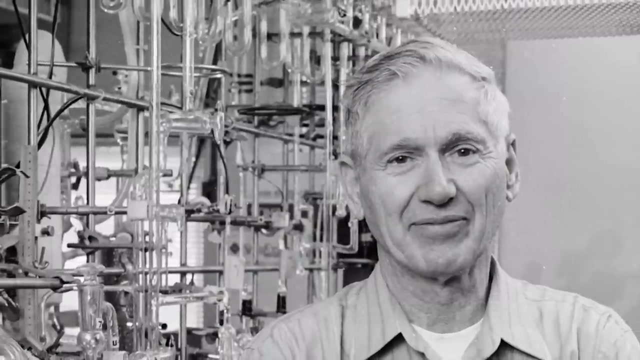 know if extra co2 causes the warming or the warming leads to extra co2. in 1958, Dave Keeling, working for the Scripps Institute, began recording accurate levels of atmospheric co2 at the Mauna Loa Observatory in Hawaii. it was the beginning of a unique record known as. 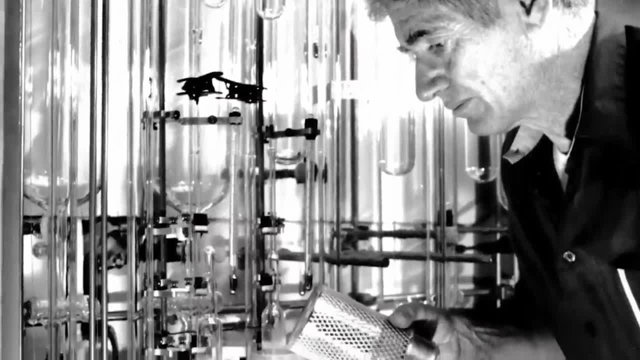 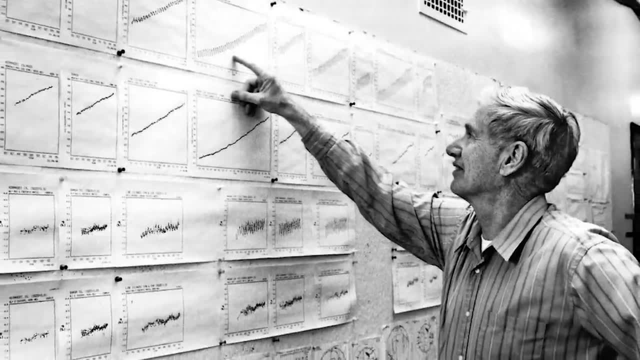 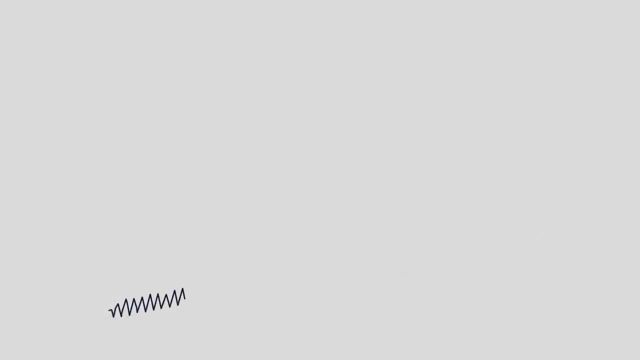 the Keeling curves. Keeling's graph revealed a seasonal variation corresponding to spring and summer in the northern hemisphere, where landmass and plant cover is greater. during the northern spring and into the summer, co2 levels dropped because of the increase in photosynthesis. by the 1970s a disturbing trend had emerged: co2. 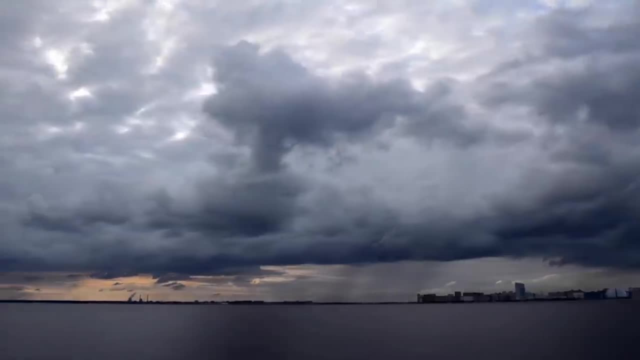 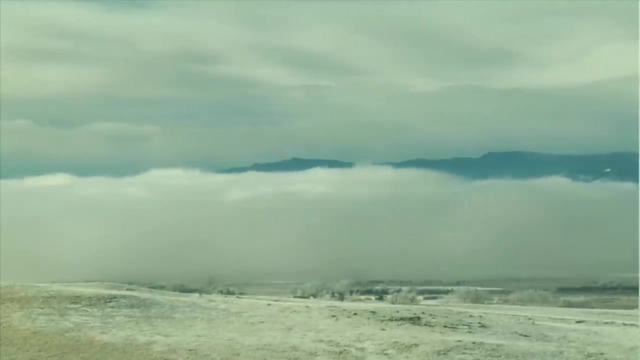 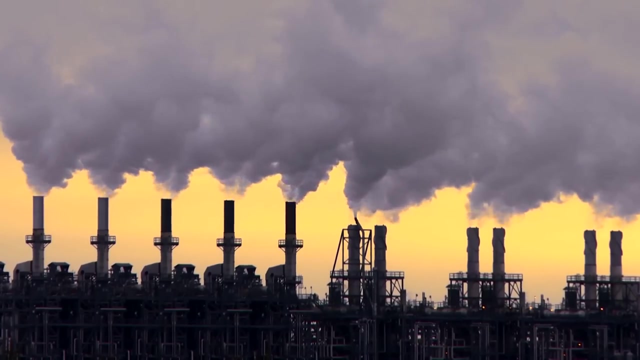 levels were in a steady rise. at first, there was uncertainty about the implications. extra co2 could trap more heat, leading to a warming effect known as the greenhouse effect. but some scientists were worried that aerosol pollution could attenuate levels of sunlight reaching the planet, resulting in a cooling environment. 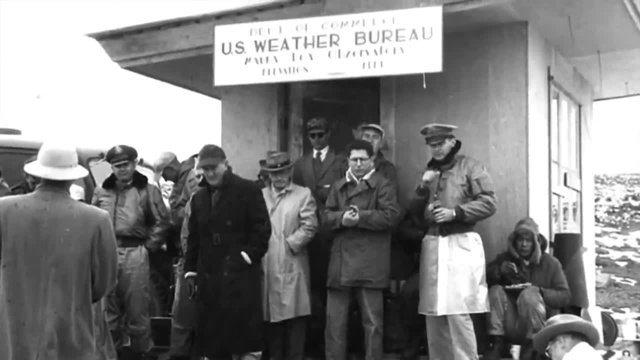 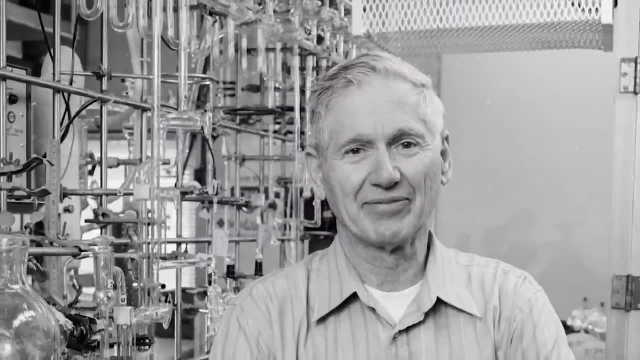 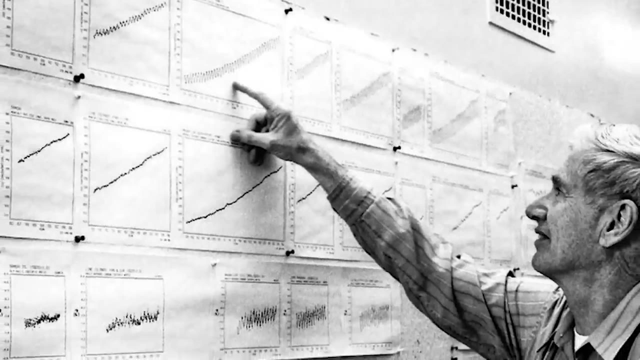 working for the Scripps Institute, began recording accurate levels of atmospheric CO2 at the Mauna Loa Observatory in Hawaii. It was the first time to record a graph of the Earth's climate in the Northern Hemisphere. The graph was called the Keeling Curves. 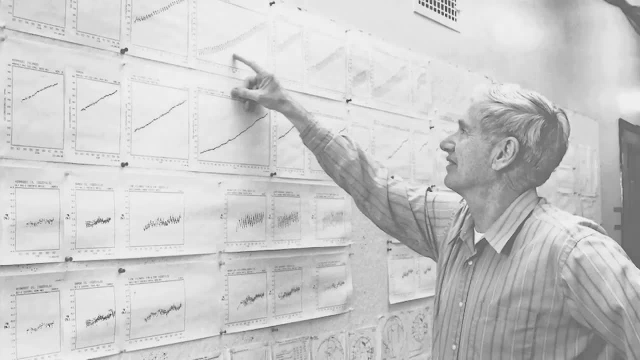 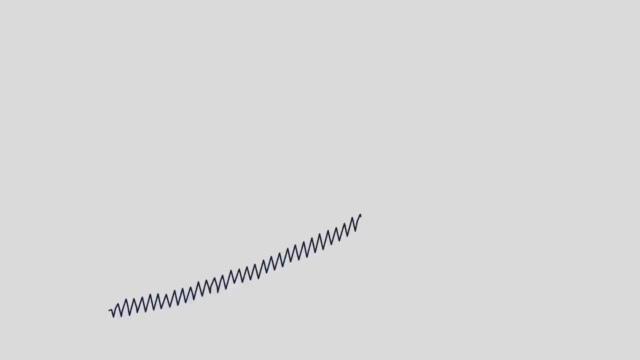 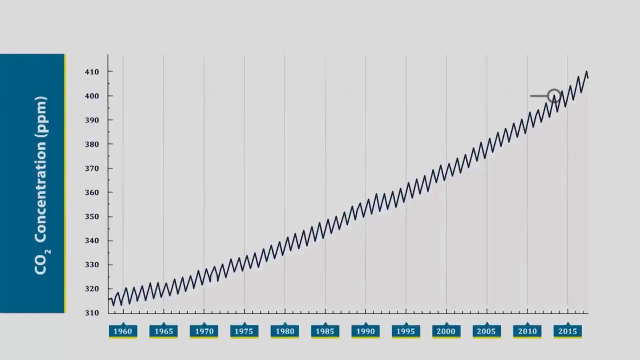 Keeling's graph revealed a seasonal variation corresponding to spring and summer. in the Northern Hemisphere, where land mass and plant cover is greater. During the northern spring and into the summer, CO2 levels were in a steady rise. At first there was uncertainty about the implications. 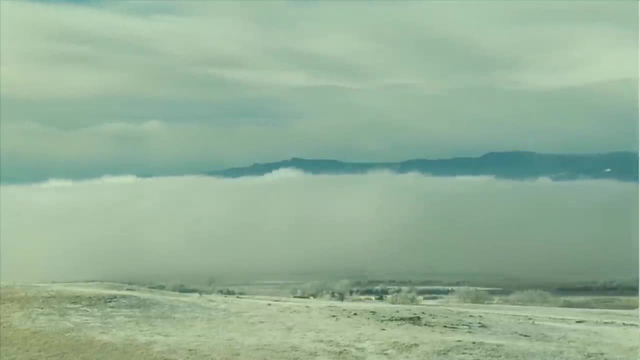 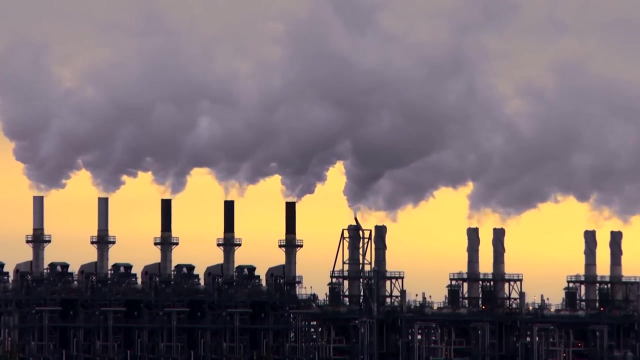 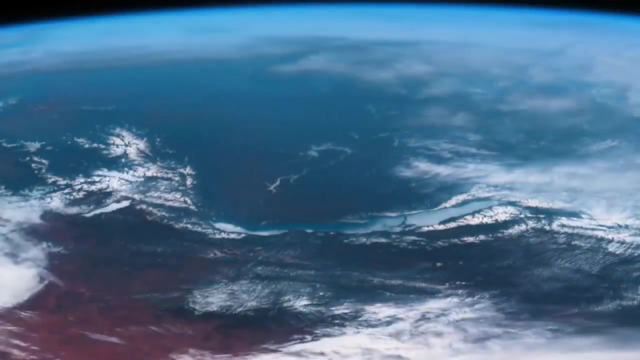 Extra CO2 could trap more heat, leading to a warming effect known as the greenhouse effect. But some scientists were worried that aerosol pollution could attenuate levels of sunlight reaching the planet, resulting in a cooling environment As the decades passed. different pieces of evidence. 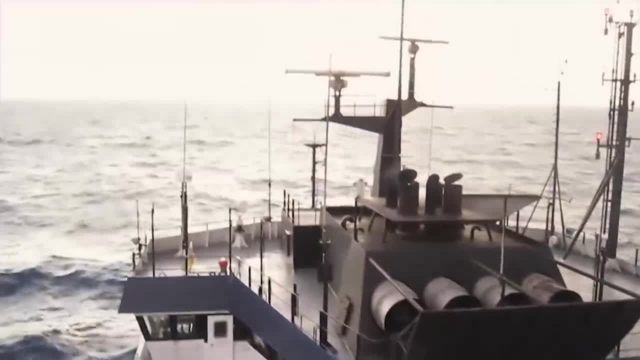 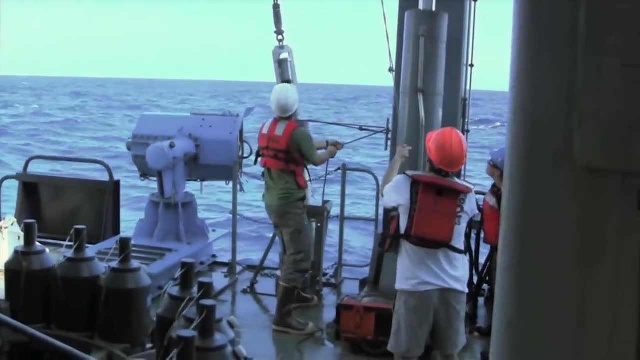 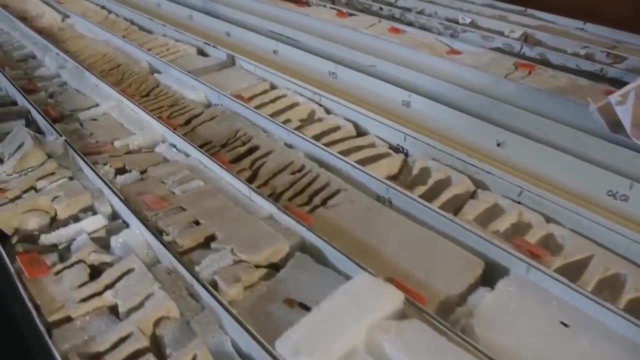 were collected, Drill cores from the ocean floor revealed that ice ages had been triggered by Milankovitch cycles, the variations between Earth's tilt and its elliptical orbit. Though these effects were minor, the correlation was obvious. If such a small nudge 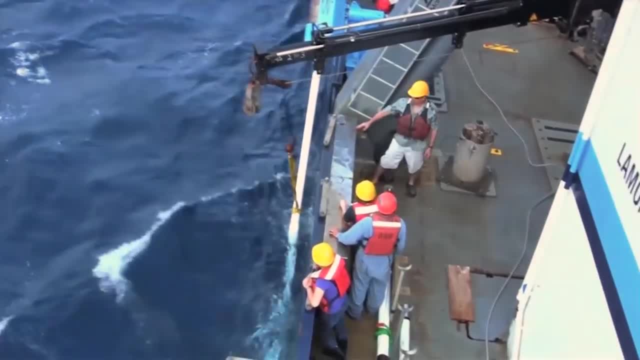 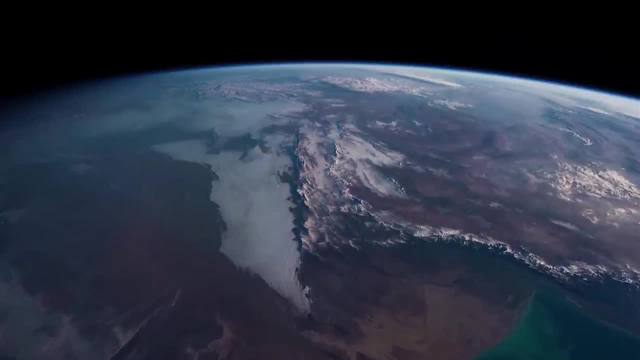 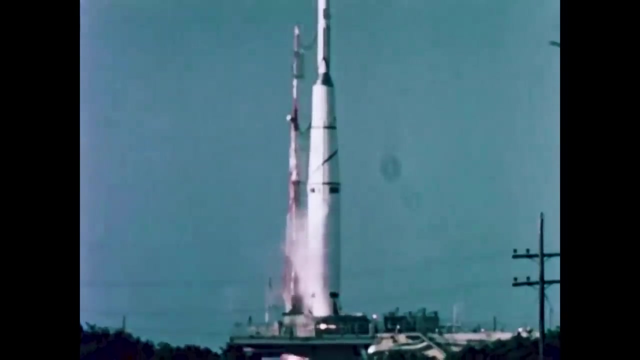 could alter the climate. perhaps changes in CO2 could as well. Scientists were realizing just how poorly they understood planet Earth. In the early 20th century. scientists were trying to make weather observations from orbit At the beginning of the space age. 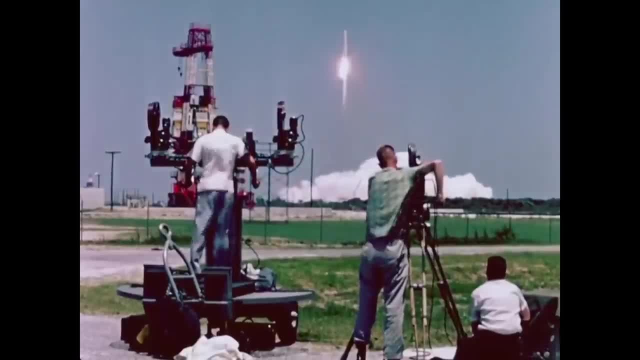 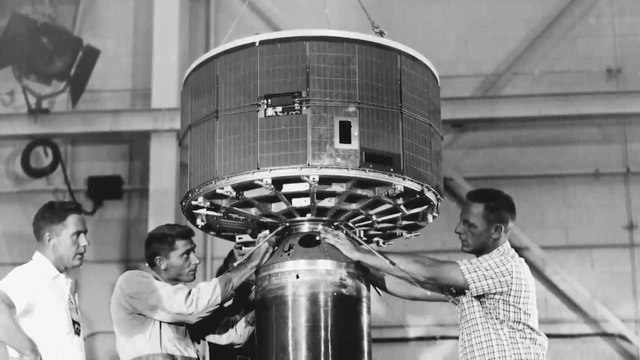 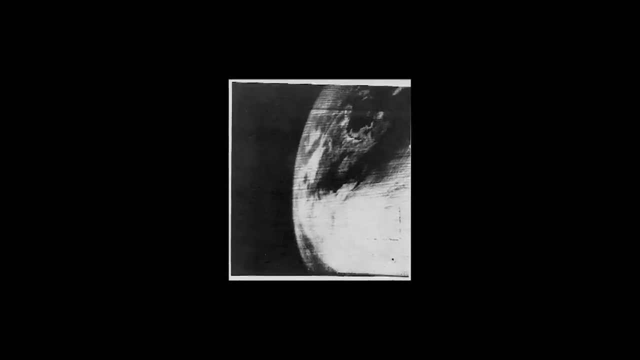 scientists were keen to make weather observations from orbit. Launched in 1960, TIROS-1 was the first weather satellite. It was equipped with two TV cameras regularly transmitting images of global cloud patterns. It provided meteorologists with a unique view. 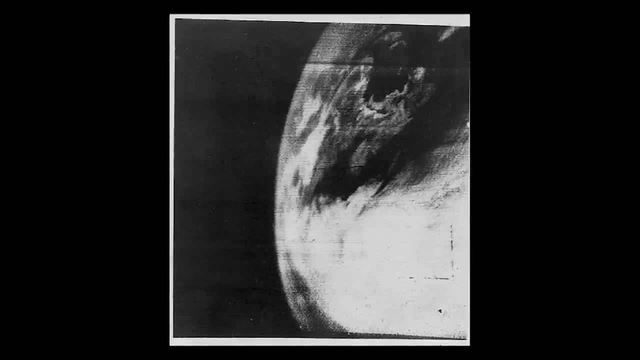 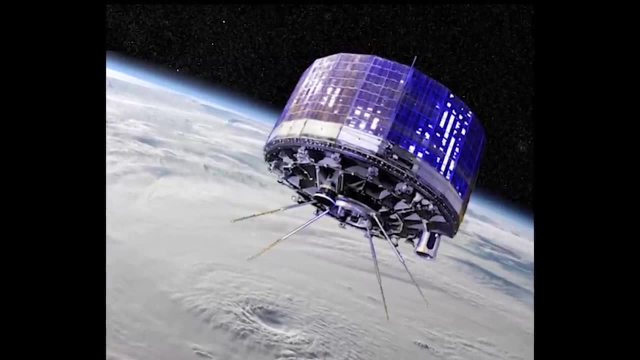 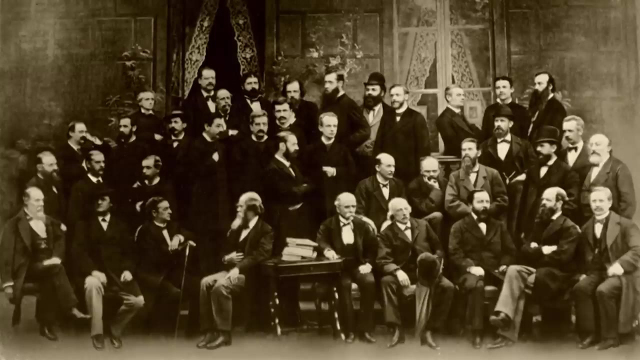 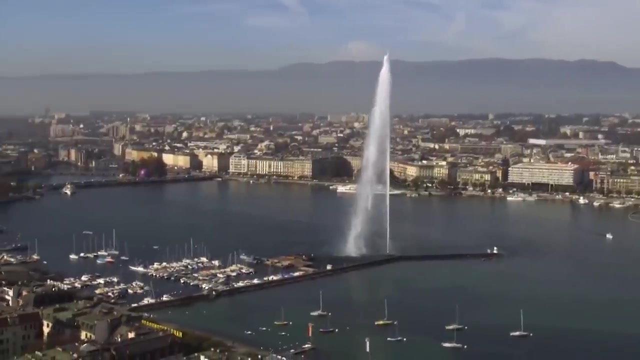 and it was followed by improved versions. Because these early satellites were in highly inclined low Earth orbits, the data gathered covered the whole planet and it was shared across the world. Since 1873, nations had been cooperating on weather prediction via the International 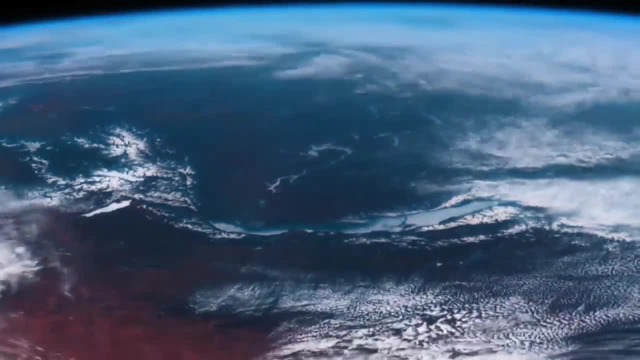 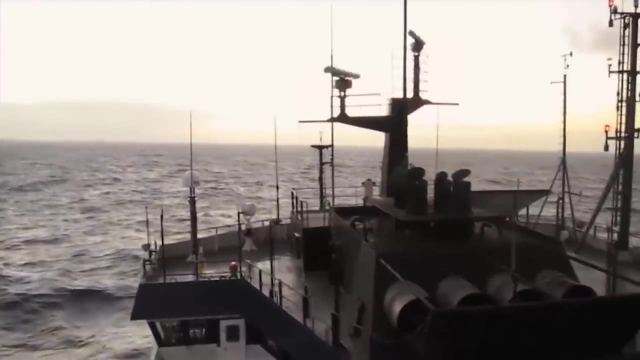 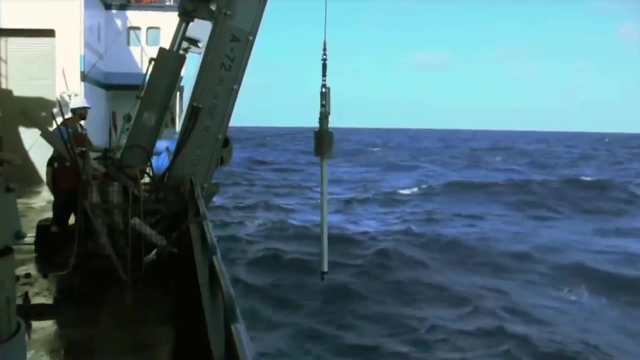 as the decades passed, different pieces of evidence were collected. drill calls from the ocean floor revealed that ice ages had been triggered by Milankovitch cycles, the variations between Earth's tilt and its elliptical orbit. though these effects were minor, the correlation was obvious. if such a small 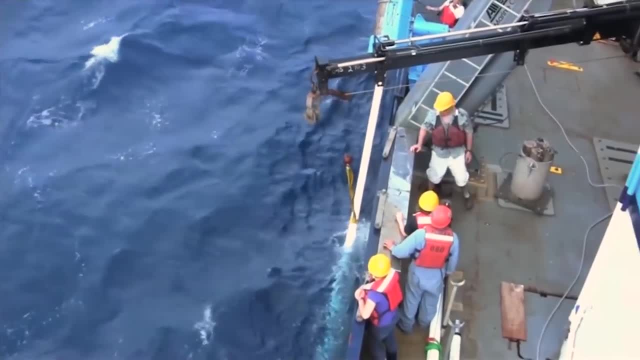 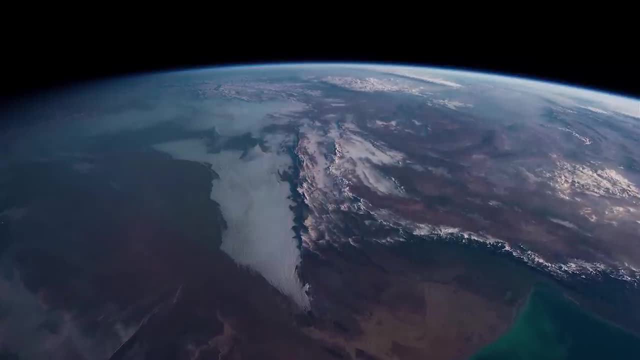 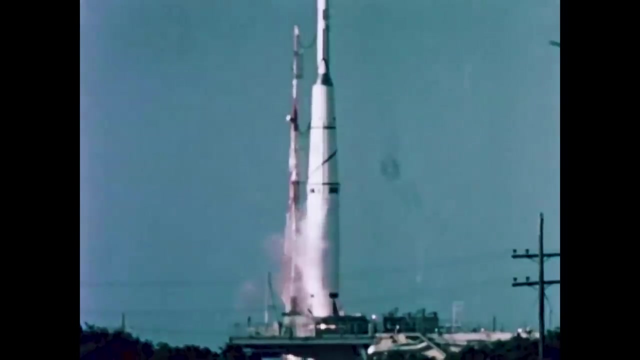 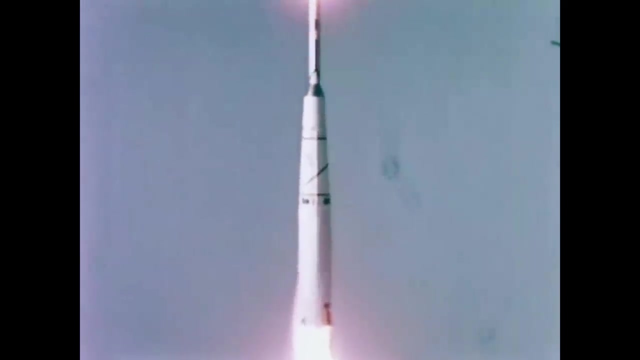 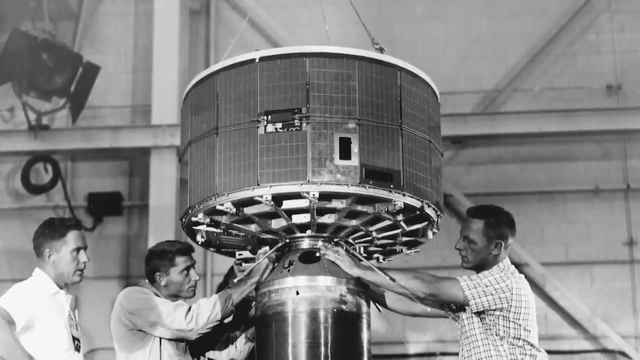 nudge could alter the climate. perhaps changes in co2 could as well. you scientists were realizing just how poorly they understood planet Earth at the beginning of the space age. scientists were keen to make weather observations from orbit. launched in 1960, Tyros one was the first weather. 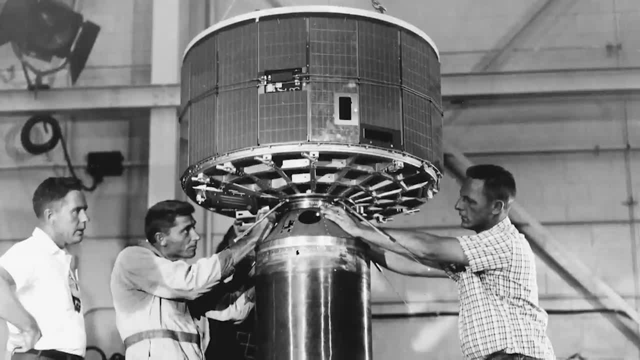 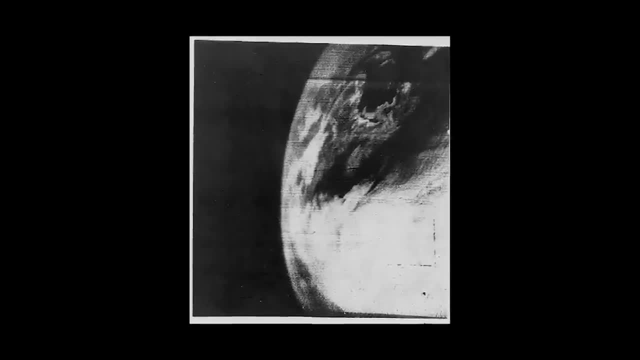 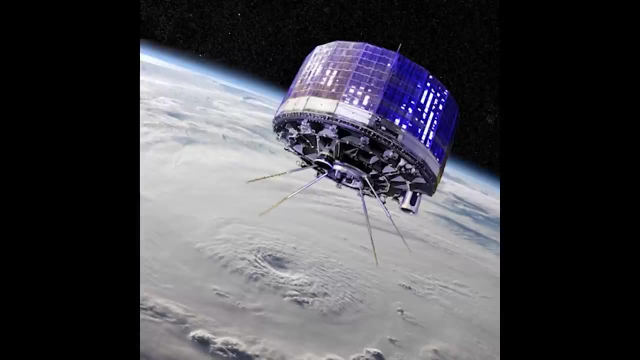 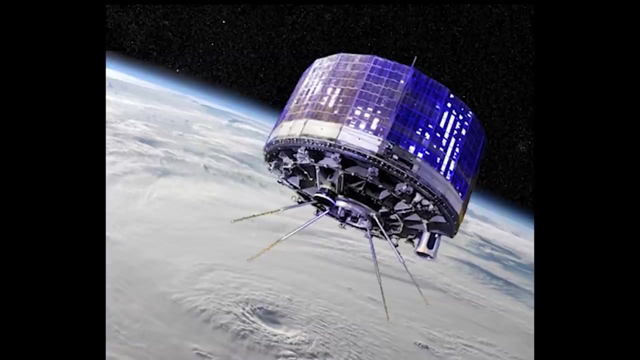 satellite. it was equipped with two TV cameras regularly transmitting images of global cloud patterns. It provided meteorologists with a unique view and it was followed by improved versions. Because these early satellites were in highly inclined low Earth orbits, the data gathered covered the whole planet and it was shared across the world. 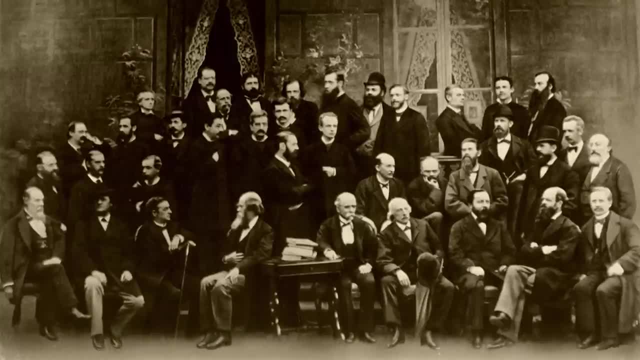 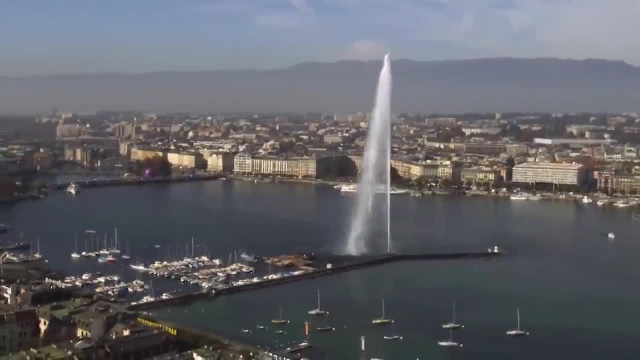 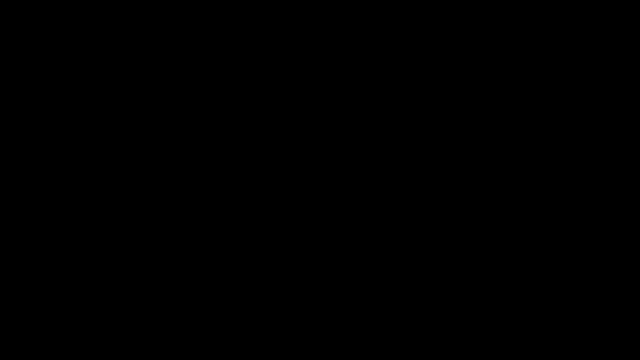 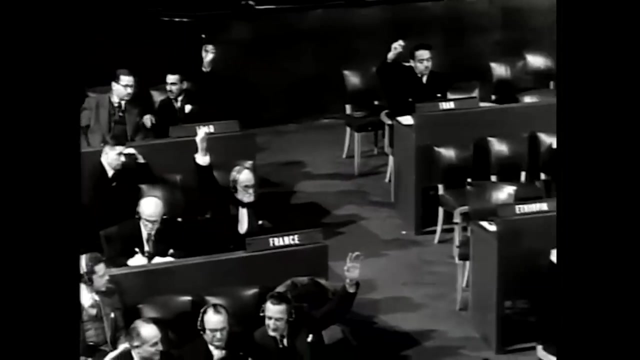 Since 1873, nations have been cooperating on weather prediction via the International Meteorological Organization, which in 1951 became the World Meteorological Organization, an arm of the United Nations headquartered in Geneva, With a UN resolution calling for international cooperation in the peaceful uses of outer. 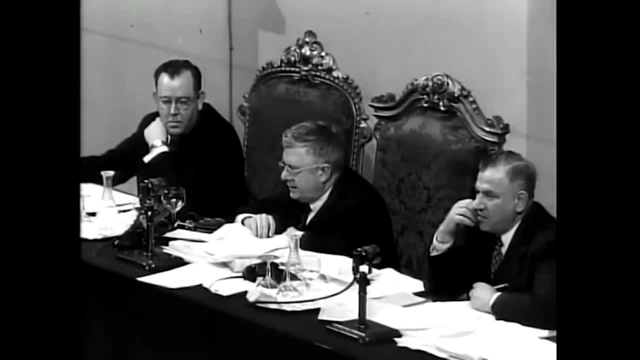 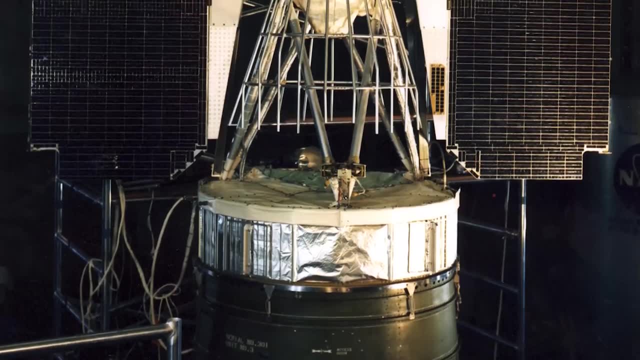 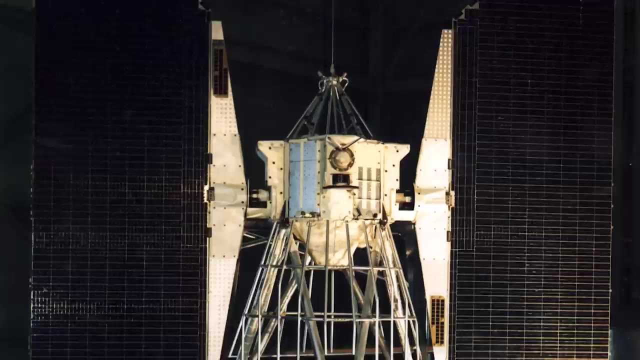 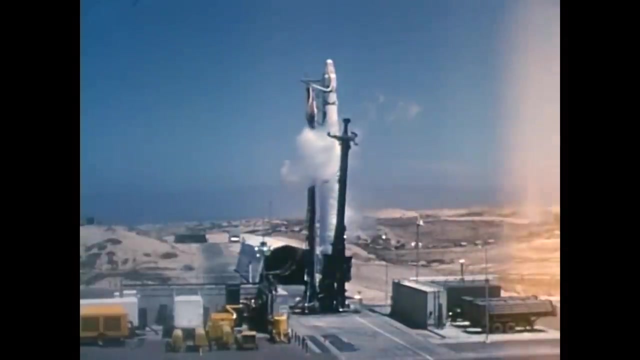 space weather satellites of different nations were soon being cooperated with by the United Nations, Coordinated for the benefit of all mankind. In 1964, the Nimbus program began. The series of seven satellites included a more sophisticated set of sensors. Nimbus was a test bed for new technologies and it gathered data about different areas. 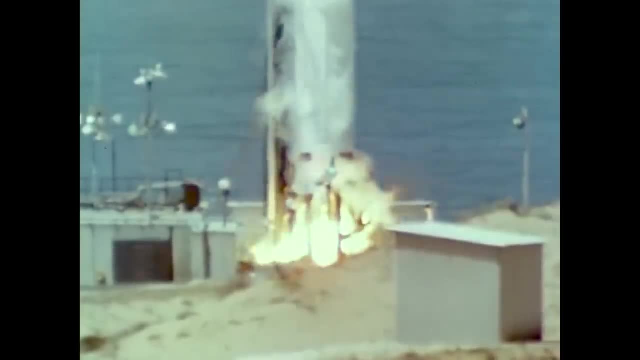 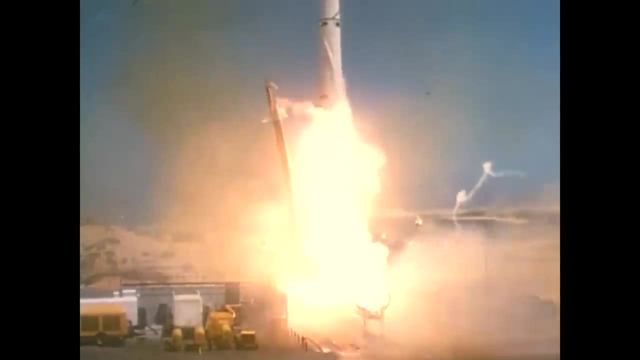 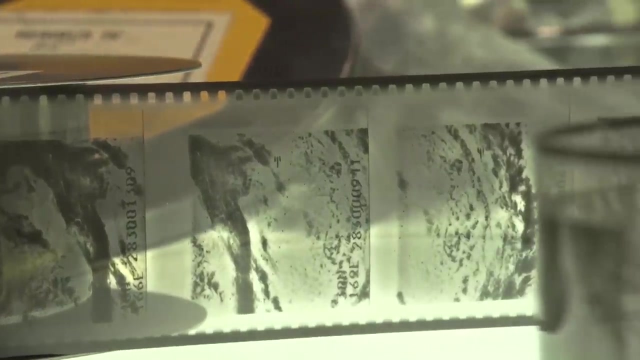 Along with cloud patterns was information about the atmosphere and sea ice. The Nimbus program was a pre-digital age and all electronic image data was burnt to and stored on 70mm film. Little thought was given to establishing an archive for future reference. 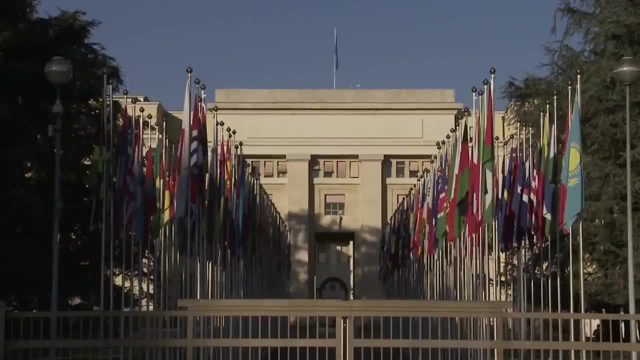 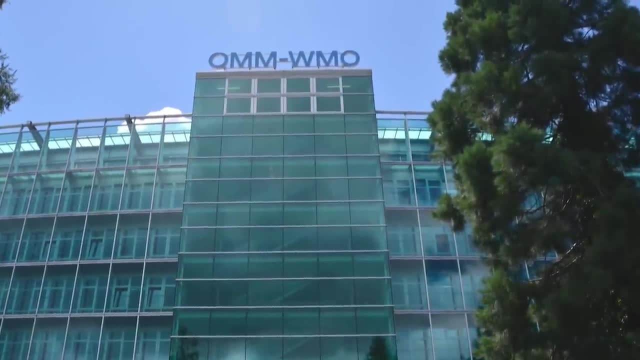 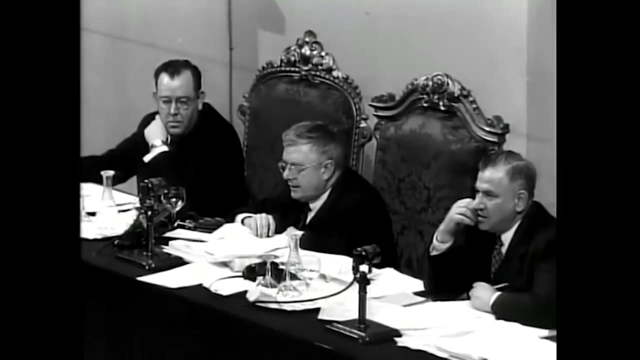 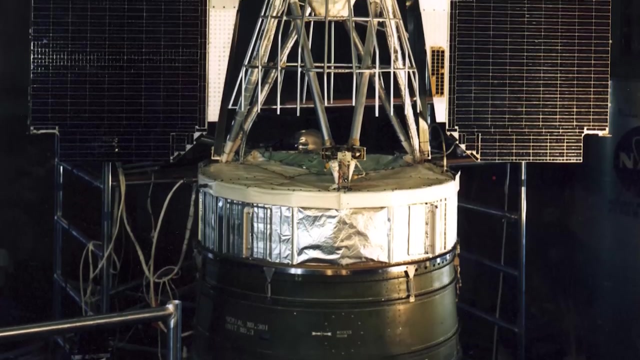 Space Agency, an arm of the United Nations headquartered in Geneva. With a UN resolution calling for international cooperation in the peaceful uses of outer space weather, satellites of different nations were soon being coordinated for the benefit of all mankind. In 1964, the Nimbus program began. 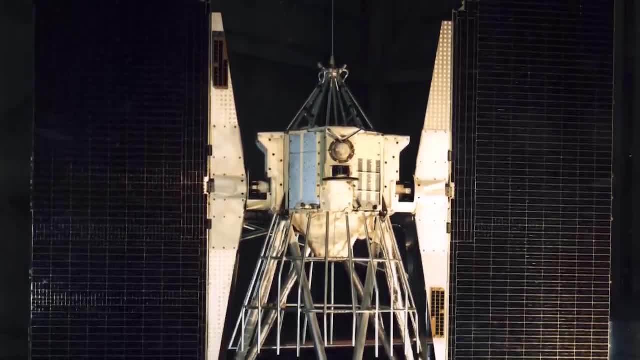 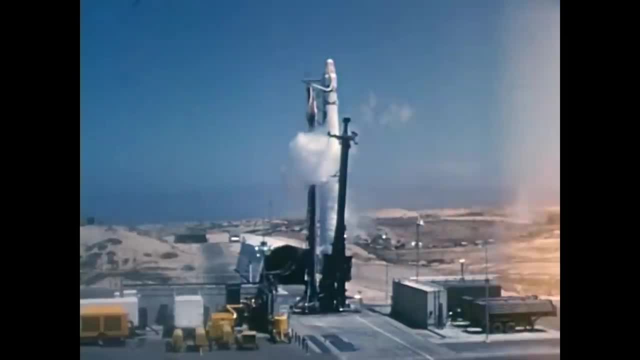 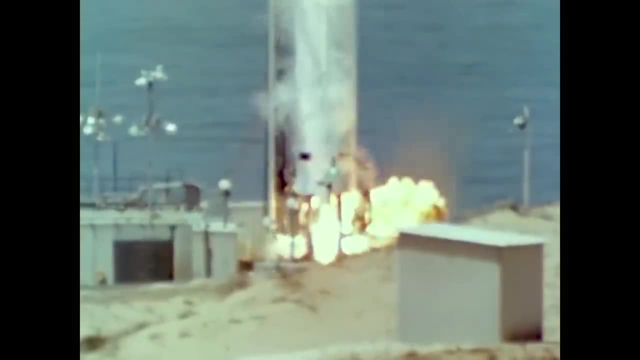 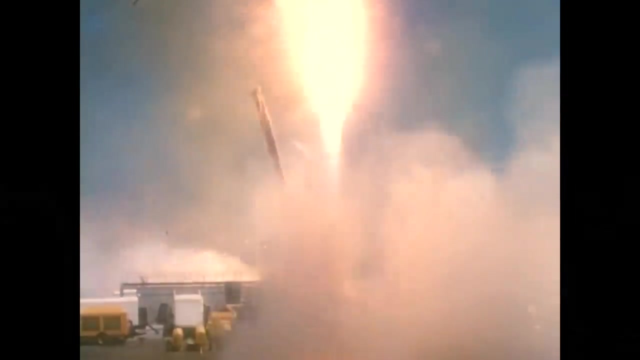 The series of seven satellites included a more sophisticated set of sensors. Nimbus was a test bed for new technologies, and it gathered data about different areas. Along with cloud patterns was information about the atmosphere and sea ice. This was the pre-digital age. 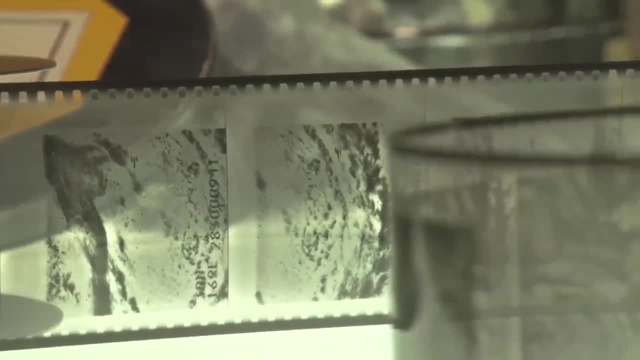 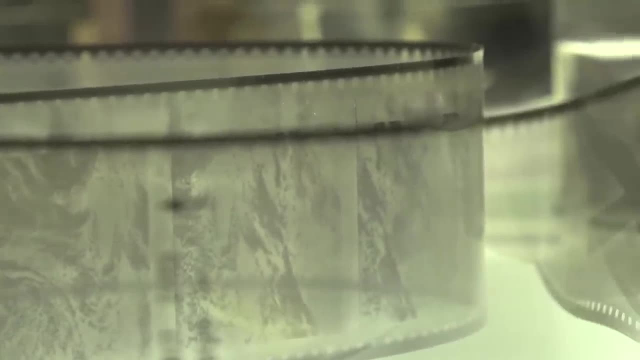 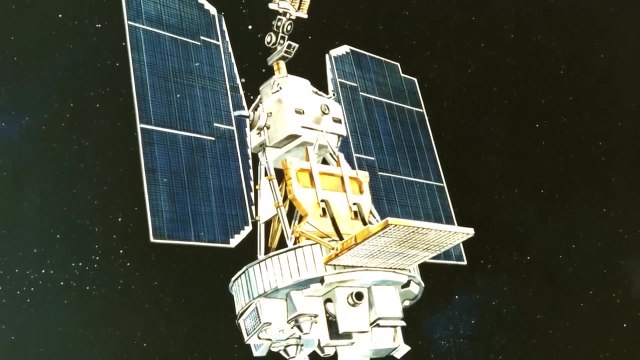 and all electronic image data was stored on 70mm film. Little thought was given to establishing an archive for future reference. The Nimbus program was an early example of Earth observation. rather than just a group of weather satellites, And meteorologists started seeing the planet. 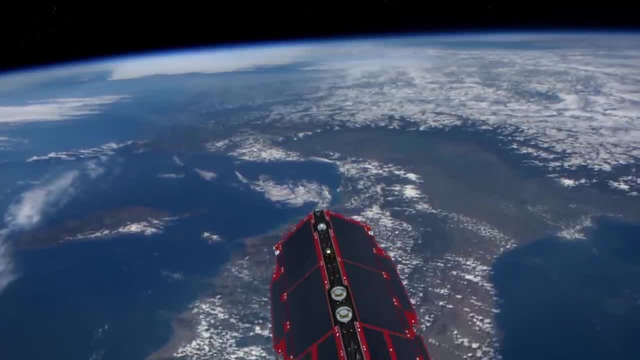 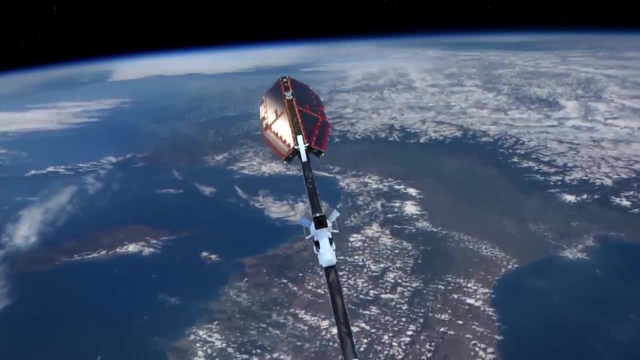 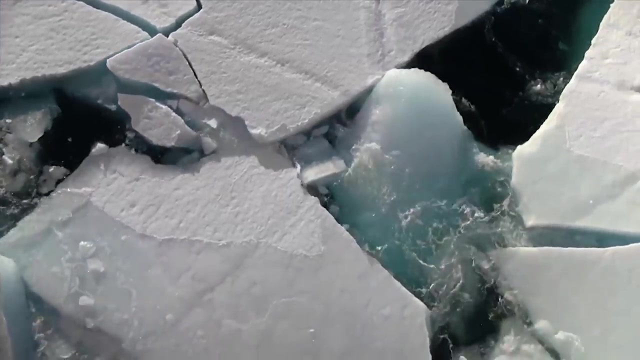 as a complex and interconnected system. Today, a fleet of satellites can see the Earth, the ice, the land and the biosphere. It is now understood that ice, particularly sea ice, plays an important role in the Earth's climate system. 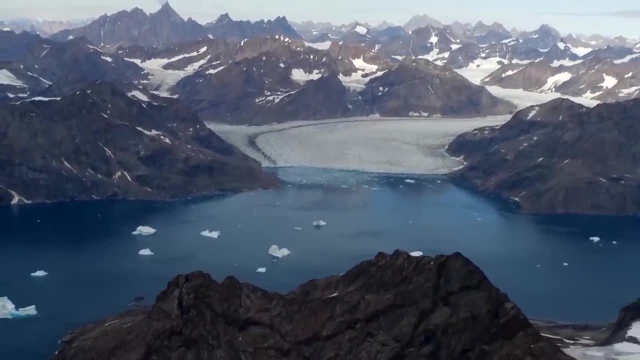 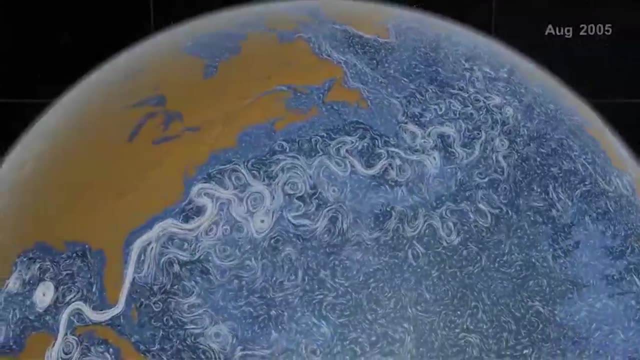 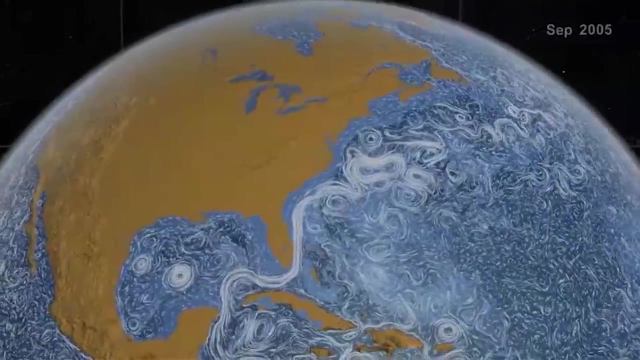 Polar ice slowly flows to the coasts where it melts, providing a source of cold water that drives the ocean currents responsible for the transfer of heat from the equatorial atmosphere. These currents also move nutrition, which is important for the survival of life. Global winds also circulate. 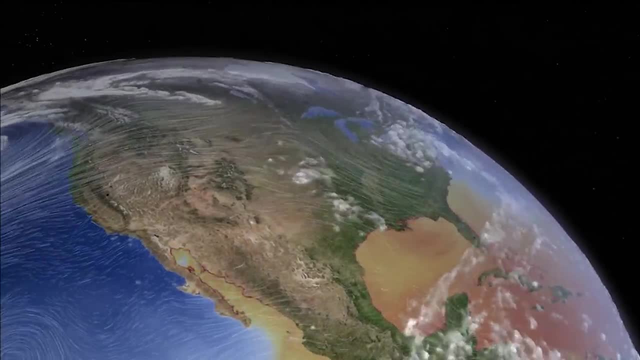 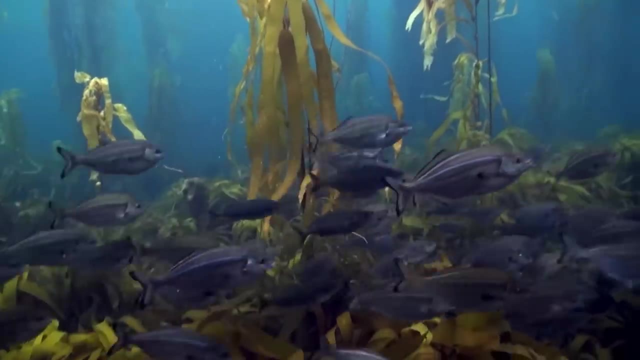 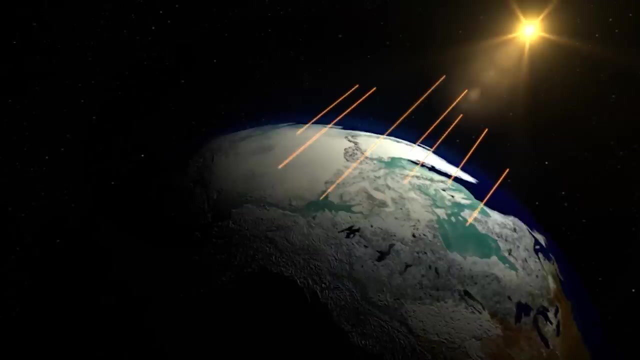 water via clouds, keeping the land moist and able to support vegetation. Plant life in both the oceans and the atmosphere removes CO2 from the air and replenishes the atmospheric oxygen. Both the ice, known as the cryosphere, and the clouds reflect a proportion of the sun's 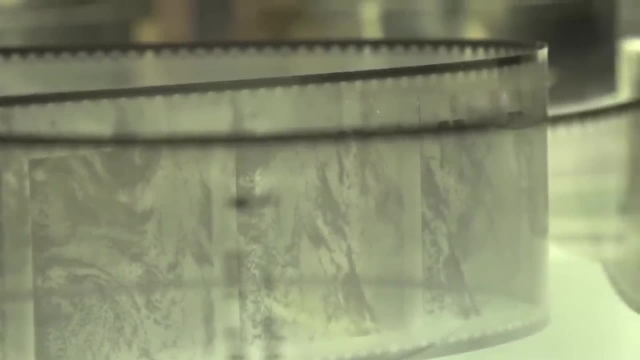 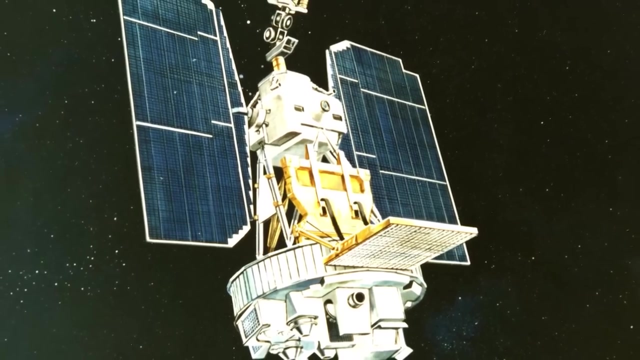 The Nimbus program was an early example of Earth observation. rather than just a group of weather satellites, A meteorologist started seeing the planet as a complex and interconnected space. The Nimbus program was the first in the world to be able to observe the Earth with a single. 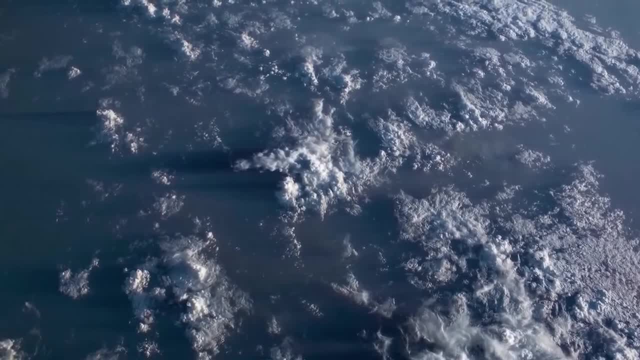 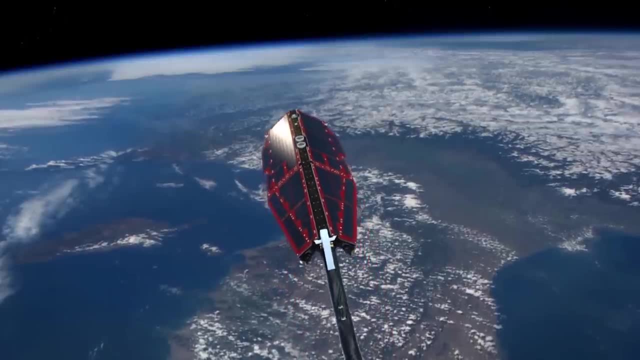 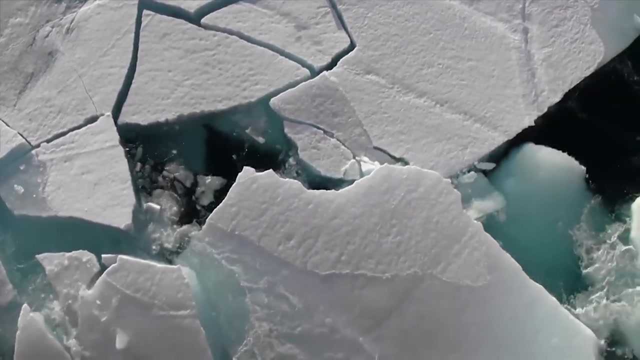 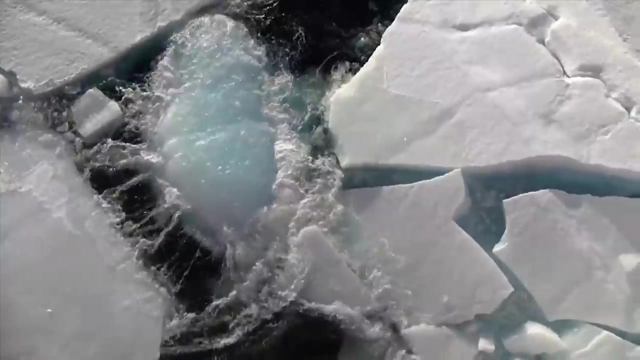 satellite system. today, a fleet of satellites is in operation, monitoring the atmosphere, the oceans, the ice, the land and the biosphere. it is now understood that ice, particularly sea ice, plays an important role in the Earth's climate system. polar ice slowly flows to the coasts, where it melts, providing a source of cold water. 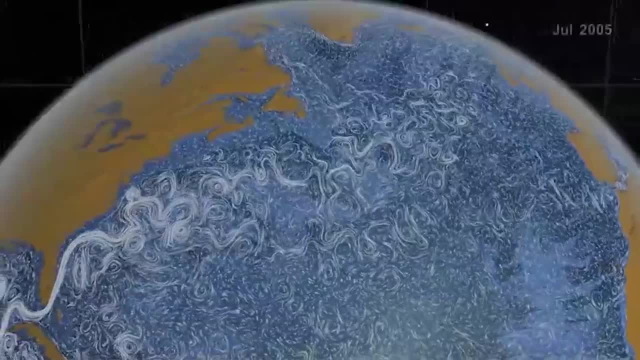 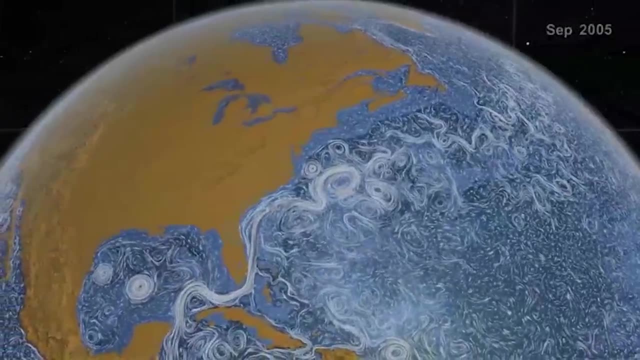 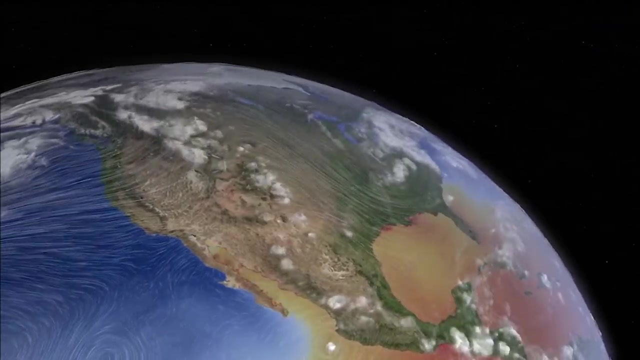 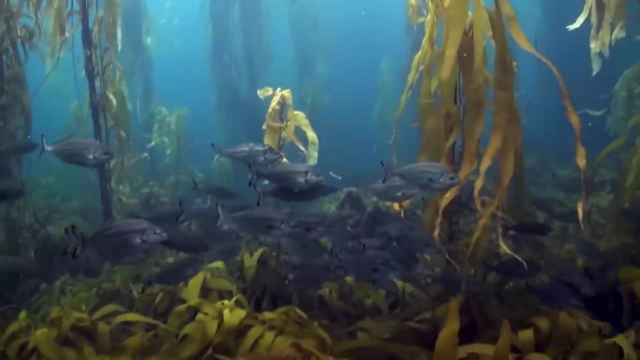 that drives the ocean currents responsible for the transfer of heat from the equatorial regions to the poles. these currents also move nutrition, which is important for the survival of life. global winds also circulate water via clouds, keeping the land moist and able to support vegetation. plant life in both the oceans and the 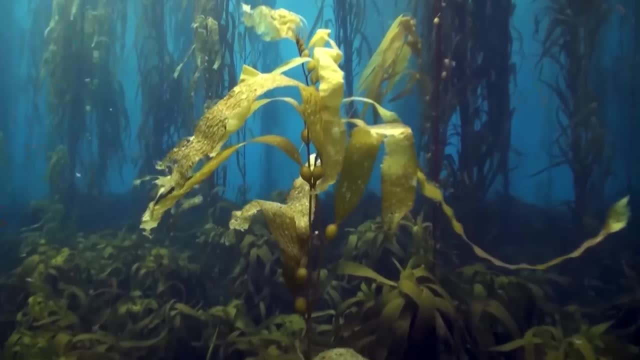 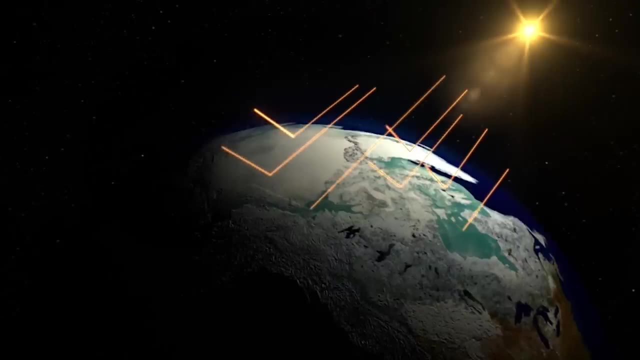 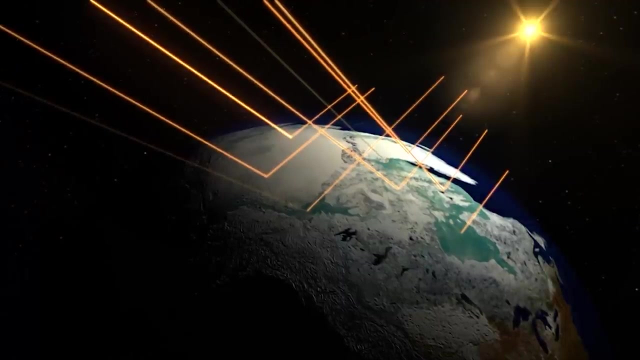 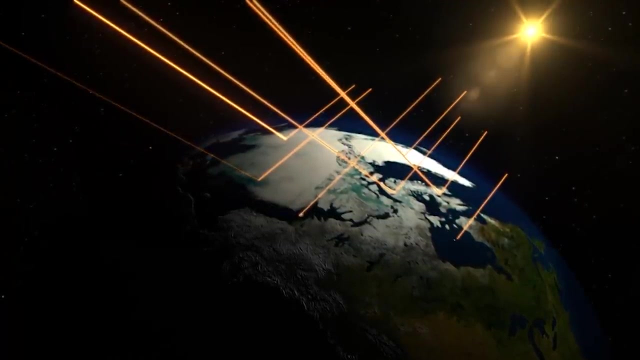 atmosphere, removes co2 from the air and replenishes the atmospheric oxygen. both the ice, known as the cryosphere, and the clouds reflect a proportion of the sun's energy back out into space. the extent of the ice and cloud cover are important factors in the Earth's energy budget. as ice melts, it exposes ocean or rock which 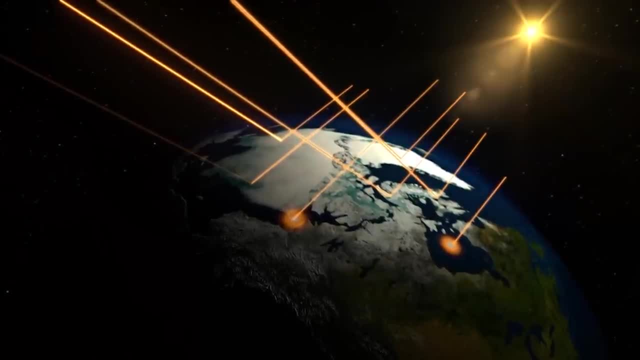 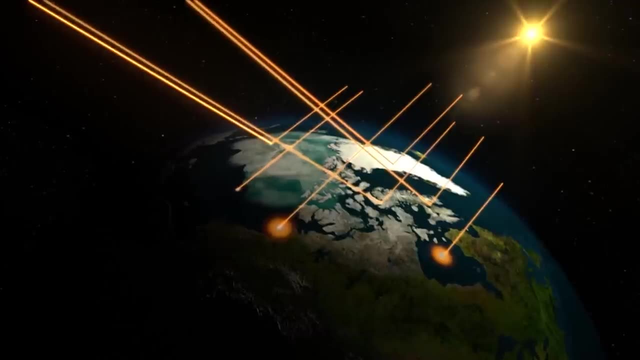 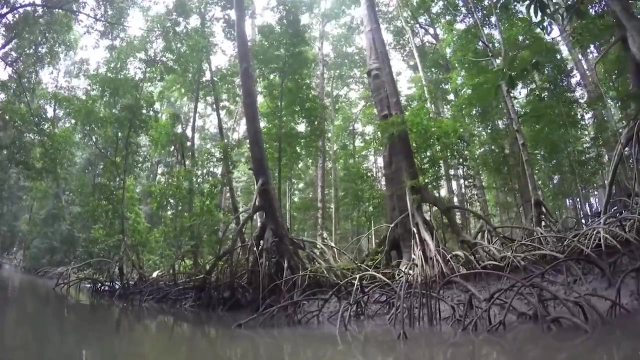 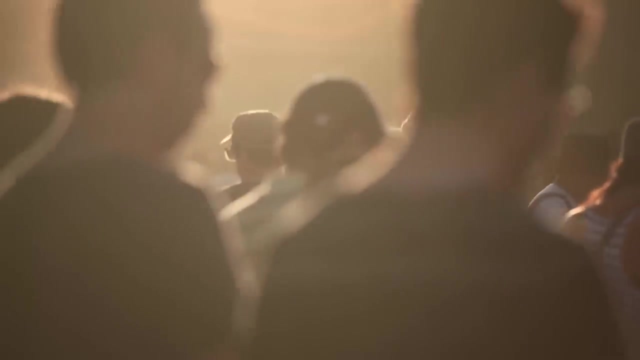 absorbs more solar energy. similarly, cloud cover or the absence of it will have an effect upon the land or sea beneath vegetation is also an important climate factor, as land plant pump huge amounts of water vapour into the atmosphere. but things are changing humanity simply through weight of. 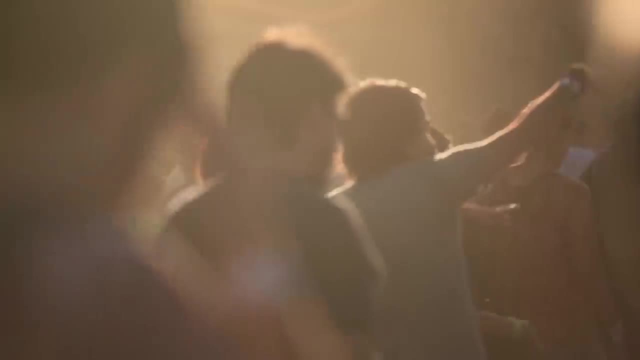 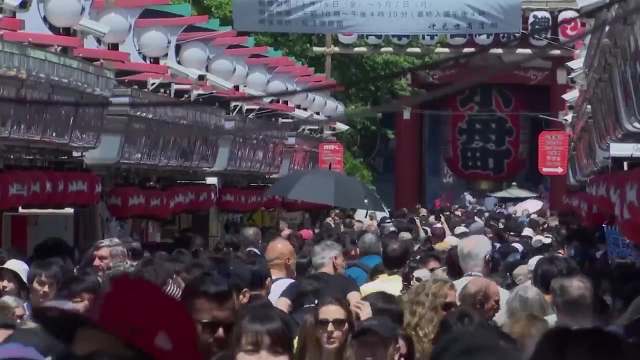 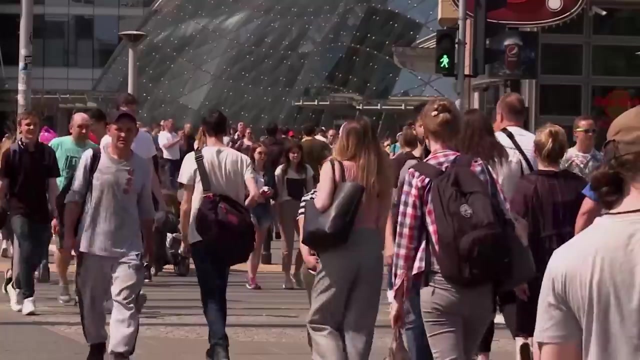 numbers is influencing key elements of the planet's climate system. in 50 years, the Earth's human population is resounding in an ever increasing form of from just over 3.5 billion to 7.7 billion. today, more people need more resources, and while there have been revolutions in agriculture and in 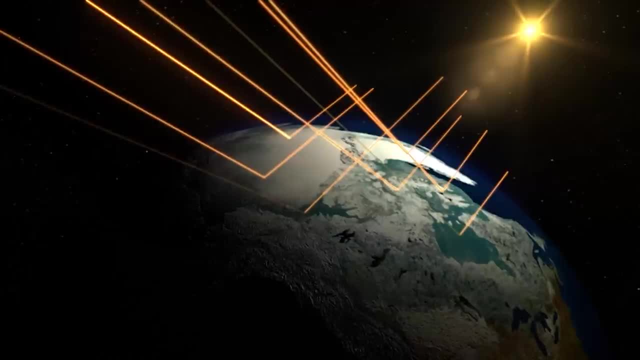 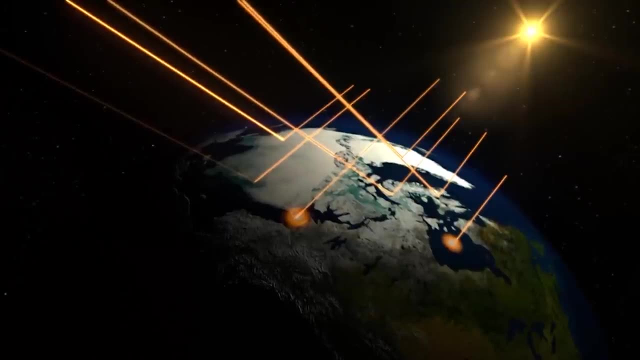 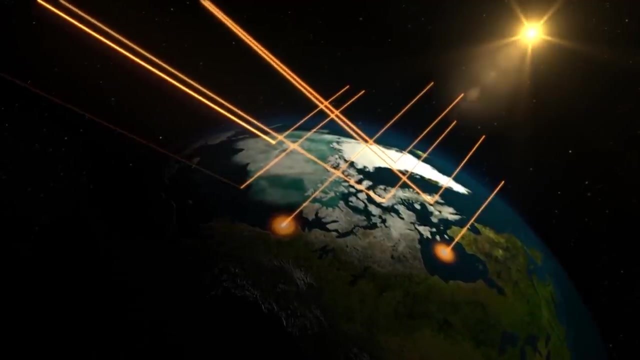 energy back out into space. The extent of the ice and cloud cover are important factors in the Earth's energy budget. As ice melts, it exposes ocean or rock, which absorbs more solar energy. Similarly, cloud cover, or the absence of it. 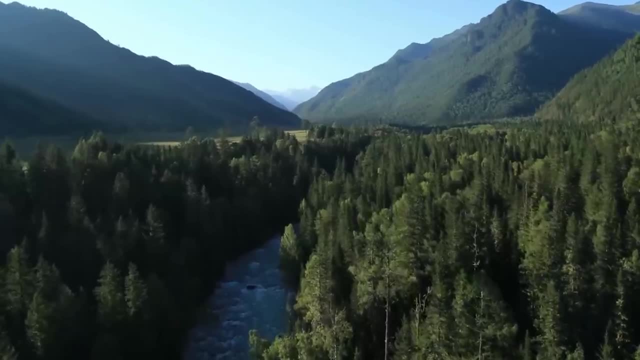 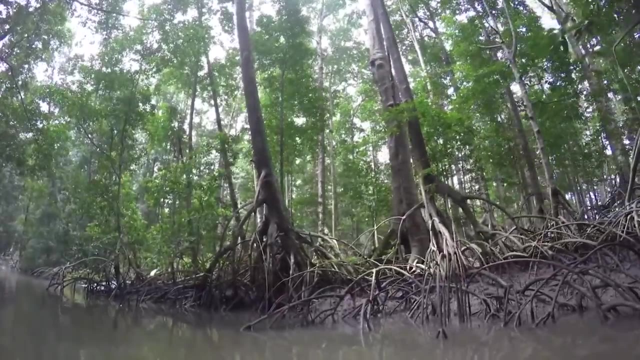 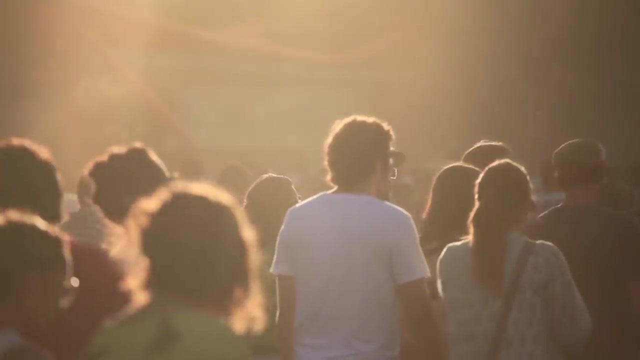 will have an effect upon the land or sea beneath. Vegetation is also an important climate factor which will pump huge amounts of water vapor into the atmosphere. But things are changing. Humanity, simply through weight of numbers, is influencing key elements of the planet's climate system. 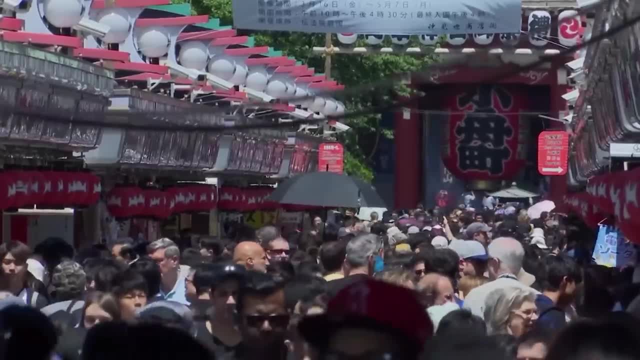 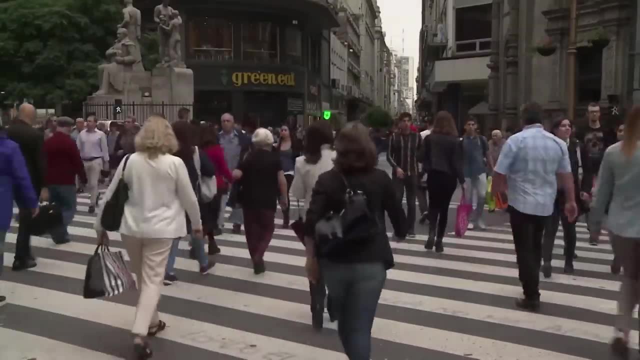 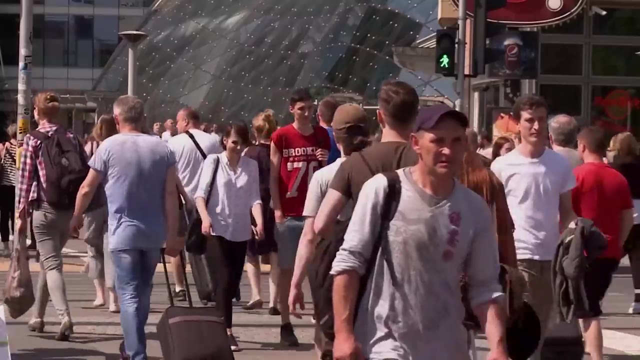 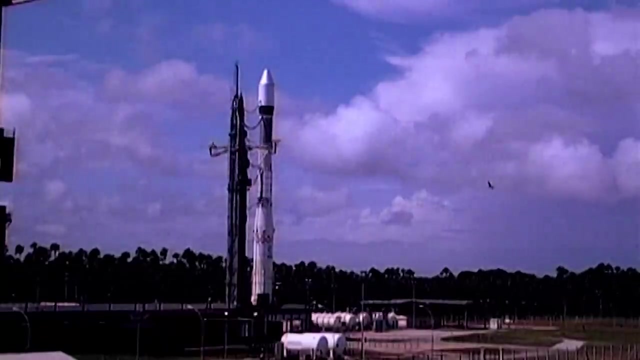 In 50 years, the Earth's human population has risen from just over 3.5 billion to 7.7 billion. today, More people need more resources. While there have been revolutions in agriculture and in technology, the Earth's reserves are not limitless. 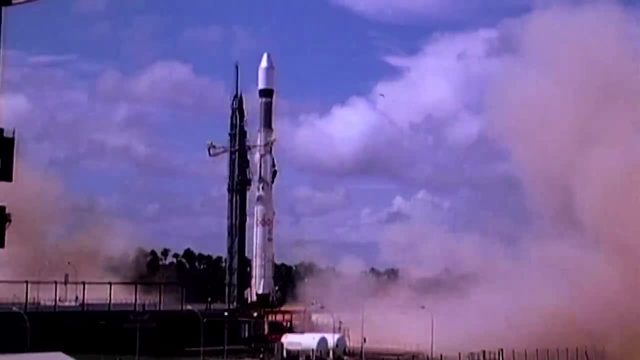 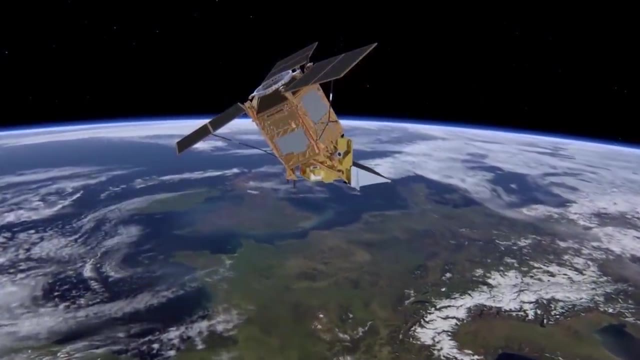 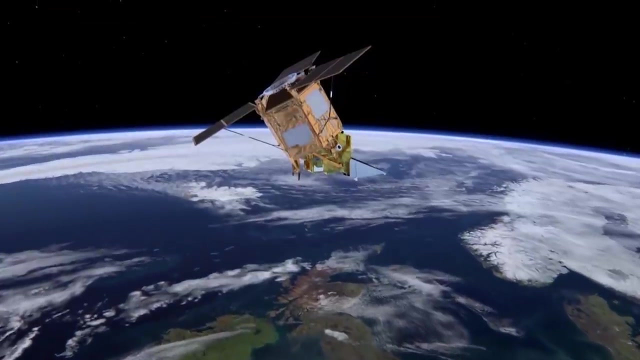 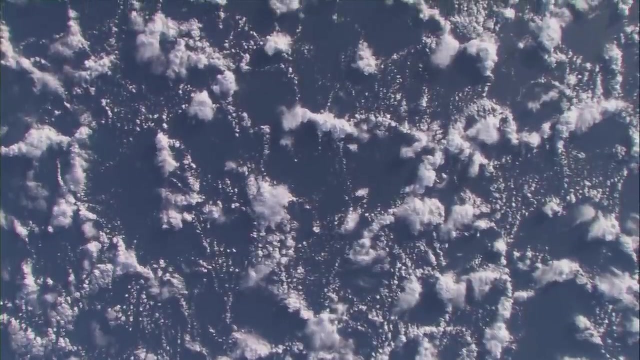 In 1979, Europe began launching spacecraft, And while the new Earth observation satellites were revealing changes, scientists were reluctant to reach conclusions about long-term trends. The Earth's climate system is still in its climate cycle, And though climate science knew about the steady rise, 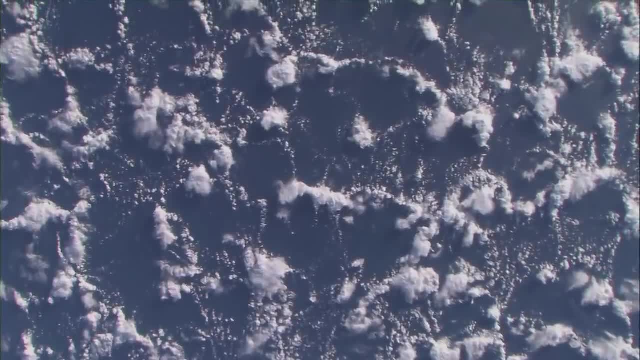 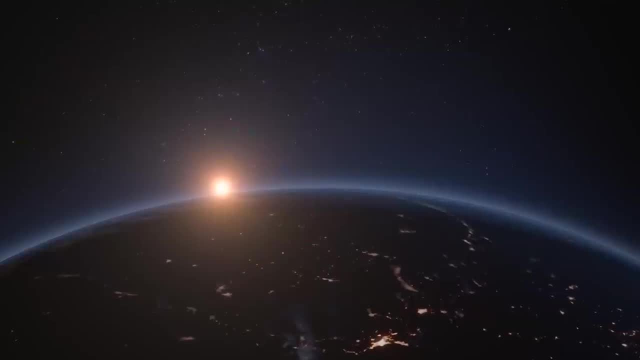 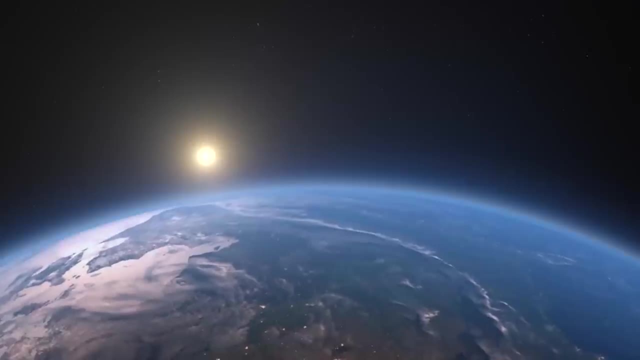 in atmospheric CO2 revealed by the Keeling curve. researchers were looking for additional solid evidence that change caused by human activity was happening. Since 1913, spectroscopy had revealed that a layer of ozone in the stratosphere was reaching the ground. 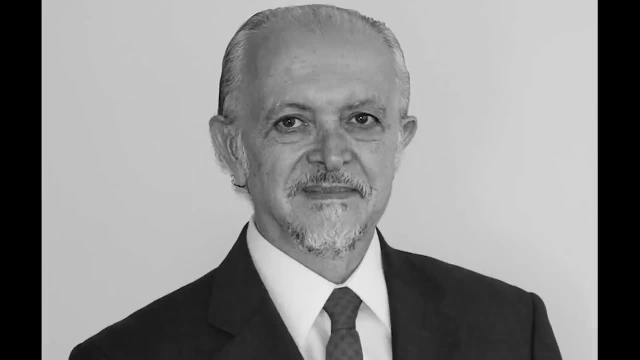 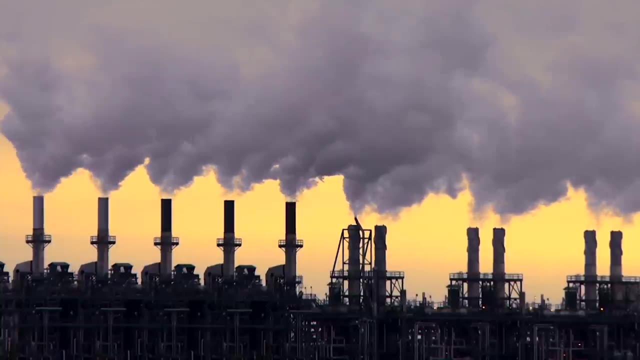 In 1974, Mario Molina, a postdoctoral fellow working on hot atom chemistry, published a paper suggesting that the family of industrial chemicals known as chlorofluorocarbons or CFCs could damage the ozone layer. 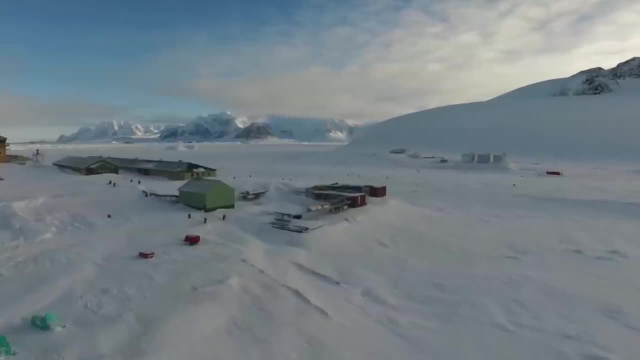 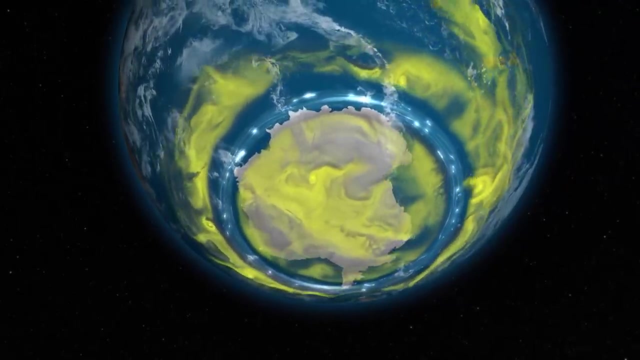 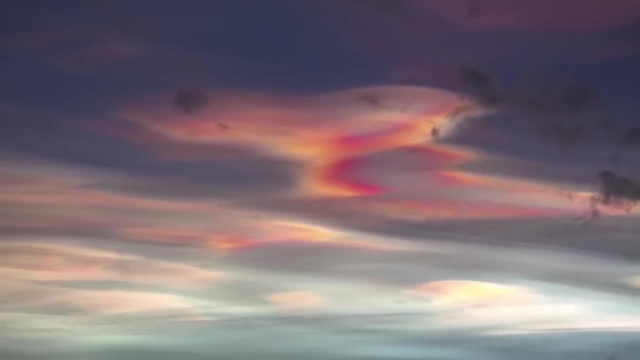 In the 1980s, meteorologists working in Antarctica found the evidence. The polar vortex above the southern continent concentrates on the stratosphere. Mother-of-pearl clouds in the polar skies contain ice crystals which, in combination with ultraviolet 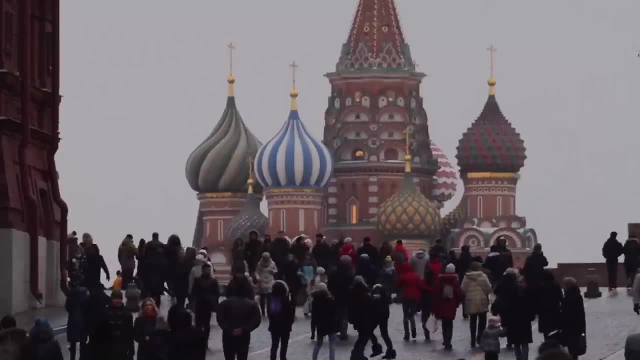 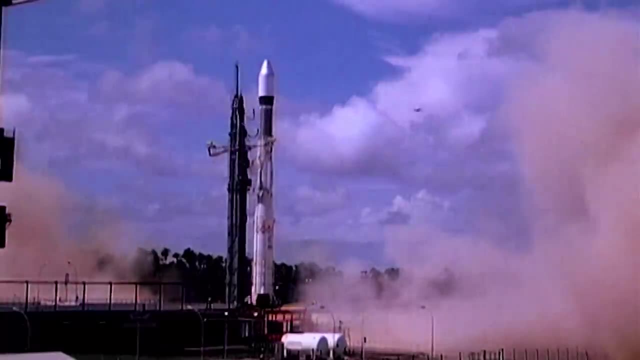 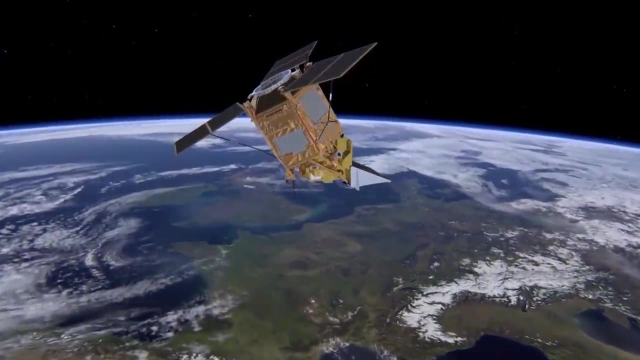 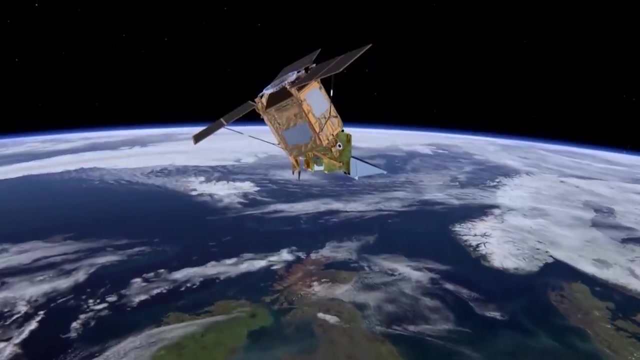 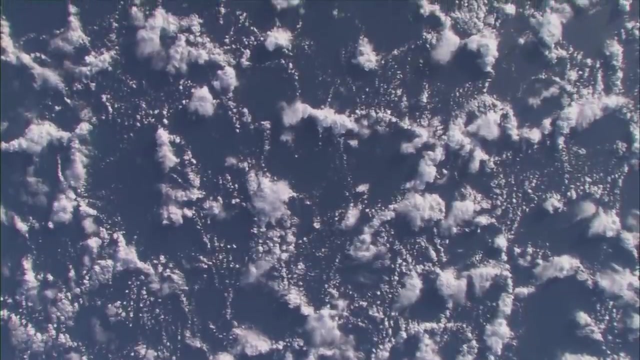 technology. the Earth's reserves are not limitless. in 1979, Europe began launching spacecraft, and while the new Earth observation satellites were revealing changes, scientists were reluctant to reach conclusions about long-term trends. they understood that there was a certain amount of variability in the planet's climate cycle, and though climate science knew about the steady rise in atmospheric 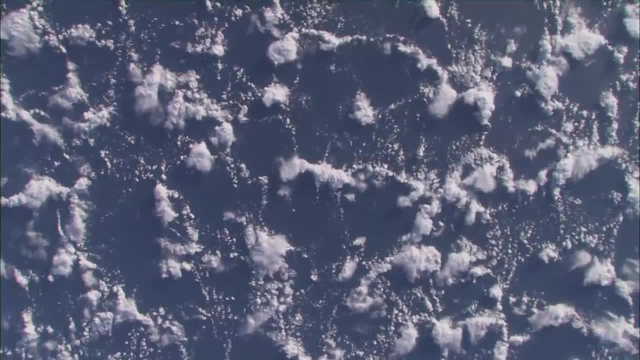 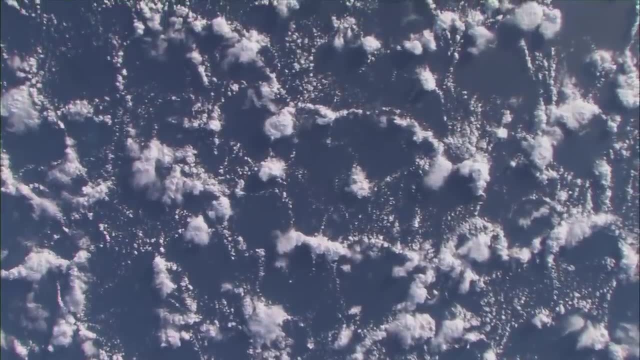 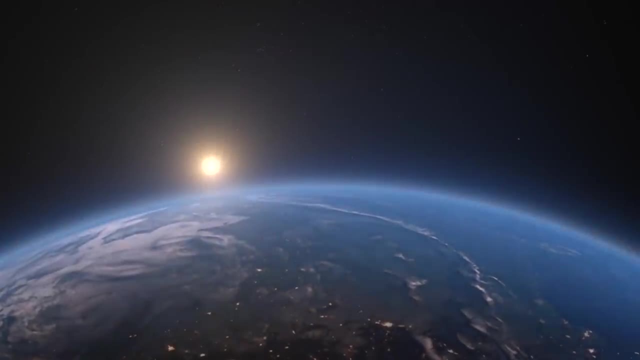 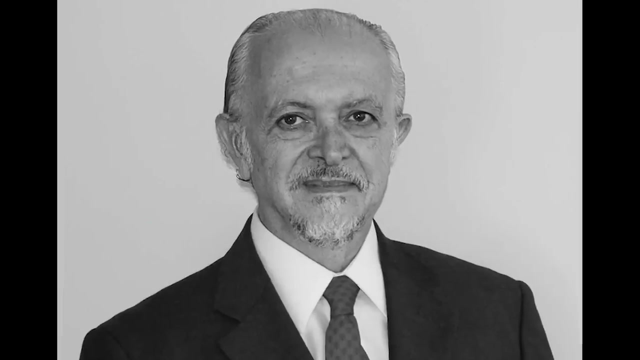 co2 revealed by the Keeling curve. researchers were looking for additional solid evidence that change caused by human activity was happening. since 1913, spectroscopy had revealed that a layer of ozone in the stratosphere blocked harmful UV sunlight from reaching the ground. in 1974, Mario Molina, a 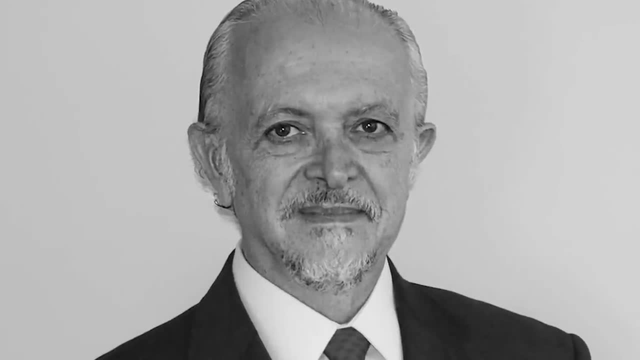 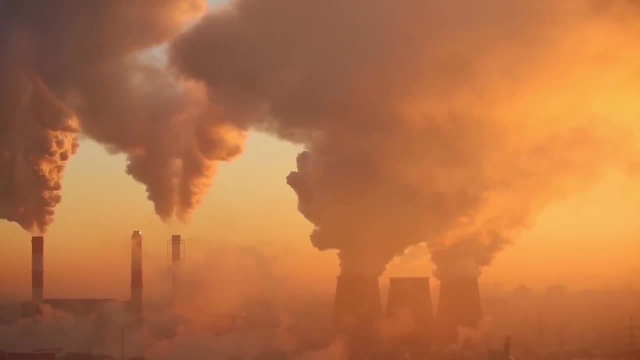 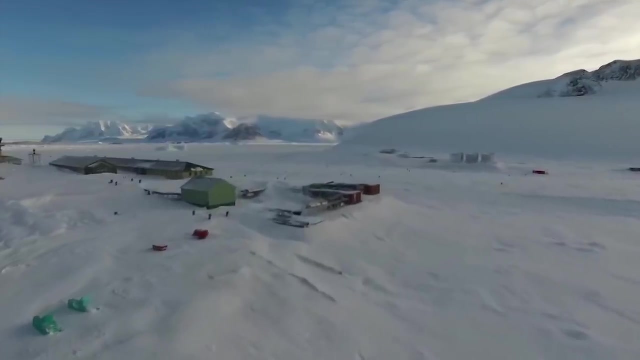 postdoctoral fellow working on hot atom chemistry published a paper suggesting that the family of industrial chemicals known as chlorofluorocarbons or CFC's could damage the ozone layer. in the 1980s, meteorologists working in Antarctica found the evidence: the polar vortex above the southern continent. 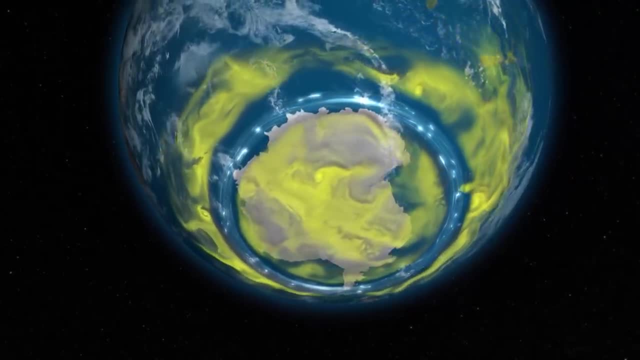 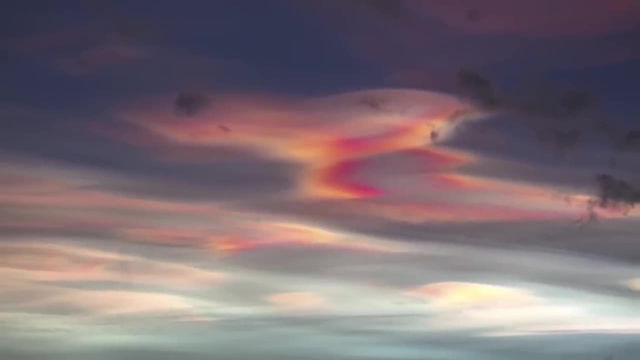 concentrates the CFC's in the stratosphere. mother-of-pearl clouds in the polar skies contain ice crystals which, in combination with ultraviolet, split chlorine from the CFC molecule. each chlorine atom is called the ZOXwh Göring media vị phytosanitet hiện. 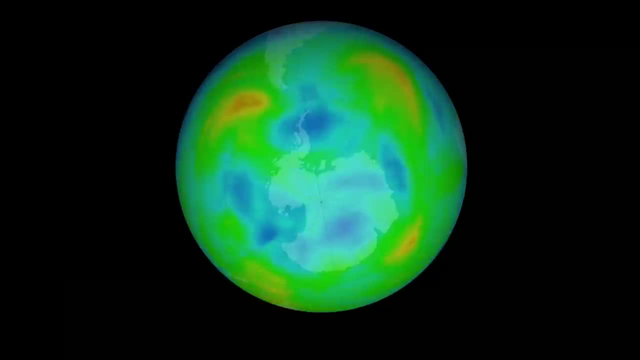 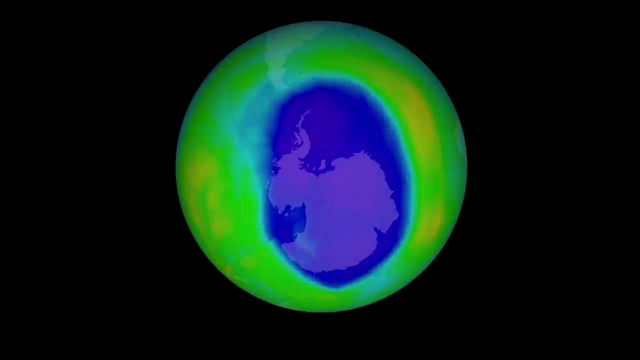 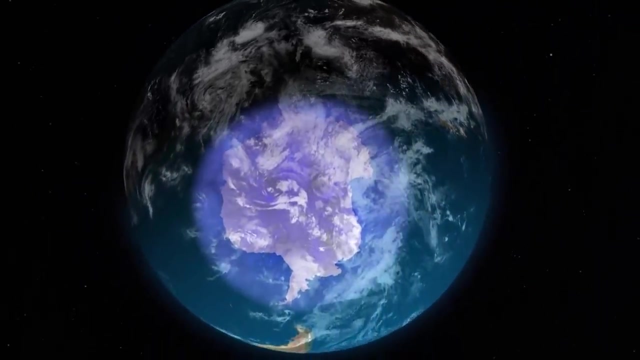 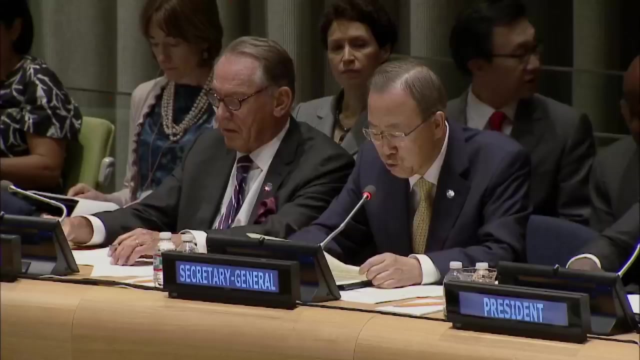 molecule. each chlorine atom can break down over 100 000 ozone molecules. a large area centered over antarctica showed almost no ozone. it became known as the hole in the ozone layer. the united nations began talks aimed at limiting the production of cfcs and, in 1989, an international 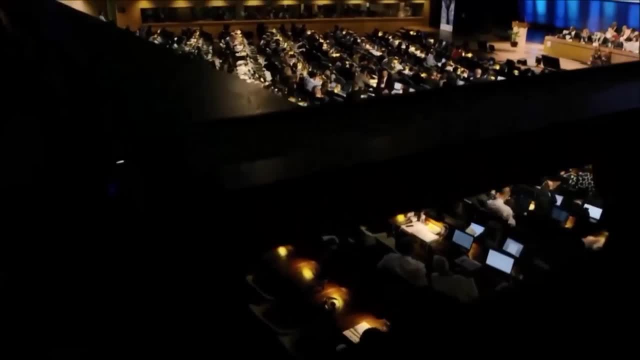 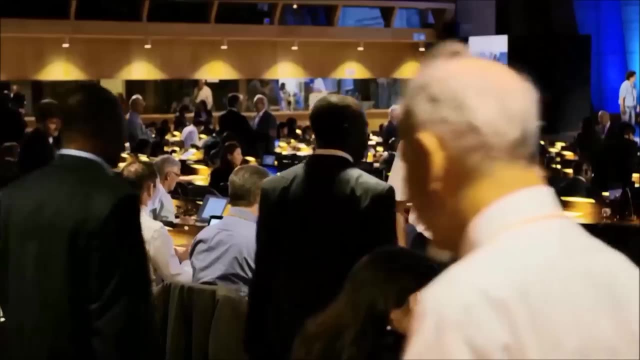 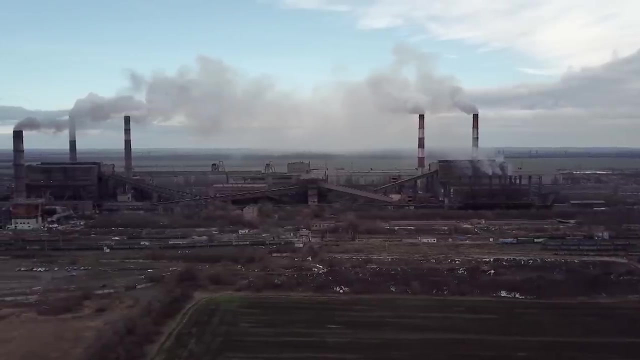 treaty, known as the montreal protocol, capped the production of cfcs and ultimately resulted in a 10-year phase-out of cfc production. all countries signed the agreement and the montreal protocol is seen as a model of international cooperation in the 1980s. an upward trend in global temperature. 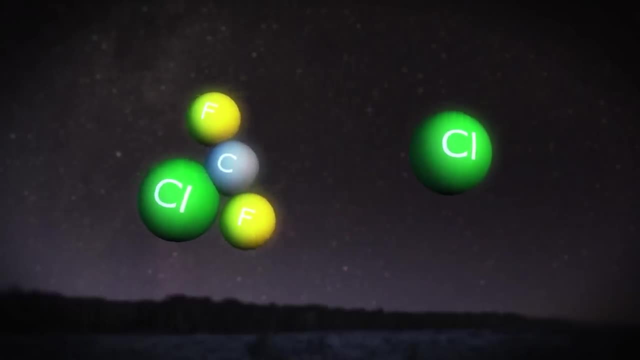 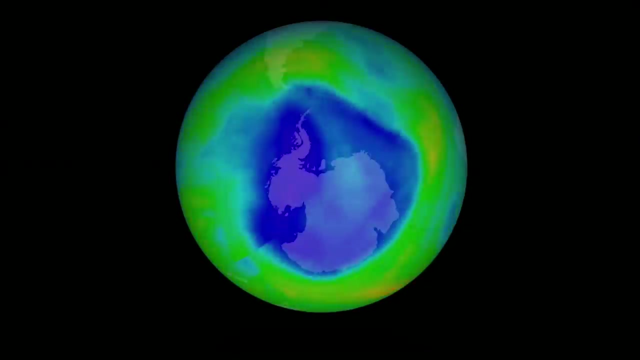 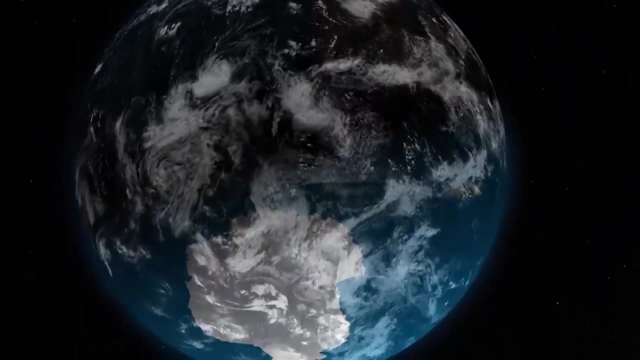 split chlorine from the CFC molecule. Each chlorine atom can break down over 100,000 ozone molecules. A large area centered over Antarctica showed almost no ozone. It became known as the hole in the ozone layer. The United Nations began talks aimed at limiting the production. of CFCs and in 1989, an international treaty known as the Montreal Protocol capped the production of CFCs and ultimately resulted in a ten-year phase-out of CFC production. All countries signed the agreement and the Montreal Protocol is seen as a model. 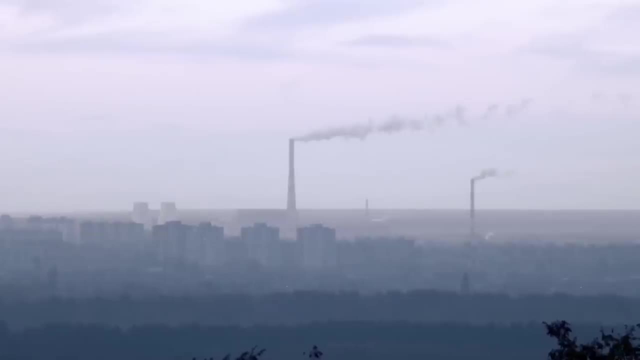 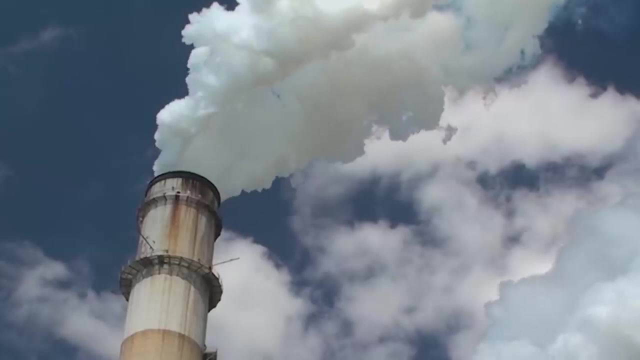 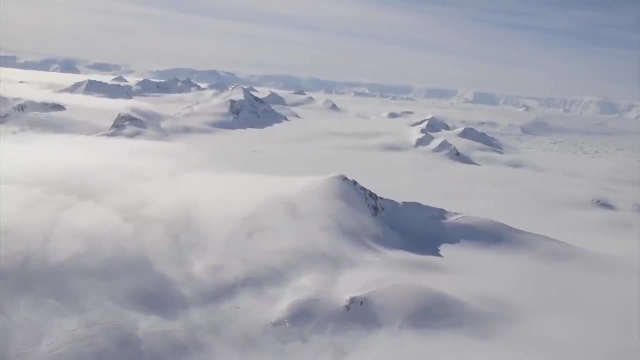 of international cooperation. In the 1980s, an upward trend in global temperature averages and a scientific consensus emerged that the burning of fossil fuels was altering the balance of gases in the atmosphere. Most of our planet's fresh water is locked in the polar ice caps. 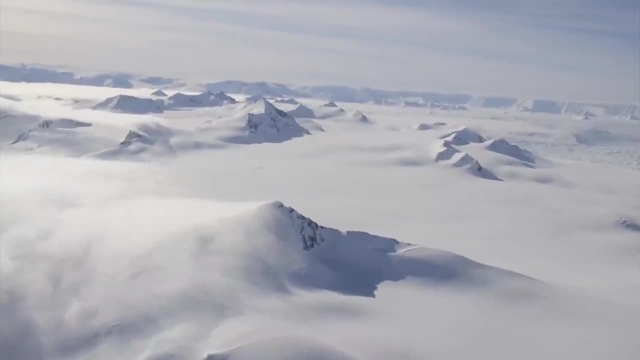 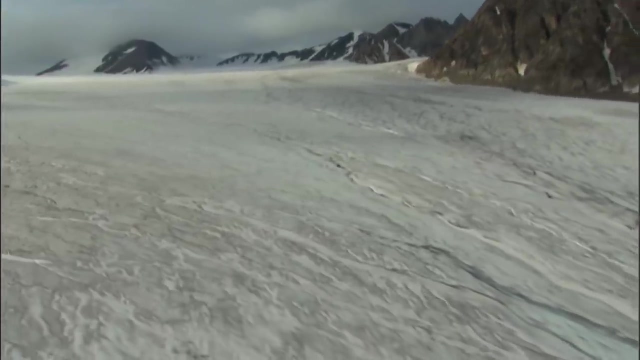 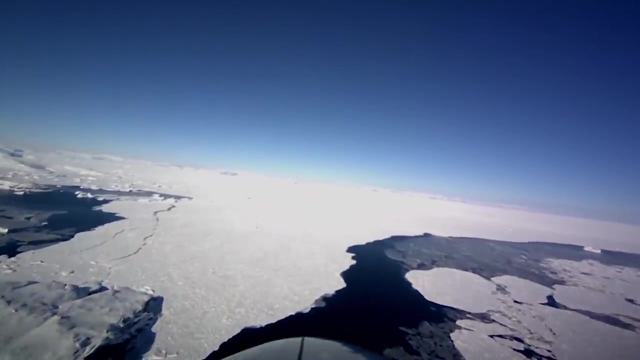 61% of this ice covers the Antarctic continent. In the north Greenland is also covered by an ice sheet. There is no land mass at the North Pole, but a large area of sea. ice grows and shrinks with the sea during the winter seasons. 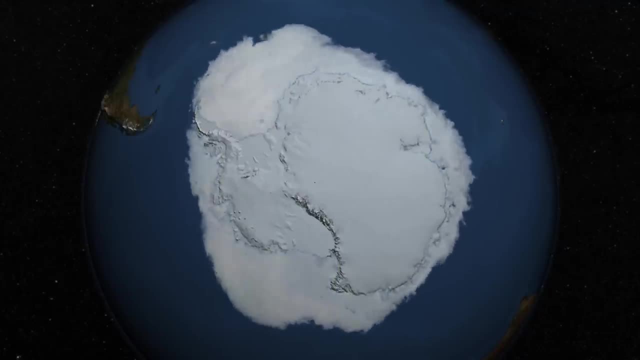 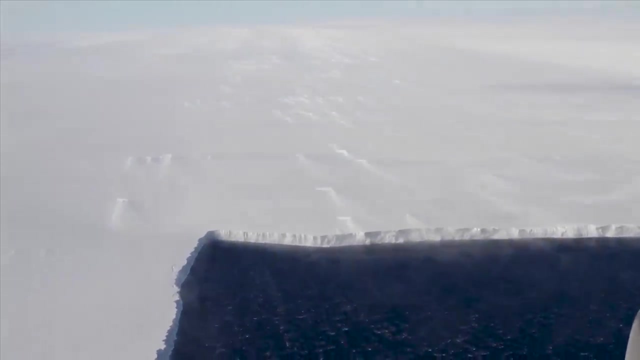 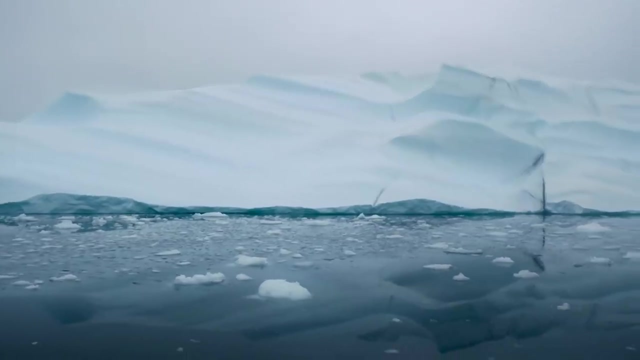 Seasonal sea ice also fringes Greenland and Antarctica. Ice shelves are a third manifestation of polar ice. These are thick layers of ice that extend into the ocean from the mouths of glaciers. Periodically, icebergs will break away from these regions. 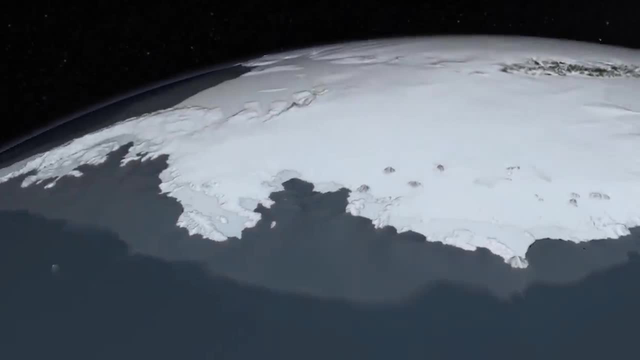 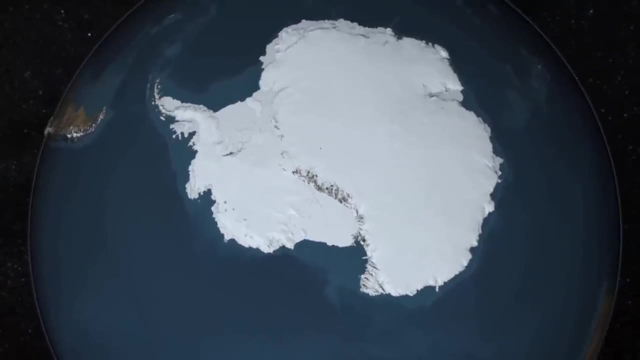 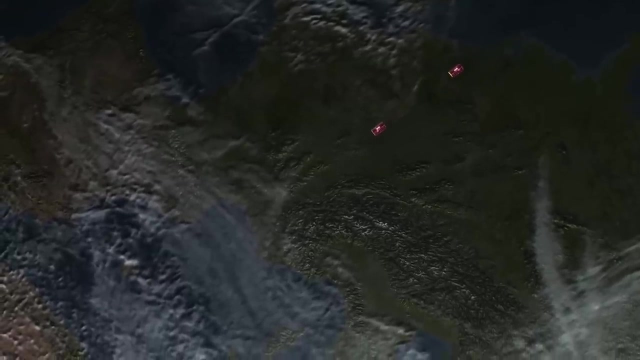 These areas are important to the circulation of global winds and ocean currents. NASA has tracked the prevalence of water in general and ice in particular via the GRACE satellites, which were recently replaced by a similar pair of GRACE follow-on satellites. The two follow the same orbit. 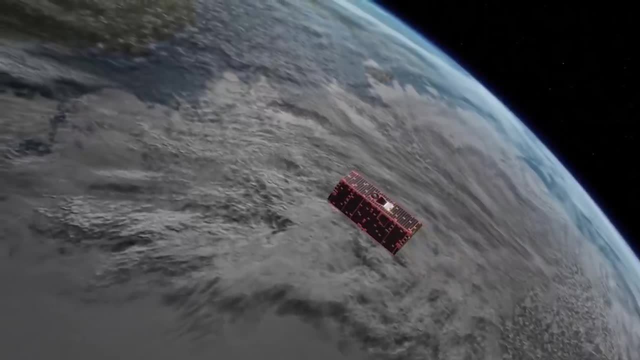 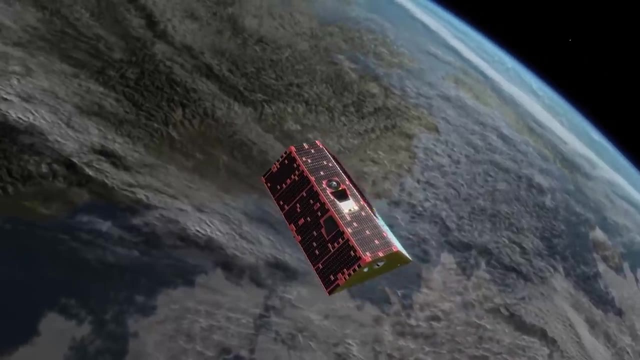 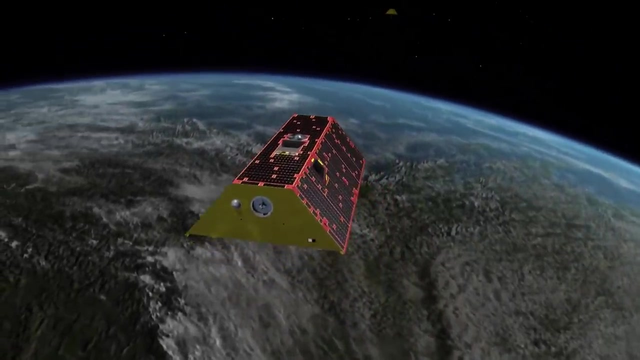 and minute. changes in the Earth's gravitational field will cause them to change speed, with a variation in the distance between them. This data is accurately measured, so researchers can record changes due to variations in groundwater or in ice thickness During the life of the first. 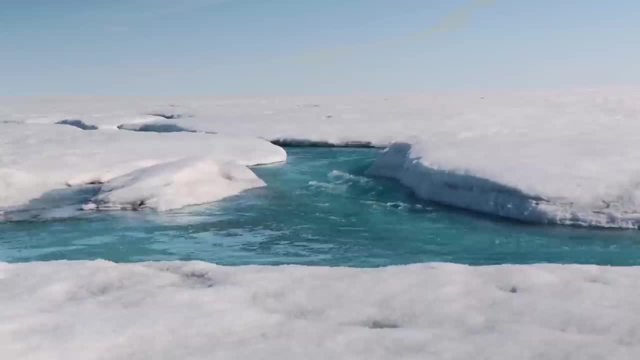 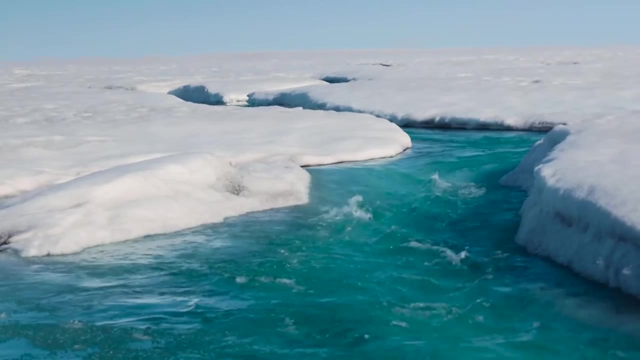 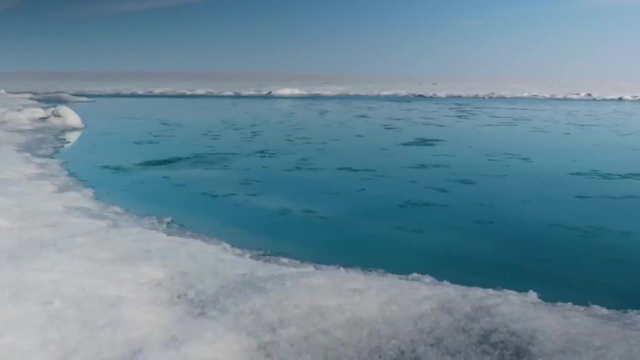 GRACE mission, Greenland lost 285 gigatons of ice per year On average. Antarctica lost 137 gigatons per year From 2005 to 2016,. sea levels rose by 3.7 centimeters due to melting ice sheets. 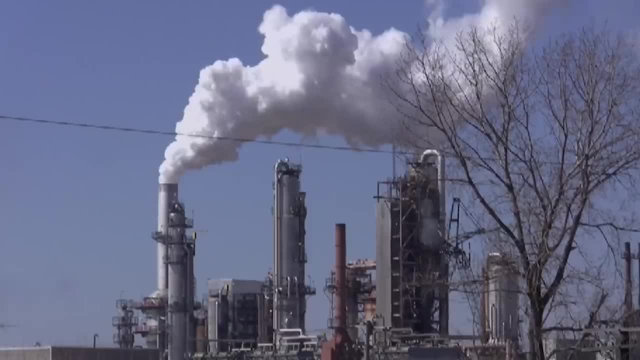 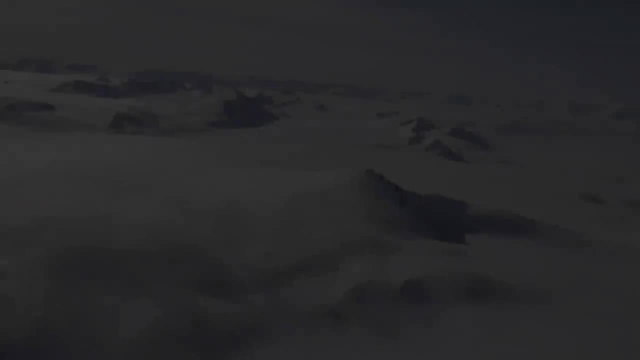 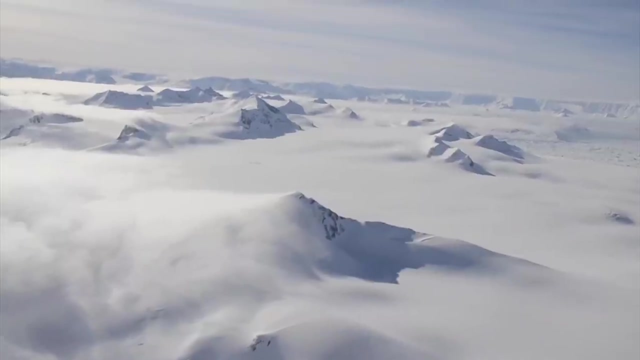 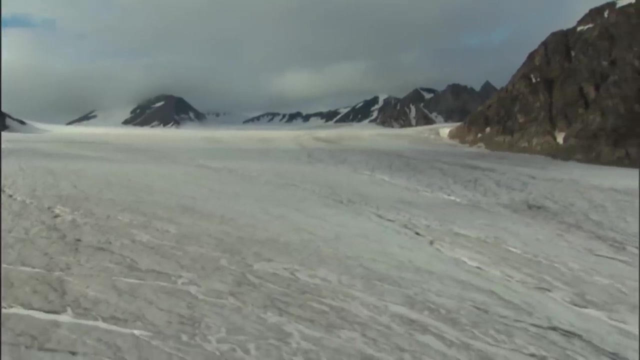 averages was becoming clear and a scientific consensus emerged that the burning of fossil fuels was altering the balance of gases in the atmosphere. most of our planet's fresh water is locked in the polar ice caps. 61 of this ice covers the antarctic continent. in the north greenland is also covered by an ice sheet. there is no landmass at the north. 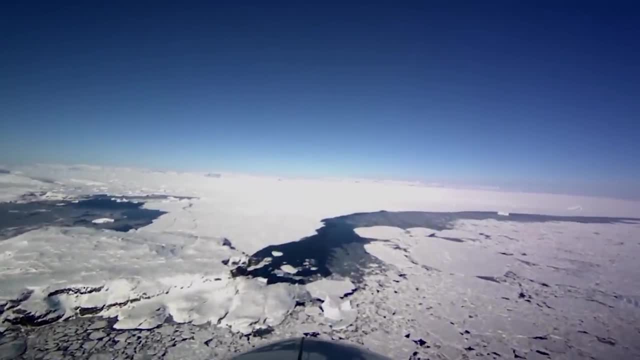 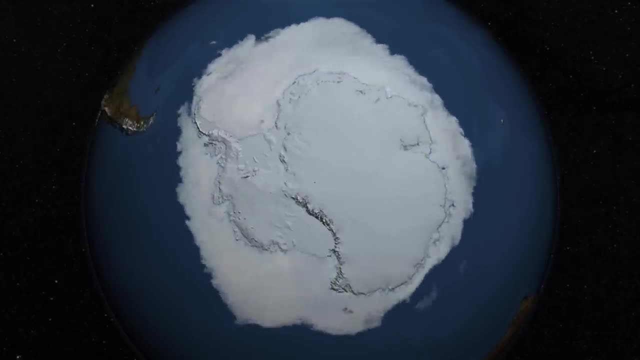 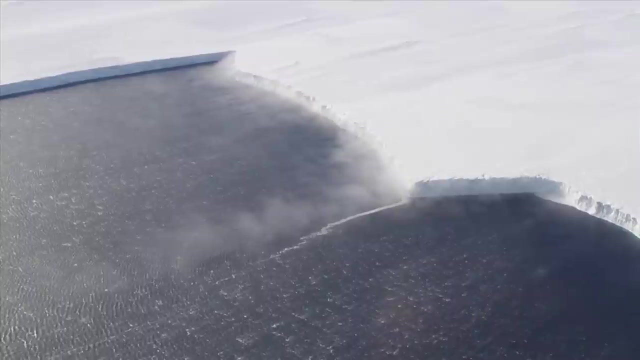 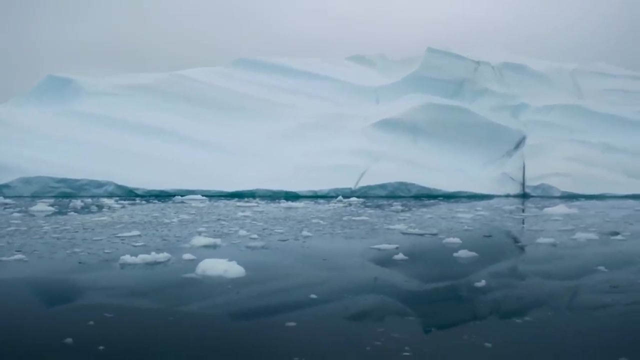 pole, but a large area of sea ice grows and shrinks with the seasons. seasonal sea ice also fringes greenland and antarctica. ice shelves are a third manifestation of polar ice. these are thick layers of ice that extend into the ocean from the mouths of glaciers. periodically, icebergs will break away from these. 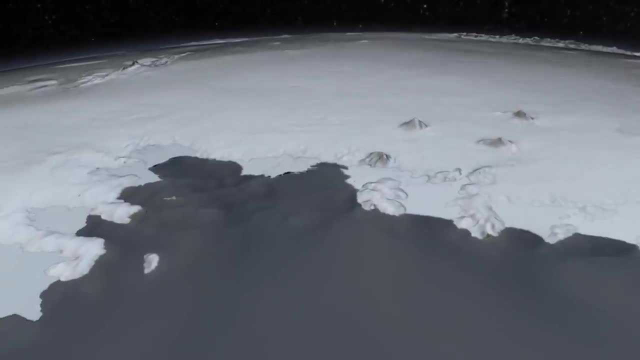 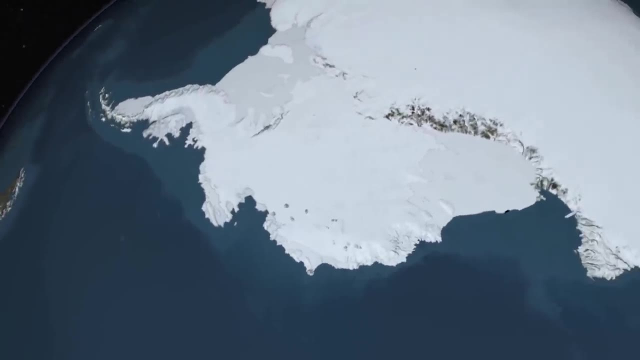 regions. these areas are important to the circulation of global winds and ocean currents and, since 2002, nasa has tracked the prevalence of water in general and ice in particular via the grace satellites, which are the most important sources of water in the world. since 2002, nasa has tracked the prevalence of water in general and ice in particular via the grace satellites, which 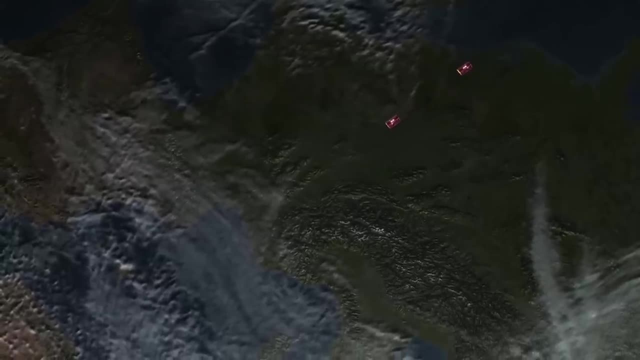 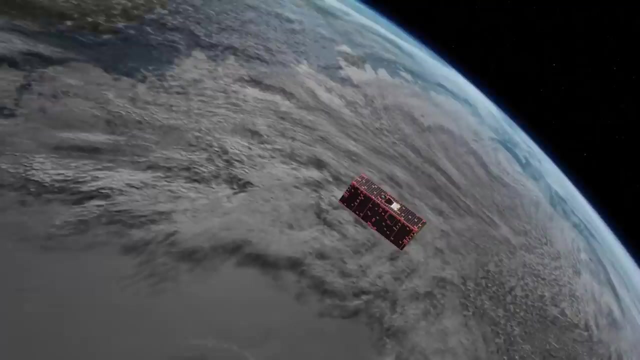 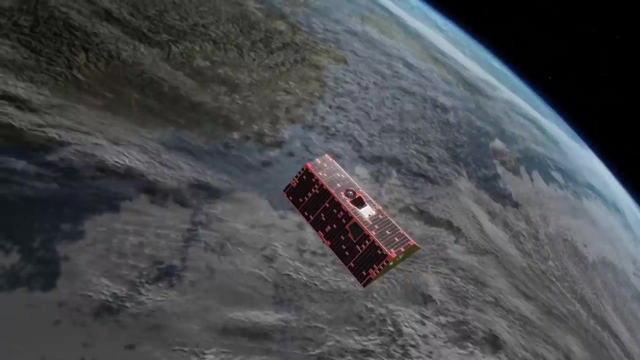 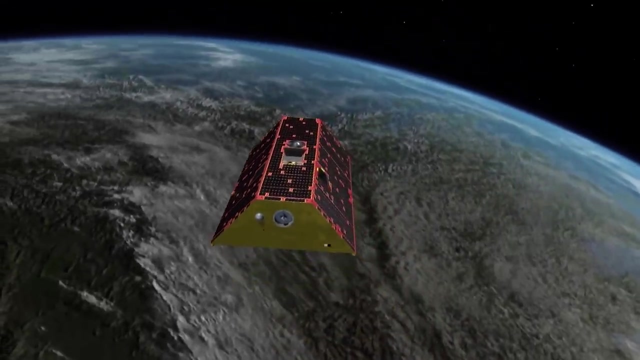 were recently replaced by a similar pair of grace follow-on satellites. the two follow the same orbit, and minute changes in the earth's gravitational field will cause them to change speed, with a variation in the distance between them. this data is accurately measured, allowing researchers to record changes due to variations in groundwater or in ice thickness. 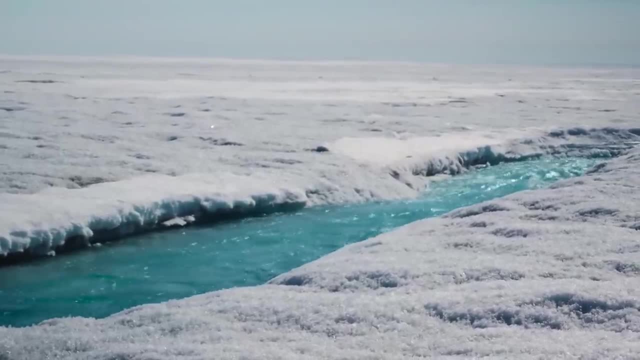 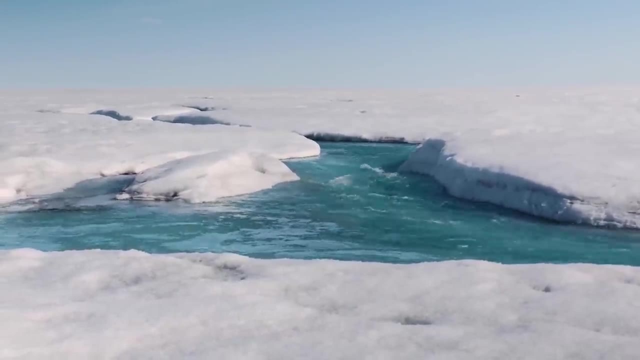 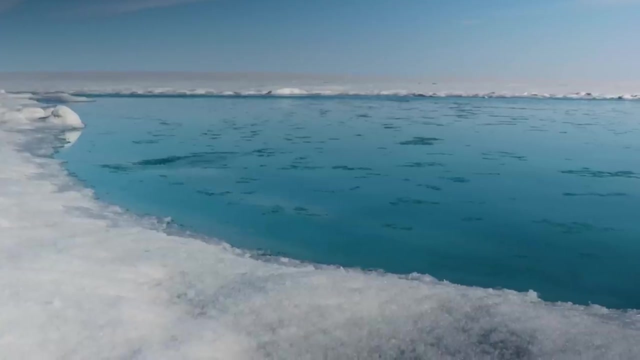 during the life of the first grace mission, greenland lost 285 gigatons of ice per year on average. antarctica lost 137 gigatons per year. from 2005 to 2016. sea levels rose by 3.7 centimeters due to melting ice sheets. 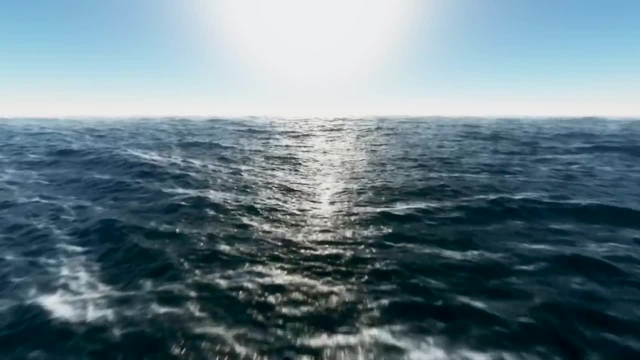 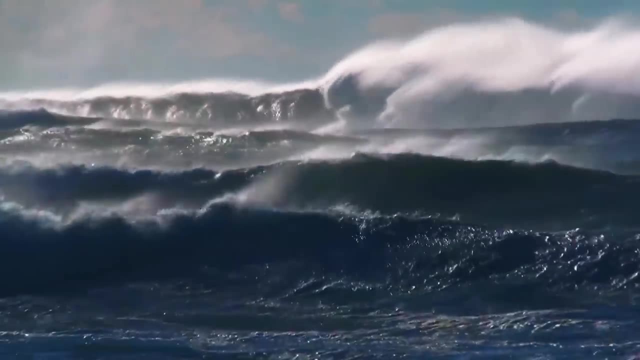 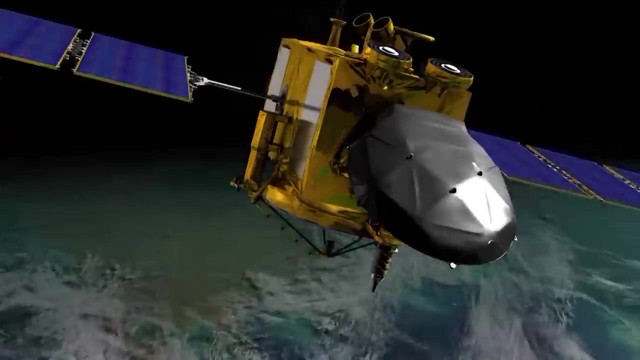 and to expansion of sea water. sea levels have been monitored from space since 1992, initially with the topex poseidon satellite and more recently with the jason series of satellites. jason 3 uses a precision radar altimeter to measure regional and global variation in sea levels. in the 20 years to 2014, the average rise was six centimeters, but the increase is not uniform. the red areas show the greatest rise, with white representing no change and blue signifying a decrease. the unevenness of the sea surface is due to a complex interaction between: 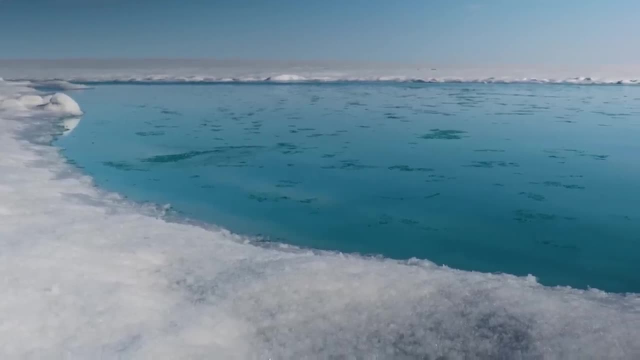 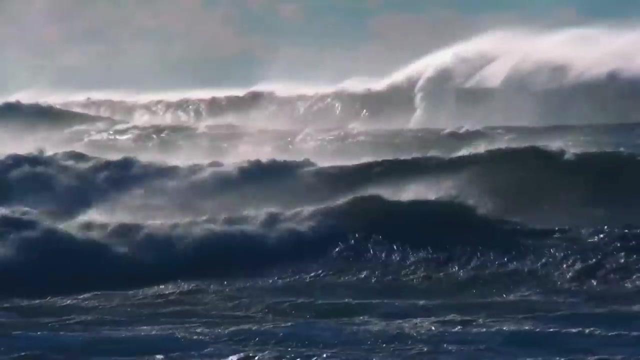 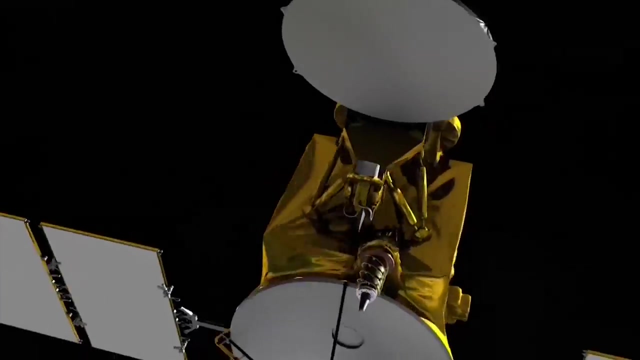 and to expansion of seawater. Sea levels have been monitored from space since 1992, initially with the Topex-Poseidon satellite and more recently with the Jason series of satellites. Jason 3 uses a precision radar altimeter to measure regional 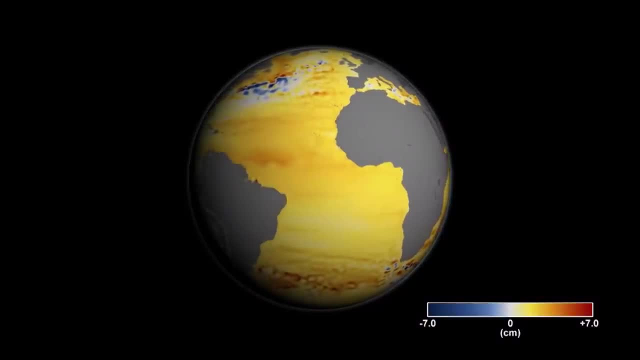 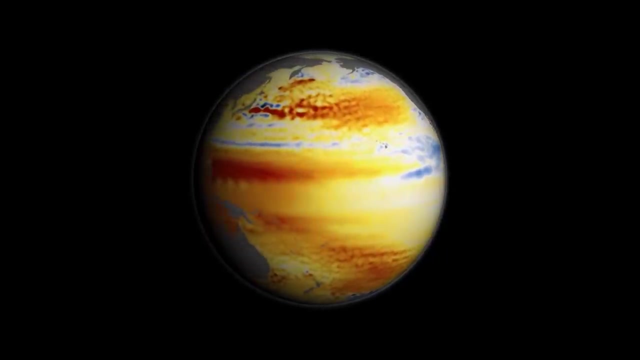 and global variation in sea levels In the 20 years to 2014,. the average rise was 6 centimeters, but the increase is not uniform. The red areas show the greatest rise, with white representing no change and blue signifying 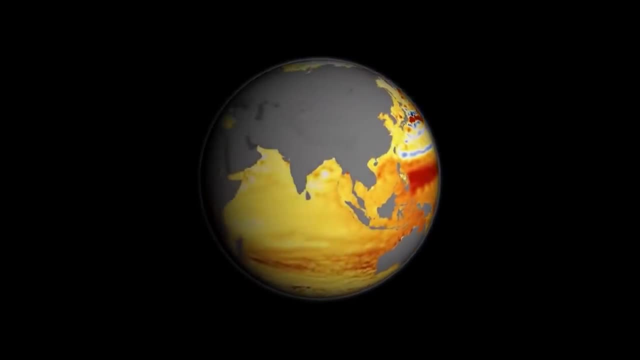 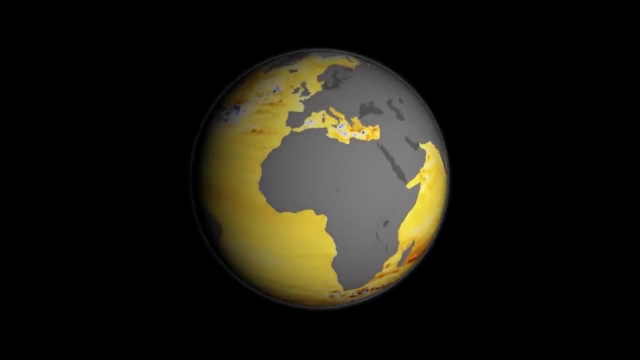 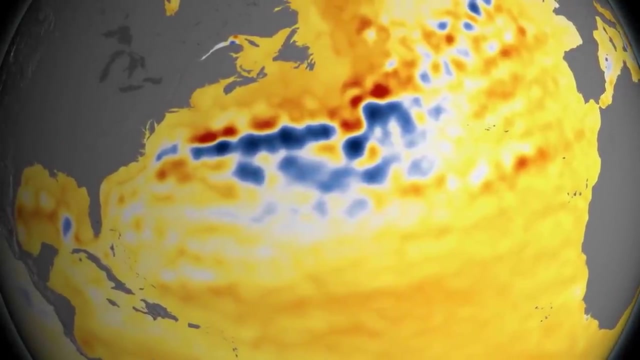 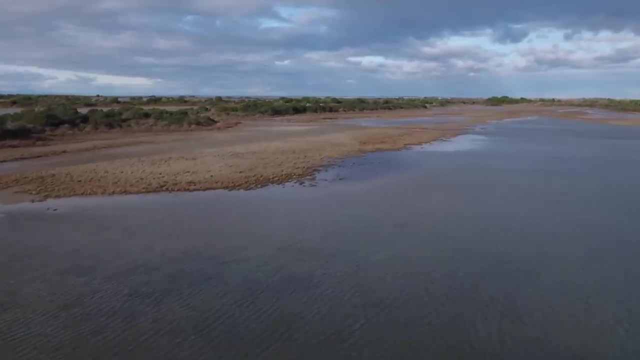 a decrease. The unevenness of the sea surface is due to a complex interaction between ocean currents, the Earth's spin and the topography of the ocean floor. These blue areas in the Atlantic show a shift in the Gulf Stream. The Comargue region. 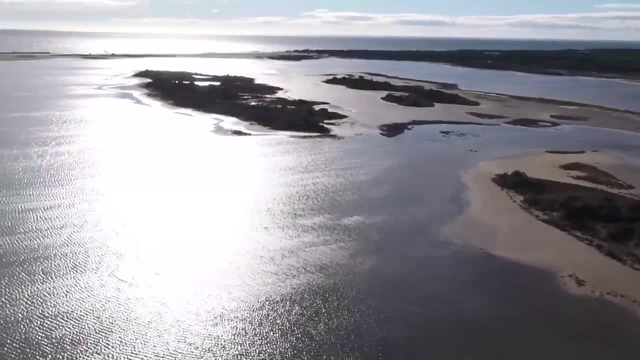 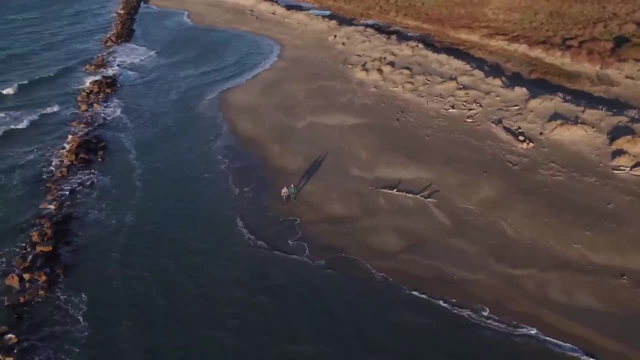 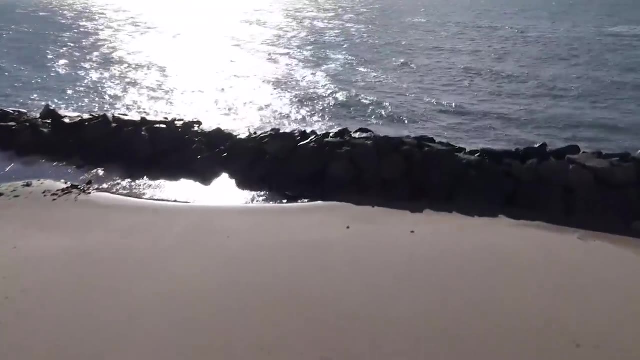 of southern France is a low-lying area at the delta of the Rhône River. In the 1980s, a sea wall was built to prevent the encroaching Mediterranean. Over the last 30 years, it has been the largest. 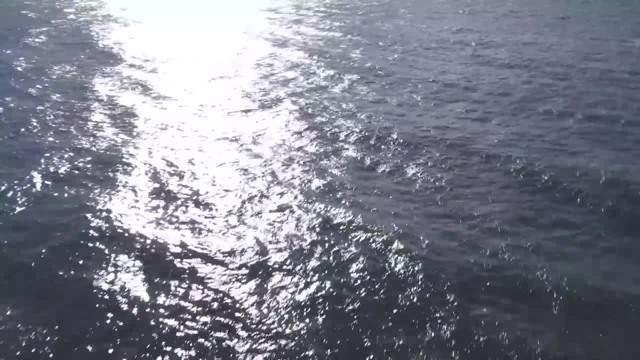 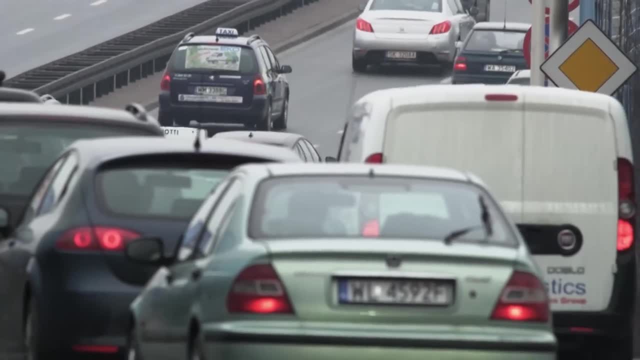 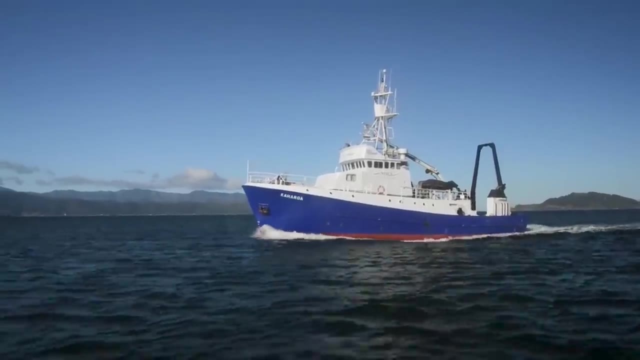 sea wall in the world. Scientists are convinced that a warming global climate is responsible and that our reliance on the burning of fossil fuels has led to an excess of carbon dioxide in the atmosphere, which traps heat. 93% of this heat has been taken up. 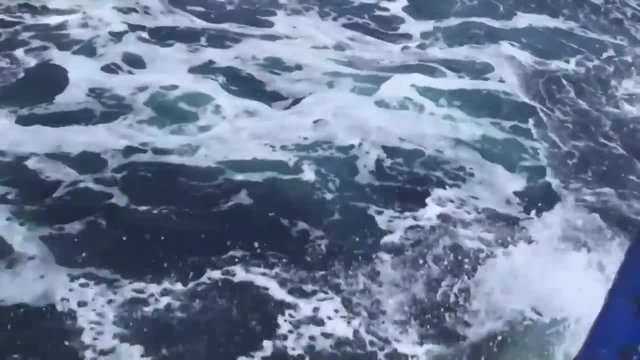 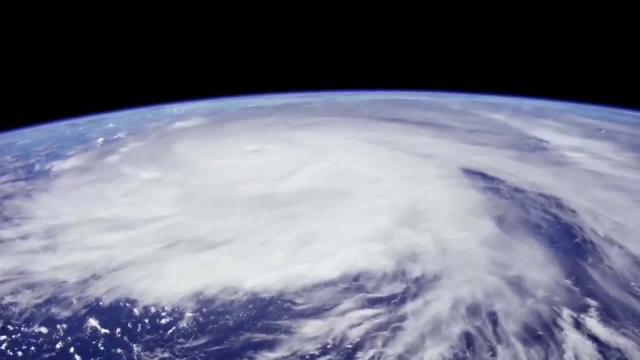 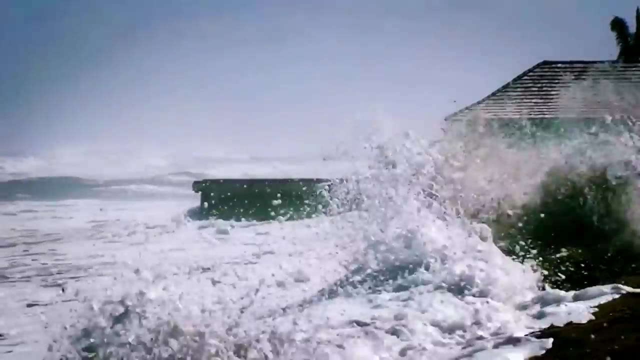 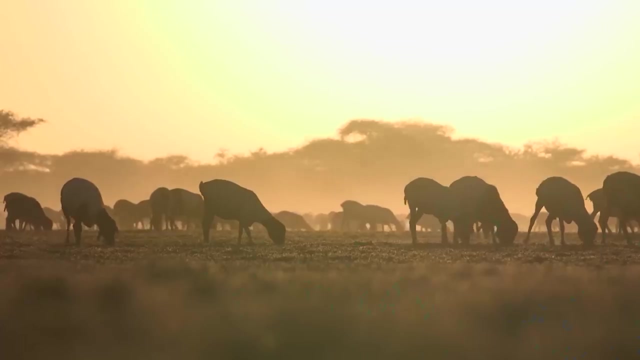 by the oceans. Data from the Argo network has shown that the Arctic Ocean is the largest ocean in the world. While this may not sound like much, meteorologists understand how sea surface temperatures drive hurricanes and cyclones and early predictions of storms of greater magnitude. 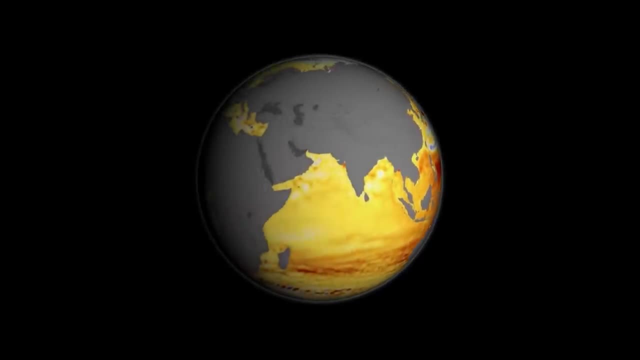 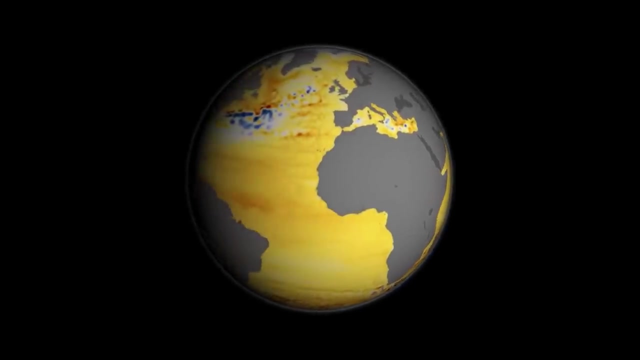 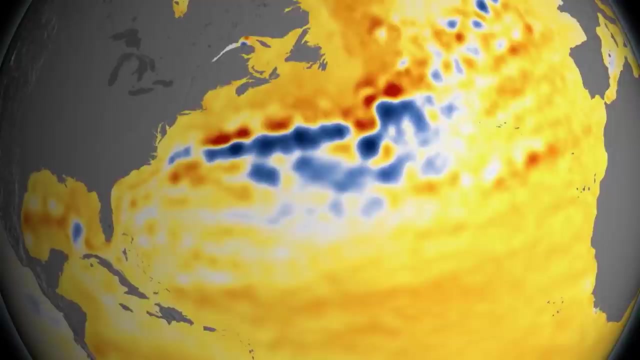 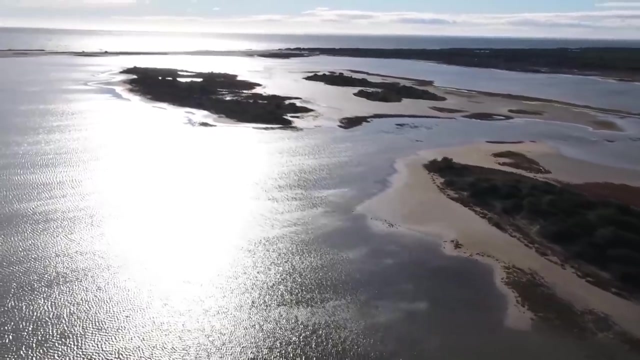 ocean currents, the earth's spin and the topography of the ocean floor. all these factors must be accounted for to arrive at a baseline against which to measure changes. these blue areas in the atlantic show a shift in the gulf stream. the camargue region of southern france is a low-lying area at the delta of the rhone river. 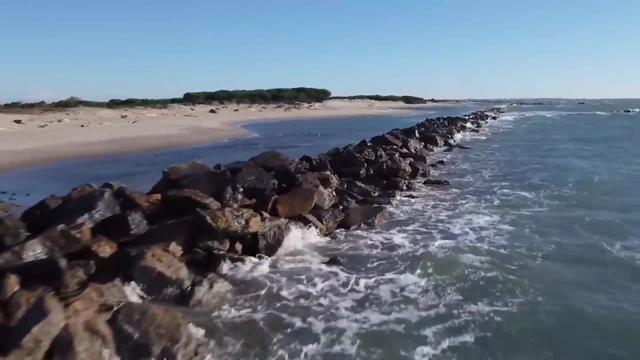 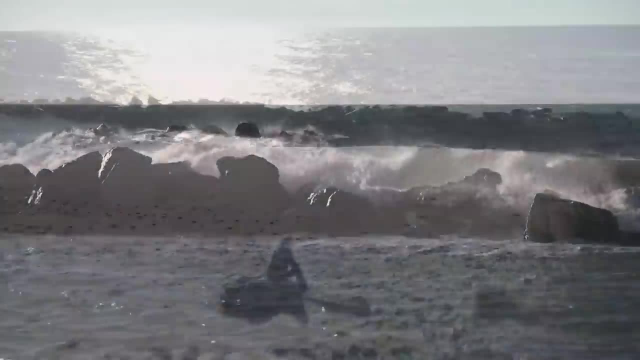 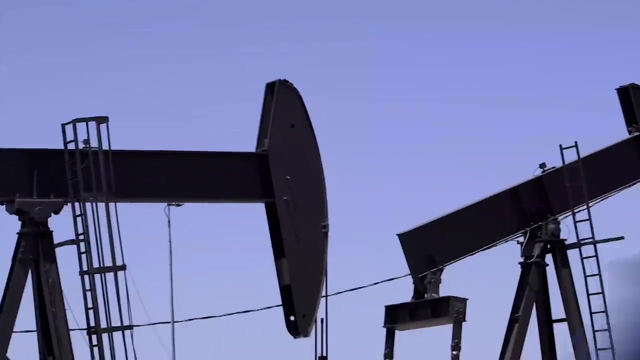 in the 1980s, a sea wall was built to prevent the encroaching mediterranean. over the last 30 years, the coastline here has been pushed back by several hundred meters. scientists are convinced that a warming global climate is responsible and that our reliance on the burning of fossil fuels has led to an excess of carbon dioxide in. 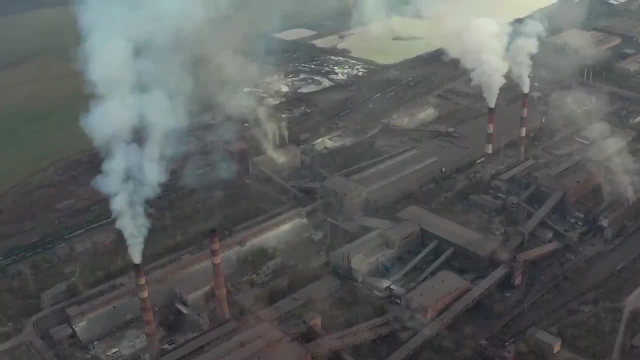 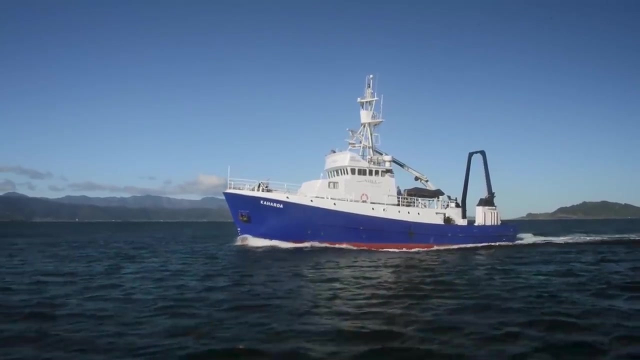 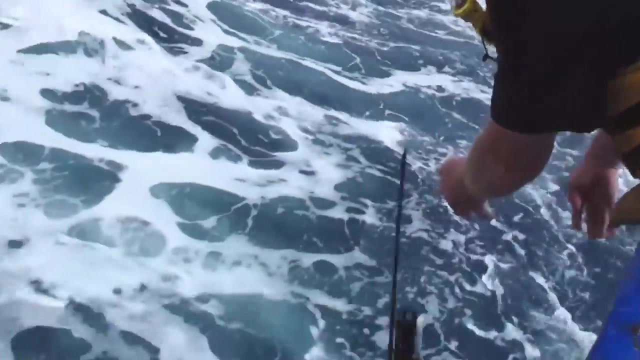 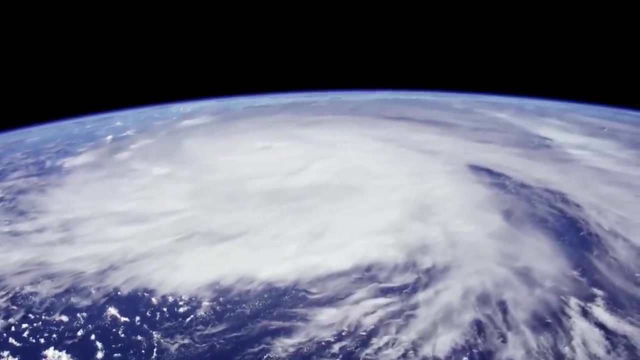 the atmosphere which traps heat. 93 percent of this heat has been taken up by the oceans. data from the argo network of ocean buoys shows an average warming of 0.9 of a degree celsius since the 1950s. while this may not sound like much, meteorologists understand how sea surface temperatures drive. 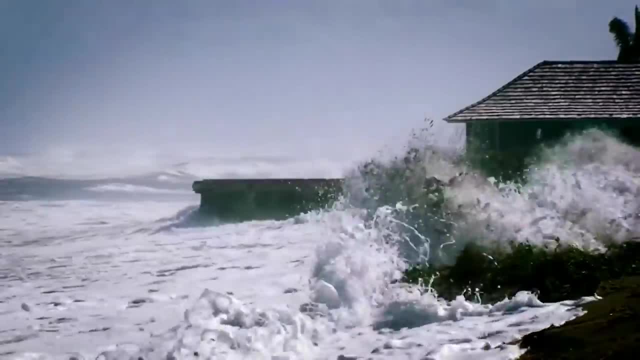 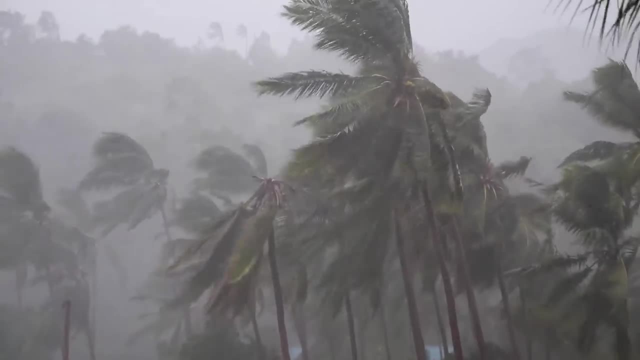 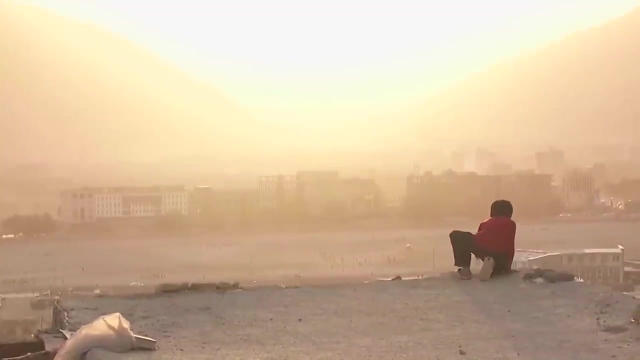 hurricanes and cyclones, but the predictions of storms of greater magnitude are being realized. long-standing weather records are being broken and broken again. in 2017, nasa, noaa and the uk met office. all agreed that 2016 had been the hottest year on record. 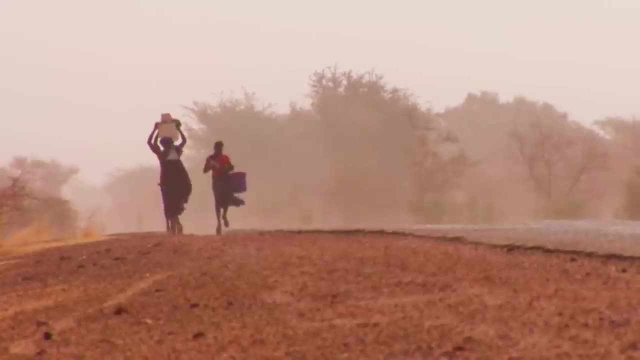 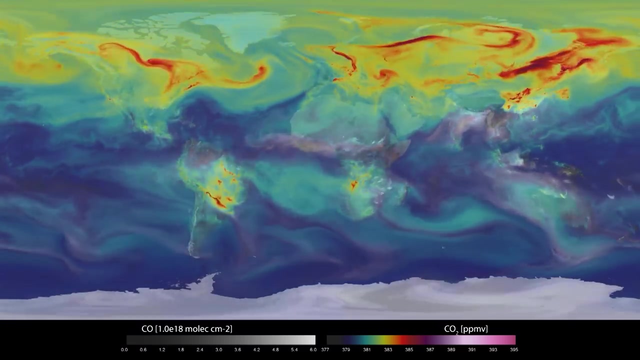 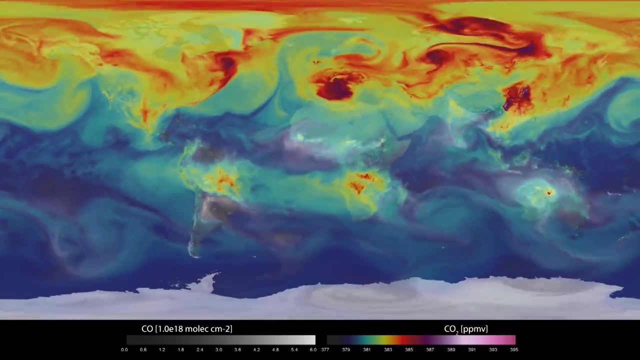 globally, 16 of the 17 hottest years have all occurred since the year 2000. both nasa and issa have been monitoring the distribution and concentrations of co2 in the atmosphere since 1992.. this visualization from data collected in 2006. 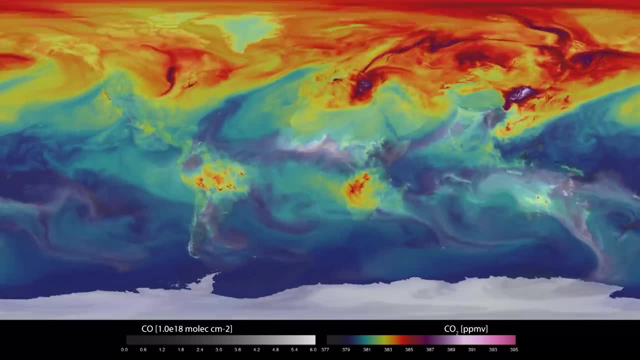 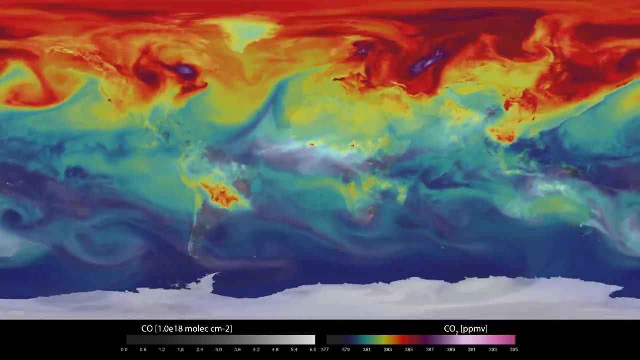 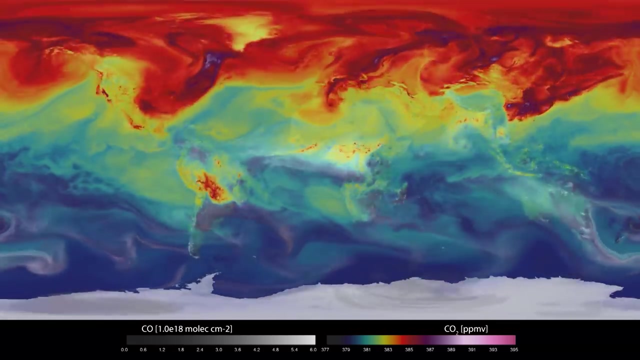 shows the yearly fluctuations of carbon dioxide and carbon monoxide. while most co2 emanates from the populous northern hemisphere, seasonal fires in africa, australia and south america generate much of the carbon monoxide. prolonged droughts and more severe forest fires are another aspect of the carbon dioxide crisis. 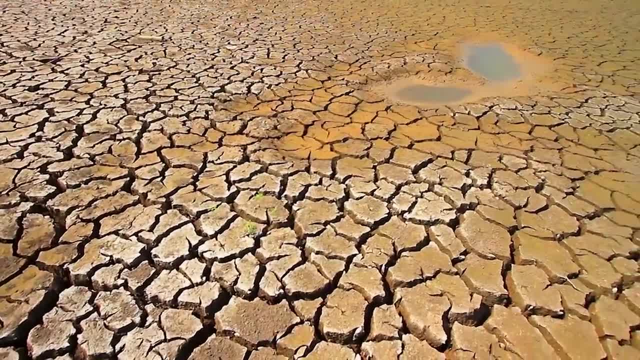 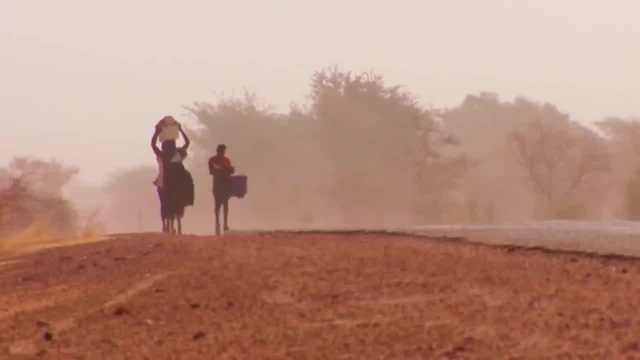 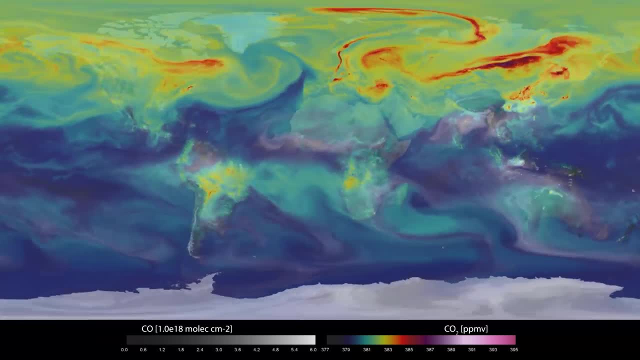 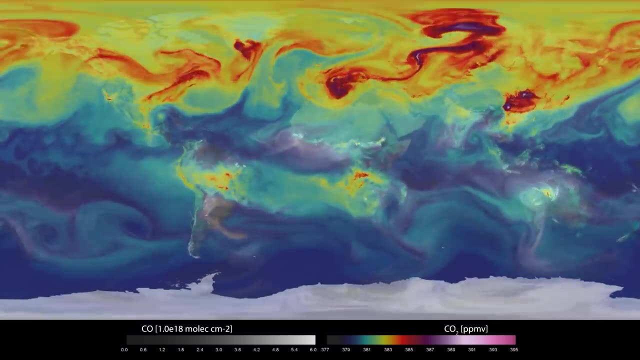 are being realized. Longstanding weather records are being broken and broken again. Globally, 16 of the 17 hottest years have all occurred since the year 2000.. Both NASA and ESA have been monitoring the distribution and concentrations of CO2 in the atmosphere. 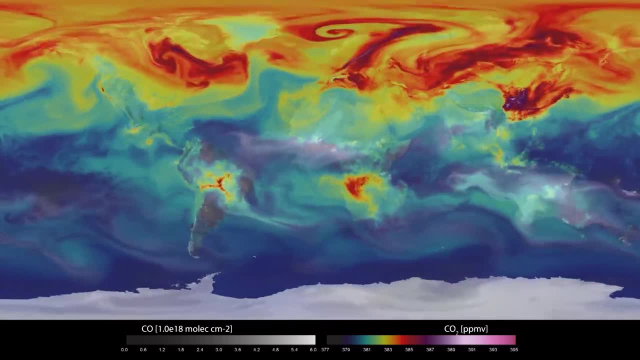 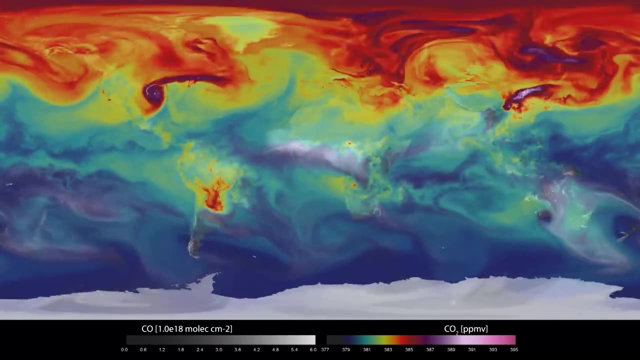 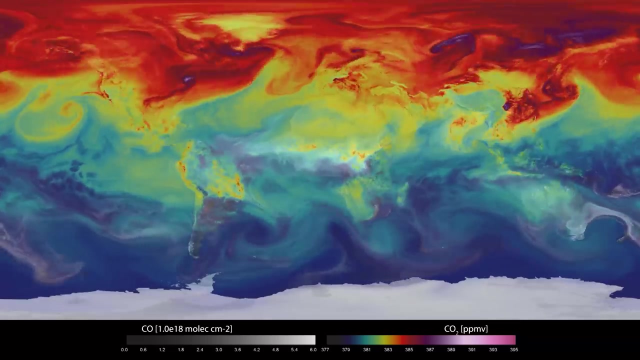 since 1992.. This visualization from data collected in 2006 shows the yearly fluctuations from the populous northern hemisphere. Seasonal fires in Africa, Australia and South America generate much of the carbon monoxide, Prolonged droughts and more severe forest fires. 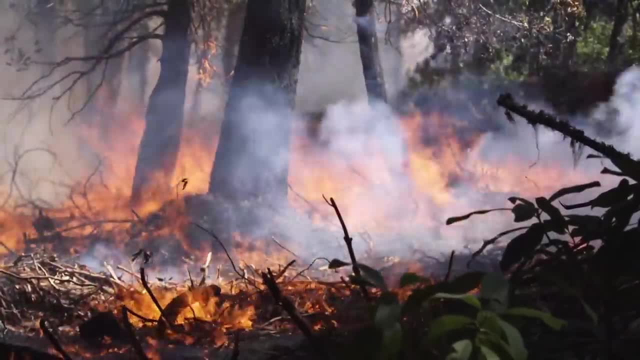 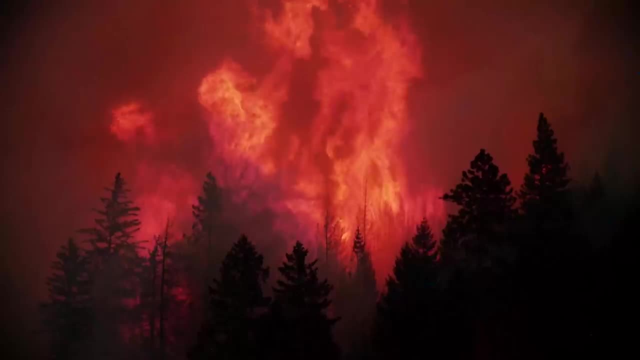 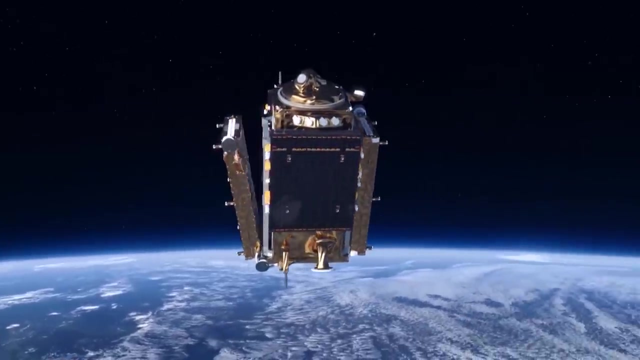 are another aspect accompanying increased levels of atmospheric CO2 that are currently unfolding. Such events inject a huge pulse of greenhouse gases into the atmosphere, magnifying the problem. The European Space Agency's Copernicus Program with its Sentinel Earth Observation Satellites. 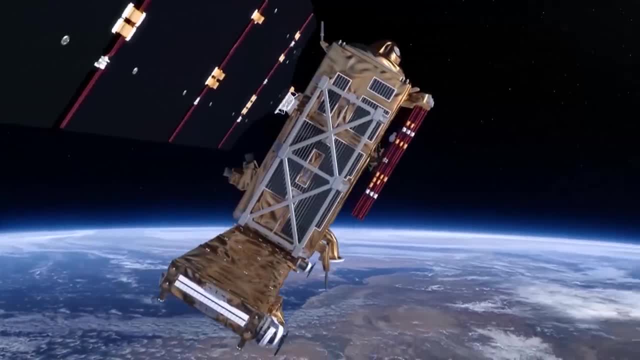 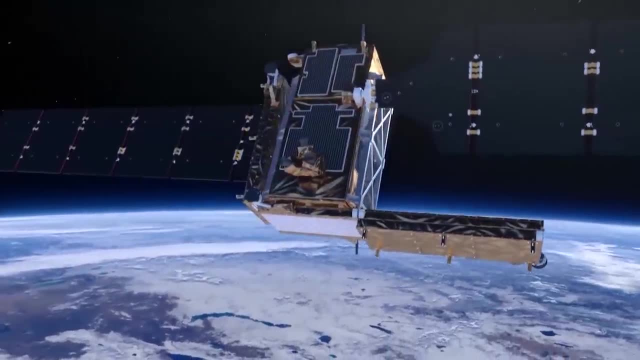 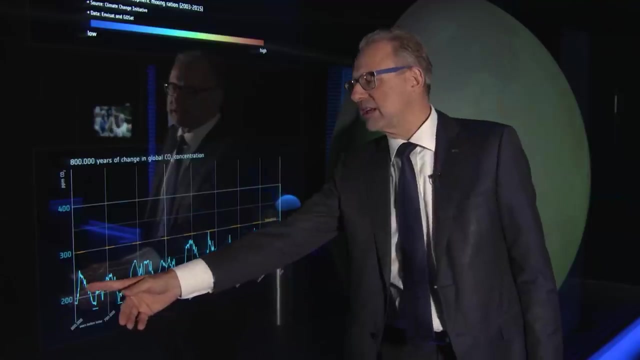 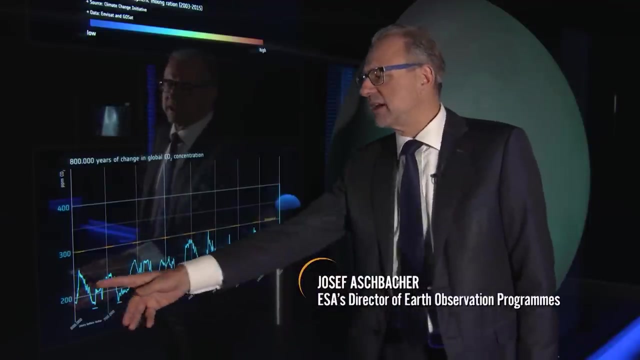 has committed to making information about the changing climate freely available to policymakers, businesses and research institutions. Josef Aschbacher is ESA's Director of Earth Observation Programs. What you see here on this graph is the CO2 concentrations of the atmosphere over the last 800,000 years. 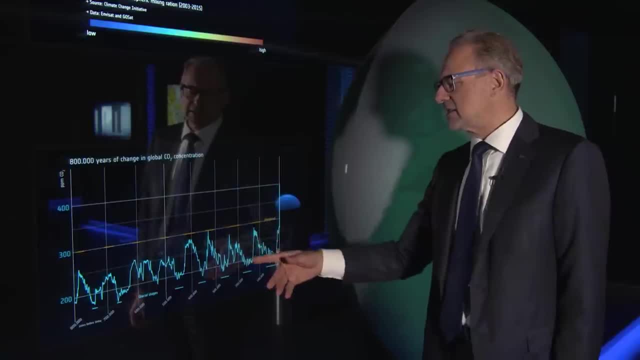 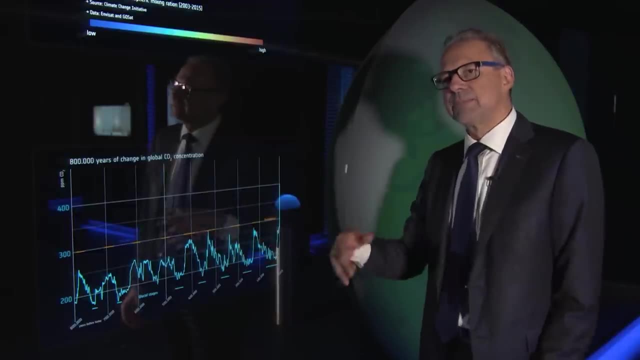 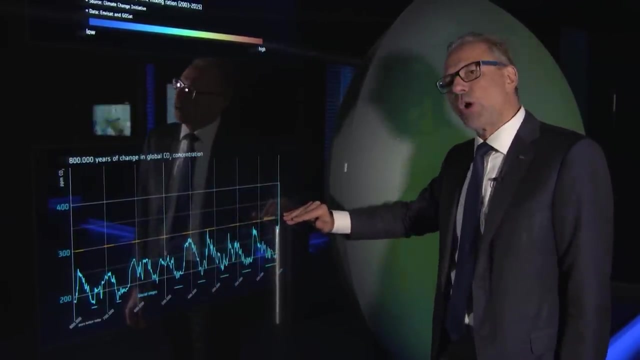 And you see that these values are going up and down in different phases. You see, on the blue lines here are indicating ice ages and the orange lines here are indicating periods between ice ages or periods where it's much warmer. But you also see that over the last 800,000 years, 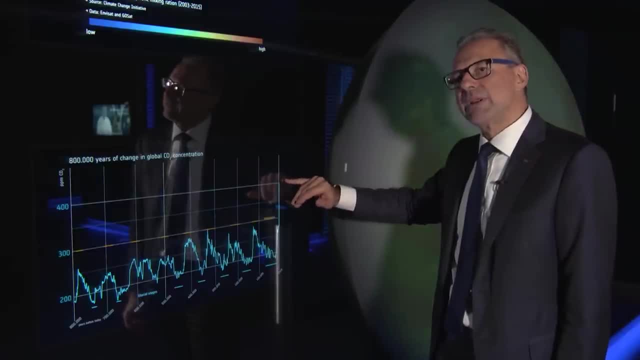 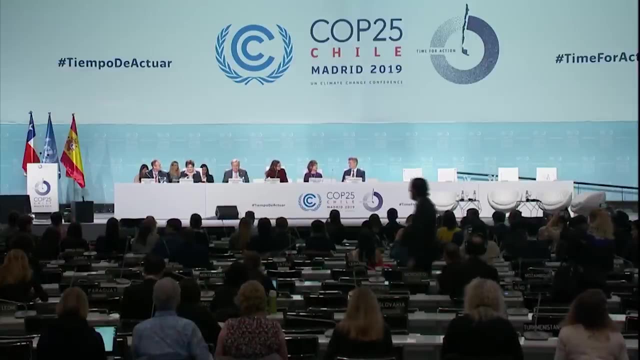 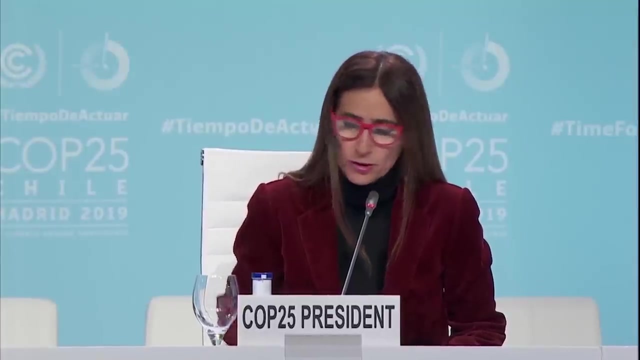 the value was always below 300 parts per million and suddenly, since the last century, the value has gone down to over 300,000.. The recent climate summit, COP25, held in Madrid, made little progress toward an international agreement to cut greenhouse gas emissions. 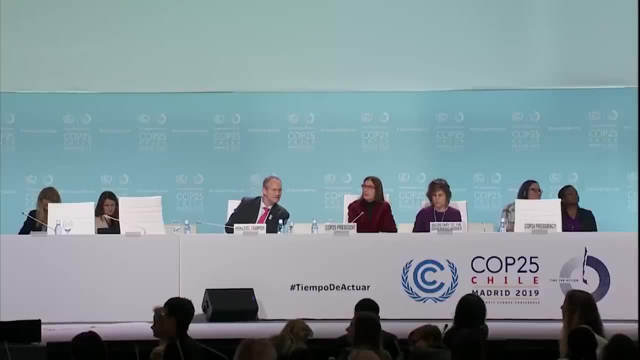 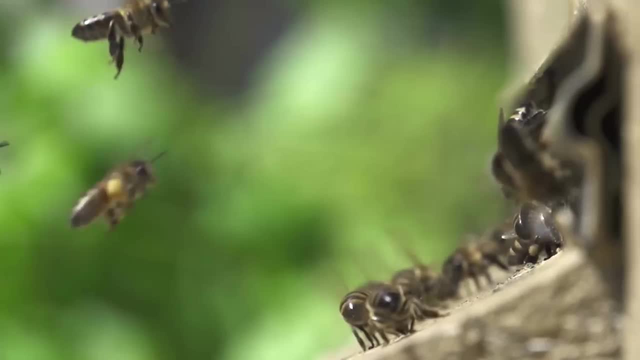 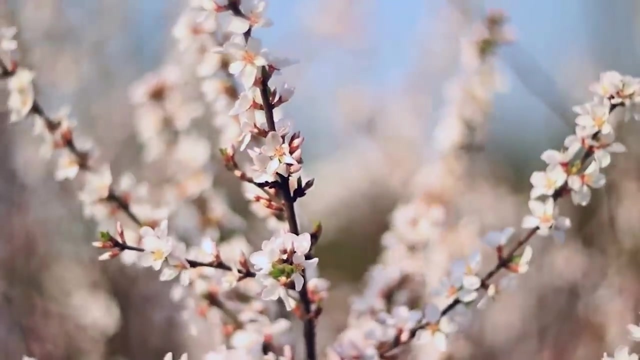 While some businesses and economies will have to adjust, that task only gets more difficult as time passes and far greater adjustments will be forced upon everyone. The Earth is the only place that has enabled this web of life is fragile Plants and animals interact for mutual benefit. 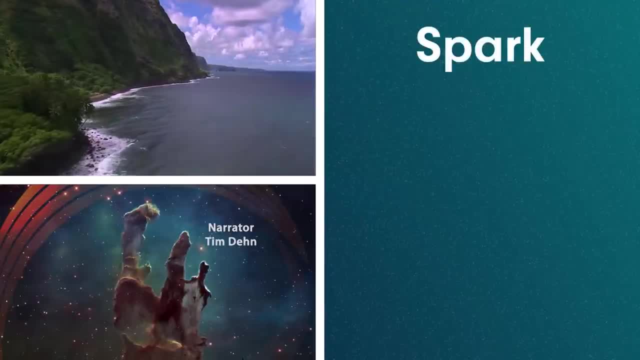 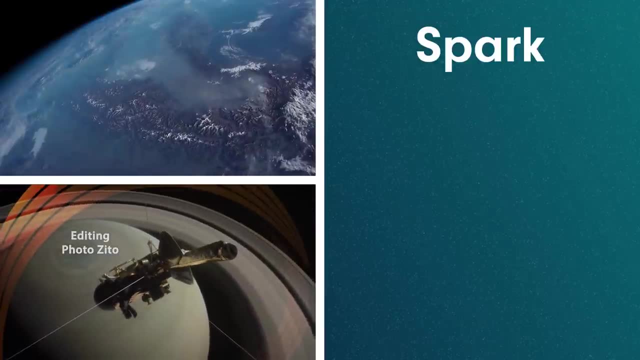 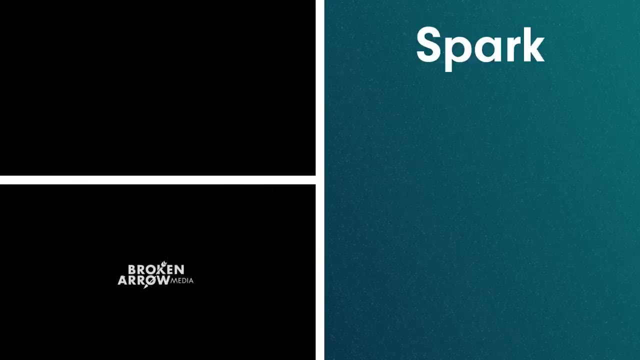 Our benign environment results from the complex and varied creatures with which we share the planet. It's important that we look after our home. For more UN videos, visit wwwunorg. 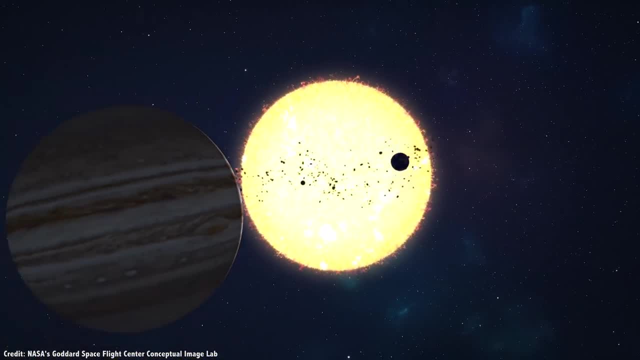 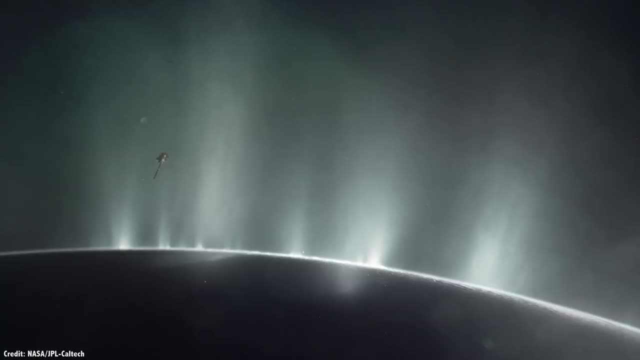 The race is on to find life in other places in the solar system, from underground reservoirs on Mars to the subsurface oceans on Europa and Enceladus. If spacecraft, rovers or even astronauts make the momentous discovery of life on another world, that'll just open. 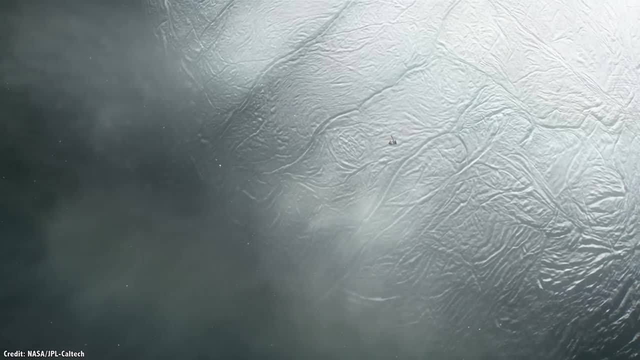 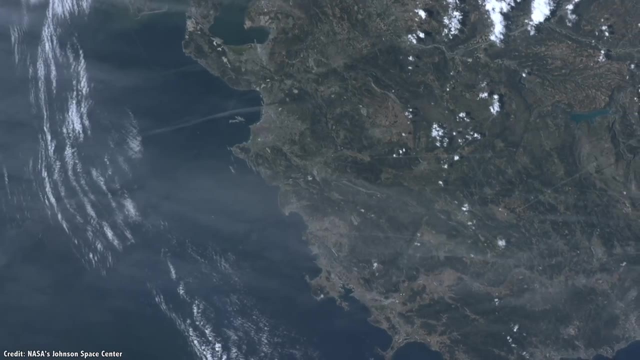 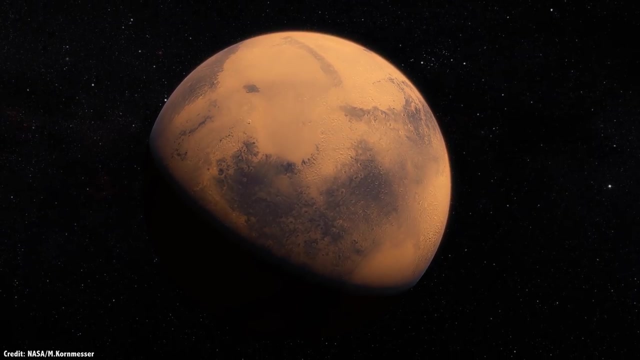 up new questions. Did it originate all on its own, completely independently from Earth, Or are we somehow related? And if we are related, how long ago did our evolutionary trees branch away from each other, Even though Mars is millions of kilometers away? it could be possible. 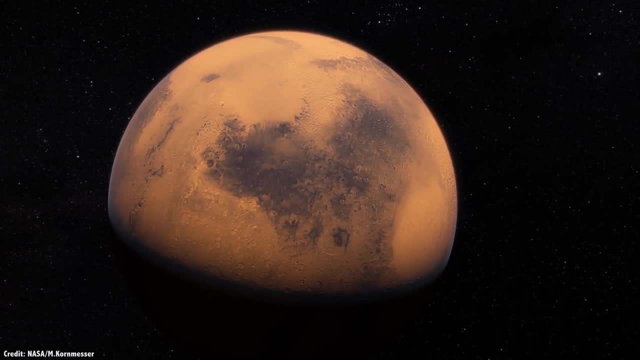 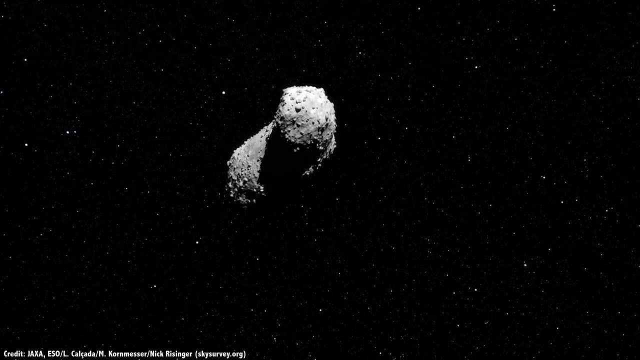 that we're still related thanks to the concept of panspermia, the idea that meteor impacts could transfer rocks and maybe even living creatures from world to world. But could you go one step further: If we find life on another star system, could we discover? 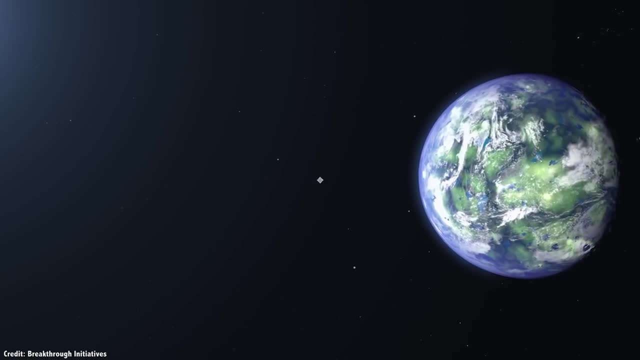 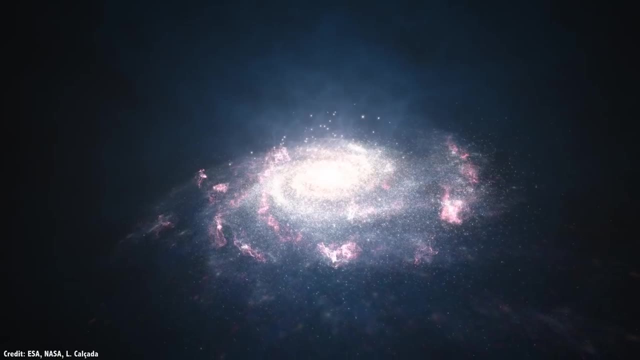 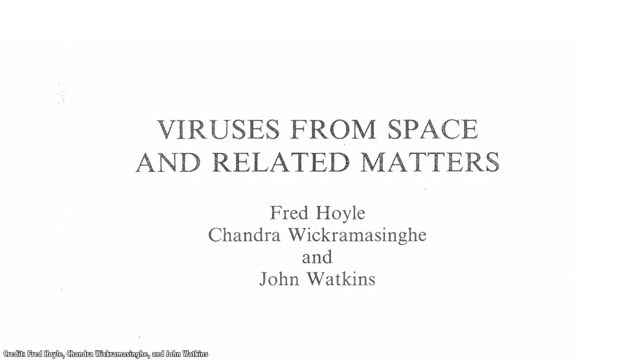 that we're actually related to them too. Is galactic panspermia possible? Before I get talking about panspermia on a galactic level, I'd first like to just bring everyone up to speed on regular old panspermia. The concept was popularized by Fred Hoyle. 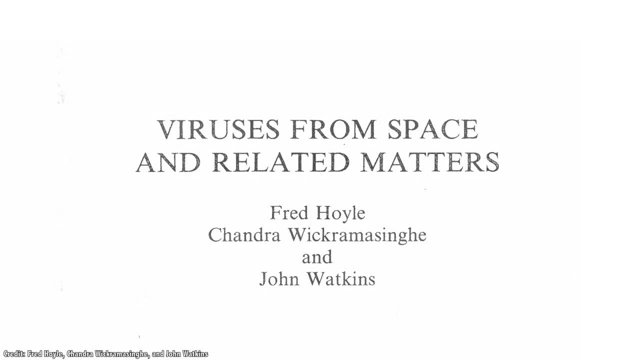 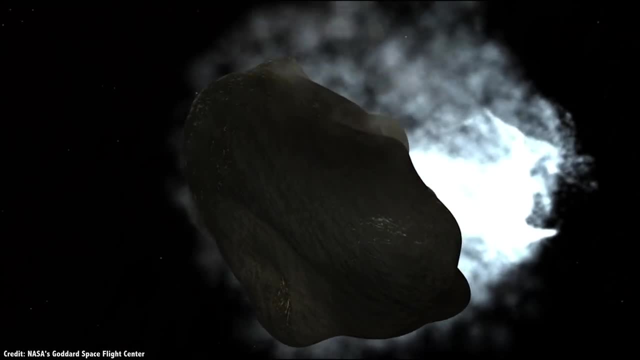 Chandra Wickramasinghe and John Watkins in the 1986 book called Viruses from Space and Related Matters. They discovered that dust in space contained organic compounds and proposed that dust could be a source of organic matter. The concept was popularized by Fred Hoyle. 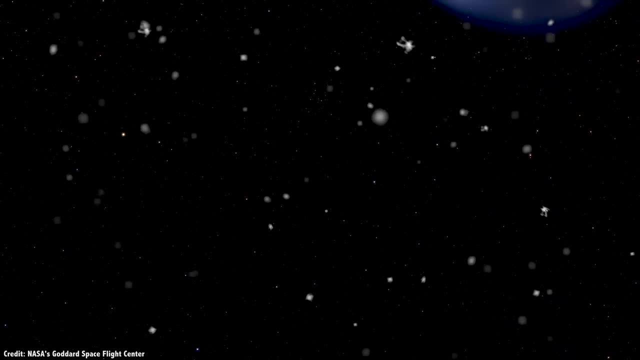 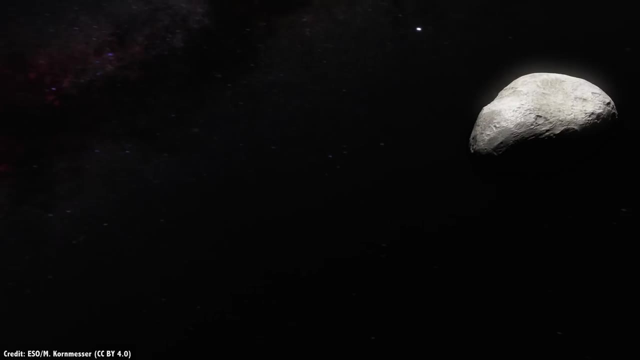 Chandra Wickramasinghe and John Watkins in the 1986 book called Viruses from Space and that new diseases could be falling to Earth from space. This would explain why disease outbreaks seem to happen randomly around the world. But planetary scientists have known for a while that larger objects do travel from world.